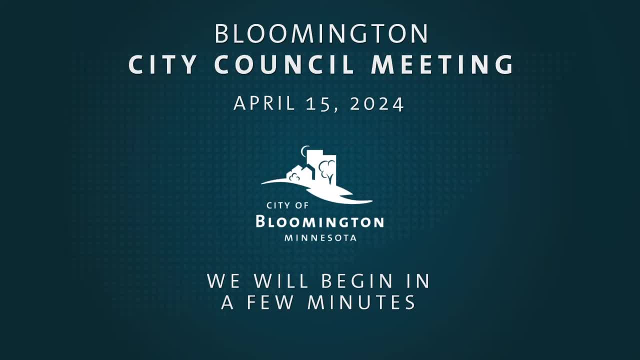 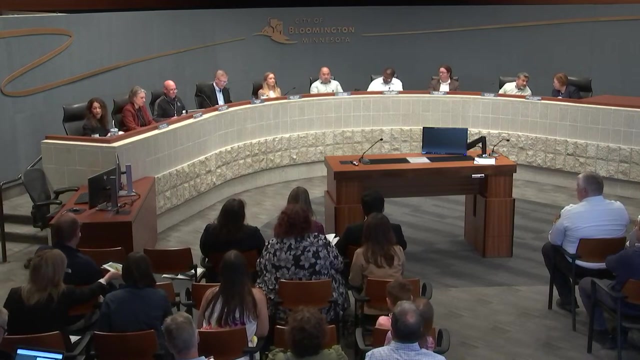 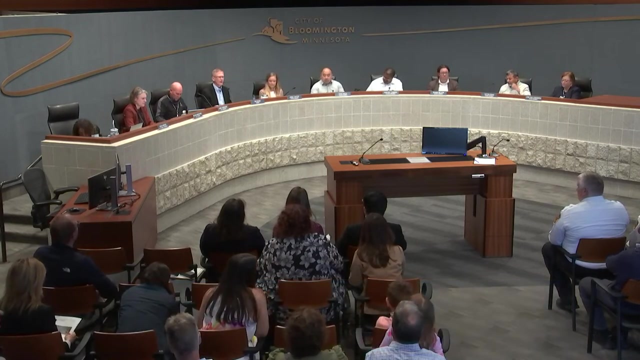 Thank you, Thank you, Thank you And welcome. I will call this Bloomington City Council meeting to order. Tonight is Monday, April 15th 2024.. Thank you all for being here in the chambers. Great to see everybody. We will start our meeting as we always do. If you're able, please stand and join us in the Pledge of Allegiance. 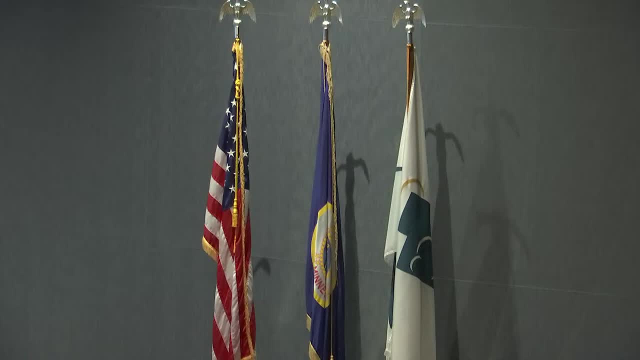 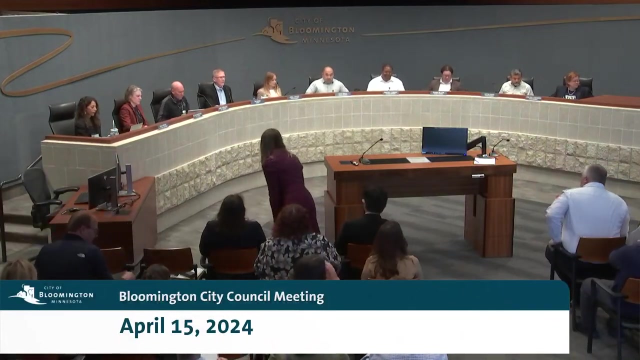 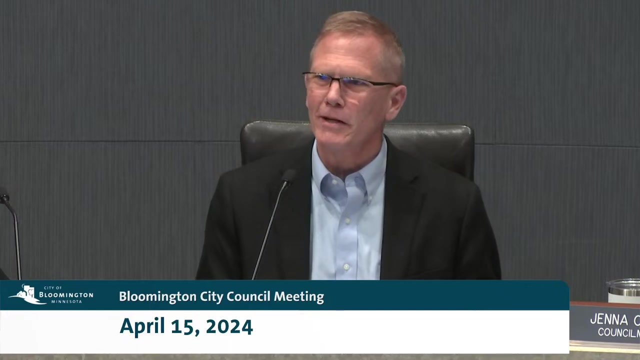 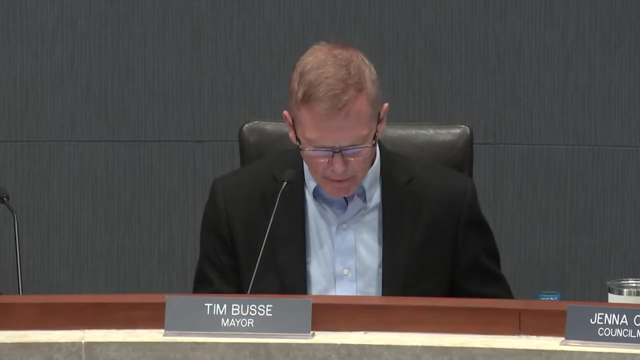 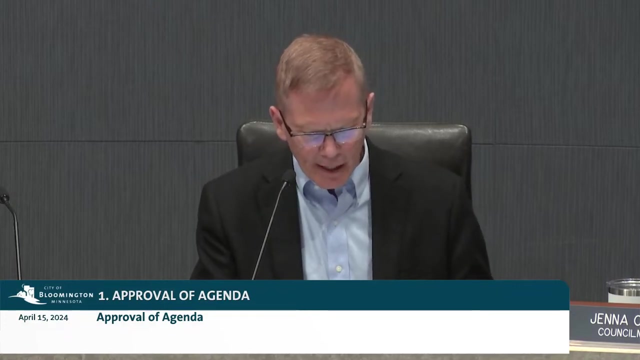 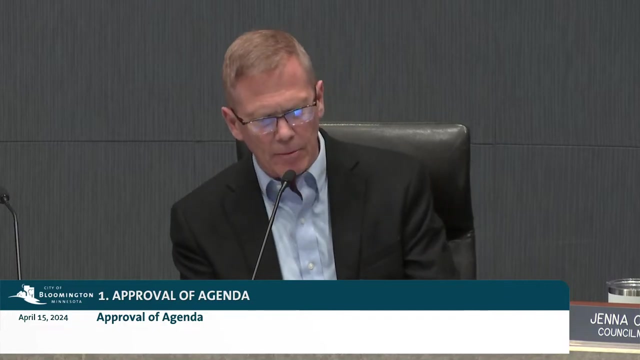 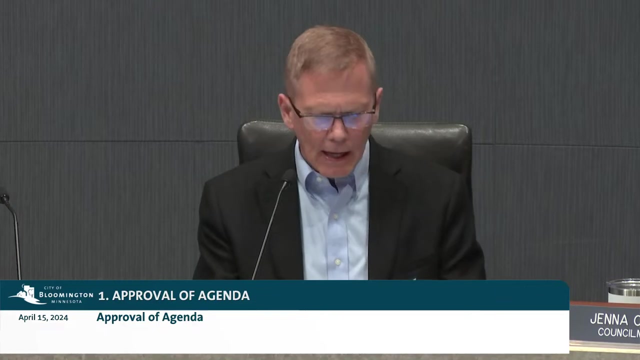 I pledge allegiance to the flag of the United States of America and to the republic for which it stands: one nation under God, indivisible, with liberty and justice for all. Thank you, I pledge allegiance to the flag of the United States of America and to the republic for which it stands: one nation under God, indivisible, with liberty and justice for all. 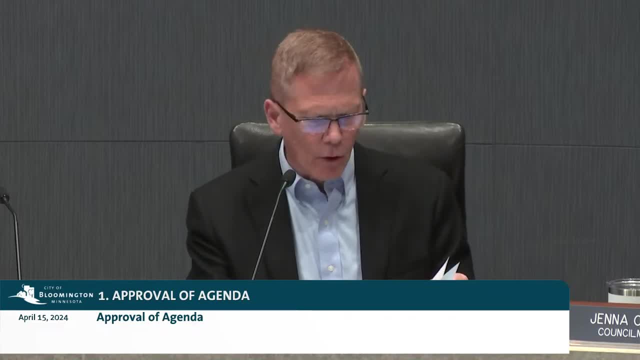 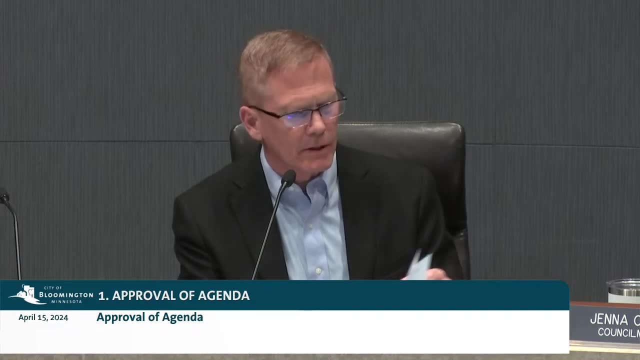 At that point in the agenda council we've got two items under our organizational business, item 5.1 and 5.2.. Those are timed items and at that point I'm going to move those two items immediately after our meeting. 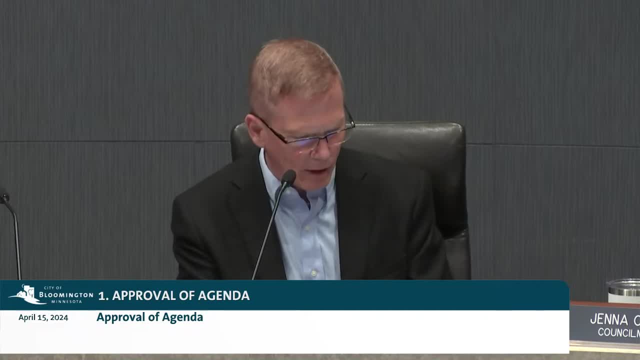 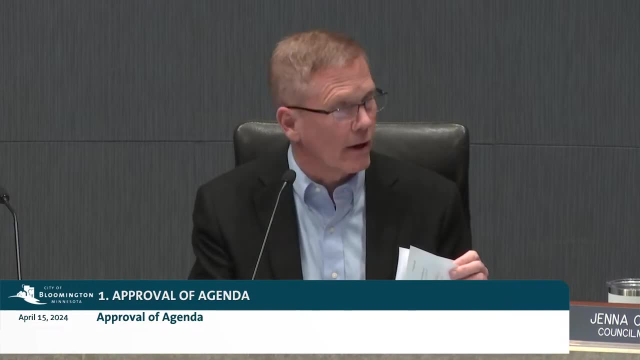 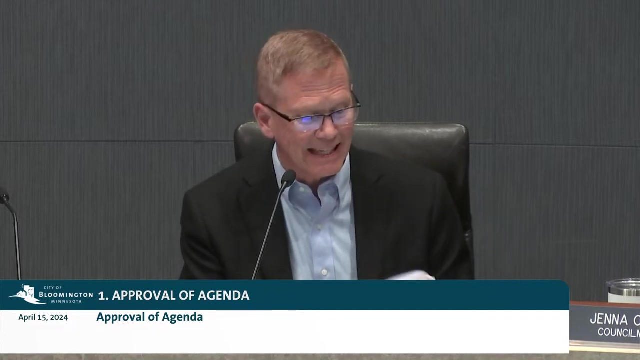 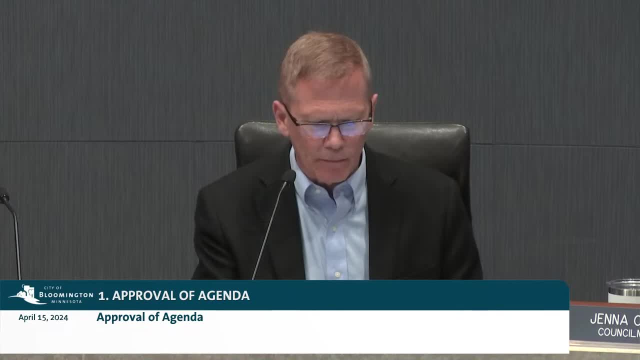 And then finally, under item 4,- item 4.5 will be 700 American Boulevard land sale and tax increment financing district discussion. We will finish our meeting doubling back to item 5, our organizational business. We will finish, as we always do, with item 5.3, our city council policy and issue update. 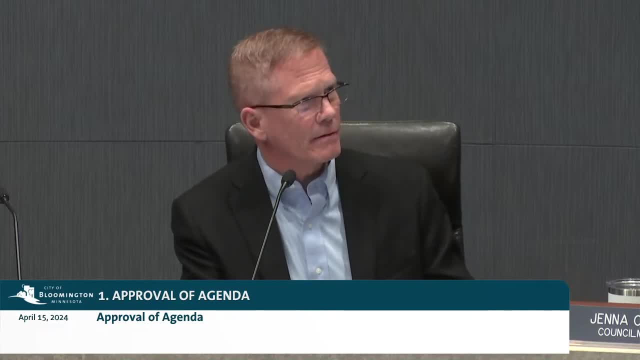 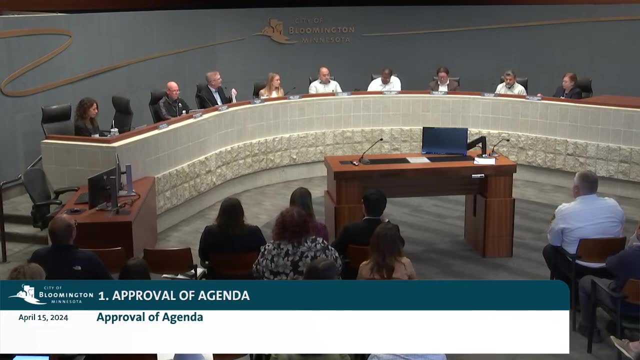 Everybody clear on what we're planning to do here this evening. Anything else to add or change or make adjustments to? If not, I will move. approval of tonight's agenda as stated. Second: We have a motion and a second by Councilmember Lohman to accept tonight's agenda as stated. 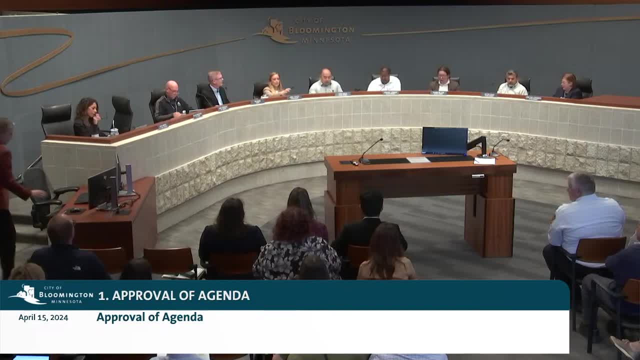 No further discussion on this. All those in favor please signify by saying aye, Aye. Opposed Motion carries 7-0, and we have an agenda. With that out of the way, we will get into our agenda. 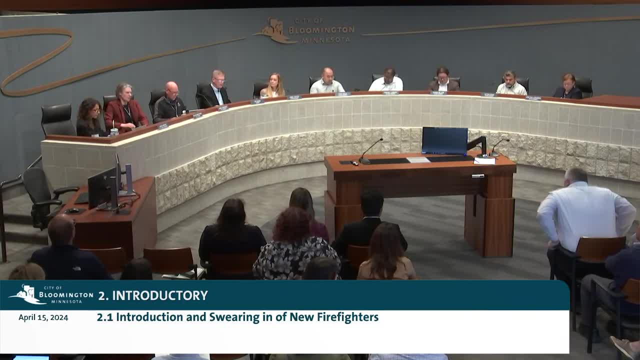 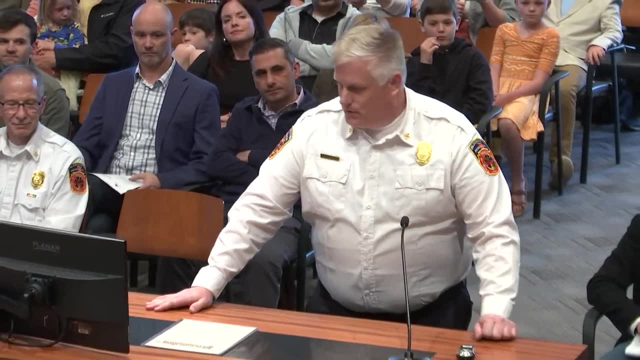 And our first order of business is item 2.1, the introduction and swearing in of our new 5.3. Firefighters. Assistant Chief. good evening and welcome. Good evening, Mayor and Council. We're here tonight to introduce our seven new full-time firefighters. 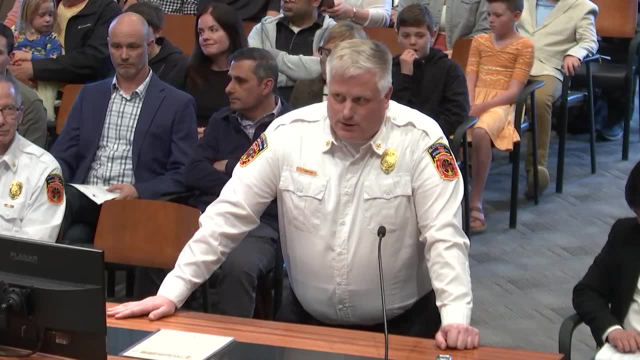 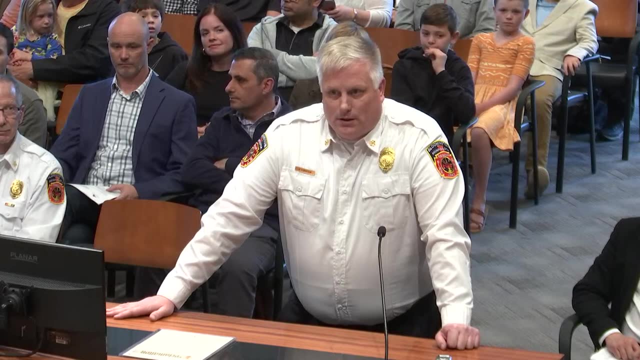 They started April 1st and they're going through their six-week training academy and they'll be out working shifts the middle of May. They'll come up here individually and introduce themselves. We just want to thank you for your continued support as we transition our staffing model. 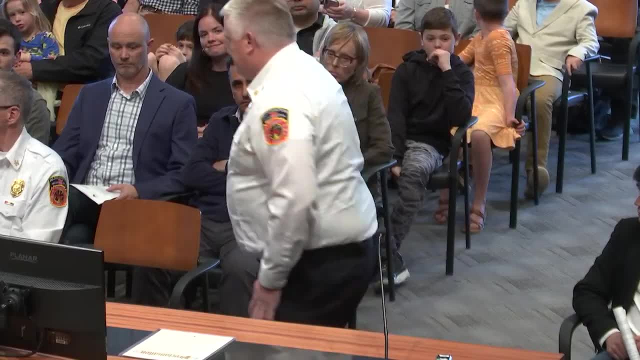 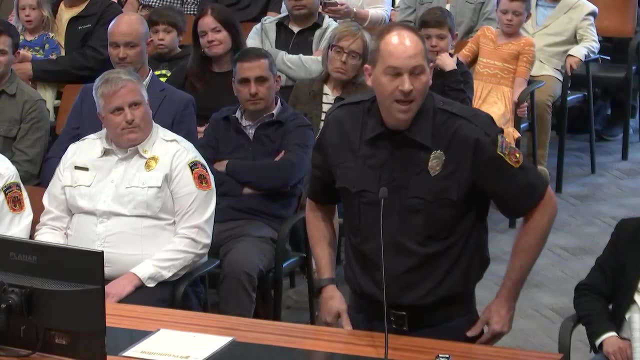 here in the city to meet the needs of the community. Thank you, Thank you, Thank you so very much And we're going to meet our new firefighters one by one. Good evening and welcome, Thank you. My name is Brad Boisher. 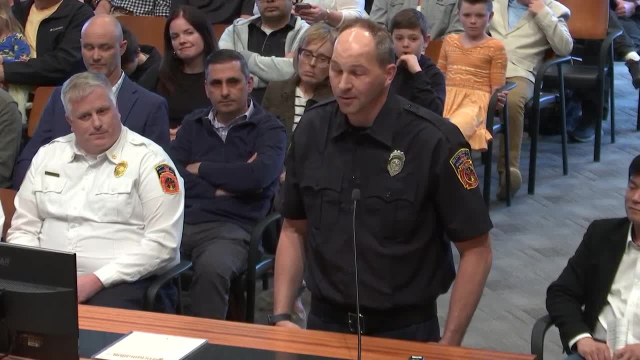 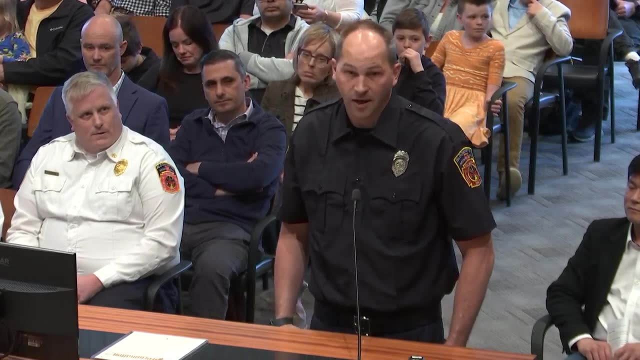 I've been a firefighter since 2006 and a paramedic since 2012.. I come from White Bear Lake Fire, where I was there as a firefighter medic for six years. I currently live up in Blaine with my family: my wife Kristen, my son Jacob and Grace. 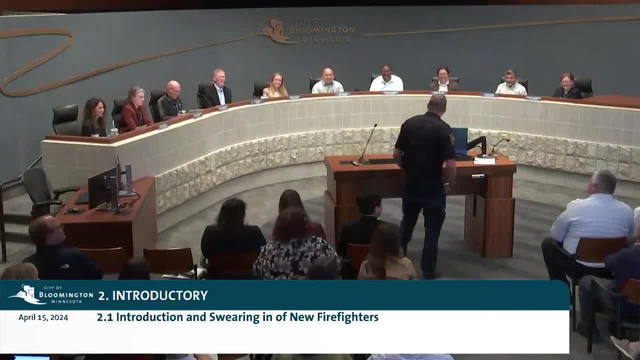 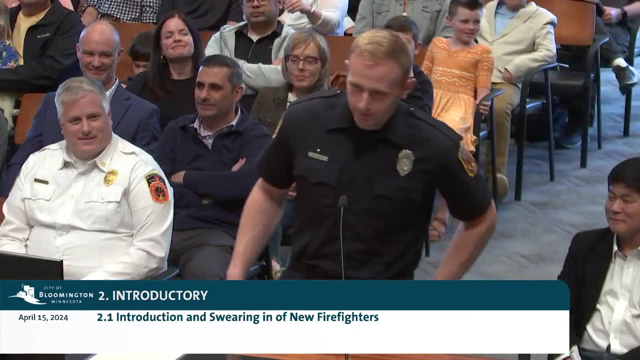 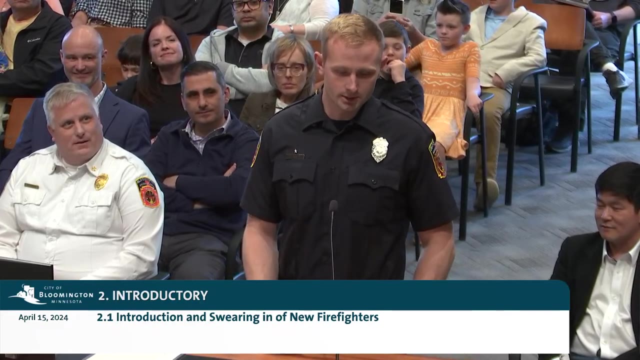 I have two dogs and three fish. Welcome aboard, Thank you. Thank you for being here tonight. Go ahead. Good evening, Council. I'm Malachi Smith. I started my fire career in 2016 as a part-time firefighter with the city of Bloomington. 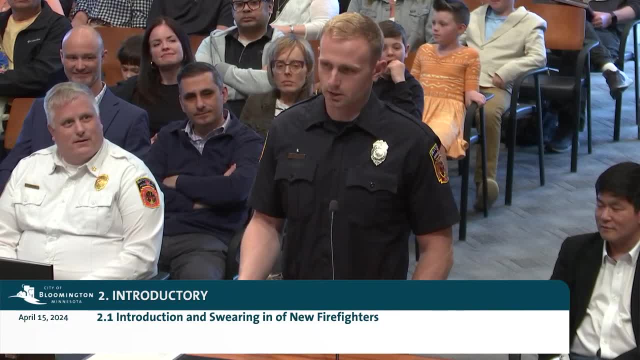 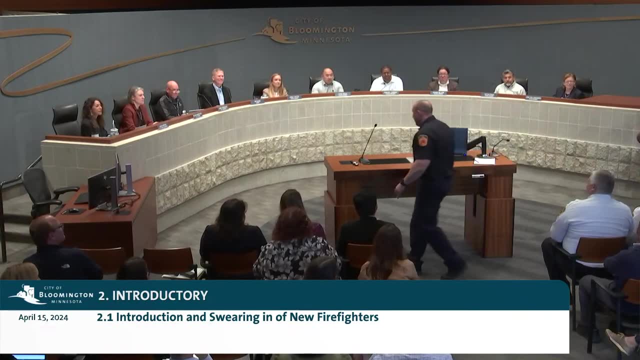 and I've been full-time with Brooklyn Park for the last couple of years and now Bloomington. Thank you Well, glad to have you here, Alex. Welcome. Good evening, Michael Campbell. I've been a paramedic for 13 years, firefighter for 10 years. 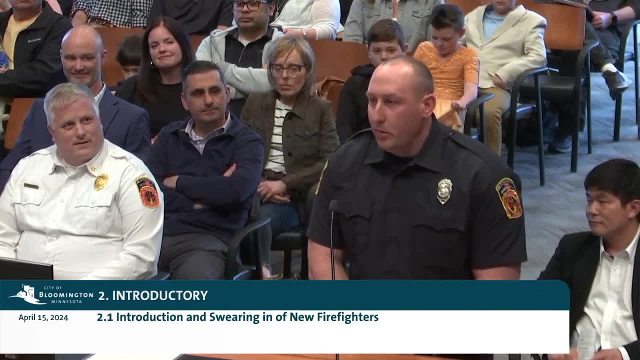 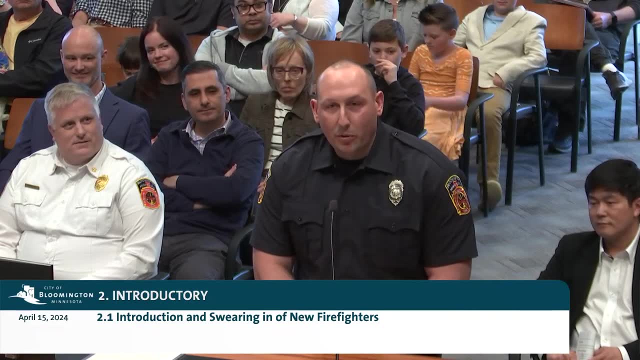 I live in Stillwater and I'm married to my wife, Jessica, and two kids, Afton and Maren. They're six and three. I'm super excited to be working for the city of Bloomington and I want to thank you guys for the opportunity. 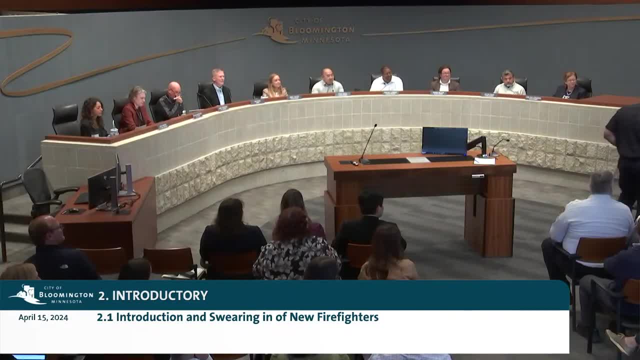 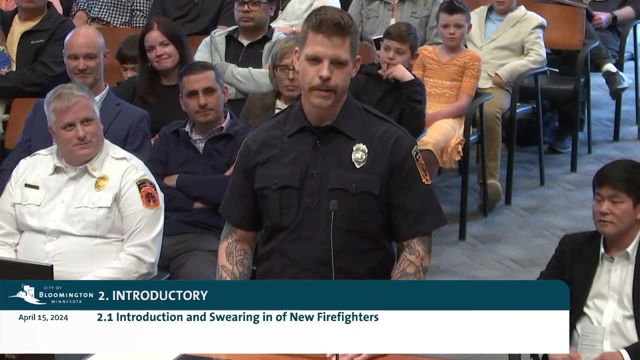 Absolutely. We're excited to have you here, Michael. Thanks for being here. Council, my name is Brandon Sharmer. I've been a firefighter since 2010,. a paramedic since 2015.. I also have a wife and two children. 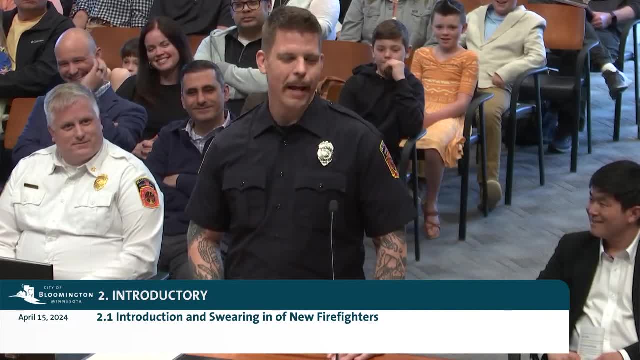 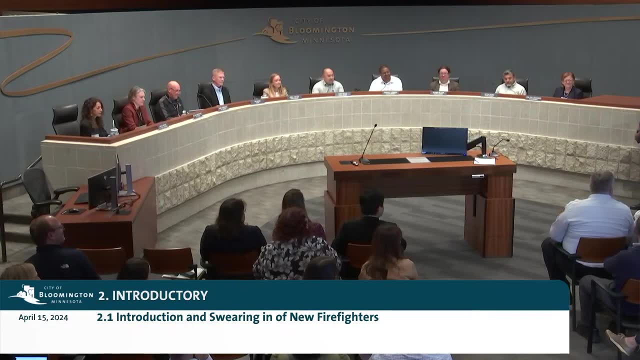 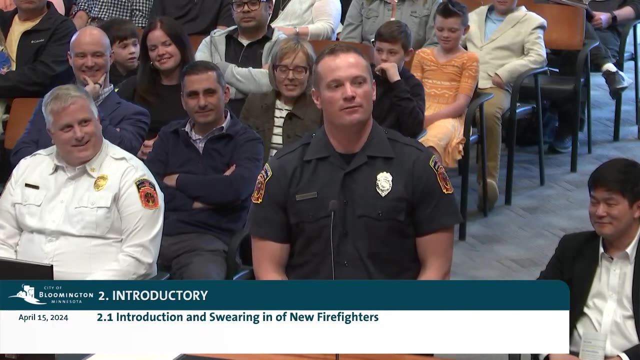 As well as two dogs. no fish, though, and I'm also very happy to be here. Welcome, Let's take those off. Hi, I'm Fritjof Ingebretson. Everyone in the fire department, vast nicknames, but Fitzy's kind of the one that's been sticking. 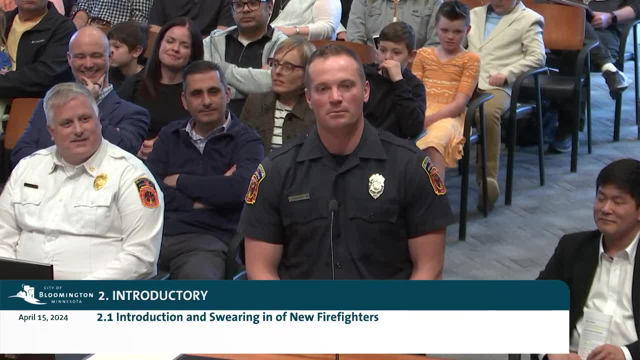 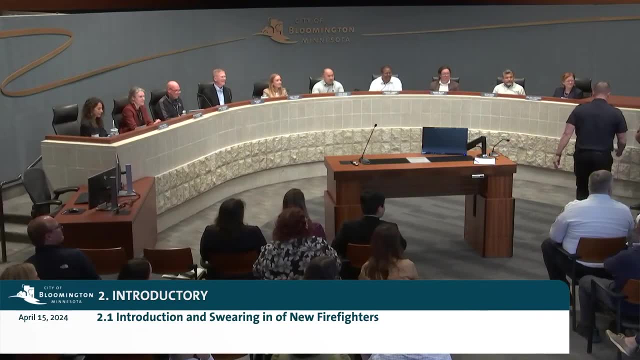 I've been with Bloomington two and a half years, Really excited and happy to be on the full-time side of things and happy to work for the city. Great Glad to have you on the full-time side of things. Thanks, Hi. my name is Dan Cerise. 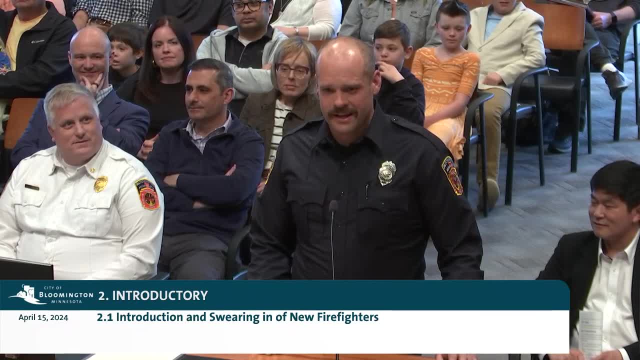 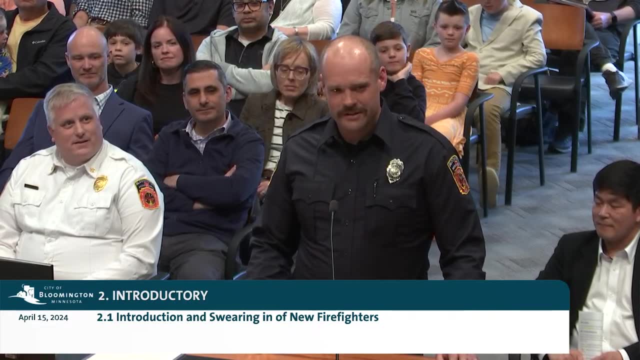 I've been a firefighter since 2005,. a paramedic since 2010.. Previous to here, I was working for the airport next door for six years. Just really excited to be here and be a part of this big investment and change that you guys are making. 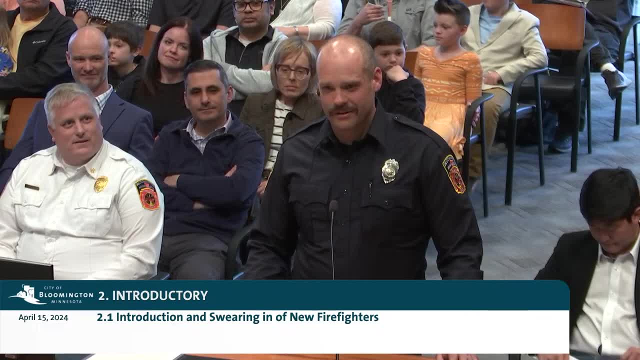 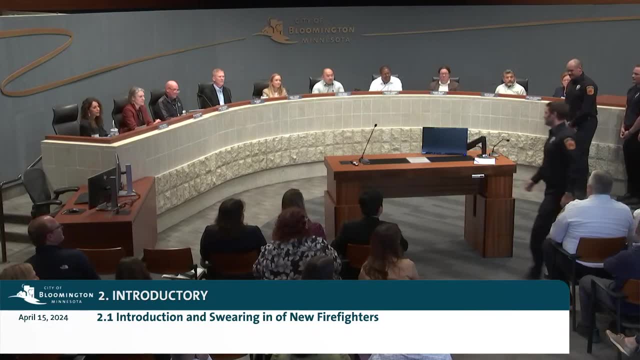 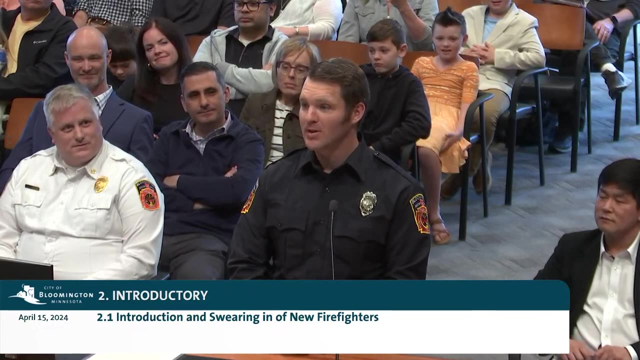 and just seeing where that goes in the future, I think a lot of good things are coming. so thank you Absolutely. Thanks, Dan. Welcome. Good evening, Dylan Gorse. I started in the fire service in 2017.. Got my paramedic in 2021.. 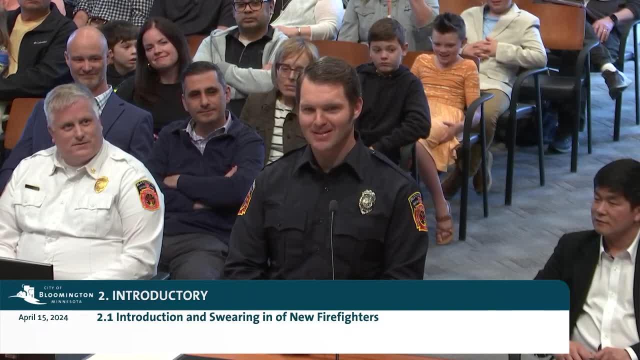 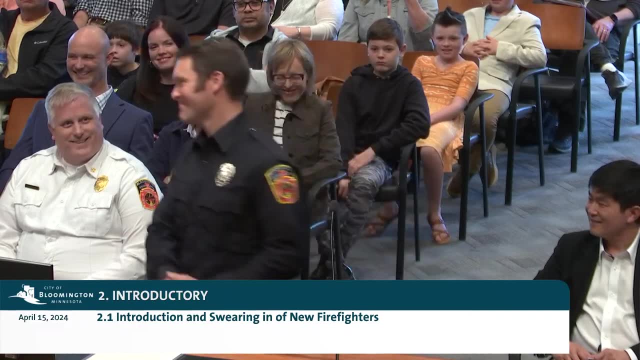 Got a beautiful wife in the crowd here with my two crazy awesome kids as well, And I'm really excited to be part of Bloomington and part of the Magnificent Seven. Nice, Well done and welcome Welcome. Thank you all very much. 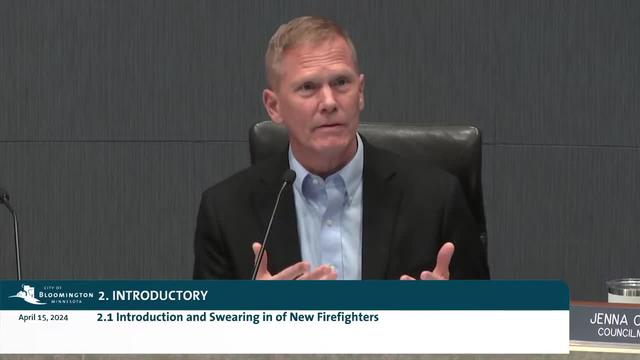 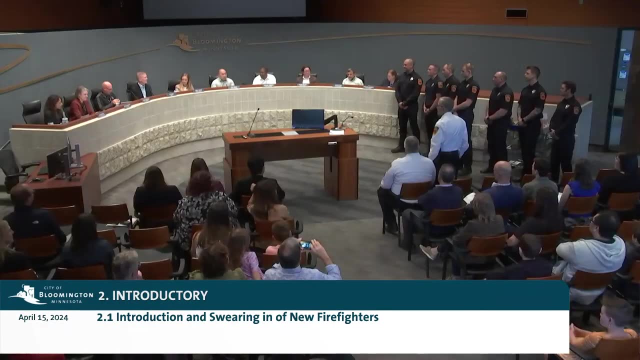 We're so glad to have you on board here And a number of you are here, And a number of you mentioned that this is an important next step for the city of Bloomington that we continue to take. It's the community's commitment to public safety and making sure that we keep our residents and our businesses safe. 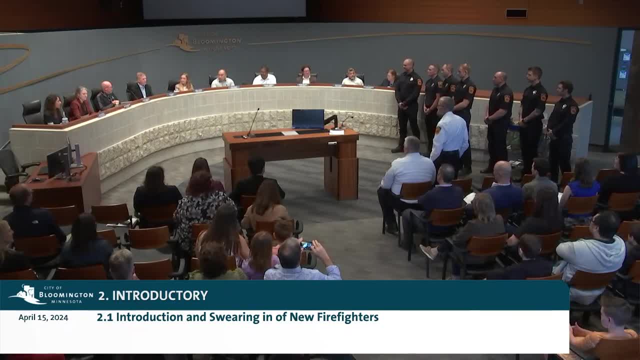 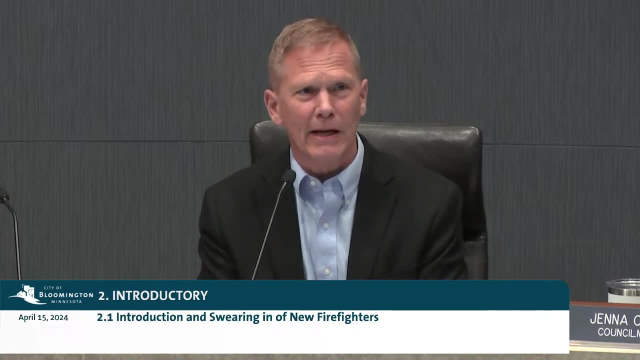 and you play an important role in that. So thank you, Thank you so very much for your commitment and your commitment to this community And White Bear Lake and Stillwater and Blaine- they're wonderful places, but you could move to Bloomington if you really wanted to. 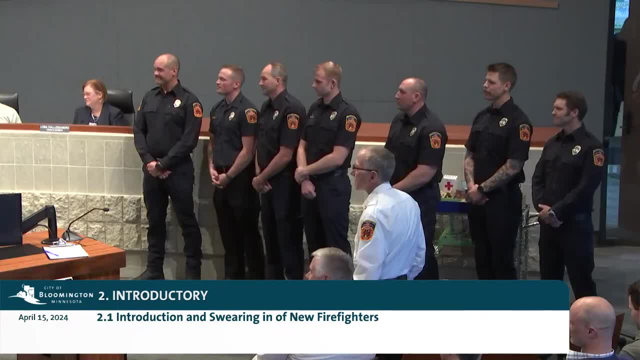 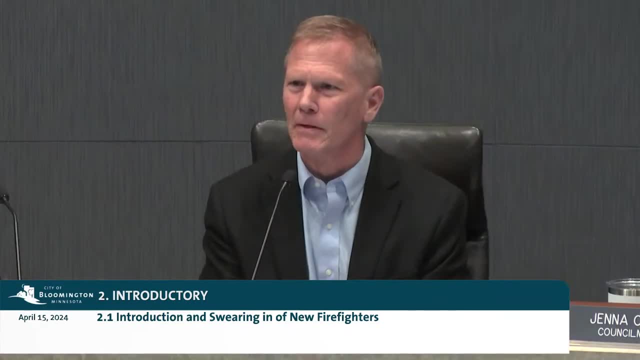 Really wanted to. We'd love to have you here, But very excited to have you here And we're excited to have all of you, All of the family members, Family members, stand up and give a wave. Give a wave everybody. 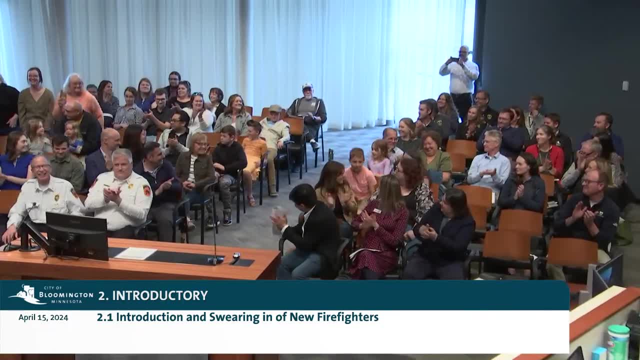 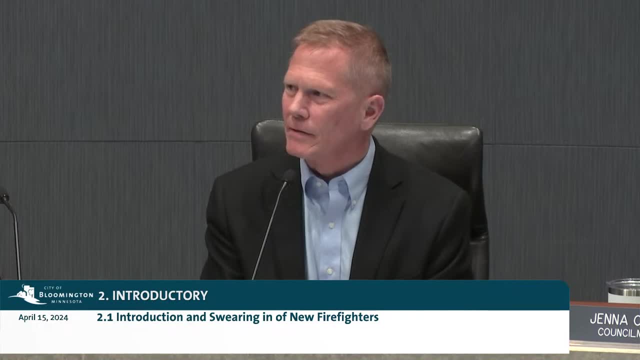 Come on, All the family members. There you go. Well done. So what we're going to do now, we're going to invite our city clerk, Christina Scipione is going to come and do the oath of office. I want to say to family members: this is going to happen once. 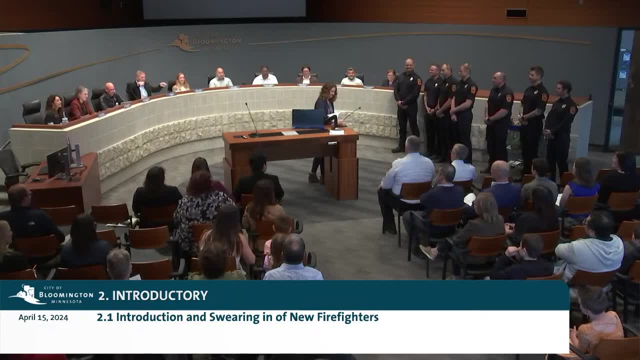 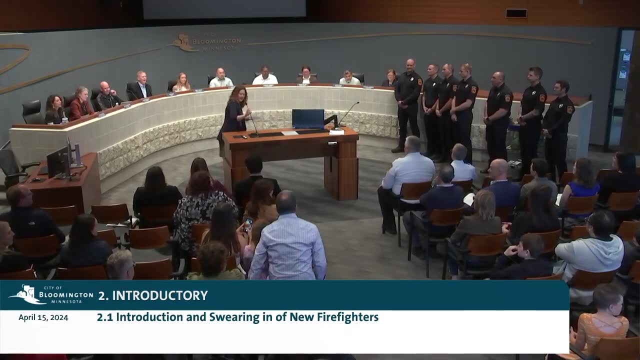 So get up and get in a good position. You can come up here and get wherever you need to get to get a good picture. We're not shy about this. We want you to make sure that you get the picture because, like I said, 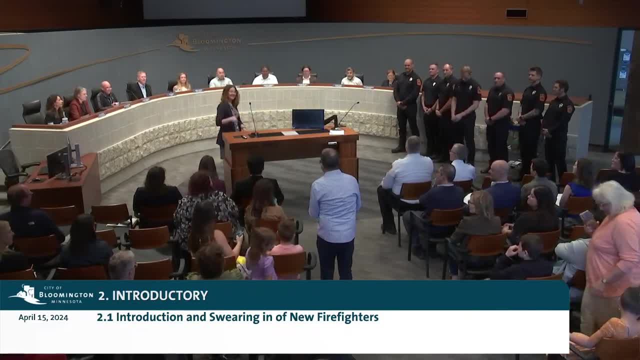 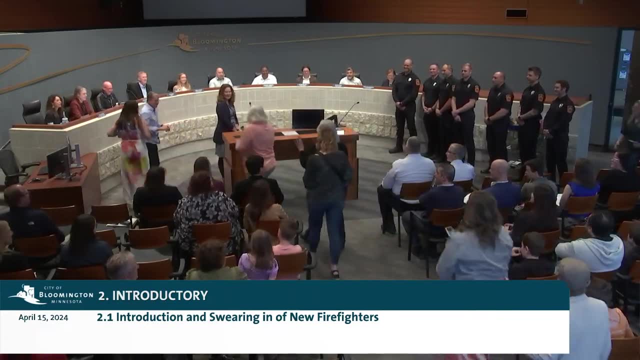 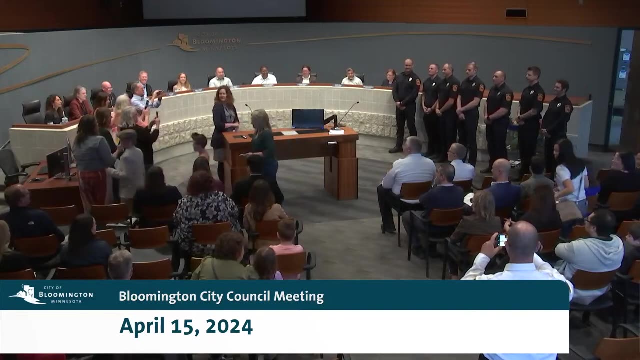 the swearing in is going to happen once. So hold on just one moment, if you could, Christina, come on up here. Come on, You can come right behind her. Yep, come right behind her, Yep, don't be shy. Everybody situated. 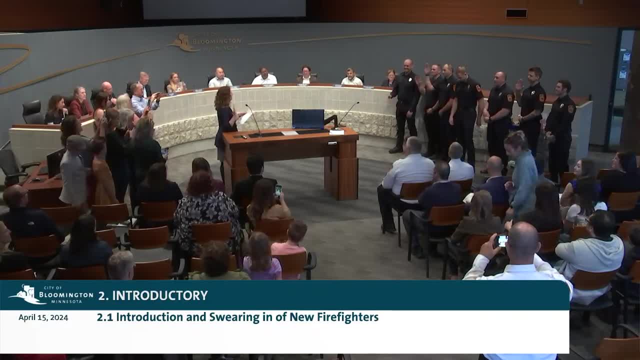 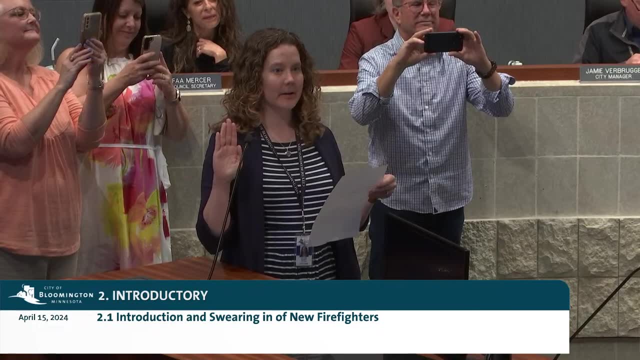 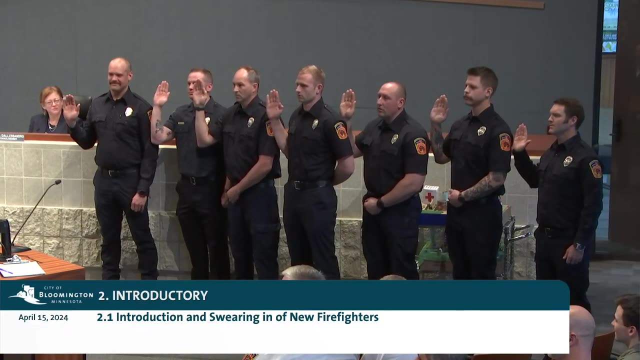 I think we're good, Awesome. Please raise your right hand Good And state your name. Repeat after me. Do solemnly swear that I will support and defend the Constitution of the United States and the Constitution of Minnesota against all enemies, foreign and domestic. 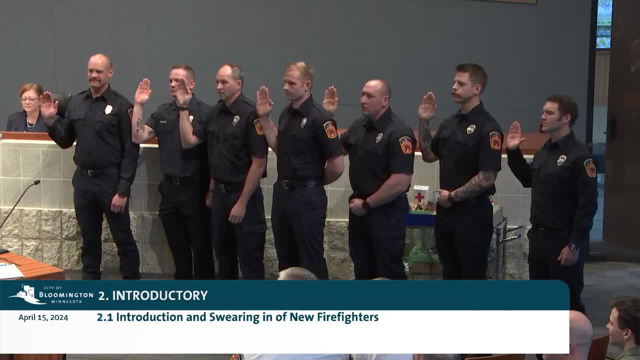 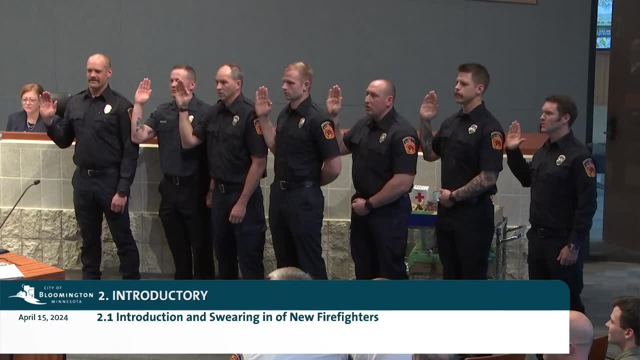 against all enemies, foreign and domestic, that I will bear true faith and allegiance. that I will bear true faith and allegiance, that I will bear true faith and allegiance to the Constitution of the United States, to the Constitution of the United States. 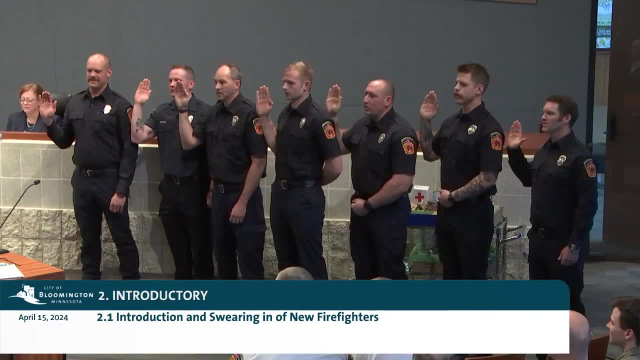 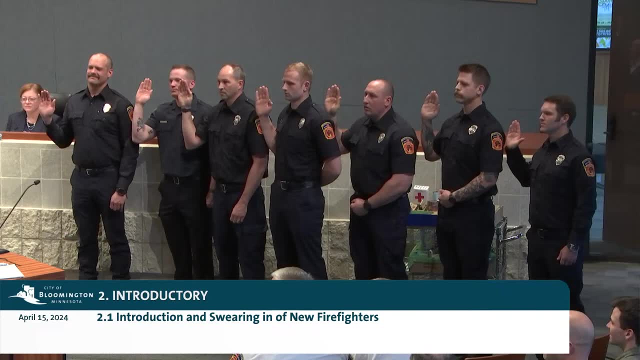 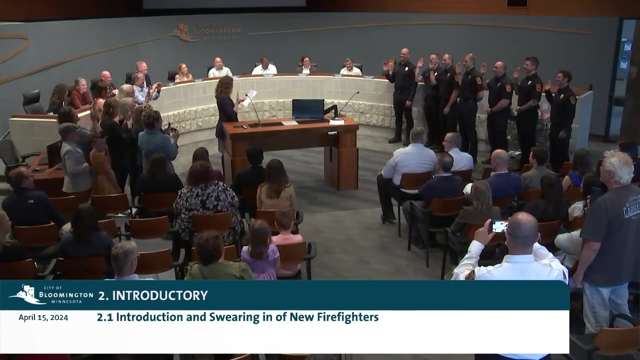 and the Constitution of Minnesota and the Constitution of Minnesota, that I take this obligation freely, that I take this obligation freely without any mental reservation or purpose of evasion, without any mental reservation or purpose of evasion, and that I will well and faithfully discharge the duties. 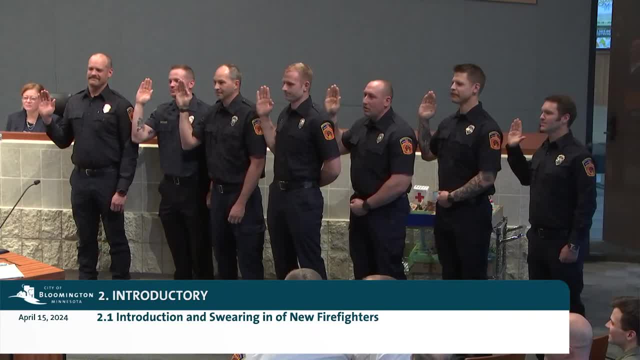 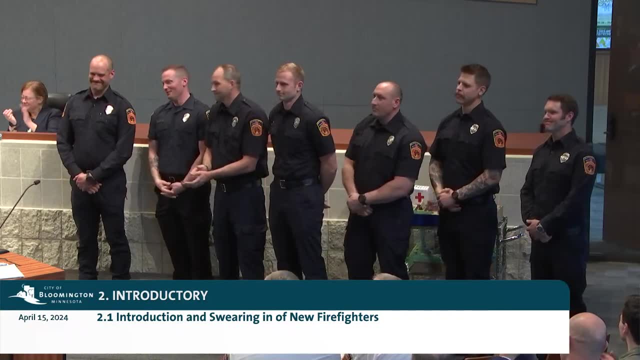 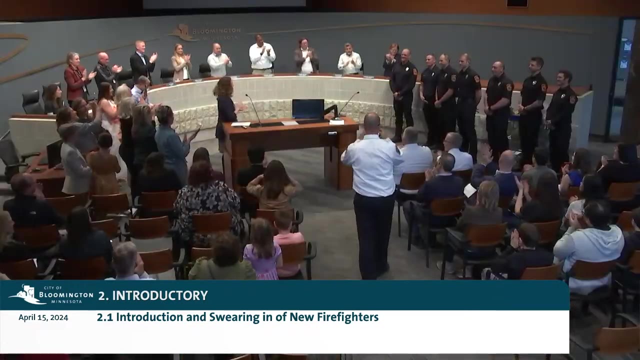 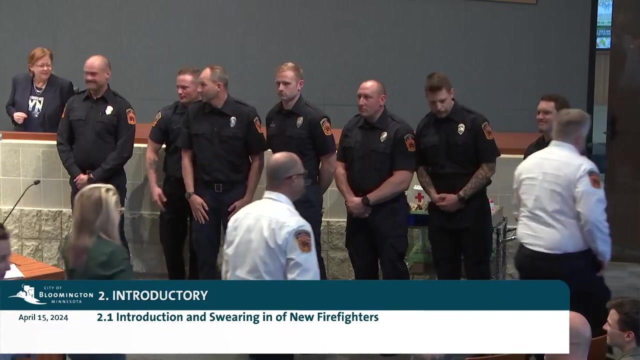 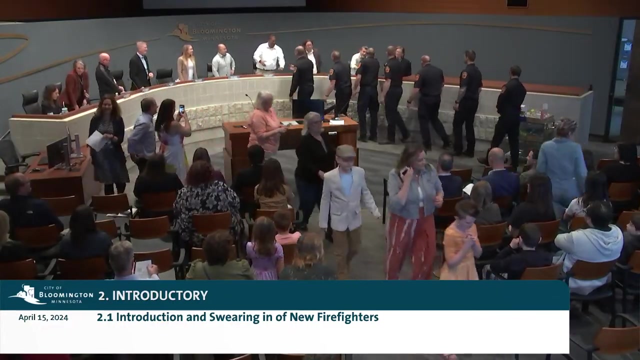 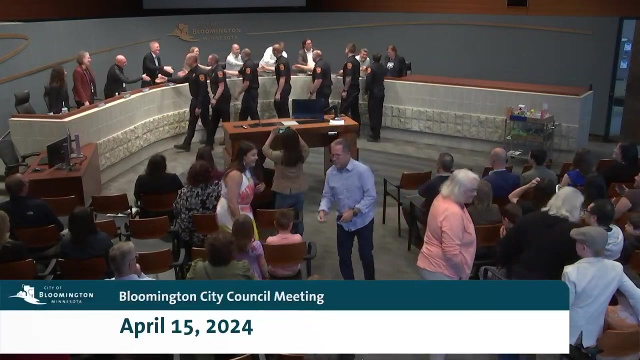 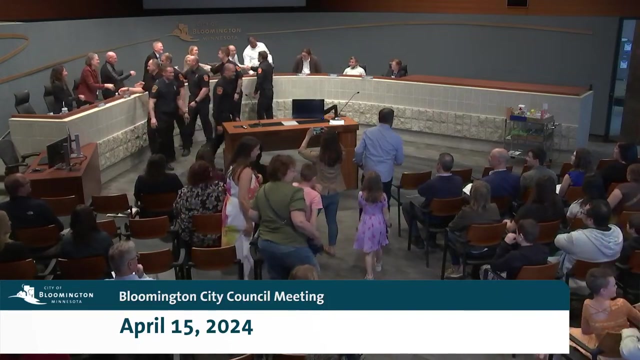 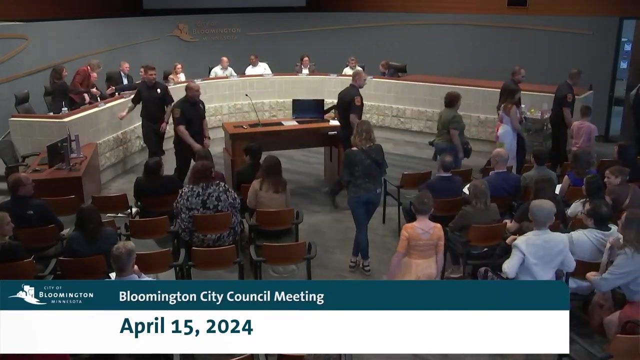 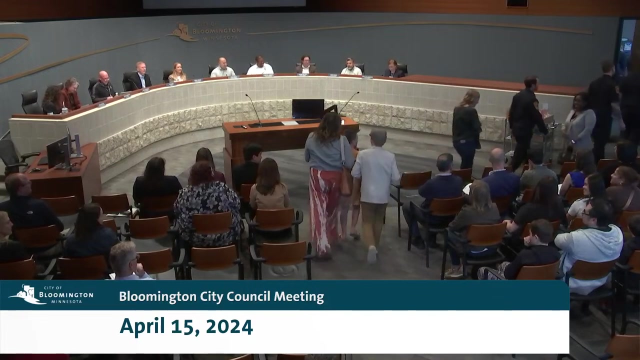 and that I will well and faithfully discharge the duties upon which I am about to enter. Congratulations, Congratulations. Well, welcome aboard, gentlemen, Glad to have you here. Thank you very much, I think the next steps- I'm pretty sure there's a party somewhere in the building here- 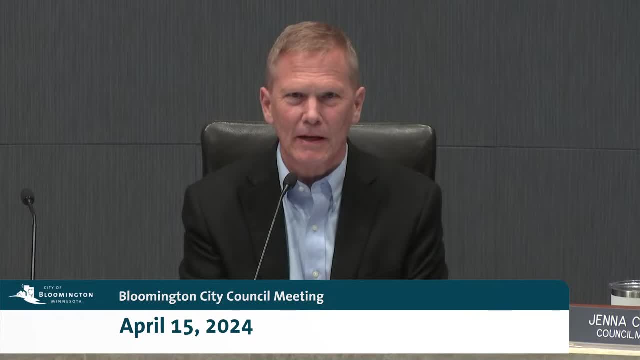 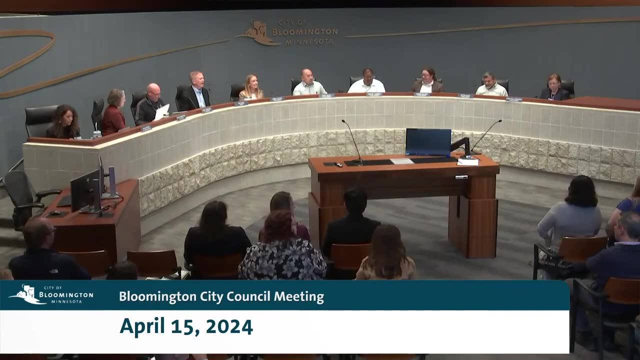 And so we're going to pause just a moment so the families can get out and make sure they join the firefighters and we move on. I see our command staff back there in white. Thanks much for the work that you're doing bringing these folks along. 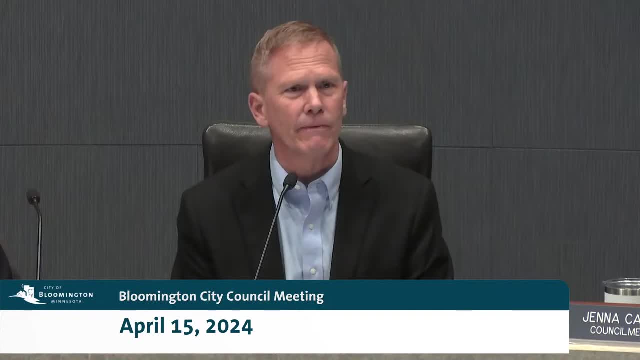 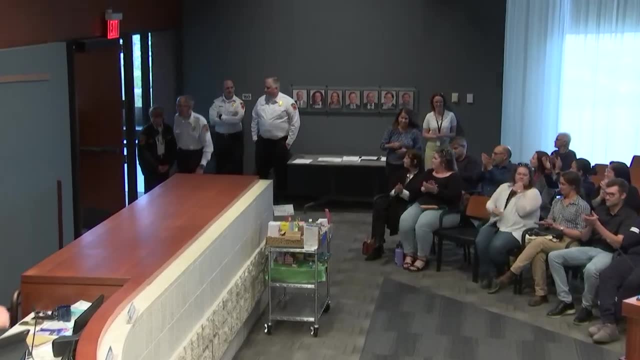 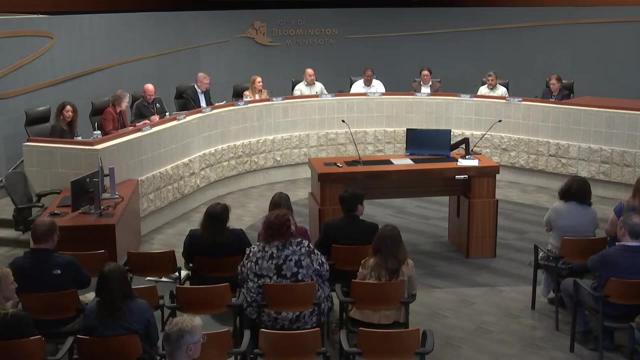 This is an important, important step that we're taking with this city, and your leadership is invaluable, So thank you. I want to give you a round of applause also for the outstanding work that you guys are doing. Next up, we have three different proclamations. 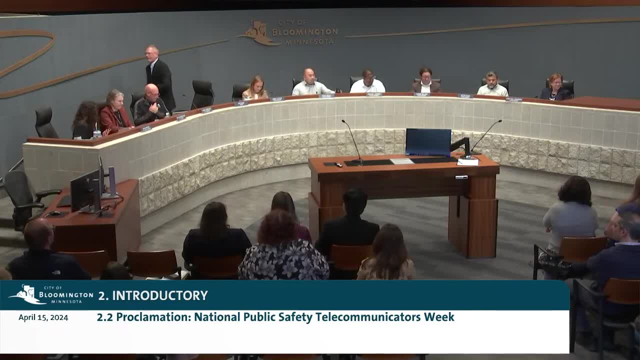 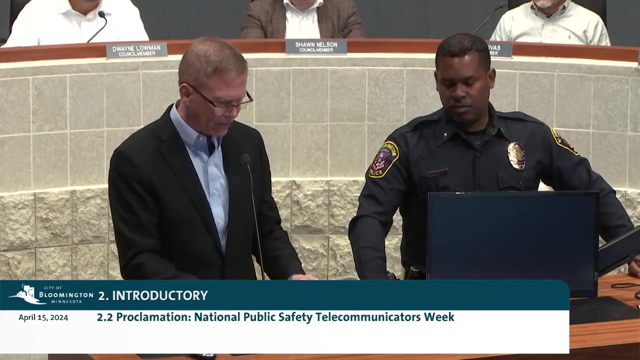 So I'm going to come down to the desk Every single time, Thank you. So we have, As I said, three different proclamations this week, And we're going to start with the proclamation for the National Public Safety Telecommunicators Week. 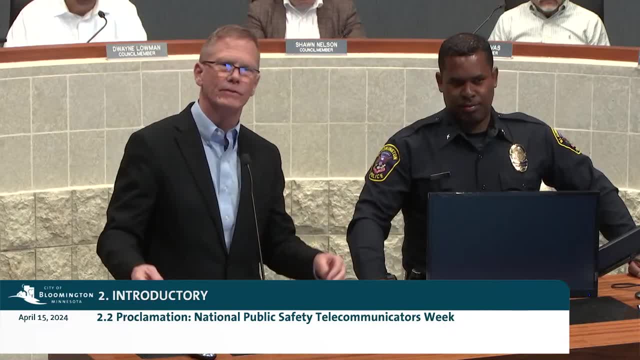 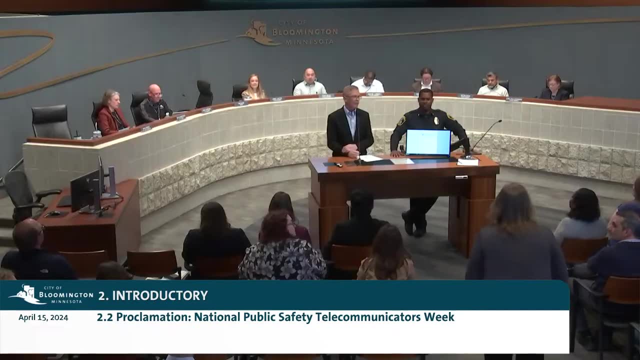 And I think wedo we have any telecommunicatordo, we have any telecommunication staff here. Do you all want to come up as well, Please do? These folks are, I mean, definitely the unsung heroes of our police department. 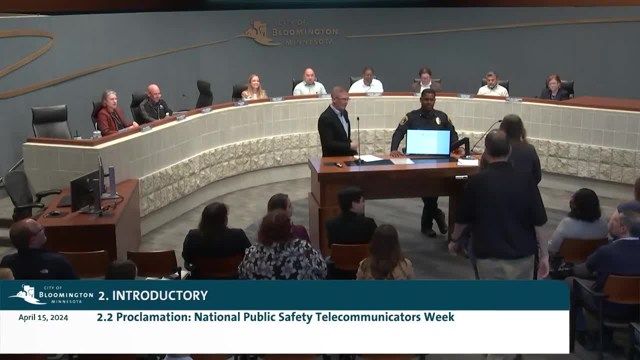 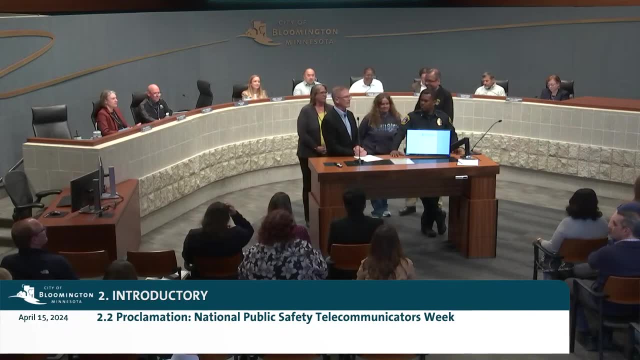 Play such an important role. income on. you got to get on camera. Come on, Play such an important role, not only with our police work but our fire work, And I appreciate that we do this yearly, that this is an opportunity. 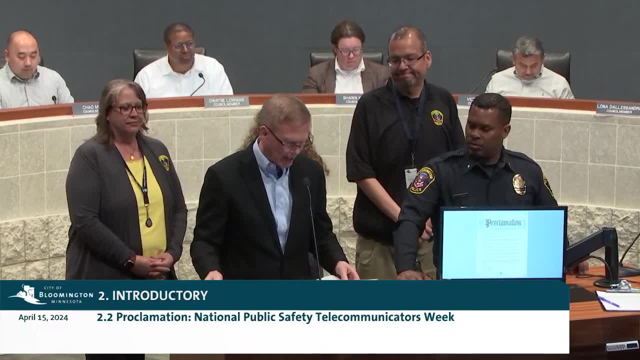 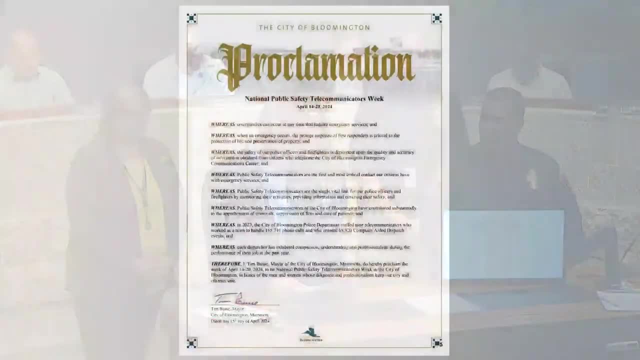 to recognize the work that we do. I recognize the great work that you do, And it's a proclamation for a National Public Safety Telecommunicators Week, April 14th through the 20th 2024.. Whereas emergencies can occur at any time that require emergency services, 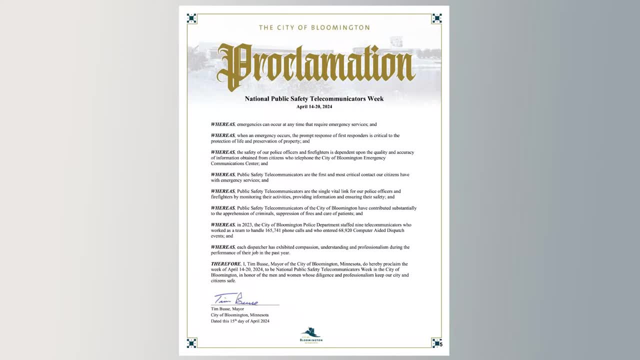 And whereas when an emergency occurs, the prompt response of first responders is critical to the protection of life and the preservation of property. And whereas the safety of our police officers and firefighters is dependent upon the quality and the accuracy of information obtained from citizens who telephone the City of Bloomington Emergency Communications Center. 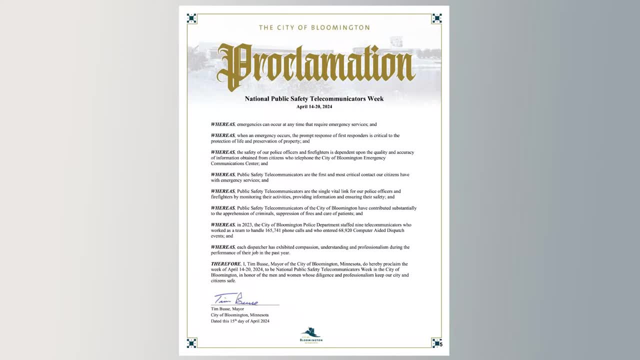 And whereas public safety telecommunicators are the first and most critical contact our citizens have with emergency services. And whereas public safety telecommunicators are a single vital link for our police officers and firefighters, by monitoring their activities, providing information and ensuring their safety. 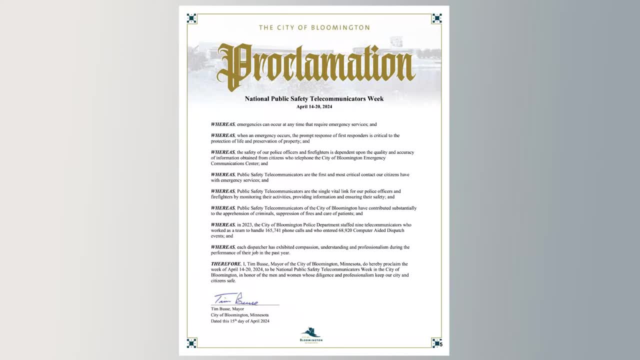 And whereas public safety telecommunicators of the City of Bloomington have contributed substantially to the apprehension of criminal criminals, the suppression of fires and care of patients, And whereas in 2023, the City of Bloomington Police Department staffed nine telecommunicators, 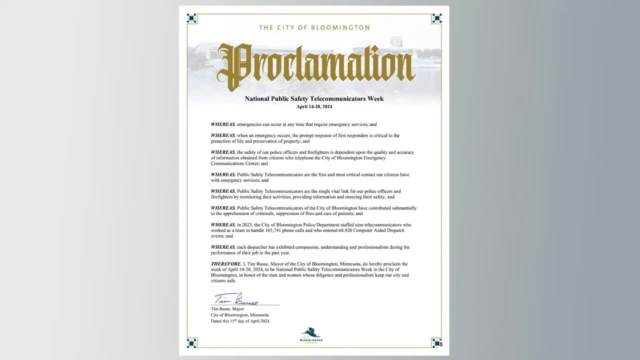 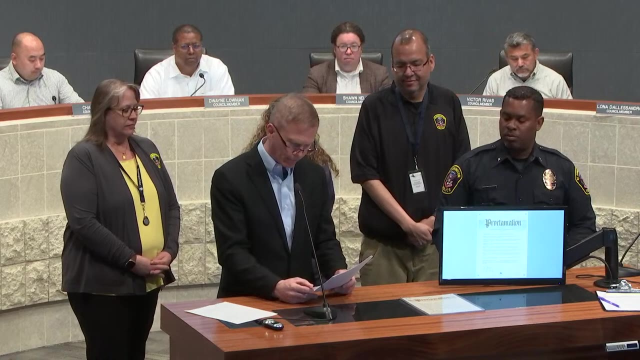 who worked as a team to handle- now get this- 165,741 phone calls and who entered 68,920 computer-aided dispatch events, And whereas each dispatcher has exhibited compassion, understanding and professionalism during the performance of their job in this past year. 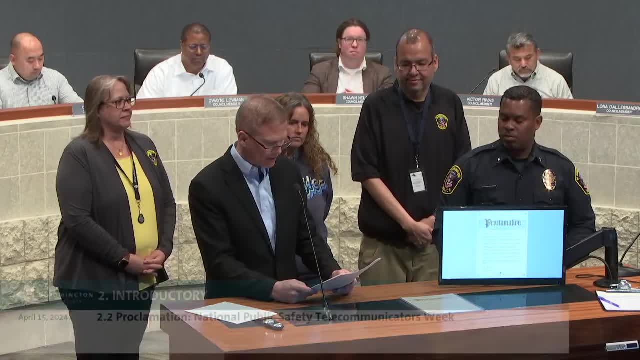 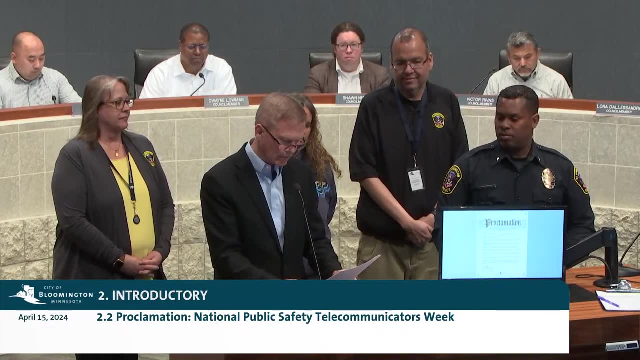 And whereas each dispatcher has exhibited compassion, understanding and professionalism during the performance of their job in this past year, Now, therefore, I, Tim Bussey, Mayor of the City of Bloomington, Minnesota, do hereby proclaim the week of April 14th through the 20th, 2024, to be National Public Safety Telecommunicators Week in the City of Bloomington. 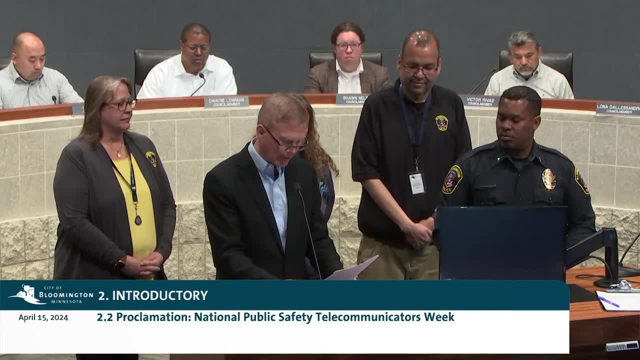 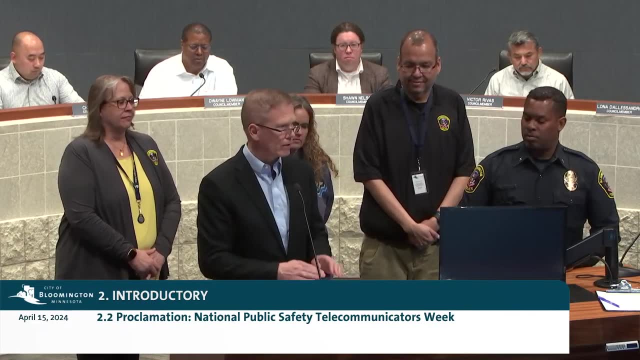 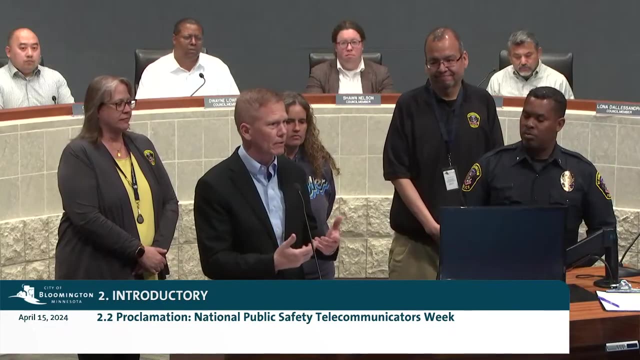 in honor of the men and women whose diligence and professionalism keep our city and our citizens safe, dated this 15th day of April 2024.. That number of phone calls to me is just staggering. The number of calls that come in and then calls that then go out to our fire department, to our police department. 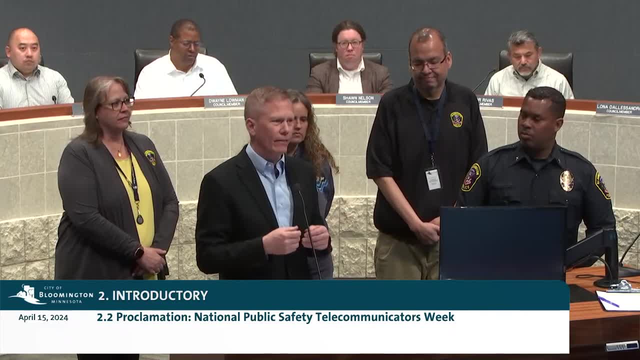 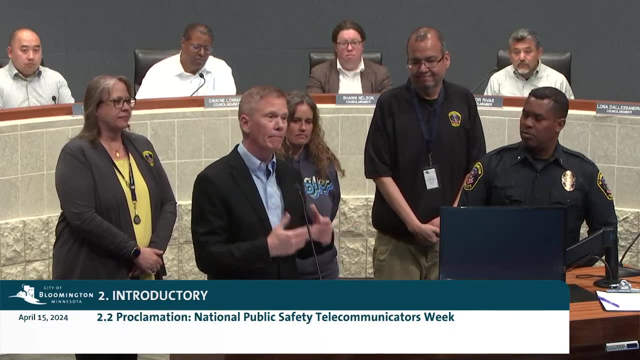 the work that goes on The integration of knowledge. there's a lot of moving parts and these folks do it so incredibly well to keep our- not only our- public safety responders safe, but the general public safe as well. So, Chief, did you want to say anything in addition? 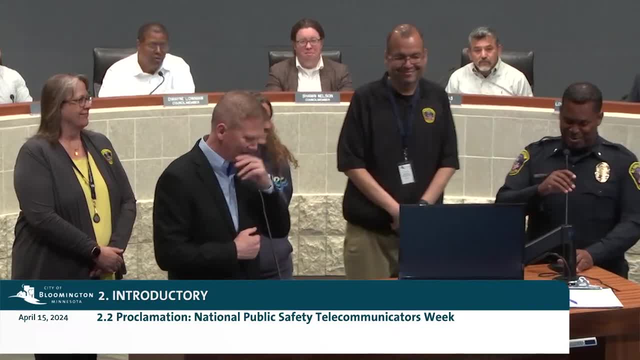 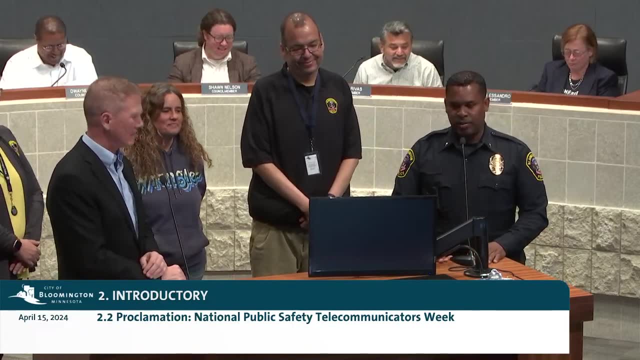 You can use that microphone. We got a joke. Wow, I got my own mic. Ooh boy, This is a scary thing. You got jokes still. In all seriousness, our telecommunicators do a phenomenal job and in Bloomington we are fortunate. 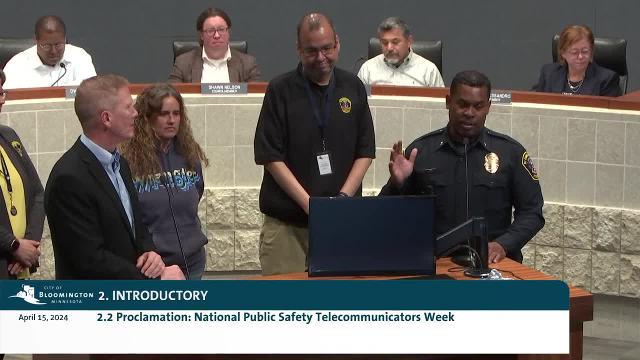 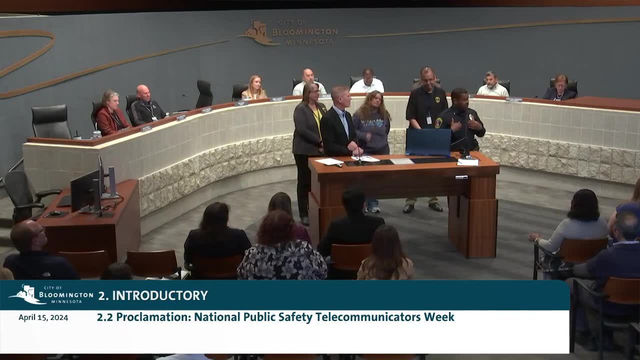 We are fortunate to have the best people doing this job And I can tell you I've been in Ramsey County, Dakota County and Scott County and at the state and never have I worked with a group of talented telecommunicators like we have here. 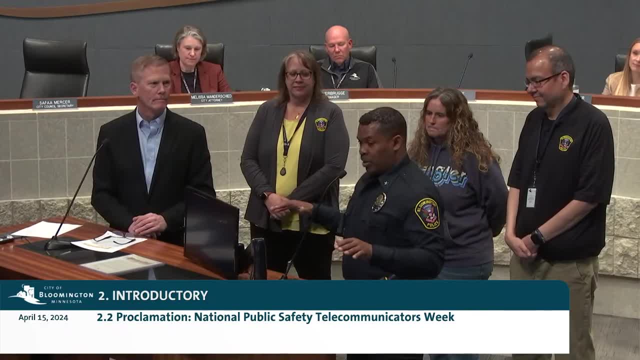 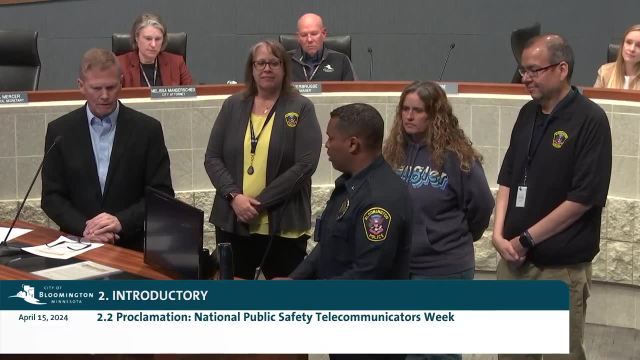 The amount of work that goes into what they do doesn't happen anyplace else And I think the citizens of Bloomington often sometimes don't get to see that, but we get to see that every day. the work that they do It's not just kissing up to them because we like their job. 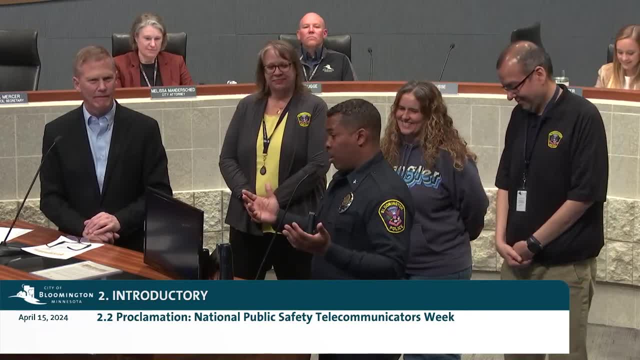 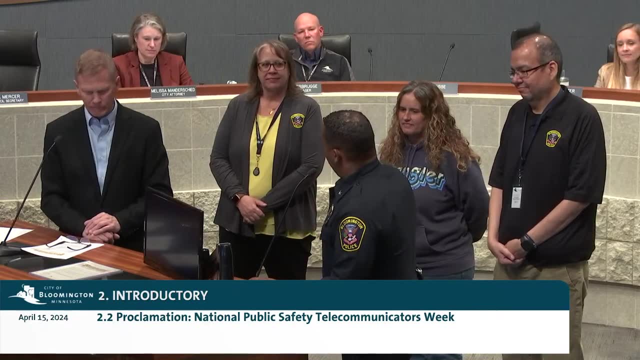 But no, they do a phenomenal job For both us and the fire department in Bloomington. we are fortunate We have our own dispatch center, so that's something that a lot of other cities do not have. So with that, I'll let the supervisor, who does the real work, come up and say a couple words. 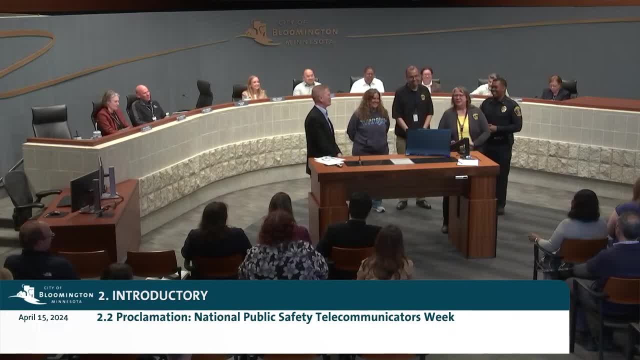 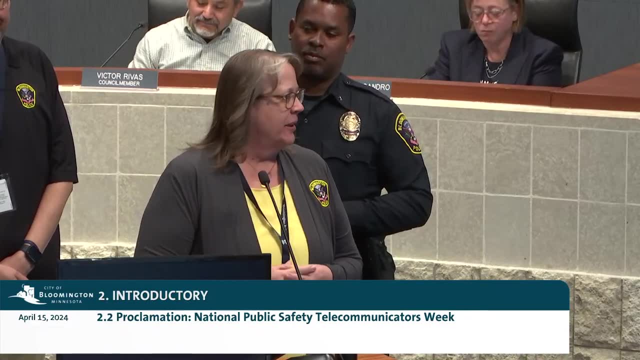 I know, You know I was going to put you on the spot. Thanks a lot. I just want to say I get to sit behind and watch them do their job, so I have the easy part, And they do a phenomenal job 24-7,, 365, no matter what's going on at any point in time. 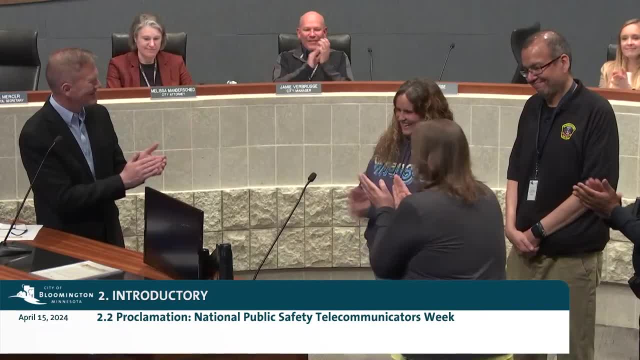 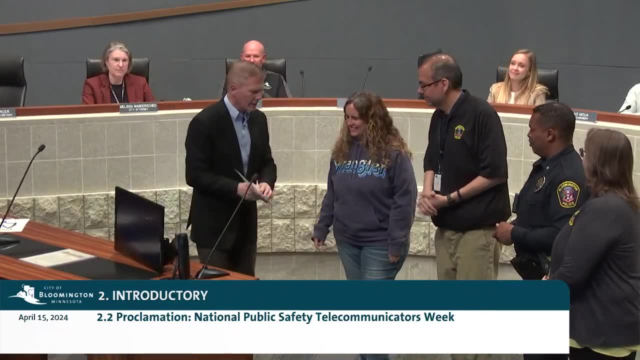 They're consummate professionals. so Thank you. So we've got the proclamation, We're going to give it to you and we're going to get a picture, because you've got to do a picture if you're going to do all of this. 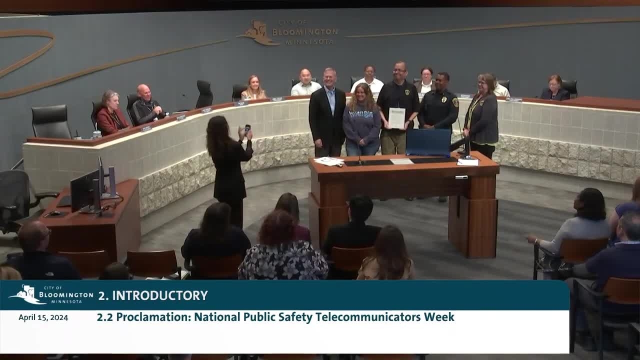 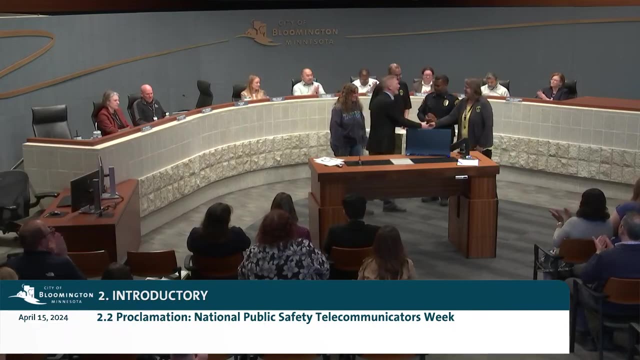 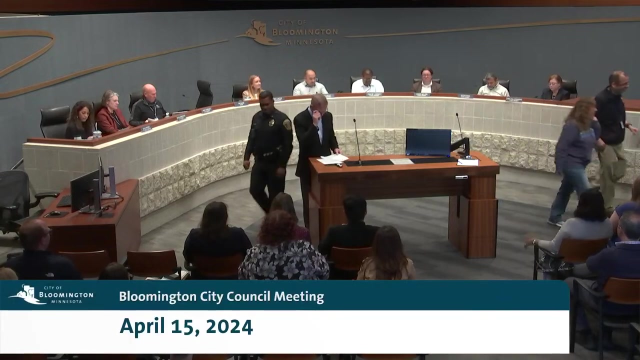 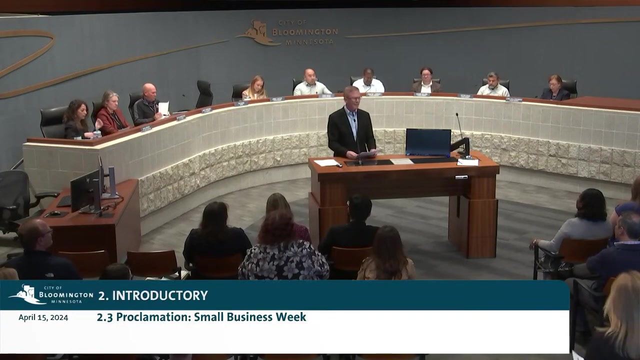 There you go. All right, No fake smile. Thank you, Congratulations, Thank you, Thank you so very much, Thanks. Thanks for being here. Thank you, Thank you, Keep going, Keep going, There you go. Our next proclamation tonight is Item 2.3, Proclamation Regarding Small Business Week. 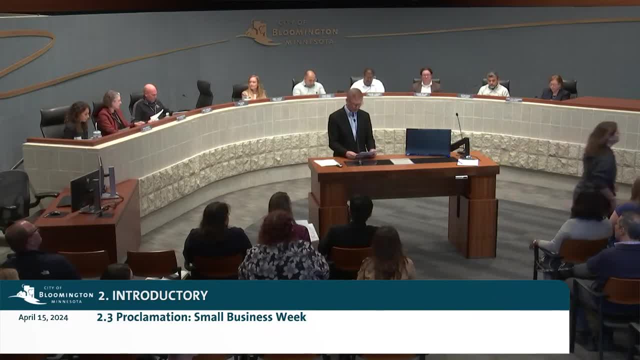 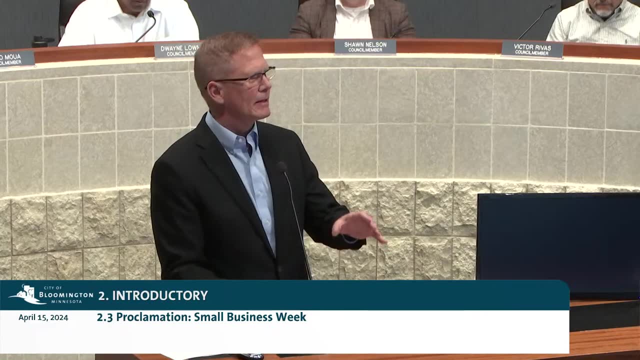 And this year the city of Bloomington partnered with our friends at Hennepin County to launch a new pilot program called CEO Start, And I'll let – we're going to hear more about this, And I'll let some folks who know it better than I do explain it. 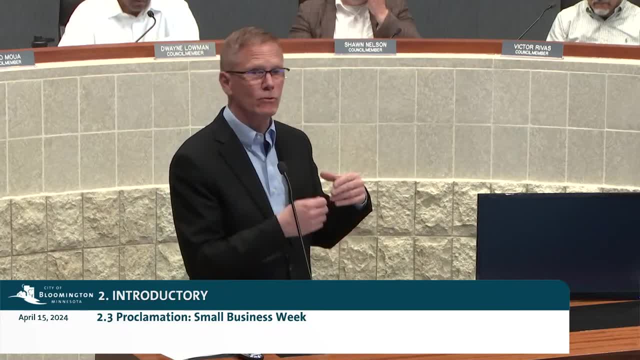 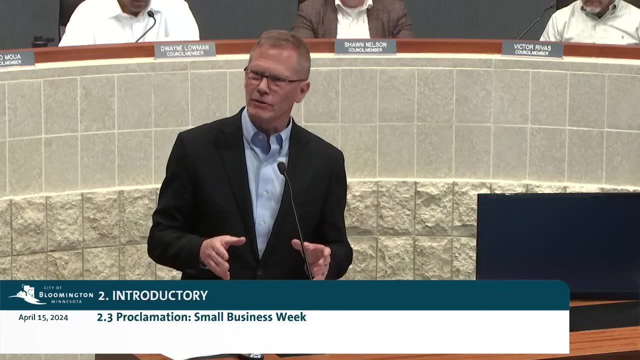 But basically it's an opportunity for folks who wish to be CEOs, who are looking to be entrepreneurs, giving them the resources to launch, to start what they were doing, And I had the pleasure, the incredible pleasure last week to be at the graduation of these 12 folks from this program. 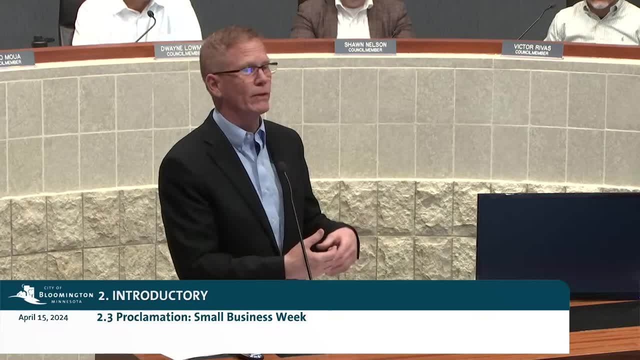 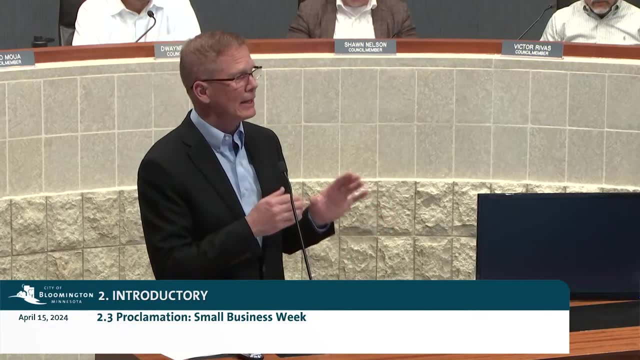 And to hear each of them talk about what their vision is, what they were hoping to do for their business, was just so inspiring, And I've told a number of people this over the past couple of days. Not one of you said I want to do this business or this business or this business because I want to make gobs of money. 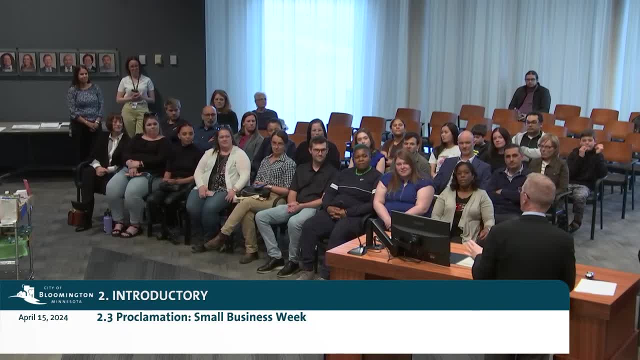 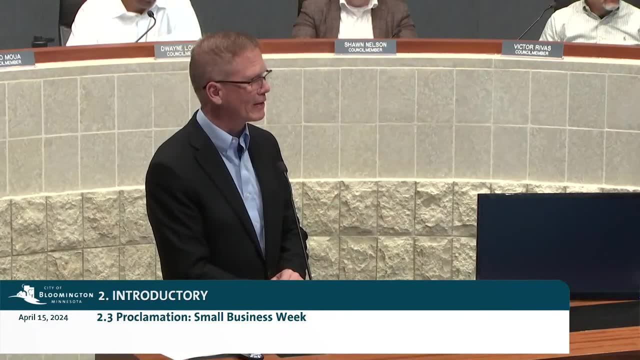 I want to be enormously successful. Every one of you talked from the heart. You were doing something that was near and dear to you And that was – it absolutely filled my cup. It was a wonderful evening last week, And so thank you so very much for that. 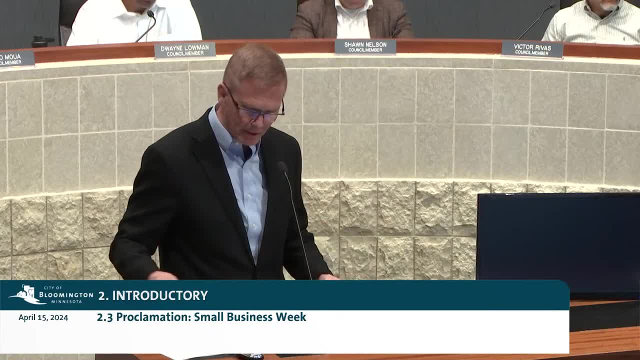 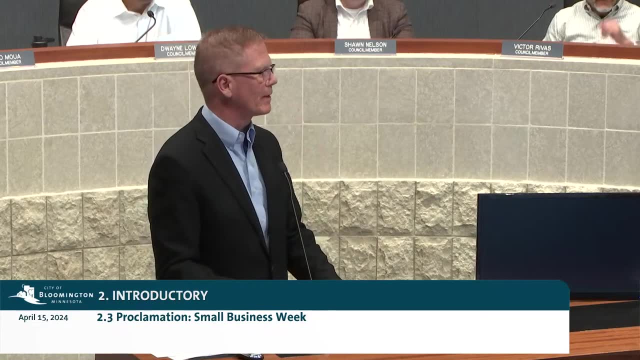 And thanks for going through the program And in our proclamation of Small Business Week. if any or all of you want to come up and stand behind me, please do. You might as well get on camera. Come on, We might as well get everybody up here. 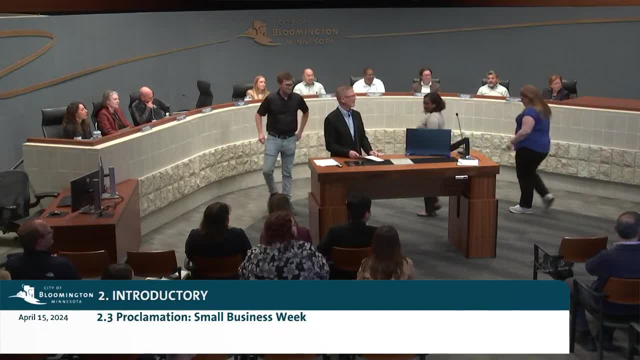 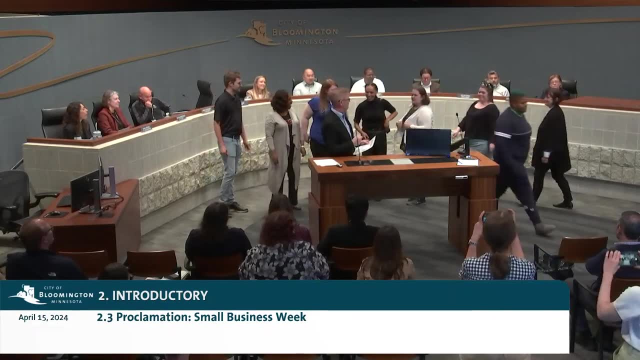 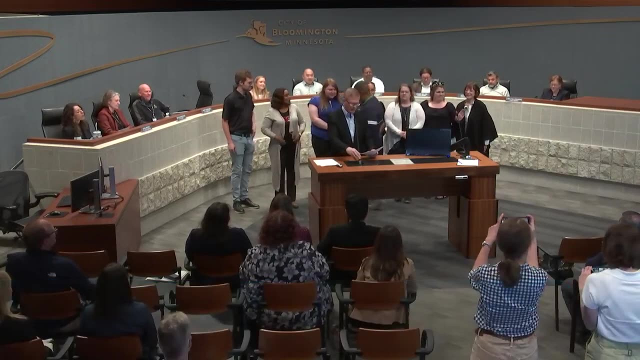 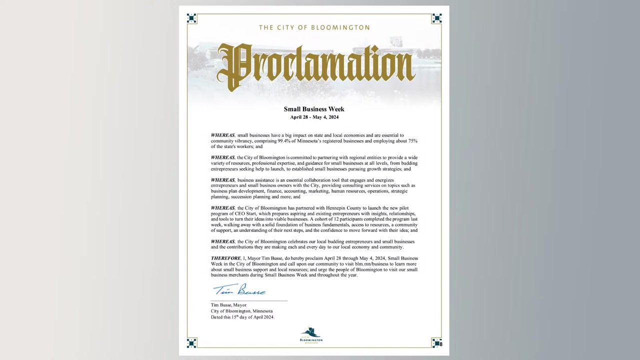 Our proclamation for Small Business Week, April 28th through May 4th 2024.. Whereas small businesses have a big impact on state and local economies and are essential to community vibrancy, comprising 99.4% of Minnesota's population, 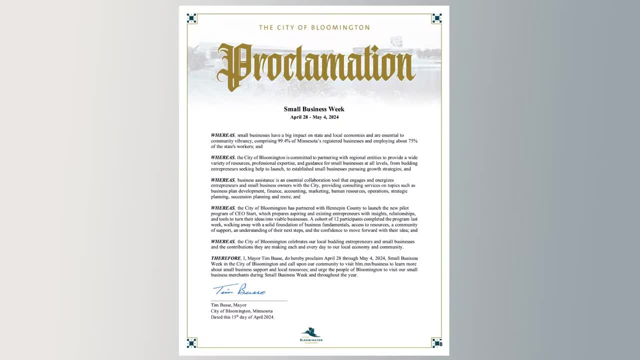 and employing about 75% of the state's workers, And whereas the city of Bloomington is committed to partnering with regional entities to provide a wide variety of resources, professional expertise and guidance for small business at all levels, from budding entrepreneurs seeking help to launch to establish small businesses pursuing growth strategies. 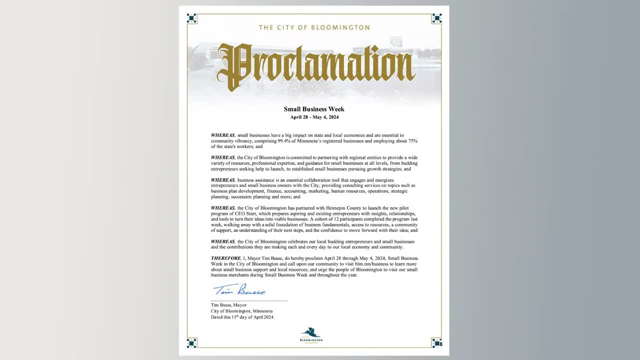 And whereas business assistance is an essential collaboration tool that engages and energizes entrepreneurs and small business owners within the city, providing consulting services on topics such as business plan development, finance, accounting, marketing, human resources, operations, strategic planning, succession planning and much, much more. 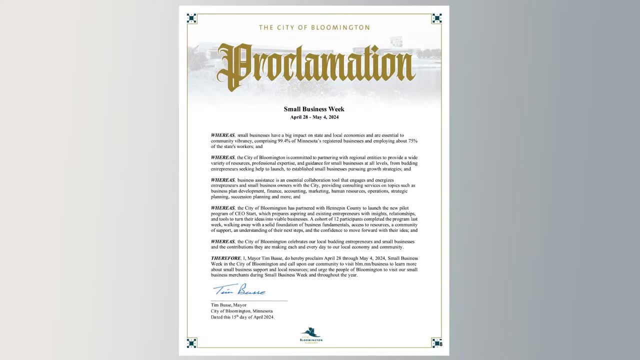 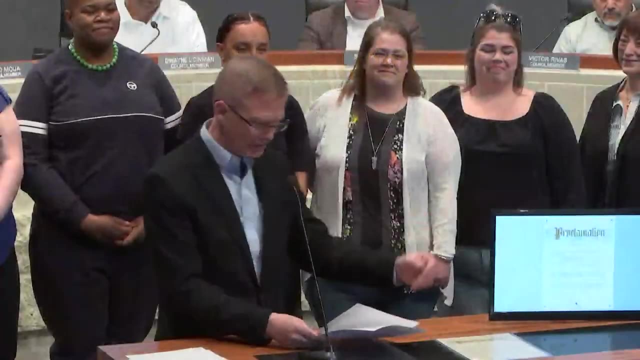 And whereas the city of Bloomington has partnered with Hennepin County to launch a new pilot program of CEO Start, which prepares aspiring and existing entrepreneurs with insights, relationships and tools to turn their ideas into viable businesses. A cohort of 12 participants- these folks, 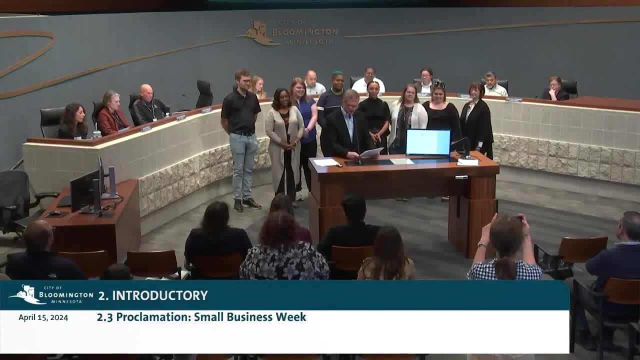 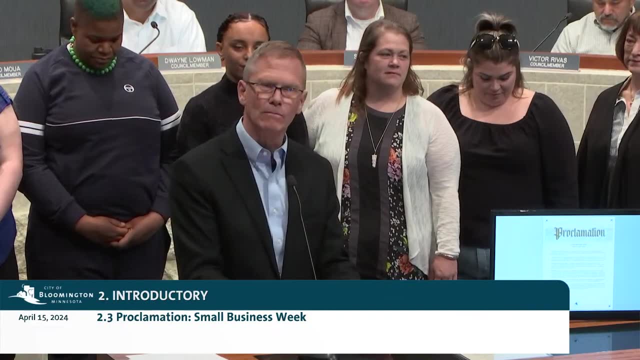 completed the program. We now have 7,000 people here the program last week walking away with a solid foundation of business fundamentals, access to resources, a community of support and understanding of their next steps and the confidence to move forward with their ideas. And whereas the City of Bloomington celebrates our local budding, 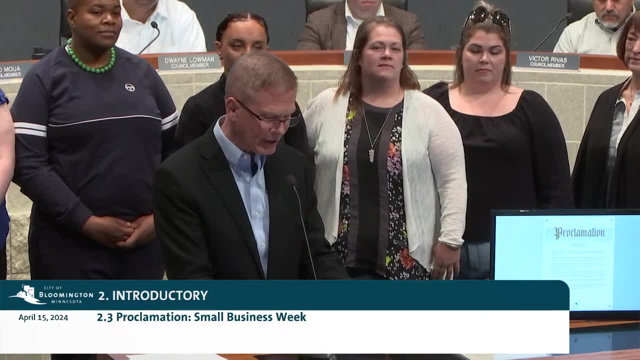 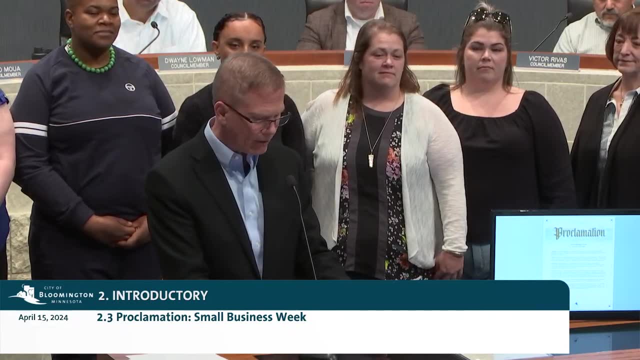 entrepreneurs and small businesses and the contributions they are making each and every day to our local economy and community. Now, therefore, I, Mayor Tim Bussey, do hereby proclaim April 28th through May 4th, 2024, Small Business Week in the City of Bloomington and call upon our community. 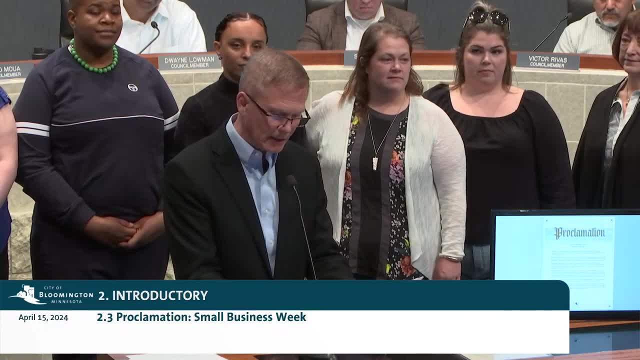 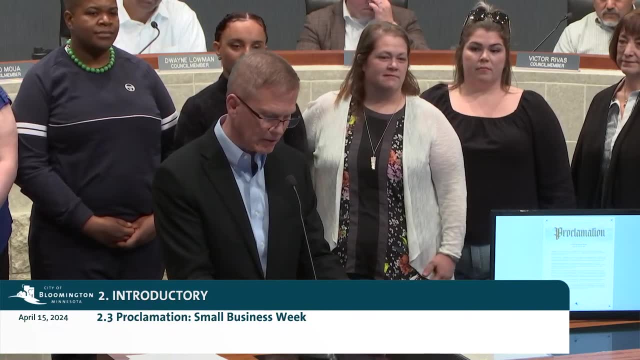 to visit blmmn forward slash business to learn more about small business support and local resources, and urge the people of Bloomington to visit our small business merchants during Small Business Week and throughout the year dated this 15th day of April 2024.. This was, as I said, a 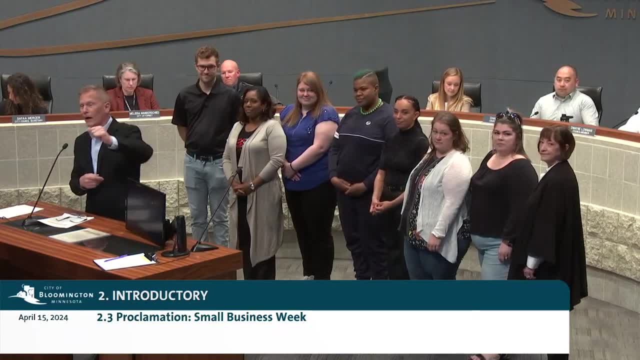 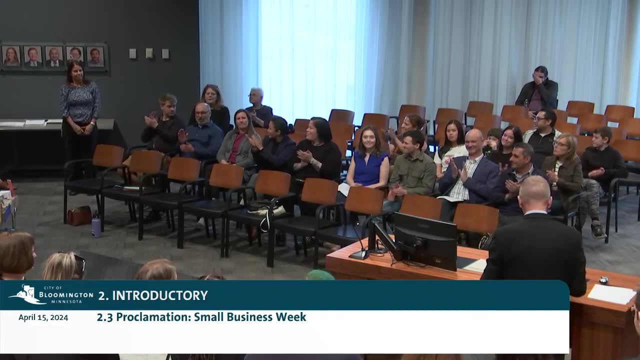 fabulous group. They did so much great work. Barb Wolf on our city staff was kind of their shepherd in leading them along and did outstanding work, And I want to thank the City of Bloomington for their outstanding work. I want to thank and congratulate Barb for the work that she did also. 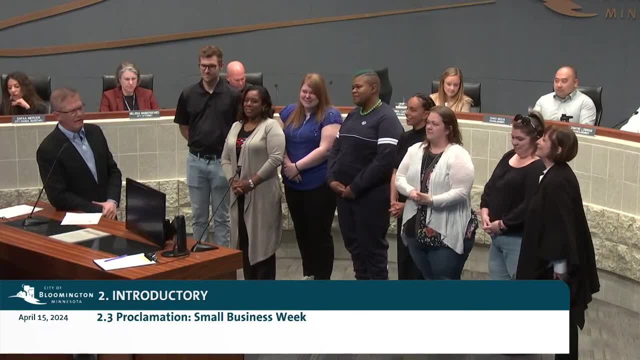 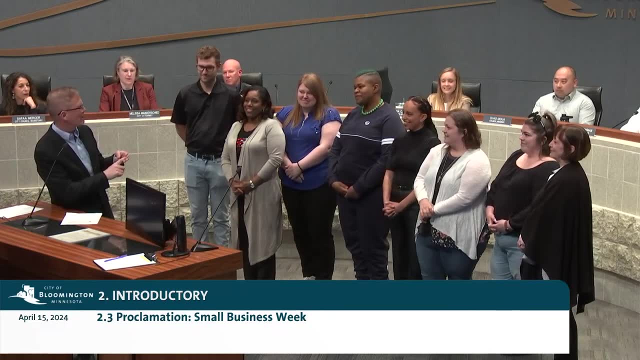 And, in the idea of marketing, I'm going to give you guys the microphone, Tell us your name, your business and, if you've got a website address, a really quick website address because you're on camera. Okay, you're on camera. All right, Everybody, step on up, Everybody. 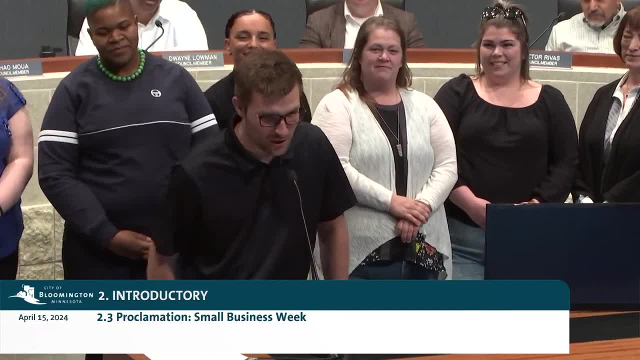 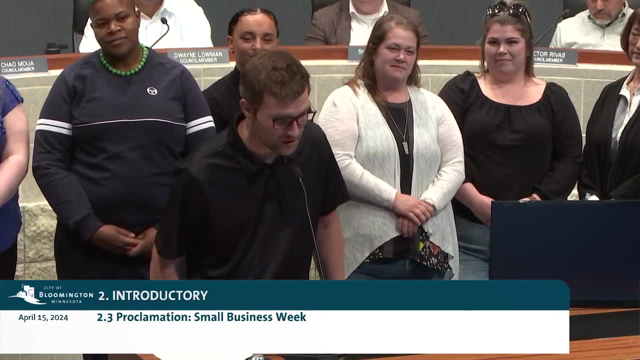 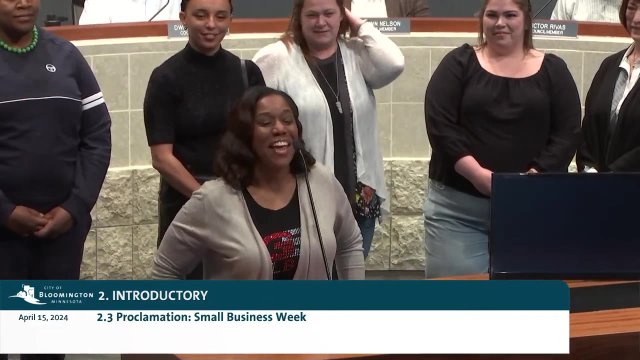 really quick. Hello, my name is Patty Morton, My business is SMB Secured Solutions and my website is SMB Secured Solutions, And my website is SMB Secured Solutions And my website is SMB Securedcom. Thank you, Hi. I'm Elise Elisa Moore's Organic Cafe. I bake vegan desserts. You can find me at my 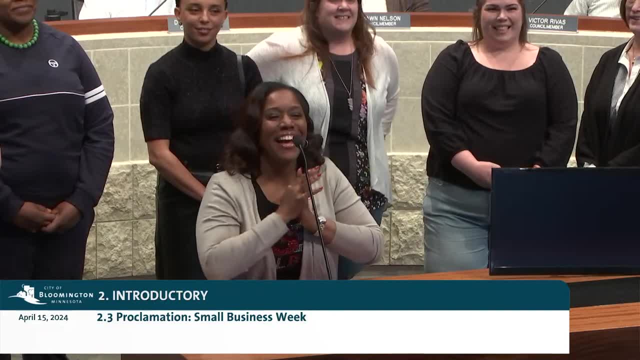 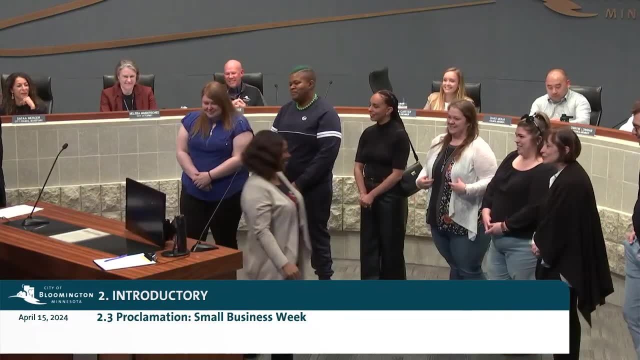 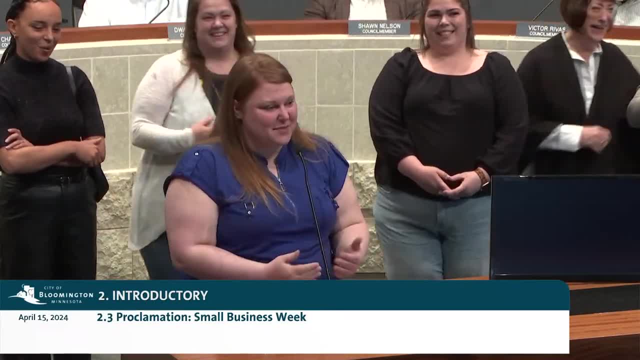 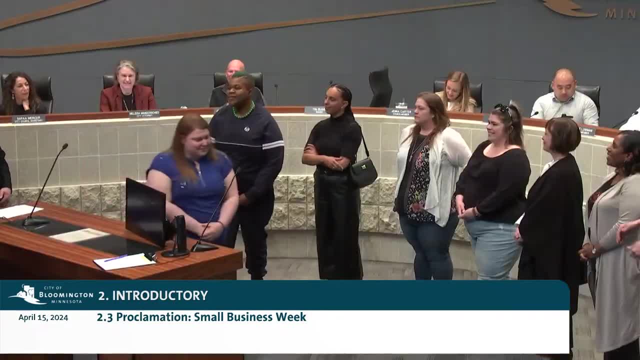 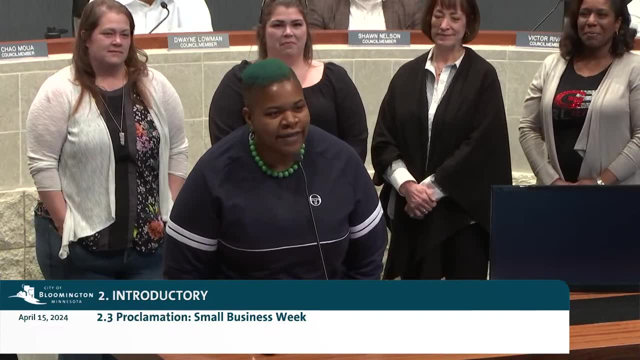 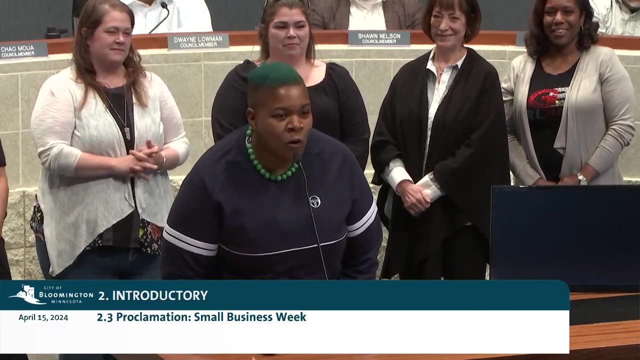 currently vividnervecom Peace. I'm Angela McDowell. I have a civic engagement cohort called LL Cool J, That's Let's Learn Collectively on our life's journey. You can visit us at llcooljorgcom. Thank you. 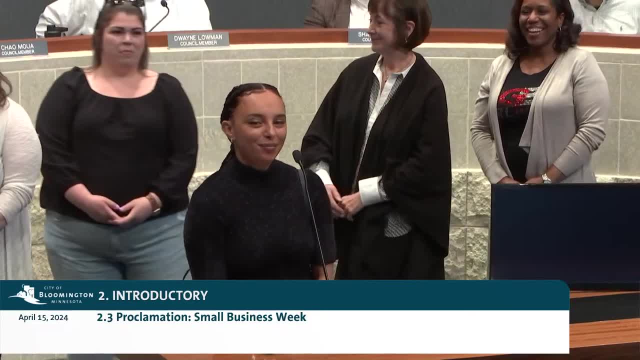 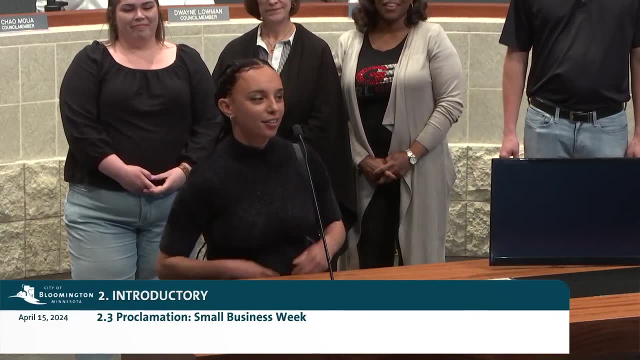 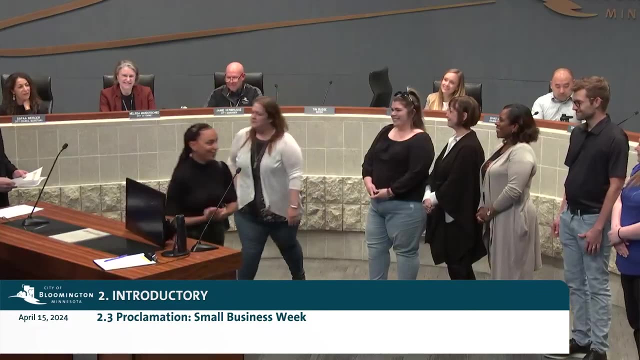 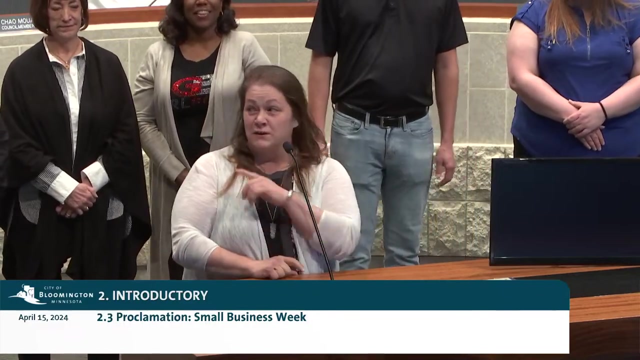 Hi everyone. My name is Rakeek Alam and my business is Nova Medical Supply. The website is novamedicalsupplyus. Hi, I'm Katie Ross. I own the Arts Creative in West Bloomington, where we are cultivating creatives with a purpose. 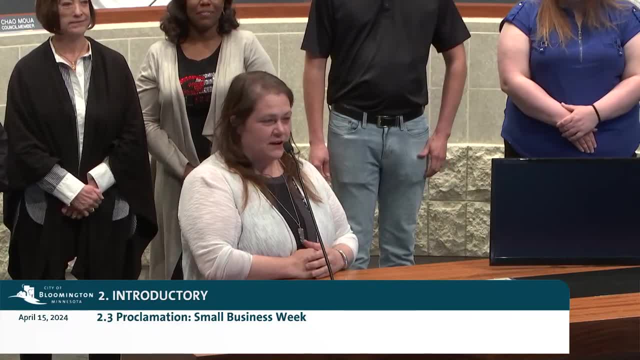 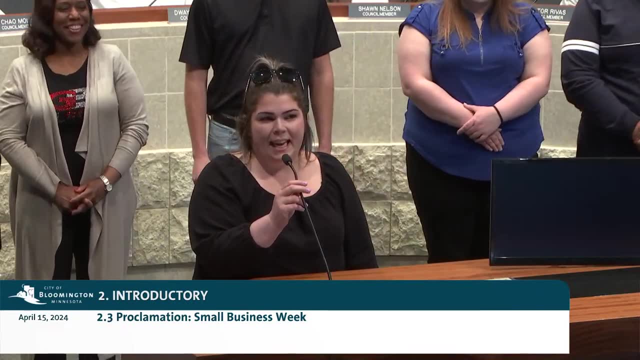 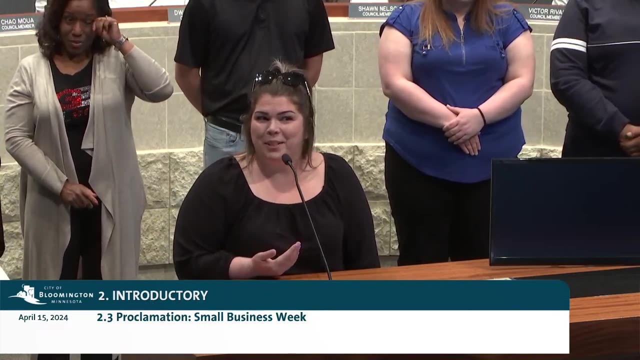 And the website is wwwtheartscreativecom. My name is Sammy Hernandez and I had the pleasure of facilitating this group of people through the CEO Start program, And I am also a business owner. I own Fitzo, which is a plus size active. 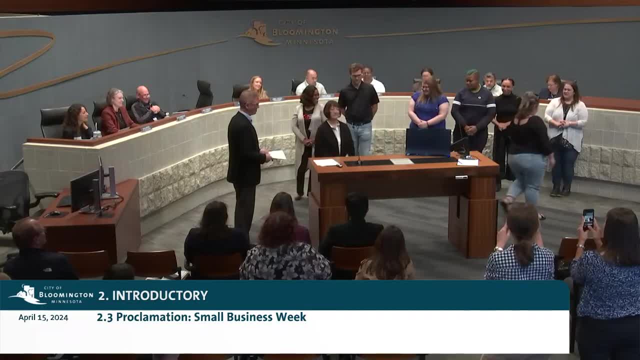 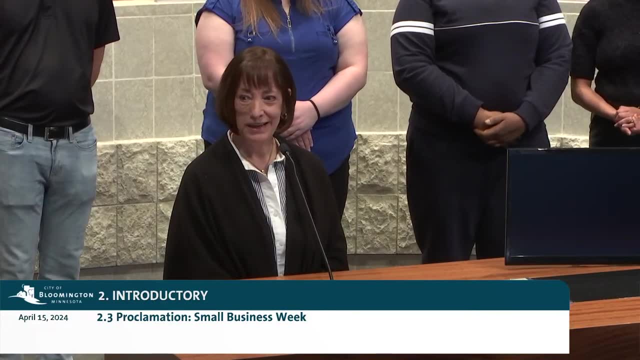 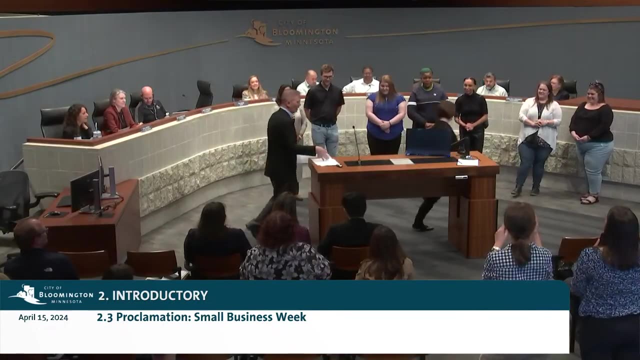 wear company. I'm Tamalyn Pepper. I also had the privilege of facilitating this group And I'm a former business owner. I had a commercial construction company for 12 years which I successfully sold two years ago. I think. to start a business at any time but but right now it takes a lot of guts And 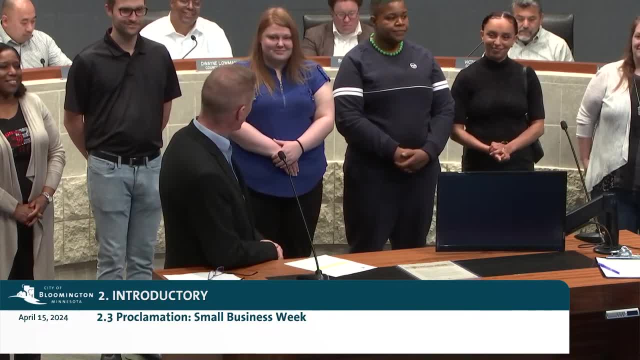 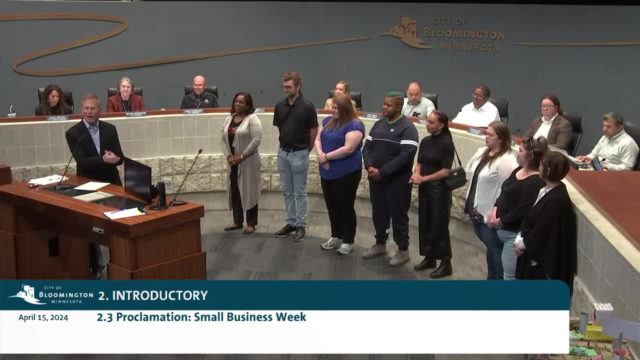 so I said this the other night. I so respect the courage and the fortitude and the drive that these folks have and the guts that they have to move forward. So congratulations. Let's give them a round of applause If you could. 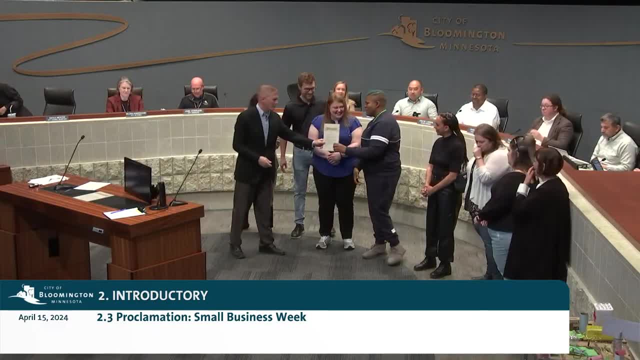 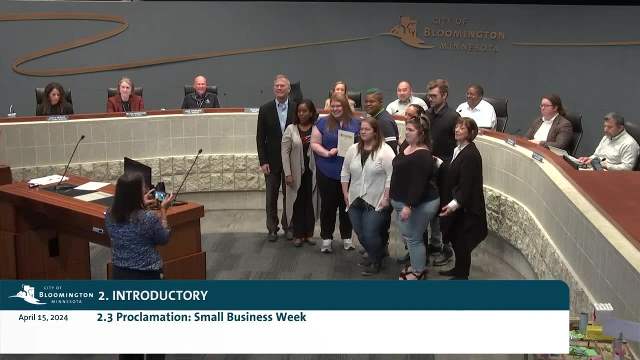 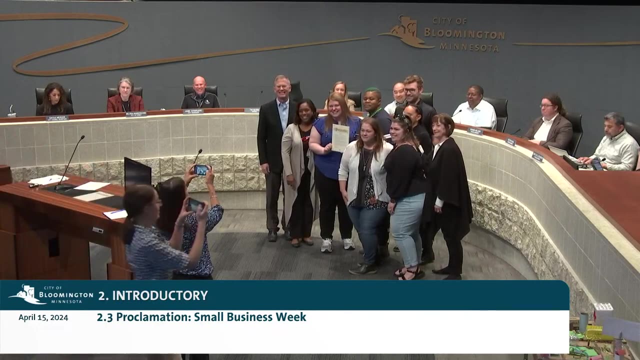 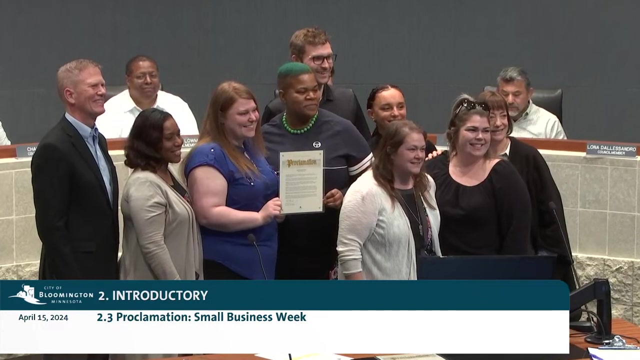 And now we all have to fit into a picture and get the proclamation in there as well. We'll start with Barb. We'll start with Barb, Barb first. Everybody's smiling right. Yes, Three, two, one, Thank you. 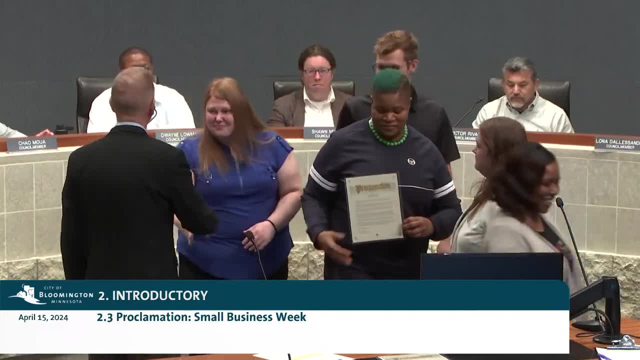 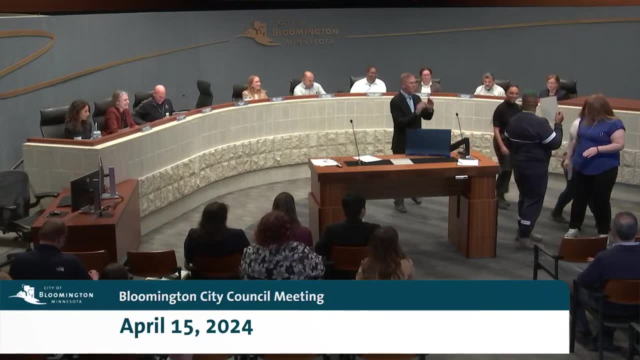 Good work. Thank you for being here tonight. Thank you very much. Thank you for coming. Thank you, Thank you for being here tonight. Thank you, Thank you, Good to see you. Thank you, Thank you, It's yours. 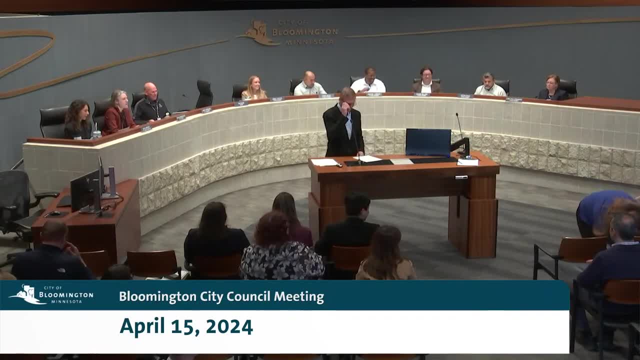 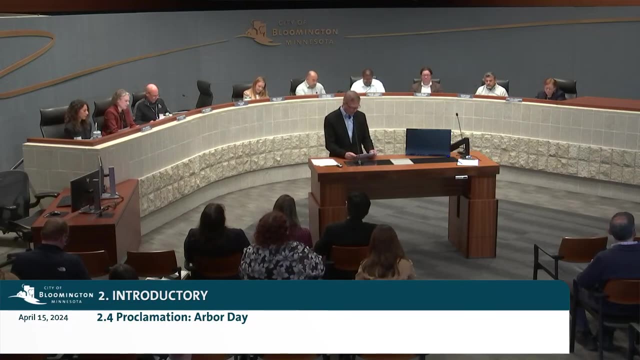 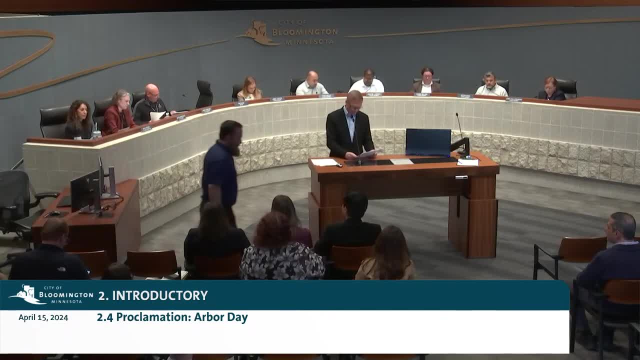 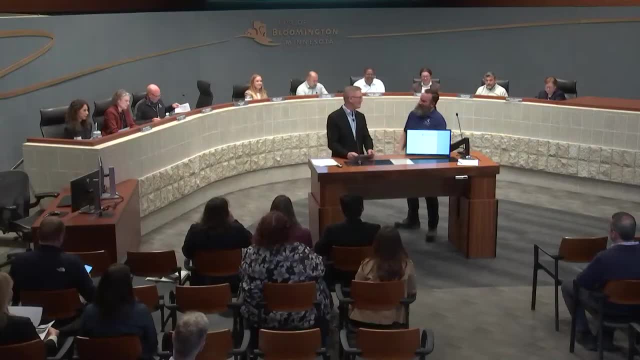 Arbor Day provides an opportunity to celebrate the importance of trees and forests to our economy, culture, history and the future of our state. Dustin, I apologize, Come on up here. I just came up without. You know the drill. You know the drill. 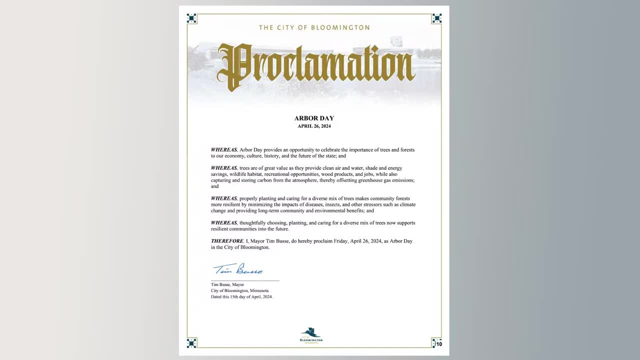 And whereas trees are of great value as they provide clean air and water, shade and energy savings, wildlife habitat, recreational opportunities, wood products and jobs, while also capturing and storing carbon from the atmosphere, thereby offsetting greenhouse gas emissions, And whereas properly. 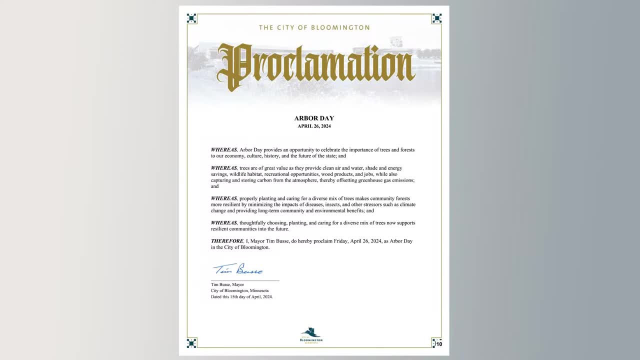 properly planting and caring for a diverse mix of trees makes community forests more resilient by minimizing the impacts of diseases, insects and other stressors such as climate change, and providing long-term community and environmental benefit. And whereas thoughtfully choosing, planting and caring for a diverse mix of trees, 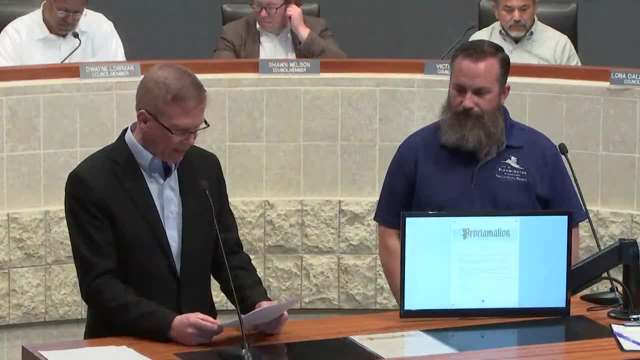 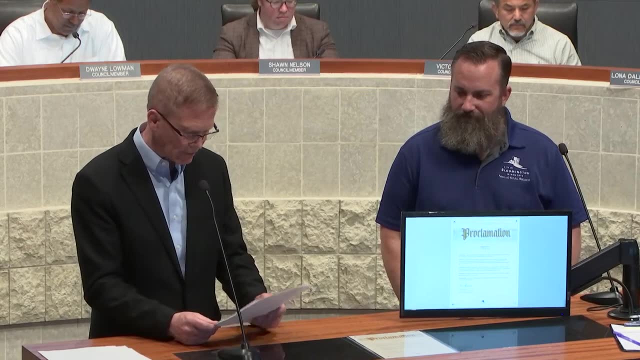 now supports resilient communities into the future. Therefore, now, now, therefore, I, Mayor Tim Bussey, do hereby proclaim Friday April 26, 2024, as Arbor Day in the city of Bloomington, dated this 15th day of April 2024,. 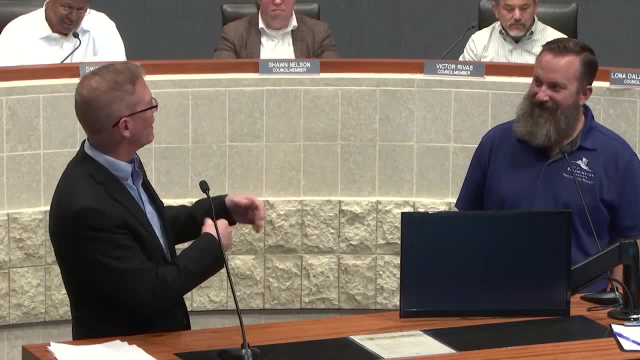 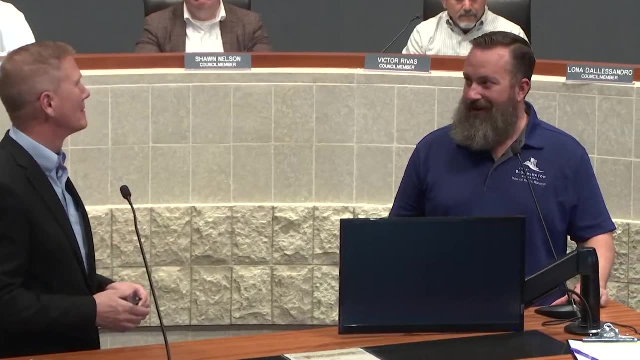 and I will turn the mic over to you and I won't steal the thunder about what else is going to happen on Arbor Day. Well, so we're again doing the tree sale. It was wildly popular this year. Unfortunately, we did run out of trees pretty early. 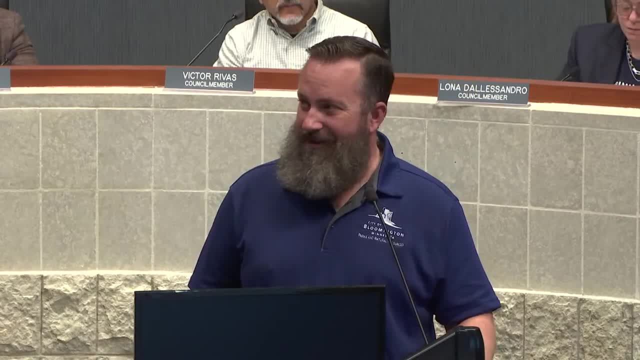 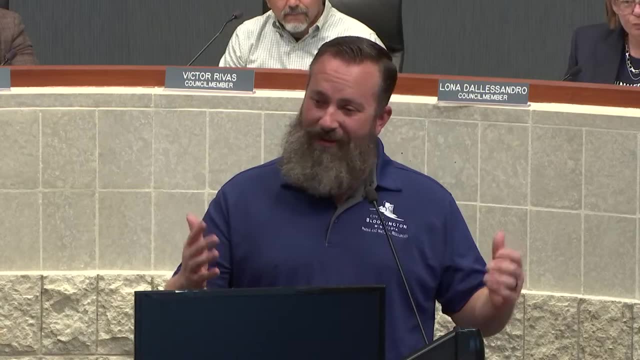 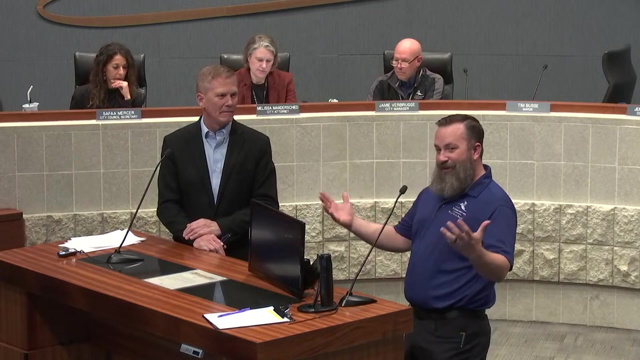 just based on how that sale went, starting in February. So unfortunately, I'm just calling out to all the residents in Bloomington to do what you can and find trees elsewhere as well. So plant trees all through the summer, even though we couldn't supply all of you with new trees. 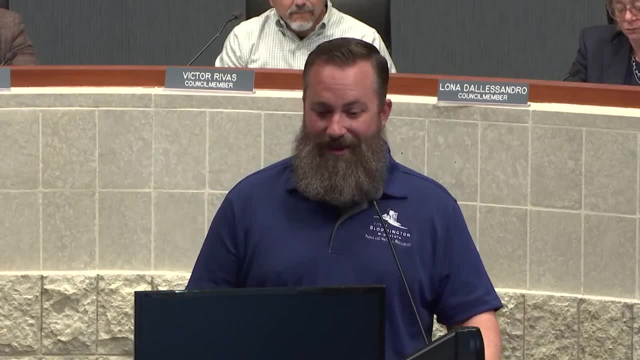 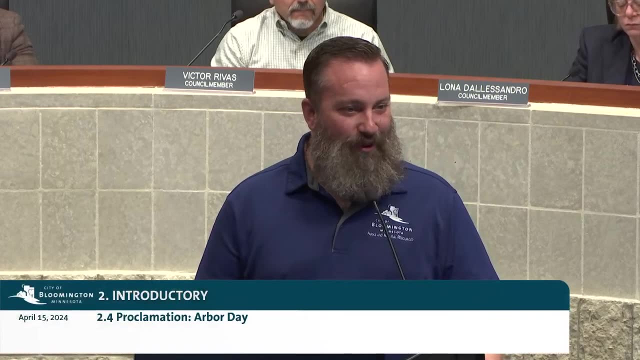 We really have lost a lot of ash in the last- I'd say probably the last five years especially. So just doing what we can to reforest as best we can. And those trees are going to be picked up or delivered on Arbor Day. is that correct? 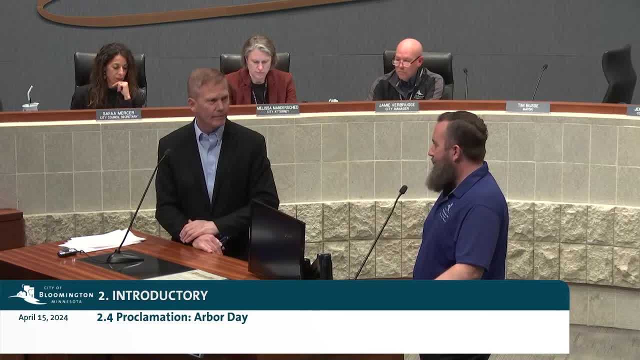 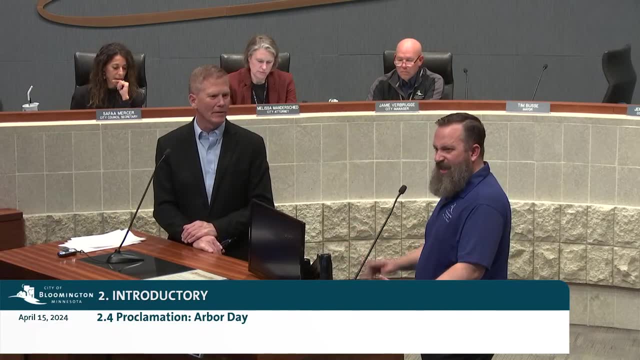 They're going to be actually delivered the following week. The following week, okay, Yep, so that'll be. let's see, we'll pick them up on the 30th and then be delivering them the next two days, kind of after that. 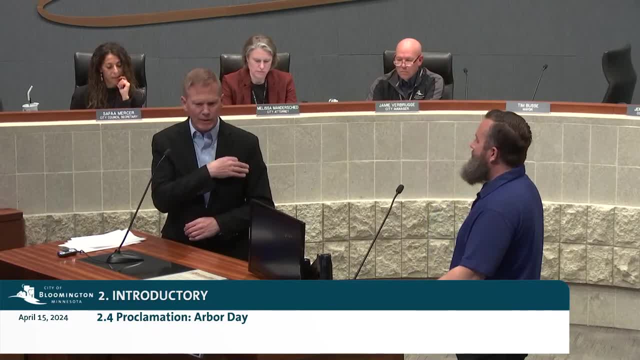 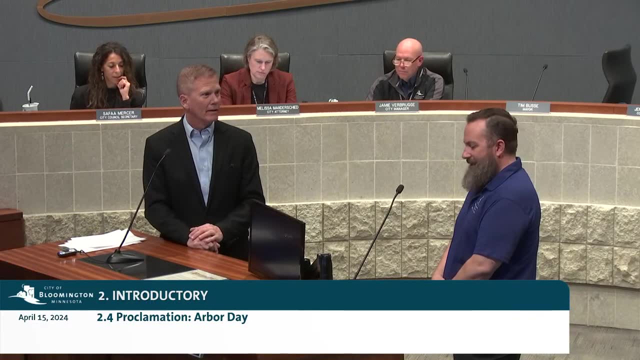 Very good, All right. Well, thank you for being here tonight and thanks for your work. I know it is a big job. That urban forest is important and I know it's under stress right now, And looking forward to where we head next as a community. 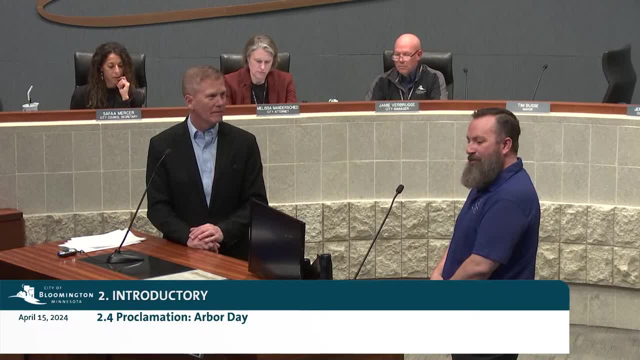 in terms of what's going to be replacing all those ashes that are coming down. Yep, very busy time, Very good, Thank you. Thank you, Hold on. we've got to get a picture If you came up here for the proclamation. 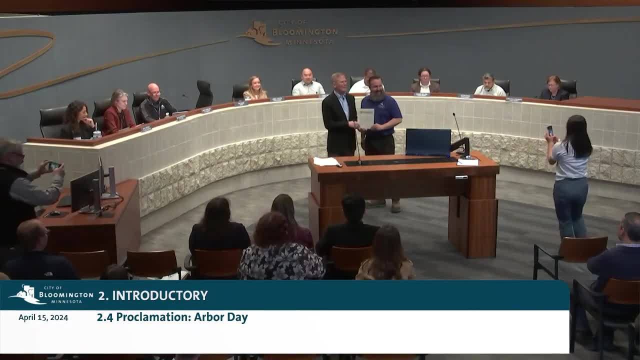 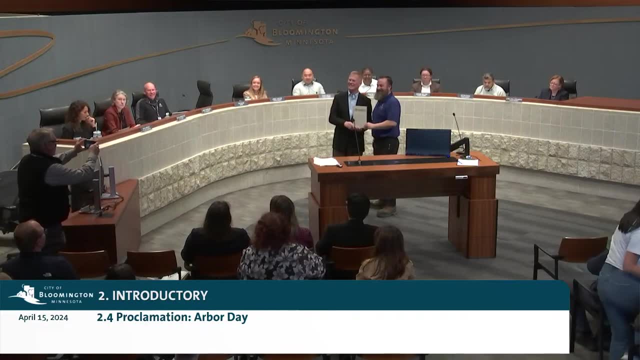 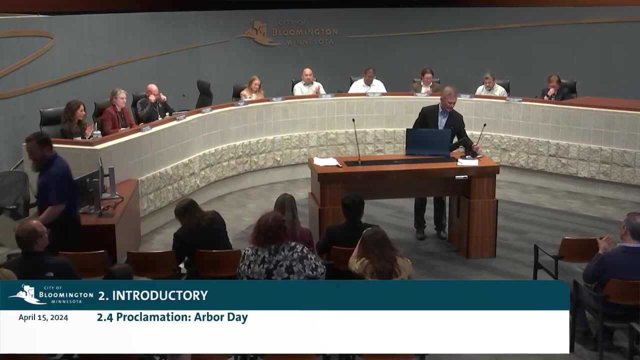 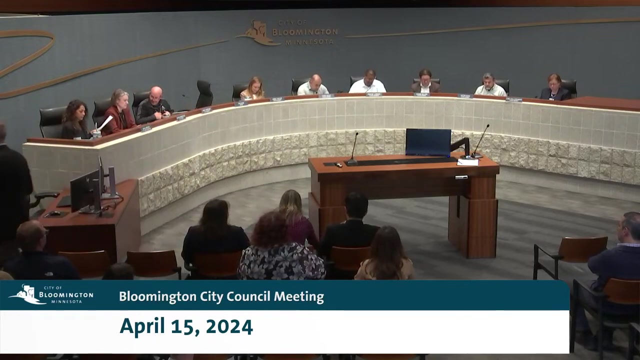 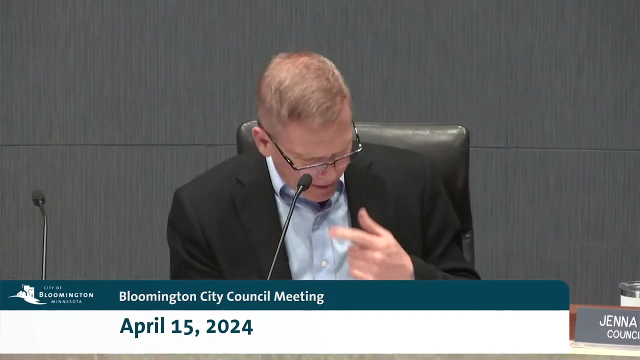 we're going to get a picture. Absolutely, Absolutely. Oh, one more, one more. Thank you. Thanks for being here. Absolutely, Thank you, Thank you. And our final item under our introductory items, we're going to have a presentation. 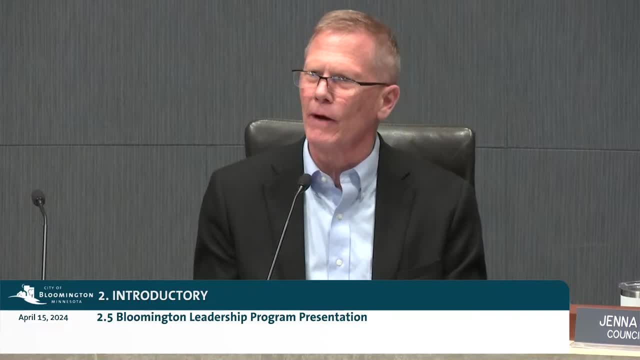 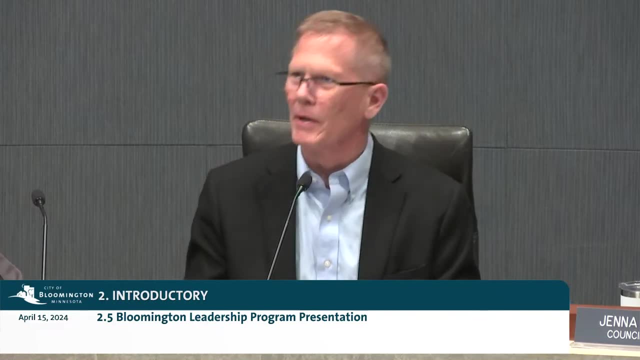 of our Bloomington Leadership Program and the graduates, And rather than try to explain it, I'm just going to turn it over to who's going to speak. There we go. You're all going to speak. That's right, And hold on, I know, Jason Liu. 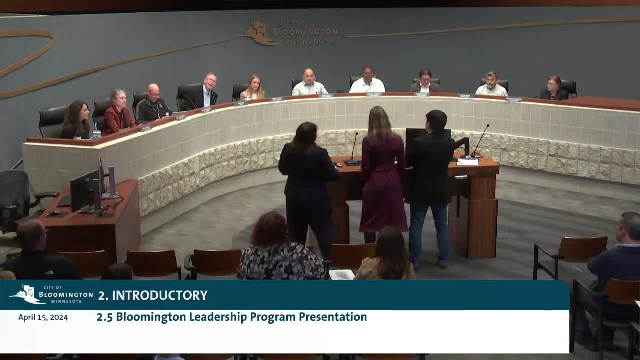 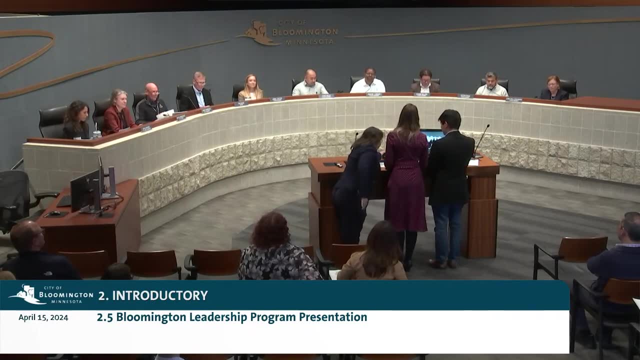 Shanna Swanson and Gina Dabogovic. Am I close enough? Yes, close enough. Okay, thank you, I apologize for that. Good evening all and welcome. Good evening. Good evening, If you could get into the microphone. 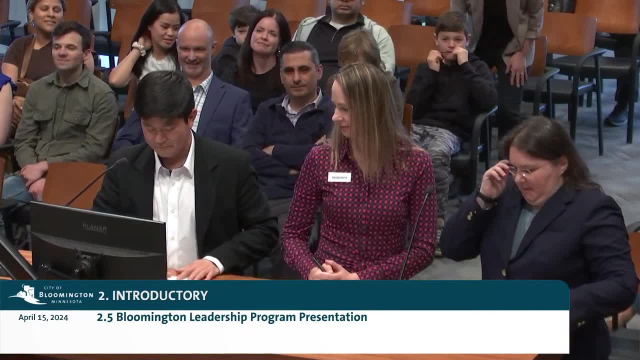 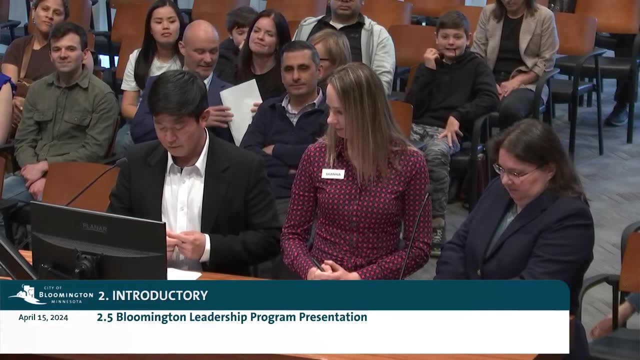 so the folks at home can hear you speak as much as we can hear you, please. Good evening council members and Mary Bussey. I am Jason Liu and I am joined by Shanna Swanson and Gina Dabogovic, as well as other members. 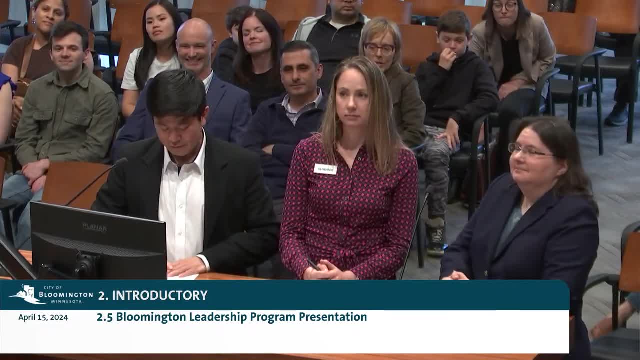 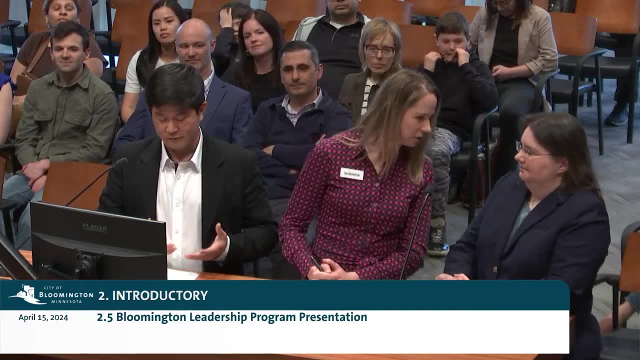 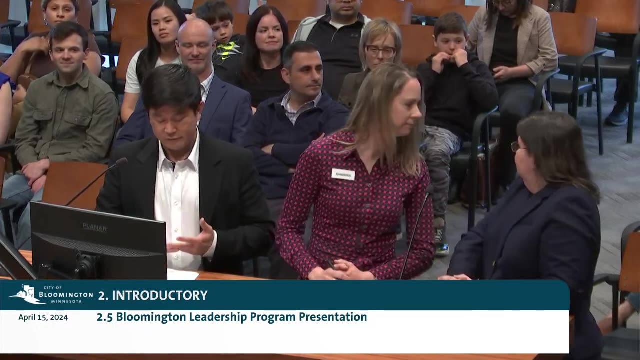 of this year's leadership program behind me. The 2024 Bloomington Leadership Program was designed to enhance civic engagement and leadership skills within the Bloomington community through a series of 10 sessions. It aimed at breaking down barriers, increasing understanding of local government. 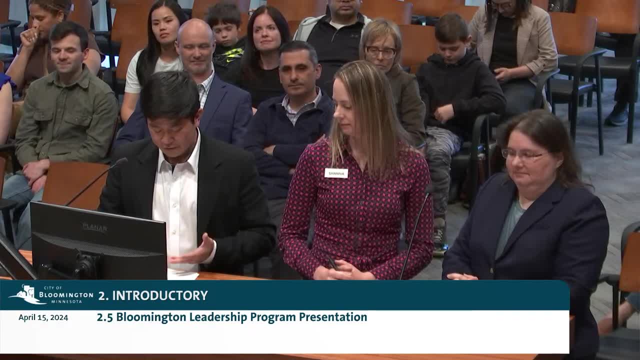 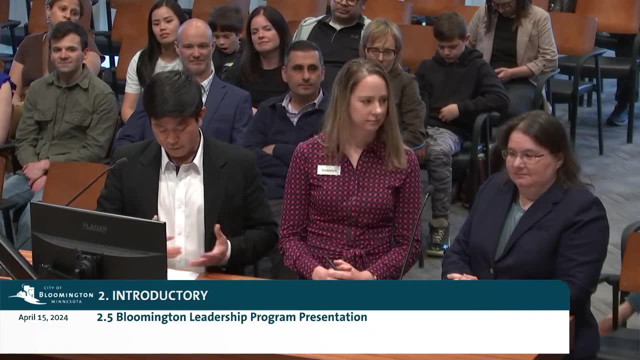 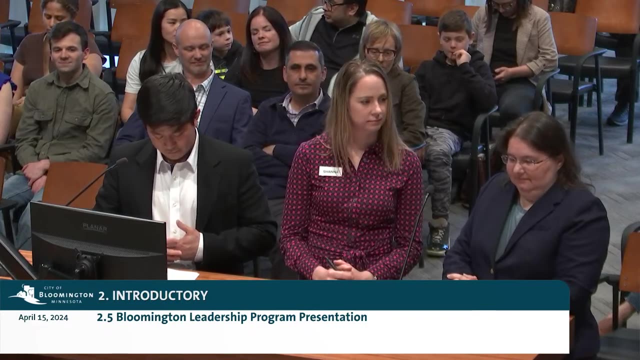 and developing community leaders. The first session was kicked off on February 1st with an overview of an exercise to identify diverse programs, and it ended on March 21st with the final session focused on reflecting on the program's impact in recognizing the leaders it had nurtured. 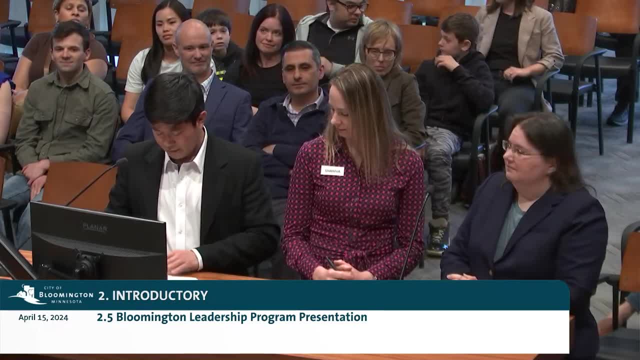 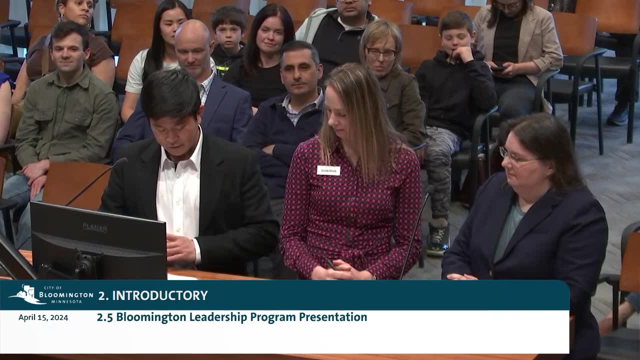 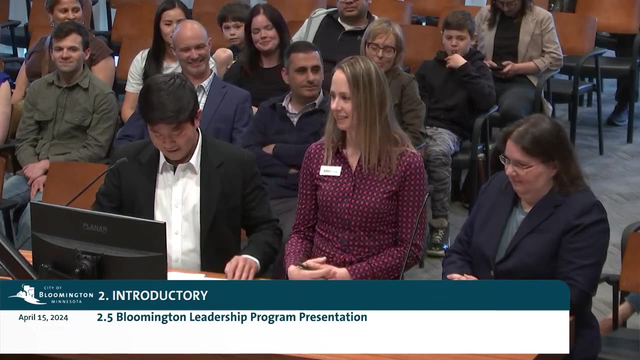 Each session was complemented by engaging activities aimed at fostering connections and insights among participants, And I would be remiss if I didn't mention about all the amazing food that we were treated to at each start of the session. All this was only made possible because of the awesome work. 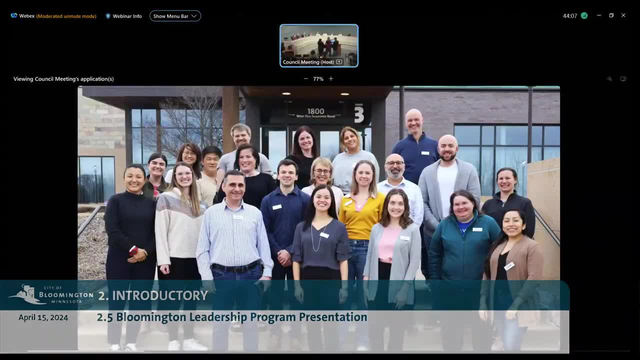 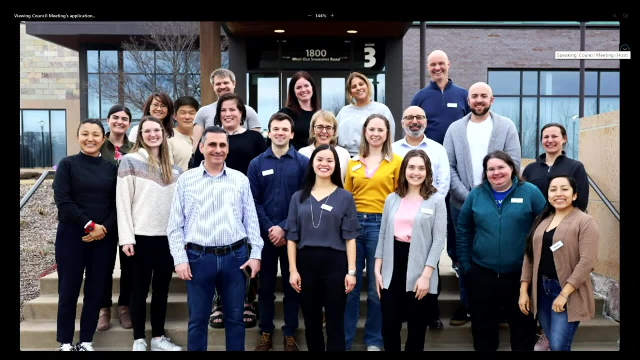 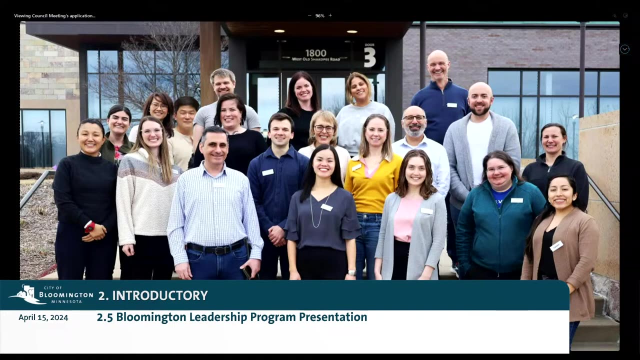 and enthusiastic support from Amanda Crombie and Emily Larson of the Community Outreach and Engagement Team. Next, we would like to provide a few highlights from the program, And the first highlight I wanted to go over is the City Council and Boards and Commissions session. 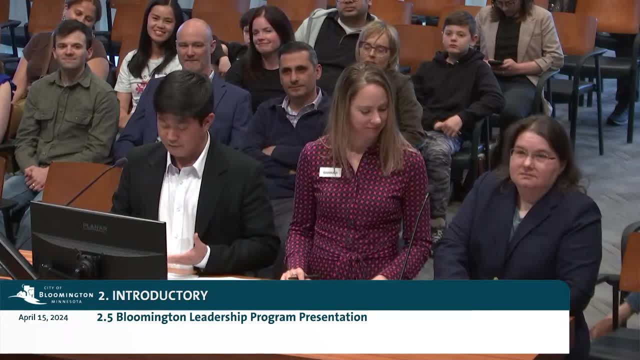 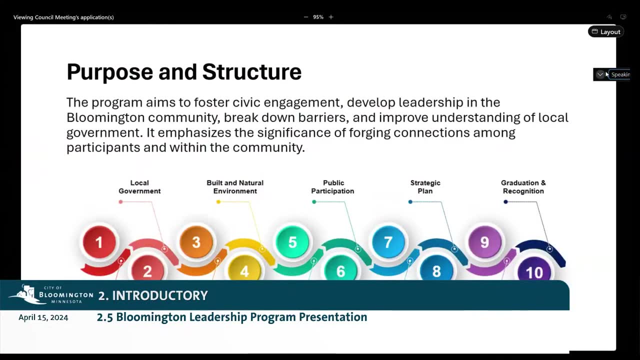 I've always long wanted to be more civically engaged with the community I live in. Being part of the Bloomington Leadership Program helped me widen my perspective on what I can truly make an impact on. This session was called the City Council, Boards and Commissions. 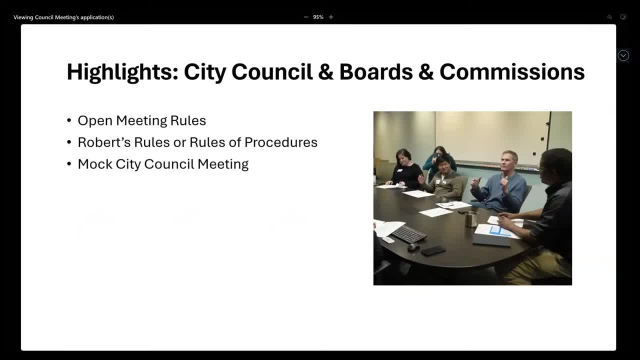 and was truly a highlight for me as we learned about the open meeting law, the talk about the basics and the purpose of the open meeting laws, and also Robert's Rules and Rules and Procedures, And we want to also thank Melissa Manderscheidt. 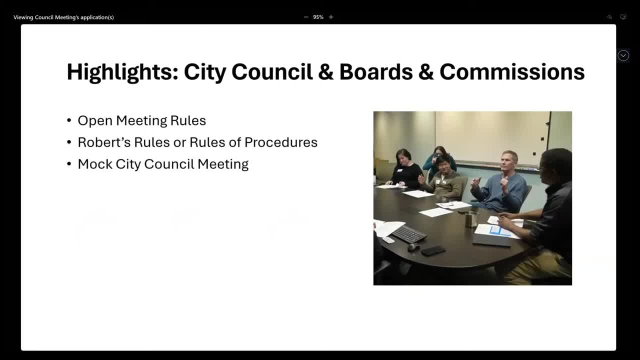 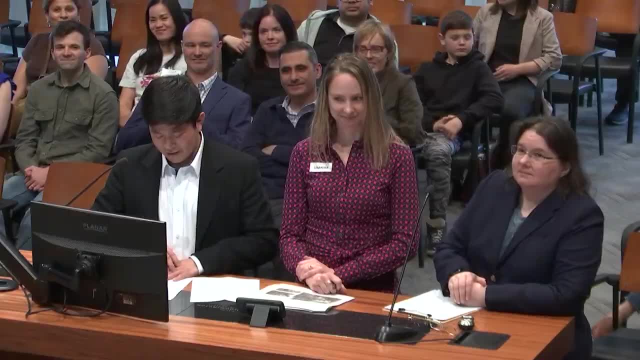 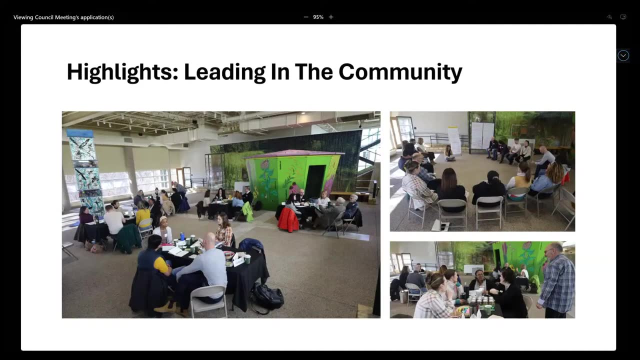 for helping educate us and explain to us the open meeting law and the Robert's Rules. And at the end of that session we also had a mock city session. Not only was that a fun exercise, but it informed me that it's not really. 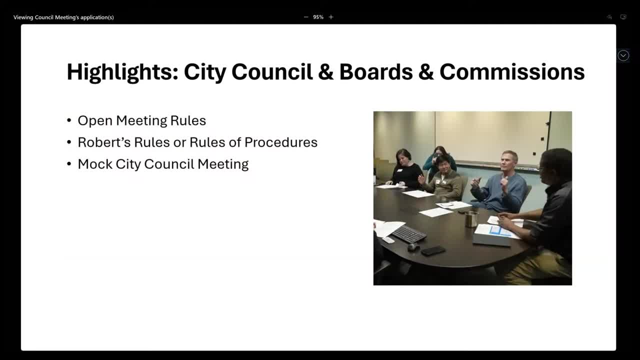 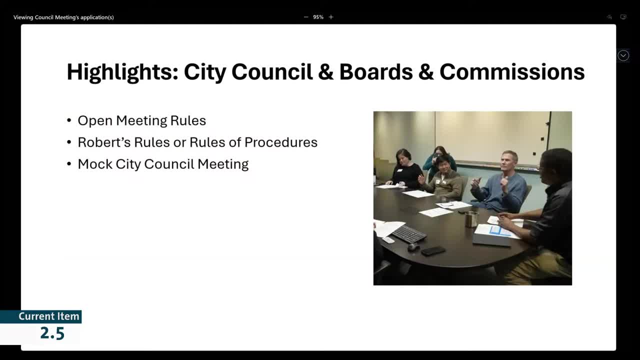 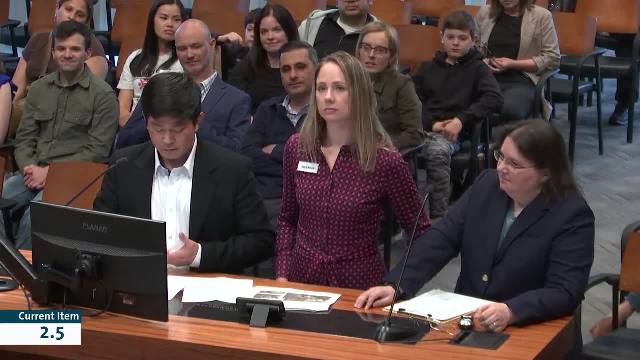 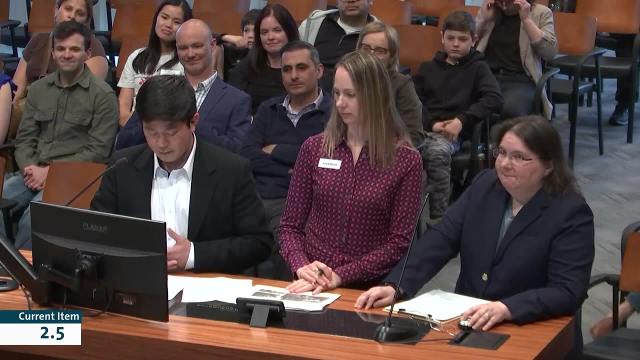 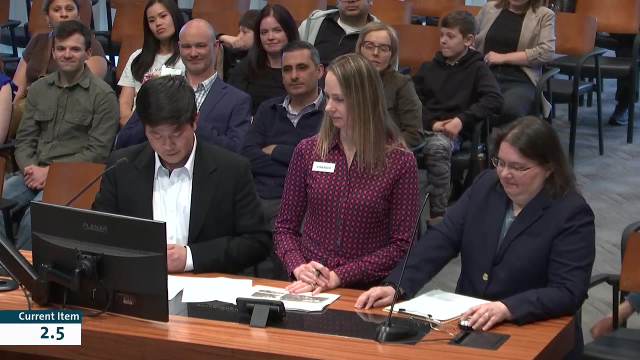 to serve my community by being a part of the city boards and commissions and beyond that, So there's definitely a unique opportunity here for me to play an important role in bringing the city forward to becoming that ideal city that we all love. So next, Gina is going to present the second highlights for the program. 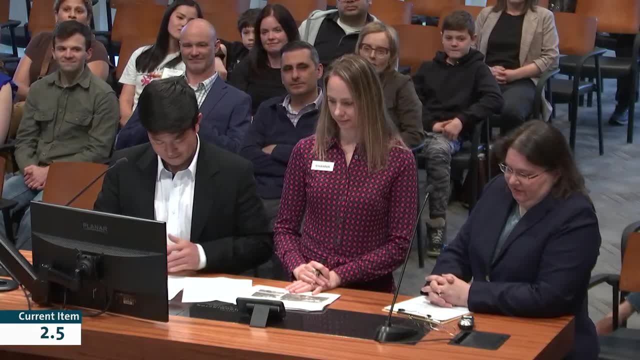 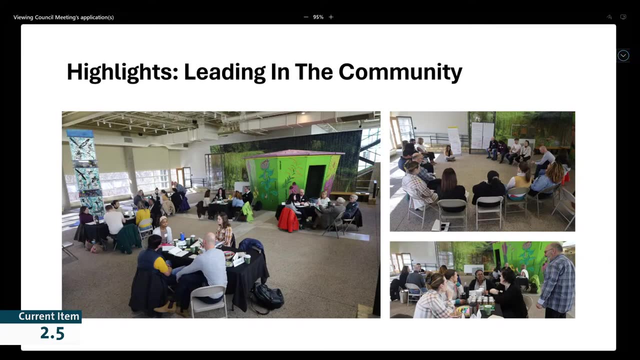 Thank you. During the fifth session of the program, our group visited the Minnesota Valley National Wildlife Refuge. This session was highly informative and engaging, as we were presented with a series of presentations from local nonprofits. Throughout this session, we gained valuable knowledge about the missions of these organizations, their beneficiaries. 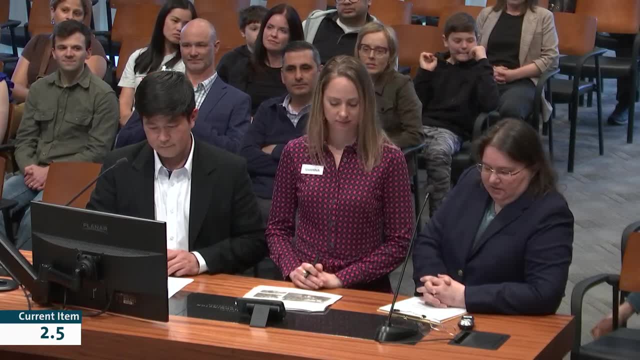 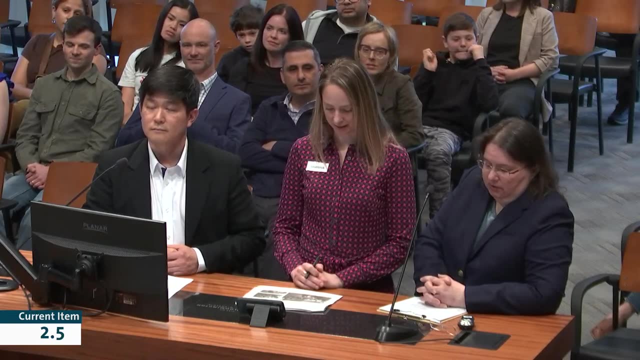 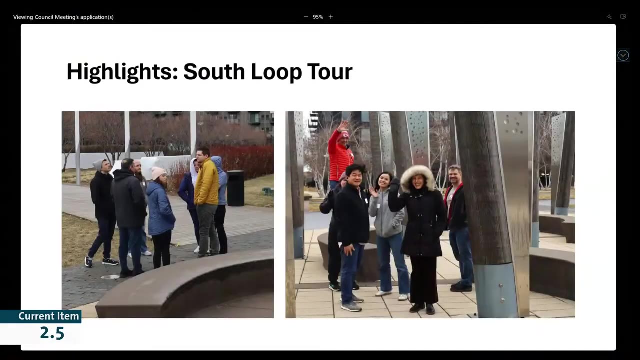 the volunteering opportunities that each organization offered. This experience not only broadened our awareness of the critical work in our community, but also highlighted ways in which we could all contribute and get involved. A highlight for me was a tour of the South Loop, where we got to see the old Cedar Avenue. 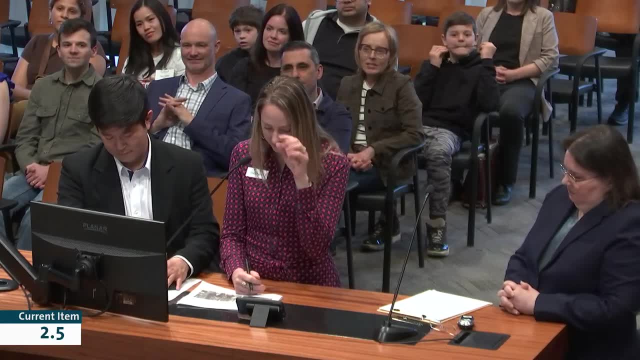 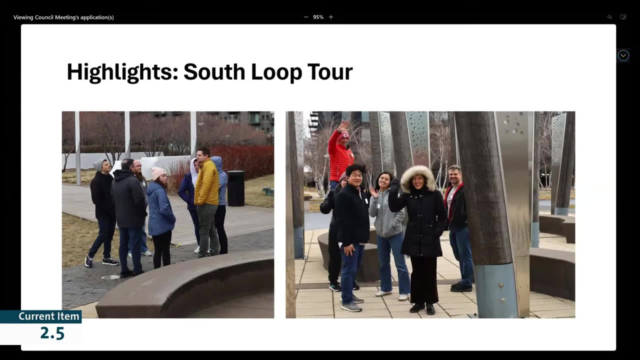 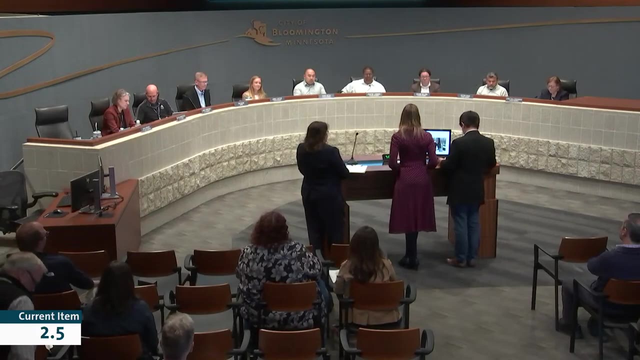 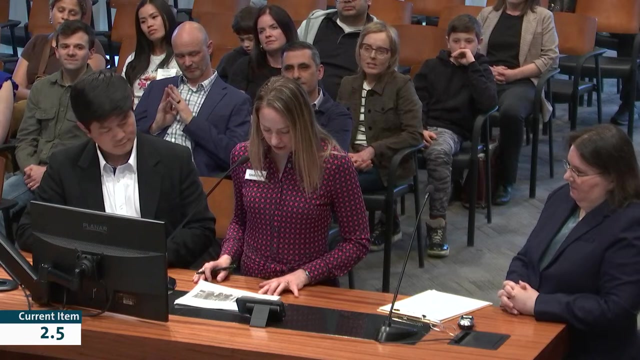 Bridge, the Nature Play area, check out some murals, Bloomington Park, Central Station, and we even got coffee at the park. We enjoyed talking to Phil, the redevelopment commissioner, and deeply reflecting on the types of businesses and organizations we aspire to attract as a city, as well as strategies. 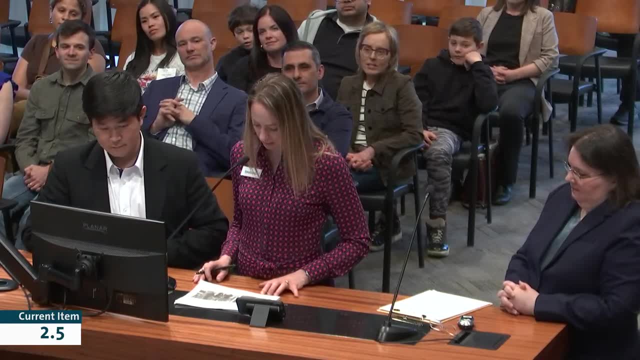 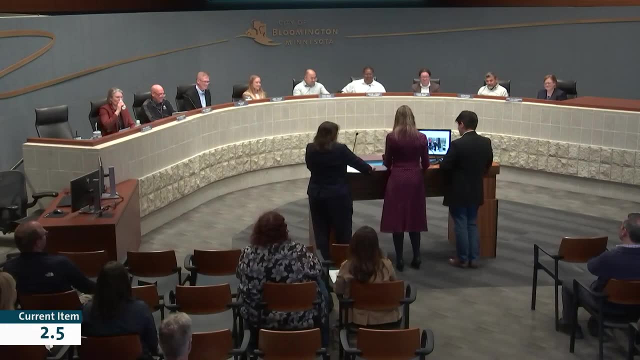 for equitable housing, public art placement and green spaces. Like I had no idea, Bloomington had a central park Next, please. Throughout the session, we had a lot of fun. We had a lot of fun. We had a lot of fun. 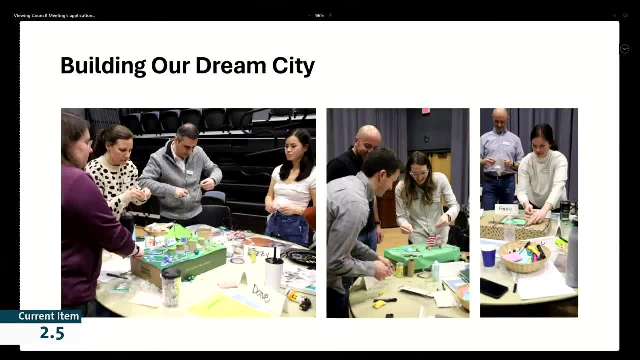 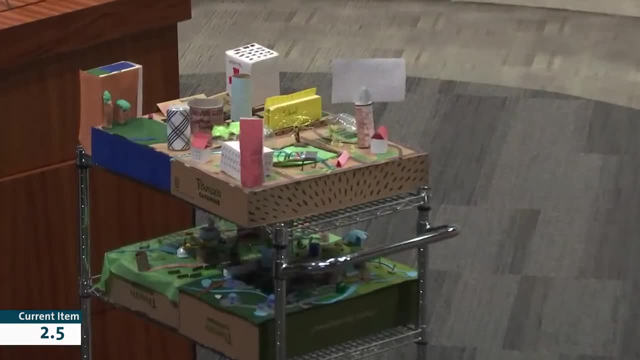 Throughout the course we had opportunities to create and build our own ideal model cities that Gina's gonna show you. We even had some names of Bloomfield and other different names. We had chances to engage in lively debates, thoughtful contemplation, collaborative discussions. 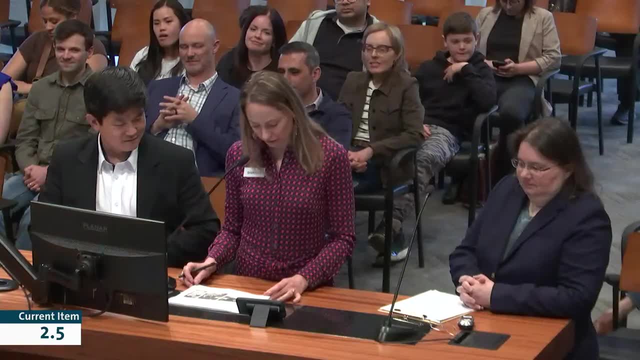 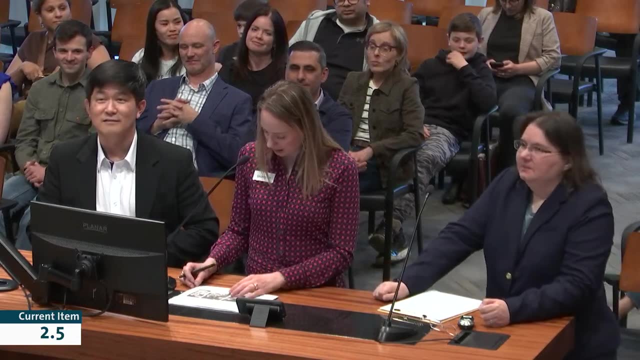 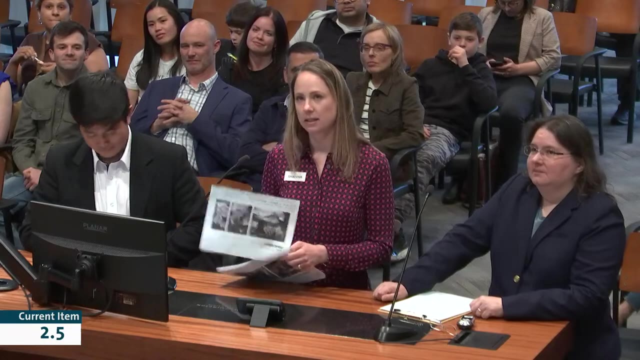 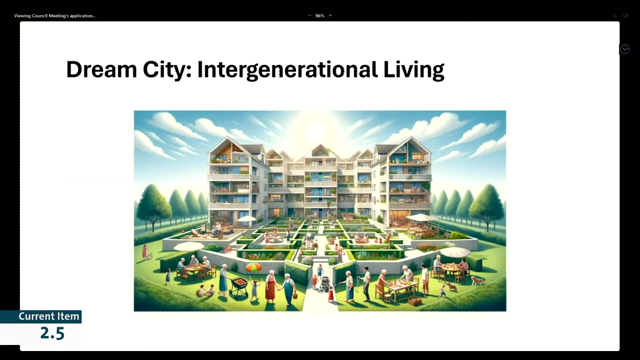 envisioning our ideal and dream cities. Therefore, we'd like to take a moment for the city council to consider our suggestions for a Movington Bloomington Forward, with three common themes that emerged from our class. The first one is intergenerational living, With one in four adults in Minnesota 65 plus. 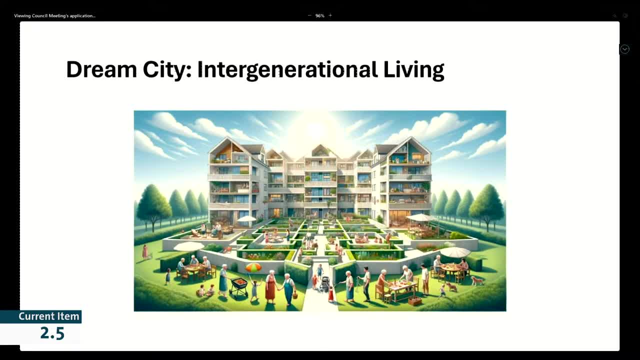 by the year 2030,. we thought it was important to focus on cities that have intergenerational housing, Intergenerational activities, like more pickleball courts, focus on connectivity, green spaces, sustainable living and accessible opportunities for all ages, backgrounds and abilities. 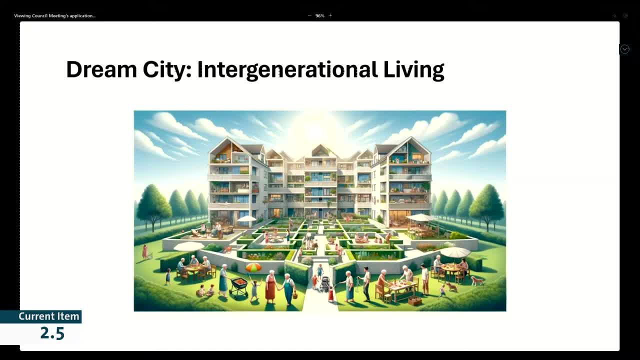 According to the Minnesota Leadership Council on Aging, age-friendly communities enables all residents to thrive at every age and stage of life. Age-friendly communities are well-prepared to meet the needs of their residents now and for future generations. Next, Jason is going to discuss another characteristic of our dream cities. 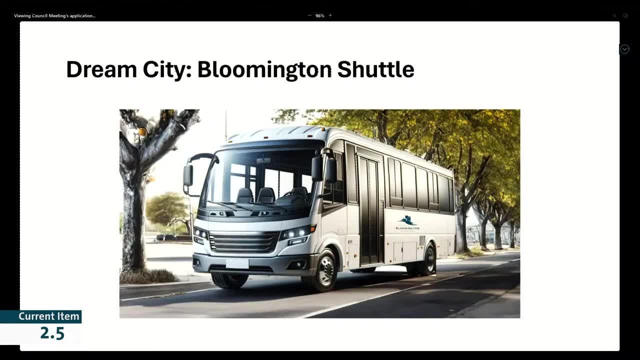 And that characteristic is a Bloomington shuttle or trolley. What this would create is to create a better mobility and connectivity for our residents, And also it can promote change. It promotes commerce and a sense of community for the residents. here- And Gina will present the last element- 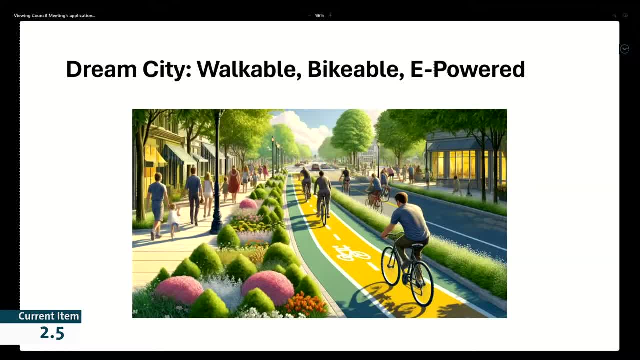 Another common component in our dream cities was a focus on embracing walkability, bikeability and e-powered transportation. Walkability isn't just about putting sidewalks everywhere. It's about creating a connected, accessible and vibrant community. It's about safe crossings. 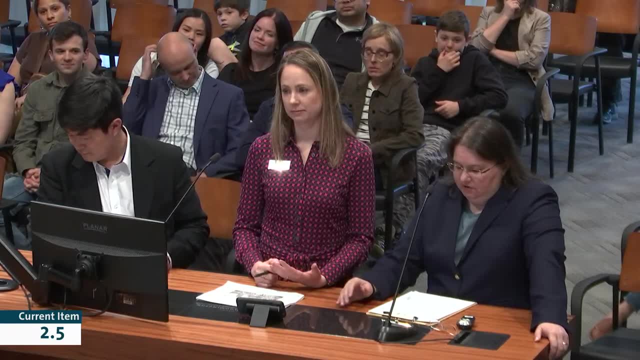 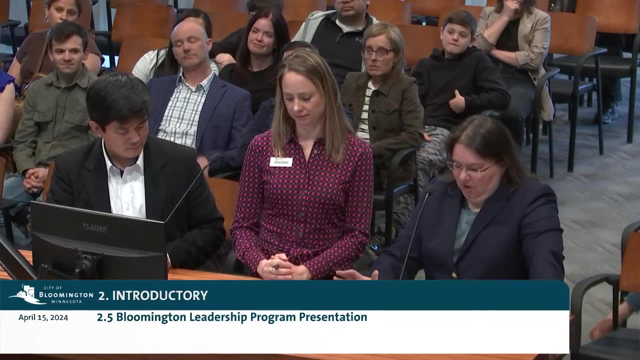 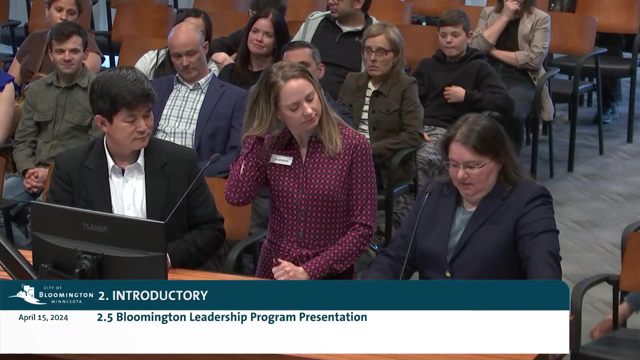 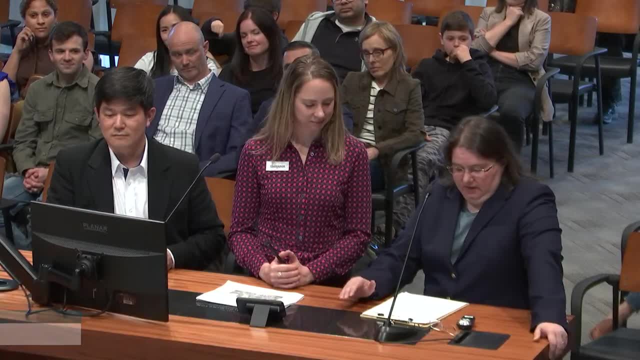 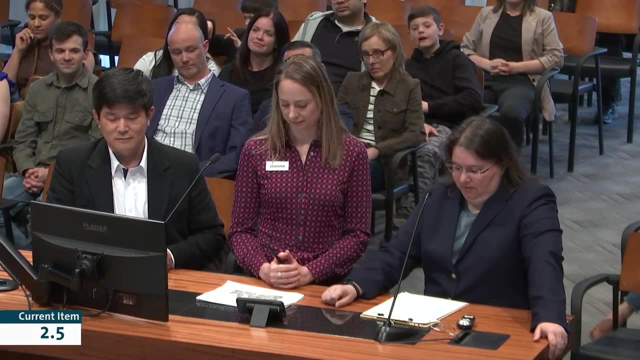 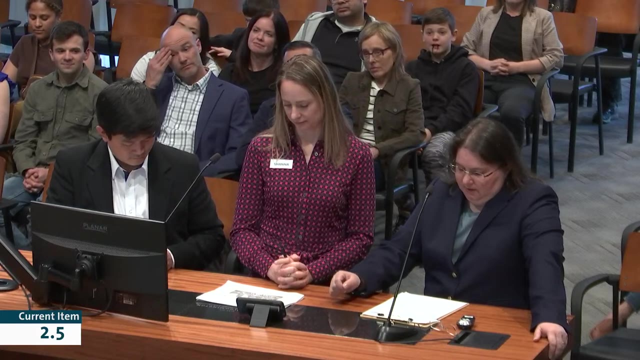 Cut carbon emissions and support both physical and mental health. Finally, the push towards e-powered transportation is a crucial step towards sustainability. This encompasses not only electric cars, but also scooters, buses and municipal vehicles. By investing in charging stations, we can significantly cut down our carbon footprint. 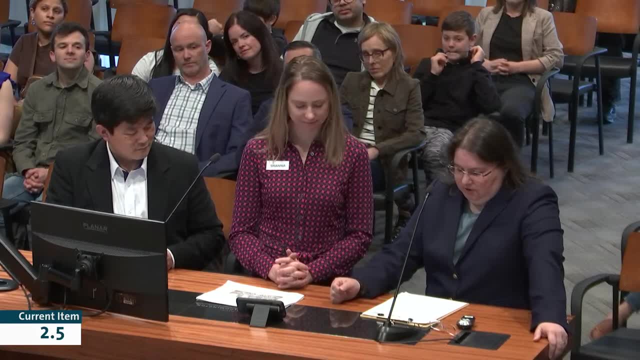 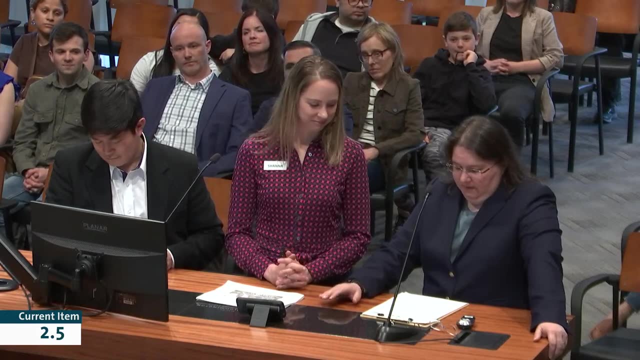 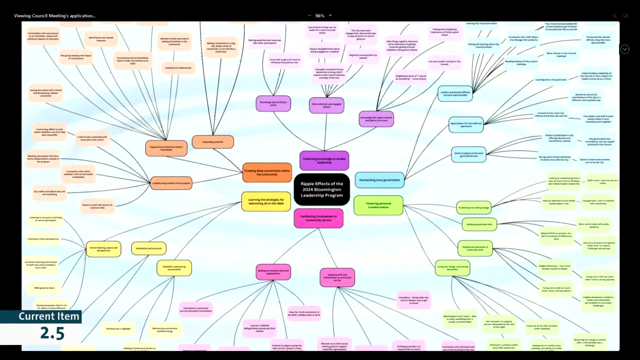 Moreover, transitioning our public transportation to electric power could revolutionize how residents and visitors move around Bloomington, making our city a leader in environmental stewardship. And lastly, let's talk about the ripples that we are all making throughout the community. 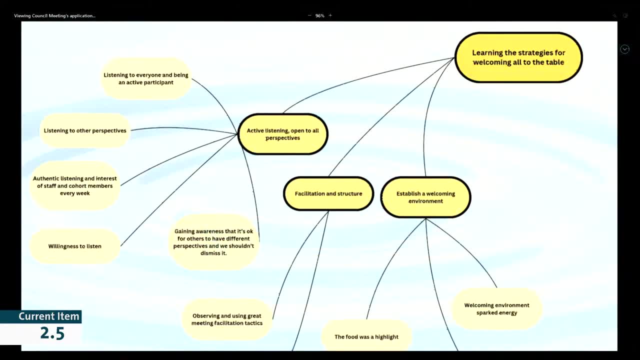 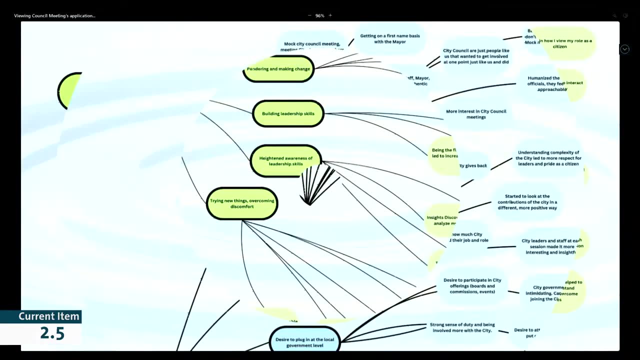 In our last session, we documented what we had learned and we put this into action through these ripples in the community. For example, Tara has already created and leads ToddPod, a nonprofit playgroup for families, and she is now thinking about applying for the planning commission. 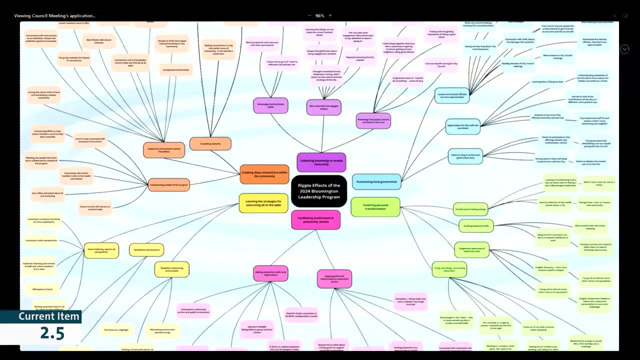 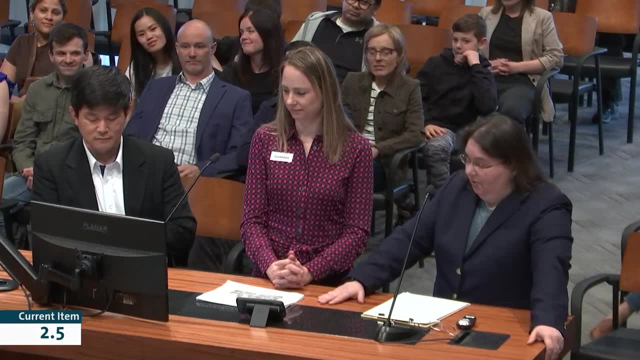 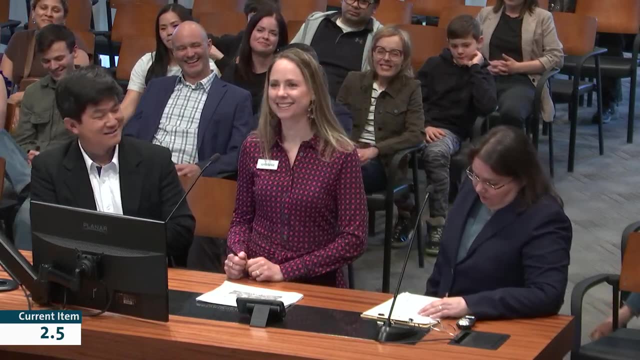 Gina serves as an election judge and tunes into city council meetings live streams and stays updated on Bloomington information and plans to volunteer for Oasis for Youth and visit all 97 parks in Bloomington. Karen is now working with the city to hopefully curtail the 4th of July fireworks litter. 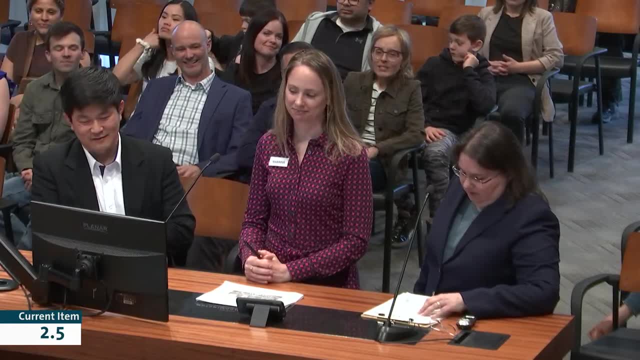 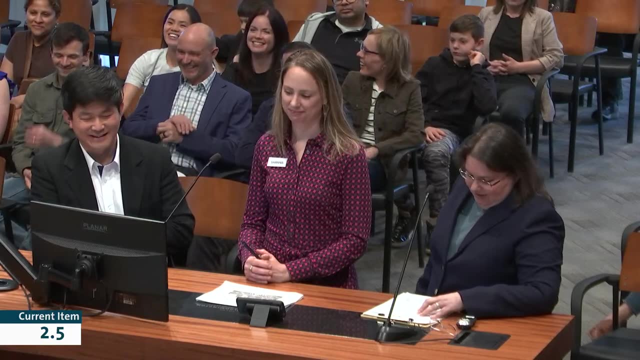 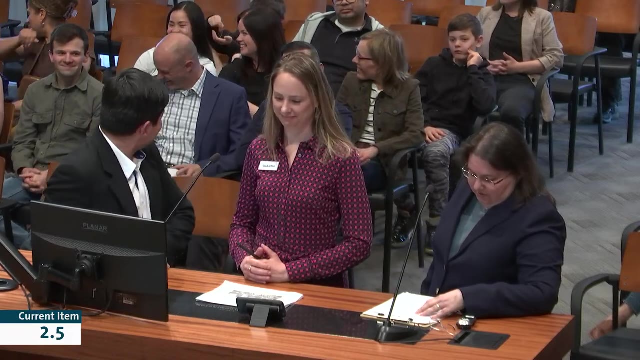 on the old Cedar Bridge and is also thinking about serving on a commission. Kat is building a free little library which will also include dog treats, and she will be planting a sustainable garden this spring. Luke continues to make salsa and pickles and distributes them. 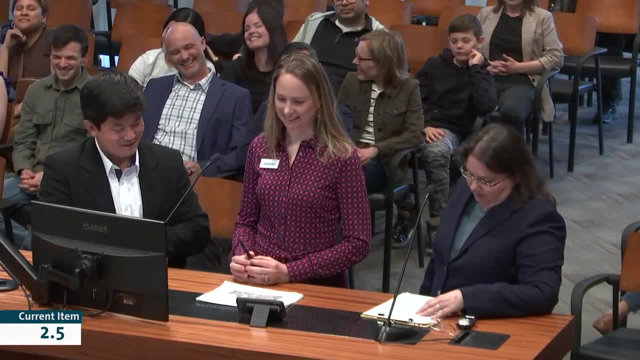 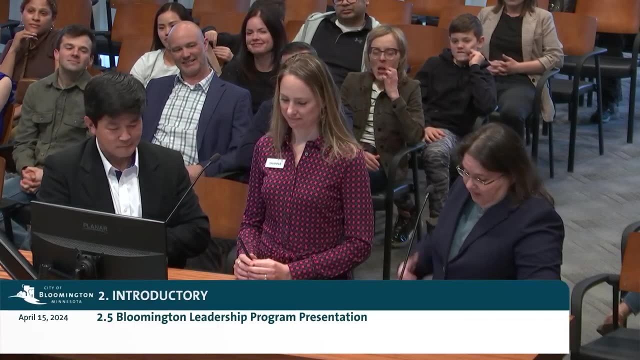 to 35 households in his neighborhood. He is also helping a neighbor till her garden and continues to pick up trash on his nightly walks, something I think we all do- And this year I have dedicated myself to doing 100 acts of kindness, primarily focusing 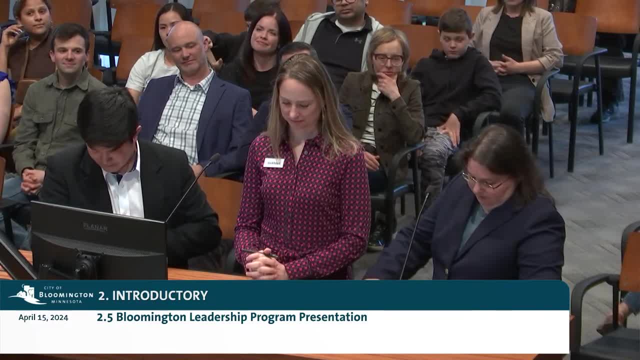 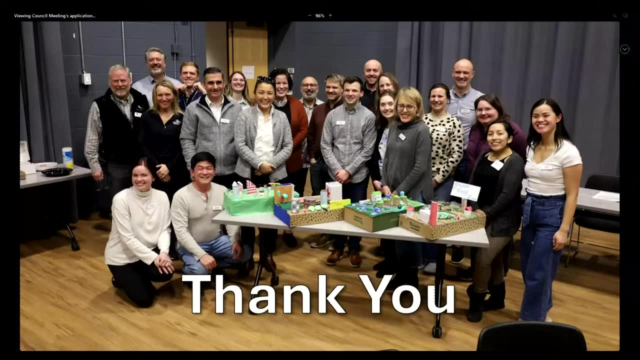 on helping people and helping others. I'm also helping to help people and nonprofits with AI and digital marketing. These are just a few of the ripples. Lastly, we want to say thank you to the leaders of the program, Amanda and Emily. 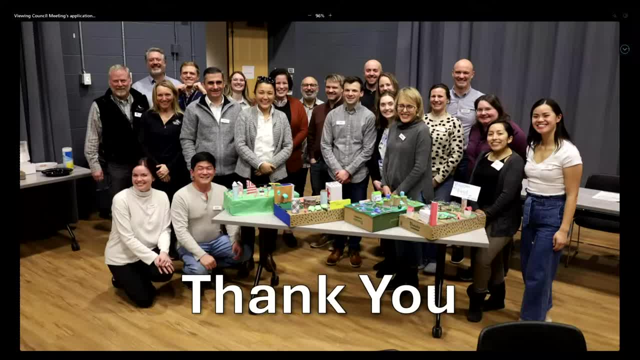 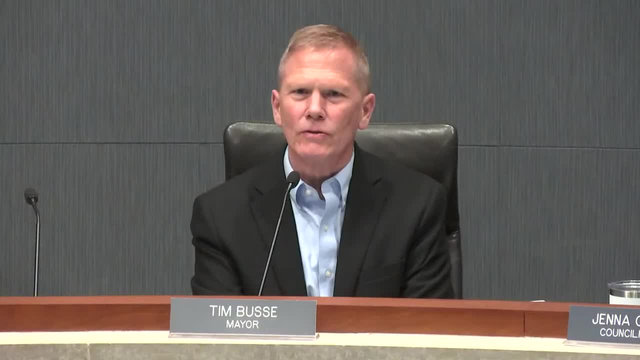 and thank you to Mayor Busey and the council for this amazing opportunity. Thank you so much and we'll take any questions. Thank you for the presentation and congratulations to you all. If you are a member of this cohort, if you could raise your hand just. 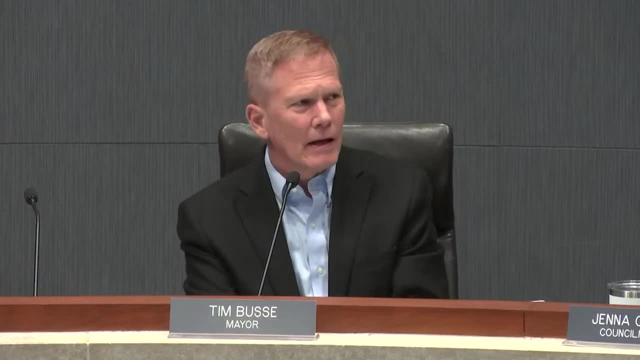 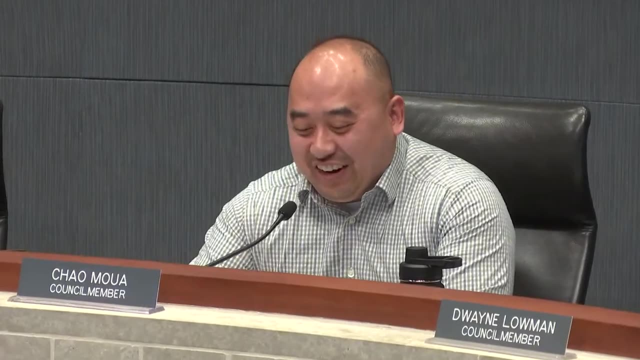 so the council can see everybody who's here. There they all are. Council. do we have any questions? Council Member Moua, why did I know you were going to be first? Yeah Well, thank you, Mayor. I just wanted to say how honored and privileged I was to be able to come. 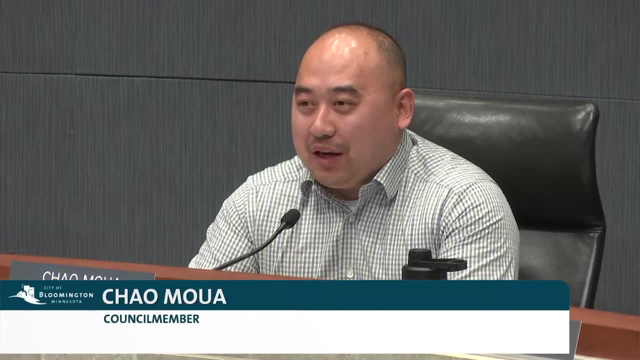 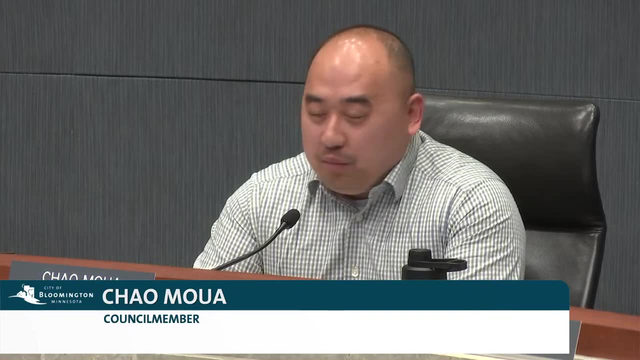 and rejoin your group for one night with the city council mock meetings. It just reminded me how dedicated people are within our city. I think we've all heard people speaking about the city, about how we want to make the community better. but this cohort, this group, 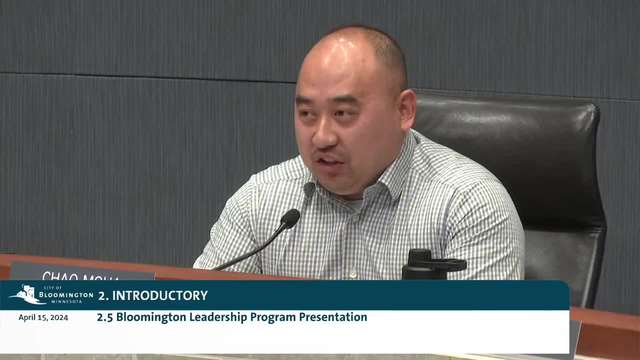 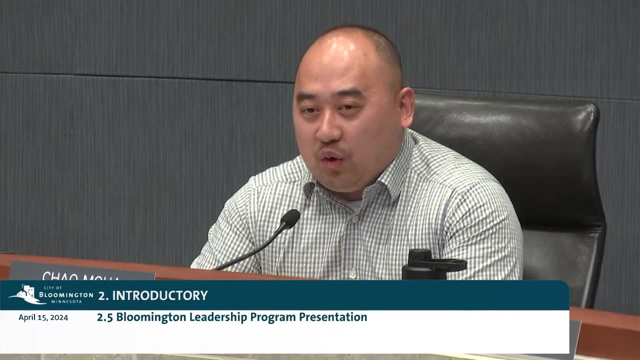 just really represents how people are taking action, and I'm so honored and proud to call you alums now as well, because I know the work, the learnings that you took from this program. you're going to expand and ripple it out into the community. 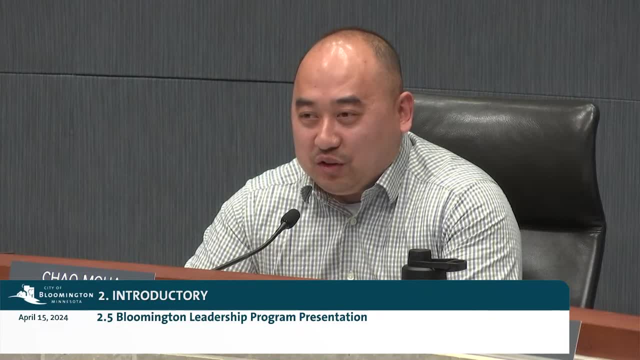 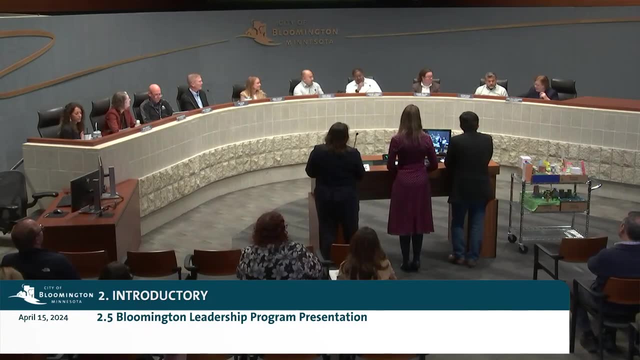 and that's only going to make Bloomington better, and so I'm so excited to see what everyone's going to do. Hopefully we'll see some more folks up here in the future. Council Member D'Alessandro. Thanks, Mr Mayor. 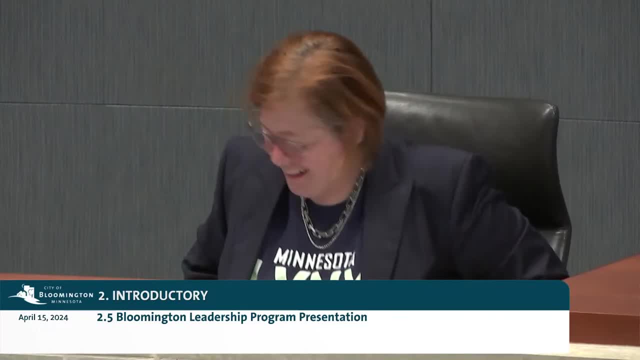 Wow, so coming for your job already? huh, Not mine apparently, right? No, thank you guys so much. 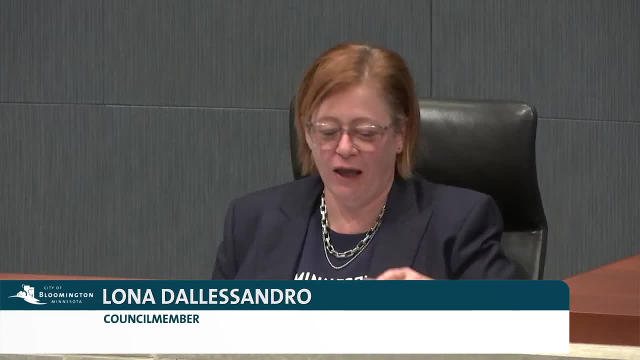 It's great. I think I know at least half a dozen of you, and Gina and you and I got to work together a long time ago, so I'm thrilled to have this group of people involved in planning the future of Bloomington. Your ideas are like you could have written them. I could have been like that's my people. 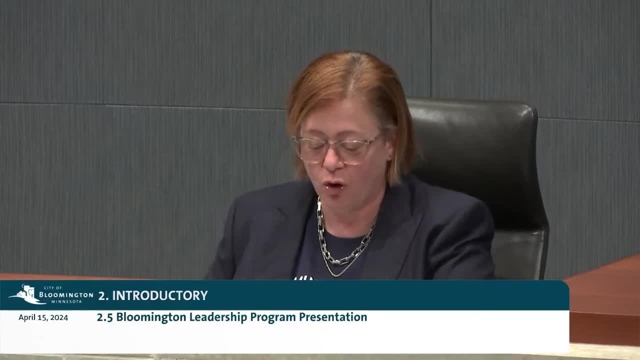 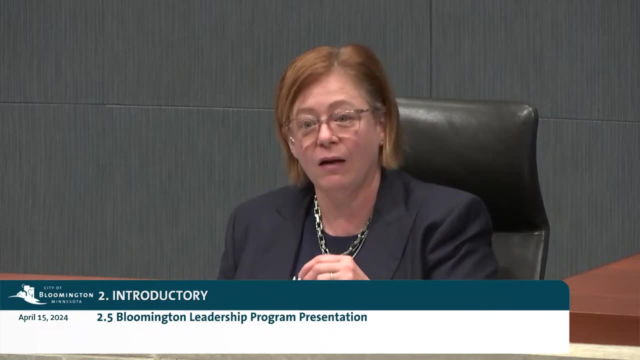 right there. I was so excited to see that. I want you all to know that those ideas are many of them are ideas that are percolating now here, and that means that there's an opportunity for you to continue to advocate for them long. 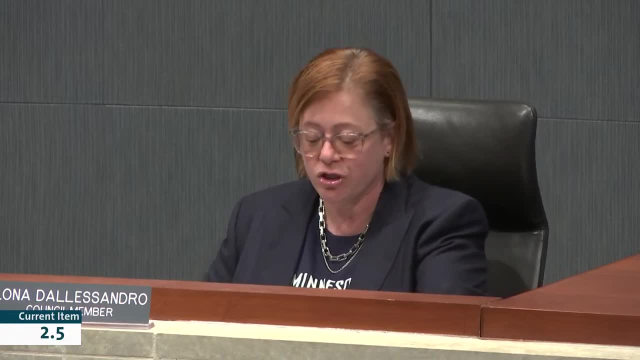 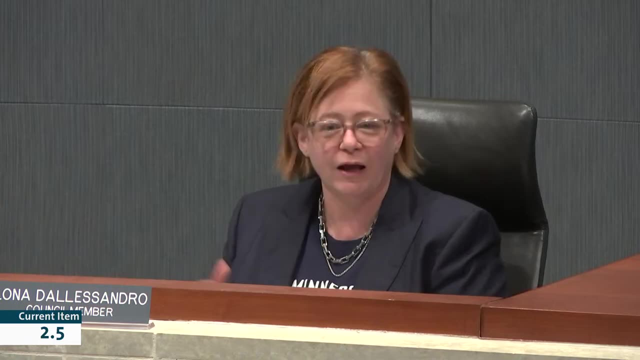 past your time on the Leadership Development Program, So I look forward to having those conversations with you. I don't want to speak for everyone here, but I know that I'm available for coffee anytime. I'm assuming any council member would take you up on that if you wanted to hear more. 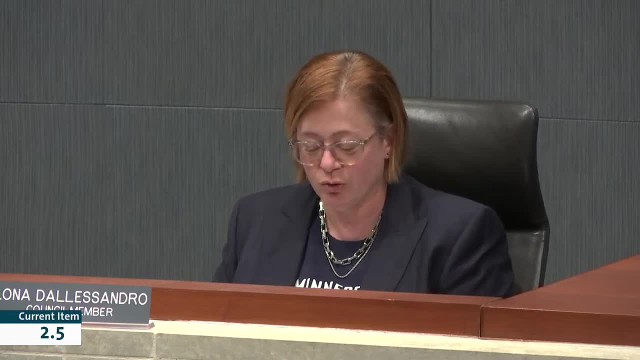 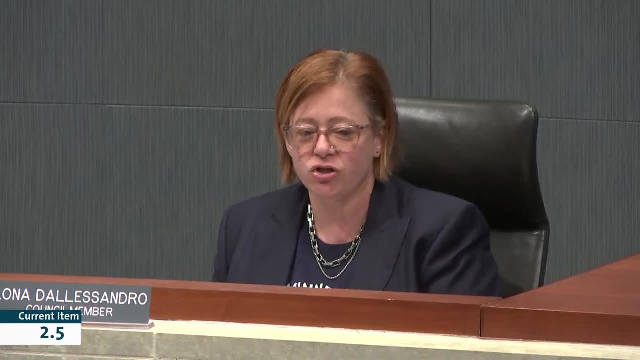 about what we're specifically thinking about, your ideas, et cetera. So let's make that happen. I have one question for you, and that is: I'm curious about the conversations that led to the distillation down to those three ideas that you chose to bring here. 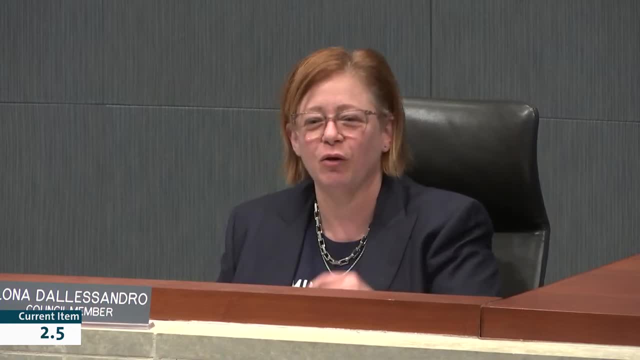 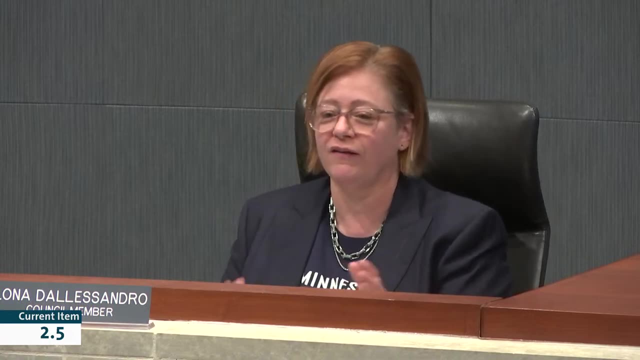 Were there ideas that you were really close to the line and you had to pick three, but if there was a fourth one you would mention it? Or was there a lot of contention around a particular one and you kind of had to you? 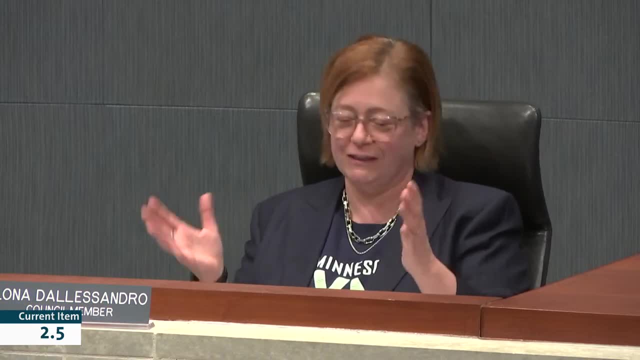 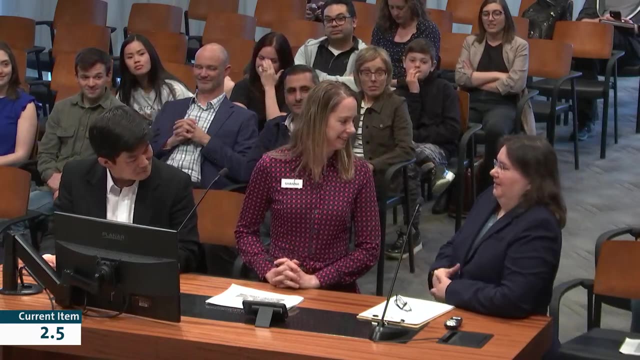 know, some group of people had to give it up and say, okay, I'll deal with it. You know, I'm just curious about what that dynamic looked like. Do you want to speak to that? You're the one who? Yeah, no, we arm-wrestled. 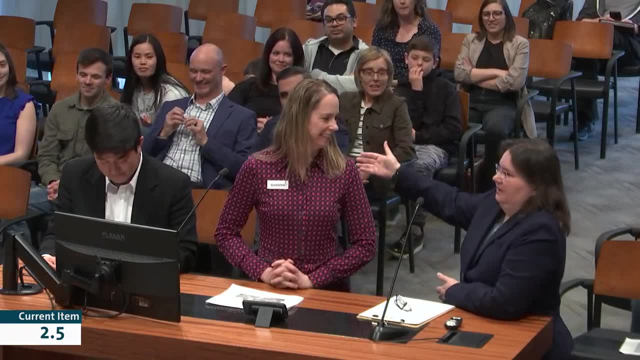 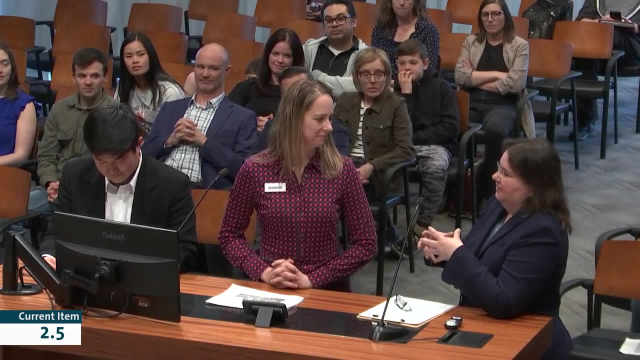 No, actually we built these wonderful, beautiful cities and we looked at kind of like that Venn diagram of the overlaps, and so there wasn't a lot of contention, We didn't need to arm-wrestle, and I think those were the three biggest focuses of those. 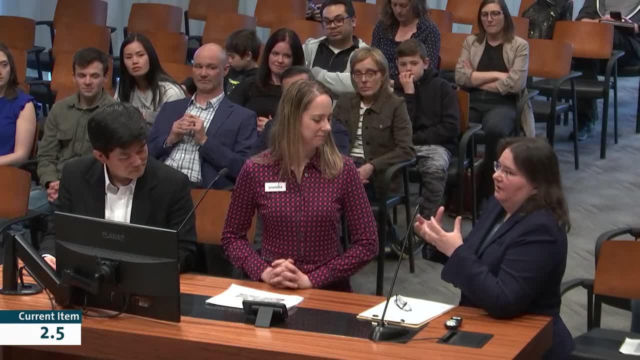 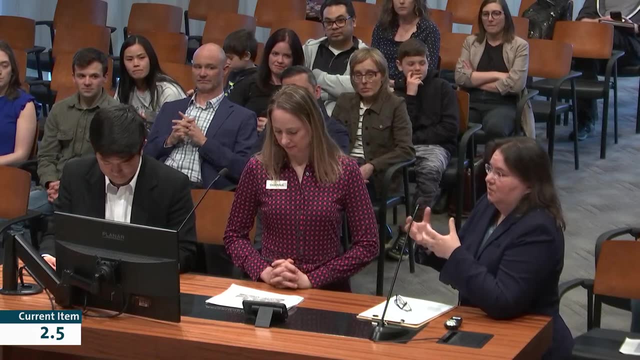 commonalities. I mean, we're all so dedicated to helping our climate and wanting a sustainable environment. I think that really ties to what Jason talked about having like the Bloomington Trolley, which would also help with accessibility and also help with decreasing, you know, carbon. 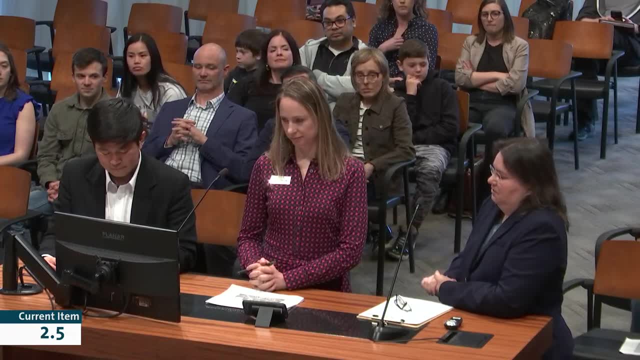 emissions, Not everybody having to Right to commute, and then also tied into the intergenerational living that Shanna talked about. So that's how we kind of came to those three. Yeah, great, Thank you, Appreciate it. 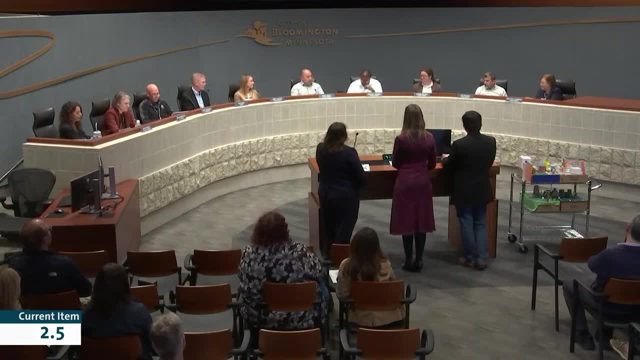 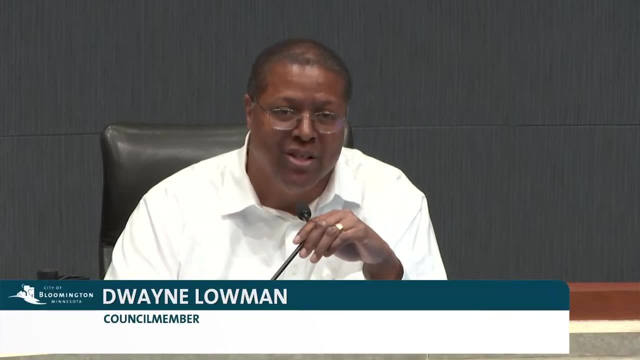 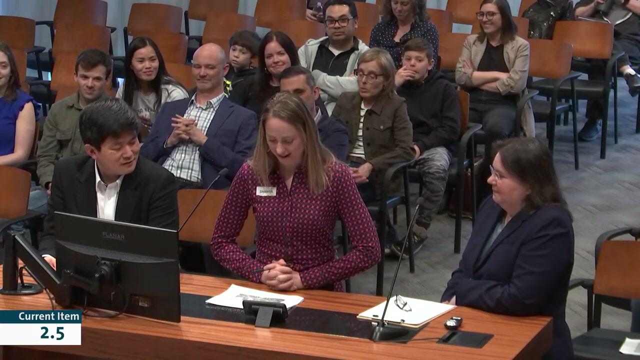 Congratulations, Mr Member Lohman. just a quick question. You had three great ideas, and certainly more I'm certain of too. Do you guys have a time horizon on those three dream cities? I think some of those things are achievable in the short term. You know, probably 2025,, 2026, and really kind of you know, by 2030, a lot of those things could be seen like a trolley, you know, being able to move people more efficiently in the city. 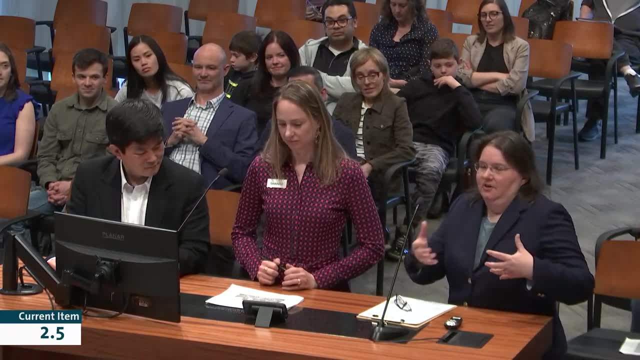 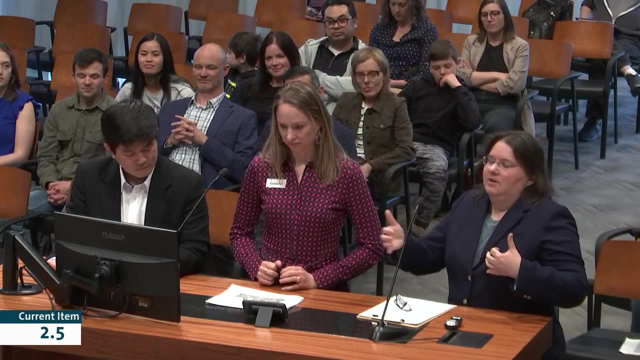 And then I think some of them also tie to Bloomington's strategic plan. you know, over the next 25 years We're not going to all switch to e-powered and bikeable and walkable, you know, overnight. but I think those are things that we can do through a phased approach. 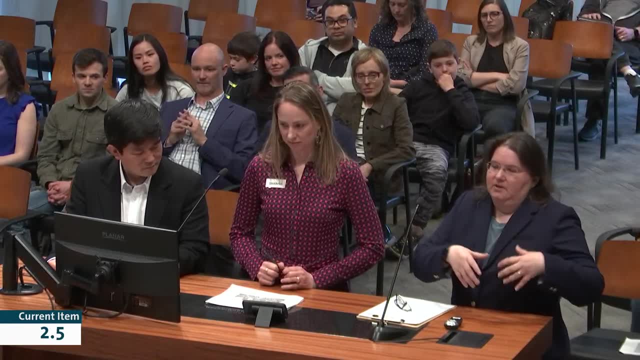 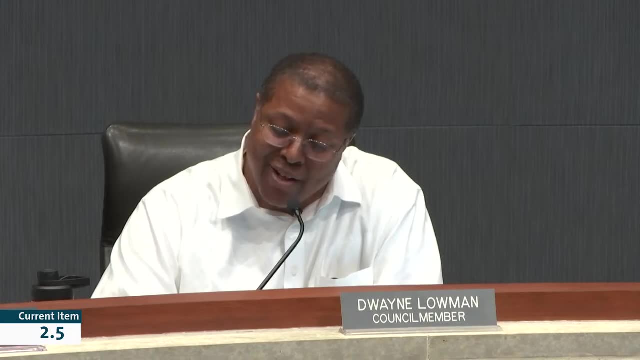 What can we do by 2025,, by 2030, and throughout that whole 25-year? I mean, I think we can do a lot of things, But I think there is more to it than just the Bloomington strategic plan. 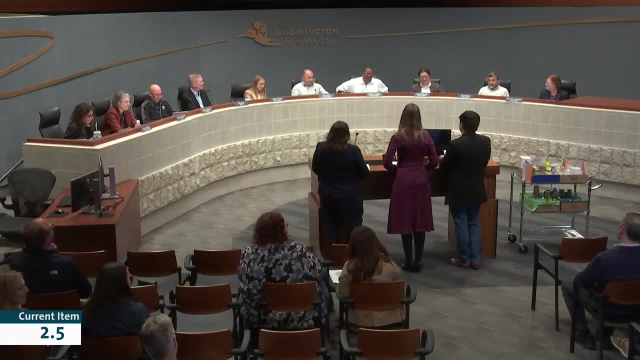 Well, thank you for all of your hard work. I know there's a resident in the back who's really excited about one of those items, I'm sure. Additional questions Council. So, Amanda Crombie, I have a question of you. 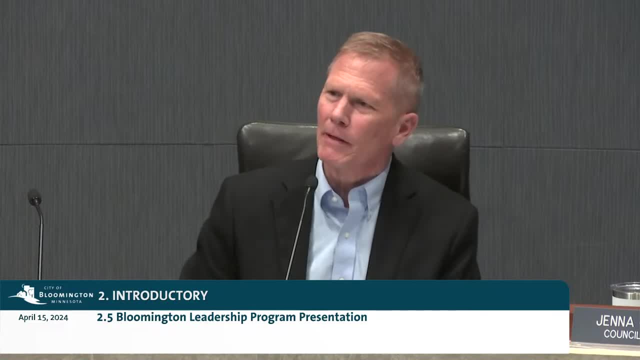 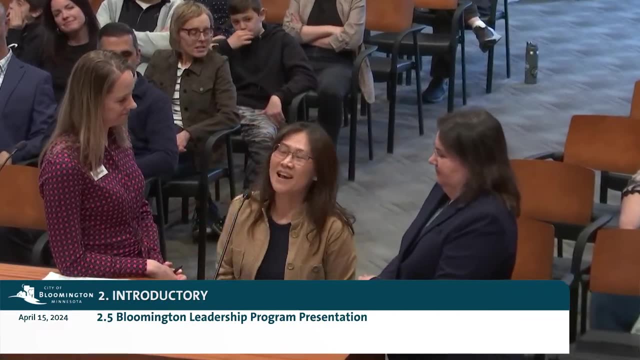 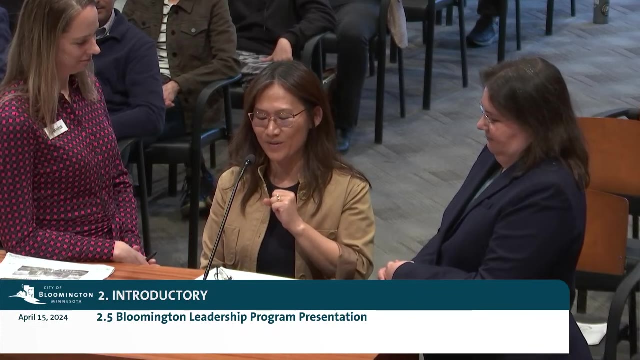 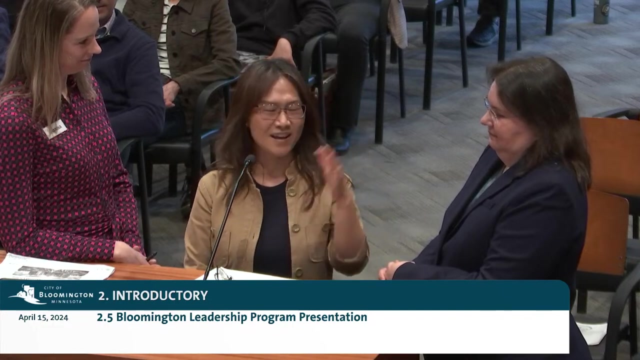 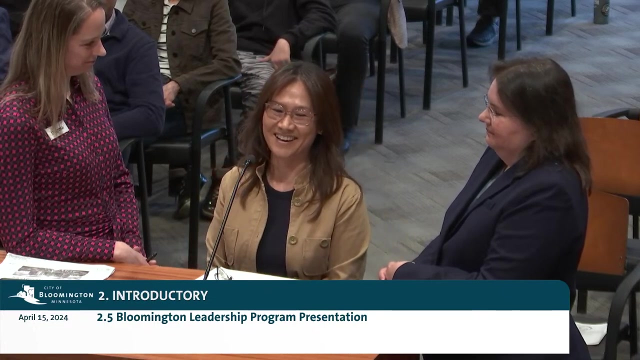 How many years have we been doing this now and how many people have come through the program in those years? Pop quiz for you, Oh my goodness. Oh well, Councilmember and Mayor, We've the first session started in 2019.. And so we graduated with this group- about 100. So we've had, I think, five sessions. we had to go every other year due to COVID or whatever. So yeah, so yeah. we had a really great group this year And they've been doing amazing work and they plan to stick together and do more work right. 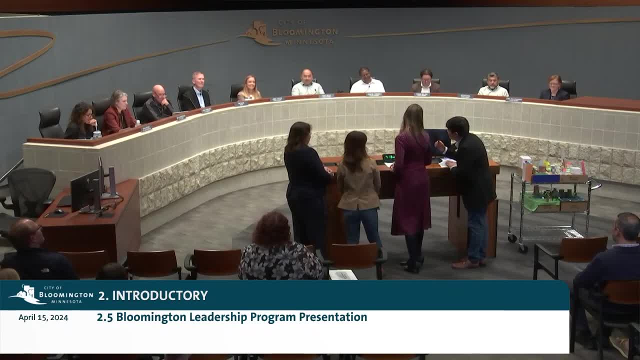 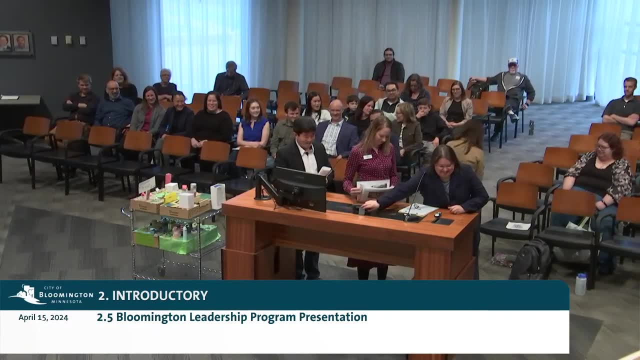 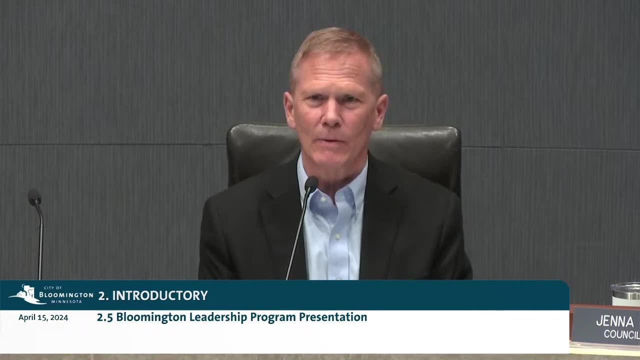 Yeah, It's great to hear, And every single one of us graduated this year Well done, Well done, Well. thank you to all who participated. Thank you for your commitment. We- I think we- talked about this at times. those were, those were Thursday nights, I believe Tuesday or Thursday nights, and you could have been anywhere on those Thursday nights And you chose to be part of this group. you chose to be part of this leadership cohort And I appreciate 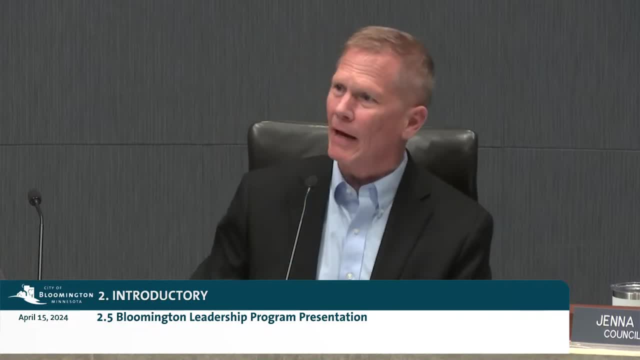 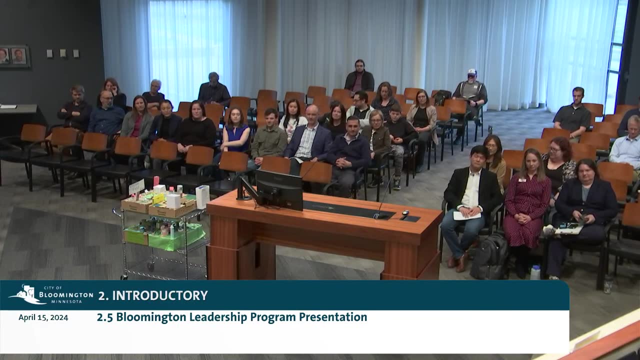 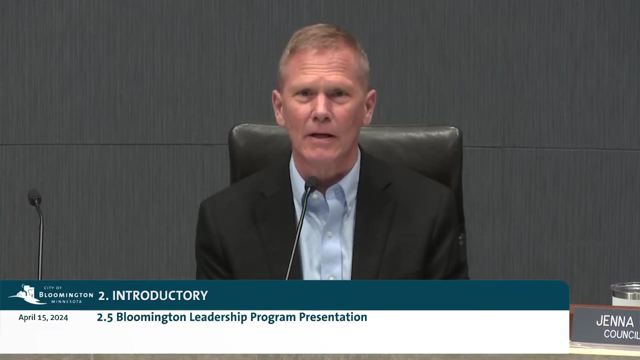 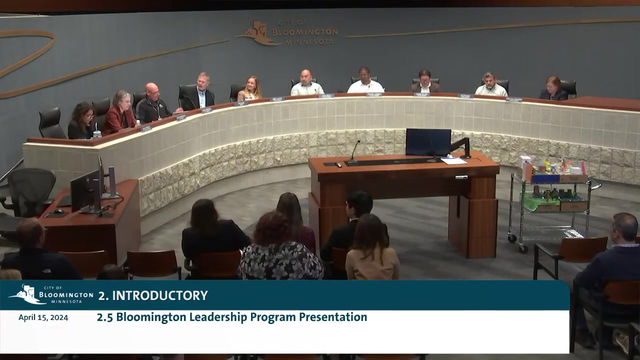 that, And I think the city of Bloomington should as well, because to have you and now 100 people who have been through this and who who see things, I think, through a different light and who are active and who are willing to to put in the time and to go that extra mile to make your community a better place, You're a great example And and you're a great resource within the city. So, thank you, Thank you all so very much. Mr Verbrugge, anything to add? You looked like you were going to say something. 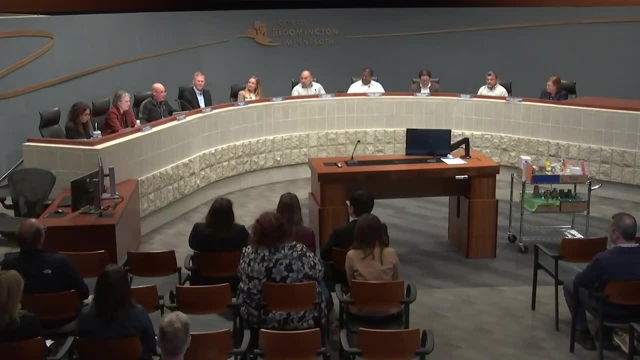 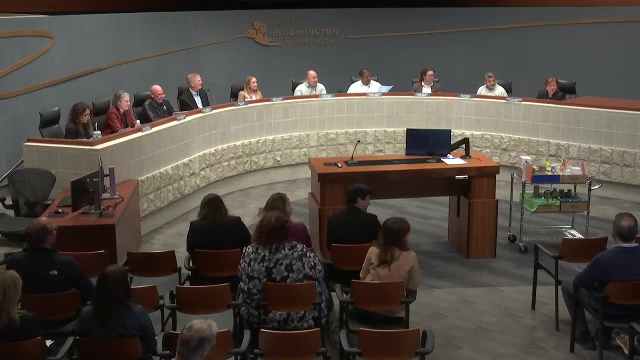 Mr Mary, I think you summarized pretty well. Very good, Thank you. Other than they were awesome group this year. Yes, they were Congratulations They were. Mr Mayor, if I may, if you haven't had any Luke's hot sauce, I recommend it. I was door knocking the first time I ran and I grabbed the cut. I got a couple of bottles. I don't know if I got the vote, but I got the bottles. 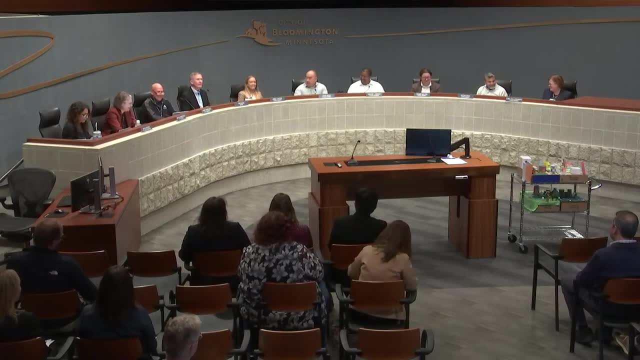 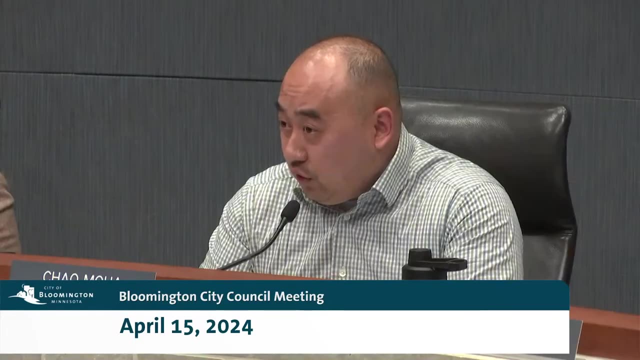 Very good, Thanks. Well, again, congratulations. Thank you, Council. I'm sorry, Council Member Moore last thought I guess this question is for the city manager or for Amanda. Will there be another cohort, And when should we be looking to? 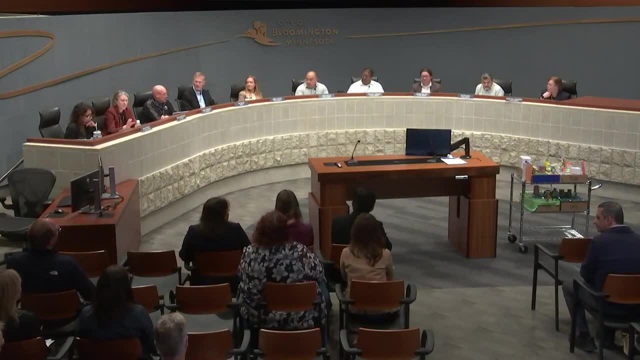 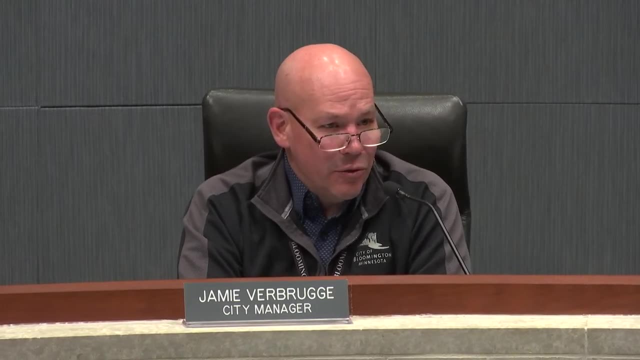 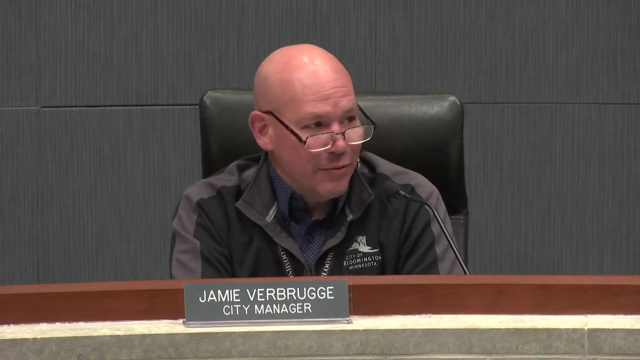 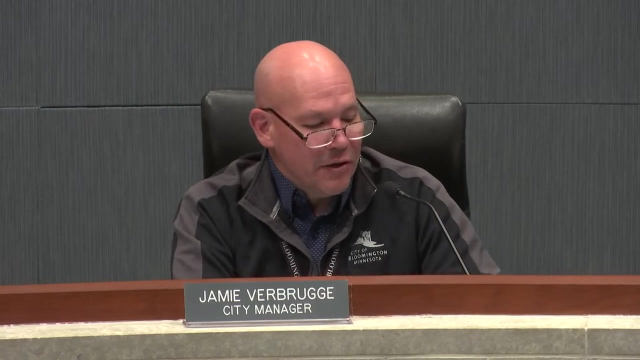 Mr Mayor and council members, we are doing one program a year. We'd love to do more than that And I do want to acknowledge the work that Amanda and Emily do to coordinate this, And it's a lot of work. So we'd love to do it more than once a year. I think that we'd have capacity just to do it at that level. So, yeah, we're not anticipating slowing it down. 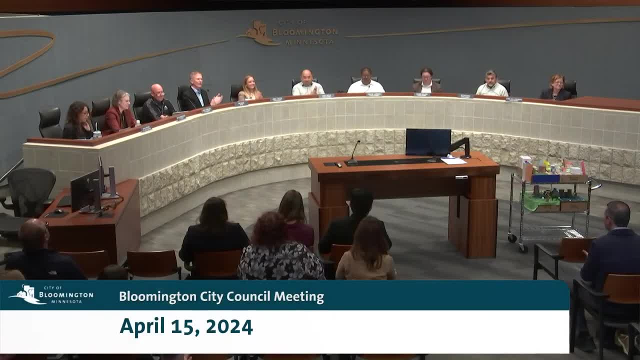 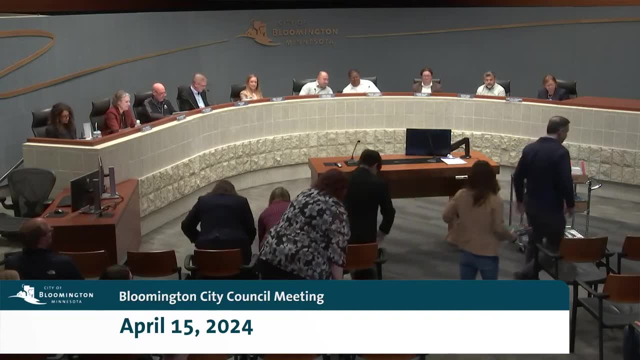 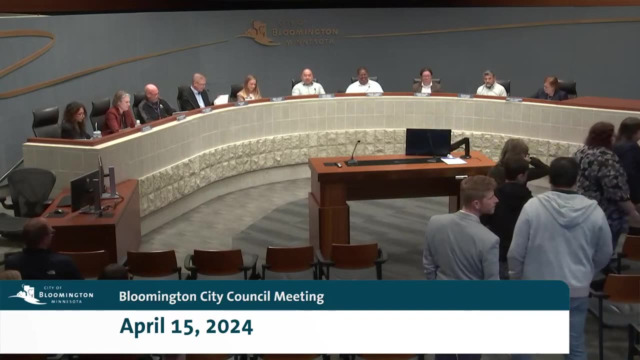 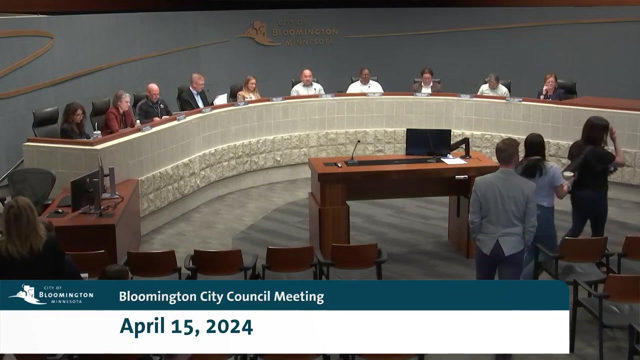 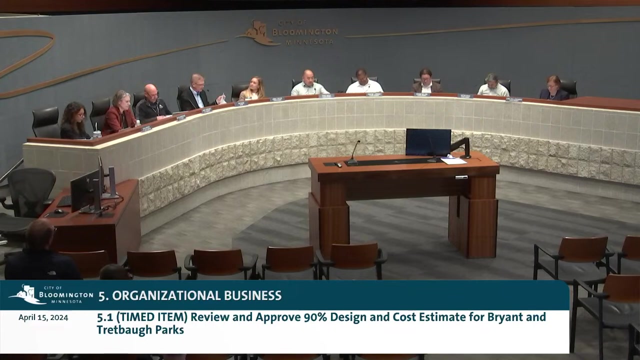 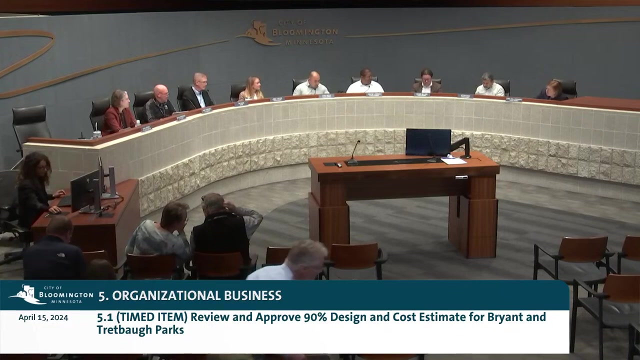 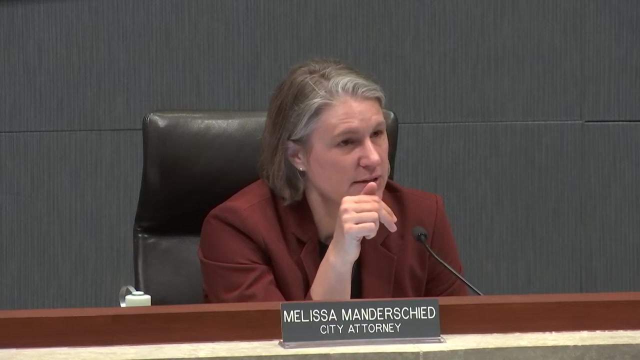 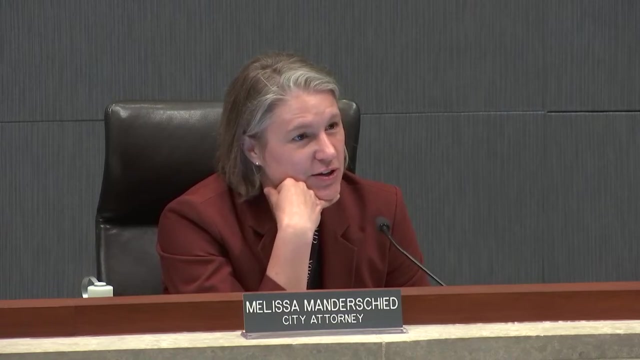 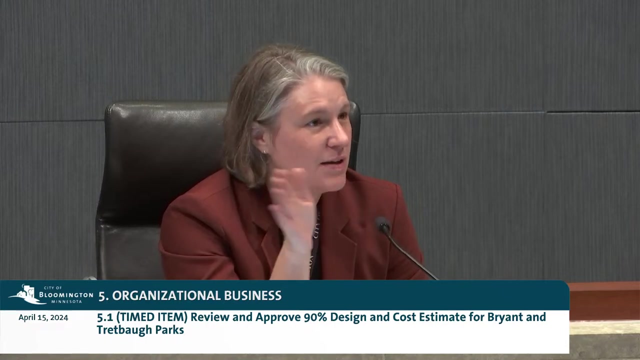 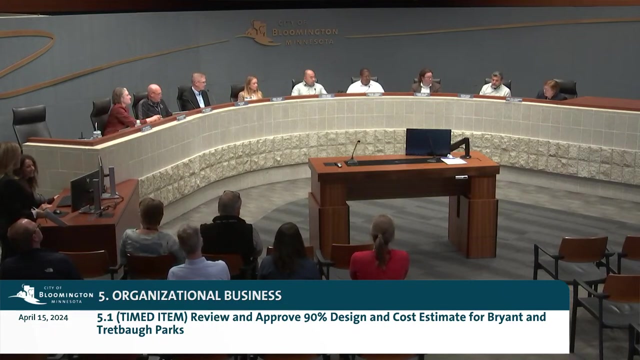 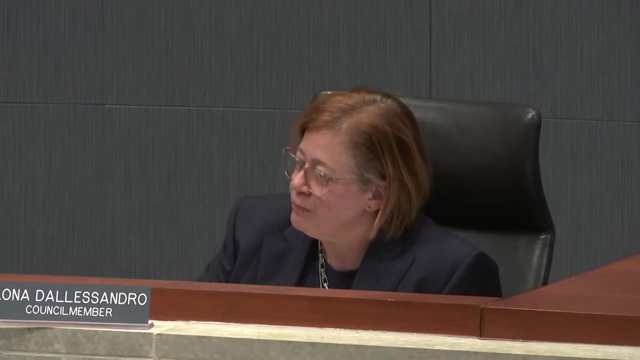 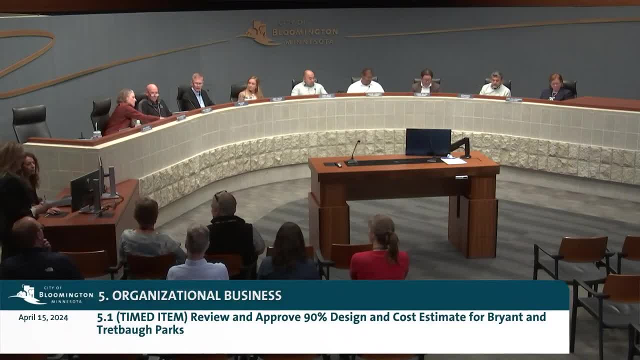 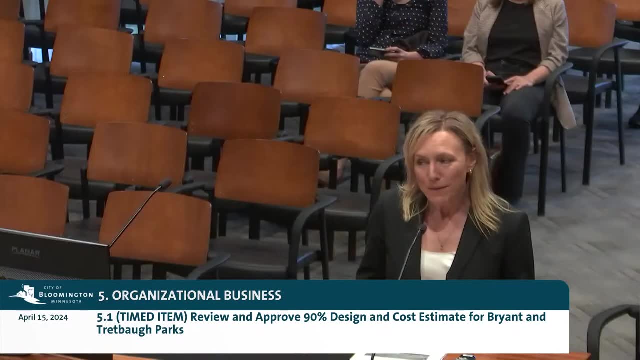 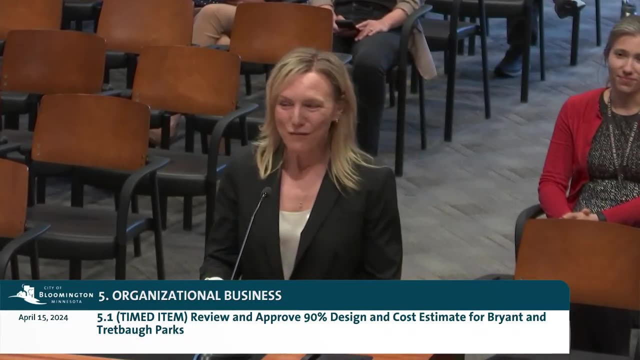 That's great. Thank you very much, Yep. Okay, All right, Ms Clark, are we ready to go? Good evening, Good evening, Mayor, members of council. I'm really excited to hopefully have one of the really exciting agenda items you consider tonight for the draft final plans for Bryant and Trebuchet. 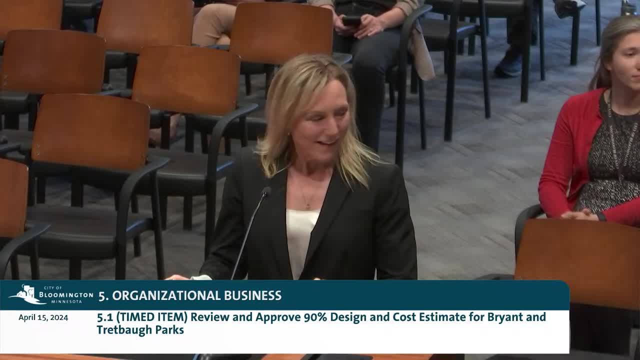 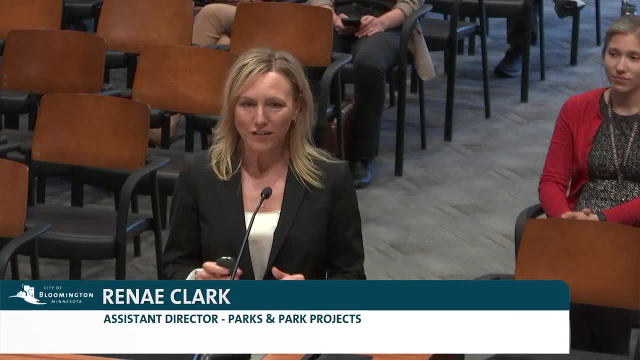 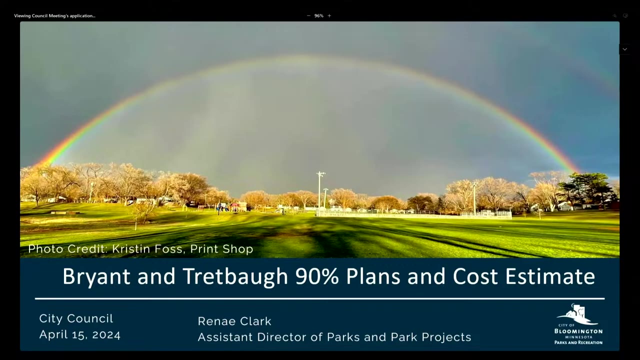 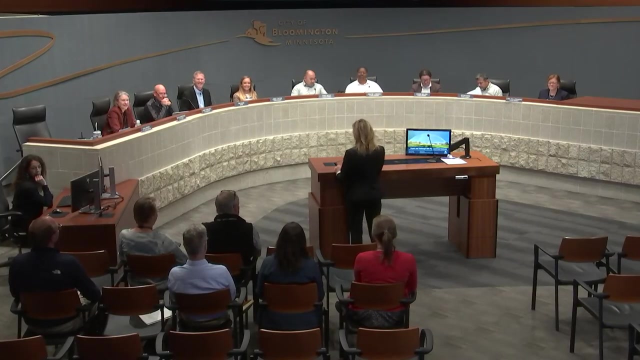 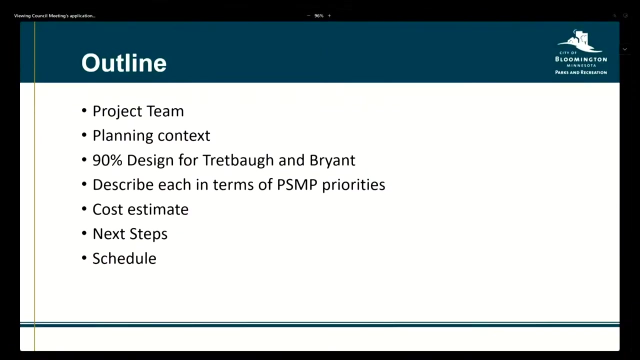 and I have a presentation that Safa is just pulling up while she does that. I'll move a bit ahead and just mention I. there's a large project team that's been working with us for a couple of years now really on these two projects and this half of the room includes that team. so tonight, in addition to the project, 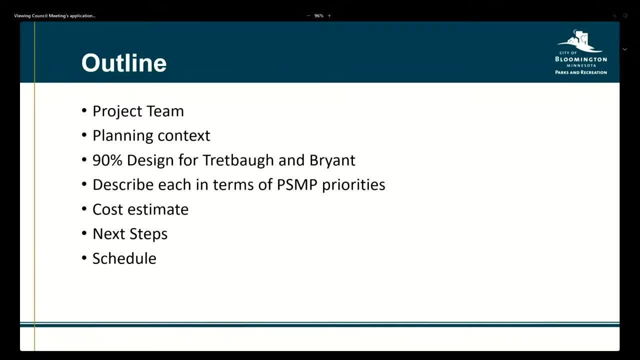 team introduction. quickly, I'll review the planning context for what we are here tonight with Bryant and Chippewa parks, cover the high level 90% design plans that were in your packet and then describe each of them in terms of the priorities from the park system master plan. 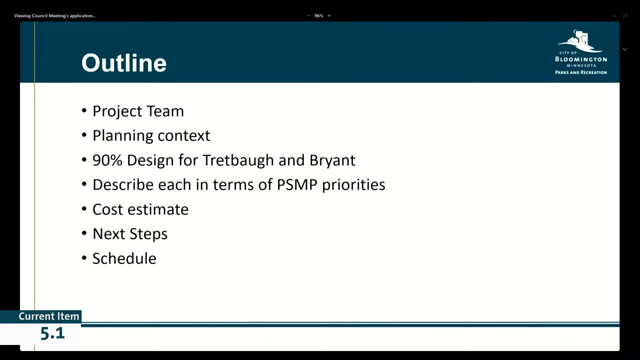 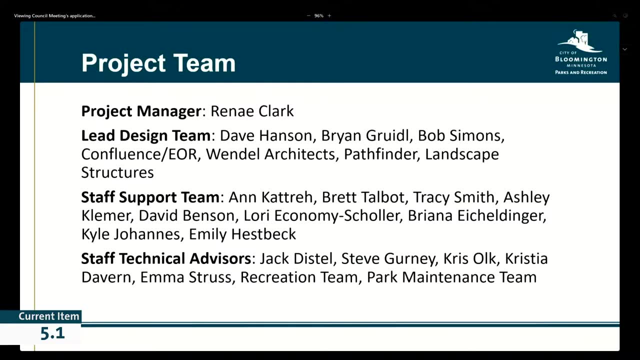 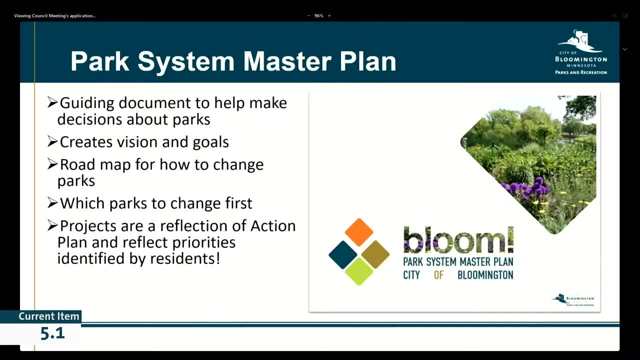 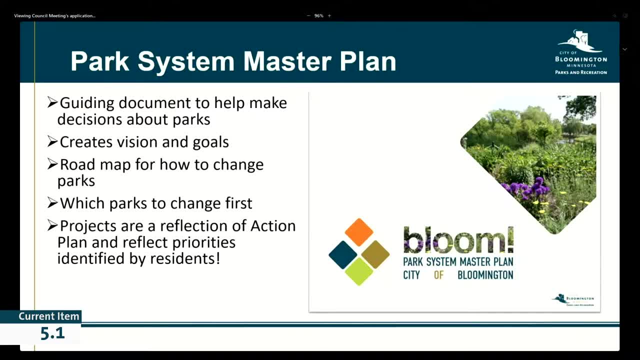 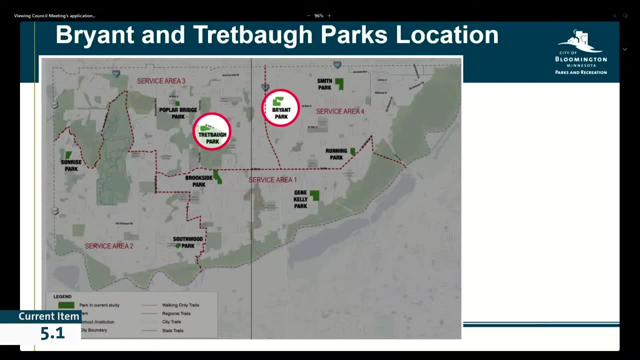 here in reference to the plan. the plan concludes with an action plan with nine sections and the things in these projects are a reflection of what's in that action plan and priorities established through that planning process by residents orientating us where we are in the community: bryant park, bryant avenue and 86. 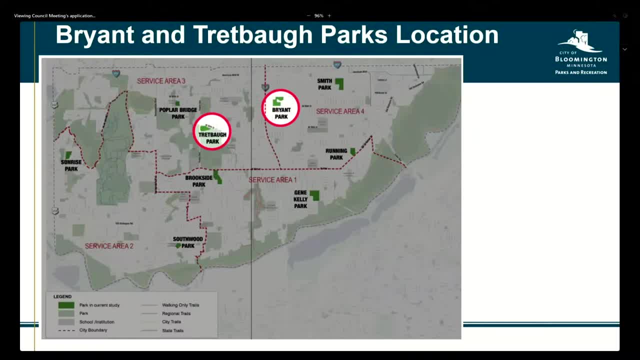 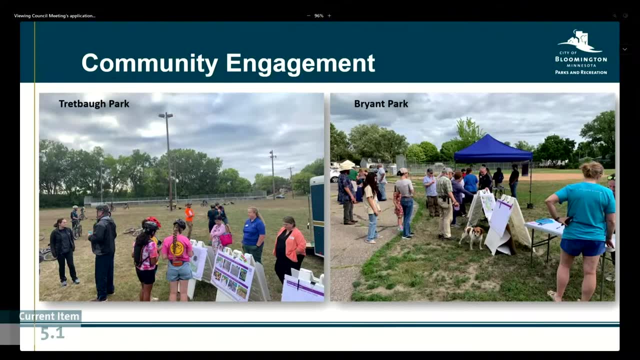 street, trepa park generally, 90th and france avenue on the north side of marsh lake. community engagement was a big part of these designs began really in 2022 when we started concept planning for nine parks. that engagement continued through 2023. all together we did four. 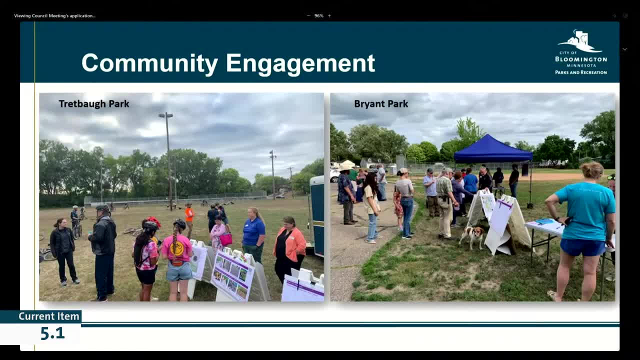 on-site engagement events in each park, plus the individual community conversations with residents, specific coordination with staff from bloomington public schools- tara, owens and the todd pod play group throughout the process have been very helpful and a really big resource for us, and then collaboration again throughout with our staff and commission. 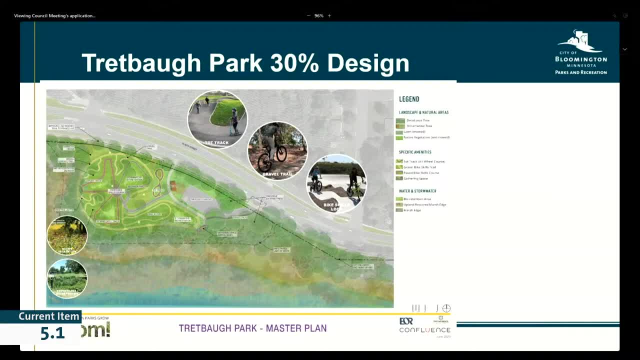 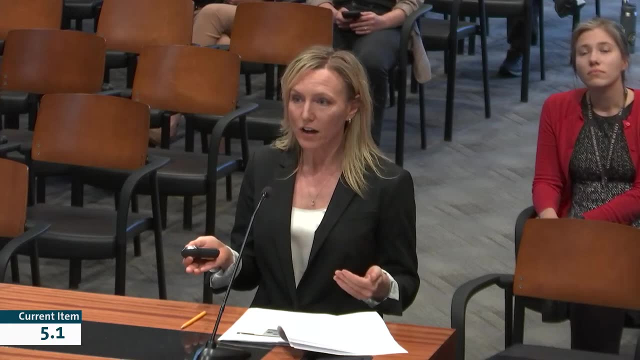 quickly going back to where we started. it was june last year, the end of june, where we looked at 30 design. trepa park hasn't changed much, but i'll recall that when we came with 30 design, one consideration was a dog park. there's a rink there that's used as a dog run today that neighbors 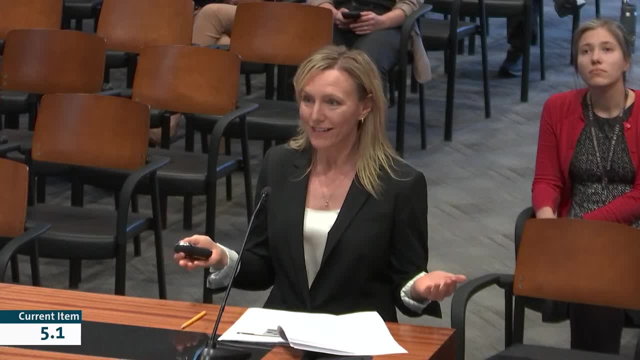 really love, and we're going to do that today, and we'll look at the design of the park as well. and we'll look at the design of the park as well. and we'll look at the design of the park as well. and wanting more of those in the community is a desire. 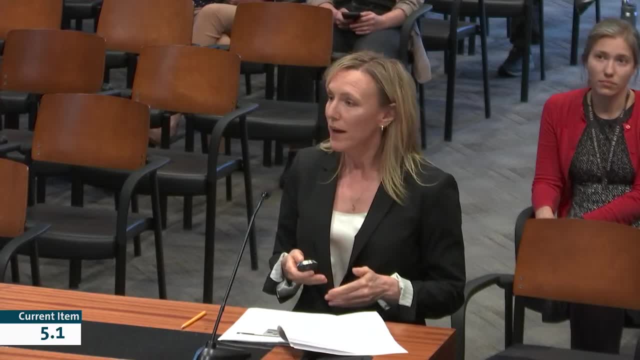 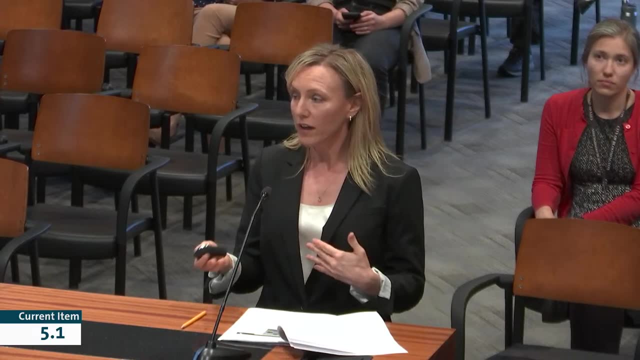 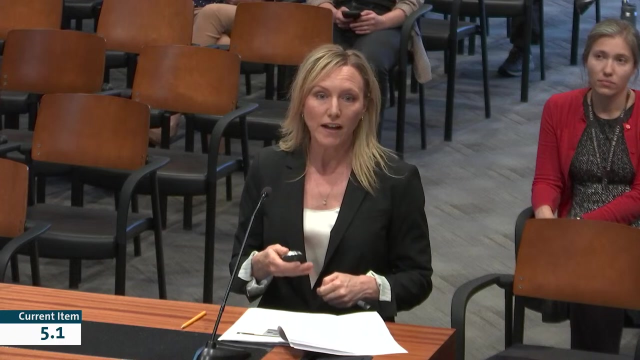 We looked at trying to incorporate that here. Some resident feedback came that dogs and bikes don't mix. We asked our Parks Commission to consider that question and ultimately we agreed with the Commission's recommendation to not try to incorporate a dog run here. but I'll note that it's on their work plan to find another location. 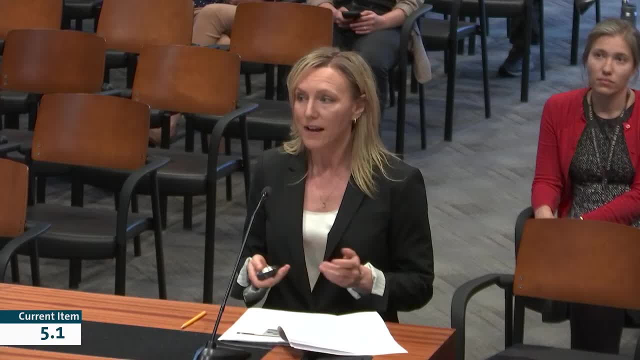 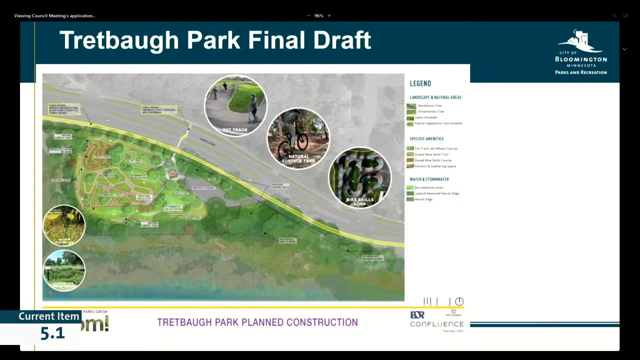 and they're actually exploring a couple locations for other dog parks and dog runs in Bloomington. The final tripod design is a combination again of a paved pump track, which is noted central in the lighter outline in red. The remainder of the site is a gravel mountain bike skills course. 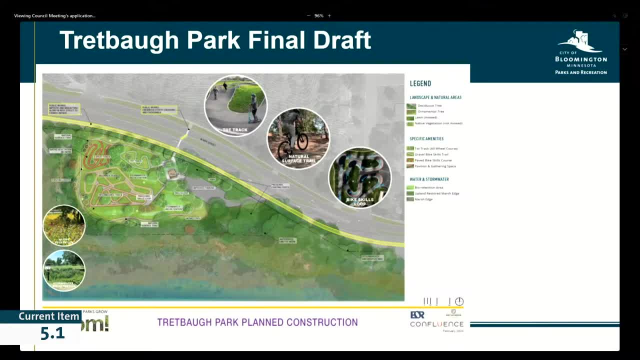 The site also includes a gathering place for hammocks. and then what's included as a bid alternate, shown in that more detailed cost estimate, is a shade structure, A shade structure for gathering- Again, natural resource, a big component of this site. 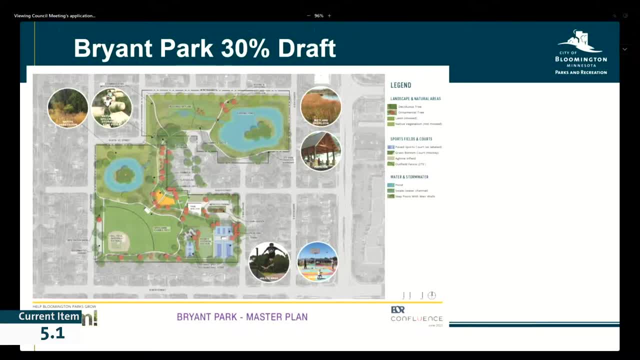 Bryant Park. looking at 30% design and comparing to where we are today are a lot more changes, The big ones here. the playground moved from where it is today in the yellow blob to where the parking lot is today, shown on that plan. 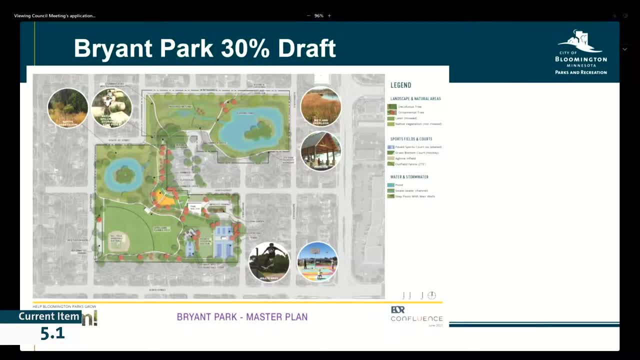 and, despite the desire by the community for more pickleball staff, are really carefully considering where we site pickleball. We've used some online research and other community experience to establish a minimum buffer of 250 feet and a desired buffer of 300 feet from homes. 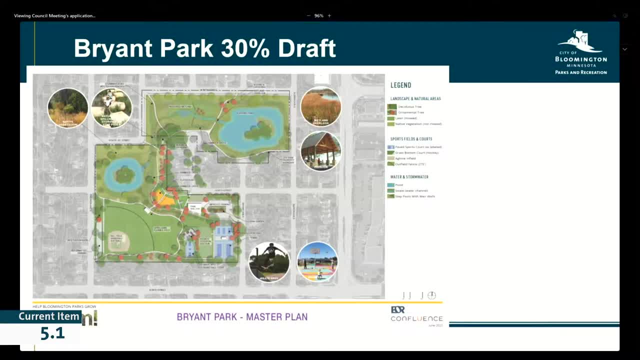 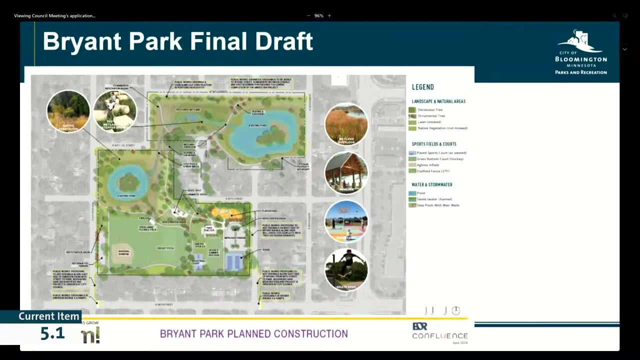 where we consider pickleball, and here it was just too close to home, so pickleball was eliminated from the design. So those are two of the major changes we're looking at here. in the final draft which I brought up, You'll see that orange blob moved to the corner. 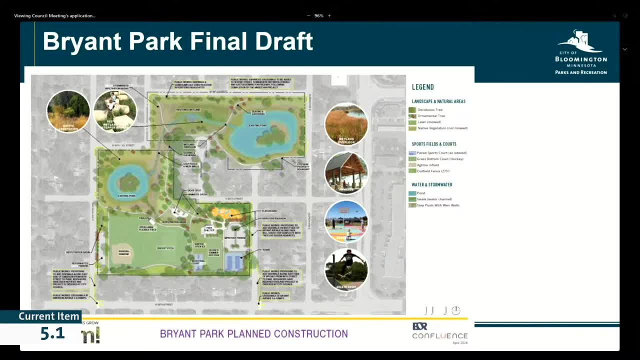 closer to parking, farther from water, which was a specific comment from residents and families. The skate spot moved to where the playground currently used to be sited. and again, tennis. there's still two tennis courts. pickleball's gone. The green space is programmed not just as a baseball outfield. 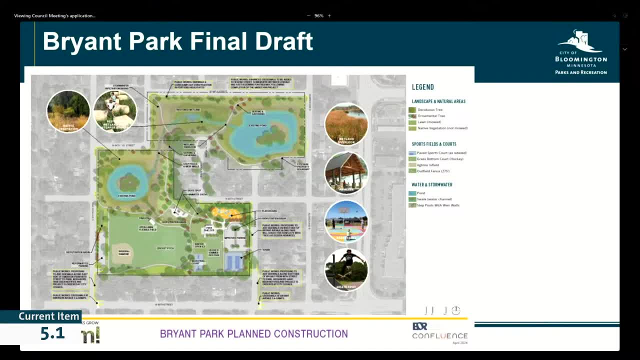 but has room for soccer to be striped as soccer and will also include a cricket pitch for tennis cricket which is played, I believe, at Bryant Park today and other communities around Bloomington. our recreation staff coordinated with that group to help determine if that would fit here. 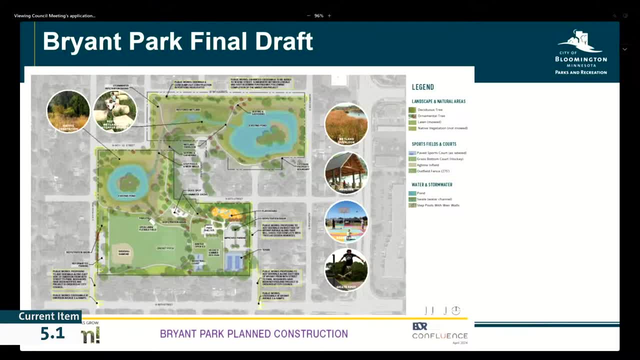 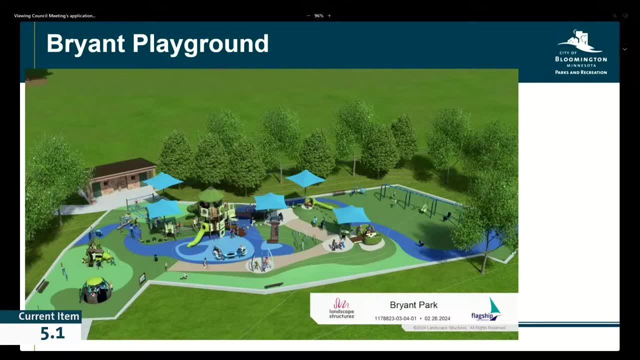 and that is something that that group is really excited about. I'm going to highlight the playground and the building part of Bryant Park for us tonight. Before you first is an image of the playground. It's Bloomington's first fully inclusive playground We received. 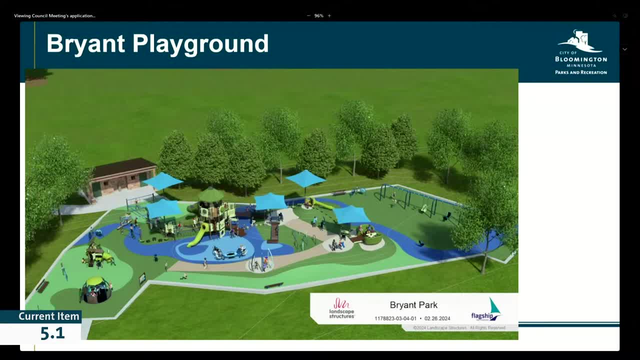 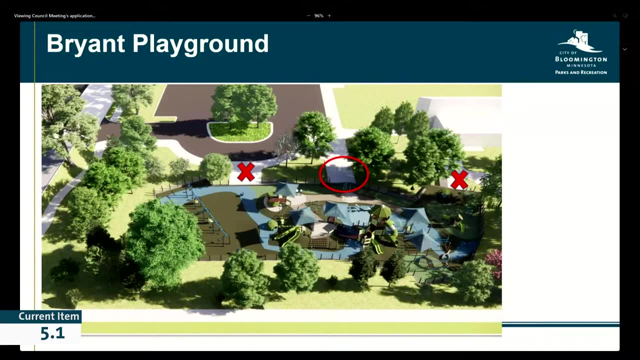 We received a lot of specific feedback on the design. I'll highlight a few of those on the next slide. but let's see. entrances were one of the feedback. We had two entrances and the community really desired one with a fence. Both are included in the final design. 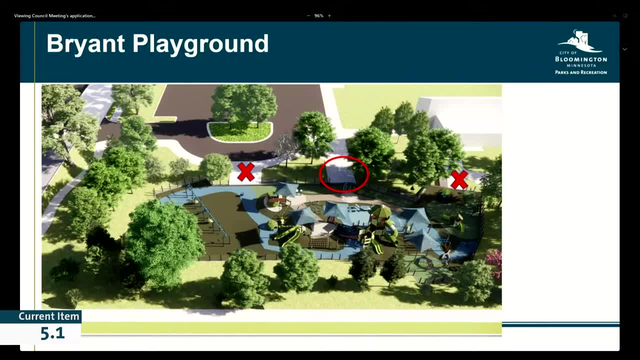 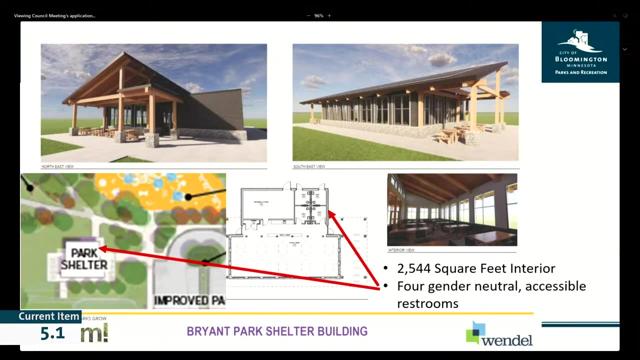 The Swing Bay was something we had a lot of iterations on with the community to really maximize the diversity of swings and the number of swings. And then the building. before I use a rendering of the building and then an image in the lower left to orientate you to the layout internally. 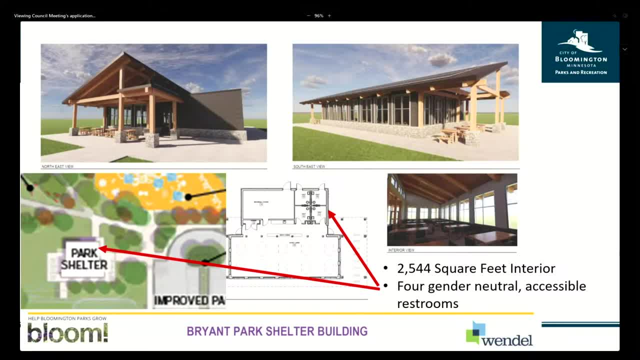 as it sits in the park, So the building itself is just over 2,500 square feet. four gender neutral, accessible bathrooms. One of those restrooms will have an adult changing station. That'll be the first adult changing station in one of our park restrooms. 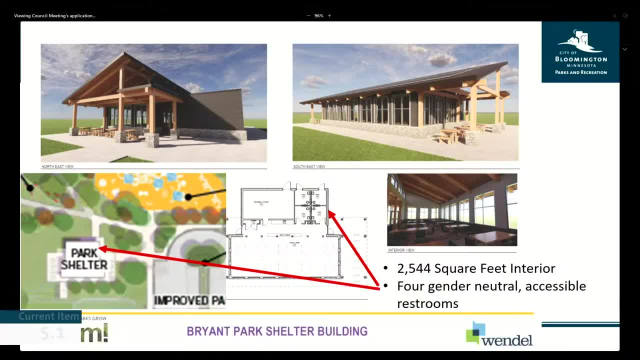 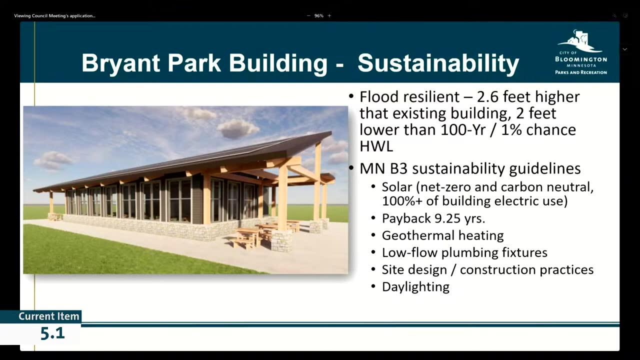 And then the image on the left orientates you to how those, specifically the restrooms, are connected to the playground. More about the building and sustainability. Flood resilience was a big consideration of the design. I'll talk a little bit more about the park in general. 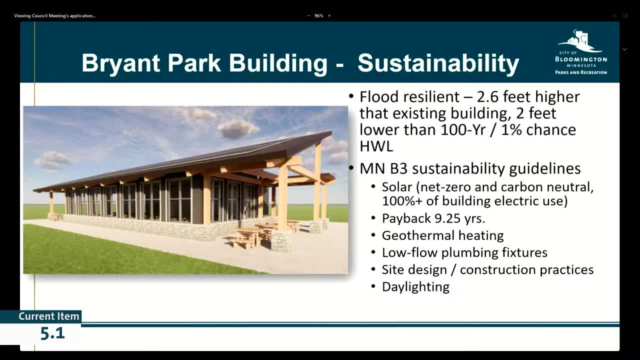 and the water resource opportunities there. but the building sits two and a half feet higher today than the current building to make it more flood resistant. And then other points of design for flood resiliency were highlighted in the packet. B3 or LEED equivalent was a desire by the design. 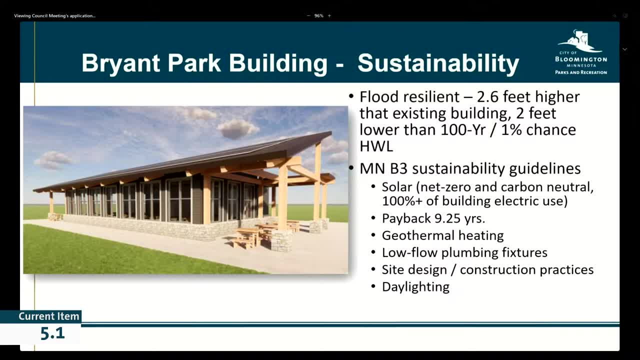 but not a requirement of the design, Something we wanted to explore the feasibility of With our design team. we believe we are meeting the B3 guidelines, although not we didn't explore. although not we didn't explore- participate in the certification process. 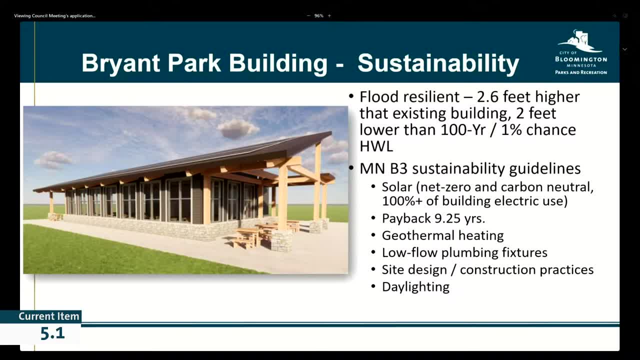 from the beginning. We are meeting those guidelines on net zero and carbon neutral building. We believe we looked at the solar specifically and the payback on that is about nine years. Geothermal heating is included in the design, adding about two and a half percent project cost overall. 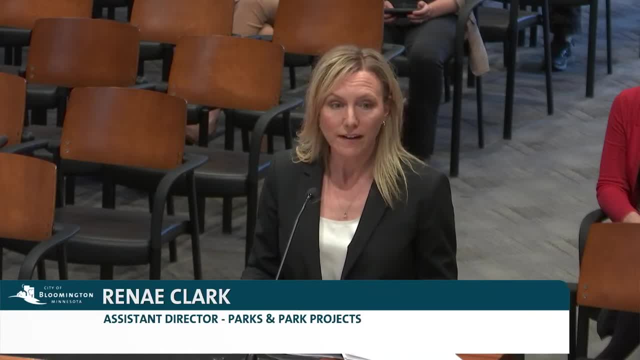 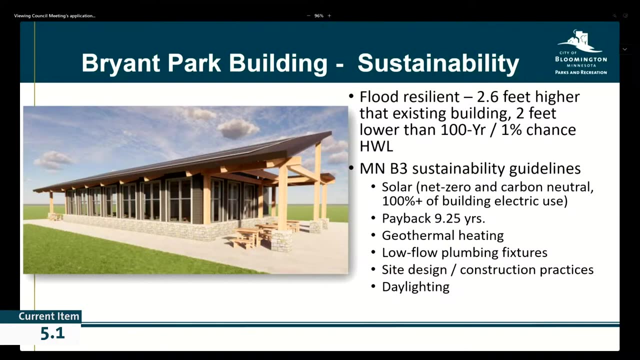 But that's part of achieving that carbon neutral. but that's part of achieving that carbon neutral and net zero by not requiring as much electricity and then just the efficiency of geothermal And then low flow plumbing fixtures, then site design, the storm water management. 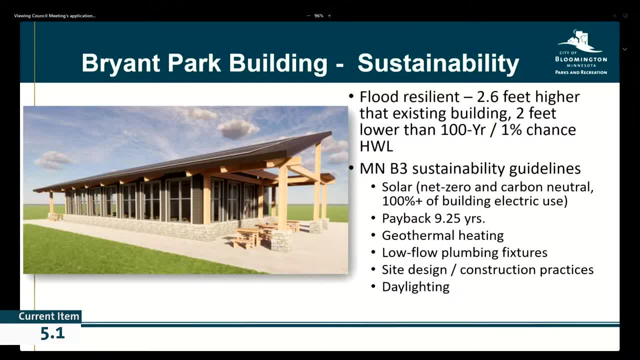 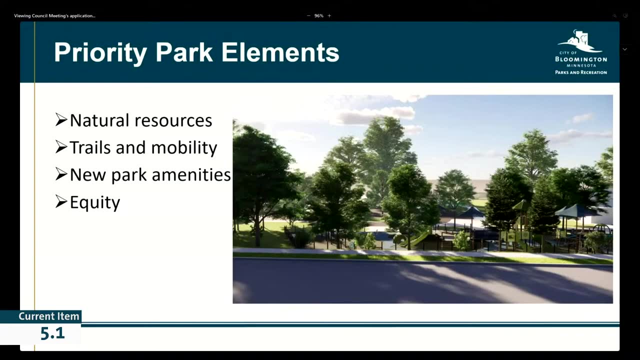 and other green infrastructure contribute to the B3 requirements, So we're really excited about using this as sort of a test on how we can achieve B3, particularly with the smaller site. I'll review each park in terms of the test and then I'll give you a little bit of an overview. 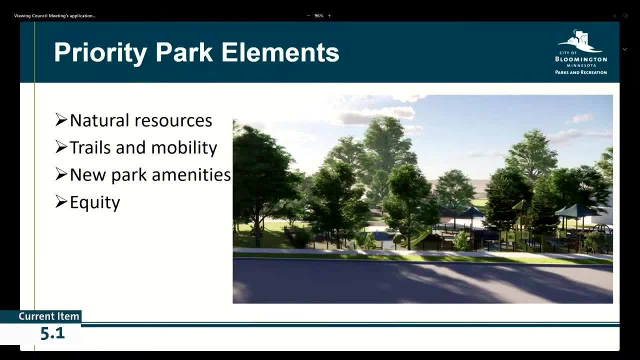 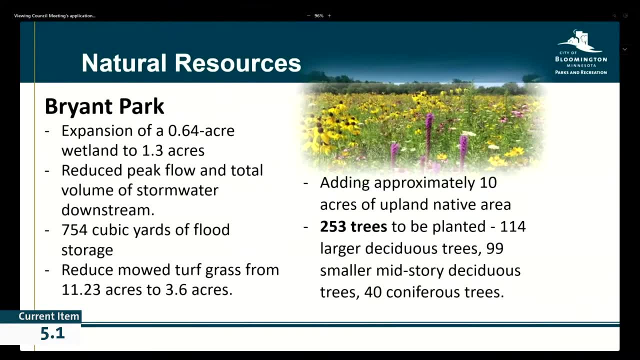 of the different parts of the plan. So we have top priority park elements Our residents identified as part of the park master plan. Those were natural resources, trails and mobility, new park amenities and equity. First in natural resources, Bryant Park was chosen. 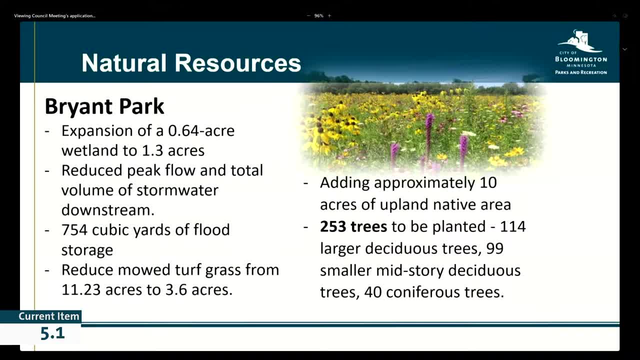 for the opportunity and challenges of natural resources, particularly water resources. Here there's a 372 acre drainage area, which is about 22 acres and about 20 is within the 100 year high water level of that area. So dealing with storm water and natural resources. 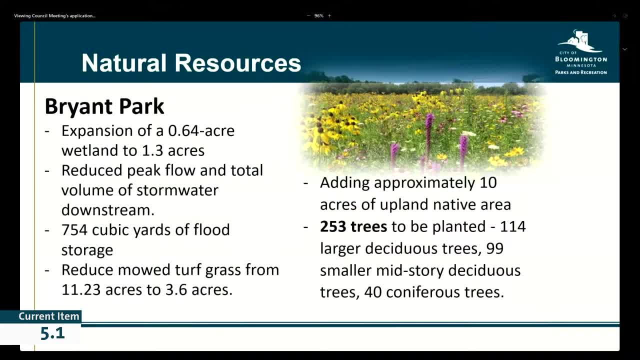 was a big opportunity and we're really excited about the outcomes here: expanding 6.4 acre wetland to over an acre, reducing peak flow and total volume of storm water downstream, adding over 700 cubic yards of flood storage on site. 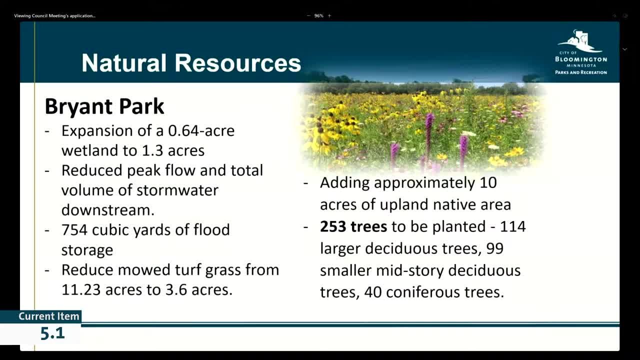 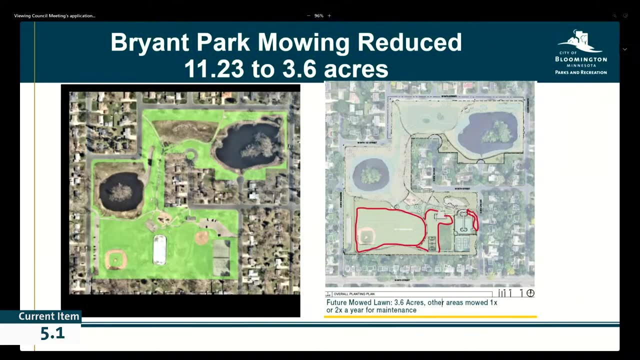 and then reducing the mowed turf. I have a graphic after this to show you, but we're going from over 11 acres to just over three acres of mowed turf here and then adding over 250 trees. This graphic illustrates, I think, really in an exciting way. 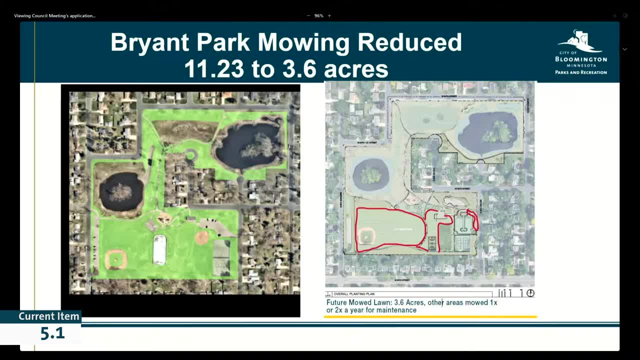 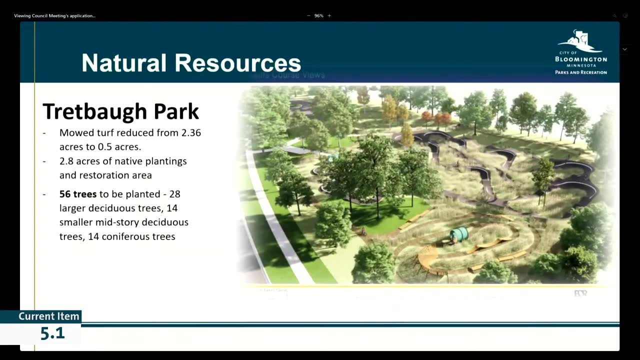 the reduction in mowing. Our park maintenance team was able to provide the graphic on the left that shows what's mowed today and the graphic on the right. the areas circled in red highlight what will be mowed. post project Trepa Park, while it's a bike skills park. 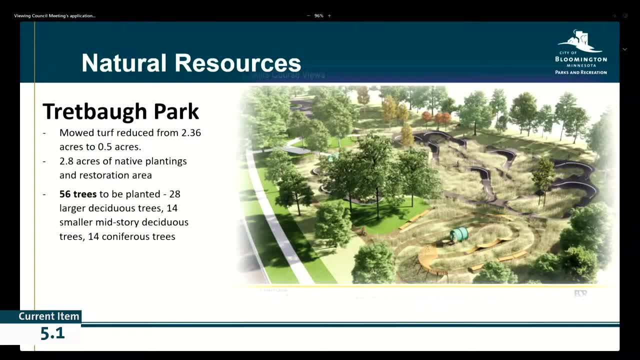 is also grounded in natural resources and connection to nature. The mowing there is being reduced also from over two acres to about a half acre, over 50 trees planted, and this, this image really demonstrates, I think, just the natural state and respect next to Marsh Lake. 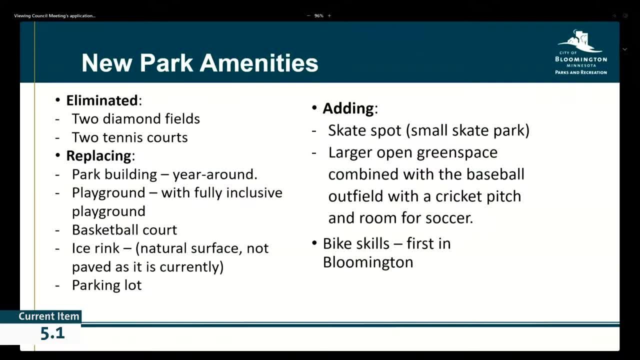 that this site provides New park amenities. another priority: Council directed staff that, as we look to eliminate things like ice skating rinks or dog parks, what are we replacing with new opportunities? And we were really mindful of doing that during these designs. 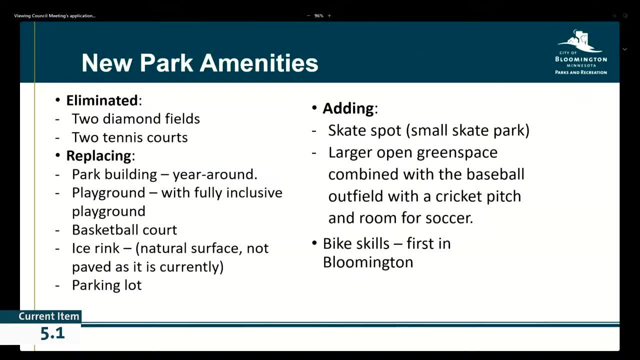 At Bryant we're eliminating two diamond fields- our park master plan- and we're eliminating two diamond fields and some with more variety. Our park center plan looked at the number of diamond fields and our staff evaluated that in terms of programming. 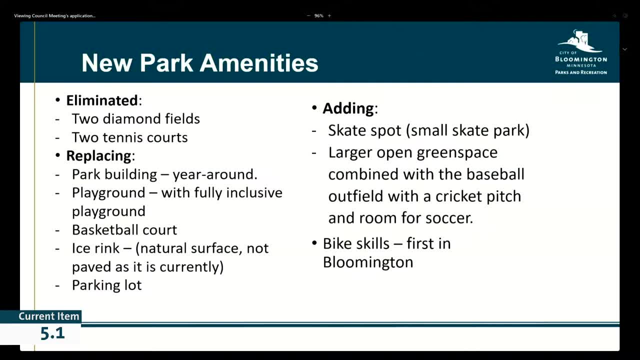 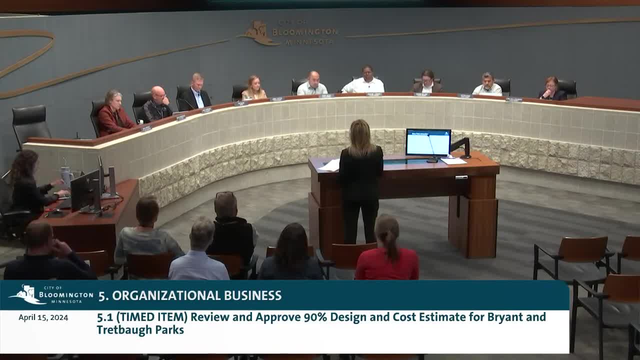 and found that we can reprogram some of those to other amenities that could get more and better use. We're reducing two tennis courts, we're adding the small skate spot, First fully inclusive playground, and then I note the things we're replacing here too. 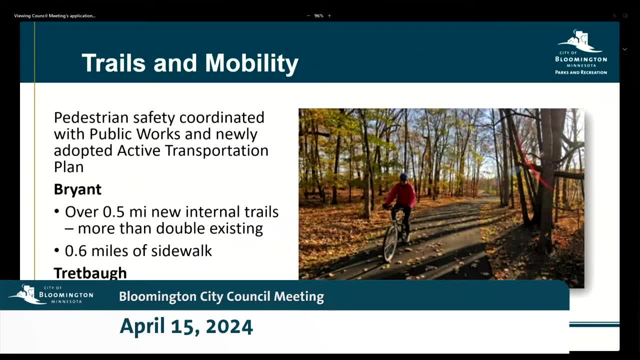 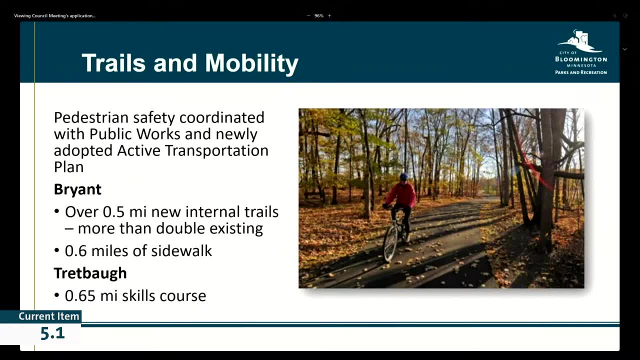 Trails and mobility Staff in parks had the opportunity to work with several staff in engineering. Bob Simons presented the plan for new sidewalks here and at Trepaw Park and the safer crossings. Those are things collectively when we talk to the community over the last two years. 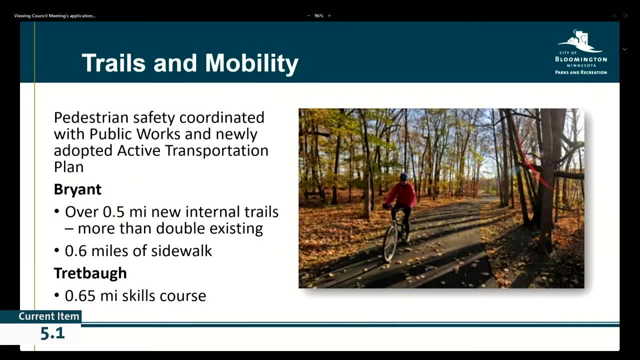 we heard about safer crossings and in different places around Bryant and Trepaw And as engineering staff worked to create the active transportation plan, some of those same things, concerns and opportunities were echoed, reflected in that plan and staff in engineering and parks are really excited that we're able to address some of those with these projects. 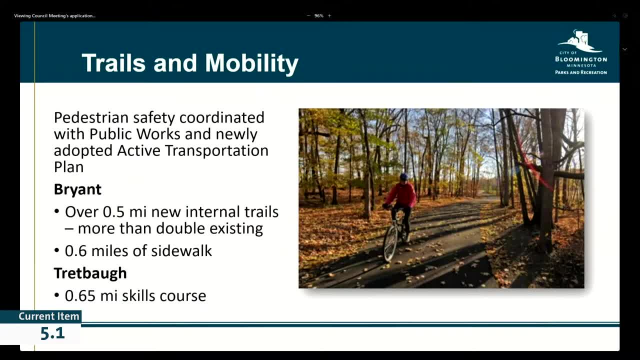 Bryant's adding over a half mile of integrated loop trails, which gets at some of the multi-generational use As well as the building that our leadership cohort identified. And then Trepaw's adding over a half mile of trail for bikes. 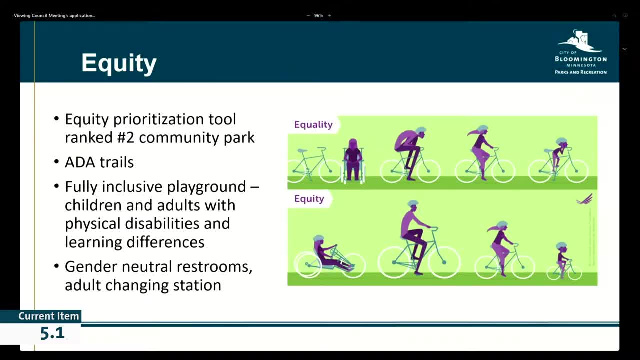 Equity is a priority for the city. It came as a priority from residents when we did our park master plan. Bryant Park is using the equity prioritization tool that was developed as part of the park master plan. Bryant Park is the second highest ranked community. 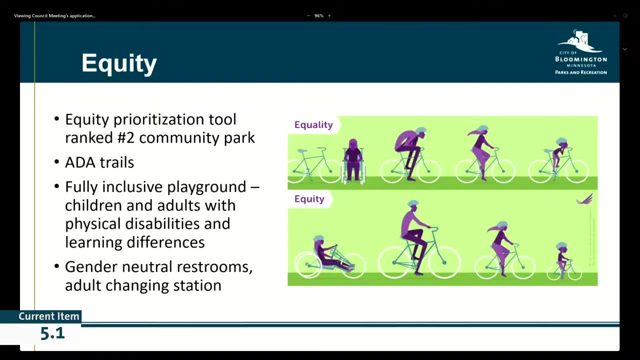 Bryant Park is the second highest ranked community park with the building, And I'll say Smith Park is the first, And that park council authorized an investment in just last year as well. So that tool has been really guiding in our work. Our trails are ADA accessible. 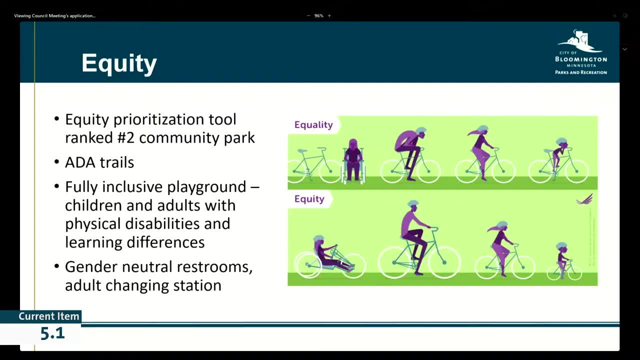 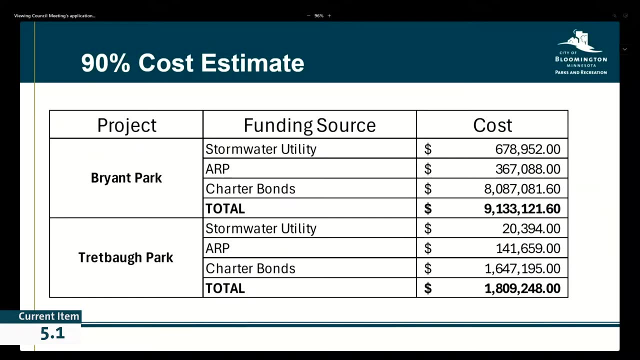 We've got the first fully inclusive playground which, I'll say, considers children and adults as caregivers, mobile and with mobility challenges. And then the gender neutral restrooms. The cost estimate: The cost estimate is in your packet. We've coordinated closely with our colleagues in finance. 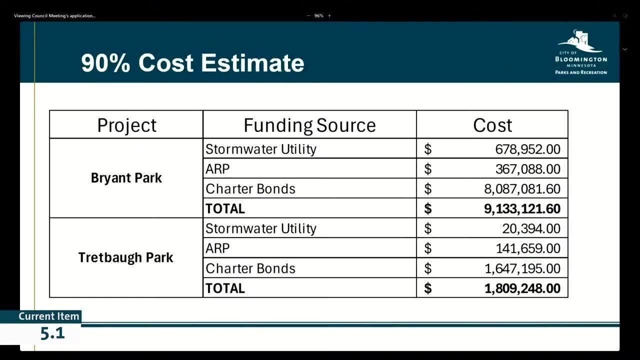 There's an agenda item to talk about the charter bond process after this. The cost estimates are quite in line with the estimates that we presented to you at 30% design. The more expanded version was in your packet. We feel that there is that our costs and the things that we have below the line. 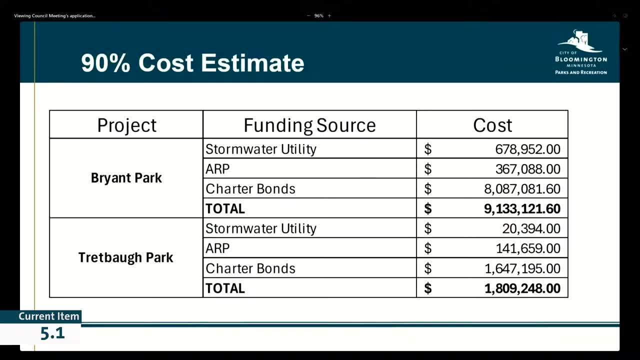 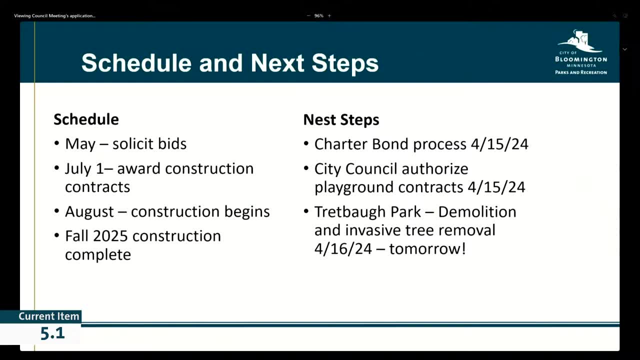 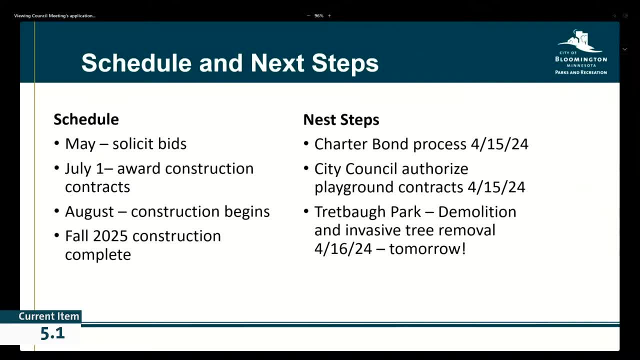 Demolition of the small shelter building and then invasive tree removal is scheduled to begin by our park maintenance team as soon as tomorrow. The schedule otherwise in May. we plan to be out soliciting bids and be back to award construction July 1 or at a subsequent meeting in July, with construction beginning this August. 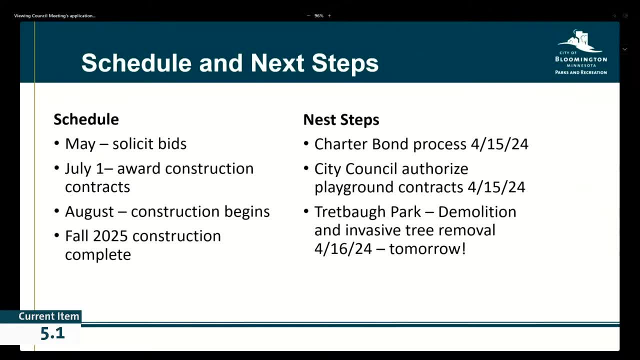 Completing fall of 2020.. With that, I can take any questions, and thank you for the support at our engagement events and as we've been working on these projects, and also thanks to our team. Thank you, Thanks for the presentation and thank you, yes, to the team for the work that has gone into this. 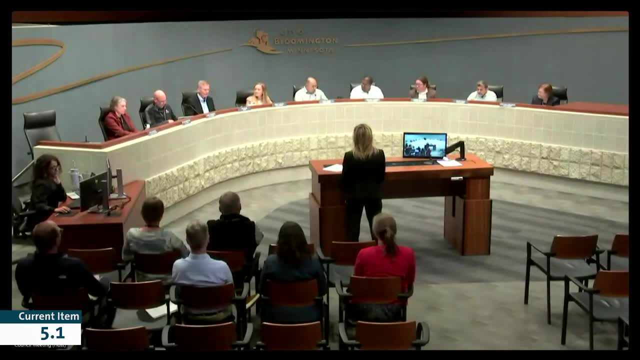 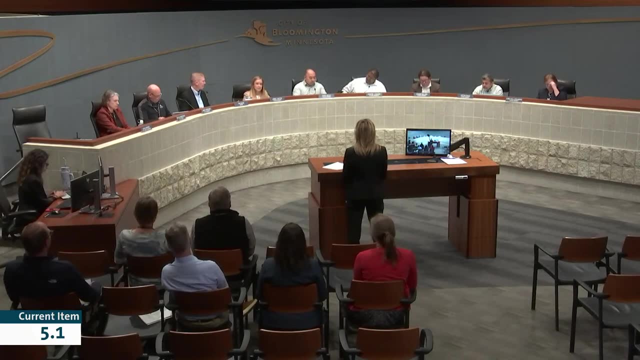 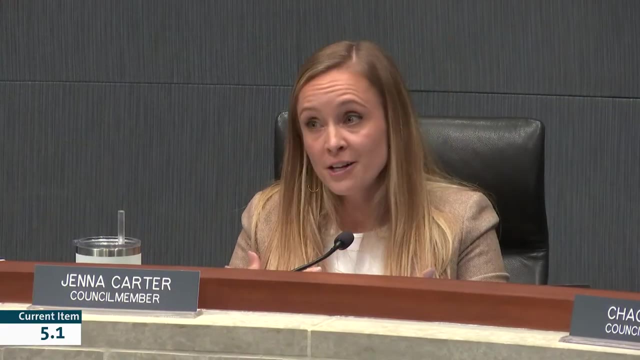 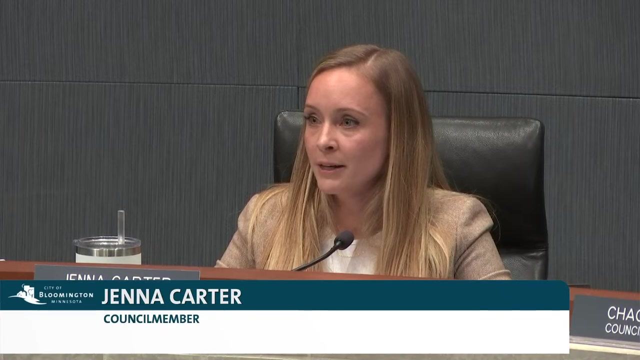 And I know it's not an insignificant amount of work that has gone into this. So thank you much. Questions: Council Member Carter and then Council Member. Thank you, Mayor. I only have one question, but I just wanted to say that I really appreciated that you started with the history and the context and how we got here- for us, but also for people who are tuning in tonight and who are interested to hear how we've got to the place that we're at and ready to make this significant investment. 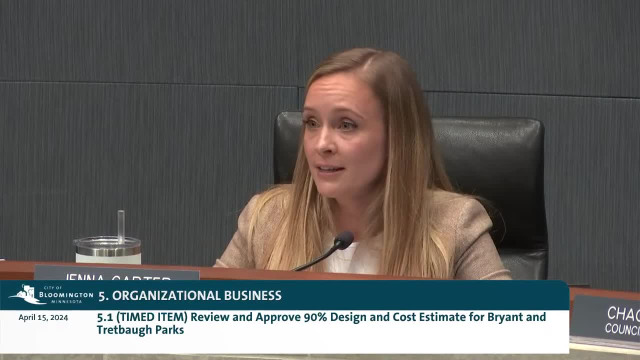 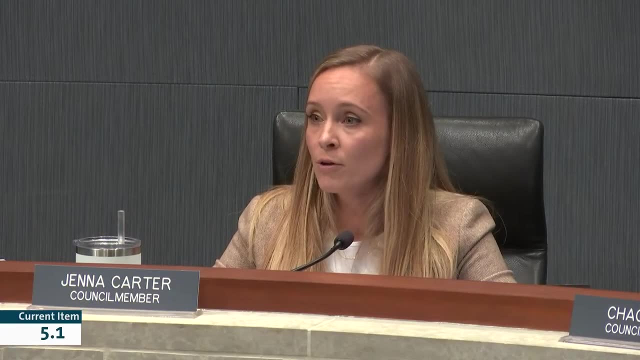 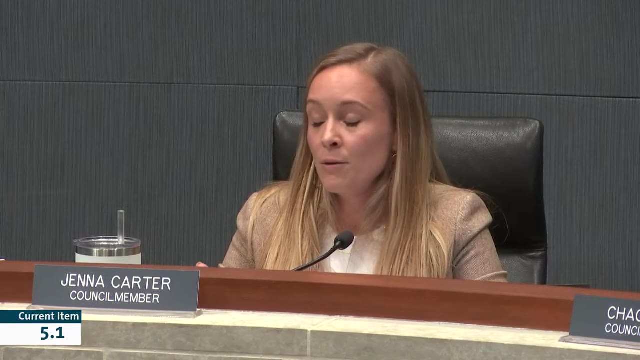 Also want to applaud you on this significant community engagement that occurred, the collaboration with internal and external stakeholders. Thank you, Thank you for having me on that And I think this really is remarkable and I think the product that we have, products that we have in front of us, really show like the most- I think that they're phenomenal products and outcomes. 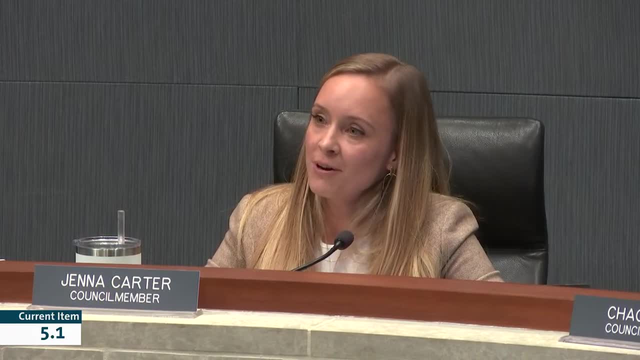 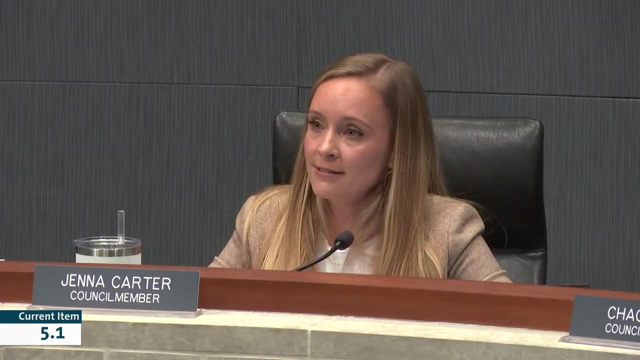 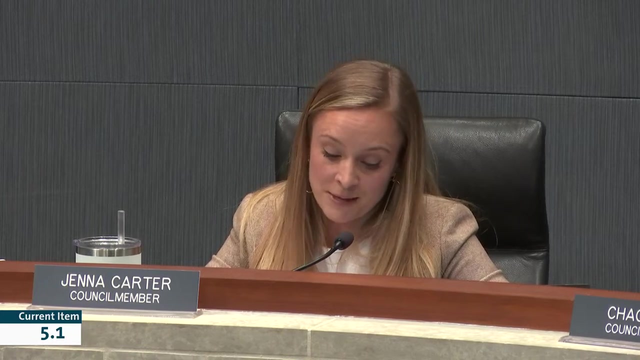 And so now we have two models to show the rest of the community- the whole community where we might be having future Park projects- at how this process works and that the outcomes can be quite significant in bettering the neighborhood and the community around. So thank you. 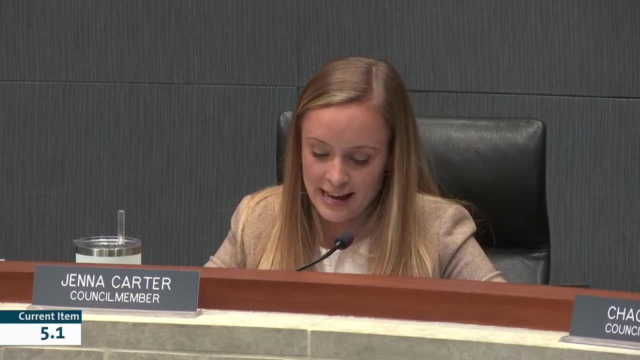 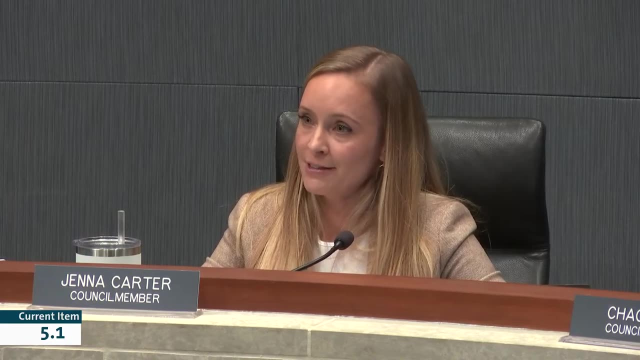 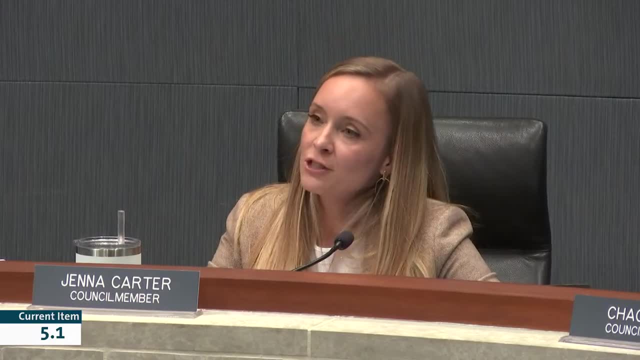 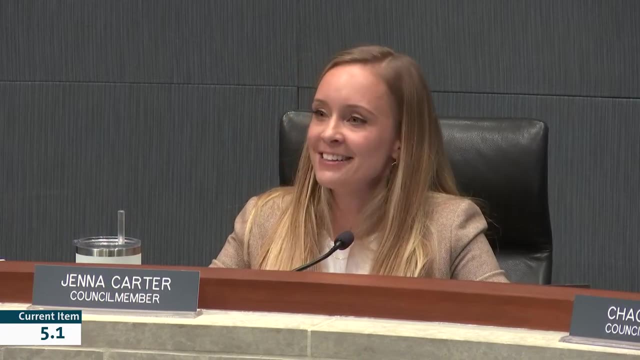 worry about them running all over the neighborhood. um, I just hope that it will be a nice fence. I mean, I'm thinking about some of the fences that we have in Bloomington, um, and I'm assuming that you've probably considered that and that's built into the cost, but I know that it can be a, you know a. 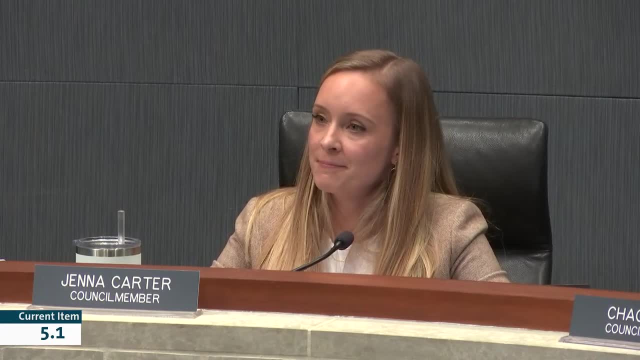 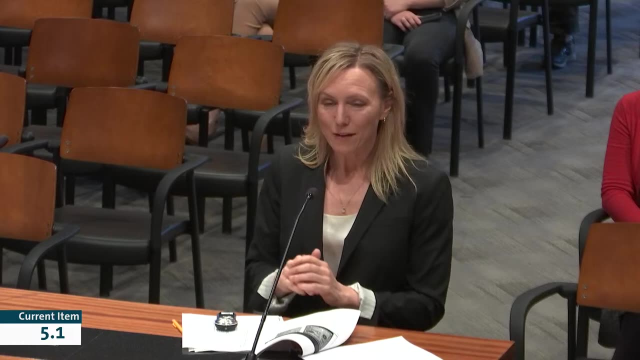 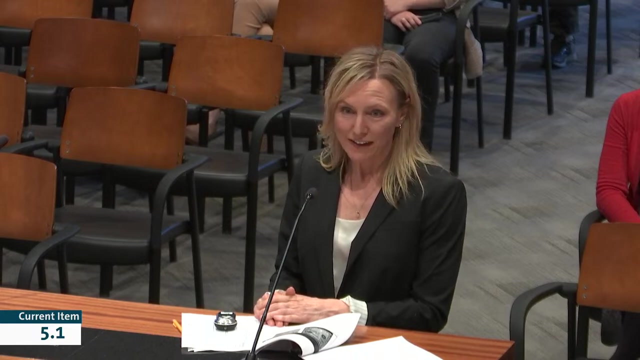 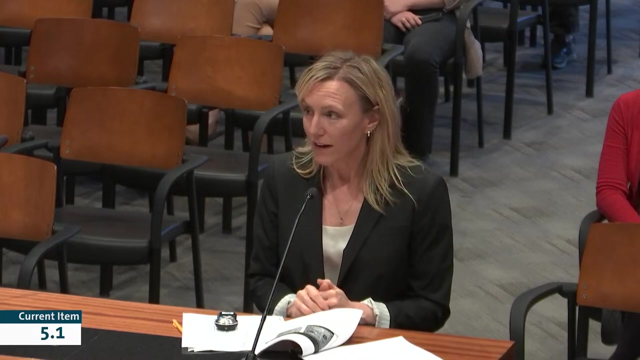 costly piece of infrastructure, but I would hope that it's um. I yeah, Mayor, Council Member Carter, the fence um currently in the specifications is a rubber coated black chain link fence that's three feet high. we are also um getting an alternative, um looking at an alternative rod iron looking. 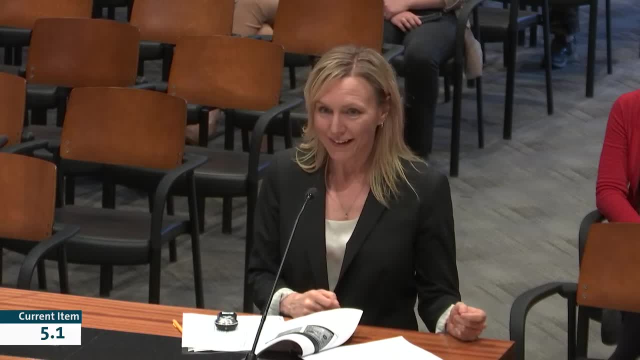 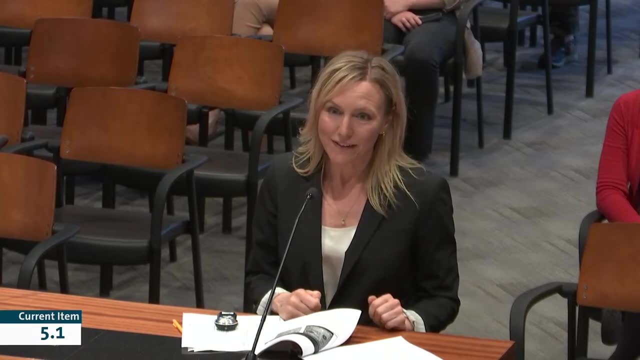 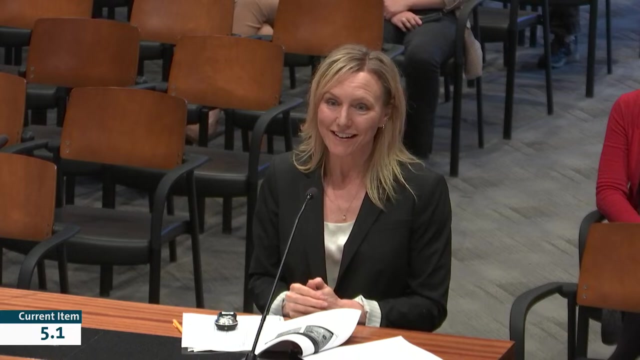 more decorative type of fence um pricing that out and evaluating if that can be an alternative, add in the bid or included in the base bid. so we are evaluate another option but the base option in the proposal tonight's a: the chain link black rubber coated. okay, the black rubber coating is at 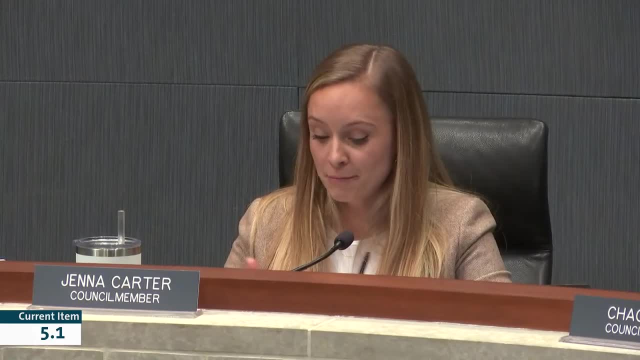 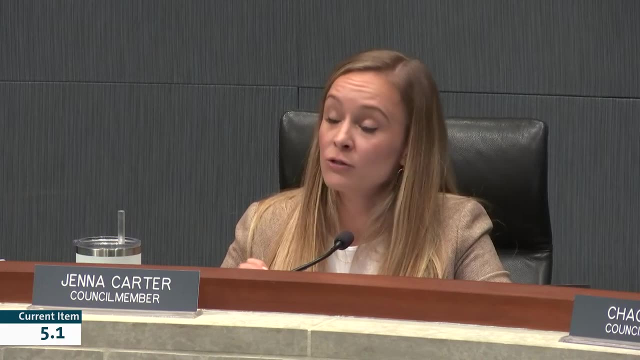 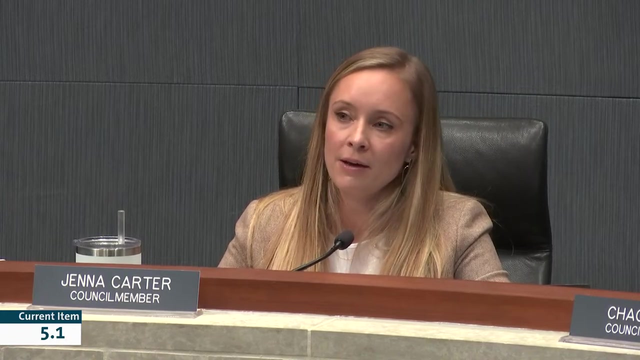 least a little bit better. but, um, I do. I would say I would prefer the other option. um, but other than that I don't have any additional questions. um, I also did want to say that I appreciate that the the park board is looking at additional options for dog parks and dog runs, because that is something that we hear about quite often in the community, totally understand the reasoning for not having one at. 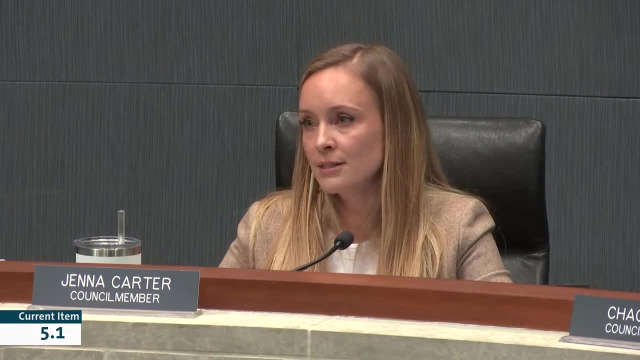 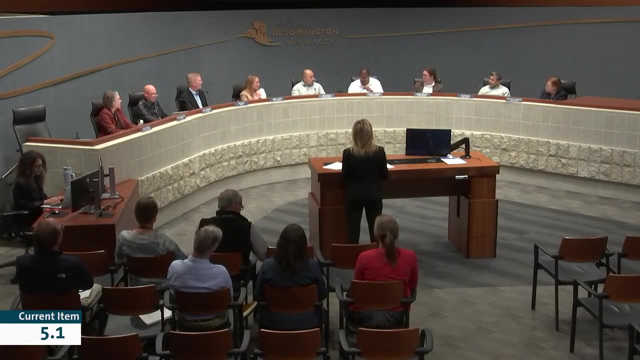 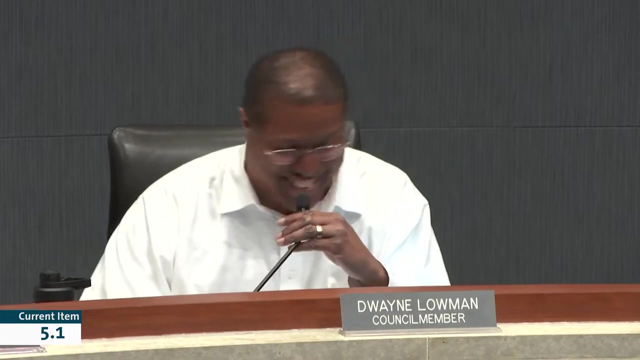 Tretbaugh, but um look forward to hearing options in the future, thank you. thank you, Council Member Lohman. well, Mayor, it's my understanding that the fence was going to be recycled from the Highland Greens area. I knew that was the shot. what? seriously? thanks Sean for that one. that was a good one. 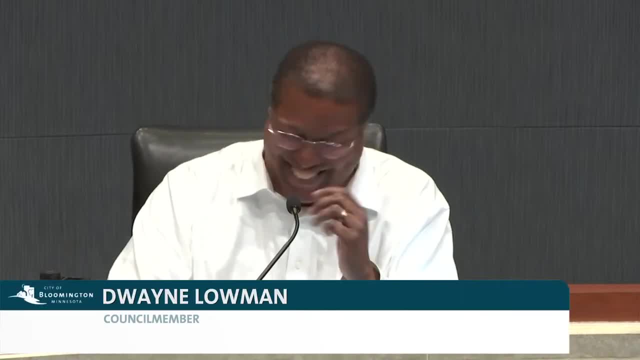 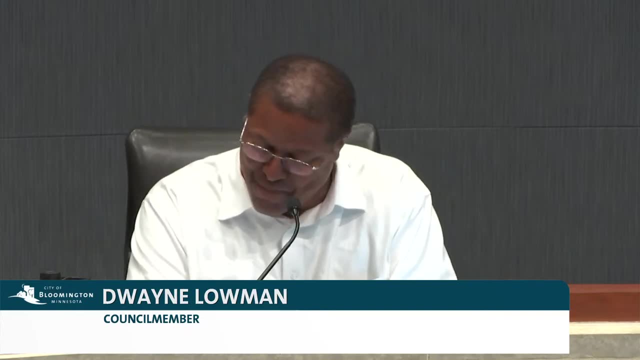 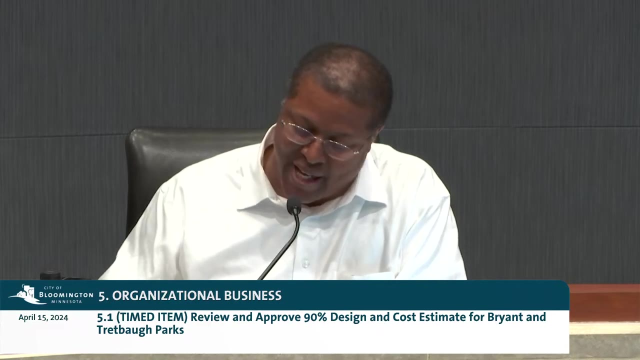 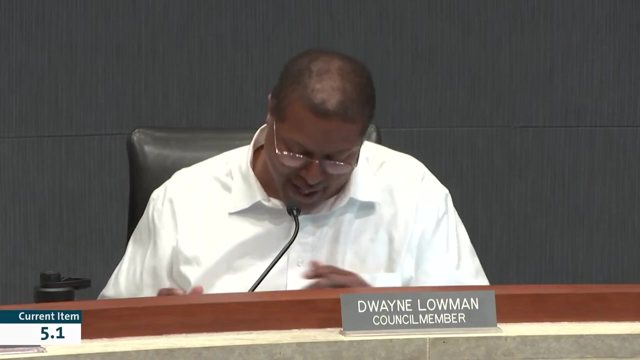 that was a good one, Sean. I like that one. um. so, as we look at this, Mayor, um, you know, in terms of this review and approval, the 90 present design piece, uh, you know, what are we looking to try to accomplish with this particular uh piece that we're doing here today? I've got 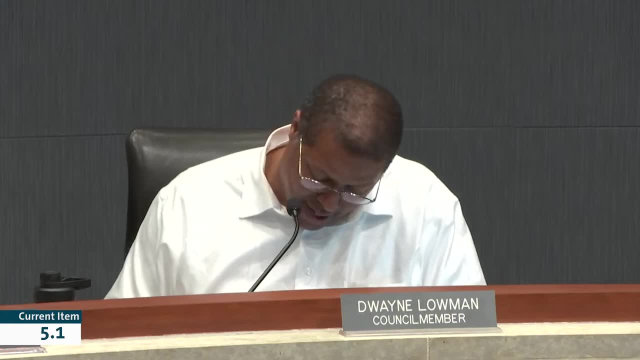 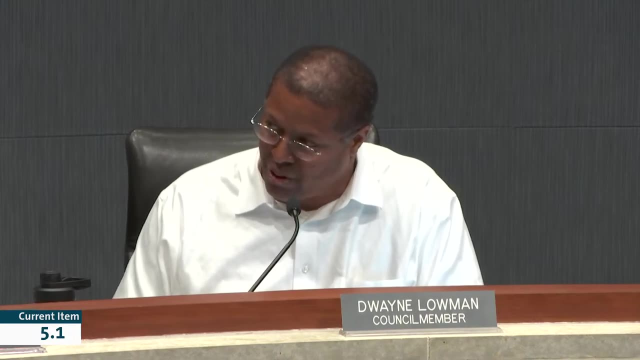 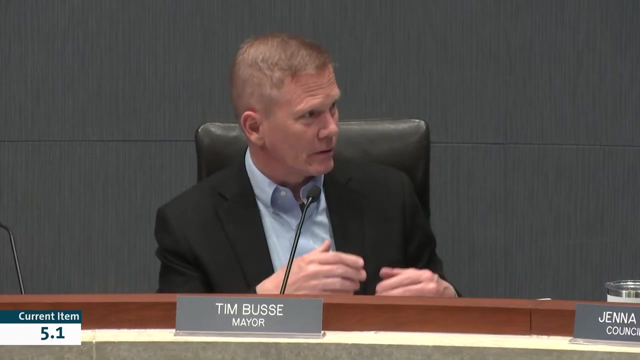 got some questions that are specific to this particular proposal. but I mean, those things can wait till later, but I just want to make sure exactly what we're trying to accomplish here with this particular motion, that we're trying to get accomplished today. Well, Council Member Lohman, I think, as we have done throughout this process, at the 30, 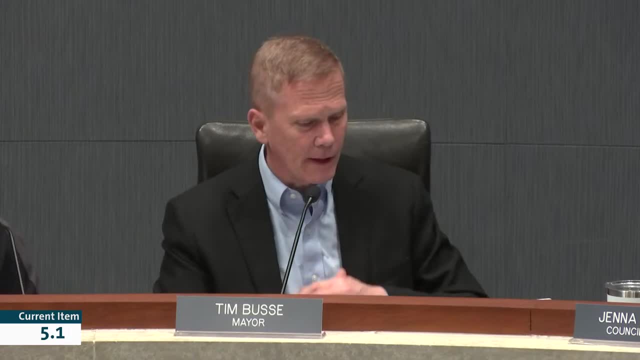 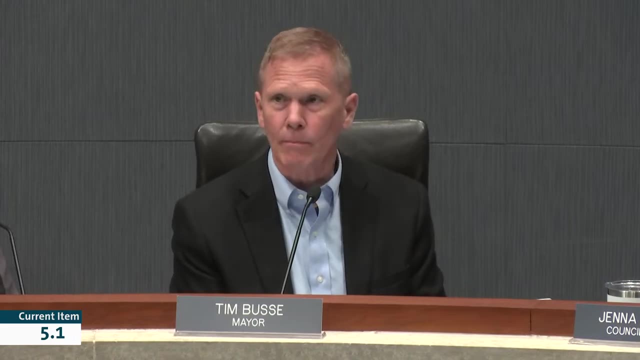 and I think did we did 30 in, Just 30. Just 30,. I'm sorry, I thought there was another one in between, but so, as we did at the 30% mark, to take a look at what staff is bringing forward, based on community input, based on the work, 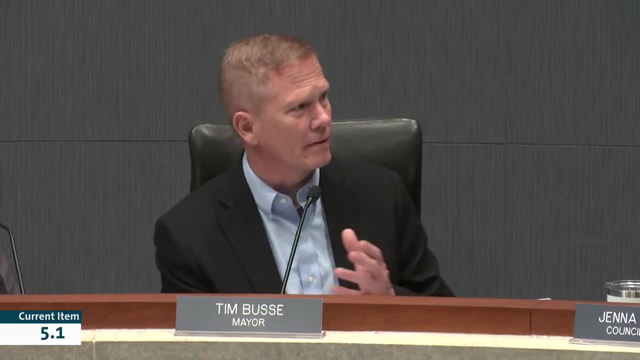 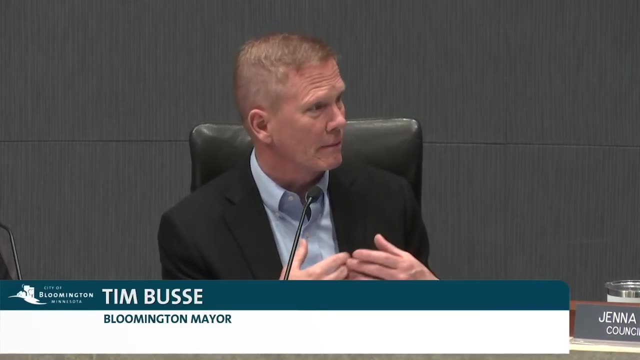 group that has worked on it, based on the budget realities, based on all the pieces and thought processes and the inputs that have gone into this. this is where they're at, and what they're looking for here is feedback from the council and then, ultimately, ideas. 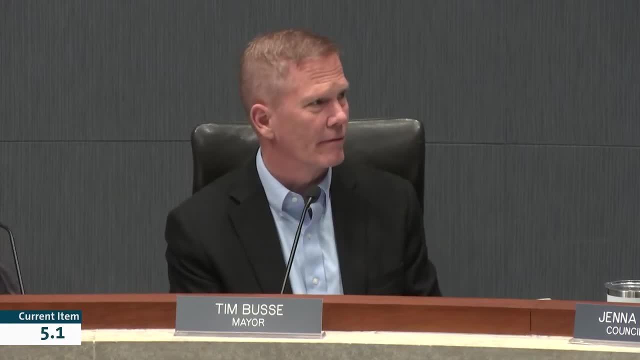 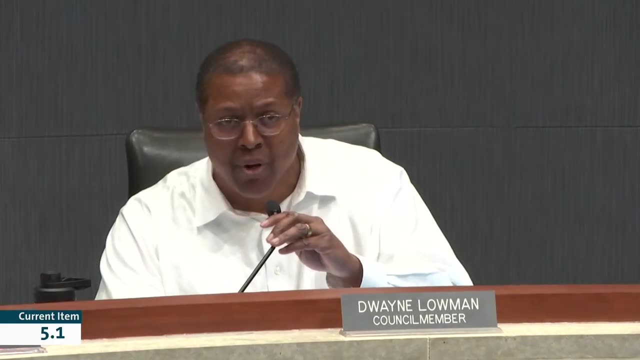 suggestions, possibilities, but ultimately a thumbs up or thumbs down on this level of design, with where they're at right now. So I think that's what they're looking for. Thank you for clarifying that, And so, with that in mind, Mayor, my 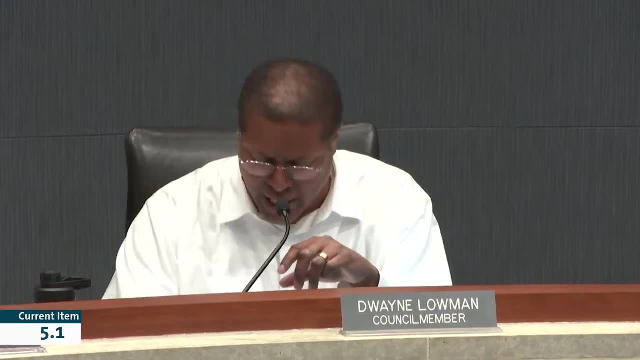 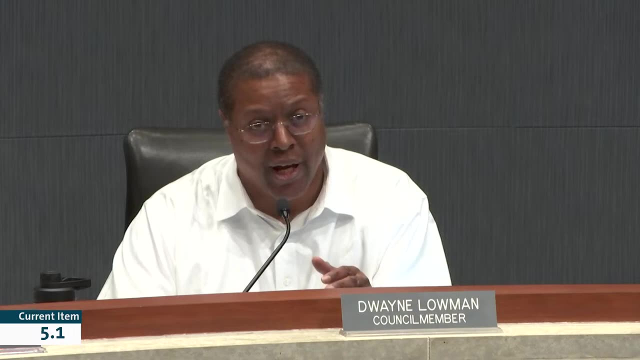 My only real question that I have. there's only these other ones I can ask you offline is: do you feel like, in terms of this proposal that you did both in the Bryant and the other park, that they're representative in terms of your civic engagement that you've had of 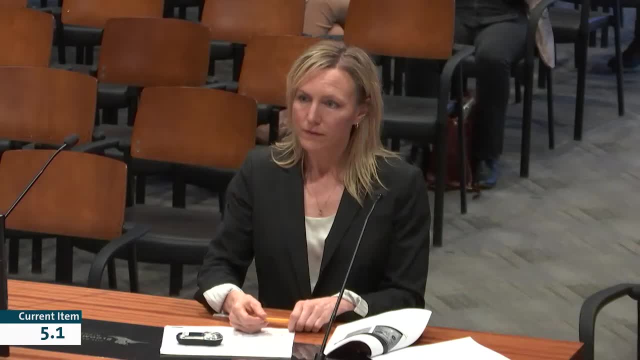 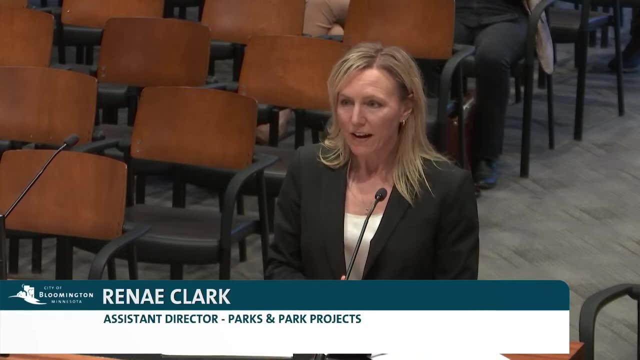 those folks that are going to be in those service areas? Mayor Blasey, Council. Member Lohman. members of council. thanks for that question. Staff and feedback from the park commissioners. Mayor Blasey, Council Member Lohman. members of council. thanks for that question. 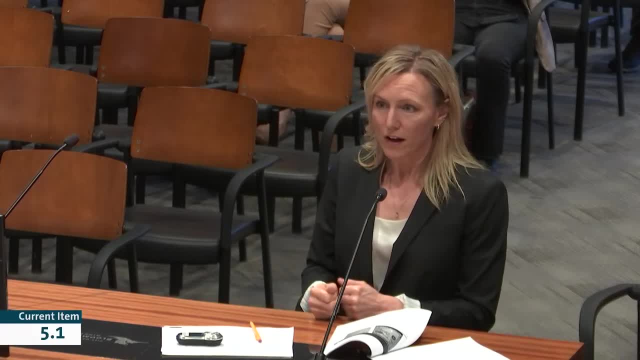 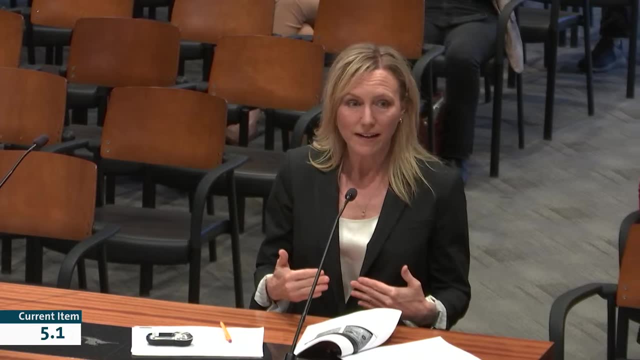 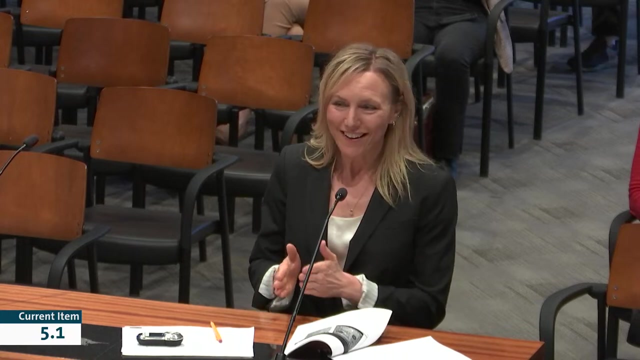 As we discussed this, are really proud of our design team and how they have listened and responded in several design iterations. I think Brian Park has been iterated on at each phase several times. With every comment we get, with feedback from groups and residents, we look to see how we 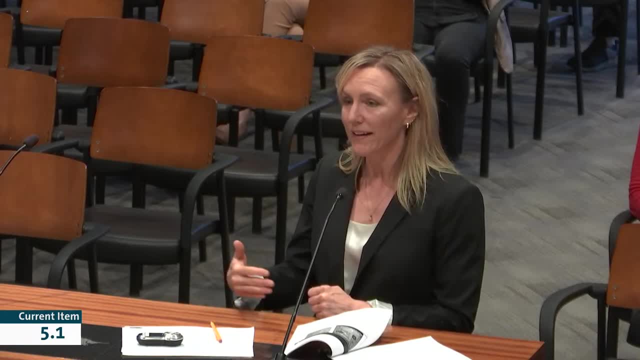 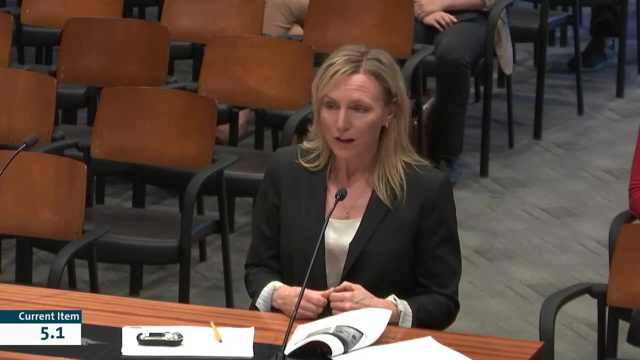 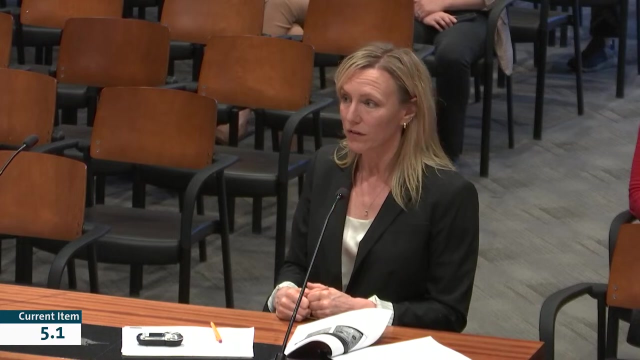 can respond in the design, how we can add clarification, how we can gain a better understanding of what we're hearing so that the designs can respond and staff feel really proud of these designs and our team in being able to respond high level to the priorities of our community, and even those 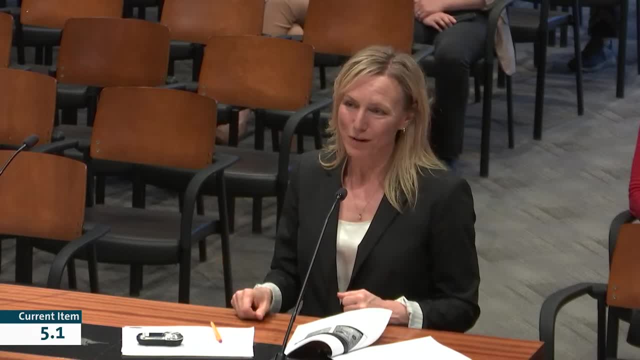 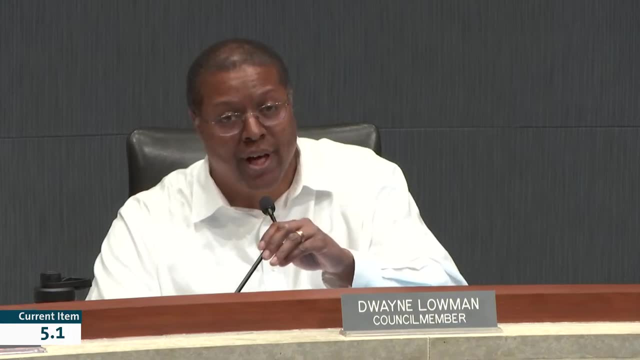 that we heard from our leadership group today, and then the specific park designs themselves. i i appreciate that and thank you, mayor, for that, because the thing that i have a question about always with that is that, as we look out many decades out, you know the things we do today. 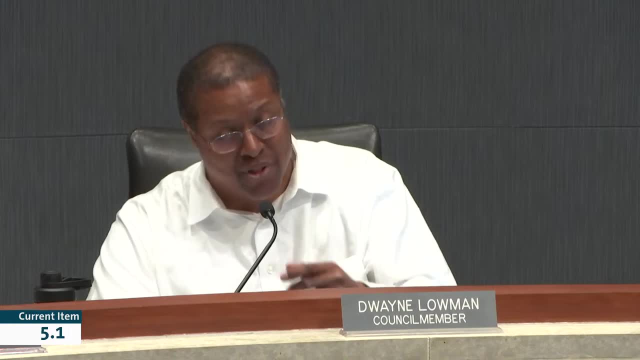 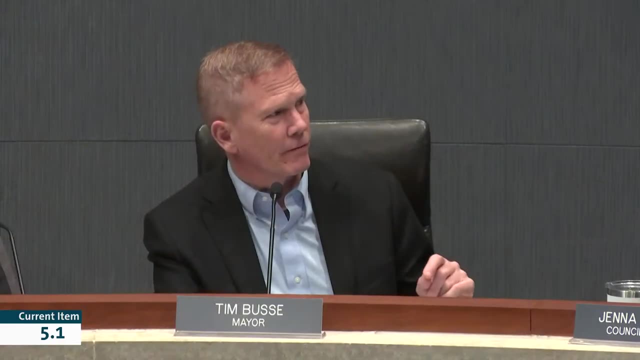 will have that impact, and so that's why i want to be sure that we're making sure that we're representative of those service areas that these parks lie in. thank you, which is a good point, council member, but understanding, of course, the reason we're doing this is because nothing lasts. 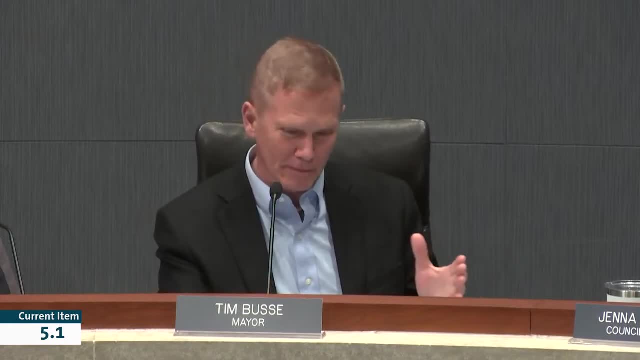 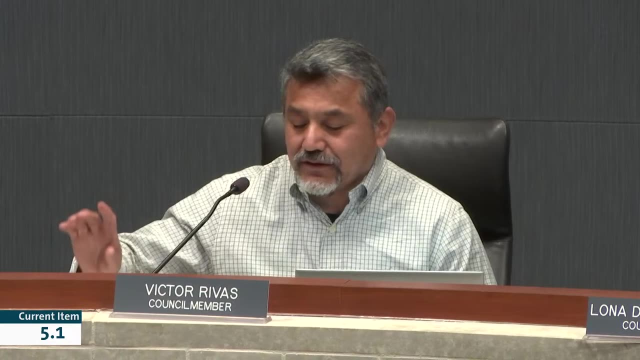 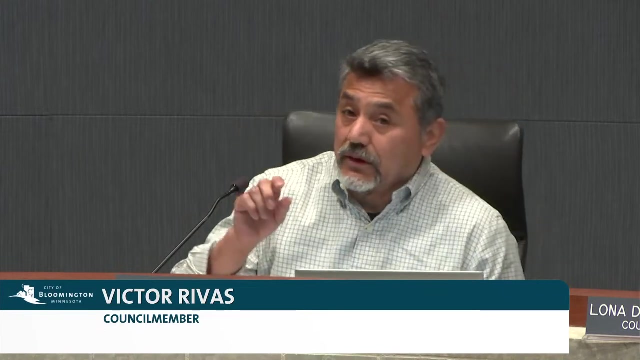 forever the. the community changes, the needs change, and so then, but i appreciate your point. council member rivas and council member d'alessandro. council member rebus. i just have a couple of quick questions. uh, in regards to the gender neutral bathrooms, would they be of private use or a more? 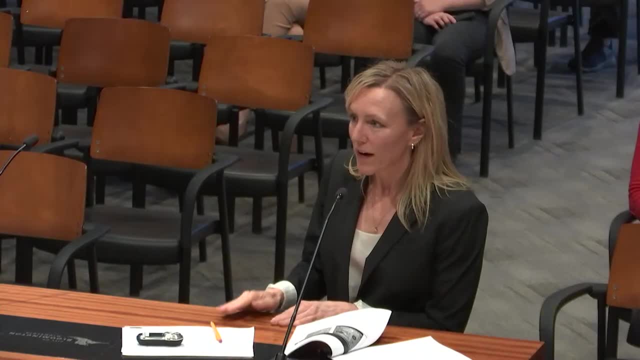 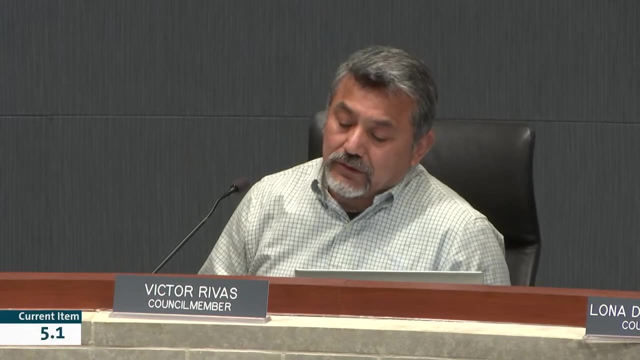 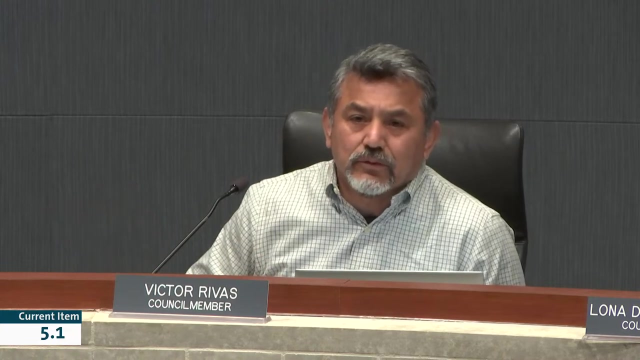 than one user at a time, single private use. okay, that's one question, and the other one is: would it be possible at all to get some of that community input for those parks? as you realize, i'm new here. i might, everybody might have that information, but i would like to read some of the information. 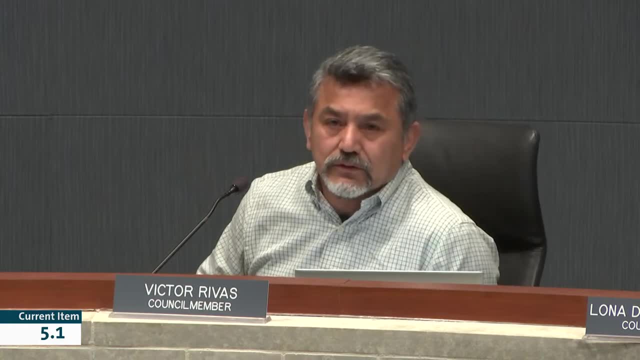 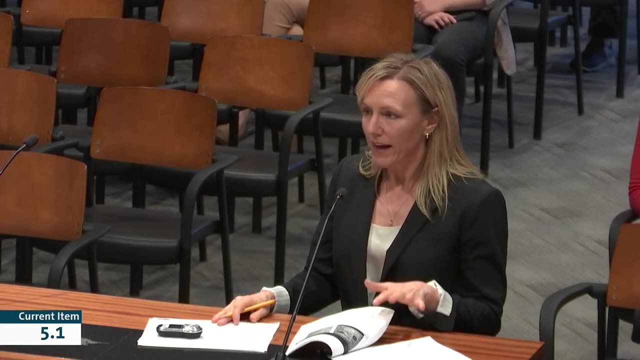 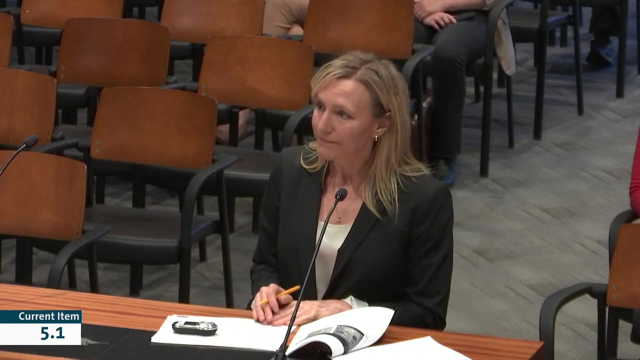 some of the input that the committee has put into the design of these parks, if that's possible at all. mayor, members of council, i can certainly share that. i provided a really high level brief summary of some of it in the packet tonight, but i will, um, i can share more of that. that would be. 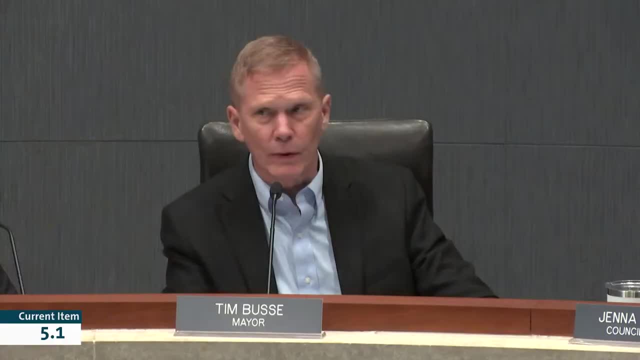 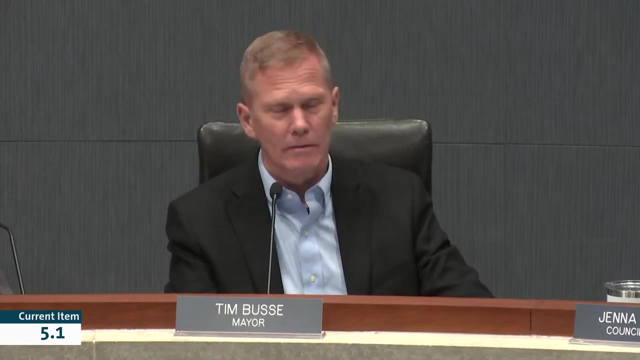 awesome. thank you, and i will say council member rivas: we we heard a number of times at listening sessions from representatives that 230 the cityいい proszę то. we heard for the last council year OF THE NEIGHBORHOOD FROM AROUND BRYANT PARK AND UH GOT GOOD, GOOD FEEDBACK IN THE LISTENING SESSIONS. 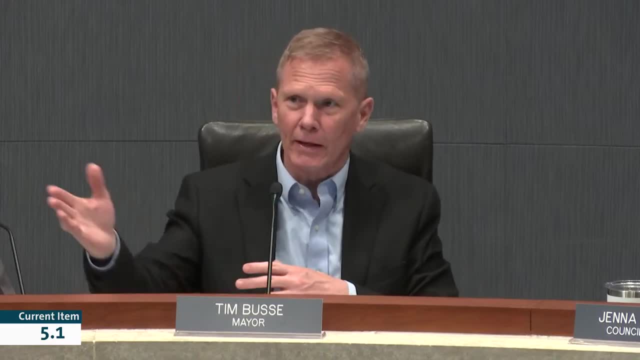 AND THEN USUALLY AFTER THE LISTENING SESSIONS, I THINK, RENEE AND AND SPENT A CONSIDERABLE AMOUNT OF TIME JUST TALKING AFTERWARD AS WELL. SO THERE'S SOME STUFF THAT. I KNOW IS WRITTEN, BUT I KNOW. 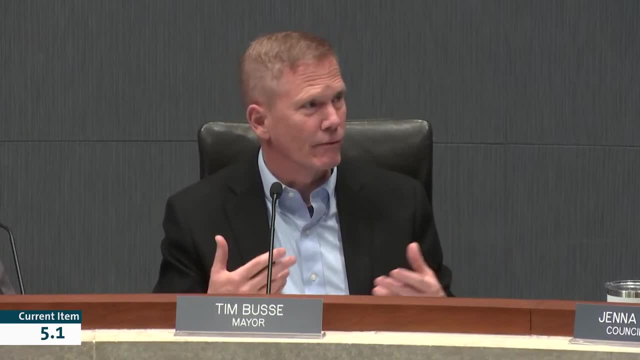 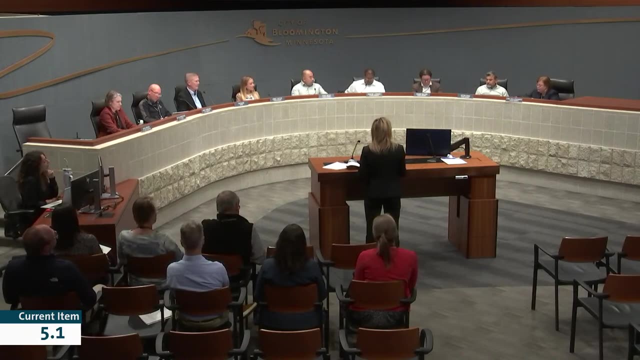 THERE'S OTHER STUFF. THAT HAS JUST BEEN THE FEEDBACK FROM THE COMMUNITY UH VERBALLY AND AND THE SHARING OF IDEAS BACK AND FORTH, COUNCILMEMBER D'ALISANDRO. THANK YOU, MR MAYOR UH. I AM SUPER EXCITED ABOUT. 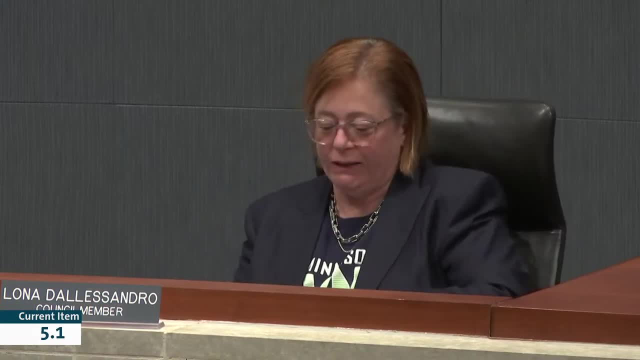 THIS AND UM AS WE GET CLOSER TO ACTUALLY, YOU KNOW, PUTTING THAT SHOVEL IN THE GROUND UH, SO THANK YOU FOR ALL YOUR WORK. EVERYBODY INVOLVED IN IT- UM, I'M ESPECIALLY EXCITED TO SEE THAT. 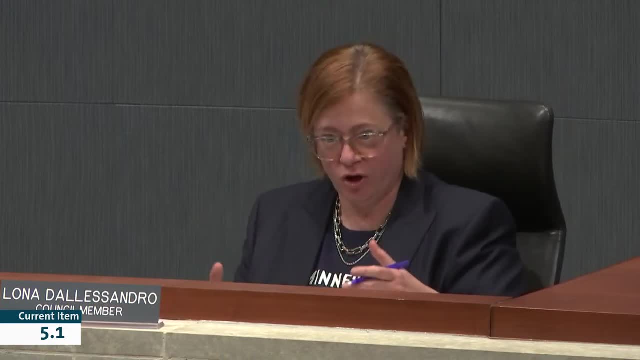 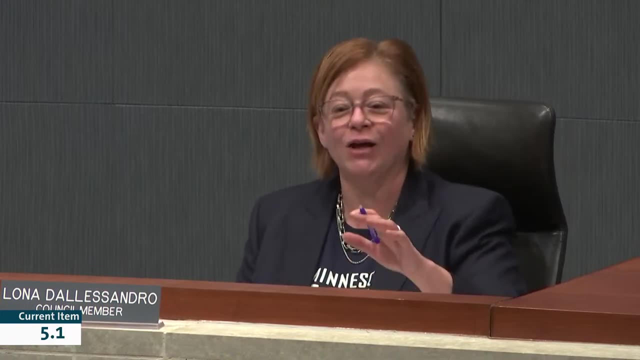 WE COULD BUILD IN UH SOME OF THE SUSTAINABILITY INITIATIVES THAT YOU TALKED ABOUT UM. I MYSELF AM ON A TENURE PLAN TO GET UH TO GET MY PAYBACK ON MY SOLAR PANEL, SO I I'M 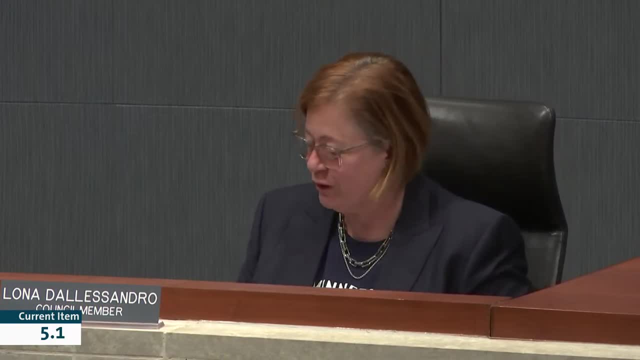 I KNOW IT CAN BE DONE, SO I'M EXCITED TO SEE YOU ALL TRYING FOR THAT. THANK YOU FOR DOING IT, UM. I HAVE A QUESTION ABOUT SO UM, AS YOU ALL KNOW, UH ESPECIALLY WITH BRYANT PARK SINCE IT'S. 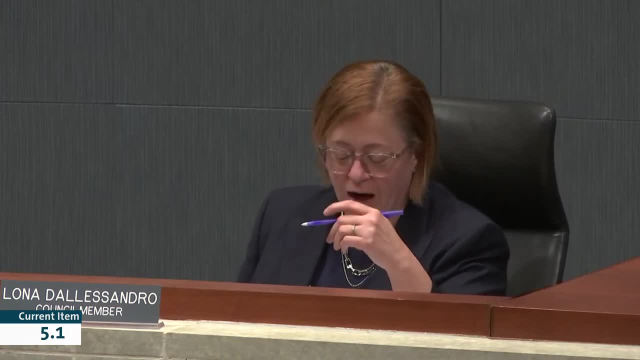 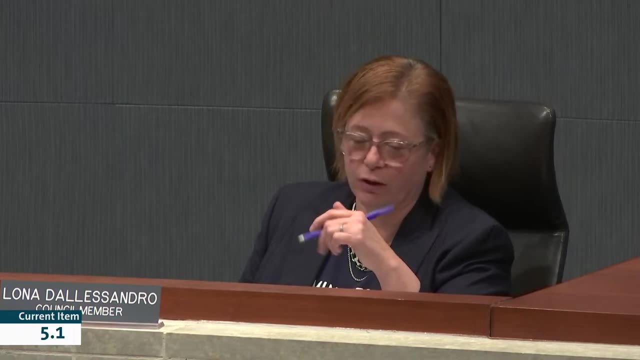 AT MY HOME PARK. I WAS UH ESPECIALLY INVOLVED IN THE COMMUNITY OUTREACH ASSOCIATED WITH THIS MY. MY QUESTION IS: UM, IF WE, IF WE THOUGHT ABOUT YOU KNOW THIS UM WITH ALL THAT FEEDBACK WAS THERE. 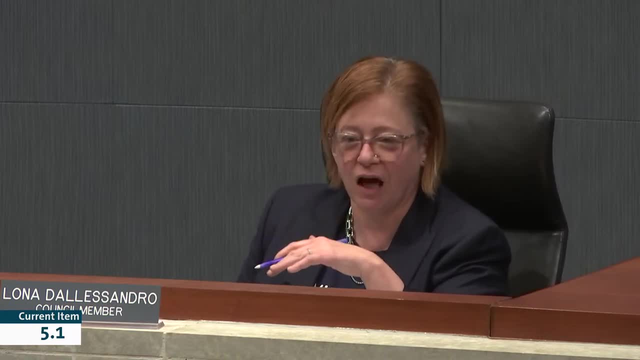 ANYTHING THAT WAS JUST BELOW THE SURFACE, LIKE THAT JUST DIDN'T MAKE THE LINE THAT IF WE, YOU KNOW, AUTHORIZED ANOTHER 25K OR ANOTHER 50K OR SOME YOU KNOW, IN THE SCHEME OF THINGS SMALLER AMOUNT COMPARED TO THE 9 MILLION, WE COULD GET DONE AND DID DID. WE HAVE THAT CONVERSATION. 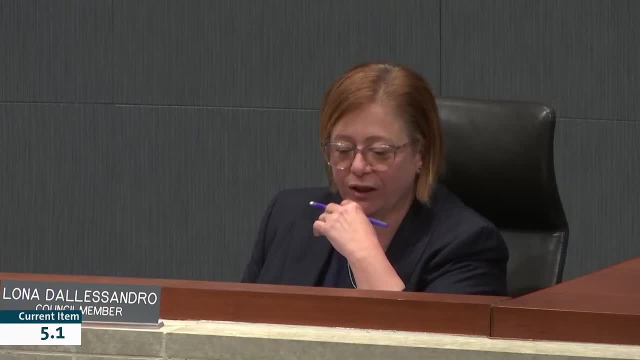 BASED ON UM, THE, THE FEEDBACK THAT WE GOT. I'M JUST KIND OF CURIOUS IF THAT PROCESS EXISTED BECAUSE IT'S IN IT'S GOT TO BE VERY DIFFICULT TO LIKE, DRAW THE LINE AT SOME POINT AND SAY OKAY. 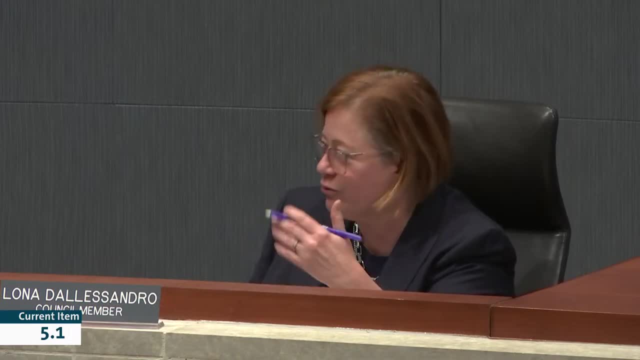 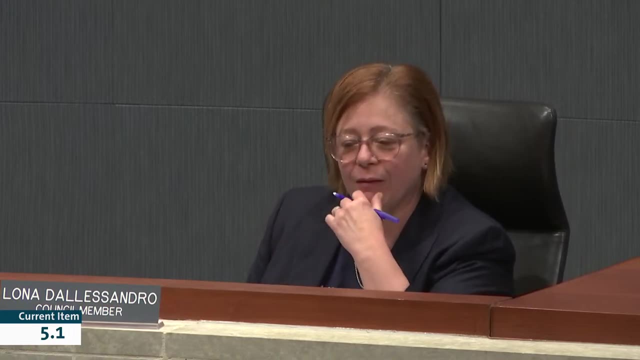 WE'VE GOT TO CUT YOU OFF, OTHERWISE ALL THE WE GET FEEDBACK FOREVER RIGHT. SO I'M JUST KIND OF CURIOUS, IF, IF YOU CAN HELP US UNDERSTAND AT WHAT POINT- MAYBE YOU KNOW, I'M THINKING SPECIFICALLY ABOUT. 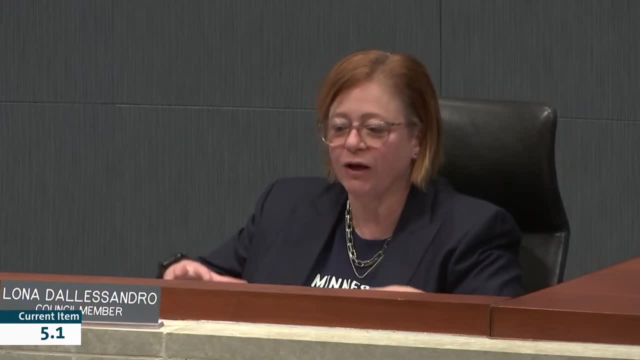 SOME OF THE CONVERSATIONS THAT HAD ABOUT UM. YOU KNOW THE PLAYGROUNDS LOCATION AND THE RESIDENTS AND THE NOISE ASSOCIATED WITH THAT AND WHAT WE'RE DOING TO MITIGATE UM OR SOME FOLKS MENTIONED THAT. 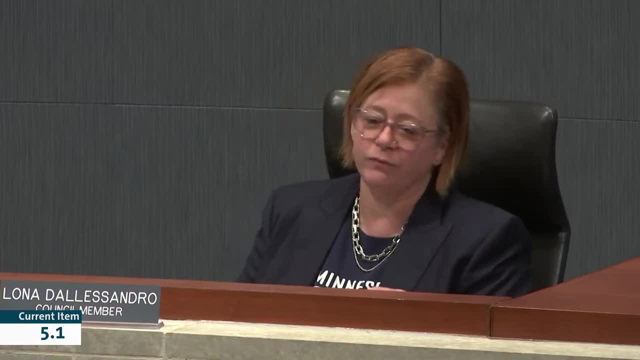 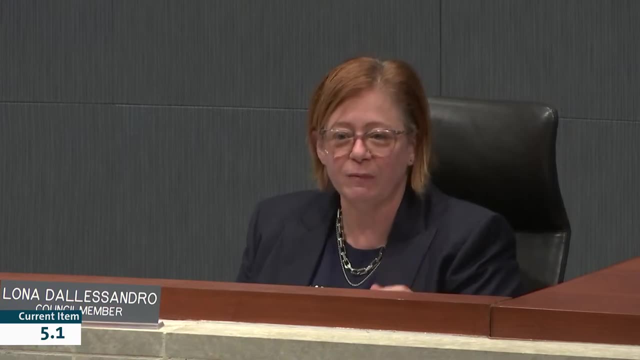 THEY LIKE TO HAVE A SECOND UM BALL FIELD UM. YOU KNOW UM I FOR ONE AM THRILLED ABOUT THE FACT THAT I CAN ACTUALLY GO AROUND THE PARK NOW WITHOUT WALKING THE STREET. THAT'S EXCITING UH. BUT OTHER PEOPLE MIGHT HAVE PREFERRED TO HAVE UM LESS WESTERN PARKS, AND I THINK THAT'S EXCITING, BUT OTHER PEOPLE 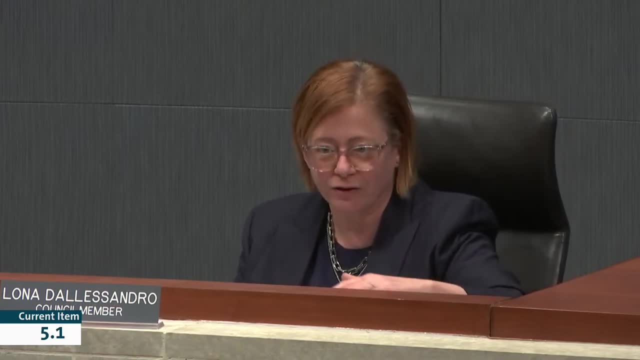 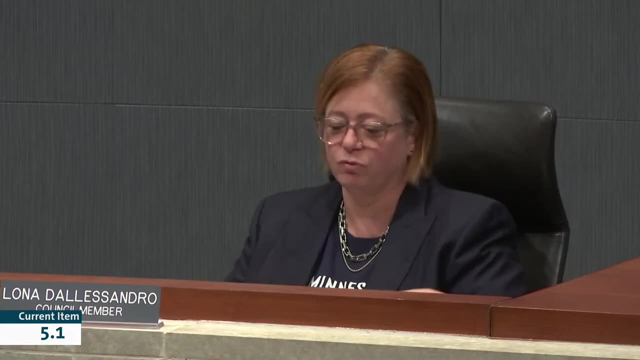 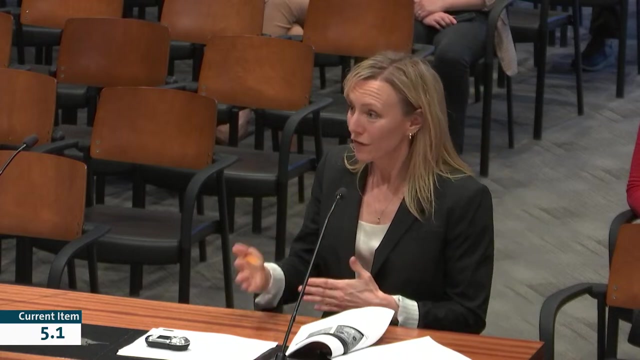 MIGHT HAVE PREFERRED TO HAVE UM LESS WETLAND ON THAT UH, ON THAT NORTH SIDE, FOR EXAMPLE. HELP US UNDERSTAND WHAT YOU MIGHT HAVE GONE THROUGH TO KIND OF- I DON'T KNOW DRAW THOSE BOUNDARIES. THANKS, MAYOR COUNCIL, MEMBER DELAZANDRO AND MEMBERS OF COUNCIL. THANK YOU FOR THAT QUESTION. IT WAS A. 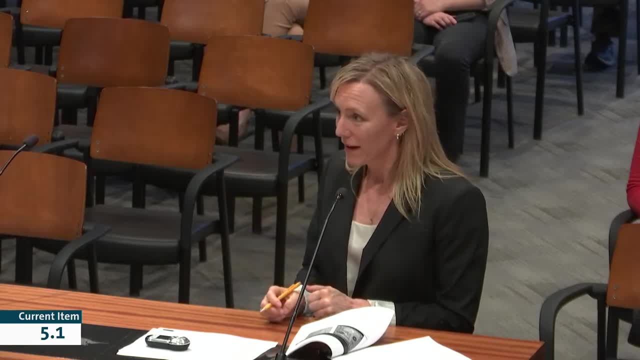 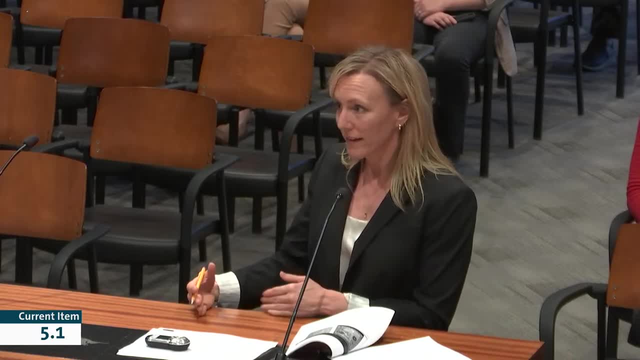 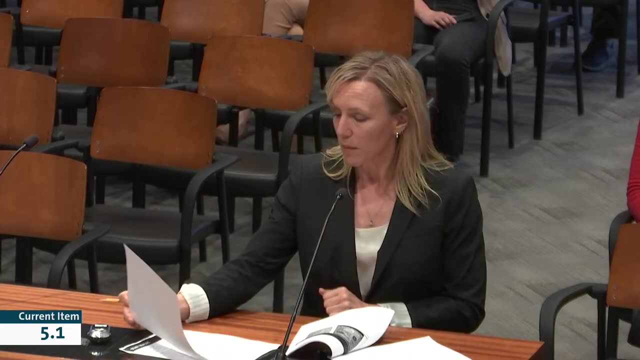 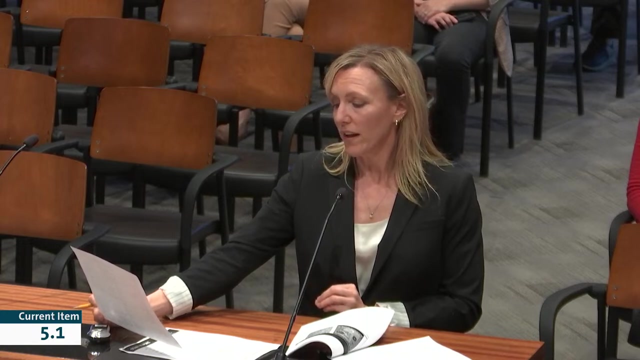 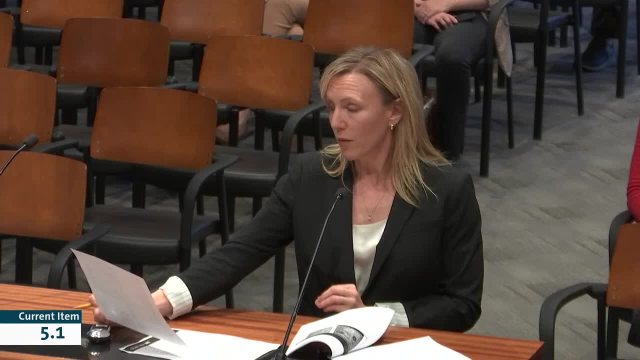 PUBLIC ART IS CURRENTLY UM. WE EARMARKED FROM DAY ONE UH 75,000 FOR TREPA PARK AND 200,000 FOR BRYANT PARK. THOSE NUMBERS ARE RIGHT. NOW I'LL CALL IT BELOW THE LINE IN THE ESTIMATE BUT. 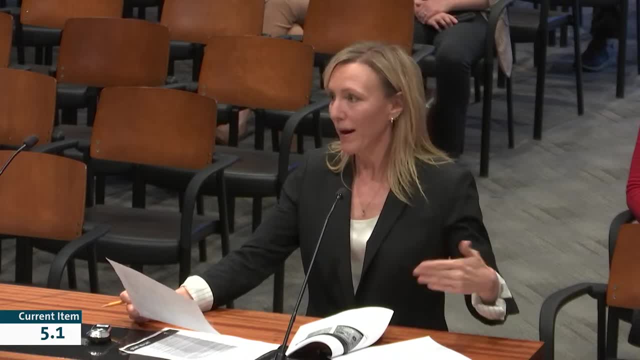 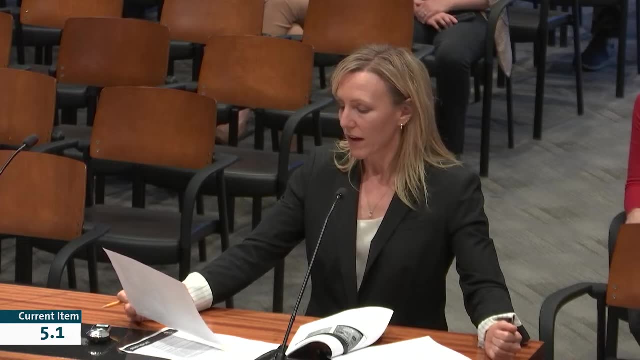 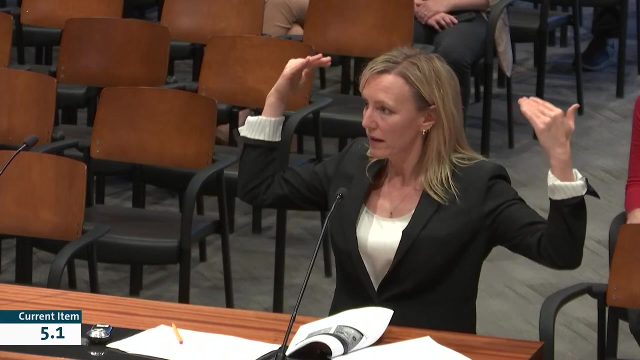 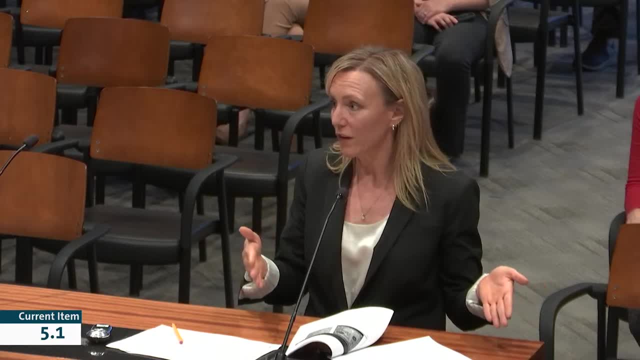 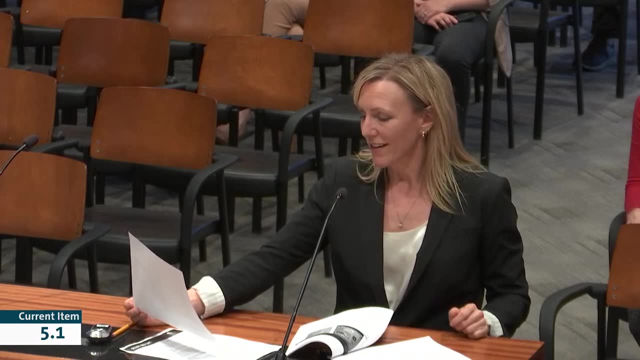 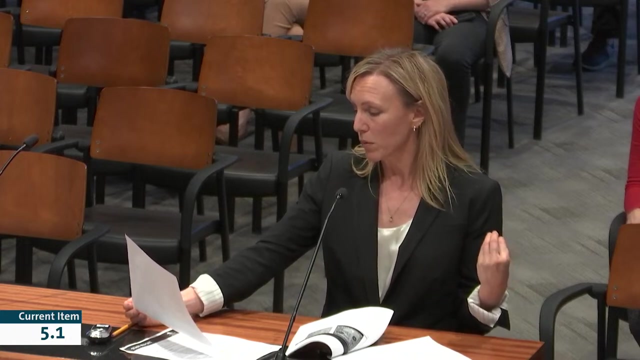 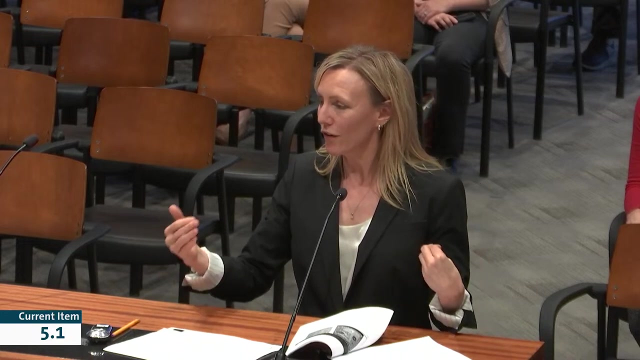 structure. Trepoff for gathering, I think is more important. Brian Park has one too. Those are below the line. and then options for Kind of recreational things- block seating, hammock lounges- below the line on Trepa, Things that we can look at to based on bids: leave in or keep out. 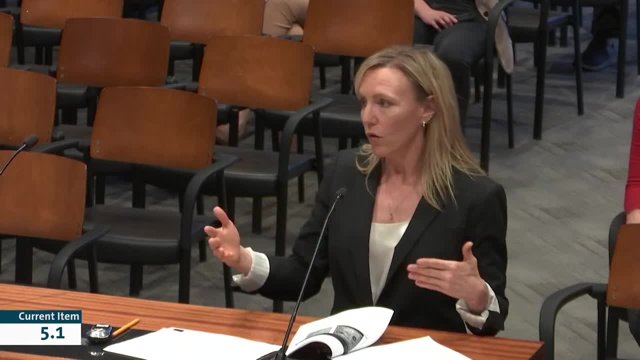 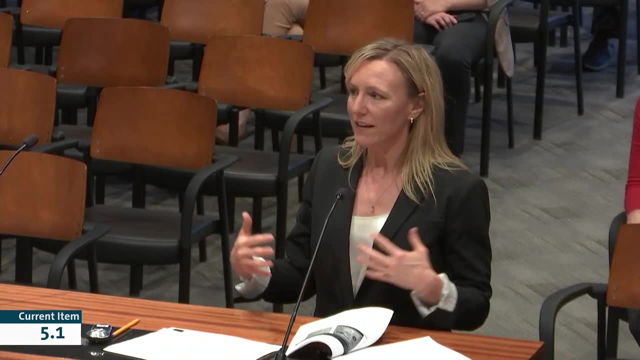 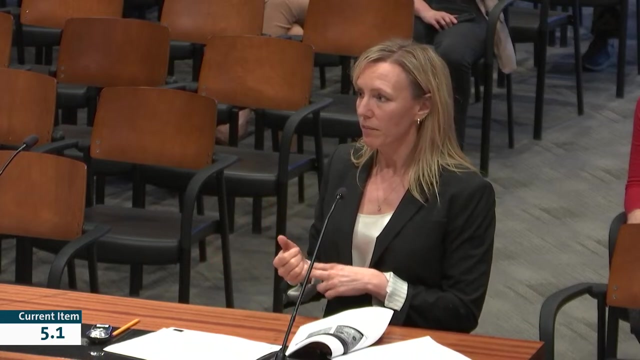 To stick within that budget. So some smaller things like that with respect to the community, I I don't. I can't recall something big that we're missing. We did hear from the neighbors. I think a couple of themes towards the end were The big change. people will see out their window on the more active side, apart of the park along Bryant. 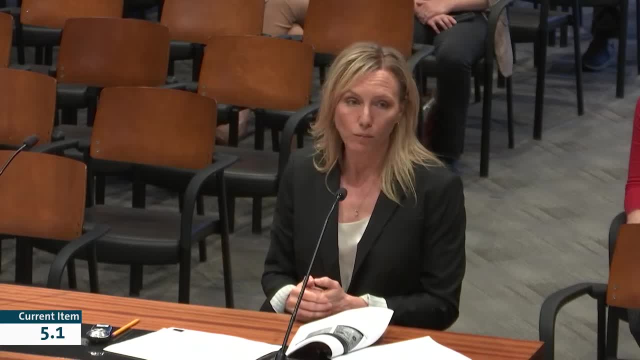 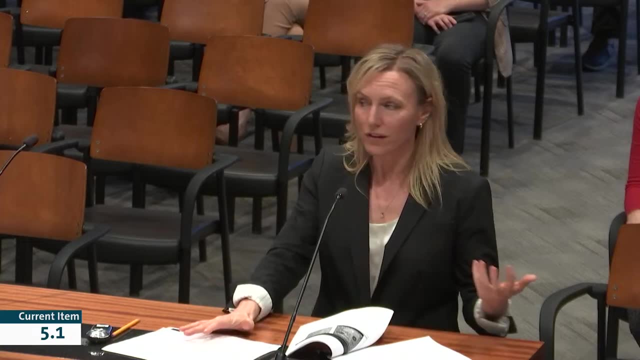 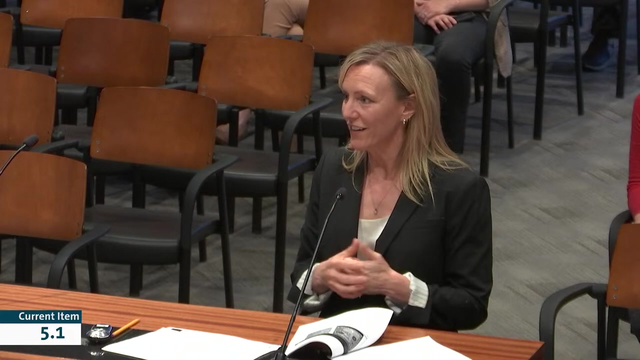 screening and trees Were really important There and we use that to them to mitigate and I feel, And the colors of the playground were chosen to try to be respectful of those concerns and Then we really weren't able to mitigate the concern of this is a lot of stuff in. 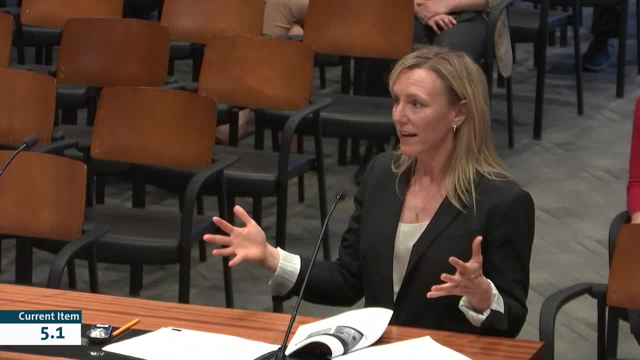 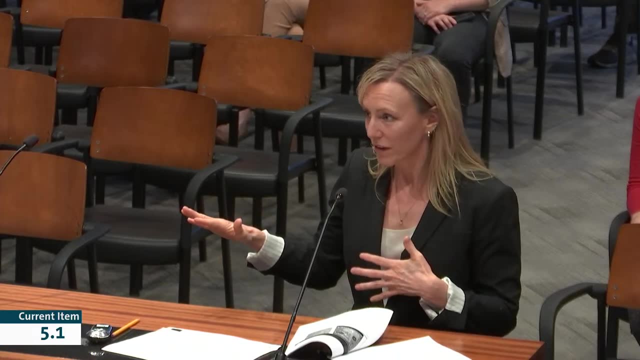 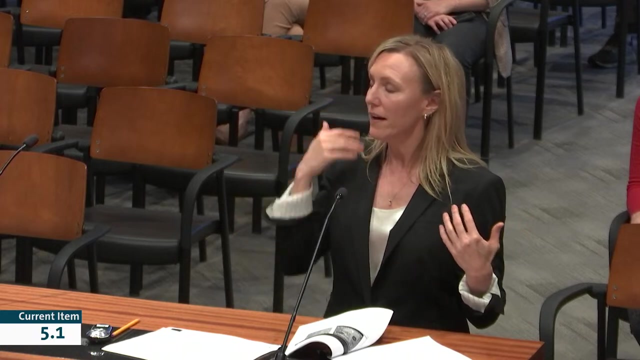 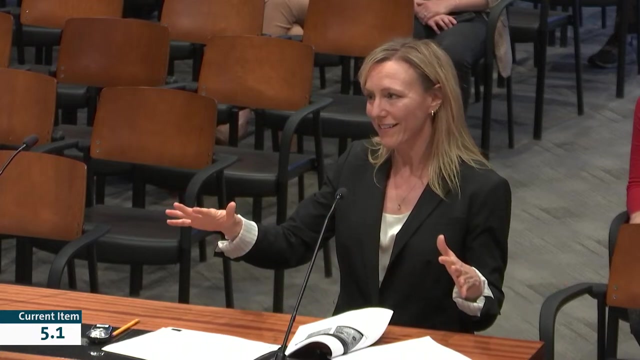 the east side of the park and By design, I mentioned the parks in the hundred-year floodplain, that area, the park, is least susceptible to flooding, still potentially subject to flooding under, you know, a hundred-year storm. But based on how the parks flooded in the past and how the parks being graded where that active play area really is today and is, 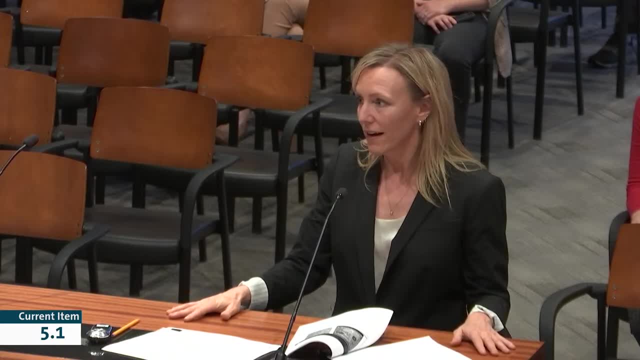 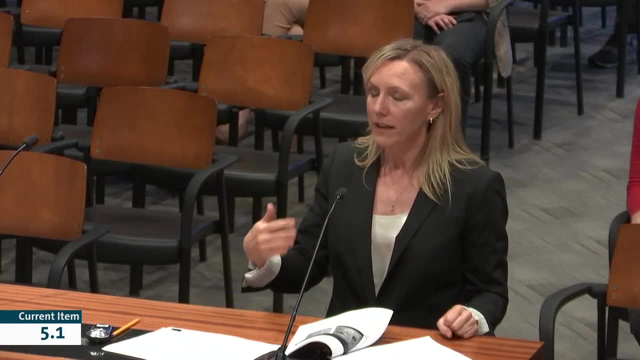 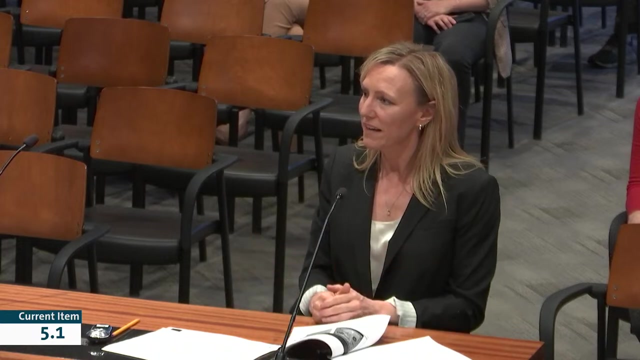 Remaining is because it's least susceptible to flooding. Then there's the ball field, and then there's the natural area that we really can't develop. So those were kind of the two that weren't, You know, fully mitigated As part of the design. I can't think of something big that we didn't include that. 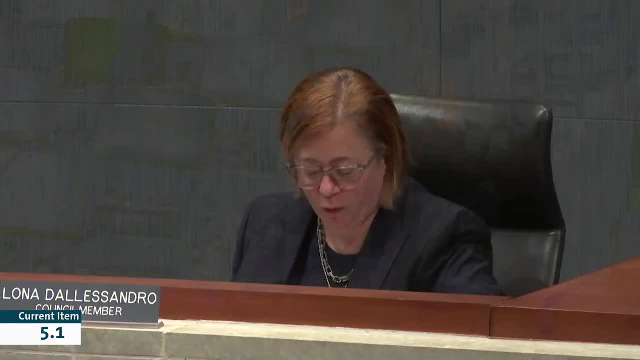 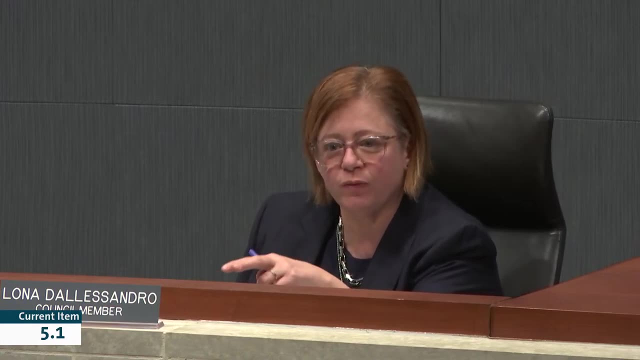 We. that was requested. great Thank you. I have two really quick questions, Hopefully, first of all related to the bathrooms. I noticed on the plan to face outward and to face inward. I assume that means that Those outward facing bathrooms will be opened at What time in the morning and closed at what time at night on a regular basis, so that they're accessible. 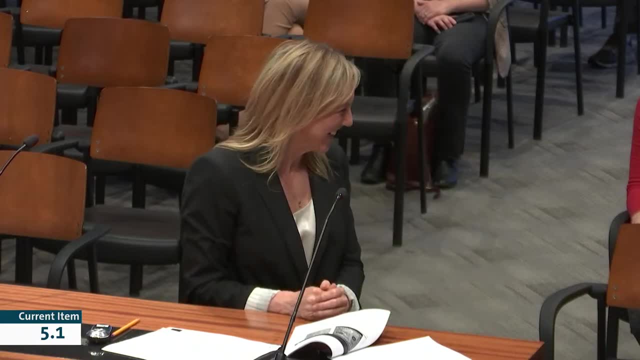 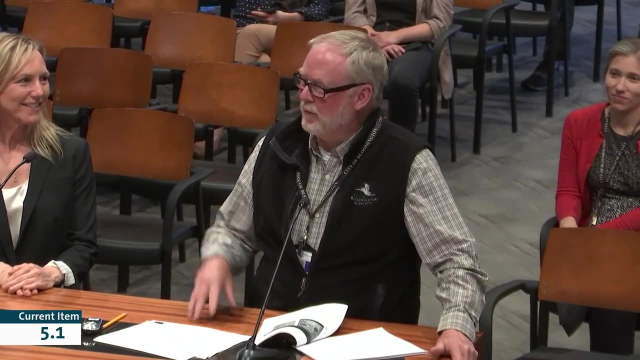 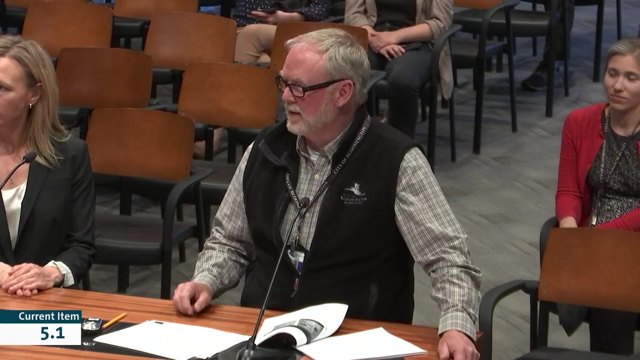 Council members. I'd like to defer that. Good evening mayor, council members. council members. We typically have those on auto locks and they're open during normal park hours, So 6 in the morning till 10 at night, and that would be 20 like 365 days a year. Yeah, okay, great. 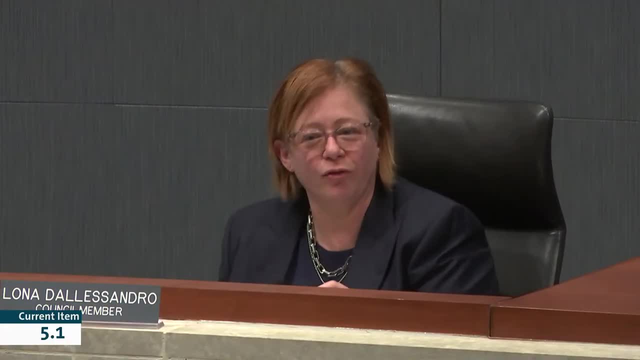 second quick question- hopefully- And I don't think I'm gonna be asking you a question date, but hang in there just in case- the Parking lot. I know one of the biggest questions we had about co-locating the parking lot to the playground was because of the 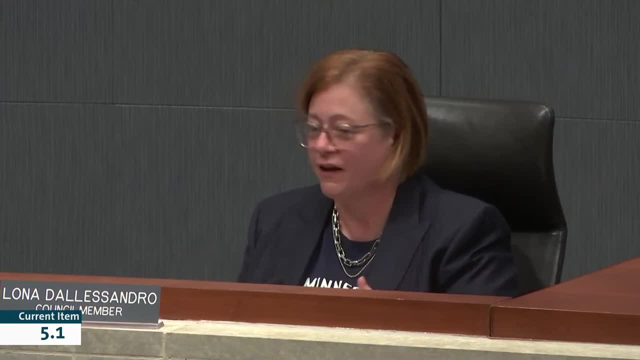 Folks using mobility Aids and vans and other things like that to have folks with with mobility issues have access to the playground a little bit more successfully. Did we read it looks like we reduced the number of total spots In that parking lot as well. How many are dedicated to handicapped parking? then there are disabled parking and then are we going to enable 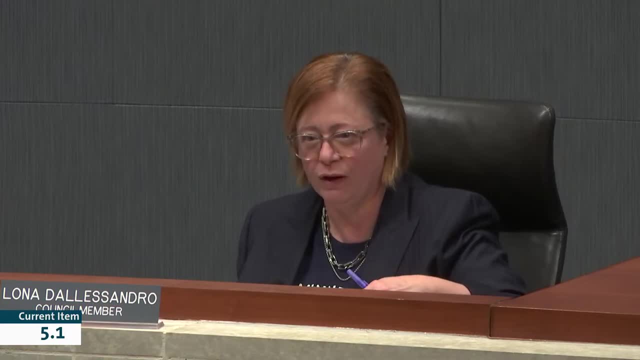 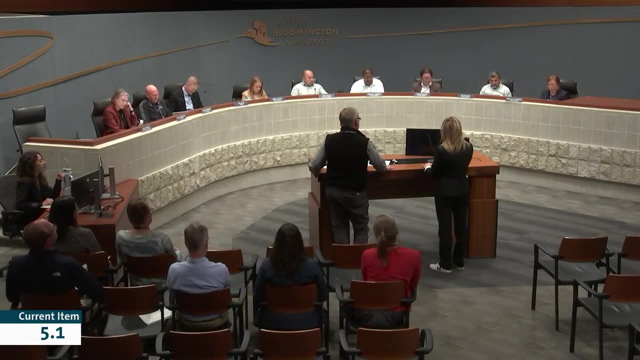 Some street parking. I think it's already available in that area, but are we gonna enable some street parking along there as well to to manage any kind of, like you know, tournaments or Other things where you know more than the number of parking spaces might show up? 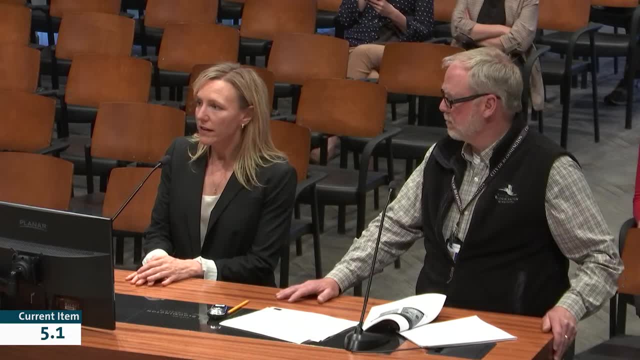 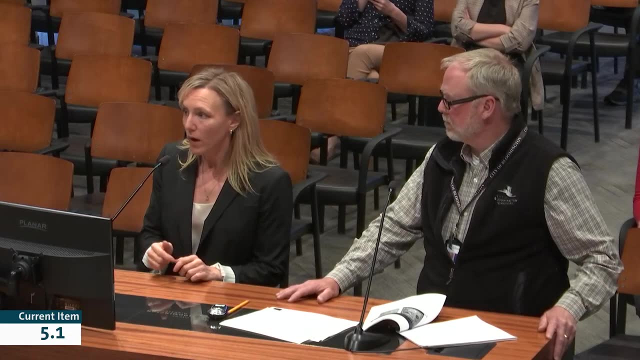 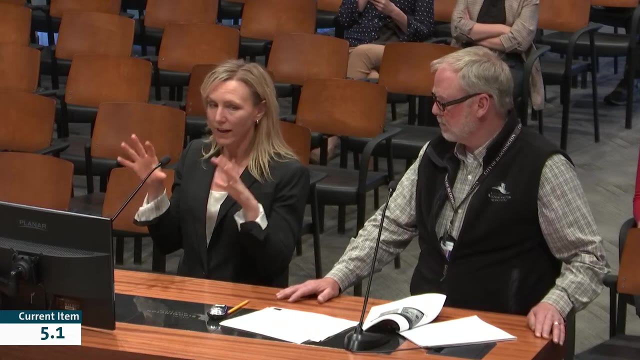 Mayor, members of council, councilman del Sandro, the number of spaces in that parking lot is actually increased a bit. There is street parking all the way around the park. in general, the number of parking spots Combined on the street and in the lots is increased by about 10. 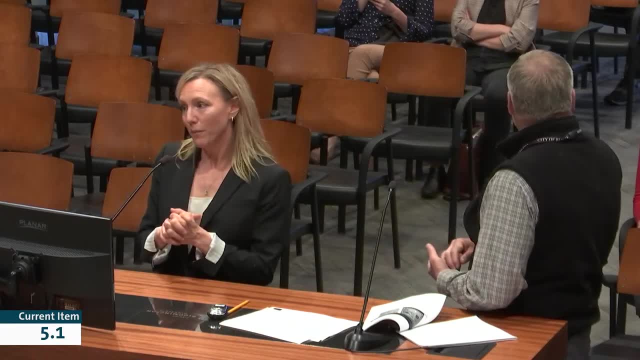 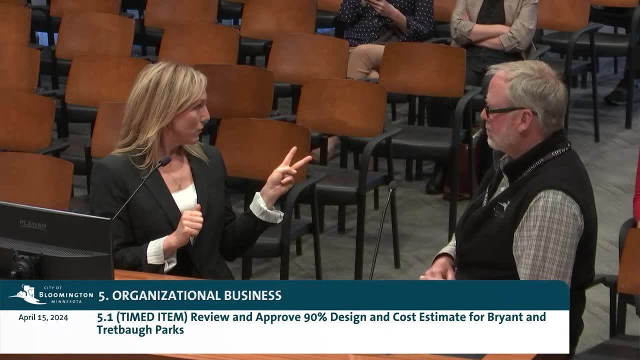 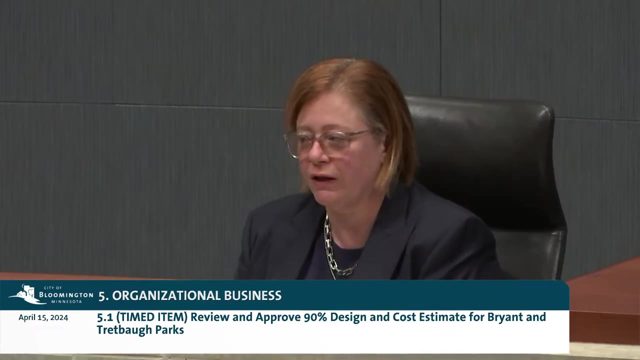 You think it's more 20. we're like 20, more like 20, and I believe each lot has Two. Each lot has two Handicap spots. Okay, Is there also parking Thoughts around van sized parking, so that people don't like park sideways across three parking spaces and that kind of thing? 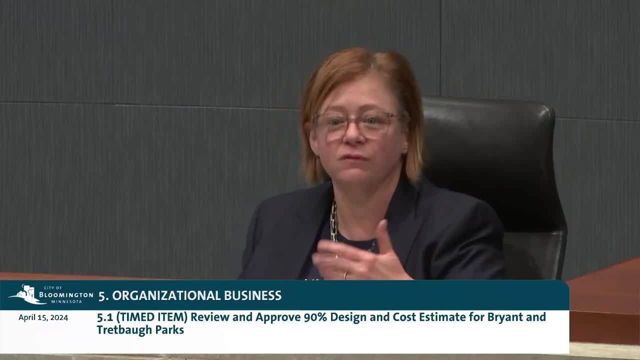 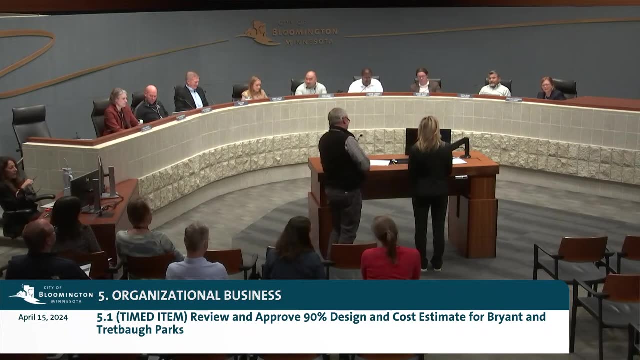 Did we consider that, knowing that we're, you know, attracting vans and other larger vehicles? Yes, Okay, great, That's all. Thank you very much. Congrats on this is: thank you, Council member Moua and then council member Nelson. council member more. Thank you, Mayor. 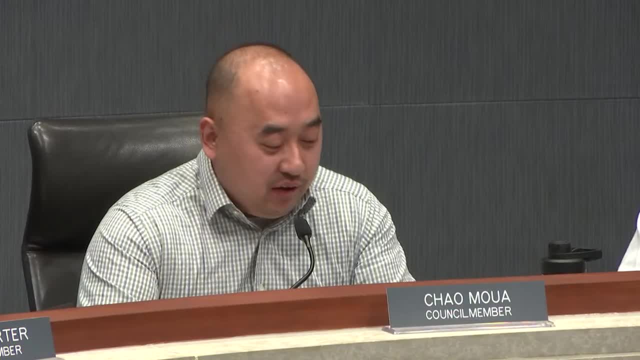 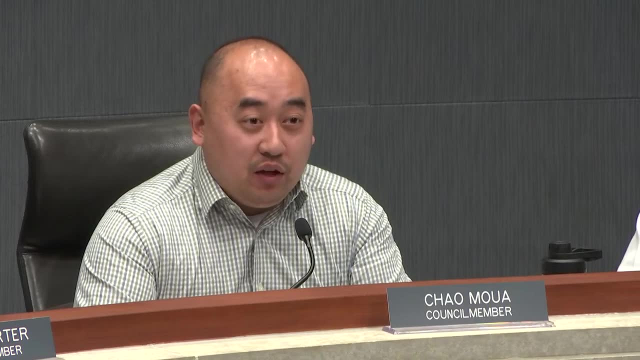 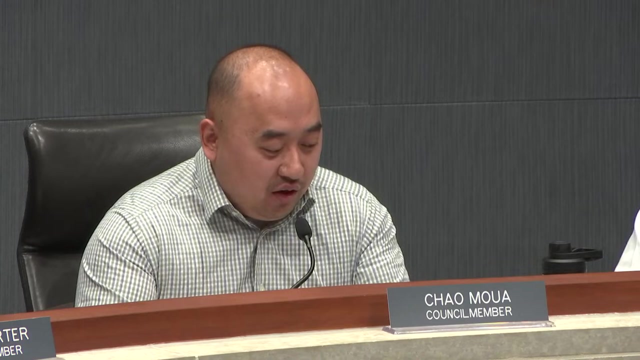 Thank you everyone so much for the work that you're doing on this. especially around the fencing around the playground, I've heard a lot of parents concerned about having multiple entrances, So moving to one is something I'm very happy to hear, especially because being the first accessible playground in Bloomington is amazing. 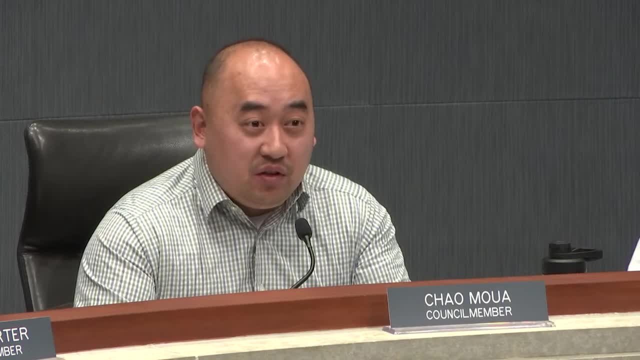 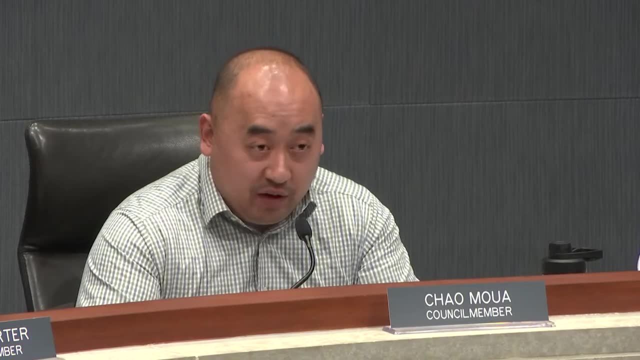 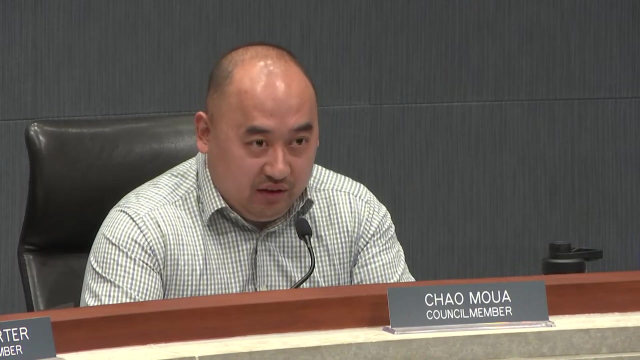 it's limited to bloomington. i know as soon as this opens, the whole region is going to be coming to bloomington to explore what we have and allow kids from everywhere to enjoy the facilities we have. my question is more around the 100 year floodplain. so from what you just said, a lot of it. 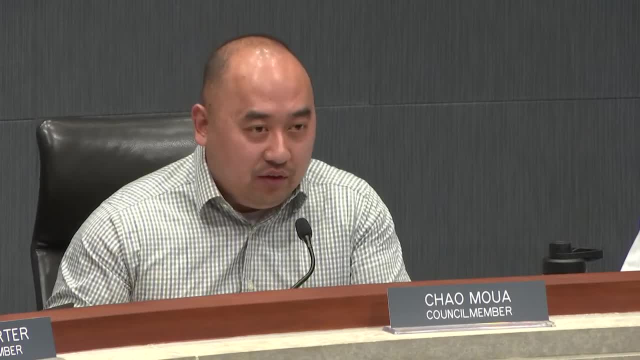 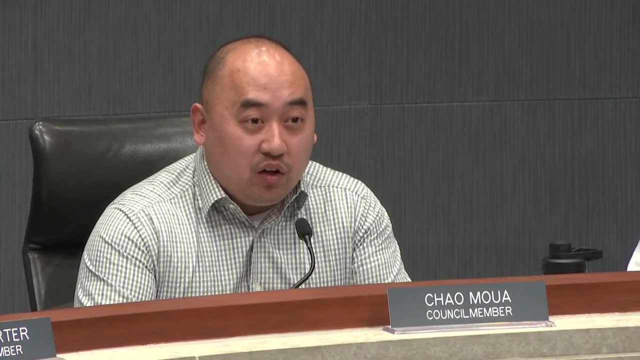 a lot of the facilities were located on the east side of the park, just given that it's not very scientific, but i feel like more of those 100 year events are happening or occurring. if we're going to invest this amount of money, have we, is the recommendation enough to ensure that we're? 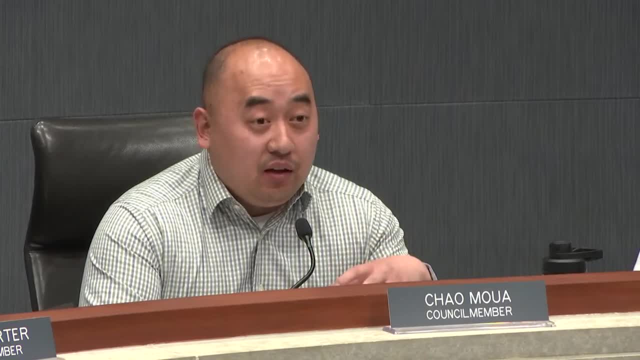 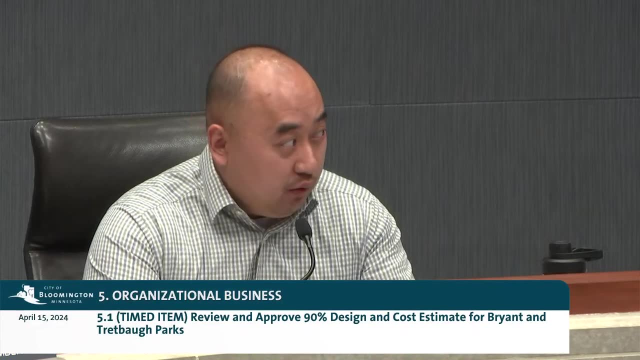 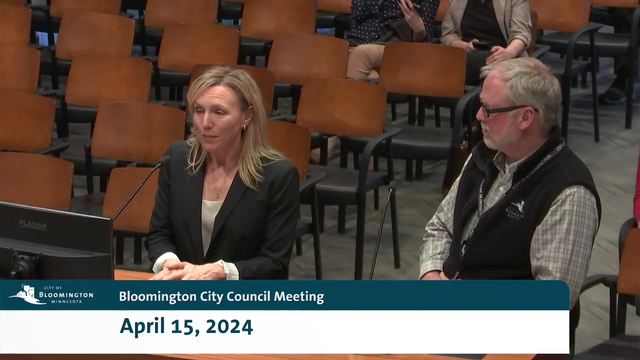 we're going to be okay if something like like a 100 year event happens, so that we're not investing all this money and then seeing it go to ruin and not being able to enjoy the, the facilities that we built. mayor, council member, moa council members, the. um, the park is less susceptible to flooding in that area. specific to the building, looking at the 100 year storm, it takes, i believe, about 13 hours for the water to get that high in an event like that and about 34 hours to it for it to retrieve lower than the building. i can't speak to exactly how. long that water takes to retrieve from the park, but i think it's going to take about 13 hours. uh, park in general, i believe, besides the building, the infrastructure, the courts and surfaces can tolerate inundation, not to say that, you know, a really significant event couldn't cause damage. 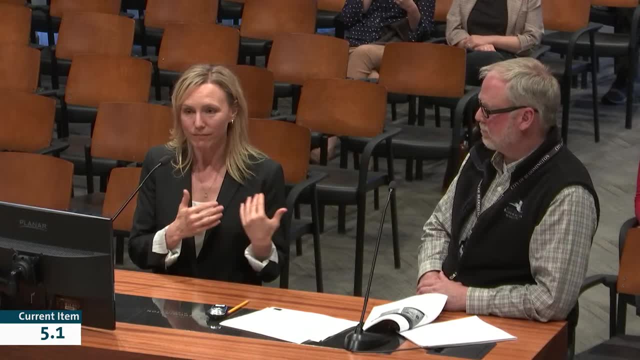 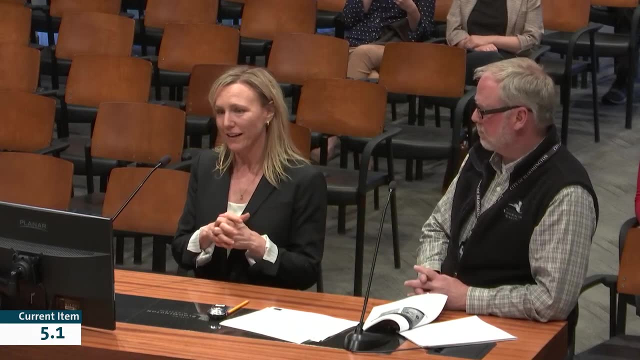 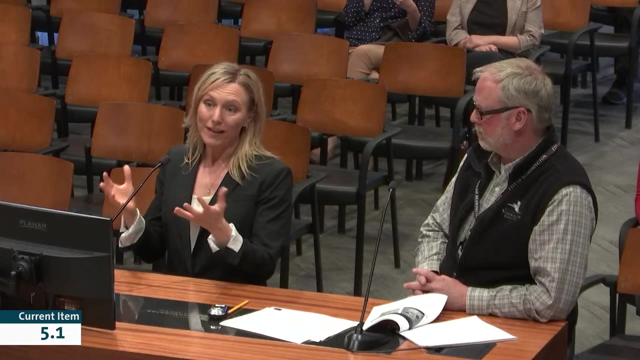 i'll use the example of 2014. um, my colleagues and engineers and engineering water resources. they've pulled up pictures and it looks like basically, that extent of the flooding covered just about up to the building. so a lot of the like where the playground is today didn't flood in that event, which was 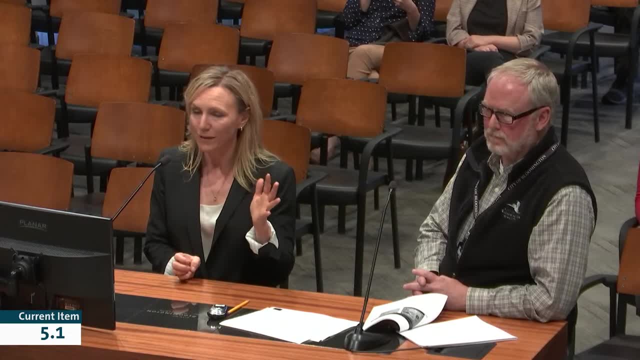 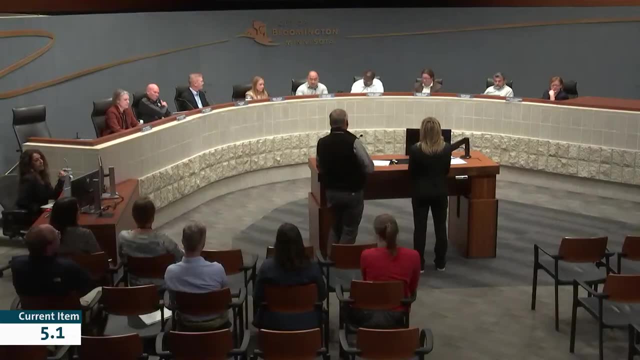 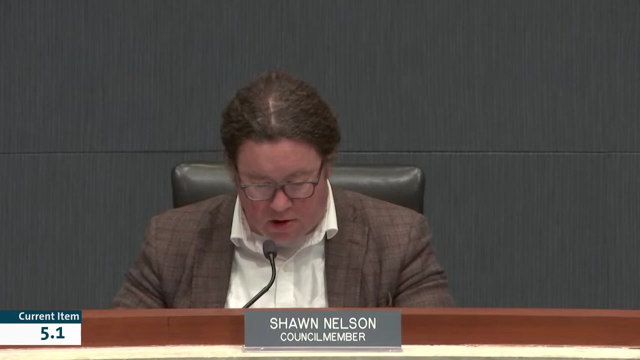 kind of the last big significant thing, approximately a 10-year event in terms of, you know, 10% chance in those terms. so the risk is there but we, we believe we've mitigated that to some extent. councilmember Nelson. yeah, Thank You, mayor. um, just a few quick things here. first, I appreciate the process that 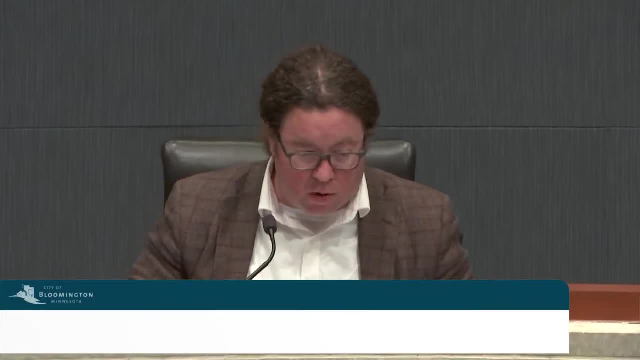 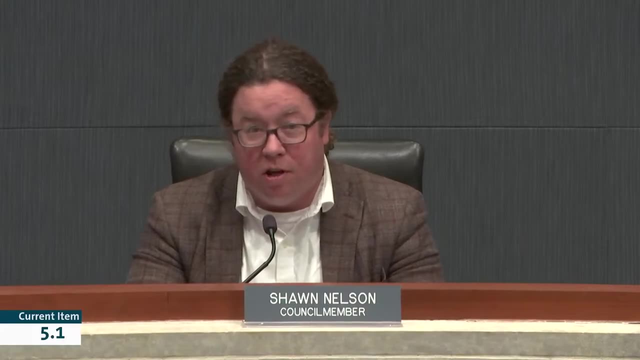 you've gone through in terms of the community engagement here. I know we have some people with concerns about another project that we have coming up down along nine-mile Creek, and I've always pointed to these projects as an example of the city's what it's looking to do for engagement with people in order to 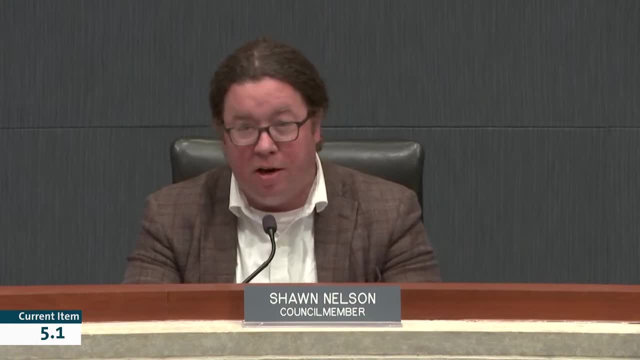 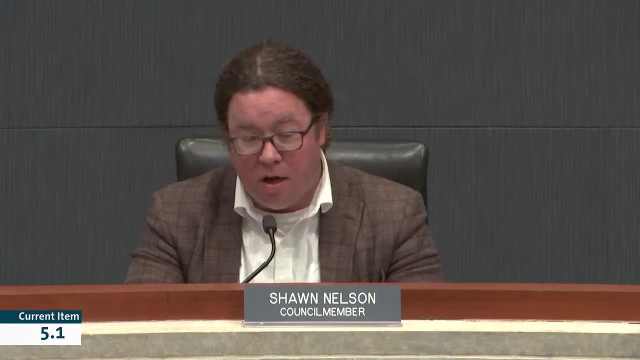 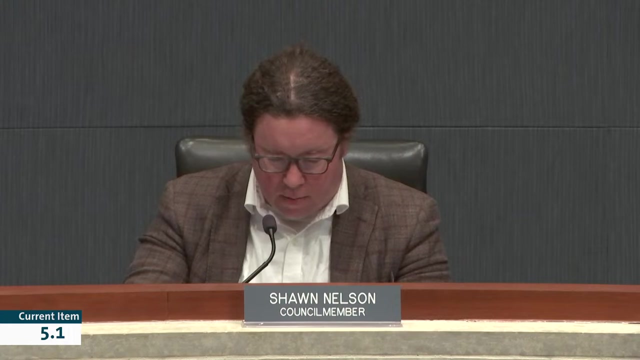 come up with those plans and you can see. you can see that there's a lot of work that needs to be done in terms of the community engagement and I think it's a great example of where I think the process works extremely well. just a couple of quick questions. the dog park. 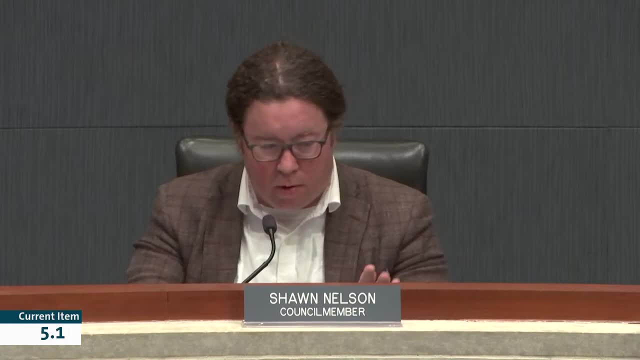 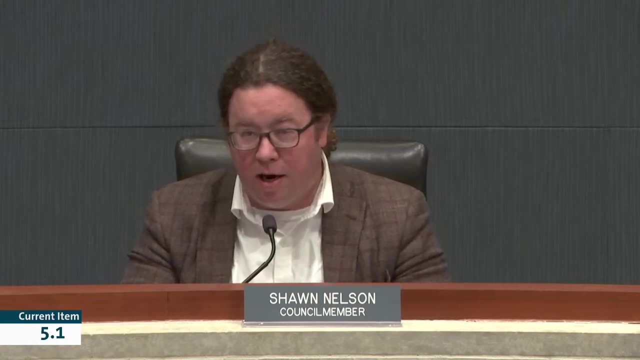 at Tretbaugh, the other locations I know when we originally looked at the park master plan, what we had divided the city into four quadrants are the locations that are being looked at. would they serve that four-quadrant mentality still, so that people, particularly in the northwest quadrant, 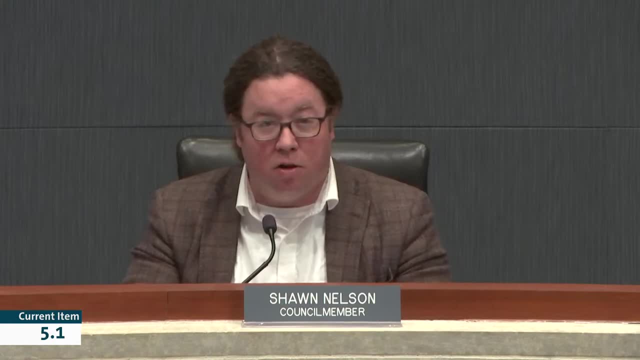 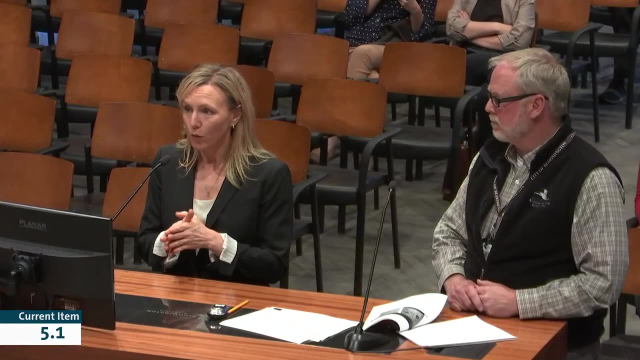 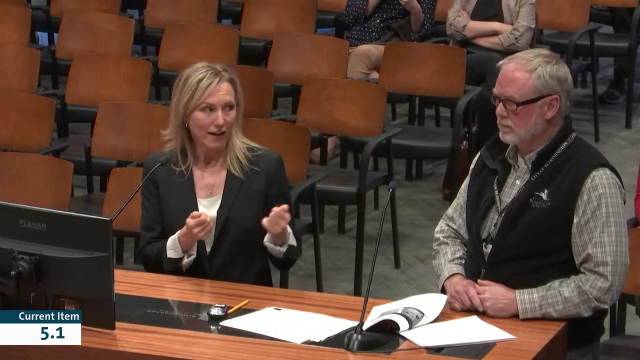 would not be without a place to take their dog that's convenient and accessible to them. mayor, councilmember Nelson, councilmembers, I'll start with Bryant Park ice rink will be equipped to be a dog run in the summer, and I'll let Dave talk about two other sites that we're currently exploring. yeah, thank you. 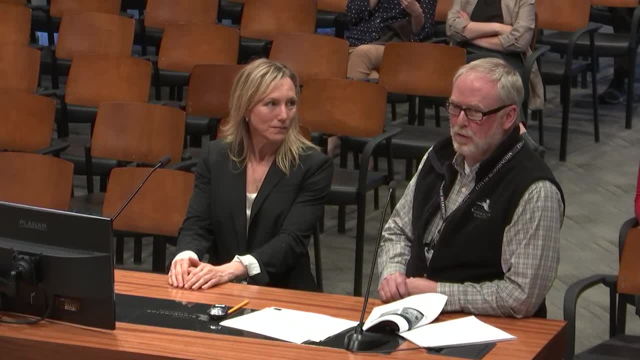 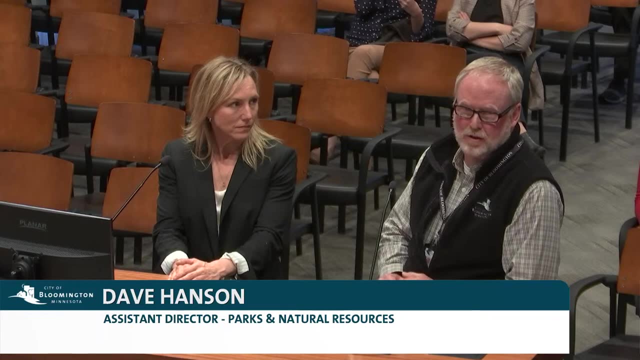 mayor, council, councilmember Nelson, we are going to put another gate up, similar to what we've had: a trap bow at Brookside, so on a hundred hundred fish and Xerxes. and then we're also looking, and this is fairly preliminary, but there is a spot. 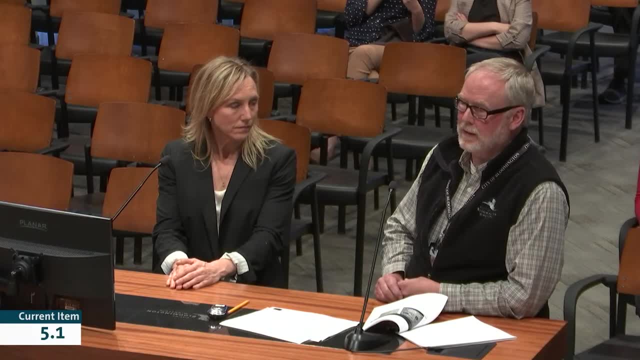 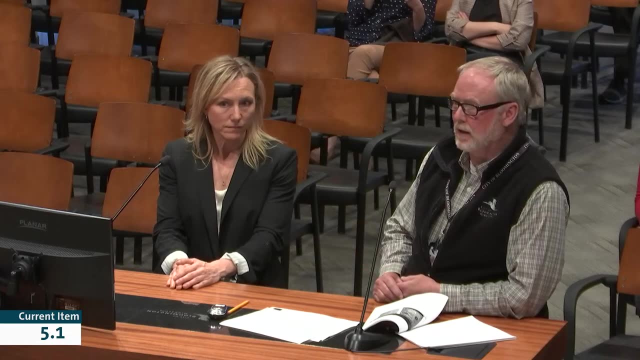 that has potential next to the archery range. some of the complications that we need to work through there is: the entrance and exit is on the county road, so we'd have to work through that process. it would likely require some significant parking lot upgrades, but we do own a piece of property there that 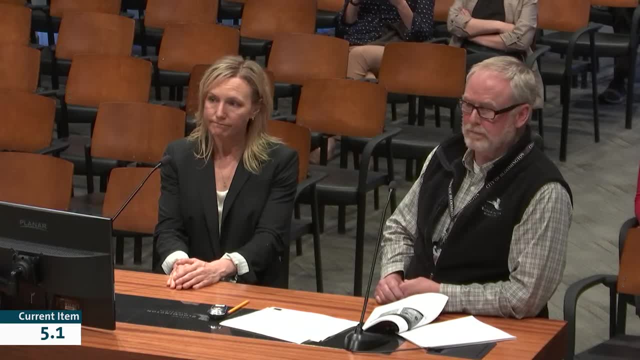 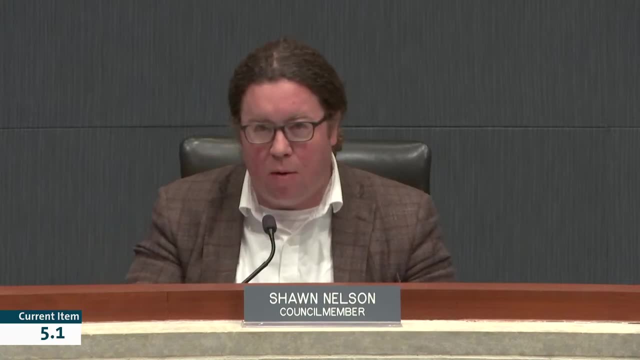 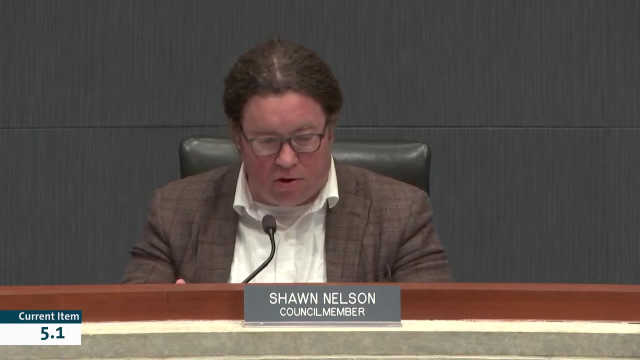 would be suitable otherwise. so we are exploring that. thank you. in terms of the overall plan, do we have any sense of the change in operational costs for maintenance parks? I know there'll be less mowing and less things like that. I also know that there is the fact that we don't have to mow. it doesn't mean. 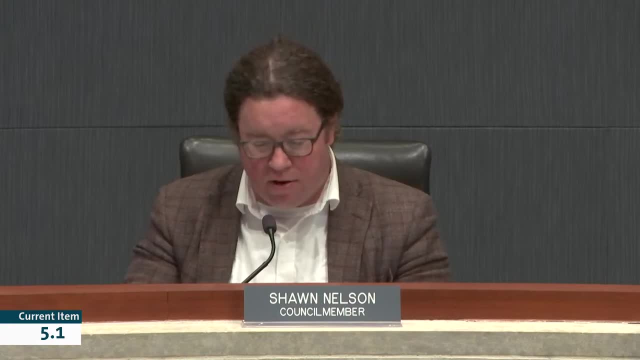 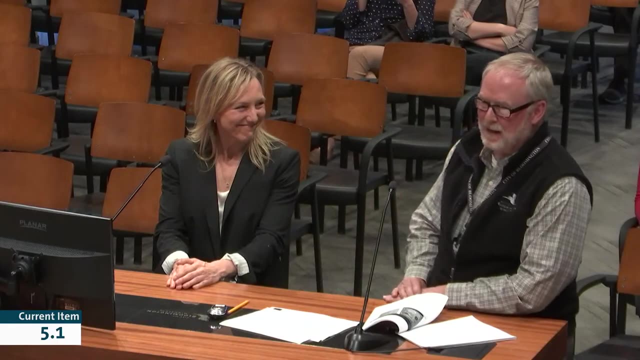 there's no maintenance for those natural areas. do we have any estimate of what change this will mean in terms of the maintenance? I don't have absolute area students. do we have any estimate of what change this will make an operational cost going forward? i'll take that one, uh. mayor. council members, council member. 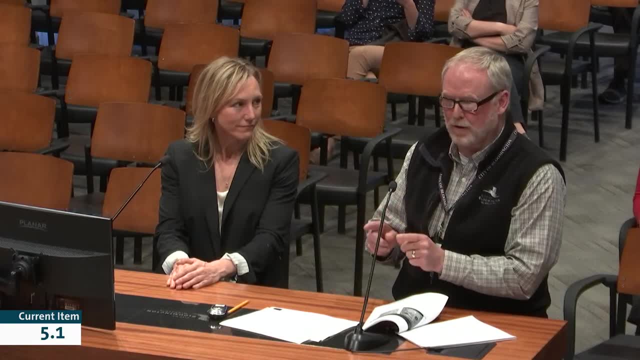 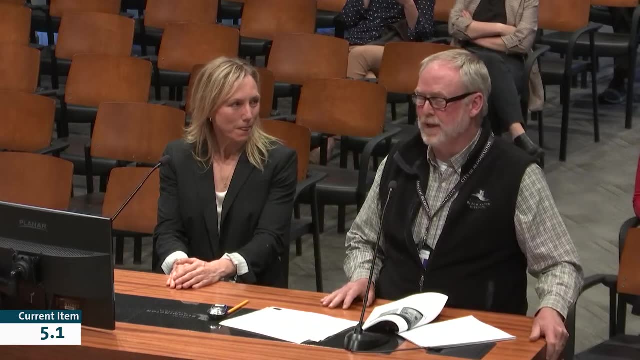 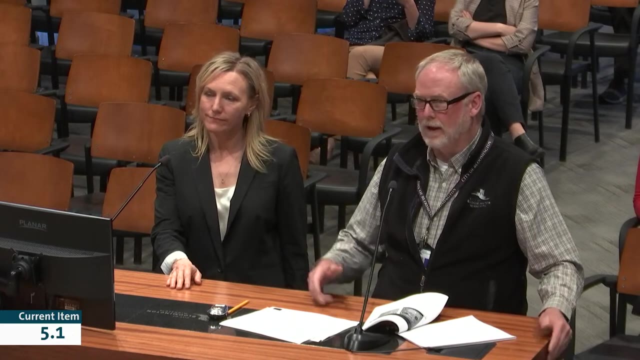 nelson, um, we haven't calculated it yet, but we got this great new plan that has unit costs. that's what i was thinking and, yes, we will be able to use the data that we have in that plan to address maintenance needs. for the rest of this, okay, development when it's time, um, and you're. 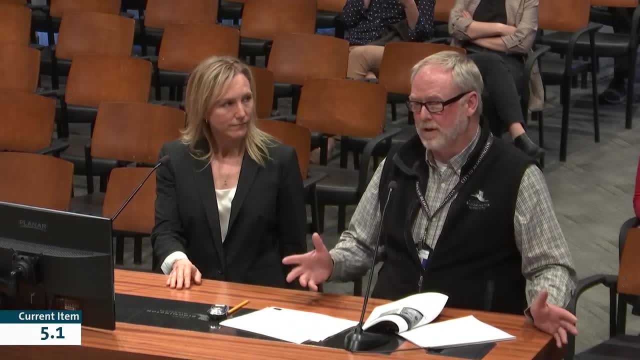 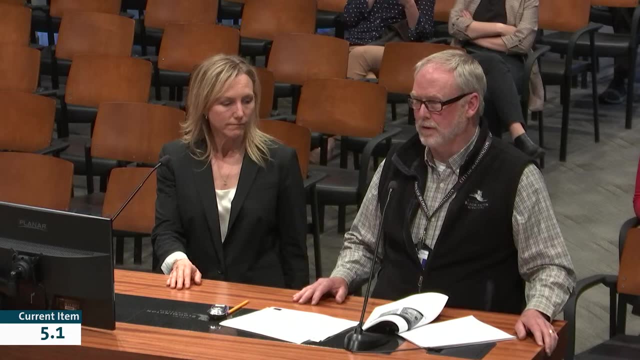 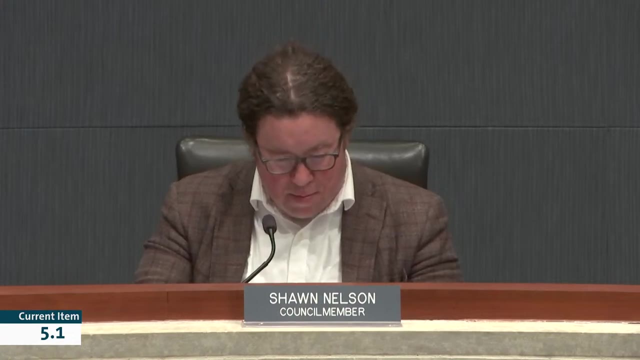 correct, also on the native plants. but once they're established, all that stuff is pretty self-sustaining and requires very little attention, so it's sustainable. that way probably took care of itself for a long time before we were here. yes, it did so, um, and then my last question. well, 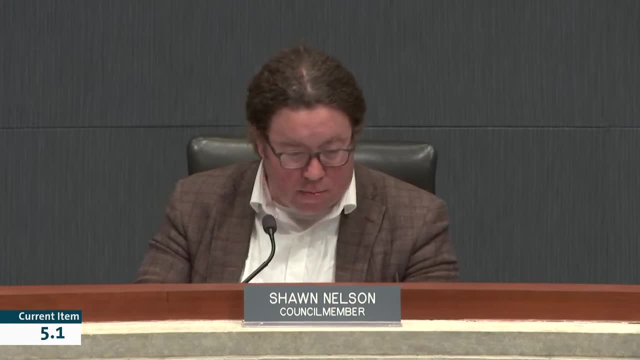 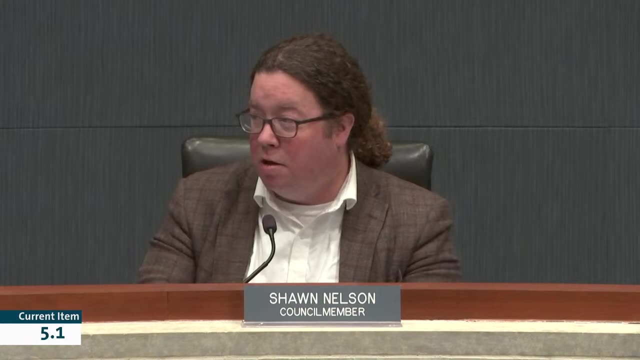 yeah, last question, uh, would relate to the building, and i just have to be honest, i'm still kind of blown away by the cost of a 2500 square foot building for 2.4 million, plus on top of that management fees. that's over a thousand dollars a square foot. 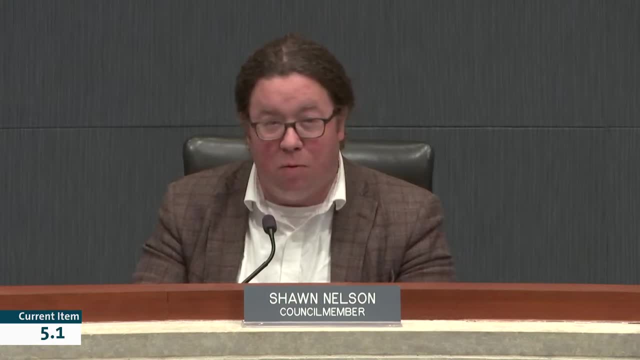 just to put it in perspective for people you know, basic rambler that'd be about two ramblers in there. i mean, it is enormous and i can't believe that's all related to the uh sustainability initiatives and things like that. um, i know we talked about this before, mike. do we really need 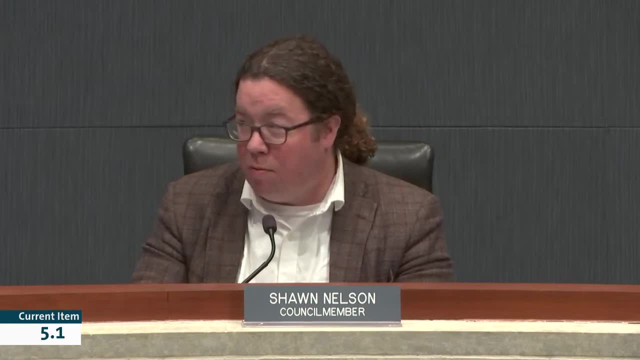 four bathrooms. can we make two bathrooms accessible from the inside and the outside? um, you know, is there that much demand in terms of usership to have those costs, because i know plumbing and fixtures and all that add costs. um, are there other things we can do to? 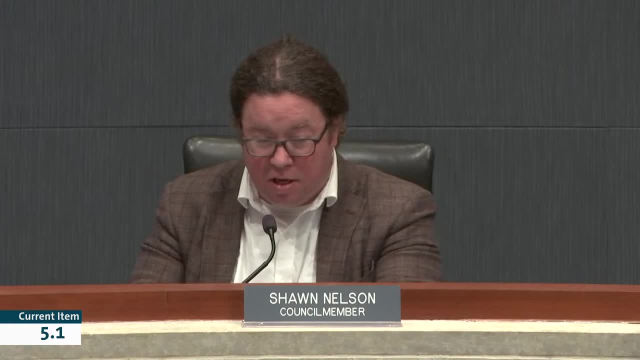 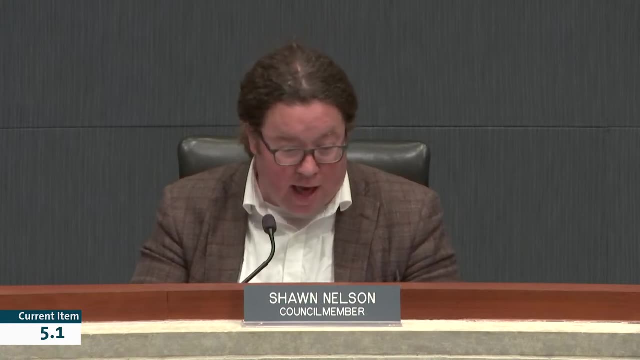 value engineer this because, from what i see in terms of the marketplace, we're double the normal cost of a building of that stature, um, and so that that is deeply concerning to me, um on there, and so i guess that's not really a question, it's just feedback, it's. 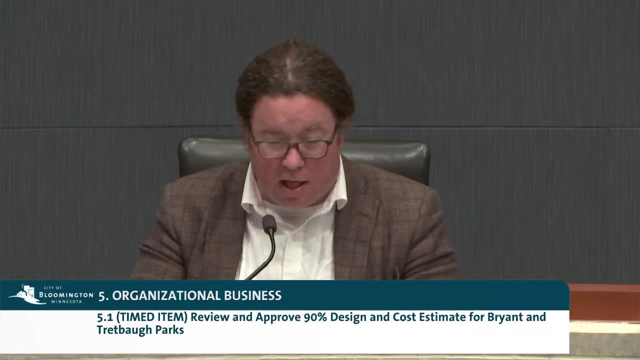 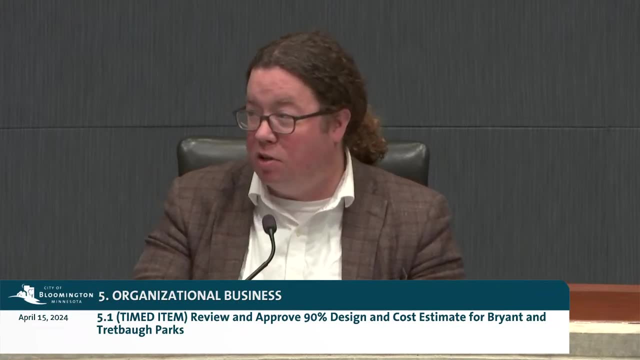 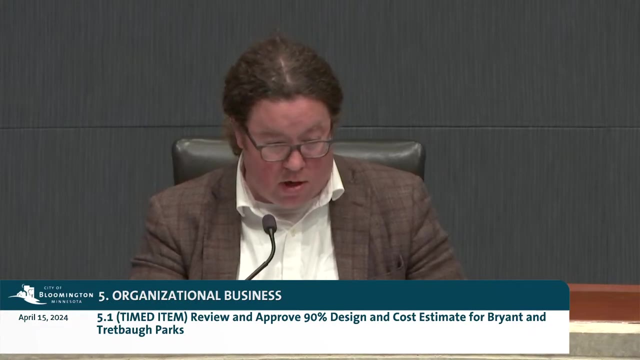 it's significantly more than, frankly, i think most of the public marketplace could just build- or private marketplace could build- a building for half that cost of the same square footage. um, on the flip side- and i don't know if this is the right location at all, but it was warm this winter. 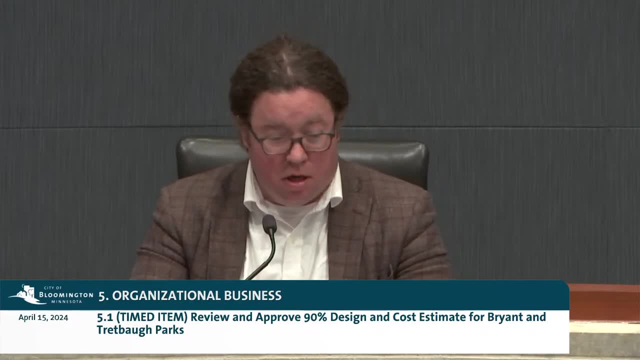 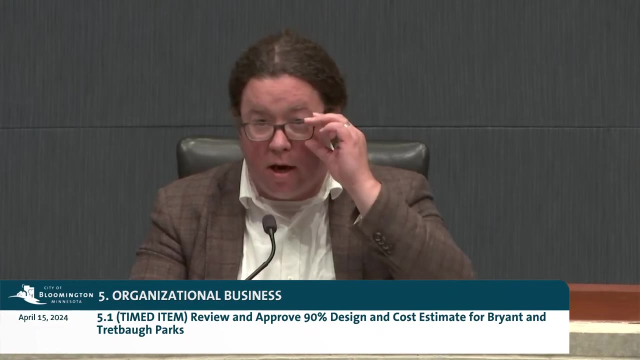 we had a very, very short outdoor ice season. has there been consideration of any type of refrigerant or, um, at least making it possible to do that in the future or anything like that to extend that season so that we maybe had a couple locations throughout the city that people knew would be available for? 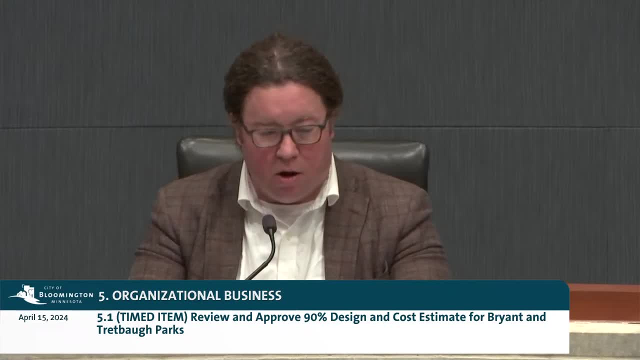 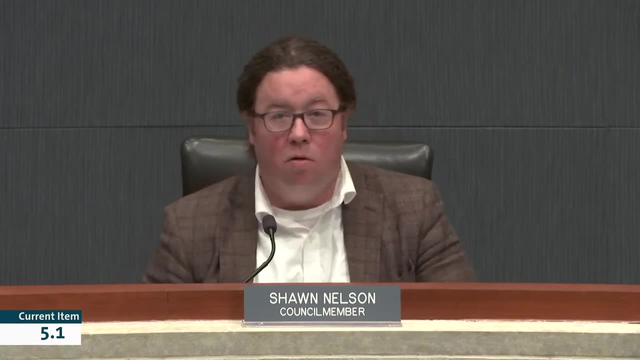 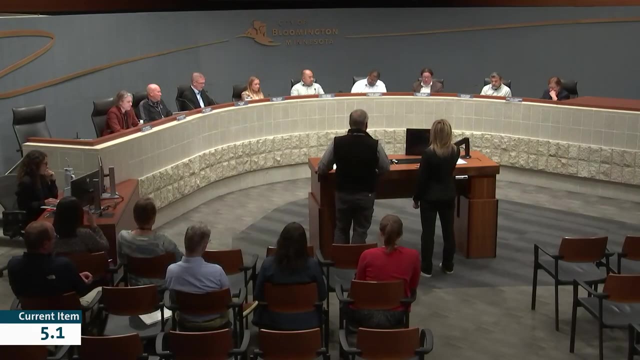 a longer season, uh, during the winter, um, because i know that you know the the demand at uh big is significant. we're obviously making improvements there. that's, that's not the answer. so so that's not really- again, i don't really, it's more of a comment- if this would be an appropriate location to 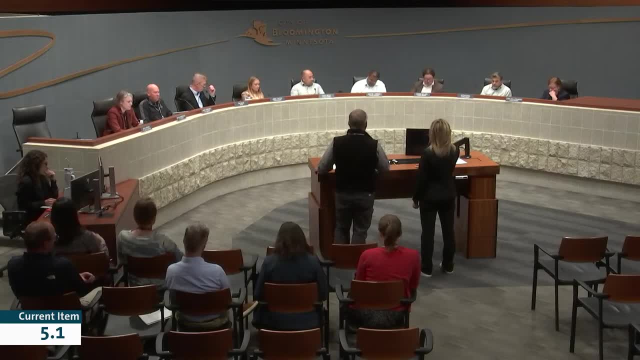 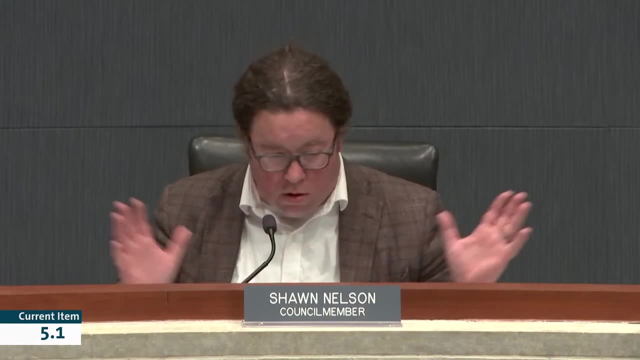 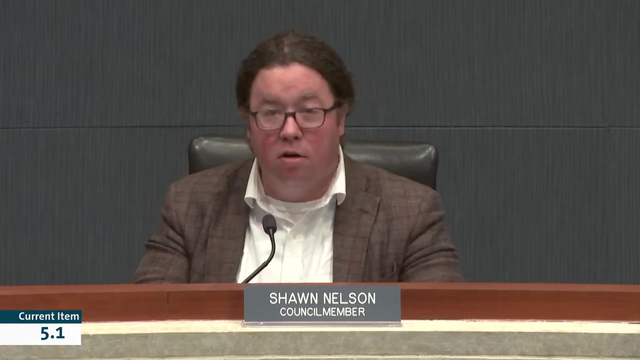 look at doing something like that. it'd be something i'd be interested in. when you look at those alternatives, you know what would something like that cost? is this an appropriate location? are there other locations? or, if you know, my colleagues and park and rec staff and uh commission think that's just a non-starter. um then let's not look at it. i appreciate your. 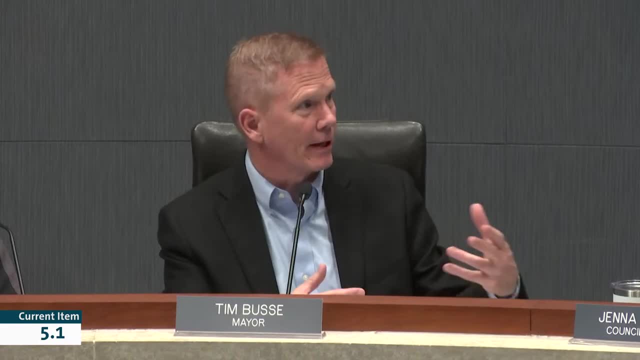 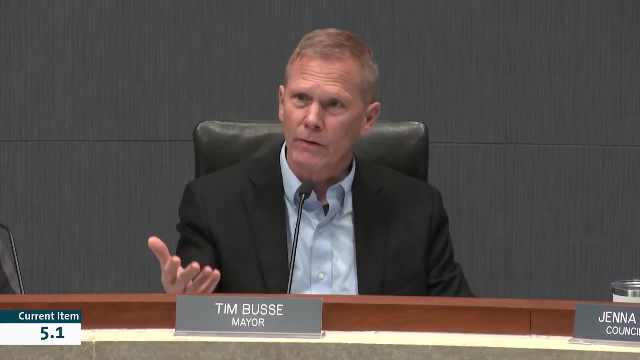 comments, council member and, uh uh, your comments regarding number of bathrooms. i mean that's, i think, what we're here for. i mean we're at 90 and sort of get that feedback. i think is a good thing. regarding the, the outdoor refrigerated rink, i know that's been a topic of discussion on and off. 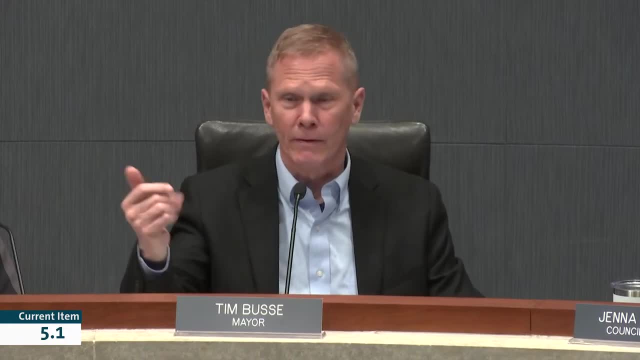 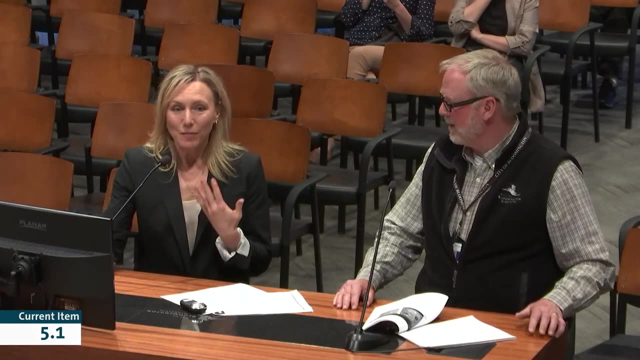 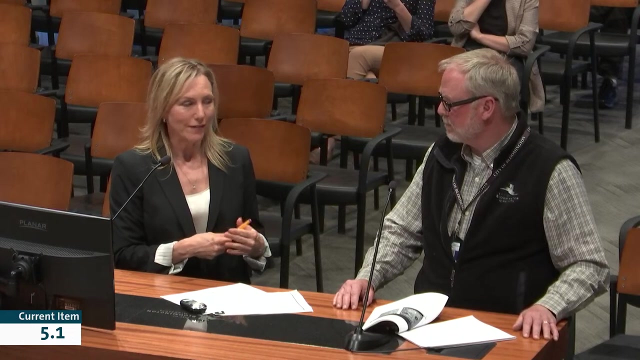 in a variety of different locations other than this. i'll turn it over um excuse me to the folks who have been having those conversations, anything to report? um mayor busi, members of council, um, we have had those conversations. in terms of its winters are warming in minnesota and that season 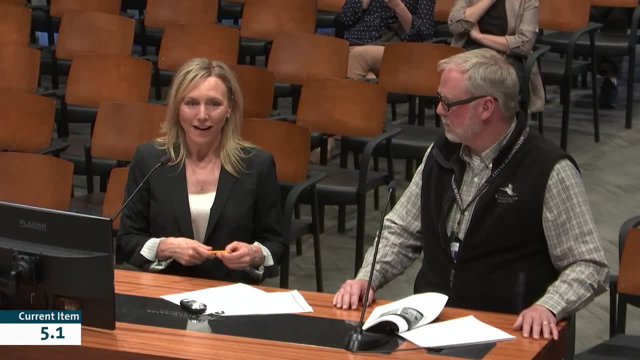 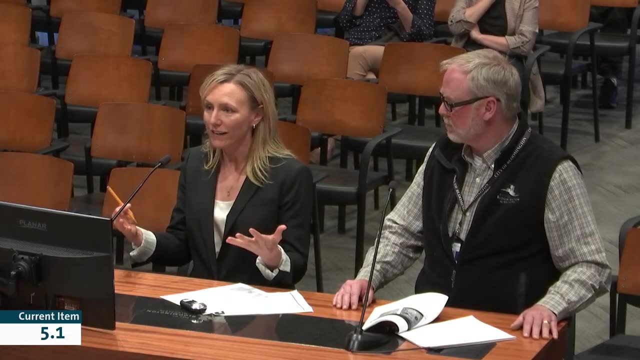 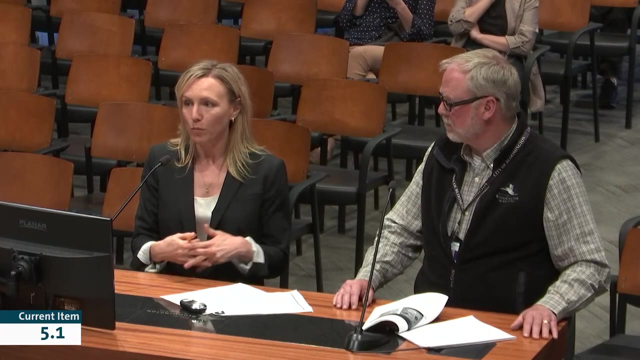 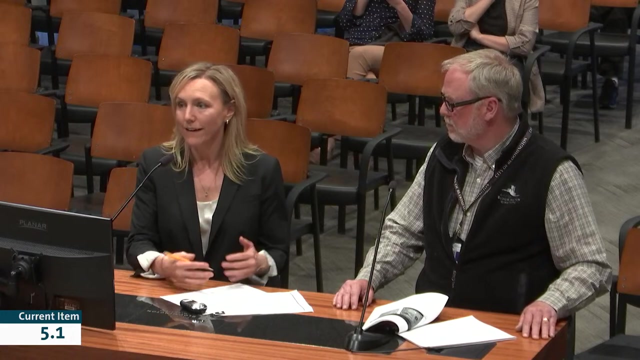 as was last year, is often threatened. how could we provide that? we haven't done any real planning on you know kind of service area level where it makes sense. but that's something that i think we could explore, probably outside of this project effort, but also ask the question: if we decide this is the site makes sense. 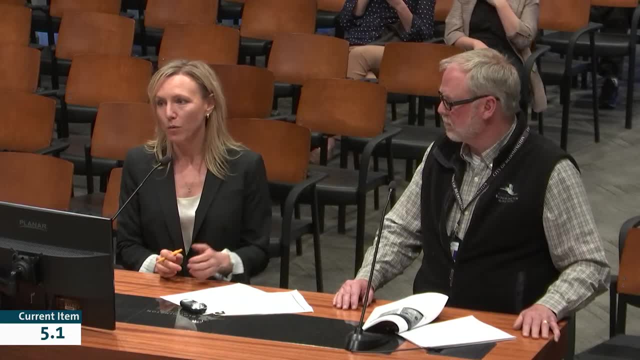 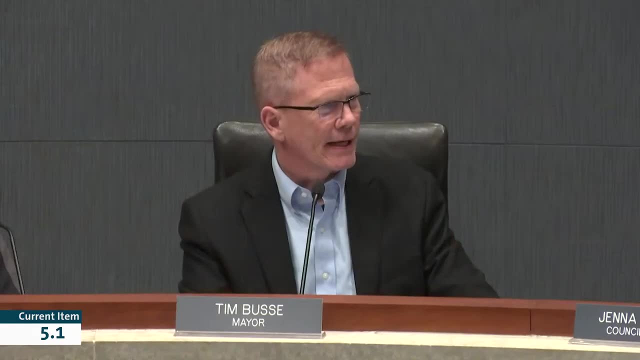 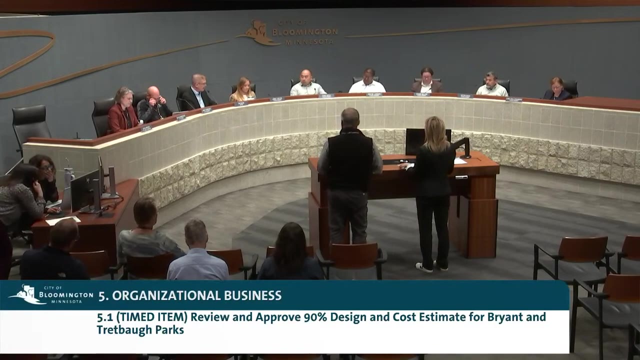 how? how might that be possible or made more efficient with this project? i appreciate that. thank you, council. i'm going to keep us moving. it's we're pushing eight o'clock now. we still have a number of things that we've got to get to tonight, um, so i want to thank staff for the presentation. uh, thanks for the information council, any. 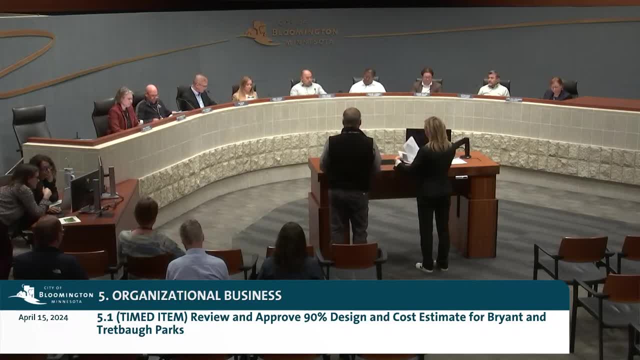 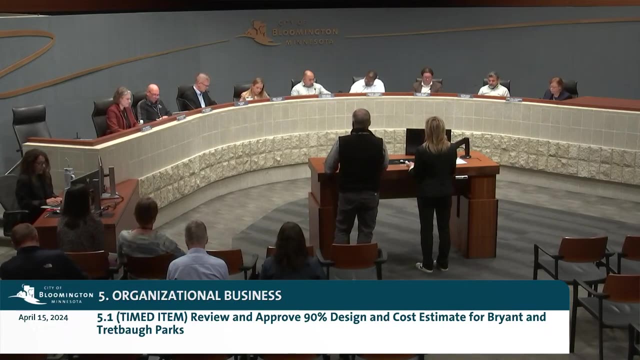 additional final comments on this. if not, i would look for action on item 5.1 this evening. councilmember carter. uh, thank you, mayor. so i would move to approve 90 design plans for the bryant and tretbaugh parks reconstruction project as reflected in the staff presentation engine and. 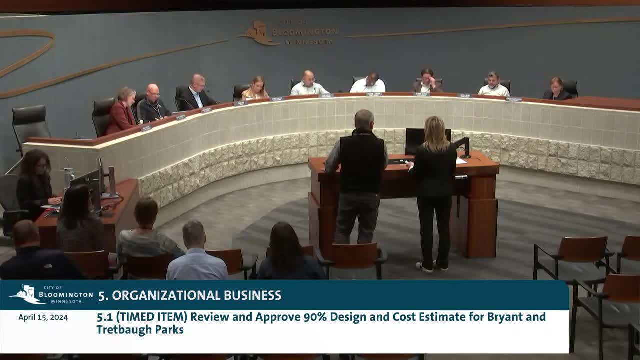 agenda materials. second motion by councilmember carter, second by councilmember loman, to approve the 90 design plans for bryant and tretbaugh park reconstruction projects. council. any further discussion on this hearing. no further comments. all those in favor please signify by saying aye, aye. 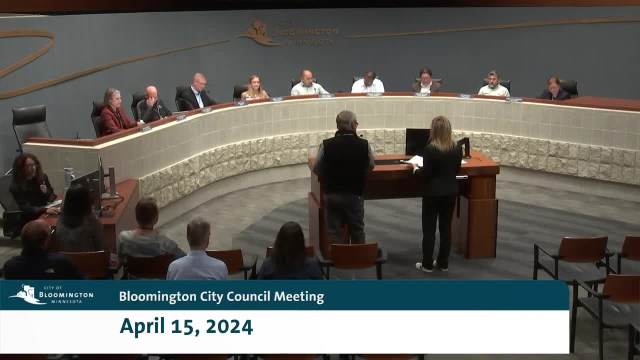 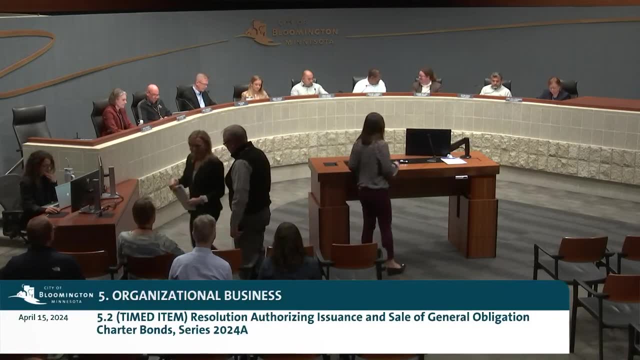 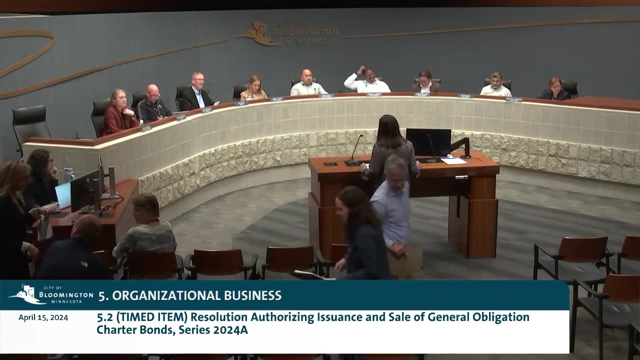 opposed motion carries at seven zero. thank you, thank you, thank you much and, as was mentioned, uh, the related item here is item 5.2, which is a resolution authorizing the issuance and sale of general obligation charter bonds, series 2024a. brianna eicheldinger is with us, good evening. 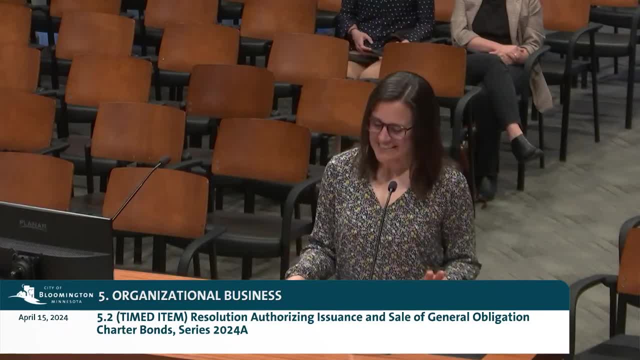 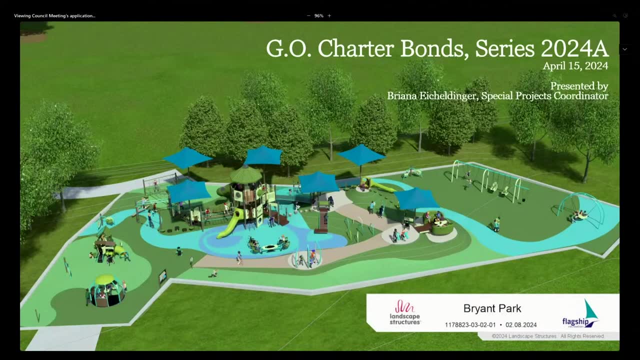 and welcome. hello, uh, good evening, mayor, council. my name is brianna eicheldinger and i'm the special projects coordinator in the finance department. i'm here today to request authorization as to the issuance and sale of general obligation charter bonds in the proposed aggregate principal amount. 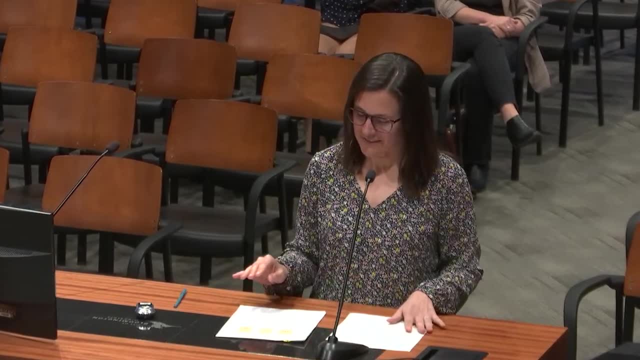 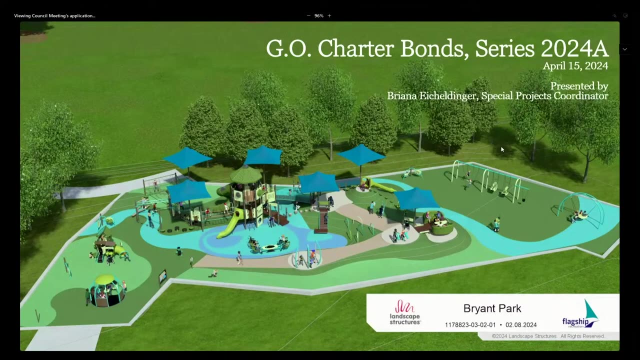 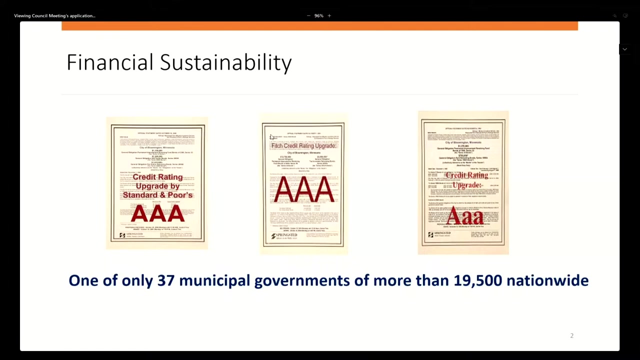 of eleven million five hundred thousand dollars, so i hope it doesn't go further, okay. so before i jump in, we like to highlight the city's financial sustainability because in order to cultivate an enduring and remarkable community, the city needs a solid financial foundation. so bloomington ranks with an elite few cities nationwide holding three. 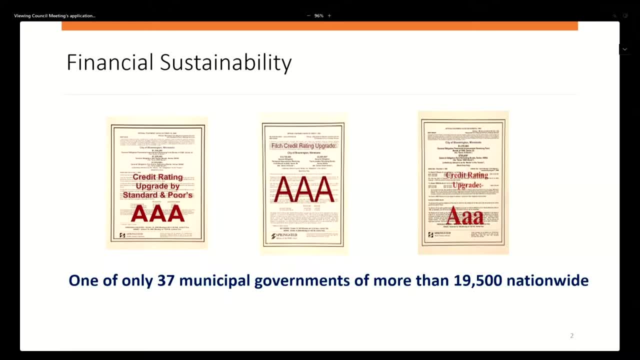 transnational and multi-billion dollar capital projects in the city of bryant and tretbaugh park. tripple a bond ratings. the city has maintained triple a status for the last 20 years from s p, moody's and fitch, which is the highest rating awarded by these agencies. 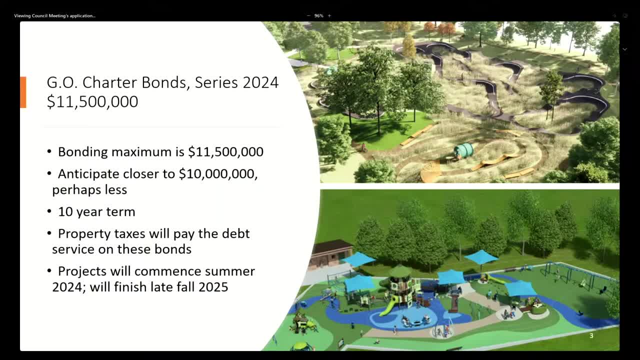 so we saw the presentation just now from our parks and rec staff. charter bonds will be utilized as a funding source to pay for bryant park and tretbaugh park projects. in addition, there's another about five hundred thousand dollars that will be used in the bond amount for. 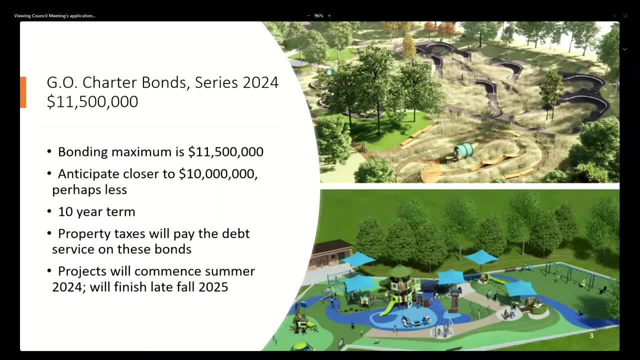 bryant park and tretbaugh park and some parking lot improvements as well, the authorization that we just passed tonight for moving forward on the parks. we won't know what the final bid amounts will be until later, and so we go a little bit higher in. 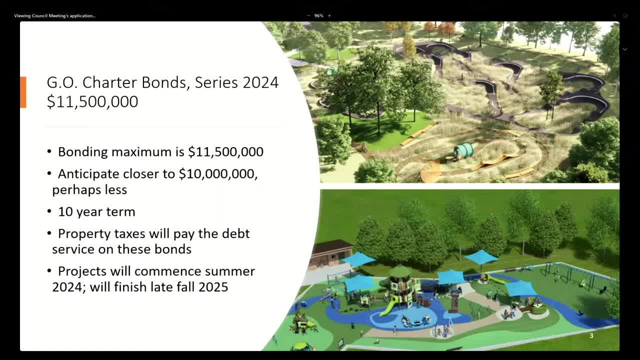 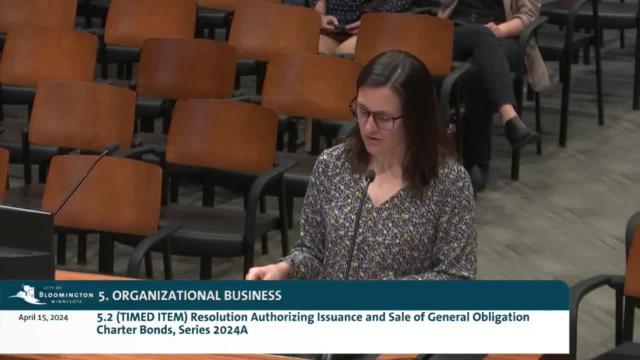 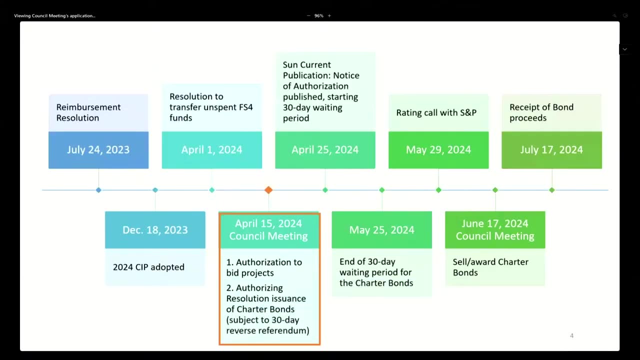 our maximum amount request. the reason we do that is so that we can cover general contingency cost of issuance in the maximum bonding amount and then any inflationary or cost changes that occur after the 90 percent design. so we want to cover a little bit just in case. so i thought this slide would be helpful to capture. 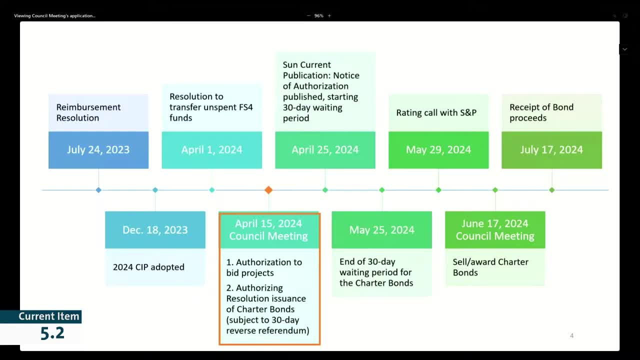 the items that have already been completed and then things that are next steps in this process to pay for the parks projects. the orange box shows where we are tonight and then, moving forward, we will have our 30-day waiting period for the charter bonds that will be published in the sun. 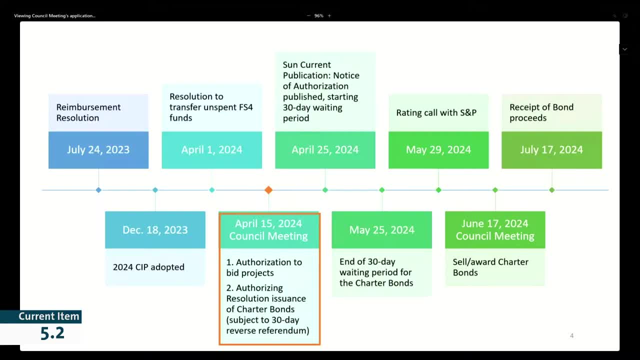 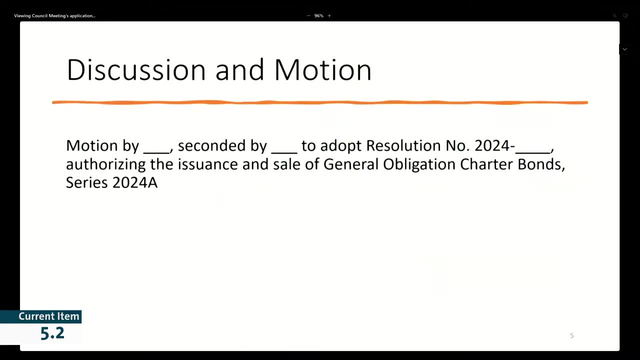 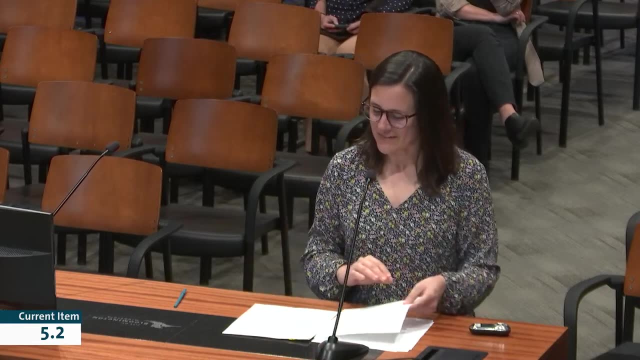 current april 25th, and shortly after that we'll do a rating call with s p and do the bond sale in mid-june, and so that's the the basics of the situation with funding these park projects. i'm happy to take any questions regarding the bond issue we also have on the phone. 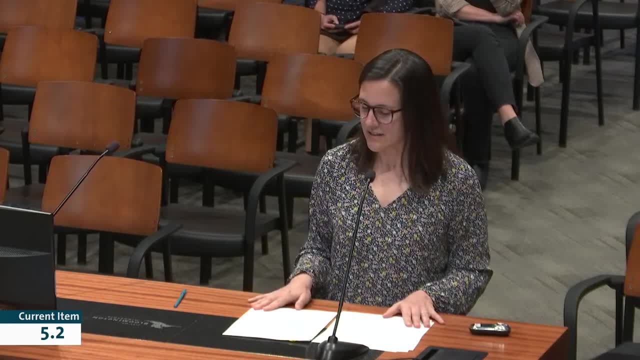 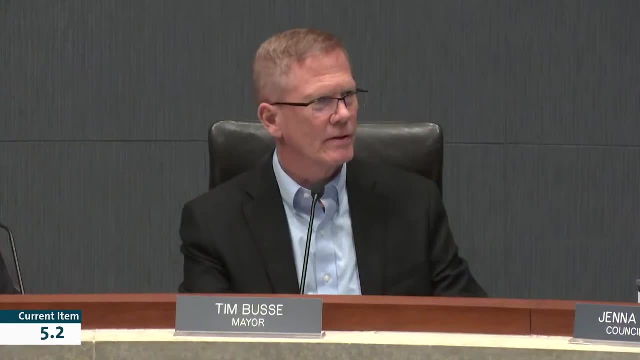 our bond attorney, julie eddington, from kennedy and graven, and then elizabeth bergman, who is our municipal advisor from baker tilly. thank you very much. council questions of ms eicheldinger. councilmember nelson. thanks, mayor um. so this does not. 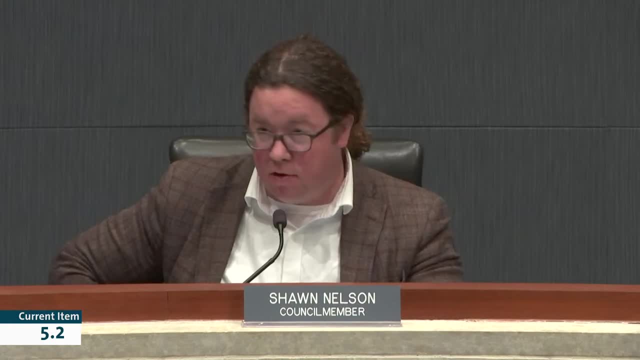 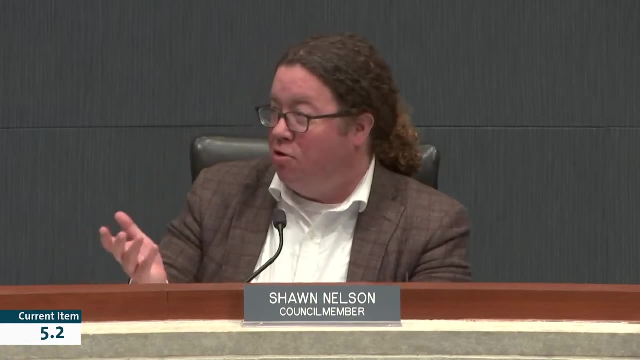 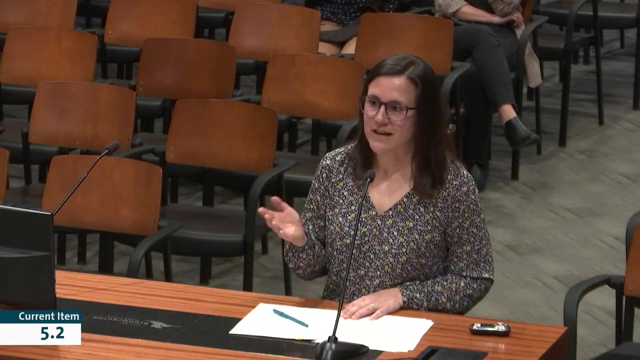 include any system that is required to operate colors, a Algun's viewpointing on the plot following the design of the park and that's actually going to be taking a little bit too much into theALL fists type of way that we areję do the work together in this project. 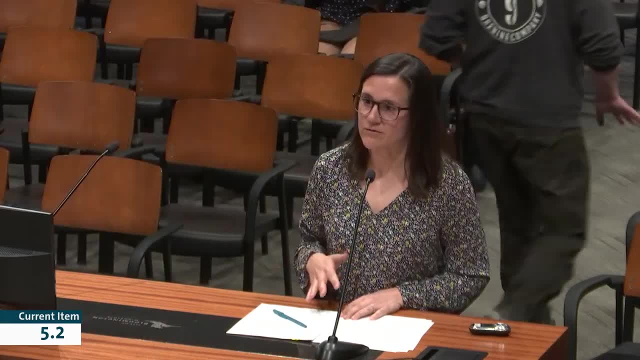 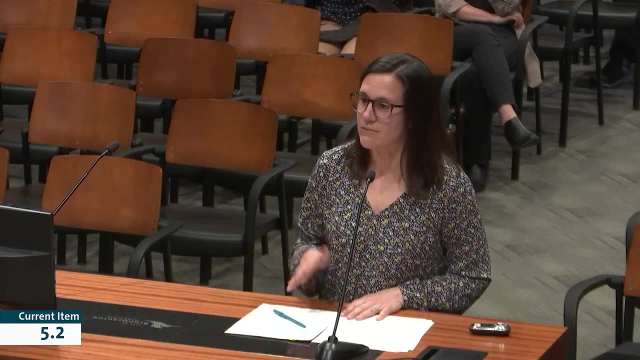 i just wanted to bring up something that people are asking of us today and méahana about the走了 board. i don't remember that i did. you know we have lot of, and so opportunities like that would be available as well. Okay, Thank you. 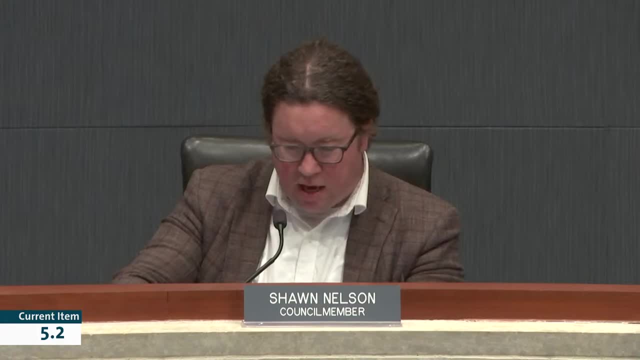 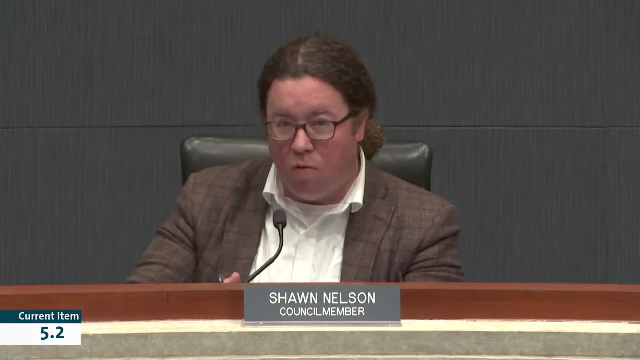 And then can I get a little bit more of a description of what at Dred Scott, because I know there's also a consent agenda item regarding Dred Scott and some of the improvements there. Do these overlap or are they completely separate? Renee is on her way to address that. 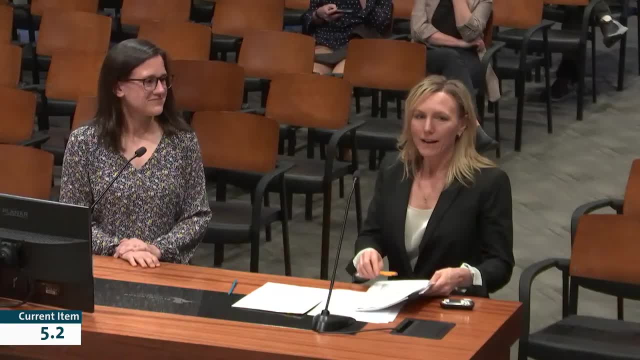 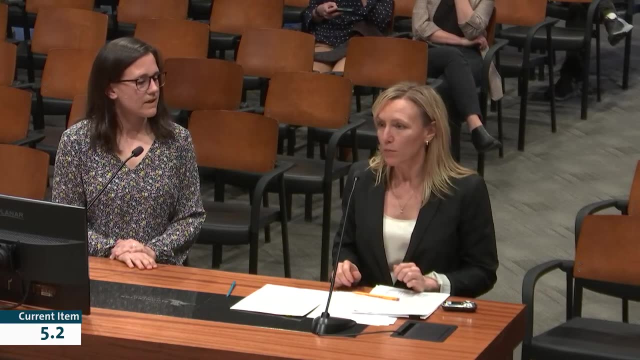 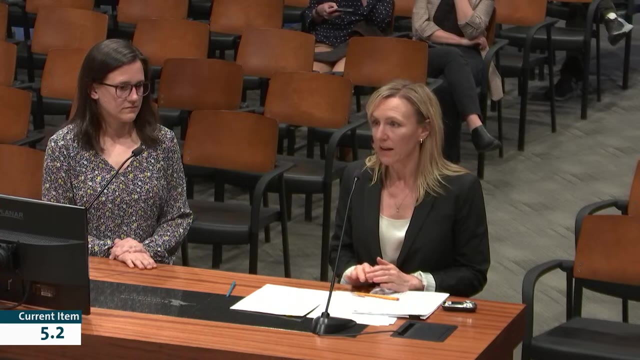 Okay, Mayor Busse, Council Member Nelson, members of council, the Dred Scott. improvement projects in total for field renovations are estimated at about $1.5 million. in our bonding package, Some of the you know part of the timing of this- we'll find out a little bit. 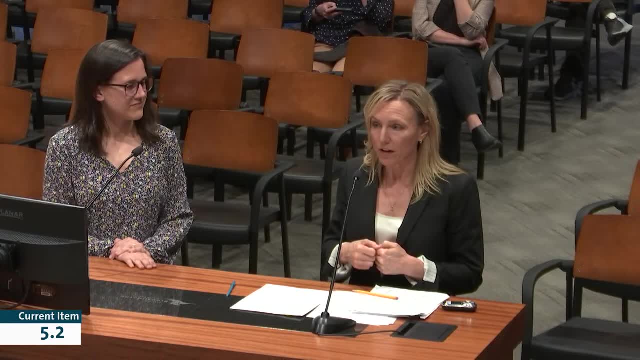 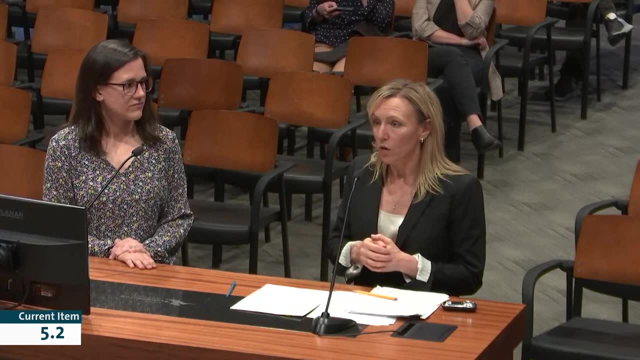 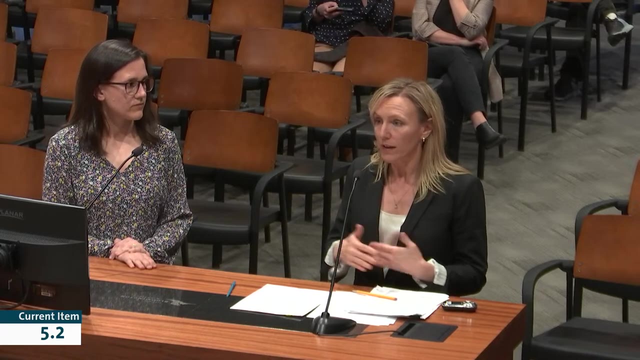 we'll know about what happens with bonding, but some of the improvements there are more time, critical and related to safety that need to be made regardless. So this fall we have planned improvements for the Dred Scott improvement projects for those fields that include really regrading. 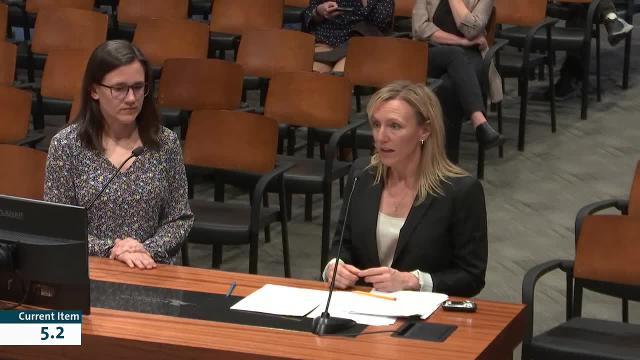 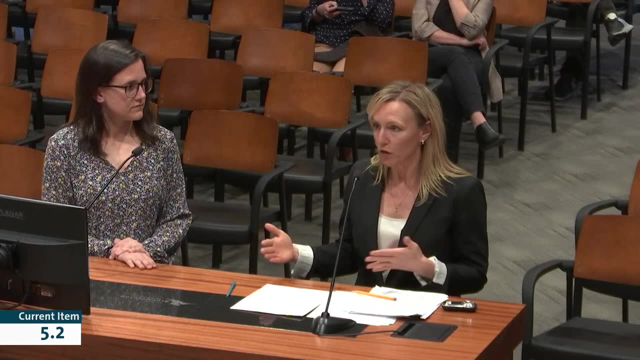 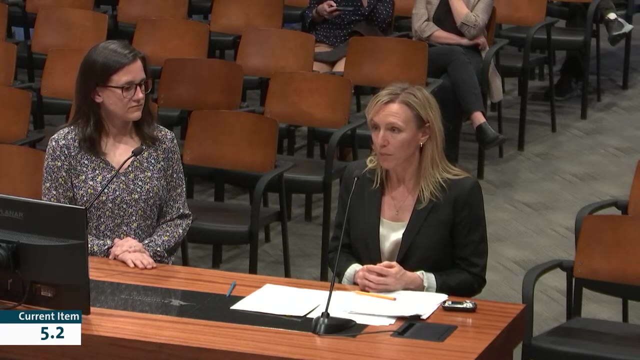 and expanding warning tracks for safety that we need to do. Some of those improvements could be, you know, part of that, $1.5 million worth of improvements could go farther with bonding or with the state bonding award, if that should happen, which would reduce what we're asking for from charter bonds. 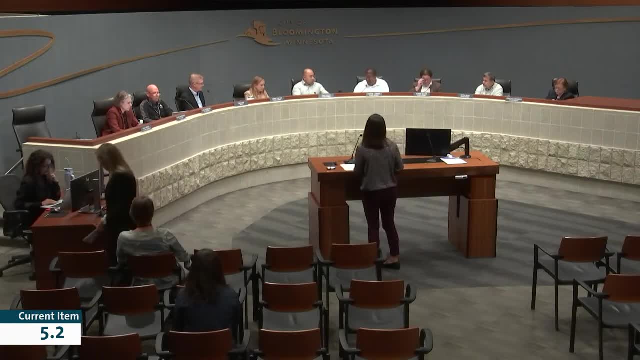 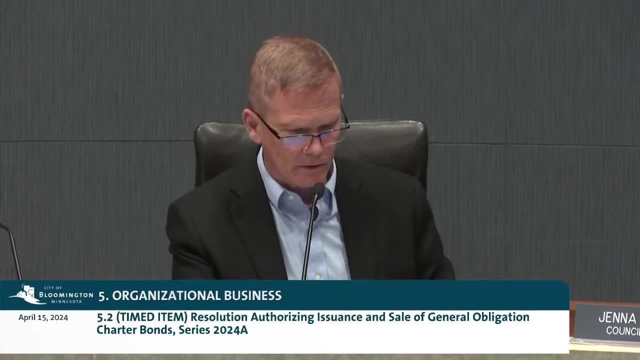 Council additional questions on this. If there are no additional questions, Council, I would entertain a motion to adopt a resolution authorizing the issuance and sale of general obligation charter bonds, series 2024A, as it relates to item 5.2. 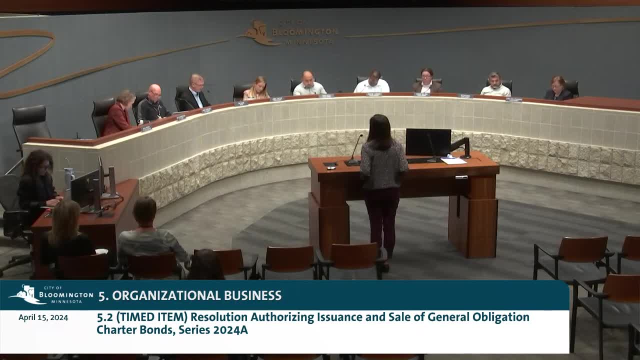 So moved. Second Motion by Council Member Lohman, second by Council Member Carter, to adopt the resolution authorizing the issuance of general obligation charter bonds. No further council discussion on this. All those in favor please signify by saying aye. 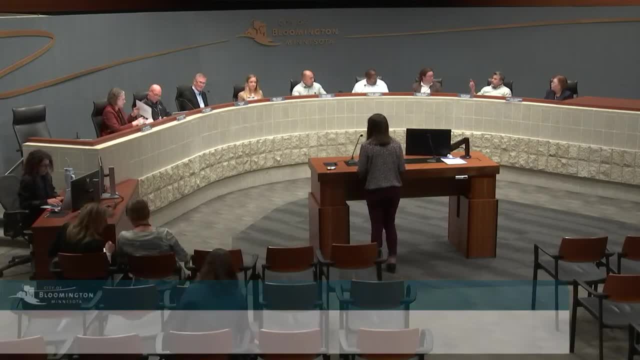 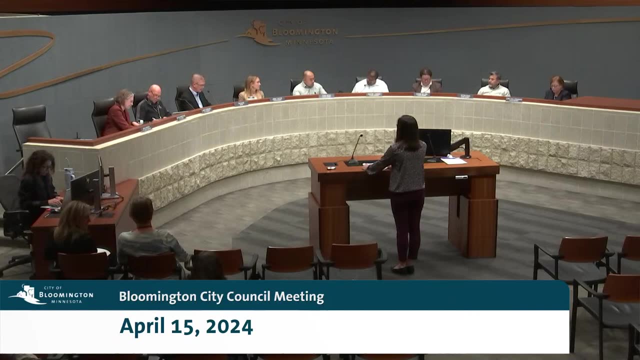 Aye. Opposed Motion carries 7-0.. Thank you very much. Thank you We have. we are at 6-1 on that vote, with Council Member Rivas voting in opposition. Very good, We will thank you. 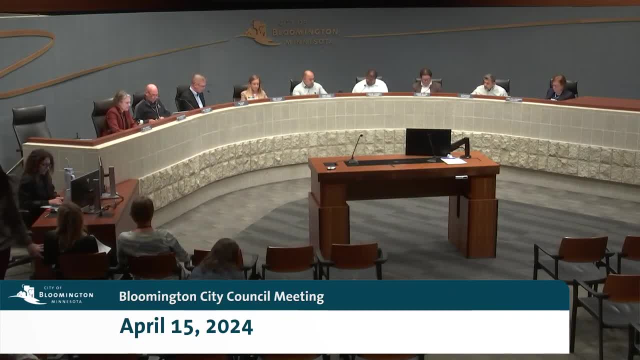 Ms Eicheldinger, we appreciate it. We will double back now to item three on our agenda, our consent business. Council Member D'Alessandro. Thanks, Mr Mayor, Appreciate it. I have a hold on 3.3 from Council Member Nelson. 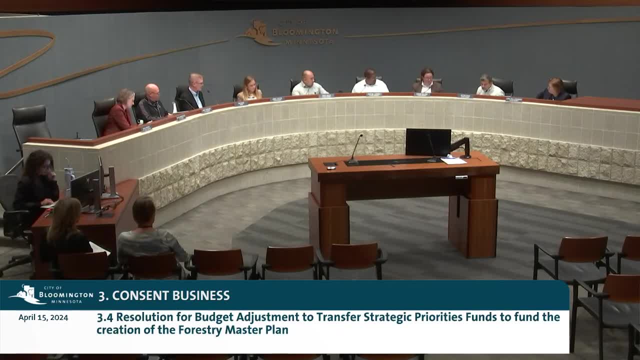 which Mayor is it? Is it still valid? Okay, great, And as customary, I'll hold 3.1,, but I don't have any other holds. Does anybody else have anything they'd like to hold? Okay, Then I will move to adopt our consent business 3.2,. 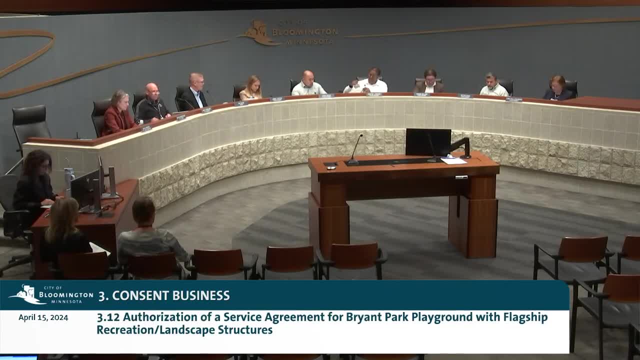 3.4 through 3.17, I think is the number. Second Motion by Council Member D'Alessandro. second by Council Member Nelson to accept tonight's consent agenda as stated. No further council discussion on this. All those in favor please signify by saying aye. 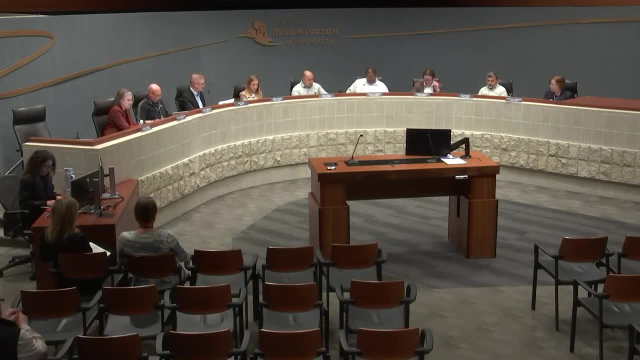 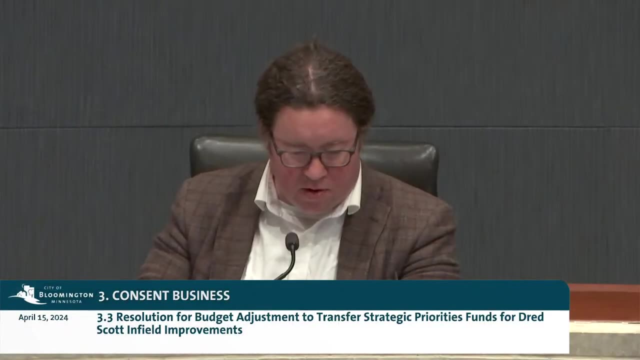 Aye. Opposed Motion. carries at 7-0.. Item 3.3, Council Member Nelson. Yeah, thanks, Mayor. First, I support this, the improvements there. My kids played a lot of softball, My wife plays volleyball there and other things. 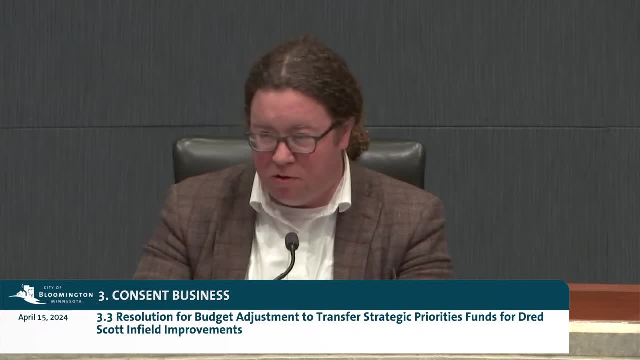 So I don't have a problem with that. This is another one of those areas of using strategic priorities money for things that I think should be in the regular budget, and just wanted to make that comment. If the situation is so dire that we know about it. 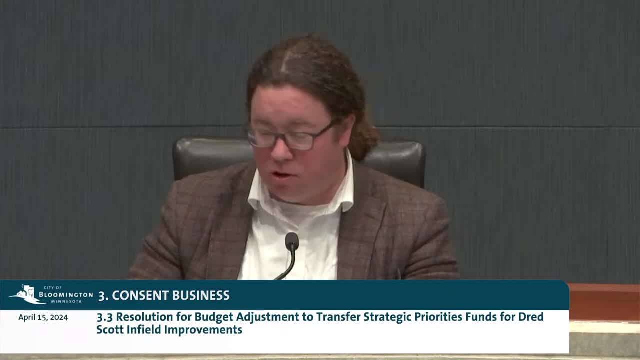 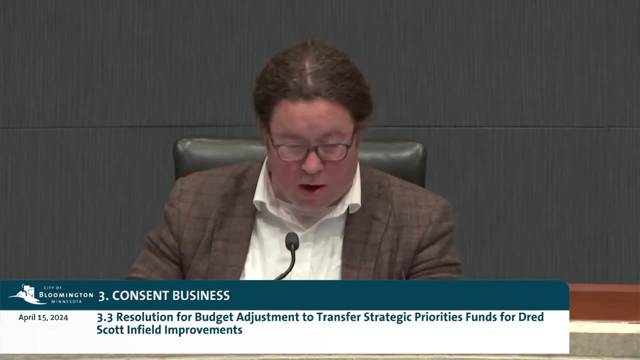 why wasn't this in the budget last year, and now we're pulling money out of strategic priorities, And so again, I think it just brings up that whole conversation about the use and need for and all of that of strategic priorities. Again, the project's great. 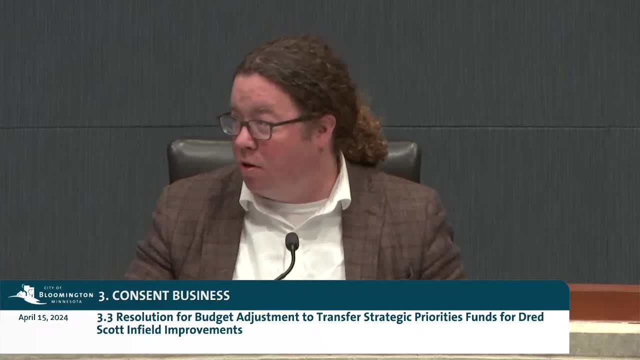 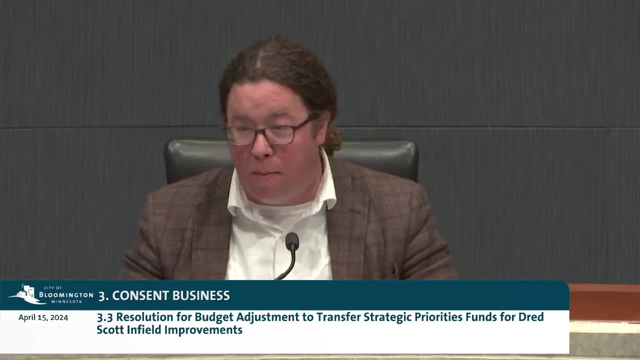 It totally makes sense to me. I remember my daughter squatting as a catcher with a broken sprinkler head in a puddle of water on one of the softball fields and definitely it's been an ongoing issue there On many of the fields there. 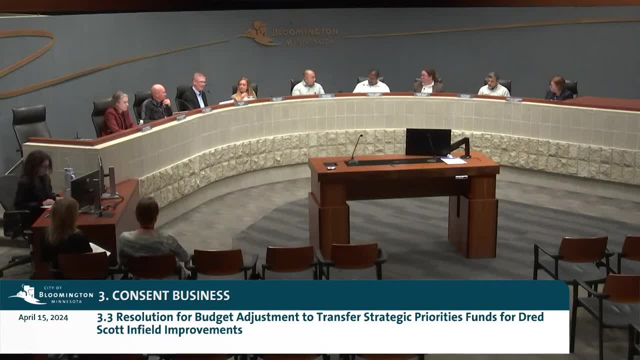 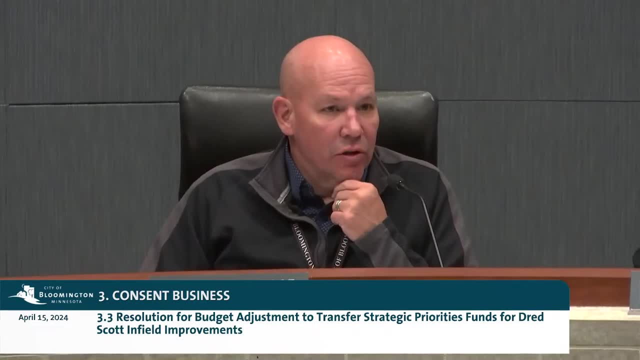 So appreciate this getting done. That's great. Just a budget question, Mr Verbrugge. Thank you, Mr Mayor, Council Members, Council Member Nelson. A couple of comments. First of all, the budget conversations Council will remember. 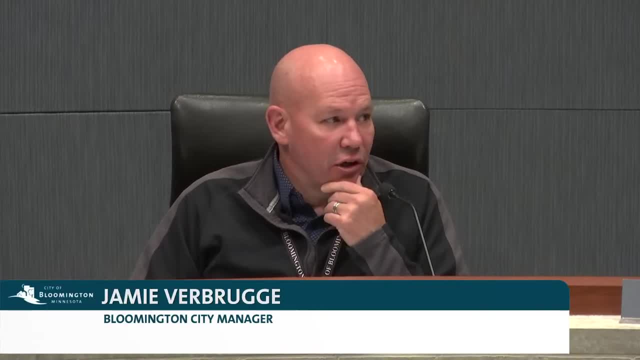 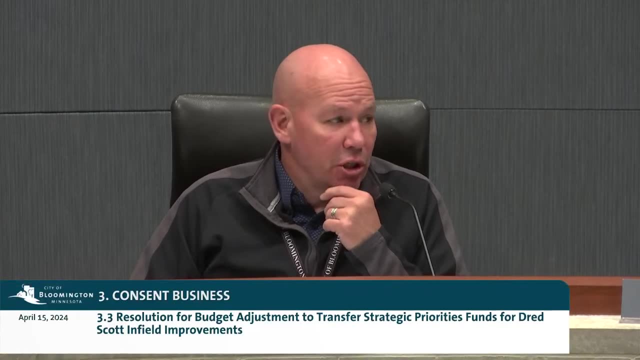 we were dealing with a pretty high levy and trying to limit the number of additions, increases in the budget. So you know, I think it's a good idea to have a budget conversation. I think it's a good idea to have a budget conversation. 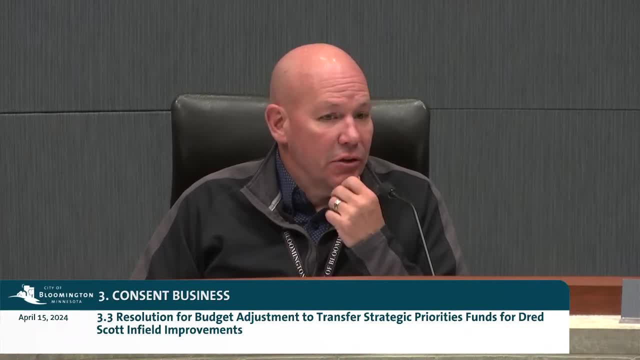 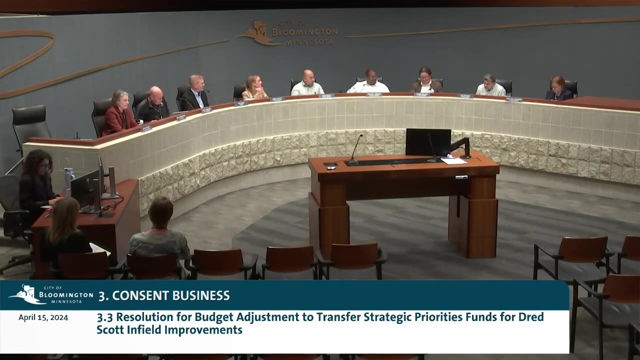 I think the project of this size would have had a substantial impact on the levy. Also, this is a capital project essentially, and we typically don't include capital projects within our operating budget. Council Member Nelson, any additional questions? Would you like to move Item 3.3?? 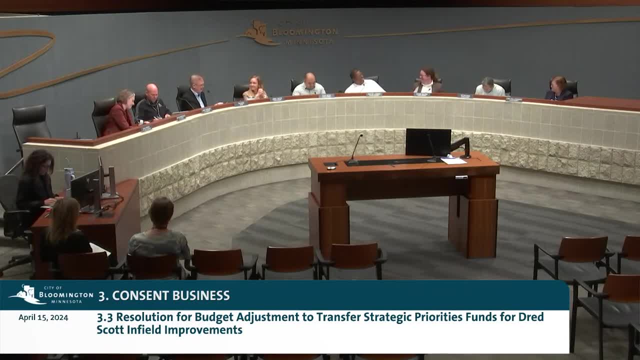 Second, We have a motion by Council Member Nelson and a second by Council Member D'Alessandro to move Item 3.3. That's a resolution for budget. The budget adjustments to transfer strategic priority funds to Dred Scott infield improvements. Item 3.3 on our Council agenda consent business tonight. 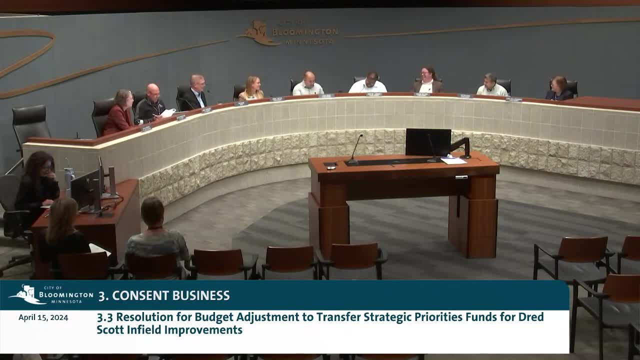 Second, We've already seconded it. We're good to go. We're good to go. Any further Council discussion on this Hearing none. all those in favor, please signify by saying aye, Aye. Opposed Motion carries 7-0 on Item 3.3.. 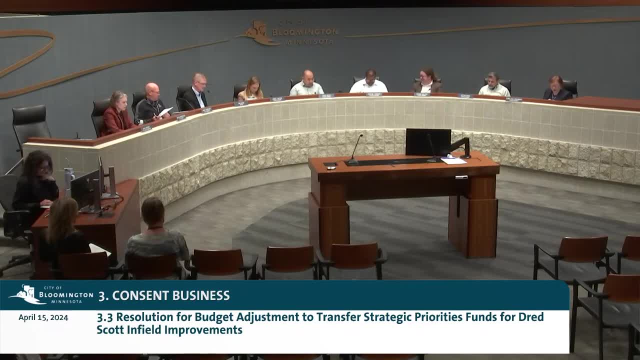 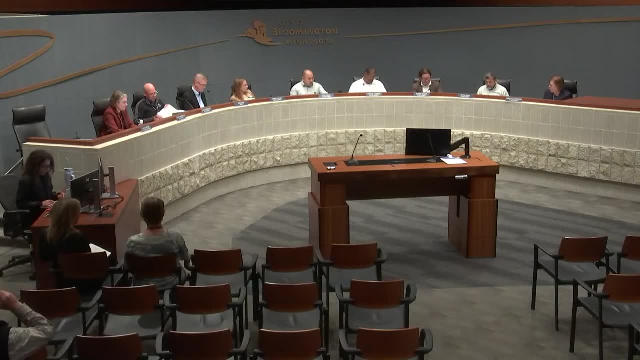 Council Member D'Alessandro, Item 3.1.. Yes, thank you, Mr Mayor. As always, just a special thank you to the folks. We're accepting donations on behalf of a number of people, both for our community service unit at the BPD. 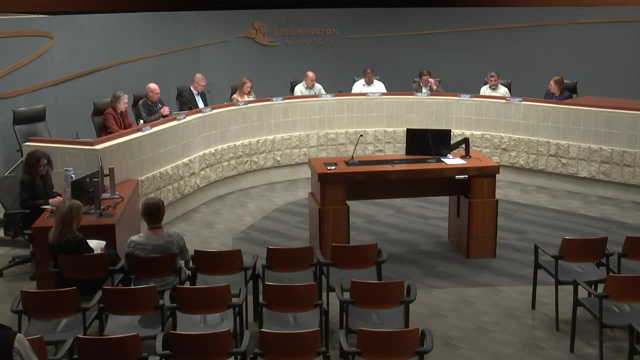 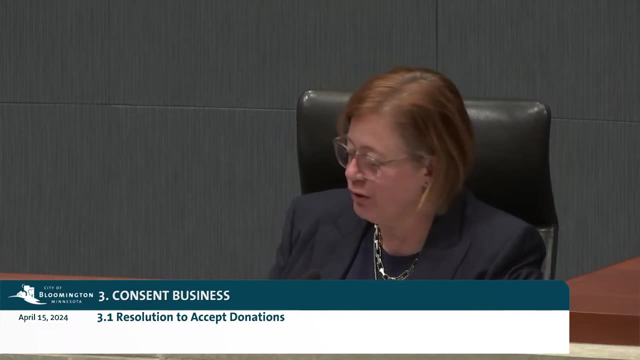 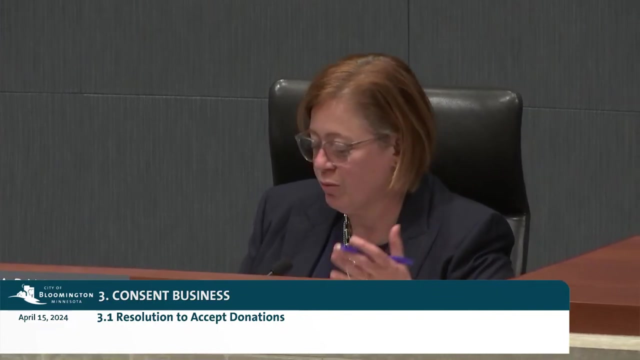 and also for the co-ed baby resource fair that we had. Obviously, as we know, people step up in amazing ways throughout this community, whether it's donating their time, joining commissions and other volunteer activities being part of our leadership development program. 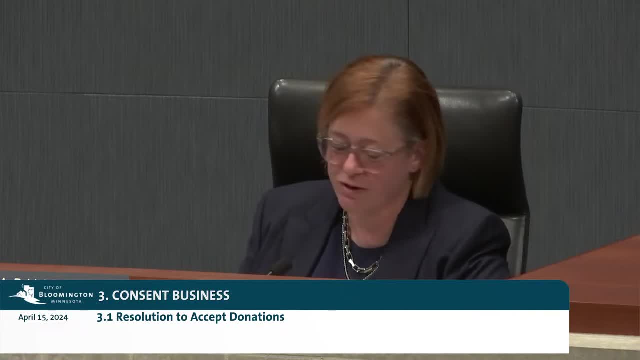 or contributing funds and resources to the support of our community. We see it every day. Just want to say thank you very much. There's lots of great opportunities to continue to do that and we're always really grateful. So with that I move. Item 3.1,. 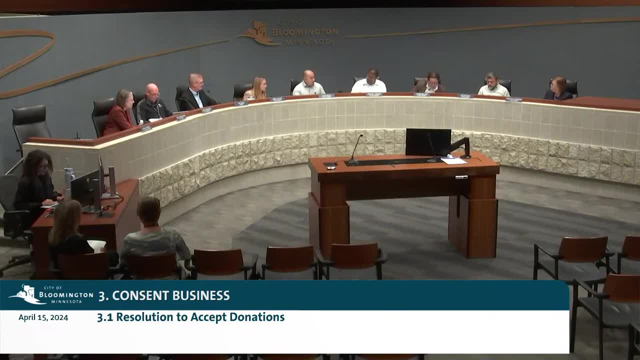 the resolution to accept donations as stated in the packet Motion by Council Member D'Alessandro, seconded by Council Member Mua, to accept Item 3.1, the resolutions to accept donations from our consent business: No further Council discussion on this. 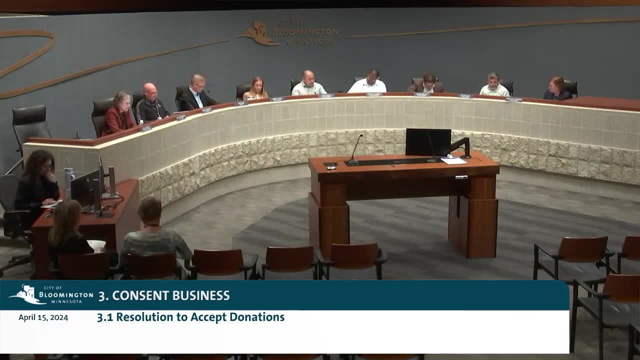 All those in favor signify by saying aye, Aye. Opposed Motion carries 7-0.. Thank you, Council Member D'Alessandro, You're welcome, Appreciate it. Thank you, Moving on to Item 4 on our agenda. 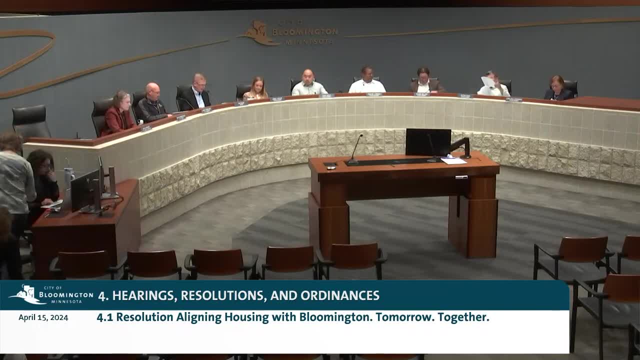 That's our hearings, resolutions and ordinances, And we have four items under Item 4 this evening or five items under Item 4 this evening. The first is Item 4.1.. It's a resolution aligning our housing policy and strategy. 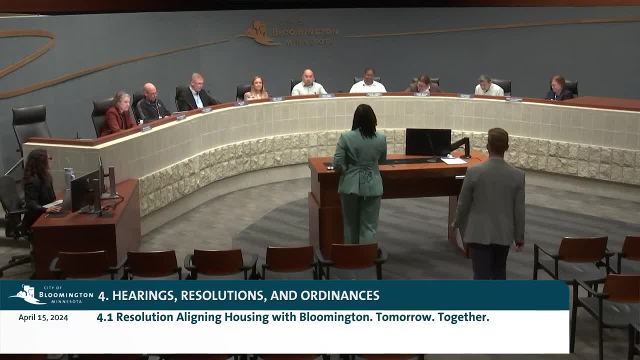 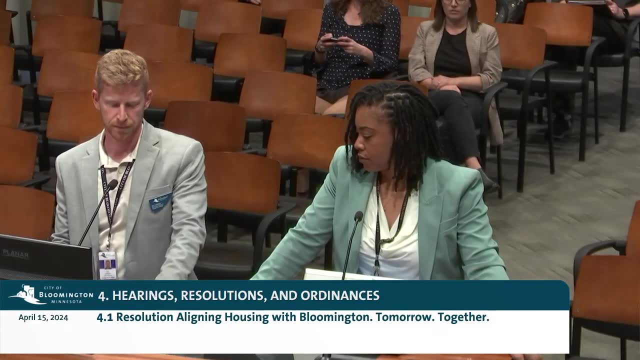 and all that we've got going on regarding housing with our Bloomington Tomorrow Together strategic plan, And Erica Coleman from our HR and Eric Holthaus from COED are here to lead us through this. Good evening and welcome. Good evening. Good evening Mayor, Council Members. 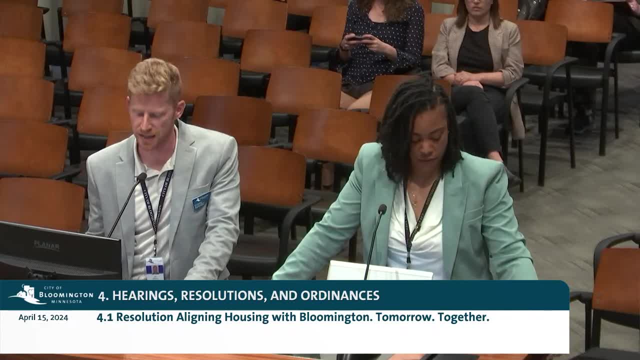 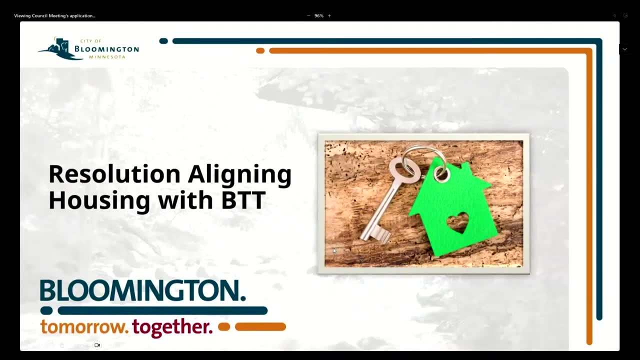 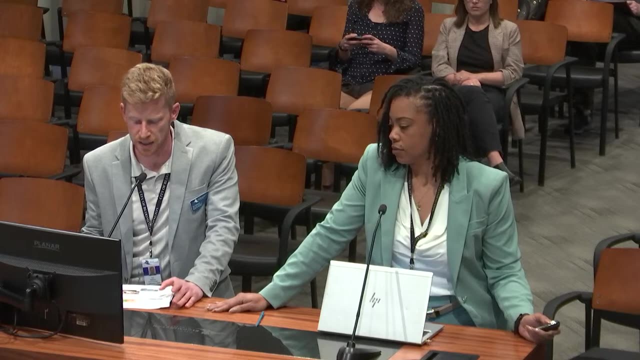 My name's Eric Holthaus. I serve as the Community Outreach and Engagement Manager. I'm also the staff liaison to the Human Rights Commission and joined by the Housing and Redevelopment Authority Administrator, Erica Coleman. tonight We are presenting the recommendation for the resolution aligning housing with BTT. 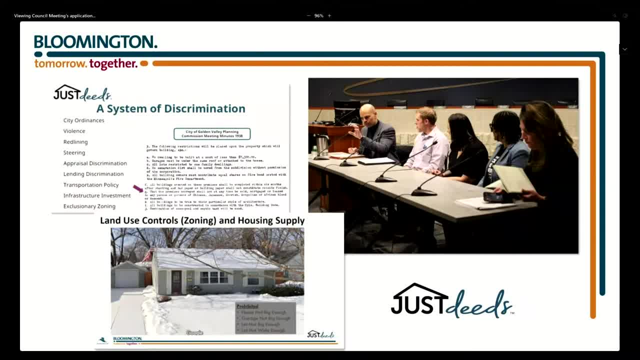 Bloomington Tomorrow Together. So efforts to grow housing access in Bloomington today build off of many efforts of yesterday, And these efforts are multidisciplinary. They involve leaders and actors in many domains: the city amongst city, council leaders amongst commissions, amongst the community. 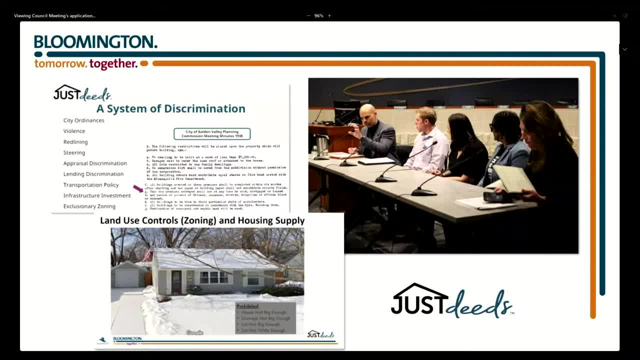 Just highlighting one special event. As the HRC staff liaison, I got to help support the special event Just Deeds and Beyond the legacy and future of housing access for all. This was a unique event that built off seminal work in 2021. 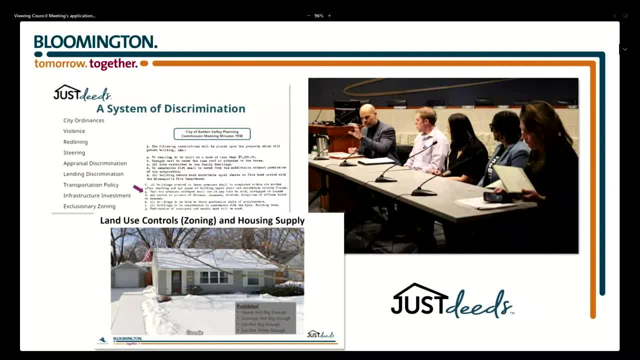 to highlight and understand exclusionary housing practices in Bloomington, across the region, across the state and country. This was sort of a repeat event to find out how far have we come. Many dozens of racial covenants have been discharged in Bloomington. 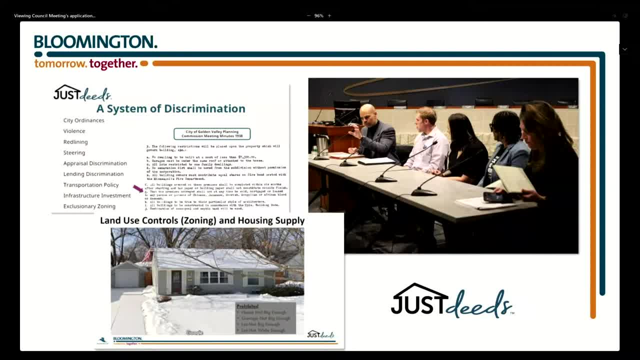 and more were discharged that night. Many other commissions joined just that evening to help make this event successful. Leaders from the community, many staff in many departments helped make that event possible as well. That's just one small highlight of how many are involved in housing. 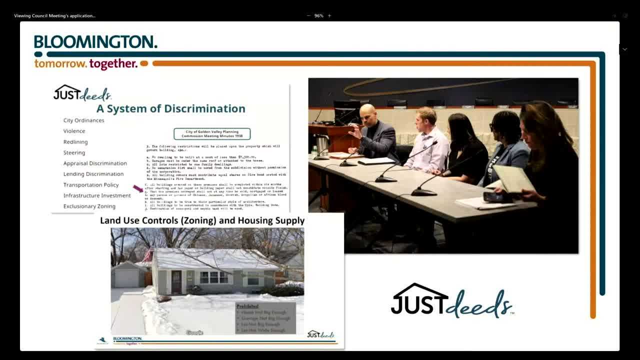 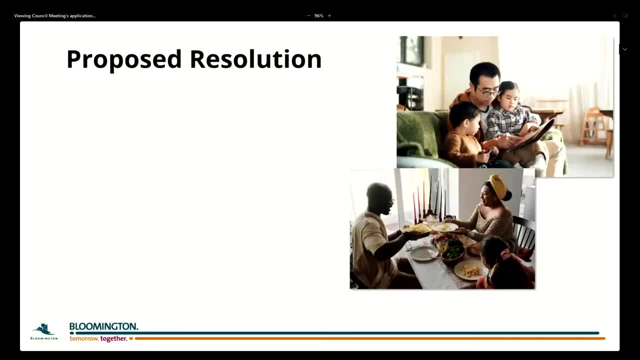 in many different ways here in Bloomington to see housing access become more and more possible for more people. The proposed resolution originated from the Bloomington Housing Action Team BHAT. BHAT is sort of another signifier of the collaborative effort that housing is here in Bloomington. 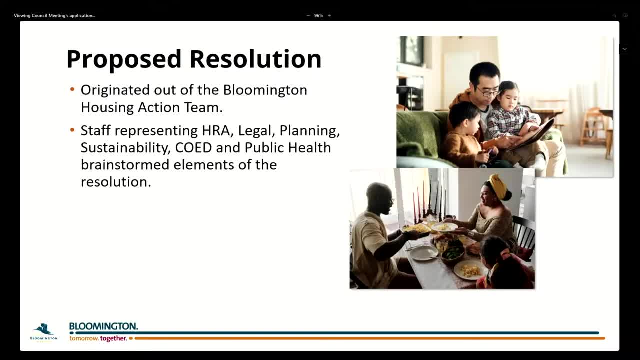 It's a consortium of staff and commissioners that are part of our many different commissions that touch housing. People that want to stay better connected and cross-pollinate these many different ideas about how housing can be furthered, how the housing access for all can be furthered. 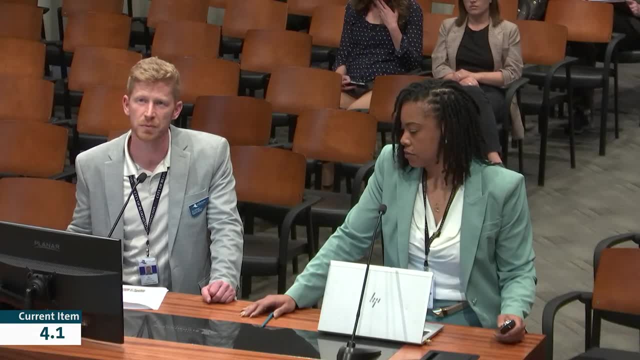 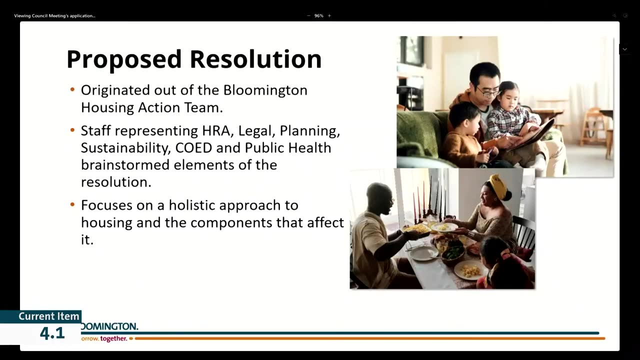 here in Bloomington. So staff representing HRA, social planning, sustainability, co-ed, public health, these are the staff that, following the recommendations from BHAT to move forward with this resolution. those are the staff that brainstormed elements of this resolution that you're seeing here. 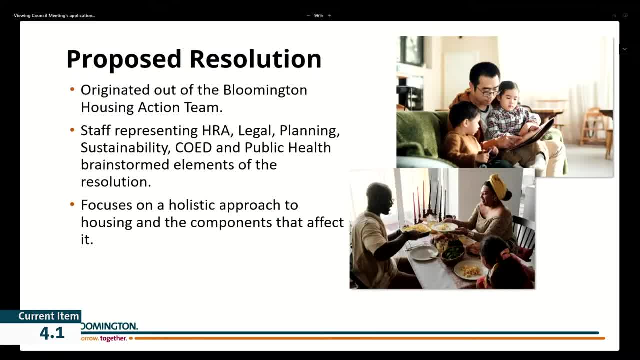 And the focus is very holistic. It's an approach to housing and the many, many components that affect it. Ultimately, what makes a house a home? There's a lot that goes into it. So, everyone, if you have any questions, 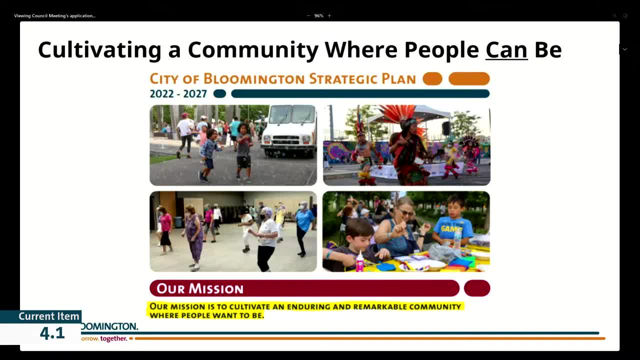 I'm happy to answer them And, of course, as familiar with the very important things that binds us together as a community and points to our future. Bloomington, Tomorrow Together. BTT, our city's strategic plan. The mission is to cultivate an enduring 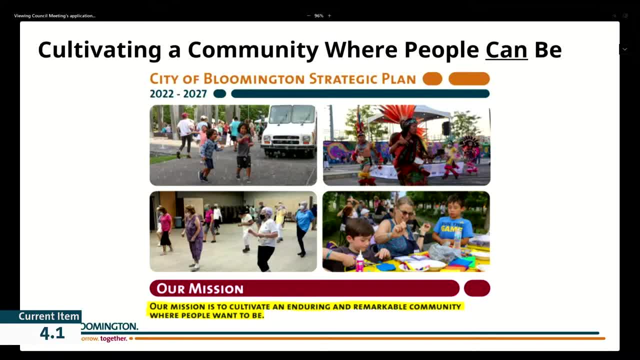 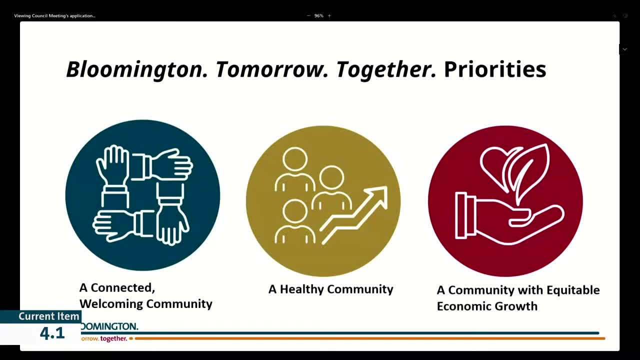 and remarkable community where people want to be, And this is very much focused on let's see that come true. let's make sure that we can cultivate a community where people certainly can be if they want to be here. off of that, Bloomington Tomorrow Together does have three main priorities for a connected 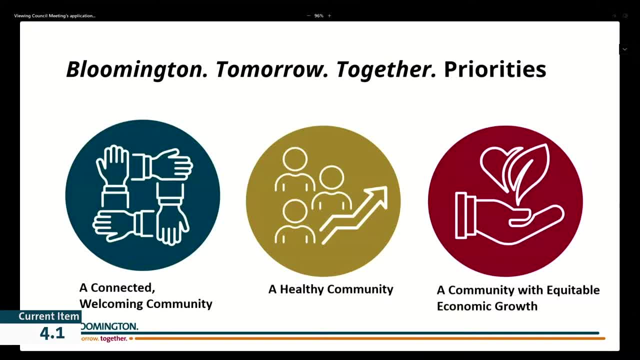 welcoming, healthy and an equitable economic growth community, and so one of the key ways to do that is housing people and housing people of their choice- affordable, decent, dignified housing options. and so how do we get there? well, I love to show this housing continuum. council member Carter. 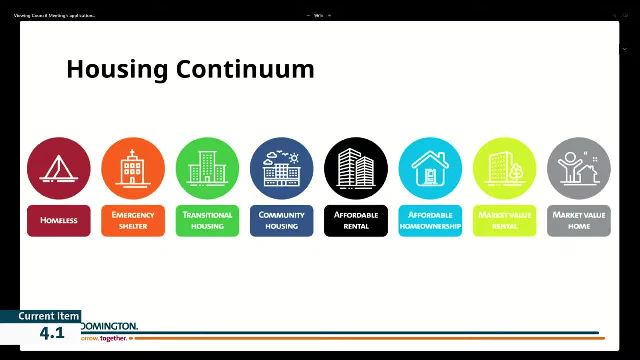 wanted to make sure that the housing continuum was present in this presentation, but what this housing continuum is is just showing that anyone can end up at any point on this continuum at more than one time in their life and there is no linear way to go about that. and the role of the HRA: the 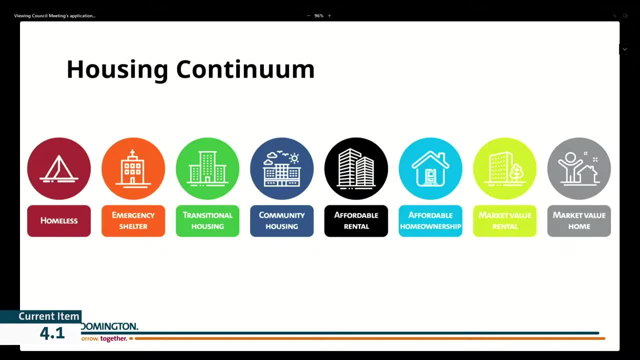 Housing Redevelopment Authority is to provide services, coordination and or programs along the housing continuum to truly meet the needs of the people of their choice, and so I think that's the key thing that really could be added, and, I think, the other things that I want to highlight. 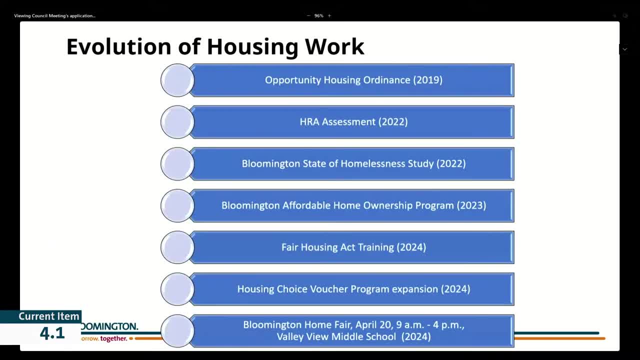 is that housing is the responsibility of current and future residents of the city of Bloomington, and so there's evolution of the work of the HRA in order to do that, and so, under the leadership of this council, the city leadership, as well as the HRA board, there are a series of things that have 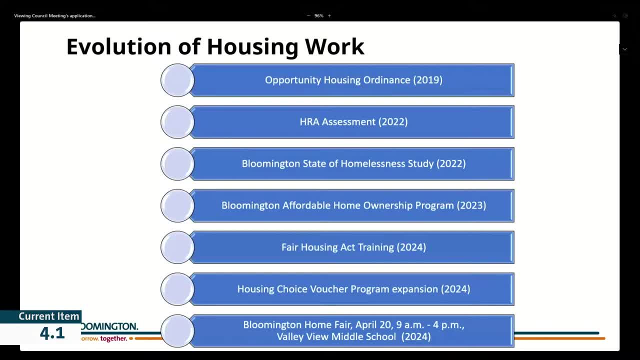 happened and we just highlighted just a few here. so in 2019, opportunity housing ordinance, which is our inclusionary zoning policy, in 2022, really taking a look at the housing and redevelopment authority in the work that it does and how that expanded to the Port Authority and the interconnectedness of not 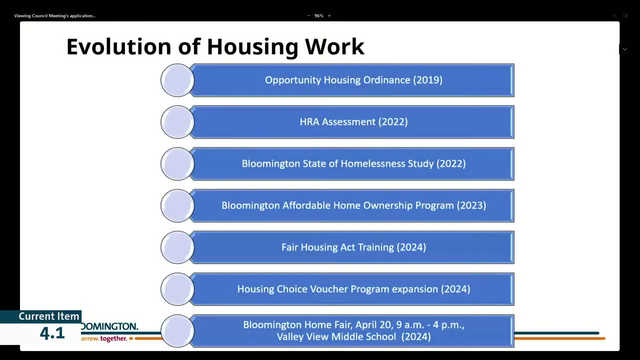 just the authorities, but the Community Development Department as a whole and the place that we hold in the city. Then, in 2022, we also looked at Bloomington State of Homelessness, of which we knew was exacerbated by the pandemic, but was not caused by the pandemic, and became a stronger. 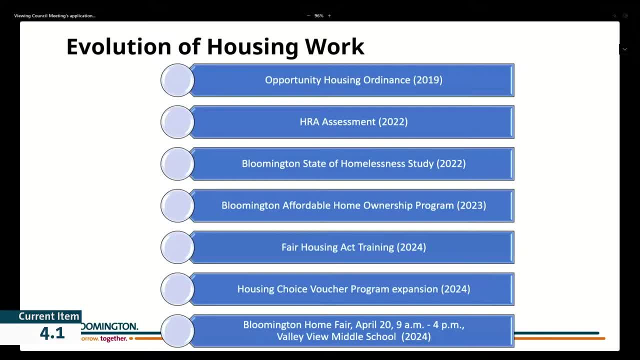 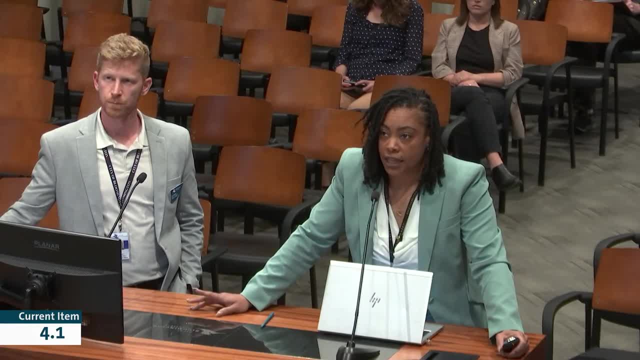 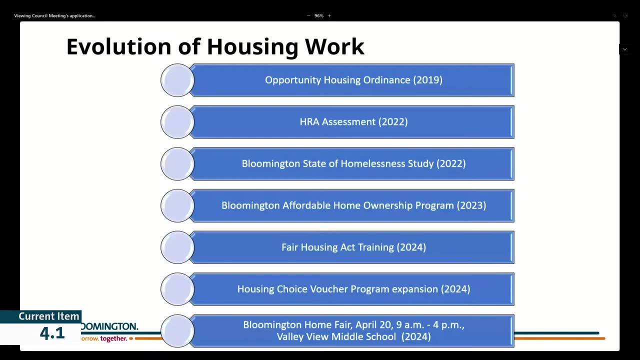 partner with Hennepin County, of which it is their role to work with the continuum of care plan and people experiencing homelessness in the county. Last year we were awarded funding for the Bloomington Affordable Homeownership Program, which is to build 27 new units of affordable 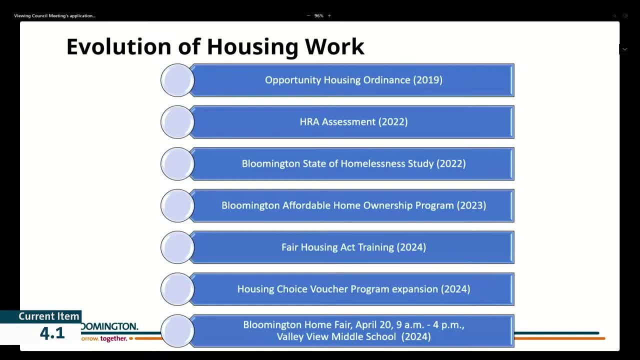 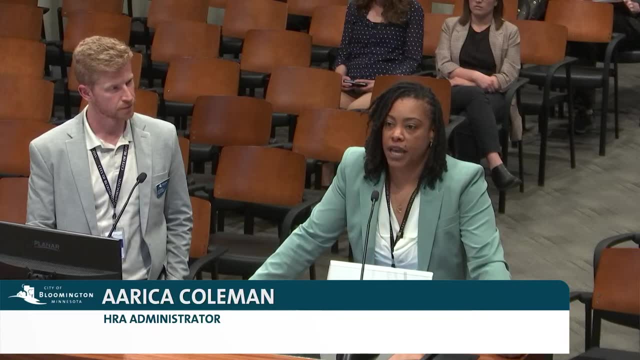 homeownership throughout the city that will be affordable at 80 percent AMI and working with small, emerging, historically underutilized and historically underrepresented developers. The reason for that gets back to that equitable economic growth in community. Next we have our Fair Housing Training- Fair Housing Act training that was completed by our legal department. 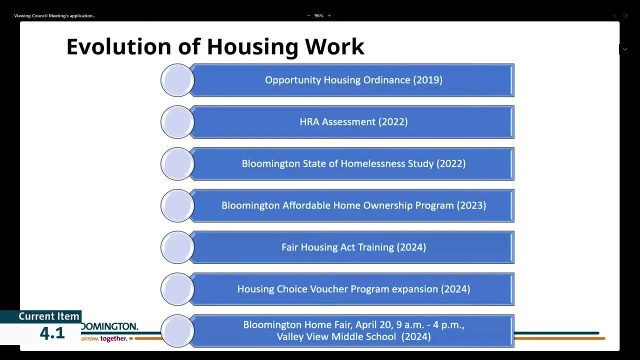 This was a great undertaking that legal did in terms of updating our fair housing policy and providing training for many, many division and departments throughout the city to make sure that we all are aligning with that. And then Housing Choice Voucher Program expansion- This in 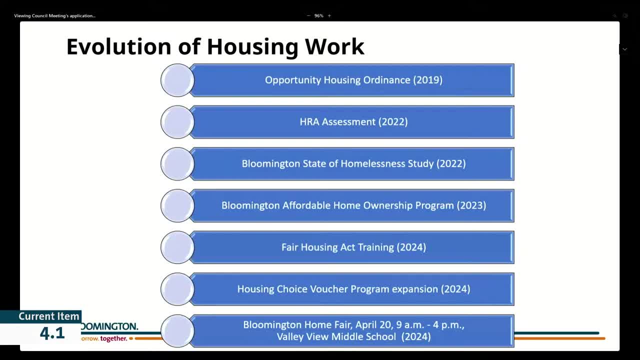 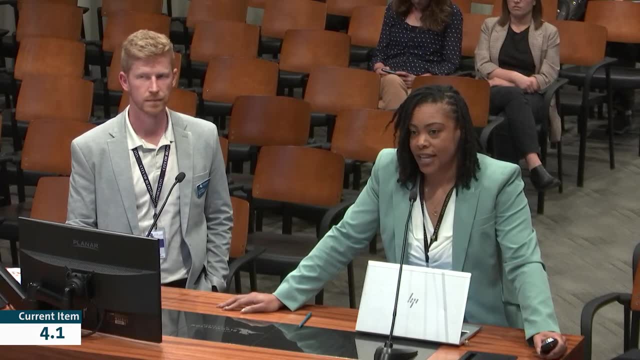 particular is for homeownership through the Housing Choice Voucher Program. Housing Choice is more commonly known as Section 8, but there is the opportunity that qualified eligible participants are able to use that voucher to go towards homeownership. And then, lastly, but 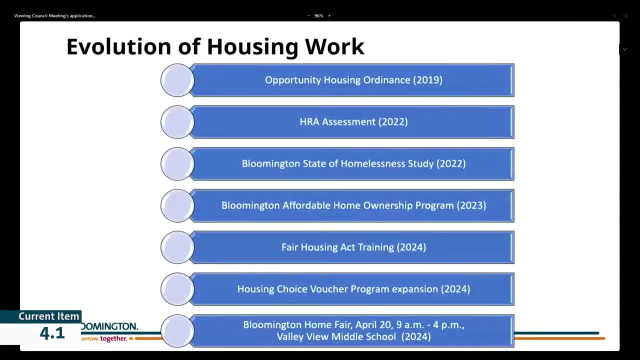 certainly, not least because I am so excited by this. this Saturday, April 20th, is our Bloomington Home Fair, from 9 am to 4 pm at Valley View Middle School. Now you might be asking yourself. 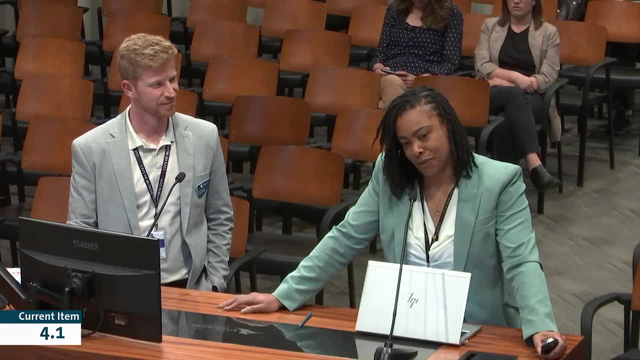 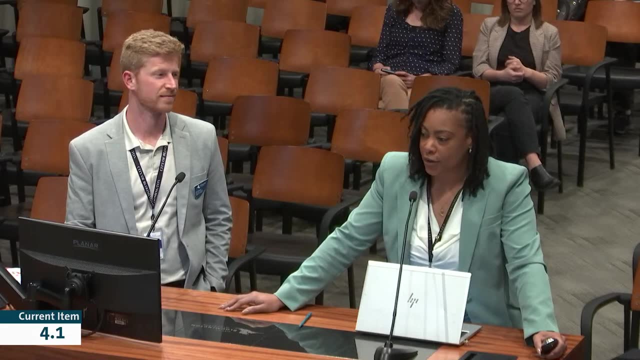 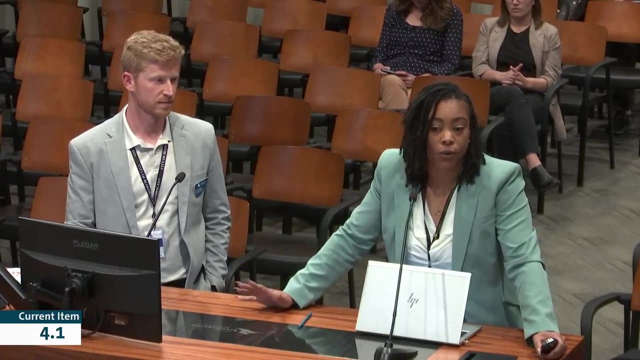 Bloomington Home Fair. yes, we have rebranded and expanded and this is no longer the Home Improvement Fair that is only for homeowners, but the Home Fair for everyone, regardless of where they are in their housing journey or living, renting, owning, wanting to rent, wanting to own. 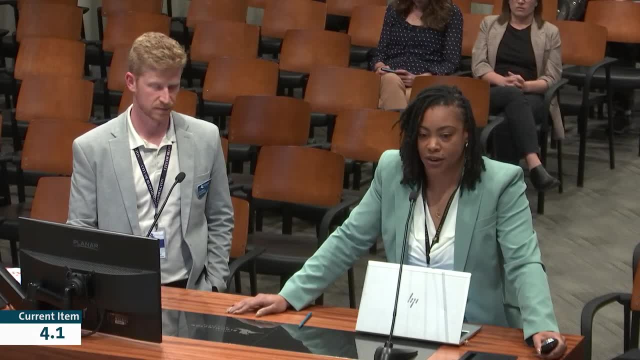 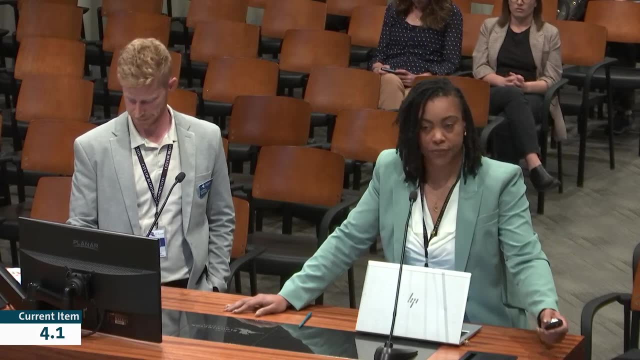 or just enjoying the wonderful services that the City of Bloomington offers. They can all join in at the Bloomington Home Fair at Valley View Middle School this Saturday, 9 am to 4 pm. And with that I can go back to the timeline of what has happened with this resolution And the. 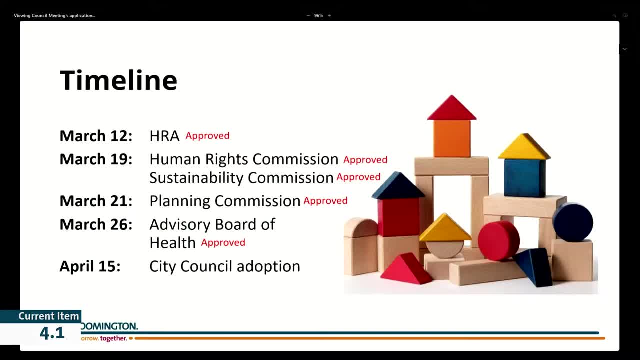 big thing about that is that the resolution, as I get to the next slide, will highlight that the Housing and Redevelopment Authority, through all of those actions in that timeline, is going to continue to work along the housing continuum and hold the place in Bloomington that it was designed. 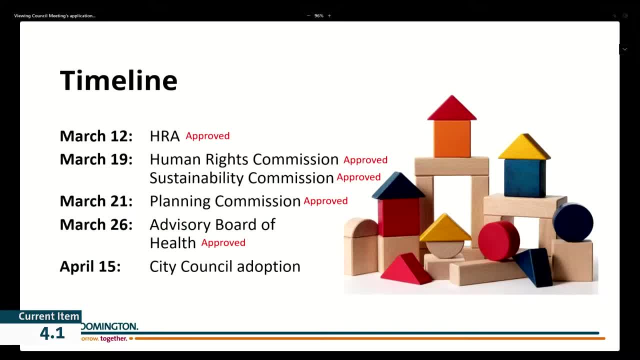 to hold, which is to help those not adequately served by the marketplace, and aligning with Bloomington Tomorrow, Together, where we're cultivating and enduring a remarkable community of homeowners. and we're cultivating and enduring a remarkable community of homeowners where people want to be, but we're making sure we're cultivating and enduring a remarkable 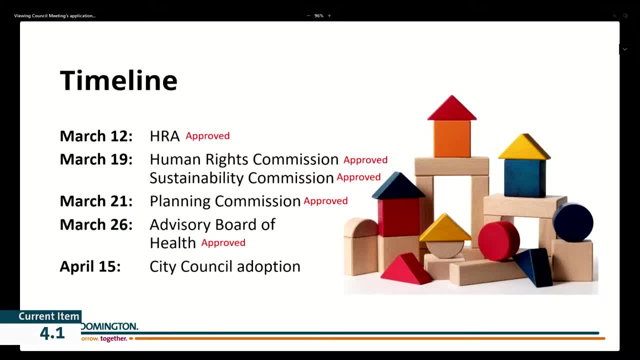 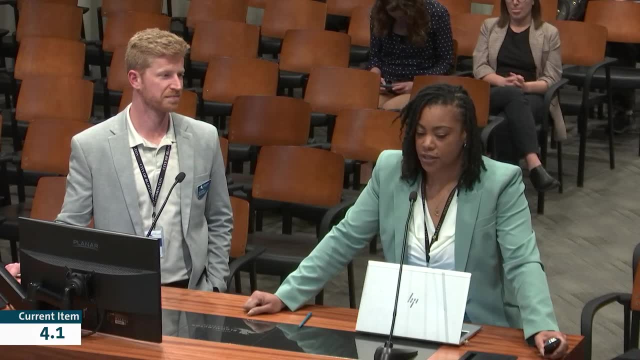 community where people can be. And so, in the month of March, this resolution was approved by the HRA Board, the Human Rights Commission, the Sustainability Commission, the Planning Commission and the Advisory Board of Health. And here we are on April 15th, Tax Day. but it has nothing to do. with this resolution, as well as Fair Housing Month for the City Council to adopt this resolution, And so Fair Housing Month That is. it is the- I believe- the 56th anniversary of the passage of the Civil Rights Act of 1968,. 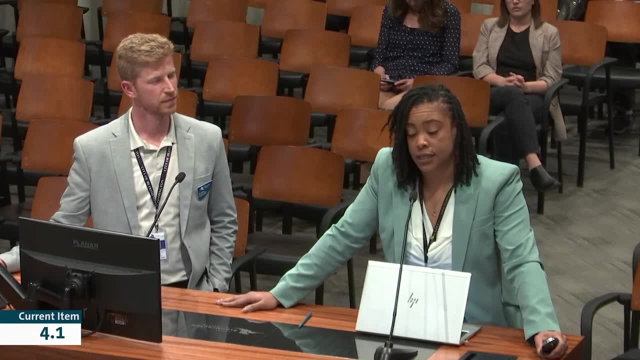 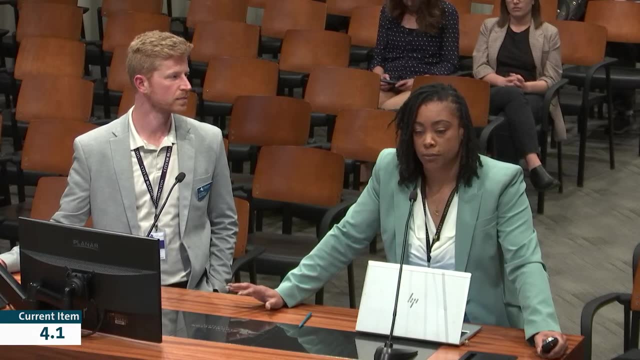 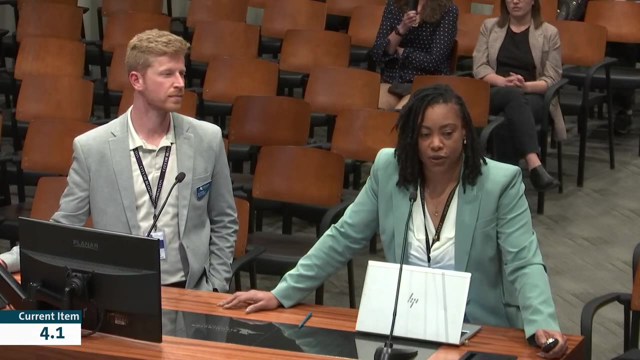 which was allowing for fair housing, which does come against discrimination in renting and buying and mortgages of just being able to maintain and obtain housing, And so we thought it was very fitting to bring this forward during this month, And with that, I'd like to thank all of you for joining us, And I'd like to thank all of our. 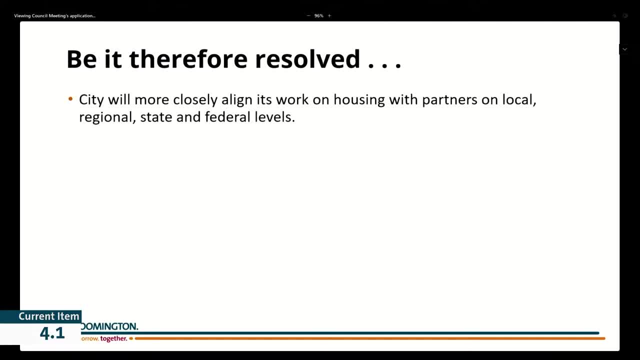 panelists for joining us And I'd like to thank all of our panelists for joining us And with that, we ask that it be it therefore resolved. The City will more closely align its work on housing with partners on local, regional, state and federal levels. HRA will continue. 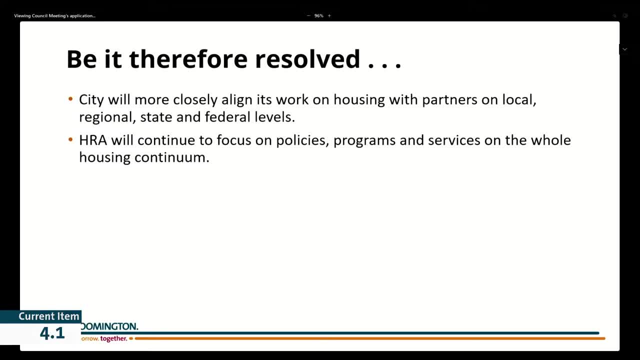 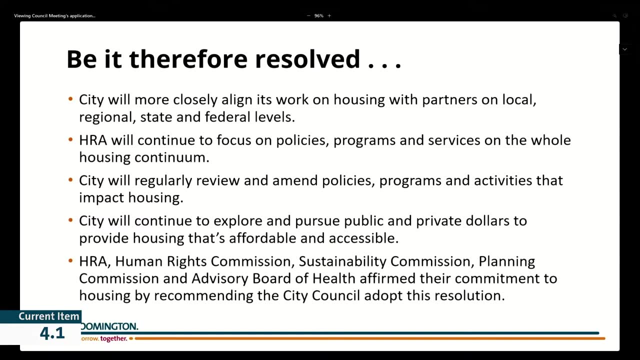 to focus on policies, programs and services on the whole housing continuum. The City will regularly review and amend policies, programs and activities that impact housing, And the City will continue to explore and pursue public and private dollars to provide housing that's affordable and accessible. And then the HRA will continue to focus on policies, programs and 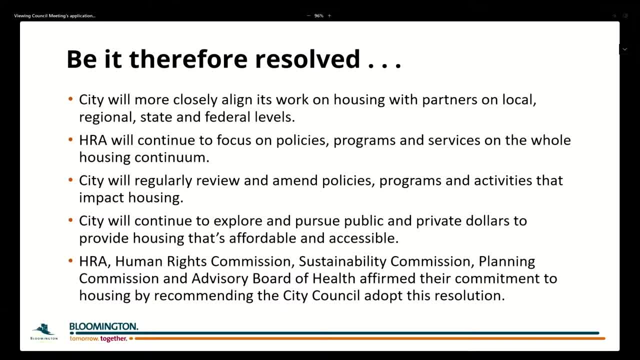 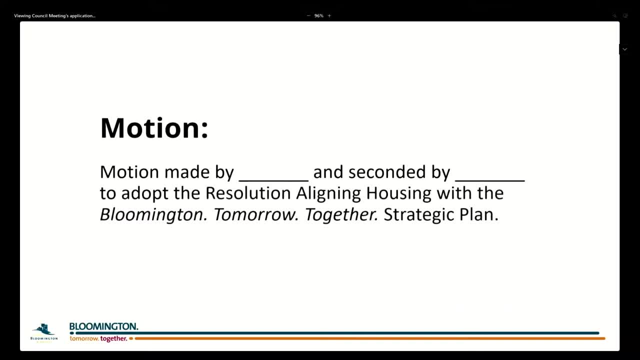 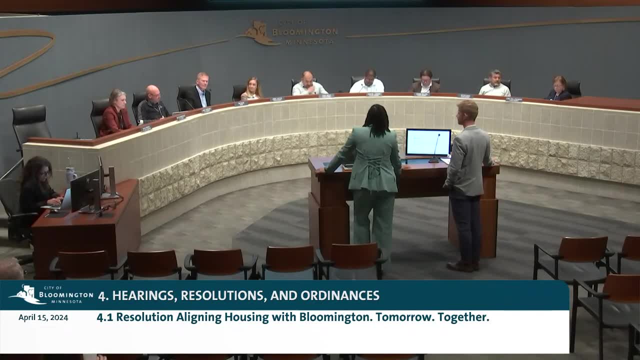 services that impact housing, that affect the community, And then the City will continue to approach, Undertaking and Motivating the Community And we're expanding the agenda on housing and치가, our HRA, Human Rights Commission, Sustainability Commission, Planning Commission and 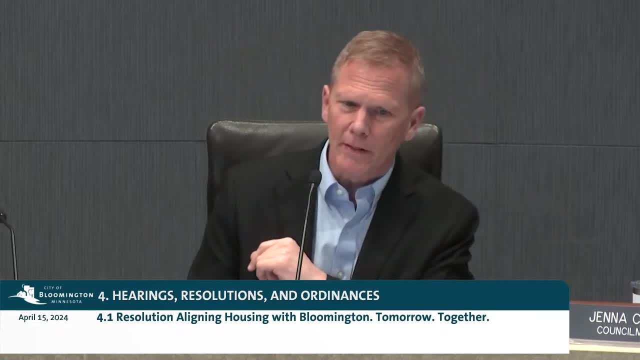 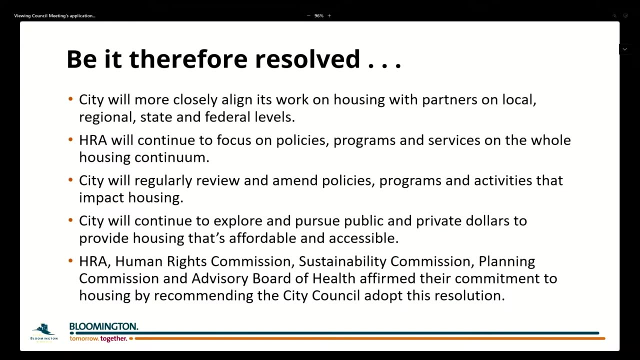 Advising Board of Health affirmed their commitment to housing by recommending the City Council adopt this resolution And with that we can stand for any questions, but we look for a motion for your our work on housing with partners on local, regional, state and federal levels, and I'm 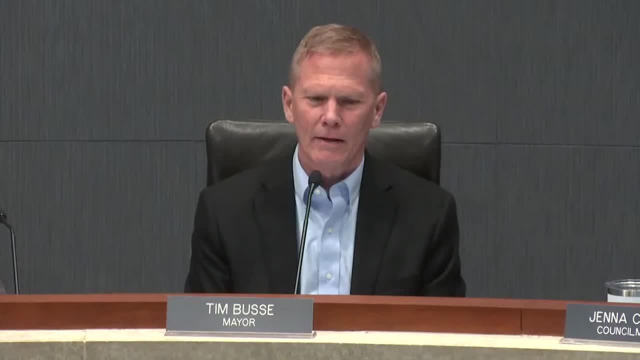 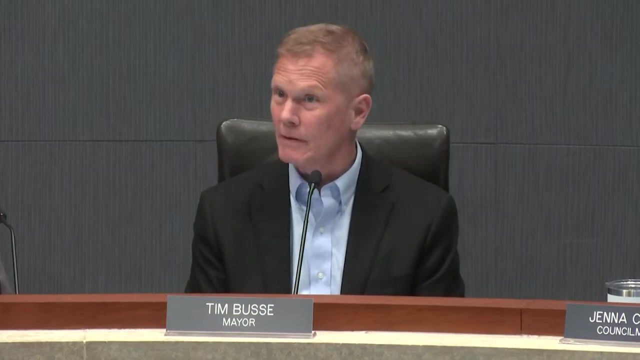 going to ask that we do even more and we try and bring along our neighbors in cities who are perhaps not working to align their housing goals with local, regional, state and federal-level partners, because we know they're there, We know that conversation is taking place right now and we know that it's. I think. 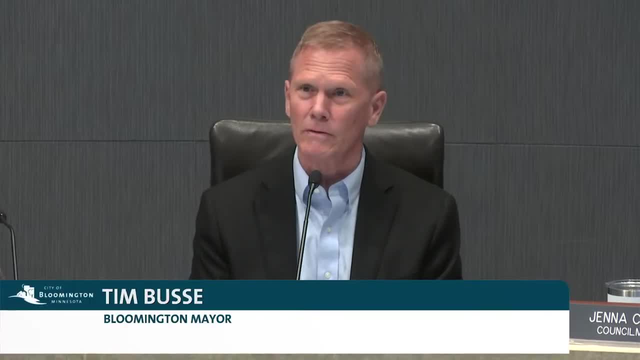 a contentious discussion among some of our neighbors in some city halls across Minnesota, and I would like to see Bloomington work in a leadership role to try and bring everybody along with us on this journey. That's what I would like to see. I don't know if it makes sense. 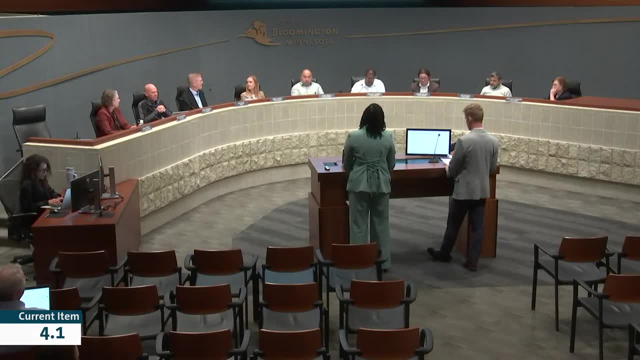 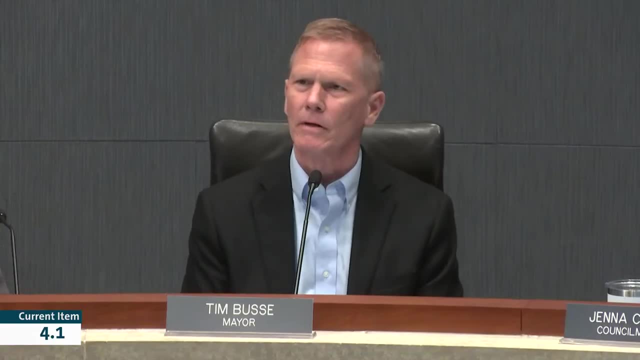 I don't know if we want to change the wording at all or just make this something that, a statement that we want to see happen, but Bloomington is miles ahead of so many other communities and would love to see Bloomington Bring those folks along, in some cases kicking and streaming, in some cases willingly. 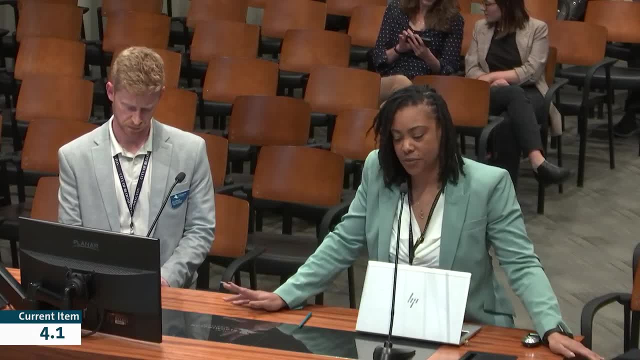 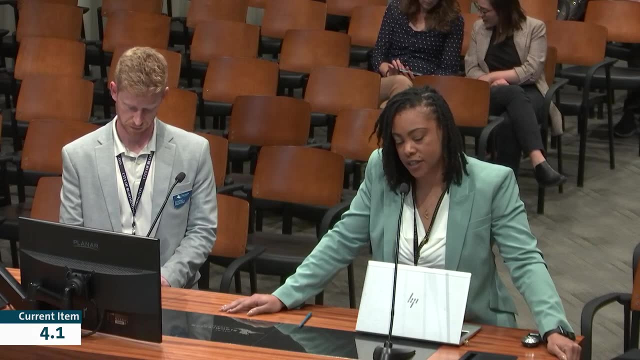 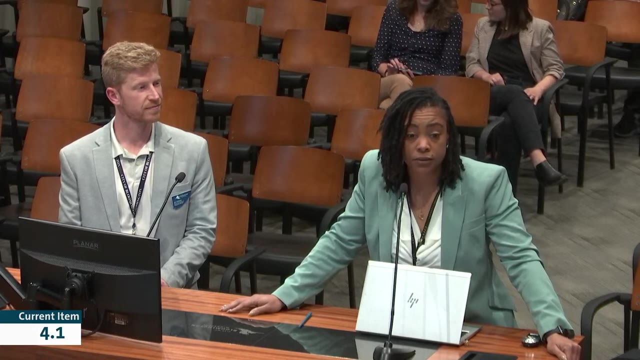 but I would love to see Bloomington bring those folks along. So thank you, Mayor and Council. I just want to add that I do know that the wonderful staff that is here in Bloomington is actively doing just that, and I want to say that it's not always loud and pronounced. 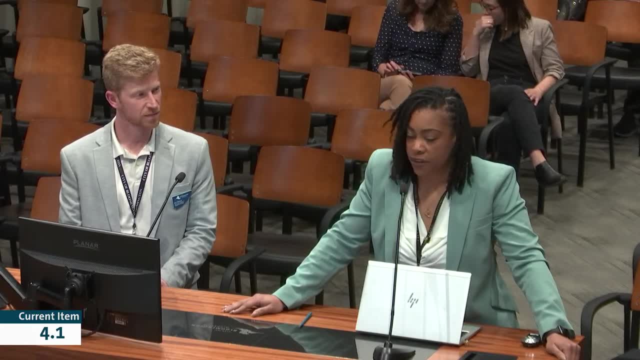 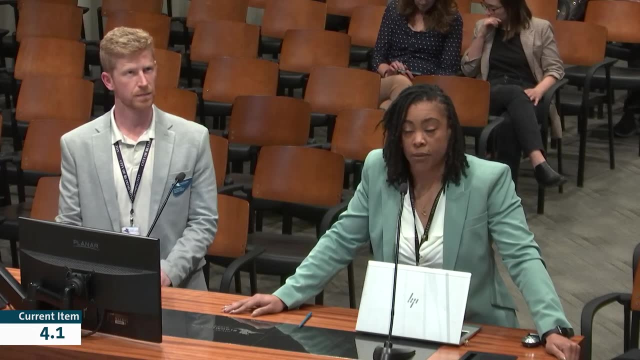 or in your face, but I do know for a fact that staff is having those conversations, conversations with their colleagues across the Twin Cities Metro, in a manner that is educating but also learning from each other, and then I would be remiss to not highlight 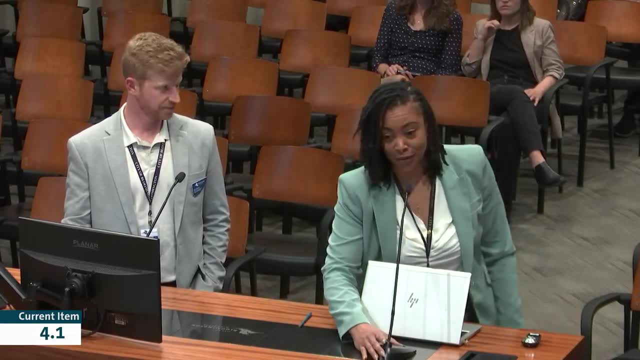 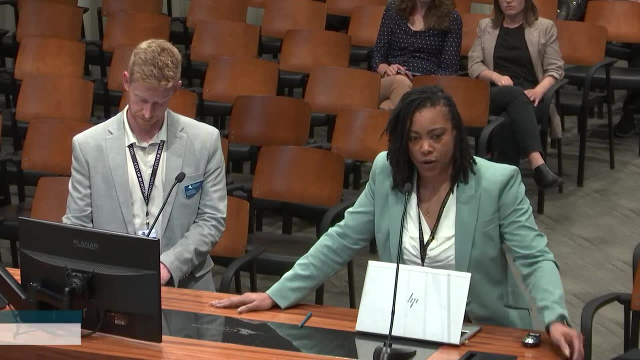 that the American Planning Association is having their national conference right now in Minneapolis, and when I talked to our wonderful manager, planning manager Glenn Markagard, he said they're all working on the same thing. It's very interesting how we're so aligned. 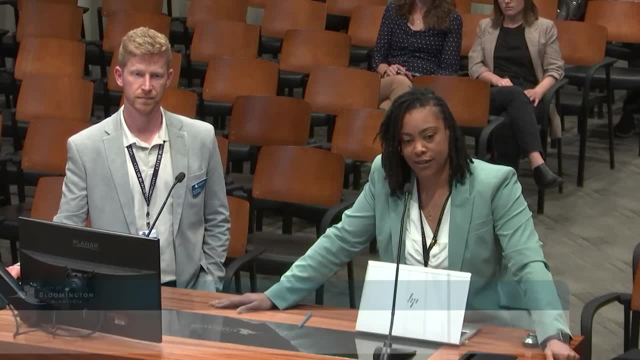 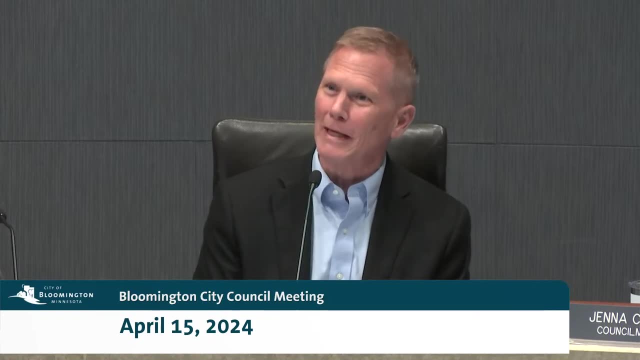 So I just want to give you that, Mayor, that it is in there, We are doing it And we will continue to do so, And I appreciate that and I will share also that your elected officials are also working in the same manner with other elected officials across the 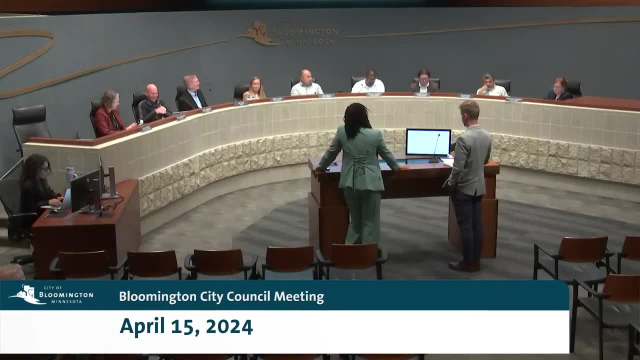 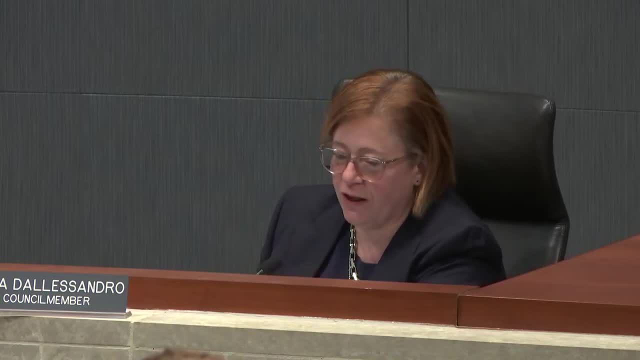 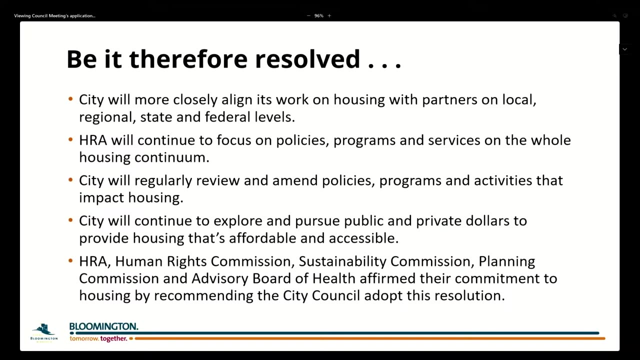 And we appreciate you And we appreciate your work as well. Council Member D'Alessandro, I saw your hand up. Thank you, Mr Mayor. It was just a proposed small amendment that we could make to that first resolution bullet point that would say something like: City will more closely align its work on housing with partners. 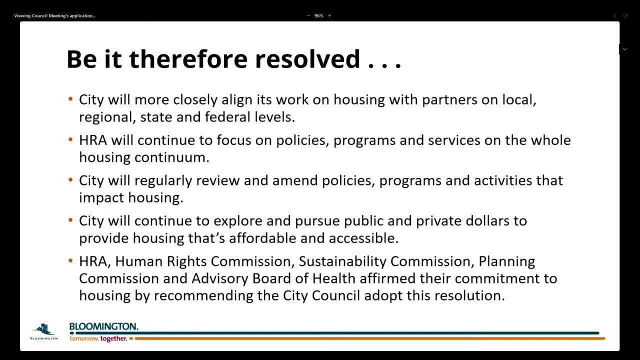 local, regional, state and federal levels, including other specific entities, if you want to note them. or we could say metro area, or we could say elected officials. I mean, we could do something that just adds the specific connotation you're trying to make there. 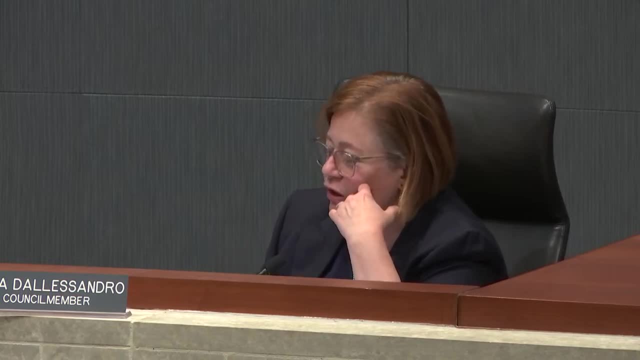 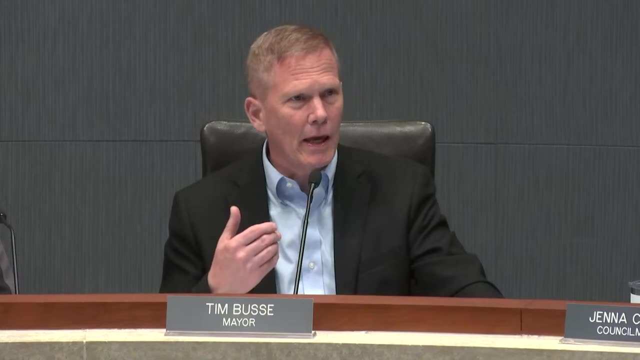 at the end of that. that might highlight the specificity you're looking for. on that part. I appreciate that, I think. My goal, I think, was align its work and leadership. I was looking for another action verb as opposed to calling heart supply. 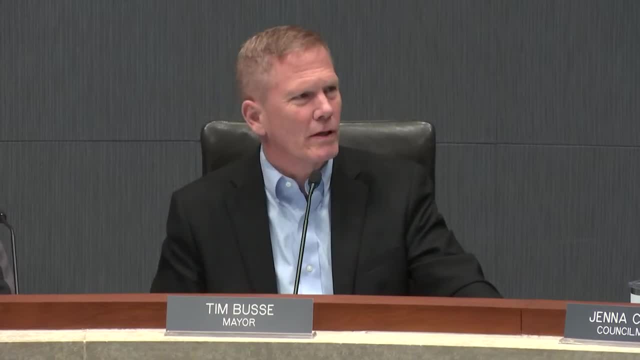 specifics. I was looking for an action verb in there that uh, yeah, align its work and actively promote. actively promote I was going to say flex its muscle, but I don't think we want to say that, uh, actively promote or or provide active leadership within, yeah, the state of. 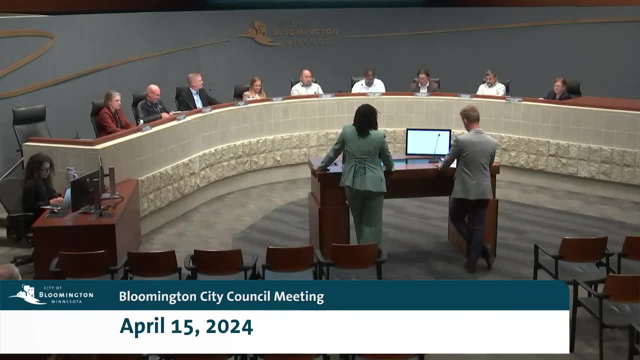 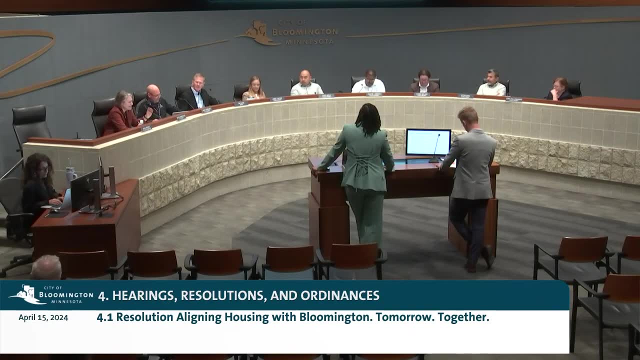 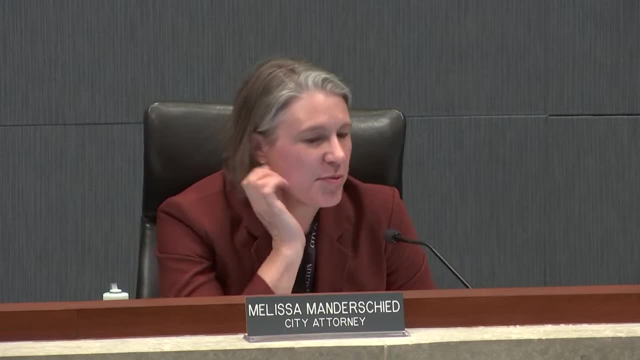 Minnesota. I think that would fit nicely in that first sentence if we wanted to amend something. Ms Manderscheid, we're we're editing on the go here. I'm sorry, mayor members. um, so the presenting staff prepared powerpoint slides. they're not directly verbatim from the resolution. the resolution's on page 131 of your packet. 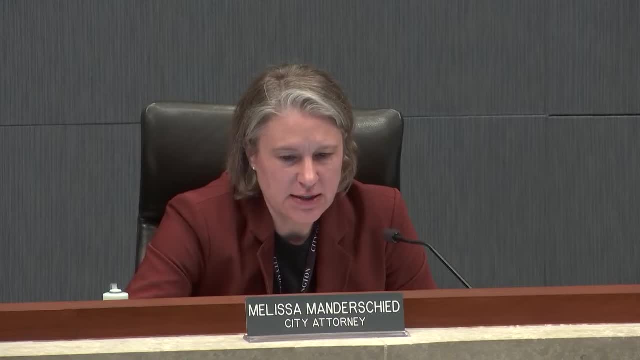 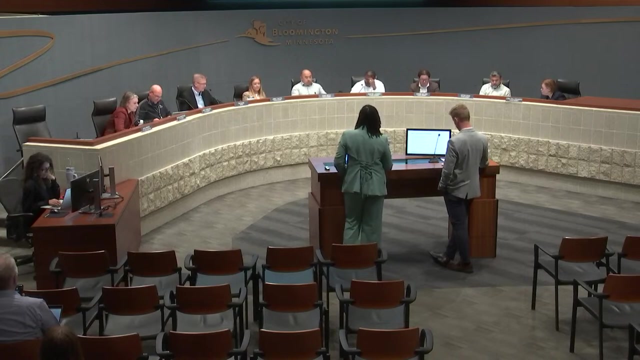 I am scanning it. I believe it's in the be it further resolved, uh. whereas it says where the well, you can read it yourself: um, uh, maybe to promote and support. um, show, um, um, To lead and promote. how about that? in federal levels, to lead and promote? 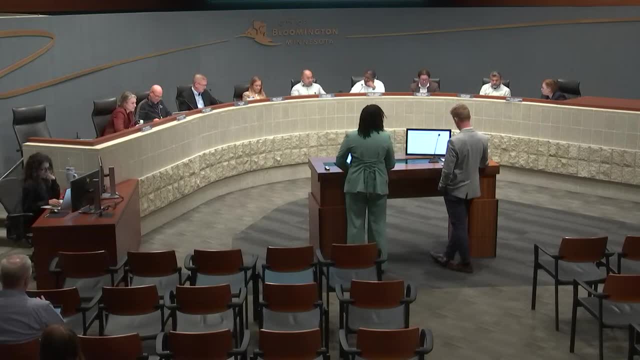 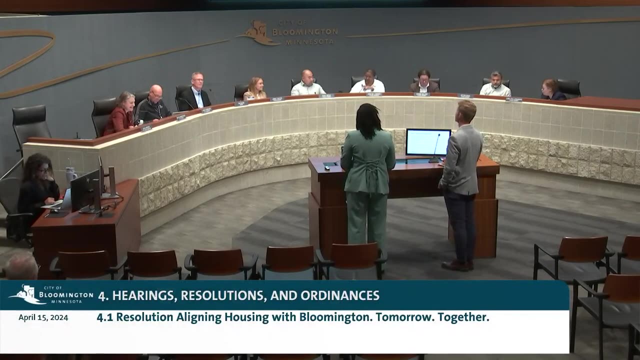 how about? is that what you're thinking? maybe I? I am thinking I yes something along those lines- a more active type of verbiage to, to encourage continued leadership by the city of Bloomington to lead comma, promote comma and support a full range. love it, Oxford comma. yeah, I'm in for that. 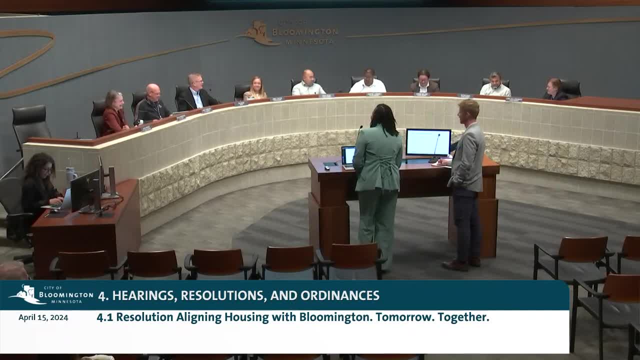 love it, you? uh? all right council questions on that, or are we? are we okay with that? what of the? which of the resolutions are we are we men amending? sorry, mayor members, It's page 131 of the electronic packet. It is the, uh, the now. Therefore, not that clause, the be it for further. 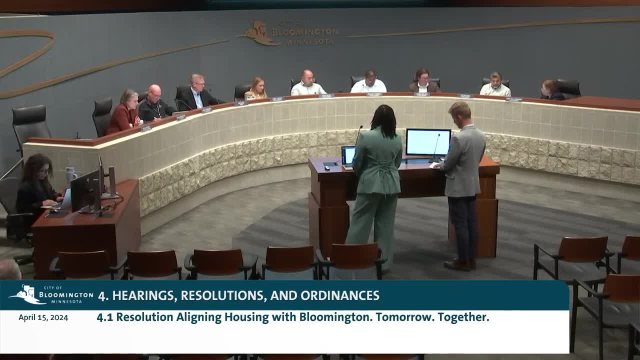 resolved, Not that one, It's the next one. be it further resolved that the city of Bloomington, warm, will more closely align its work with partners on the local Comma, regional Comma, State Comma and federal levels to lead Comma- and If the now Therefore not the cause, that further resolved, not that one, It's the next one. Be it further resolved that the City of Bloomington more. more closely align its work with partners on the local Comma, regional Comma, State Comma and federal levels to lead Comma with partners, trusted organizations on the local Comma or regional, requesting for their comments as an incr松 Angeles to et al and support a full range of. 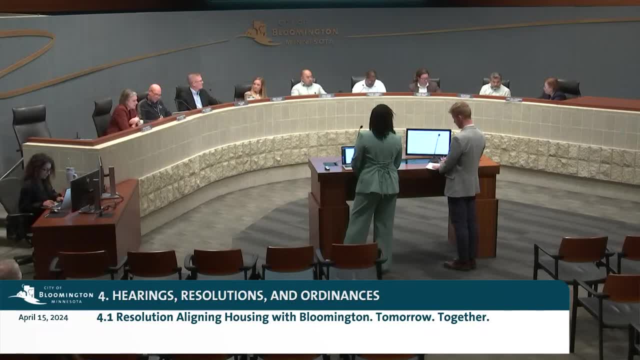 housing choices throughout Bloomington, et cetera, et cetera. Does that work? Not just Bloomington, though? right, Right, No, I just stopped talking. Yeah, Yes, So a range of housing choices throughout Bloomington, and 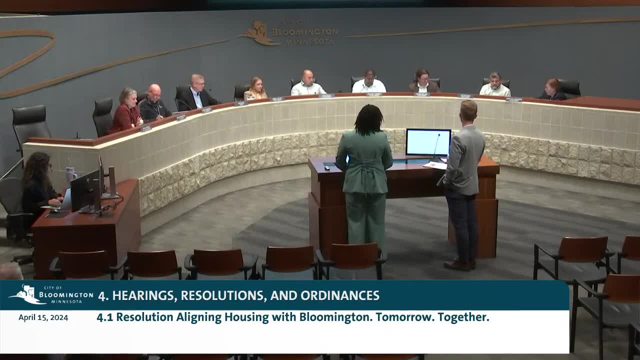 throughout Minnesota Or the metro area or whatever you were. That was the other piece of it. I thought That's a good point. That's a good point We could remove throughout Bloomington and make it a full range of housing choices throughout Bloomington and 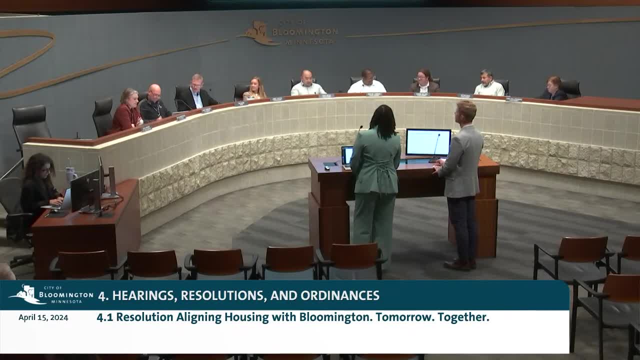 the region- Okay, Let's do that All right, In federal levels to lead and promote and support a full range of housing choices throughout Bloomington and Minnesota And the region And the region. Okay, One more time In federal levels to lead. 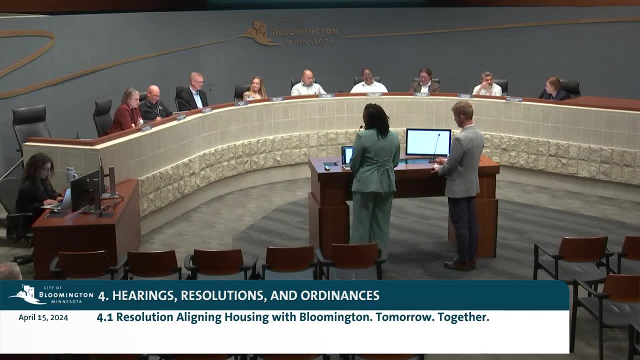 promote and support a full range of housing choices throughout Bloomington, the metro, excuse me, the region, Minnesota. yeah, that meets the needs of people at all income. yeah, okay, everybody comfortable with that sense? staff, are you comfortable with that little wordsmithing on the go here? but I think it's important to to call out the 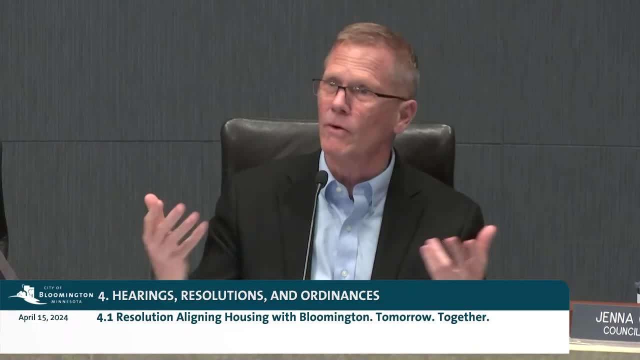 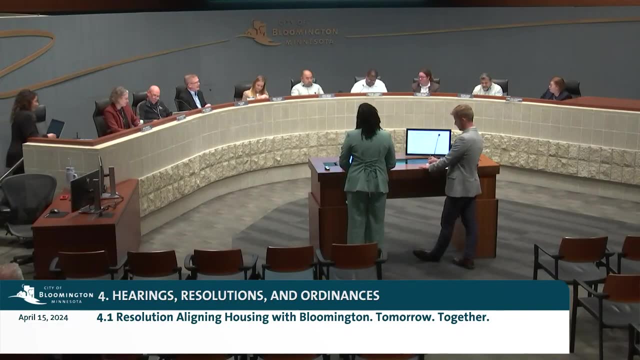 leadership that you have shown, that, that we have shown that this community has shown on this issue. if that's fair, it is- thank you everybody, comfortable with that council. all right, any additional questions, any additional comments? here you advance one more council. I would look for action then. happy to make the 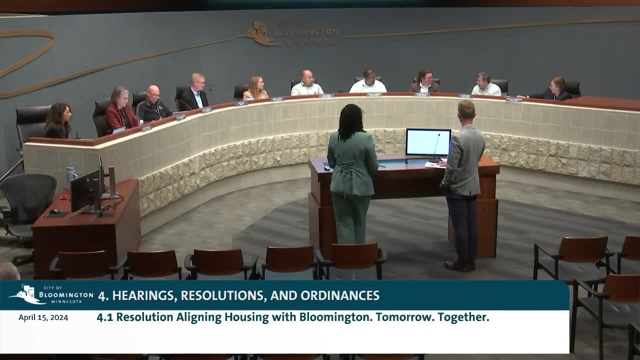 motion: mr mayor, councilmember D'Alessandro- fantastic, I didn't even say it, he's seconding it. I love it. I move to adopt the resolution aligning housing with the Bloomington tomorrow together strategic plan, as noted in the council meeting. we've got a motion by councilmember D'Alessandro, second by: 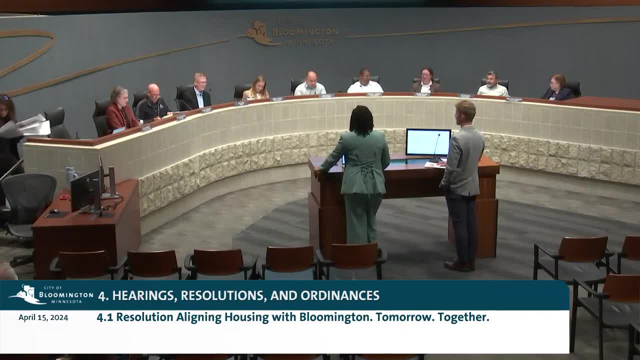 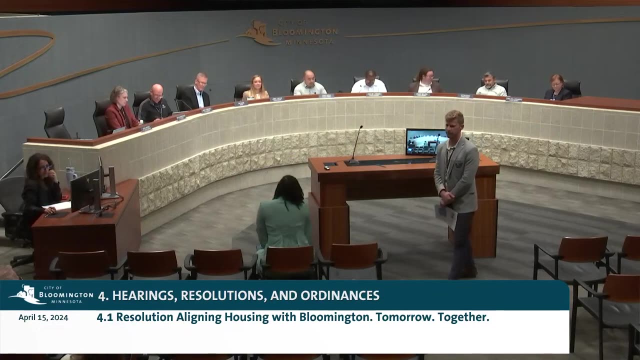 councilmember Rivas to adopt the resolution aligning housing with the Bloomington tomorrow together strategic plan, as noted in our council discussion here in the council meeting. any further council discussion on this hearing none. all those in favor please signify by saying aye, aye. opposed motion carries 7-0. thank you, thank you much. item 4.2 on our 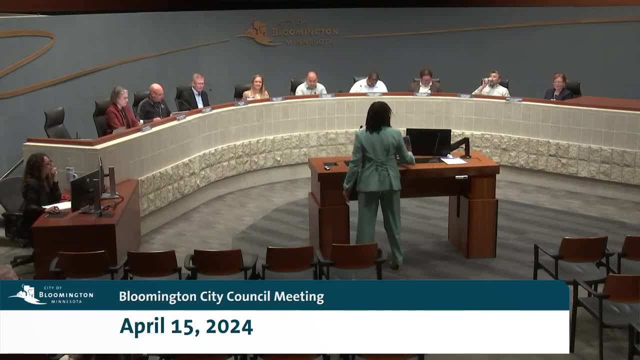 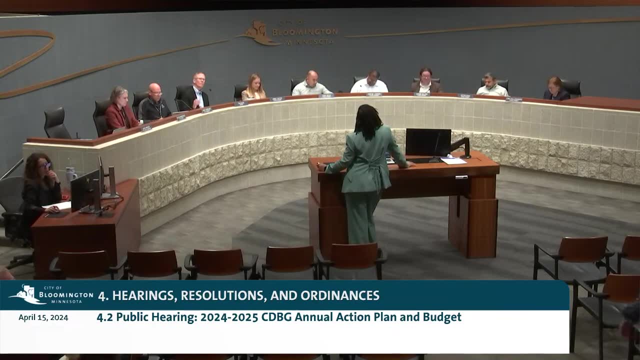 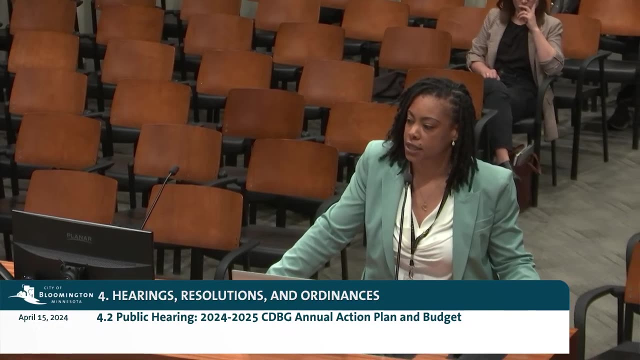 agenda is our first public hearing of the evening. this regarding the 2024-2025 community development block grant annual action plan and budget. mrs Coleman is back once again. yes, guess who's back? okay, so thank you. I will be presenting this evening around our Community Development block grant. 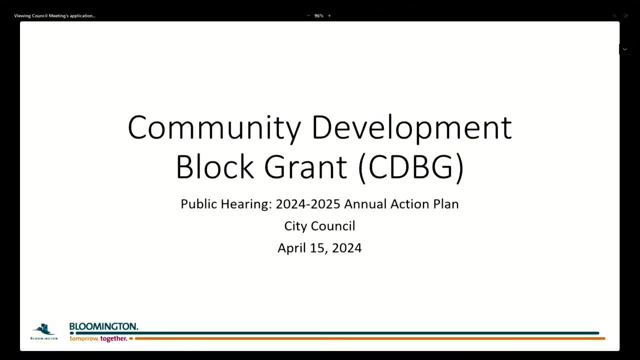 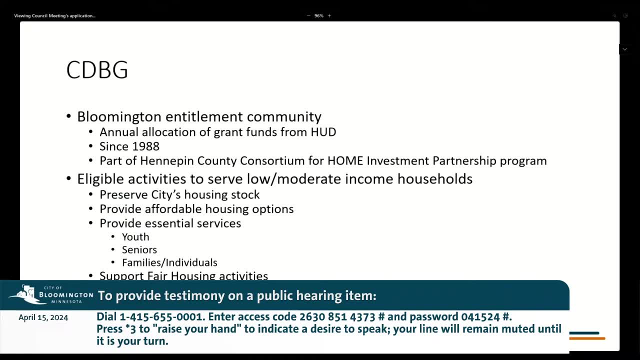 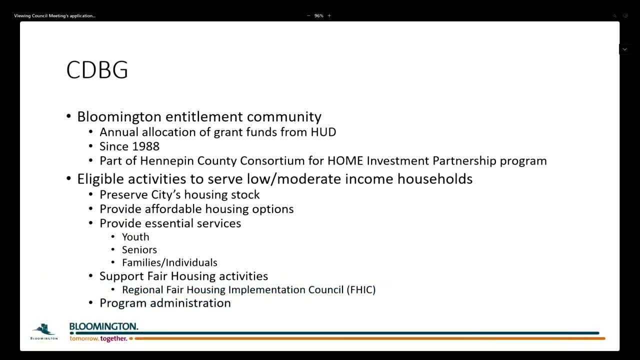 annual action plan and budget. this is the 2024- 2025 annual action plan. so what is community development block grant, CDBG as we more commonly call it? Bloomington isn't entitlement community. what that means is that we receive a a direct allocation of grant funds from HUD on an annual basis. We have been an entitlement. 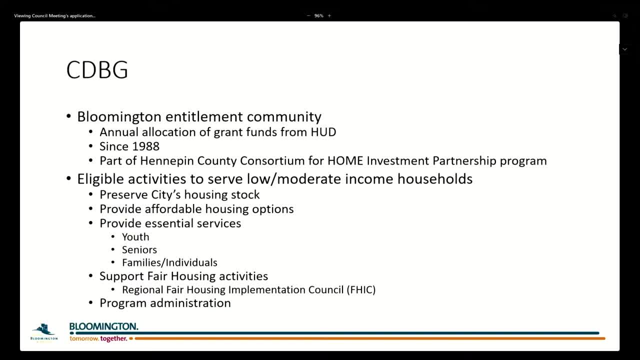 community since 1988, and we are a part of the Hennepin County Consortium for Home Investment Partnership Program. HOME is not an acronym, It does not stand for anything, It is just HOME. The eligible activities to serve low and moderate income households through using the CDBG funding. 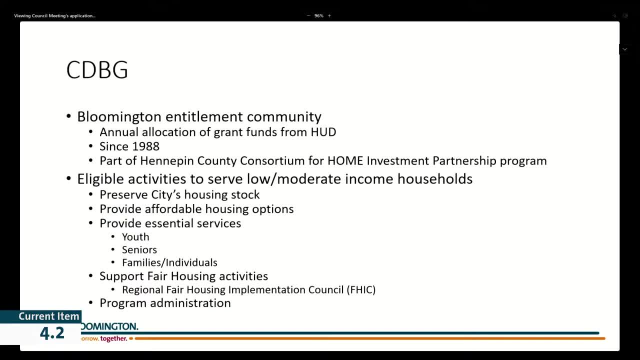 are to preserve the city's housing stock, to provide affordable housing options and to provide essential services, pinpointing specifically populations that consist of youth, seniors and families, as well as individuals. We also support fair housing activities. It's Fair Housing. 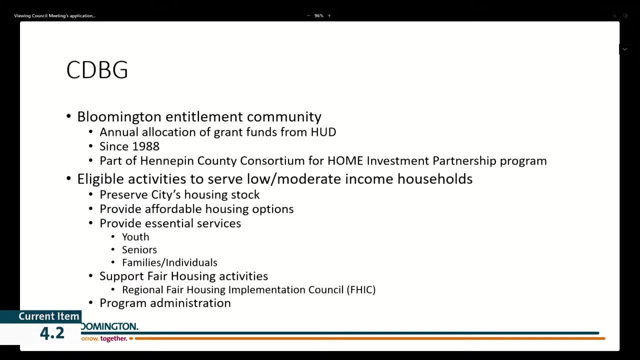 Month, And so we are a part of the Regional Fair Housing Implementation Council, better known as the FIC, and we do provide program administration with these dollars. So the timeline of action steps. We went to the HRA board on March 26,. 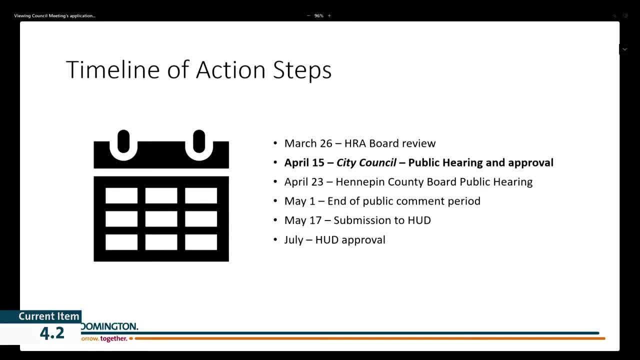 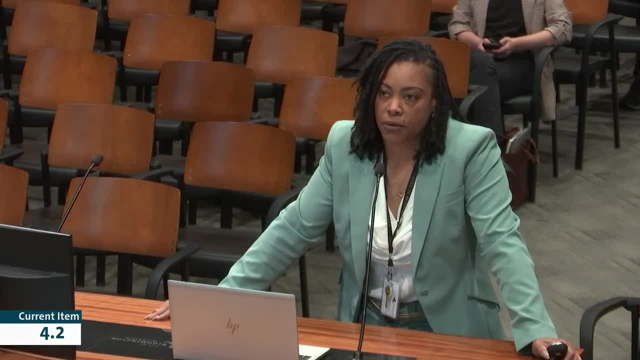 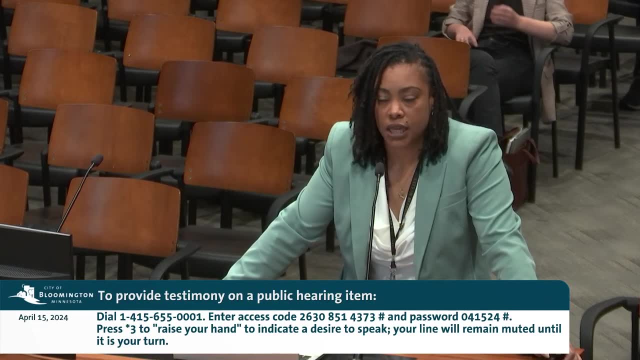 for review and recommendation of approval to the city council. We are here this evening for a public hearing. This is a public hearing that was noticed in the paper twice. And then the Hennepin County board hearing does take place on April 23rd. May 1st is the end of our public comment period. 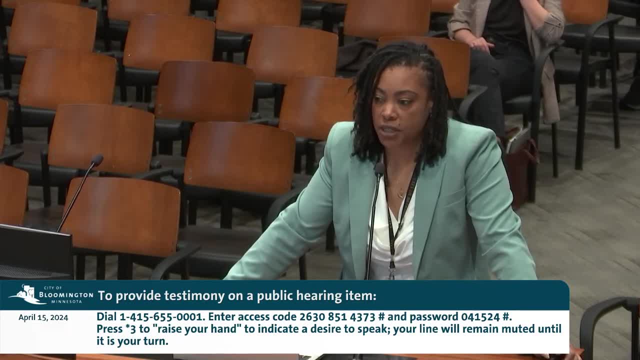 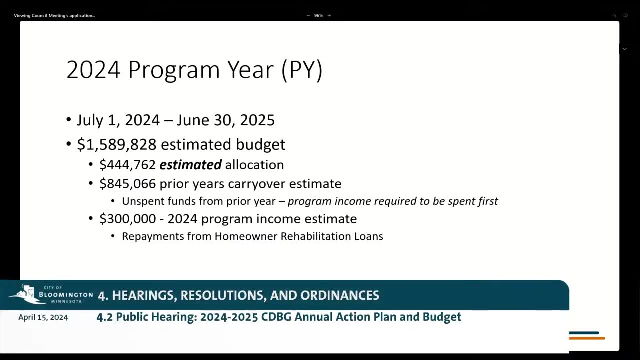 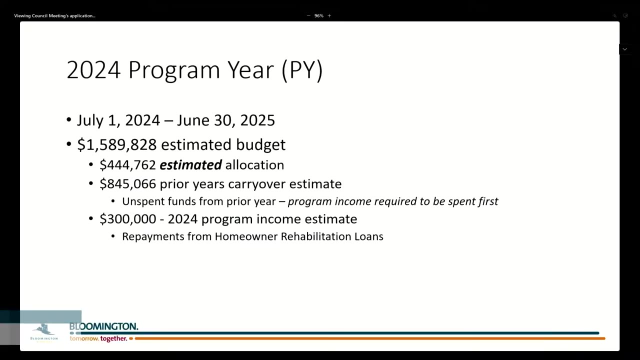 with a submission to HUD by May 17th and an expectation of HUD approval in July. So program year 2024.. So that's what PY stands for. First off, our budget year, our program year for CDBG, is July 1st 2024 to June 30th. 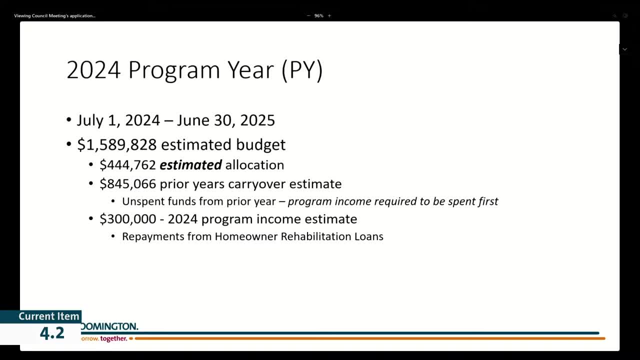 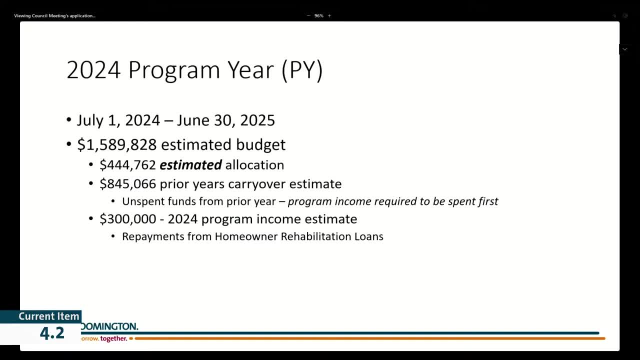 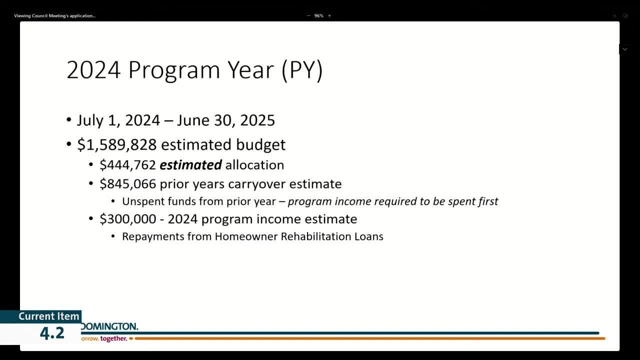 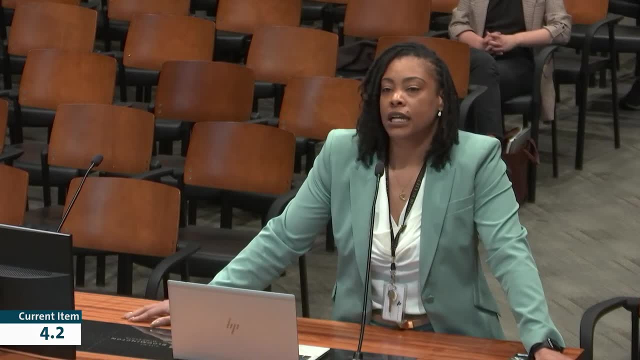 from the president, as well as the response he's getting back. Next, I have prior years carryover estimate of $845,066.. The reason for this being this amount, which is less than last year's carryover, is because of unspent funds from prior years. 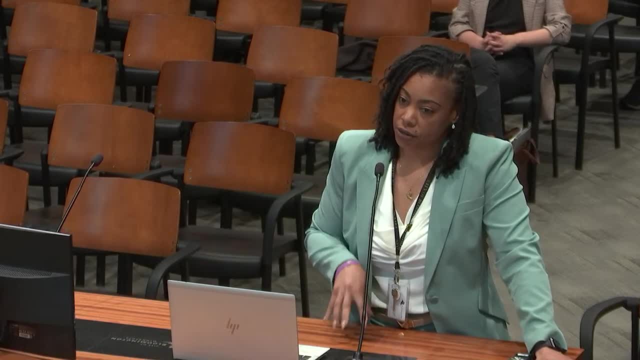 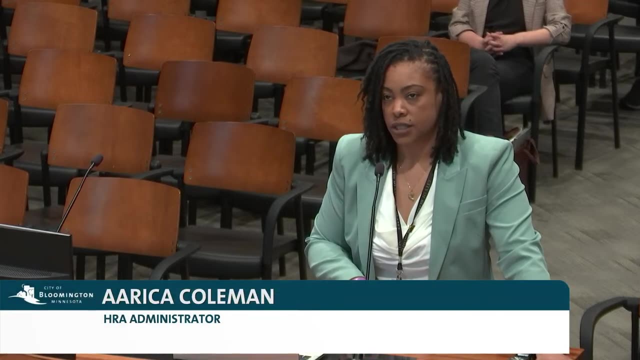 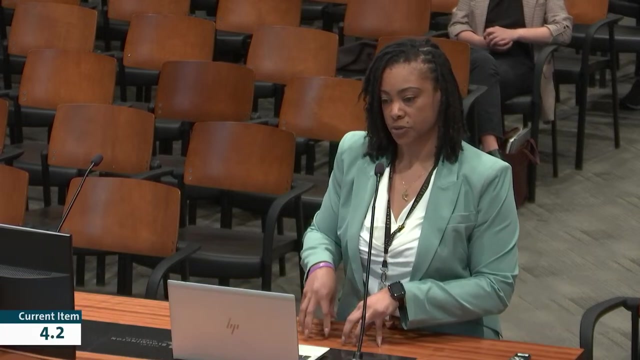 When we do this program for Community Development Block Grant or CDBG. one of our main programs, our largest program, is our Home Improvement Loan Program. This is the funding that we use for income-qualified eligible households to do eligible repairs, And we have to say eligible repairs because it is through the program. 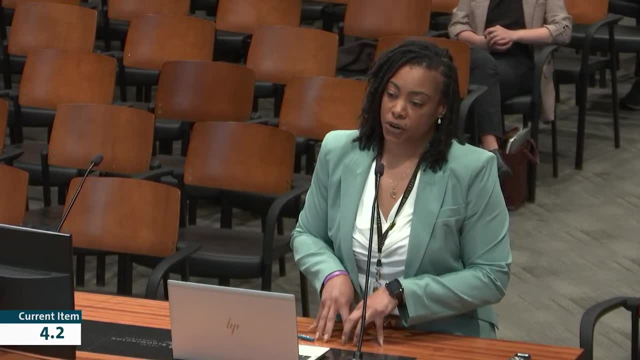 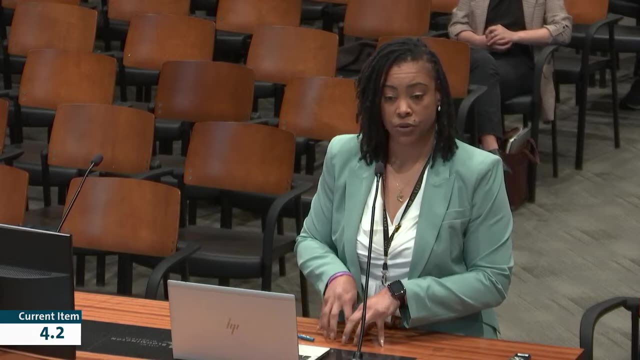 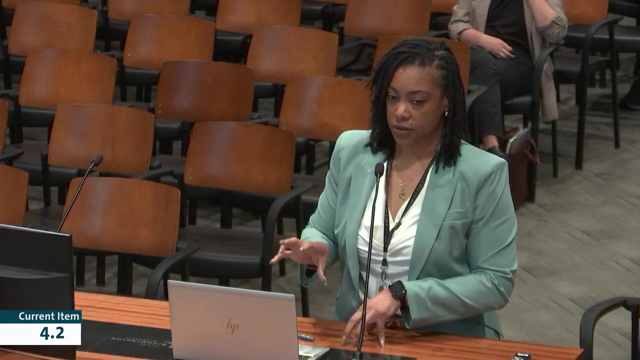 On their home, And then it is deferred. So the loan does not require any payments for 30 years. So it's deferred for 30 years And we do have 2% simple interest for the first 10 years. This program has been in operation for many, many, many years. What we have seen is beginning in 2020: record amounts of repayments. This aligns with the housing market. So what has happened? The problem is: from 2020 to 2022, we actually received quite a bit of money. It was well over a million dollars in repayments. 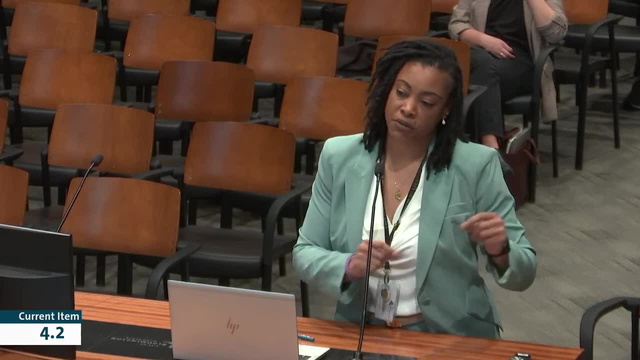 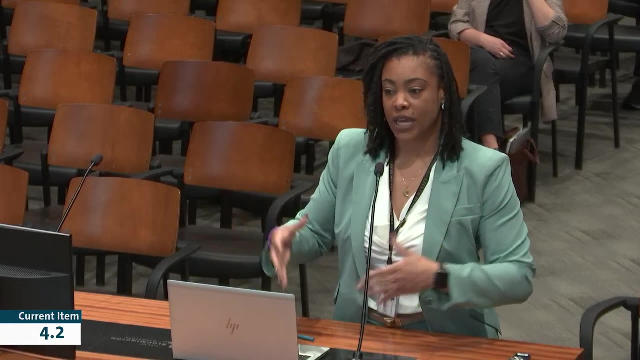 Because of that, program income is required to be spent first. So even though we may get an allocation of around $400,000, $450,000 a year, we cannot touch that money on the eligible activities until we spend all the program income. And if program income comes in while we're spending, we're going to have to spend all the program income, And if program income comes in while we're spending money, we have to go back and spend the program income first. Because of that and having to spend program income first, we have funding from years 2021 and 2022. 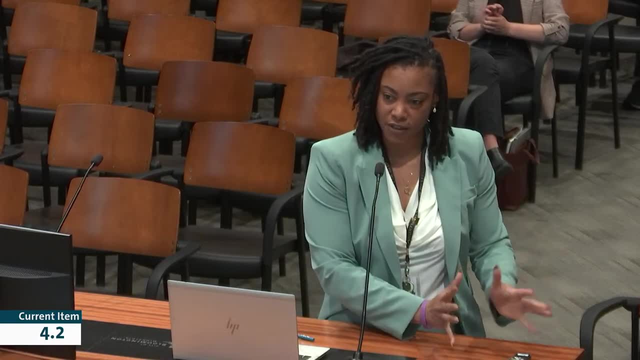 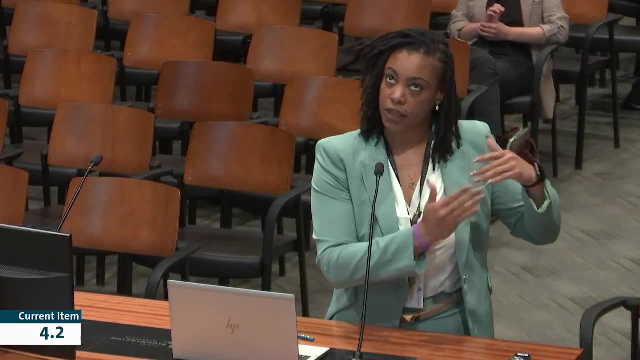 So also in that we have to spend the program income first, run through that, Then we have to go back to the latest year- the most, yeah, the latest year, not the most recent, the latest year- and spend that allocation before we can start touching the new allocation. 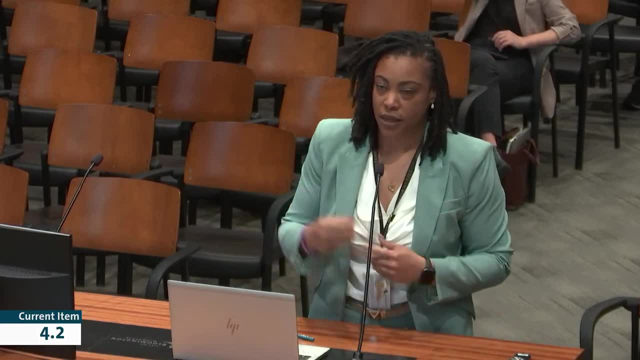 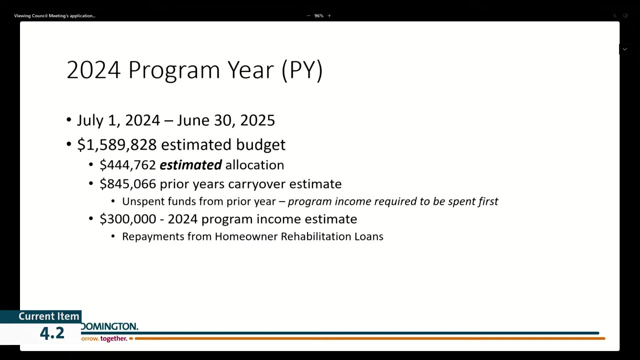 So when we do all of that, we get a larger number that we potentially carry over. I do want to highlight this is a carryover estimate because I'm still in the 2023 program year, which does not end until June 30th of this year. However, HUD requires that we turn this information in by May 17th. So with that, I'm estimating $300,000 of repayments. This is less than what I estimated For 2023, I estimated $400,000 of repayments and we have received about $340,000, $350,000 already. So kind of on the nose, just about. So I'm estimating it lower just because interest rates, if people aren't selling their houses, they may not be paying these loans back as soon as they were before, in 2020 to 2022. 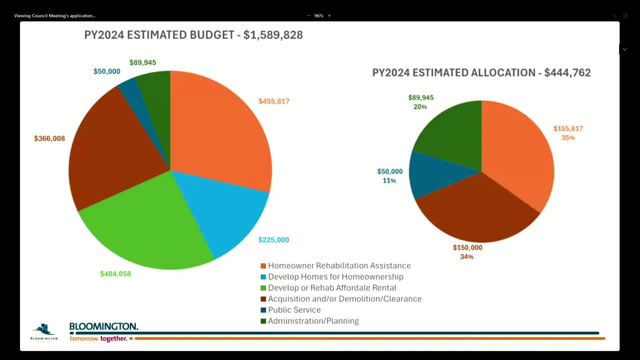 So now I have a pie chart just to describe pretty much what I just said. However, this breaks it down for the eligible activities, between what the estimated budget total is and then what the estimated allocation is. So let's look at the big pie chart. 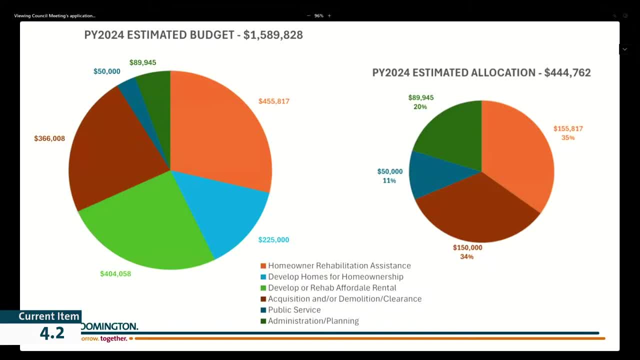 The big pie chart is showing that, through the estimated budget of $1,589,828, it is being broken up to support homeowner rehabilitation assistance, developing homes for homeownership. This is our partnership with HUD. This is our partnership with West Hennepin Affordable Housing Land Trust, better known as Homes Within Reach, where they buy and rehab at least two homes a year. 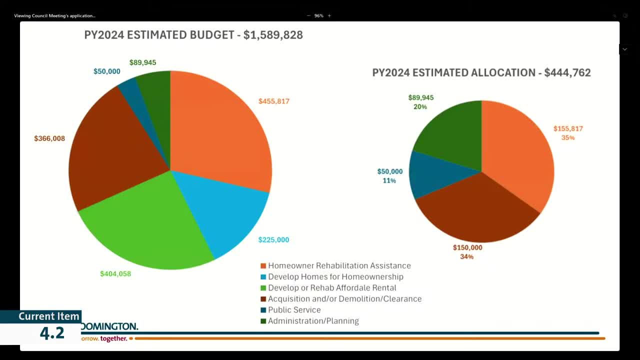 But in the last few years they've been doing three homes a year. So it's $75,000 per home in Bloomington. Develop or rehab affordable rental. That is the green, the light green color Acquisition and or demolition and clearance. 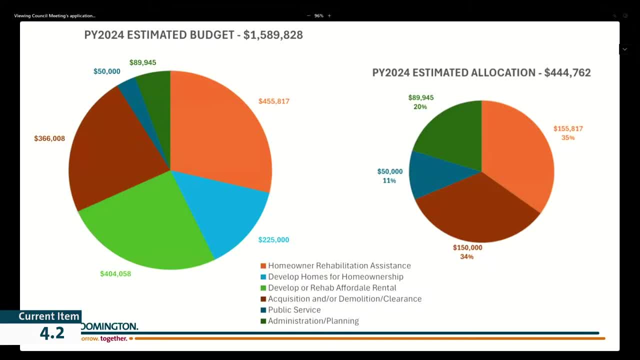 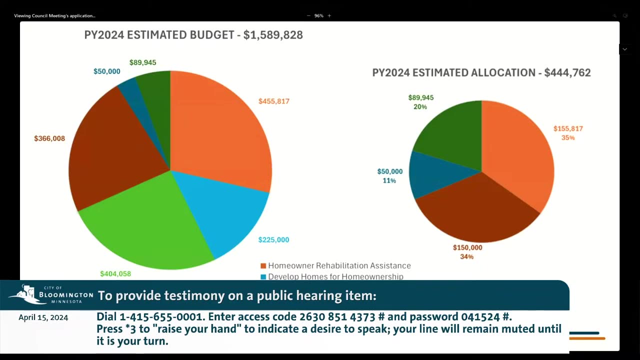 Public service, which is where we are getting at supporting our seniors and our youth In particular, And then administration and planning. This goes towards some of the admin planning that we do in this process here, but also some of the staff that work on it, and then the other fees that are aligned with it. 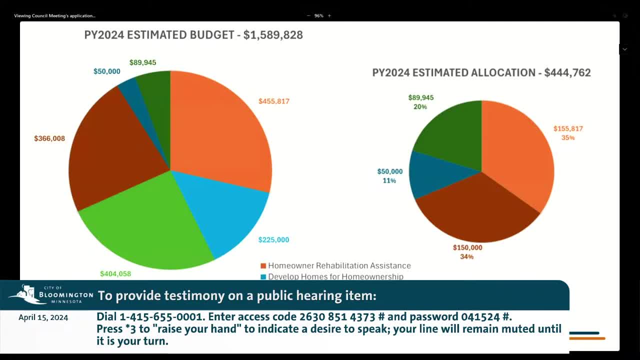 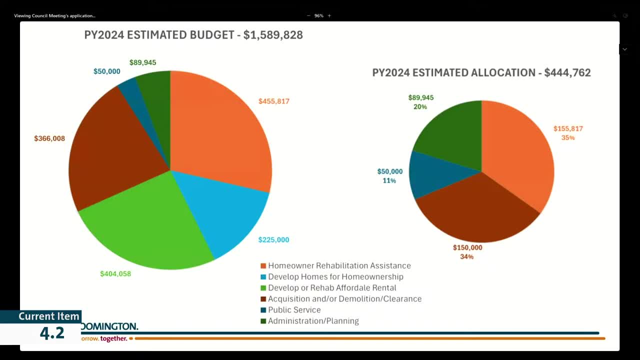 Now, when we look at the smaller pie chart, which is an estimated allocation, so that's what I would estimate we're receiving from HUD for program year 2024, of $444,762.. If you notice there are- There are a couple of colors missing, because I'm not recommending that we add additional funding from the allocation. 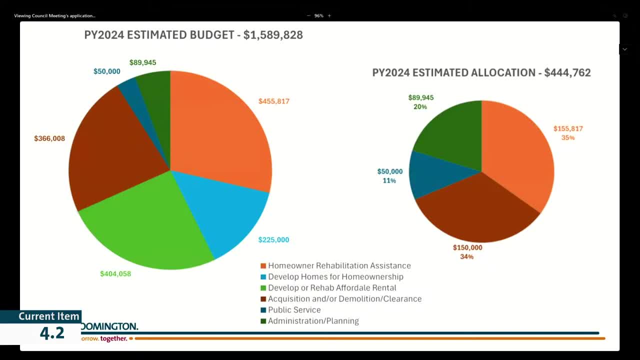 And so the first one, the green, which is $89,945, and it's 20%. The reason the percentages are in there is because for the 20% is our max we can spend on administration and planning, So we cannot go over. 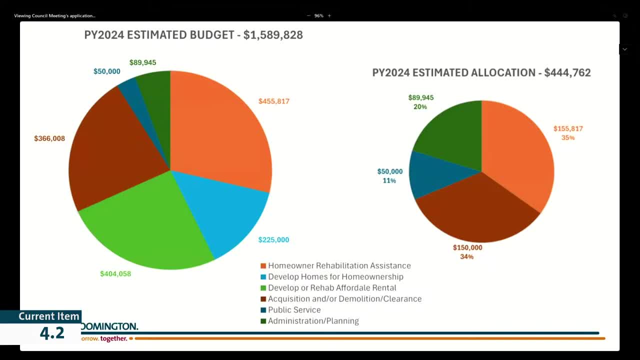 20% of our allocation and our program income And when I do this budget and present it to you, I do not estimate admin based on program income because we could just get in trouble trying to estimate that, So I only estimate it on the allocation. 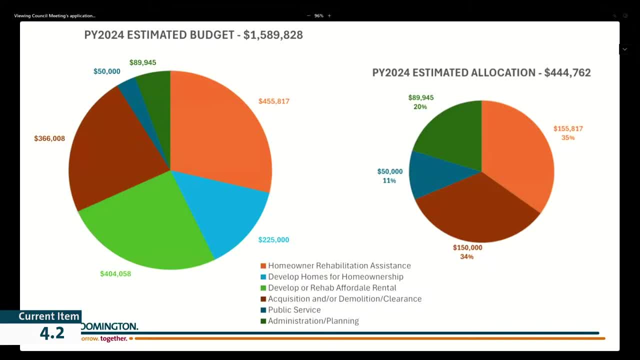 Next, the $50,000 at 11%- excuse me- is for the public service, Then at $150,000, the 34% is for acquisition and or demolition and clearance. Where this has really shown up- and this was something that you approved in an amendment- was the ability for using these funds to purchase properties that are dilapidated and need to be torn down so that we can remove that and allow for greater opportunities for new affordable housing- usually homeownership, because we're usually doing single family homes. And then the last one at $155,817,, which is $35,000.. And then the last one at $155,817,, which is $35,000.. Is the homeowner rehab assistance. Yes, that sounds small, but I just said we're carrying over funds from prior years and program income and so that funding is going towards the rehab loan program. 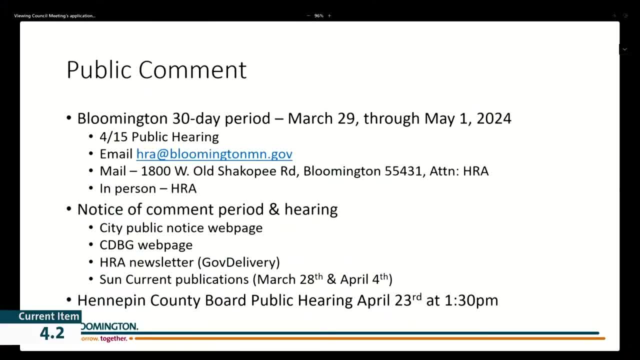 So where are we? We have a public comment period. It is a Bloomington's 30-day period, which is March 29th through May 1st. We are here this evening for a public hearing which we can take any comments that anybody wants to provide. 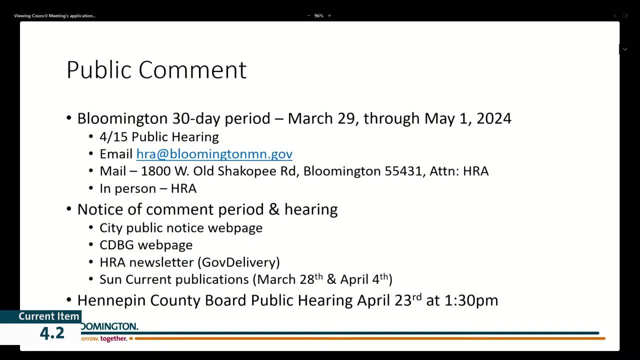 They can also email or mail them, or they can stop by the HRA and provide their comments. The notice of the public comment period and the hearing went out on the City Public Notice webpage, the CDBG webpage, the HRA newsletter and the Sun. Current publications, both in the March 28th and April 4th publications. 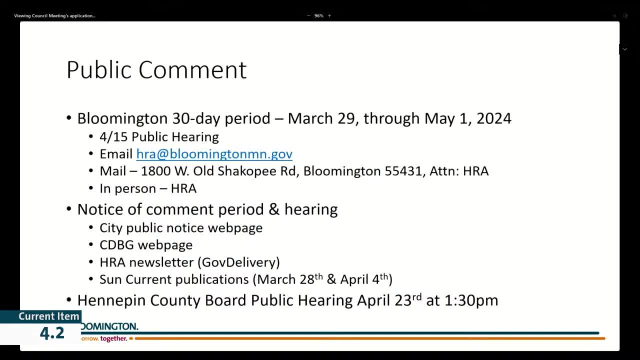 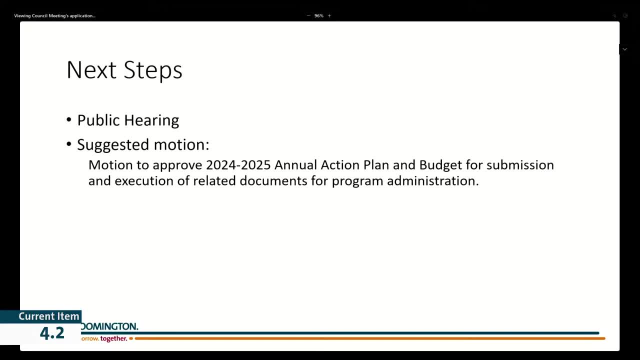 The Hennepin County Board public hearing will be held on April 23rd at 1.30 pm. Next steps: I would ask that you ask any questions. If you have any questions that you have of me, open and hold the public hearing and then consider the suggested motion. 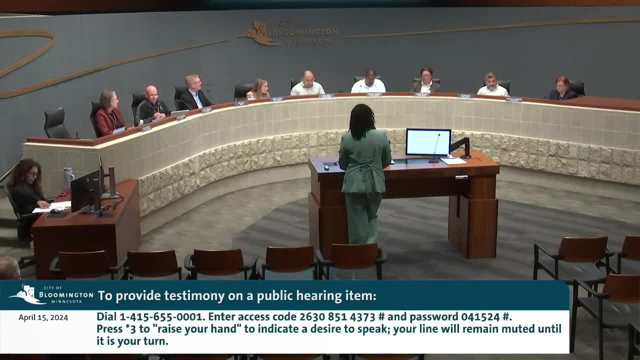 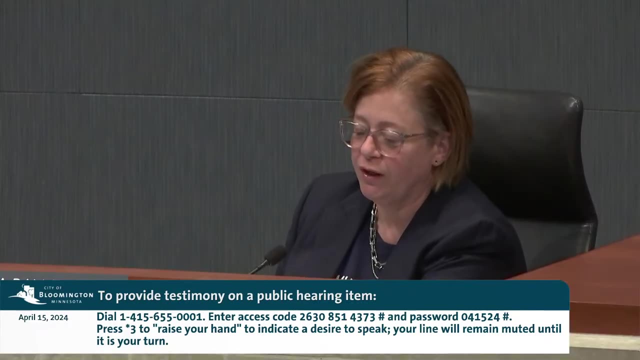 Thank you, Council questions on this. No questions, All right, Oh, Council Member D'Alessandro does have one. It's probably not related explicitly to the budget, but just a question for us here. Thank you, Mr Mayor. by the way, 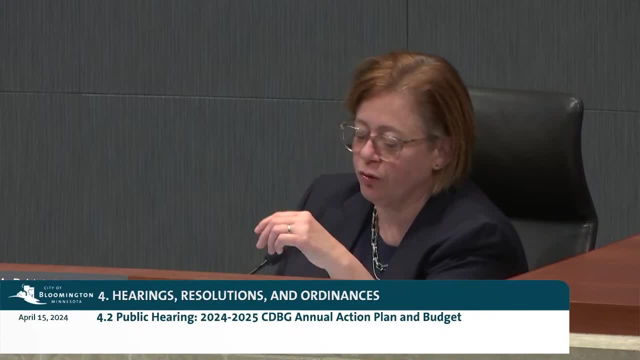 I noticed that we- I appreciate that you're doing your administration calculation against allocation as opposed to potential budget. That's prudent and I appreciate the fiduciary responsibility associated with that. I'm just kind of curious: are there costs that we should be considering covering on an administrative level to kind of get in front of some of those potential investments? 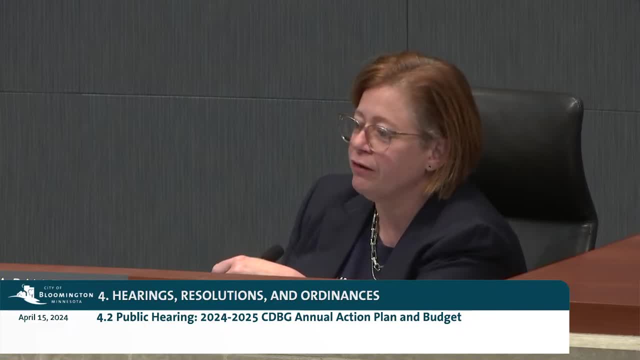 And what I mean by that is, you know, is there a development aspect to the work that is more. I don't want to use the word risky, I don't mean it that way, but more prospective right, More prospecting oriented about, you know, finding those dilapidated homes, for example, and potentially, you know, managing them. 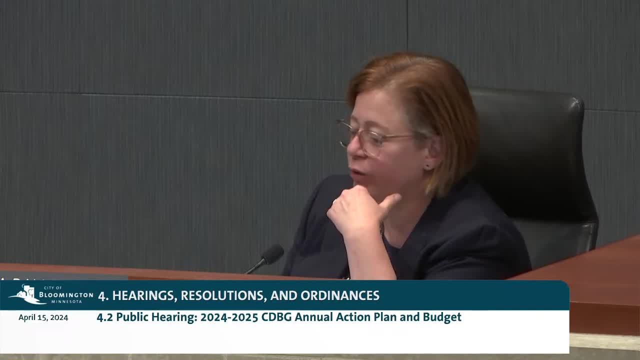 Or business development associated with, you know, additional grants or other things like that That that Would allow us to, over time, impact this particular grant program. you know this particular block program. I'm just curious if that might be prudent for us to be considering an investment in that space as opposed to just like: okay, we're budgeting, we're planning to have the enough administration to manage the plan as we can guarantee it. 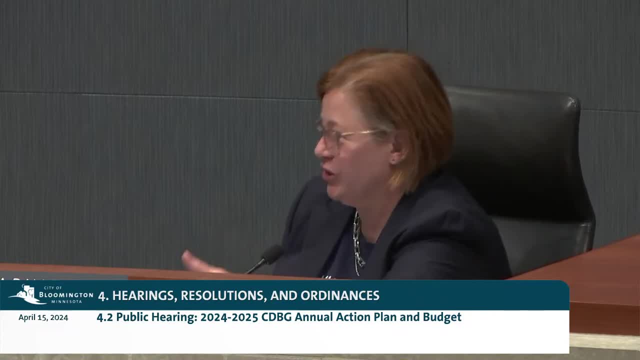 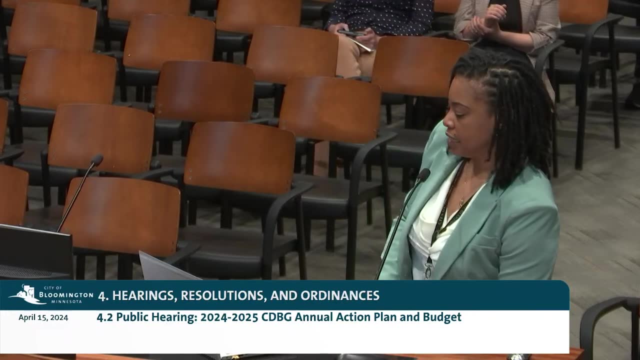 But we're not really planning ahead to say what if it grows. How are we managing that? That's more or less my question. Yeah, Thanks, Thank you, Mayor and Council Member Alessandro. members of the Council. So how do I want to put this? 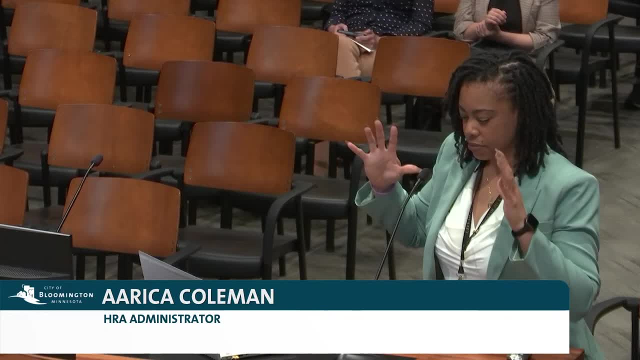 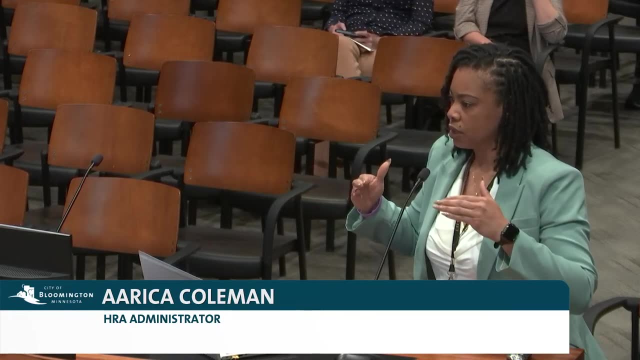 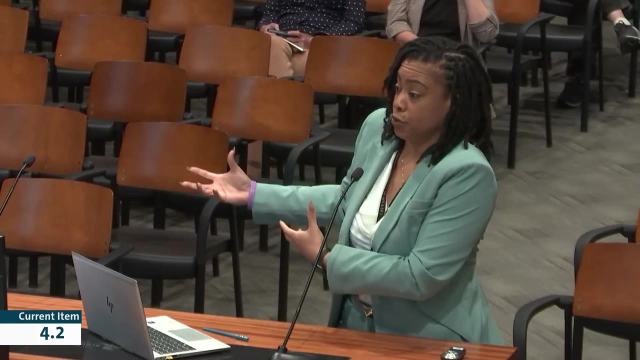 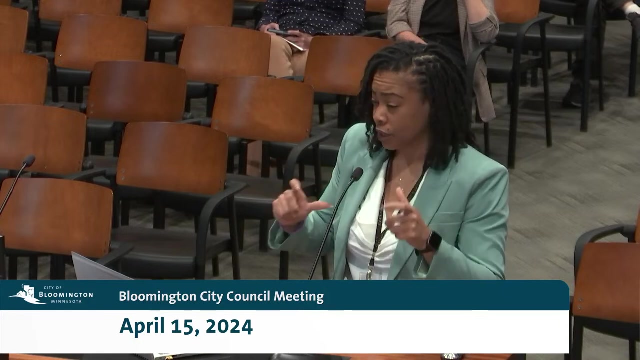 One. we are estimating that admin and planning based on the allocation, but that's not like covering a staff person, So what that is doing is like the posting. That's covered through admin and planning. There are other things that we do in terms of legal services or accounting. 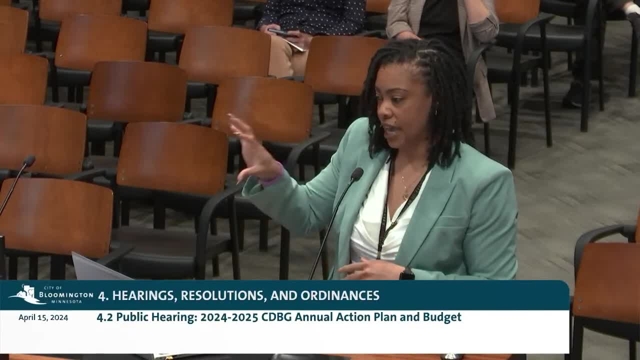 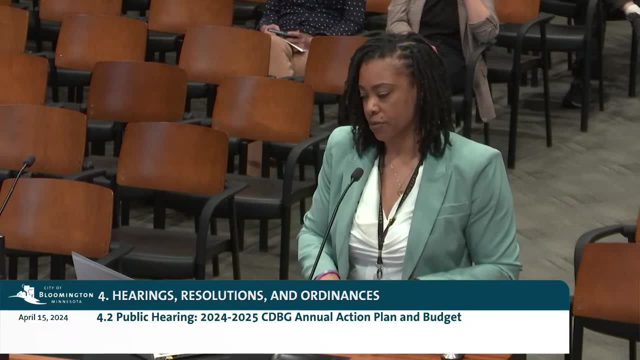 We're doing different things like that, where we are able to do that. That's just the admin and planning piece. The second part is that we are coming up on our five-year plan. We're five-year plans all over the place at this point, right. 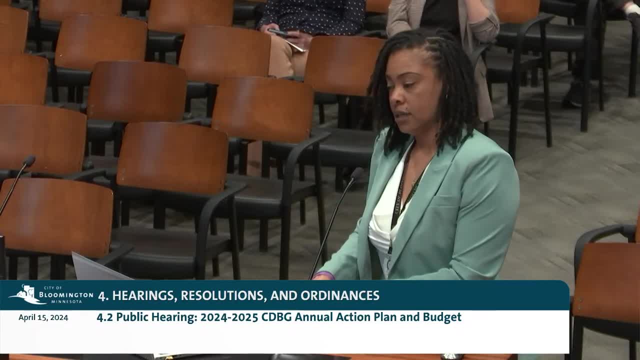 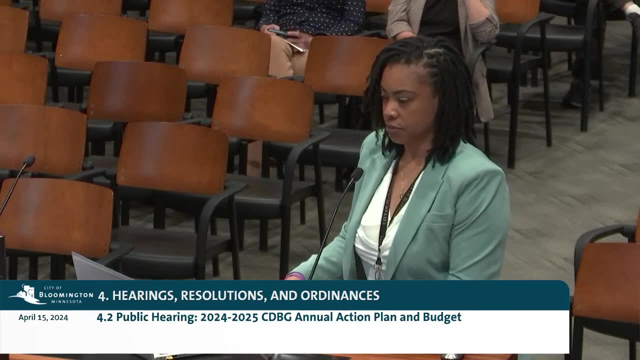 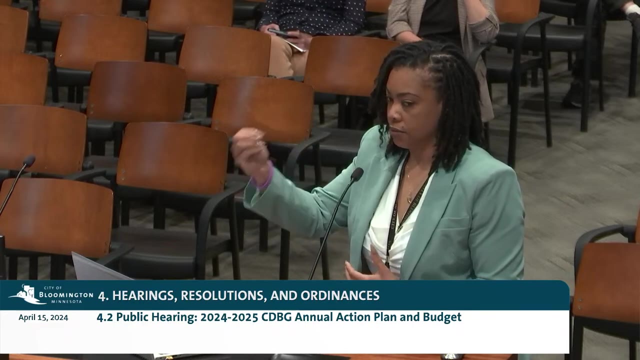 So the five-year consolidated plan is actually a requirement by HUD And in that consolidated plan is where you list all the different goals and priorities. So in our current consolidated plan we do have things for Economic development and businesses and things like that. 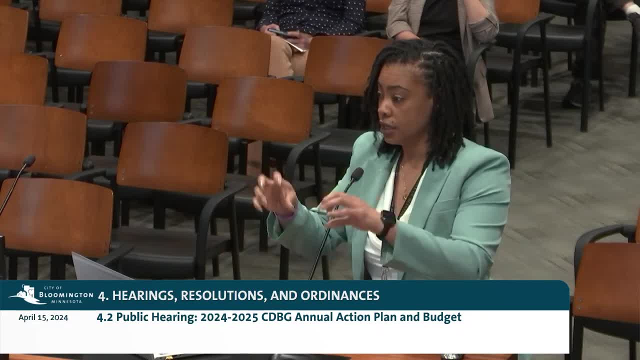 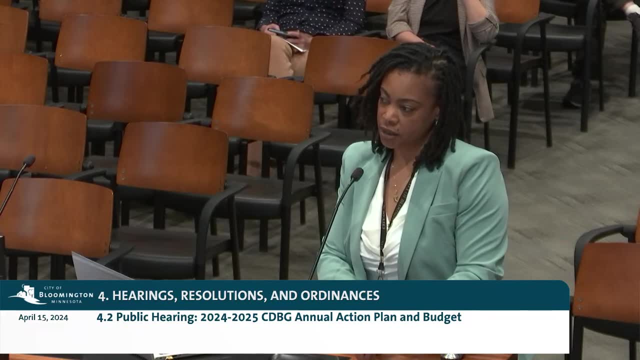 So those things, still they're eligible and can be used in the CDBG program. We need to make sure that we are ready to roll that out when we put it in our annual action plan, because we have to draw, have those activities done. 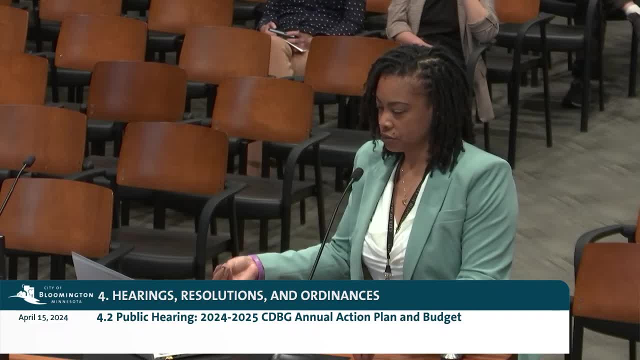 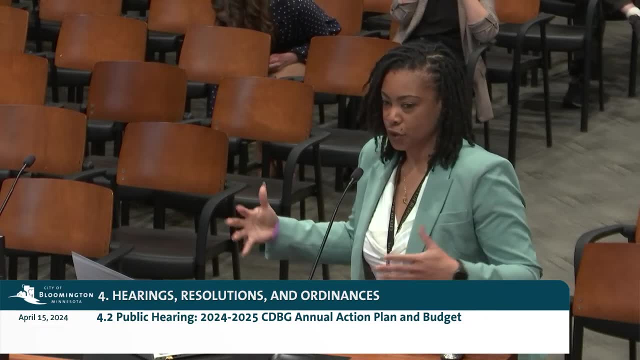 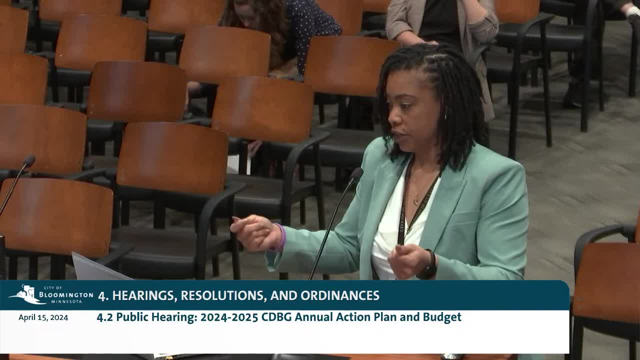 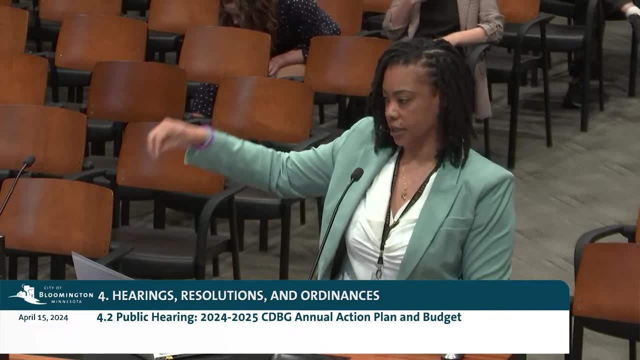 So we don't even have a full 12 months to roll out on spending the funding and they want to see it out the door very quickly. so there's that. so i want to say this: that's in the current consolidated plan and it will be in the next consolidated plan. 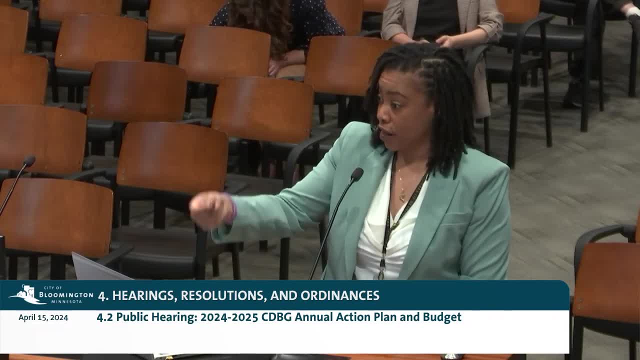 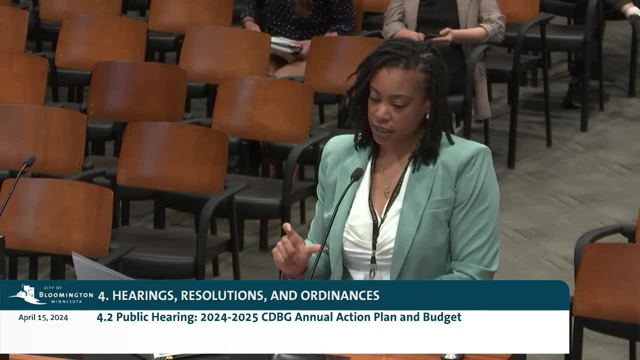 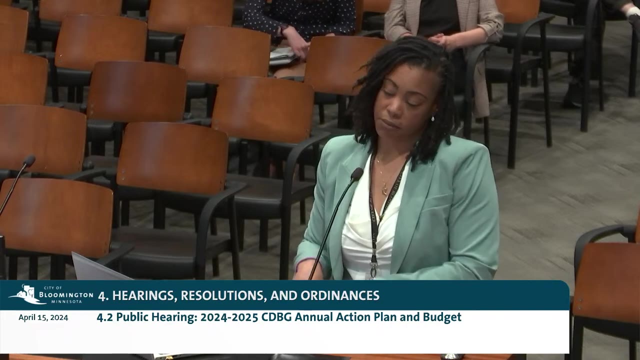 because it's already been identified and discussed, as it aligns with the priorities of the city of bloomington in terms of economic development. lastly, when you talk about development, we can do it. there's nothing against us doing it in terms of buying something and maybe. 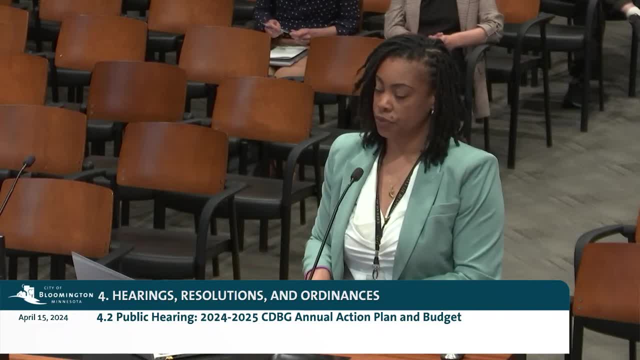 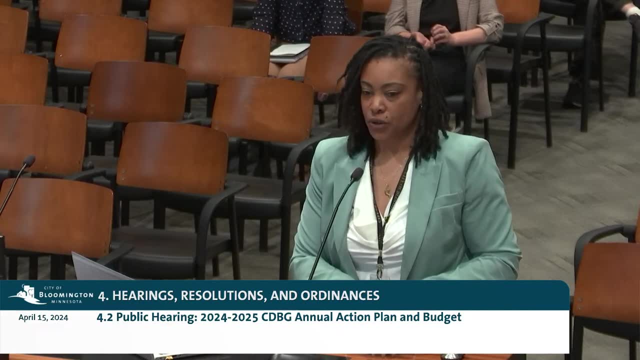 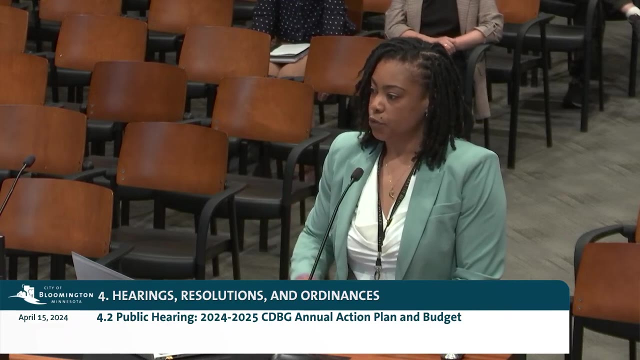 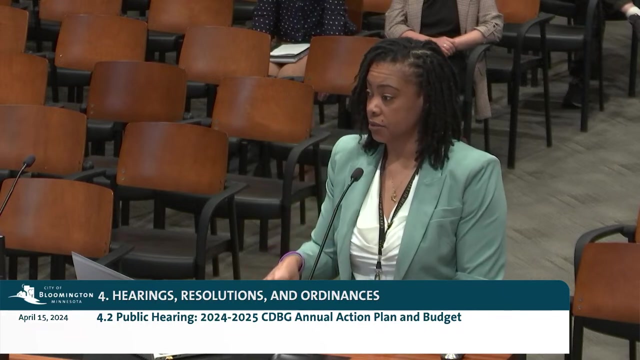 maintaining it or holding on to it with cdbg. however, any funding that comes in for that property is program income. so, for instance, the hra has the rental homes for future home buyers properties. if we buy a property with cdbg, all the rent minus expenses has to come back into cdbg. so we have to be very careful on how we're doing that. if if we're looking 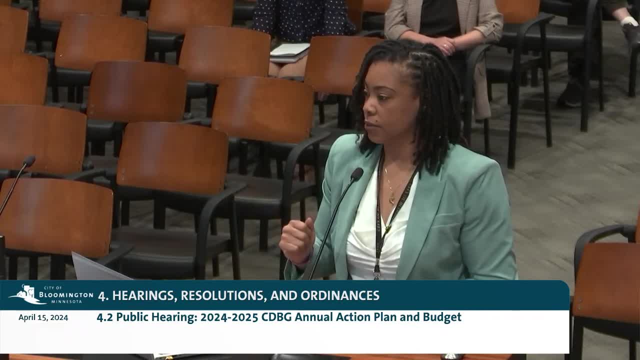 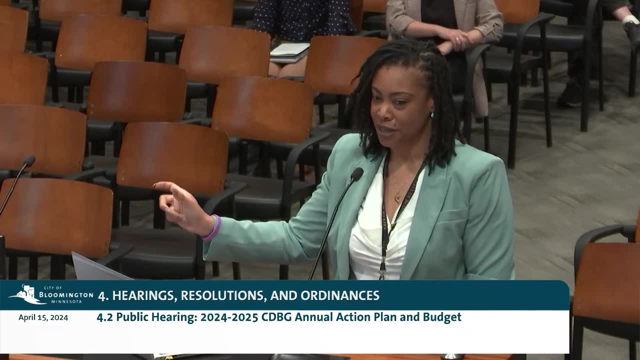 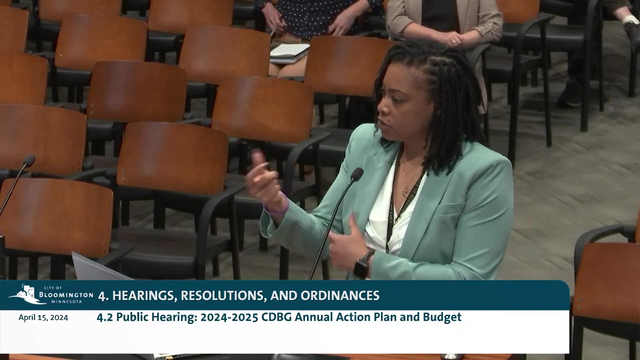 to operate that program a little bit differently. so one of the things about that program is a portion of the rent paid is escrowed towards that participant to be able to purchase a home right anywhere in the country. well, we don't want that to be program income, so we have to be just a. 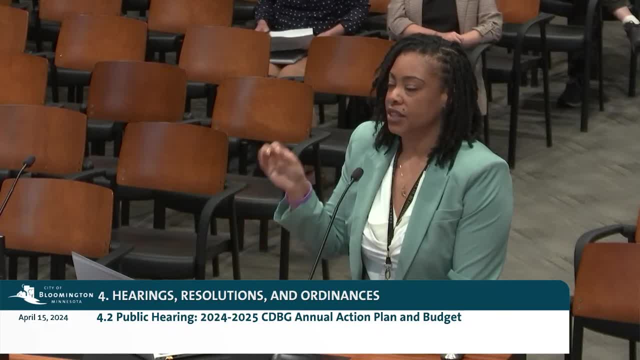 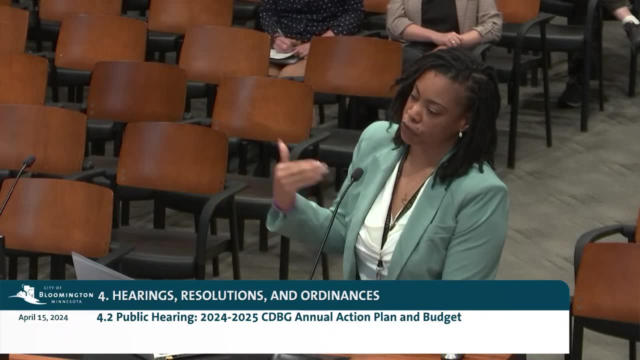 little bit more strategic on how we use the funding. and then the very last thing that we have to be a little bit more strategic on how we use the funding is is there is, um, something called section 108, which is the ability to borrow against your future allocations for economic development and or housing activities. this council has previously 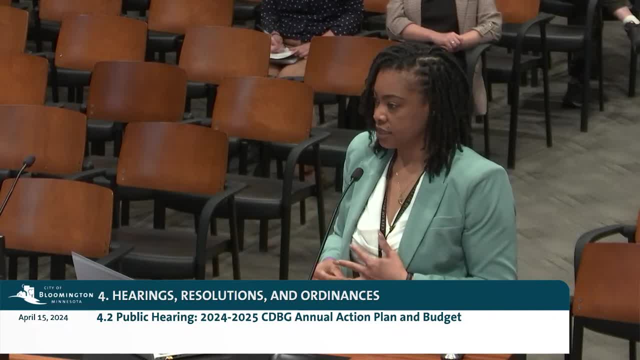 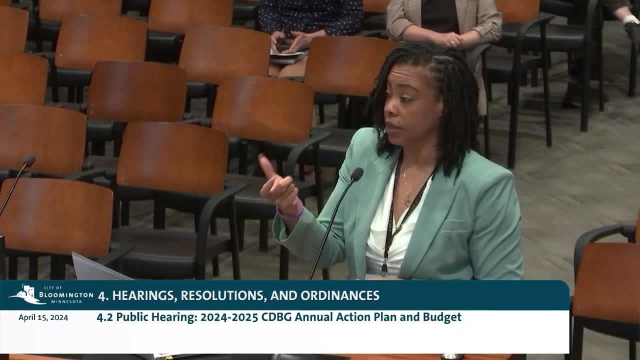 approved, uh, doing that and going through that process, and then it was submitted to hud, but then there were changes and we haven't come back because we haven't- we don't have a, a development or a project just yet to bring back into that. so i just want to highlight that, yes, we can do the 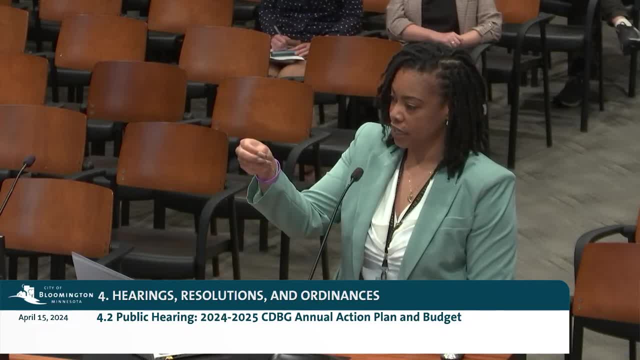 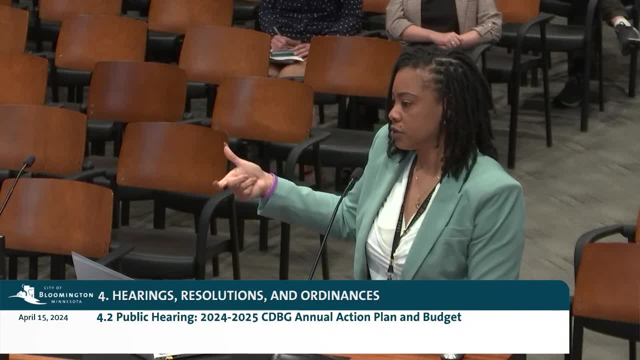 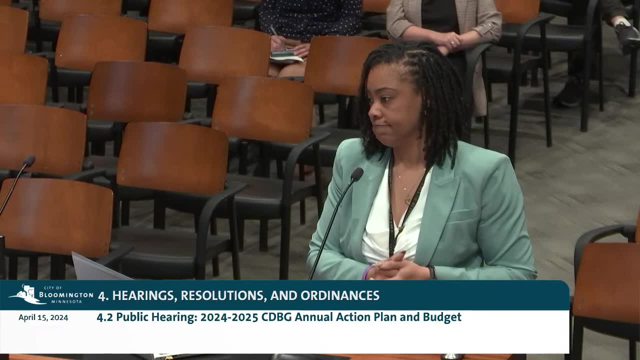 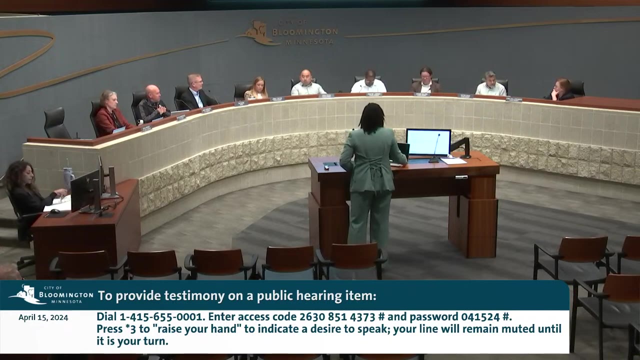 and what is the best use, whether it is using hra dollars, which sometimes we like to use hra dollars instead of using the federal funding, that may have more strings attached. right, that makes sense. thanks, appreciate it. thank you for that answer, council. no questions. if not, uh, this is a public hearing. 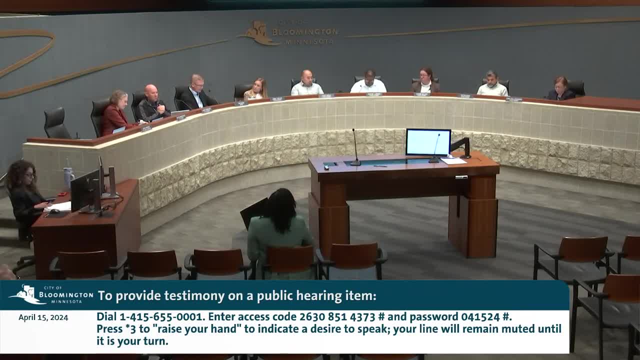 and right now i will open the public hearing on item 4.2. public hearing regarding the 2024- 2025 cdbg annual action plan and budget. is there anyone in the council chambers wishing to speak to item 4.2 this evening? safad, we have anyone on the phone wishing to speak. 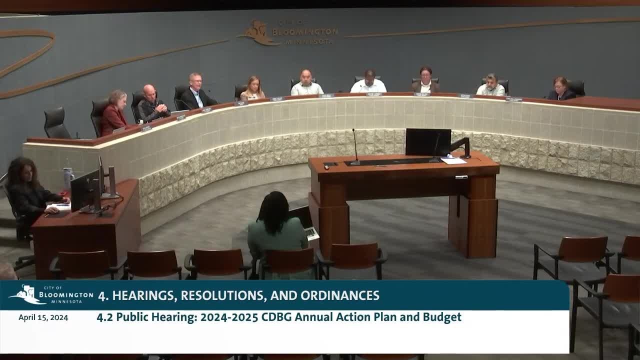 last call for anybody in the council chambers, council, with uh, no one on the phone and no one in the council chambers wishing to speak on item 4.2, i would look for a motion to close the public hearing on it. 4.2 so moved. second motion by council member lowman. second by council member mua, to close. 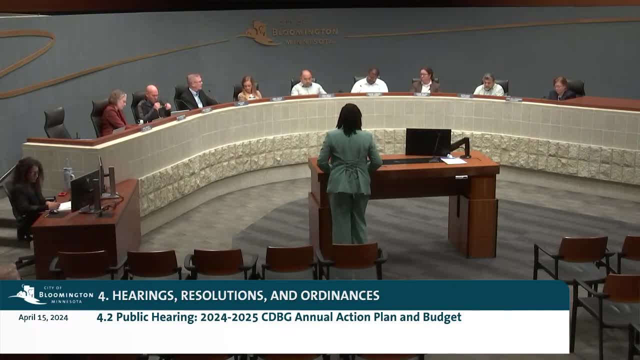 the public hearing on item 4.2: no further council discussion on this. all those in favor, please signify by saying aye, aye, opposed motion carries 7-0. to close the public hearing. uh. council discussion on this or action on this. council member mua. i'd be happy to do that, mayor, please. 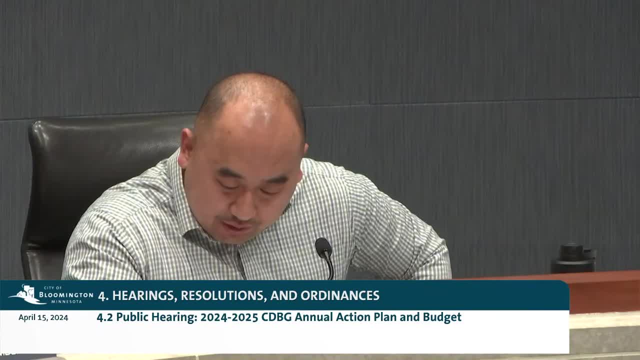 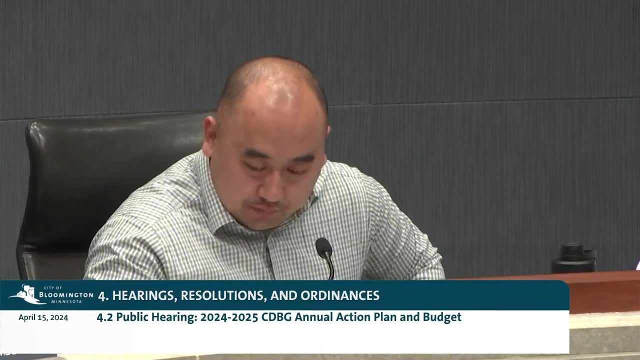 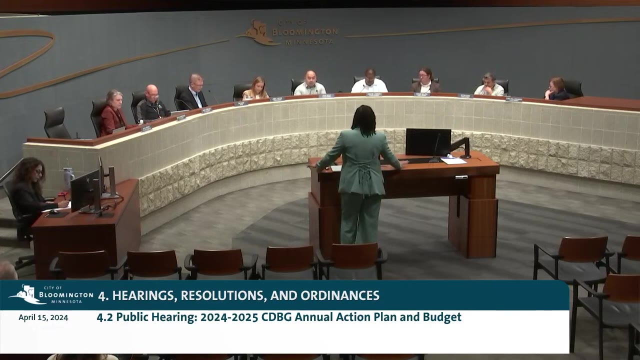 um. i would move to approve the 2024-2025 cdbg annual action plan and budget for submission and execution of related documents for program administration. second motion by council member mua, second by council member carter, to approve the 2024-25 cdbg annual action plan and budget. 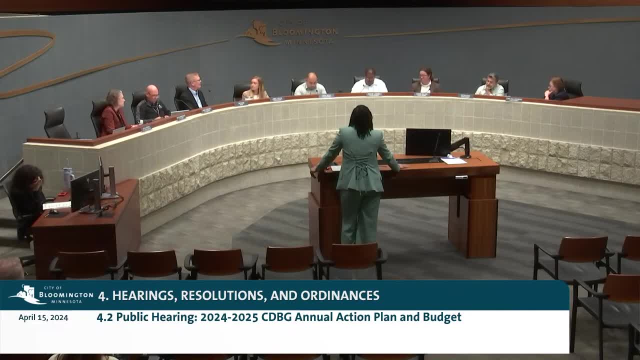 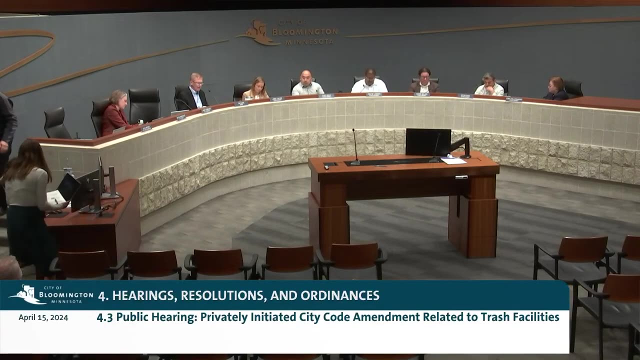 for submission and execution: no further council discussion on this. all those in favor please signify by saying aye, aye. opposed motion carries 7-0. thank you very much, thanks. moving on to item 4.3 on our agenda, this is a privately initiated city code amendment. 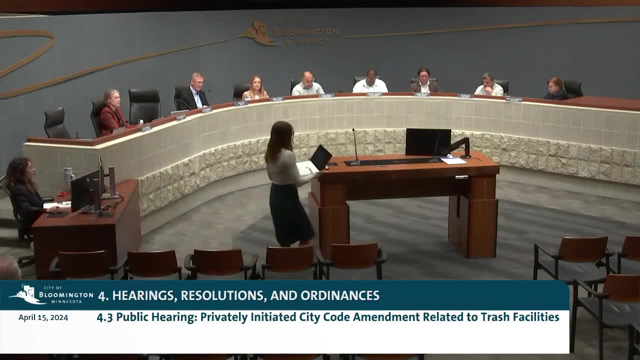 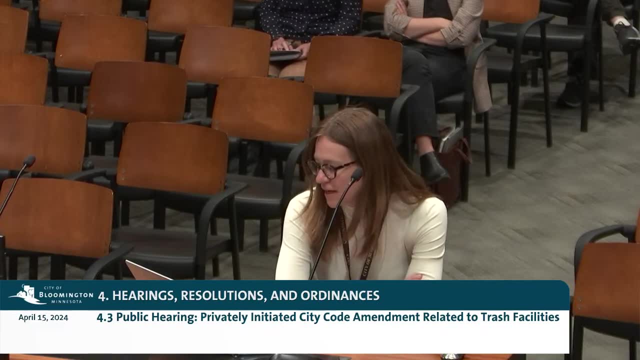 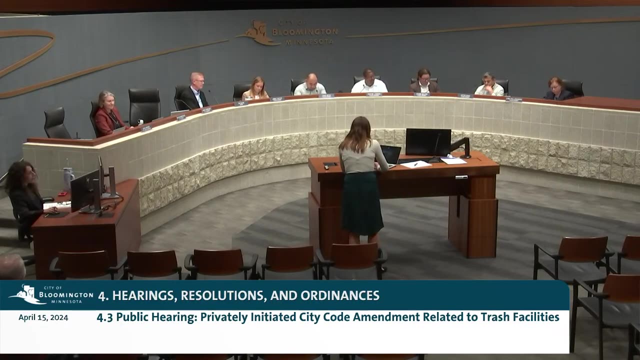 regarding two trash facilities and lizodee. lizodee from our planning department is here. thank you, good evening and welcome, mr. mr, can you promote me to panelists? i'm on the webex. thank you, yeah, i'm under attendees. thank you all. right, there we go. thank you. 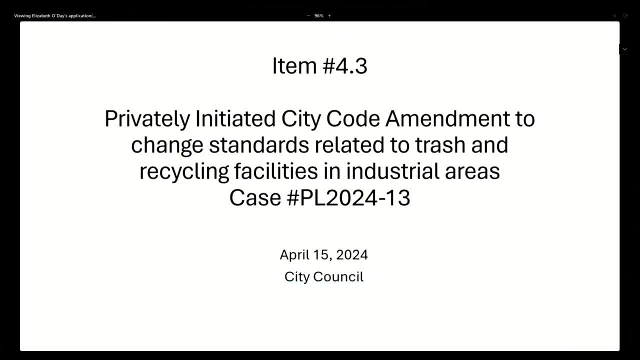 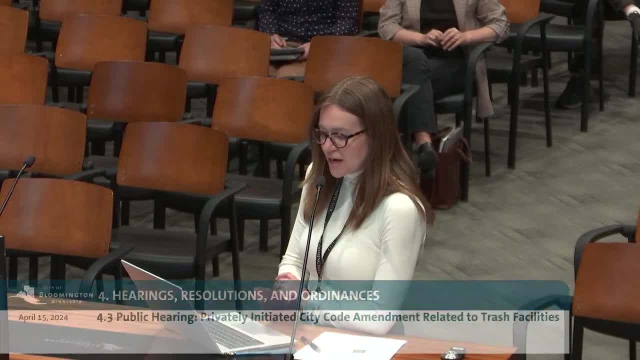 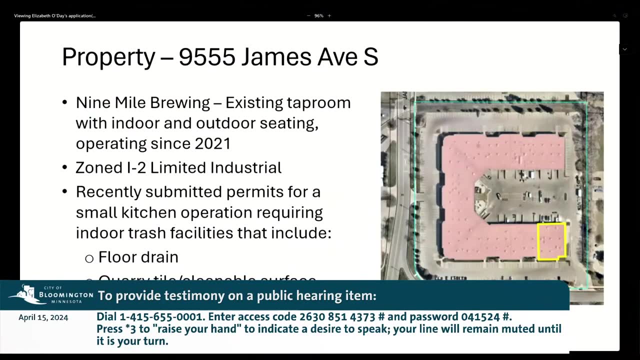 all right. thank you, mayor and council. item 3 on the agenda this evening is for a privately initiated city code amendment related to our trash and recycling facilities in chapter 21 of the city code. So this is a privately initiated city code amendment and the applicant is nine mile brewing company. 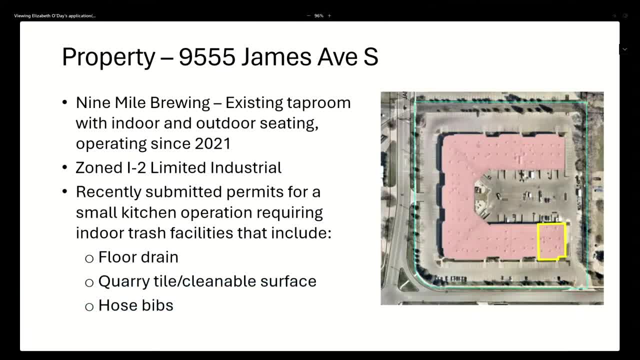 They are an existing tap room with indoor and outdoor seating. They've been operating since 2021 and they operate at 95- 55 James Avenue South, which is an industrial zoned Office warehouse building and not too far from here, and their tenant space is outlined in yellow on the screen. 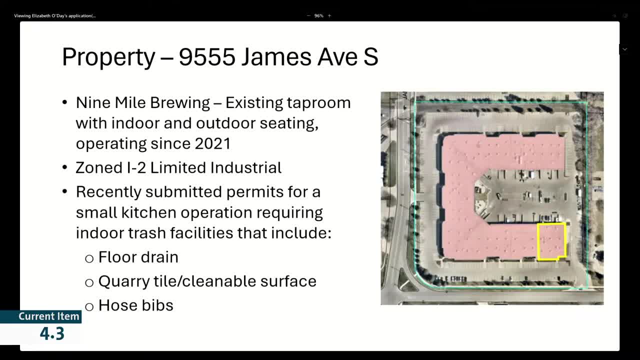 Recently they submitted a building permit to expand Or operate a small kitchen operation in-house, and so that triggers Something in our city code for indoor trash facilities, including Design standards such as floor drain, quarry, quarry tile, cleanable surface and hose bibs, and that's specifically for 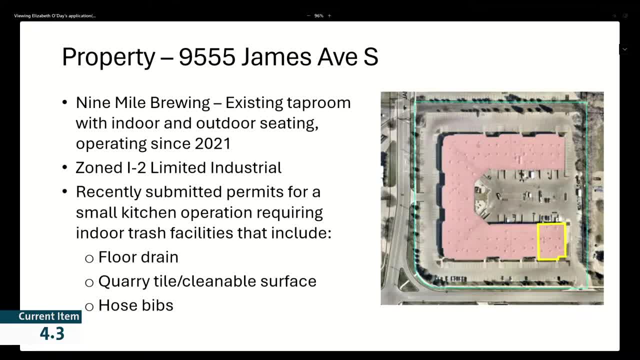 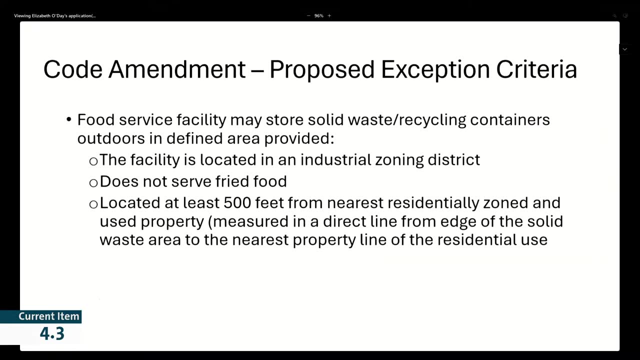 food related Uses in our city code, and so their option was either to provide a code complying trash room with these design standards or Amend the city code, and that's why they're here this evening. So they put forward this city code amendment for food service facilities That have to meet some criteria, and so these food services facilities have to be. 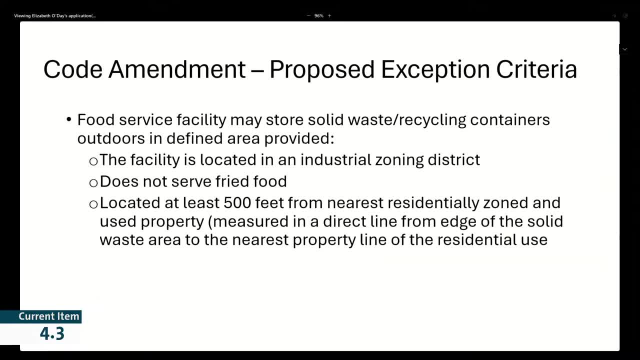 Can store their solid waste containers outside, Provided that the facility is in an industrial zoning district. The facility does not have fried food and it's located at least 500 feet away from nearest residentially zoned and used property. So if those standards are met, then they have to meet. 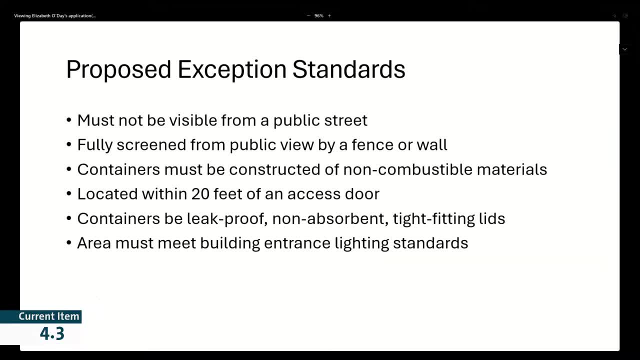 some additional standards, performance related standards. so the area has to be not visible from a public street, fully screened by a Fence or wall. containers have to be constructed of non combustible materials, Located within 20 feet of an access door. that gets at kind of the security aspect. 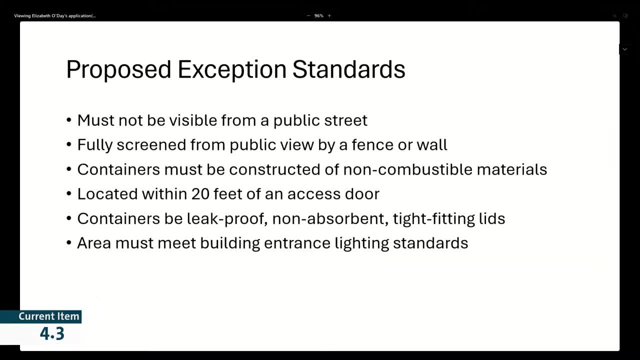 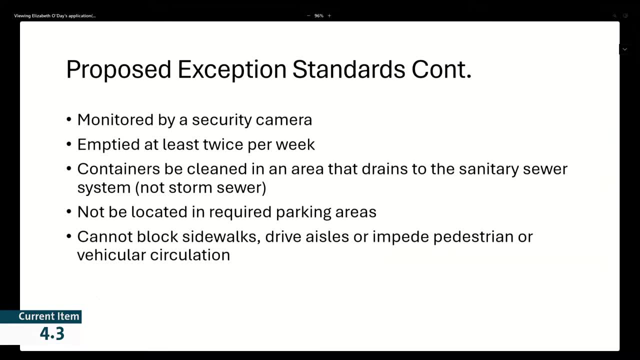 Containers must be leak proof, non-absorbent, tight-fitting lids and then must meet building entrance lighting standards. that also gets at security And then continued monitored by a security camera. empty at least twice a week And then must be cleaned in an airtight Area that drains to the sanitary sewer. 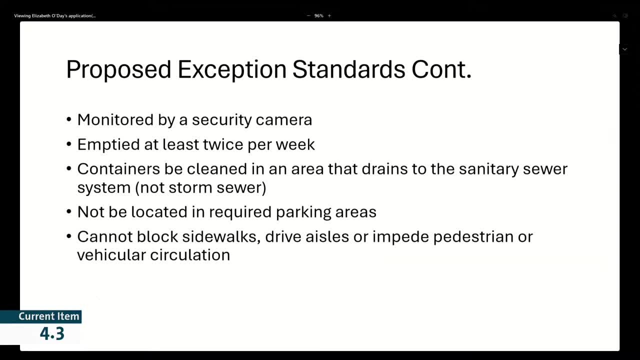 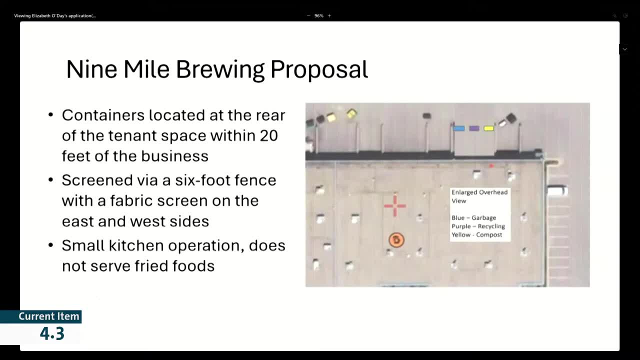 System and not the storm set storm sewer system, Which is really important, and then not located in parking areas and drive aisles, sidewalks etc. and So a little bit about their proposal, specifically Their containers. they would have three containers: trash, recycling and compost. they would be located at the back of their site. 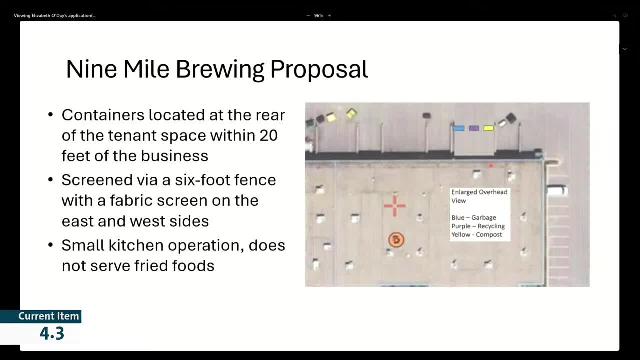 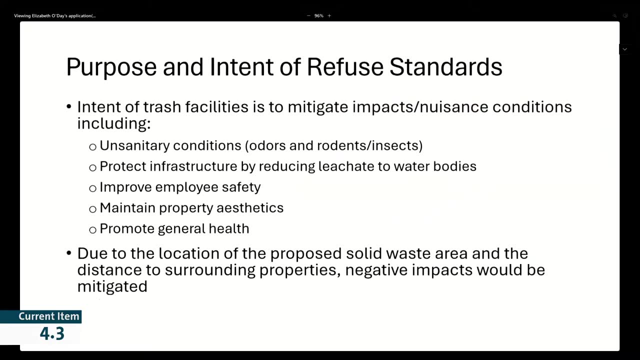 located within 20 feet of the business. They have overhead doors Just behind those bins, and then they're planning on screening it with a fence, and then Just to note that their operation does not serve fried foods. and so when we receive these privately initiated, Initiated city code amendments, We look at the purpose and intent of that ordinance. 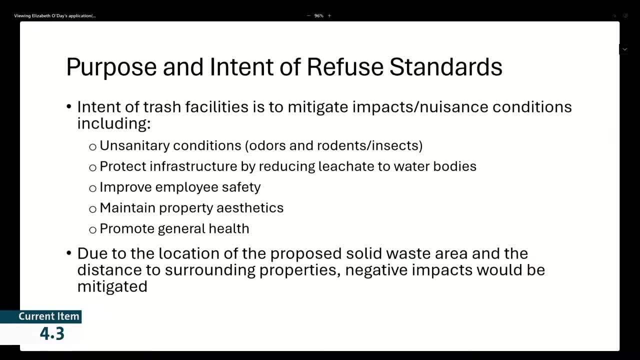 and so the purpose and intent of our trash ordinance is related to mitigating certain impacts, so, such as on sanitary conditions, like odors and rodents and insects, protect our infrastructure and then improving employee safety, maintaining aesthetics and then promoting an overall health. and so, due to kind of the uniqueness of the 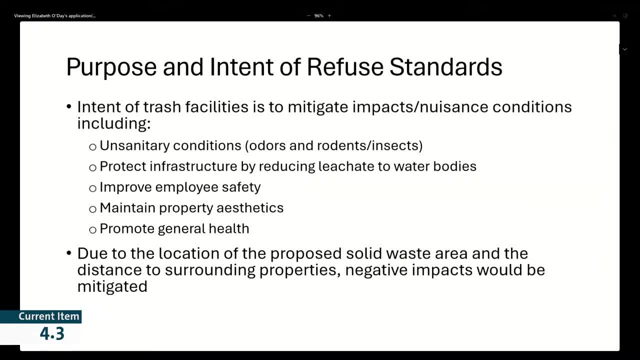 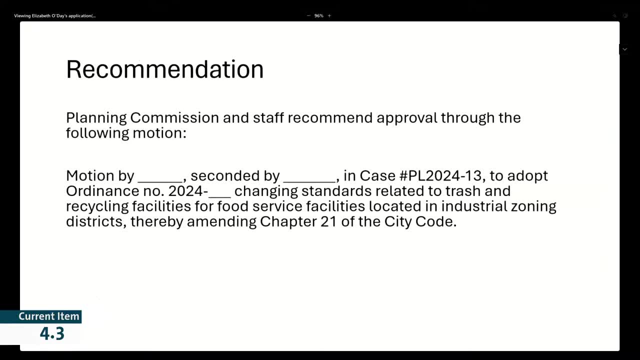 site, as well as the area being far away from surrounding properties, negative impacts would be mitigated, and so, with that, the Planning Commission and staff are recommending approval, and mr countryman is in the audience should there be any questions. thank you, miss O'Day. we'll get to mr countryman in a 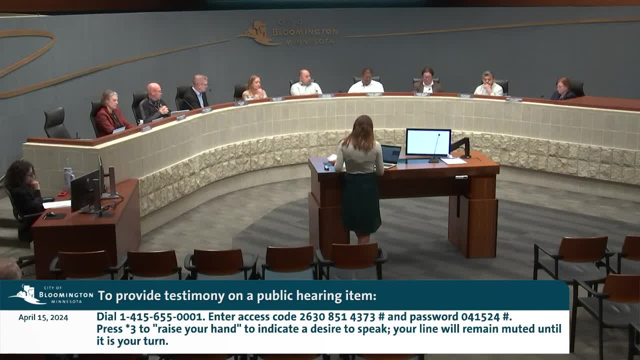 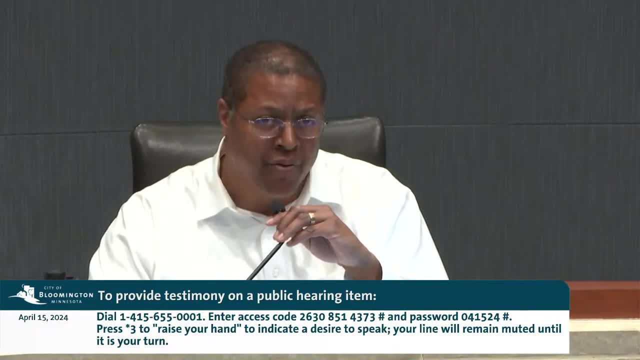 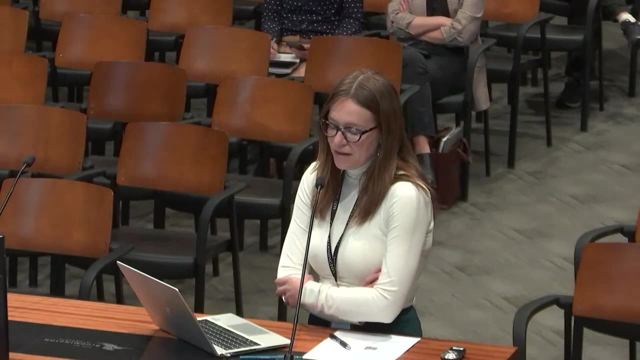 moment here I counsel questions of miss O'Day regarding this. council member Lohman. thank you, just a quick question. so if there's a new tenant, would, with this standard, if we pass this tonight, continue forward or would it have to be replied? mayor and city council member Lohman. so this would provided that they meet the 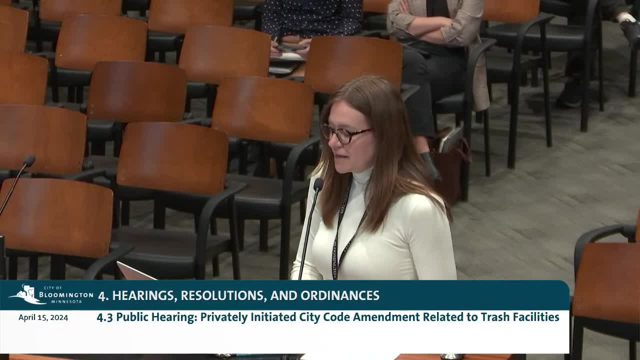 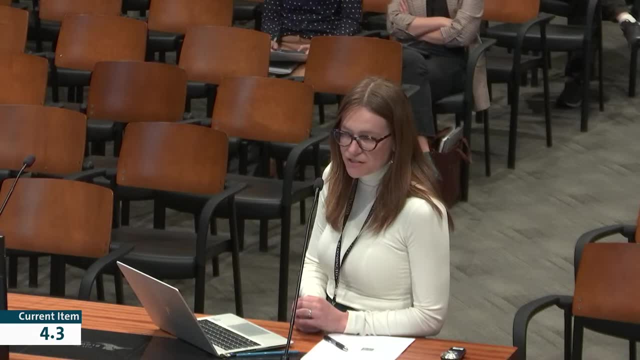 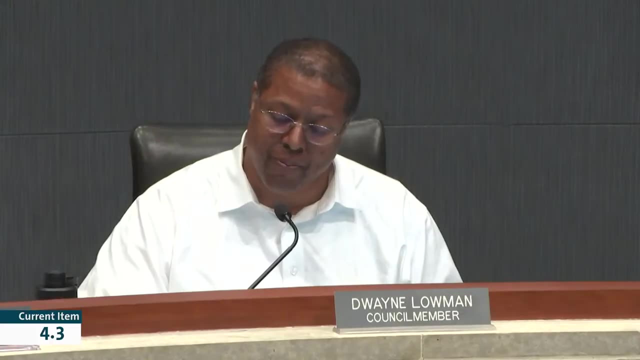 same standards. they don't serve fried foods and it's obviously still an industrial zoning district, so, provided that's all true, then this: they could store their containers outside. this is a code amendment which would change the code. it's not tied to a specific property. thanks for the clarification. 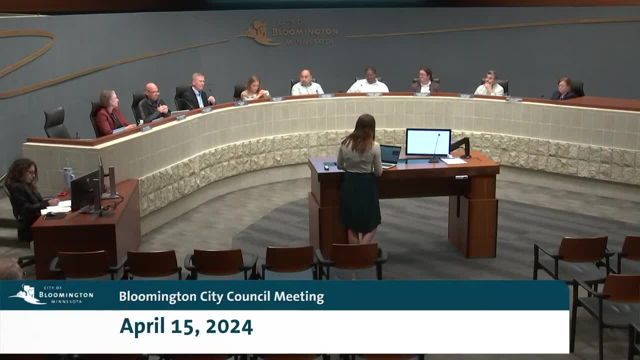 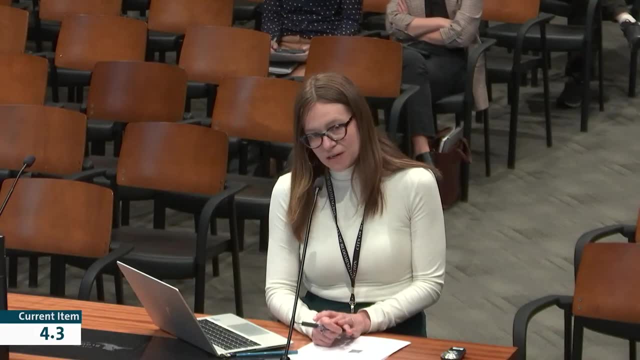 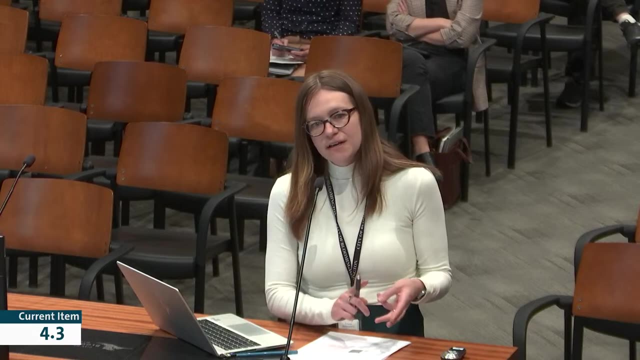 additional questions. so where else would this be applicable city wide? where else would we see this be put to use? Thank You, mayor. so we did do an analysis and we didn't find any other properties that would be impacted with the criteria of the industrial zone, the fried foods criteria and then the 500. 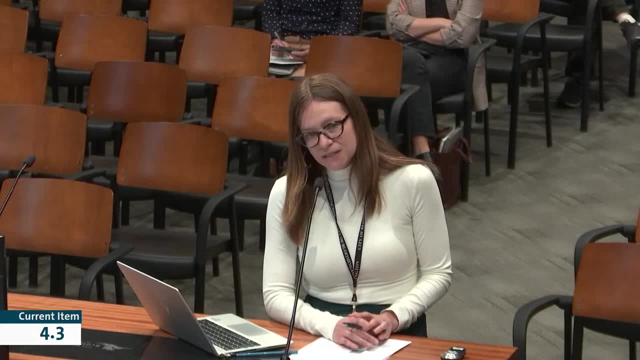 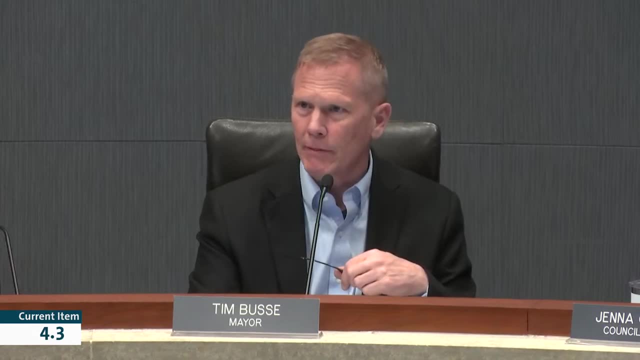 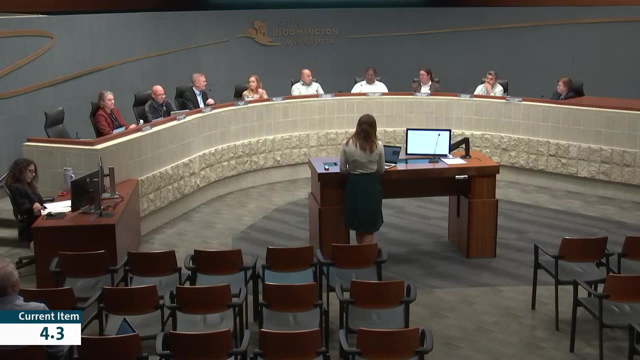 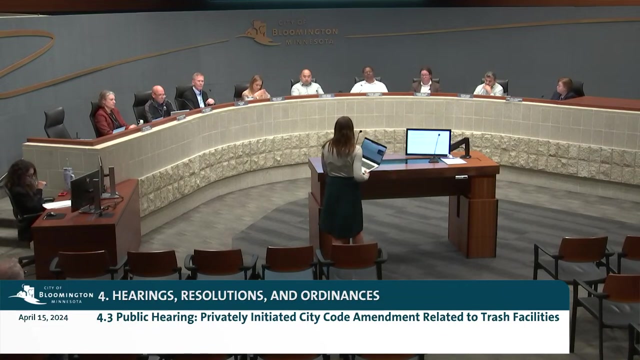 feet away, so nine miles, is the only property that would be impacted. but that's not to say it couldn't be applicable in the future if someone met those standards and was doing the same type of thing. that's good to know. council additional questions. very good, why don't we, before we open up the public hearing, mr countrymen and 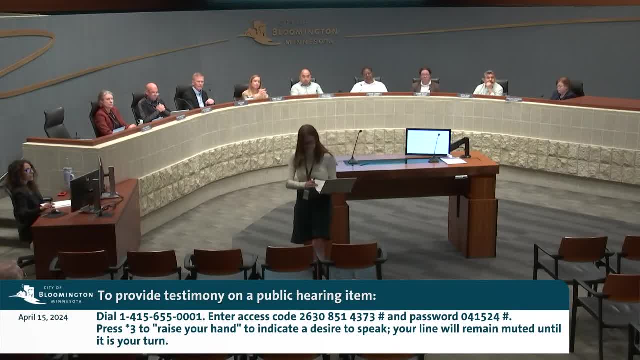 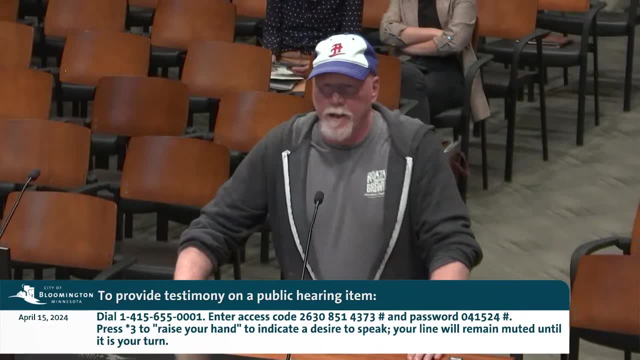 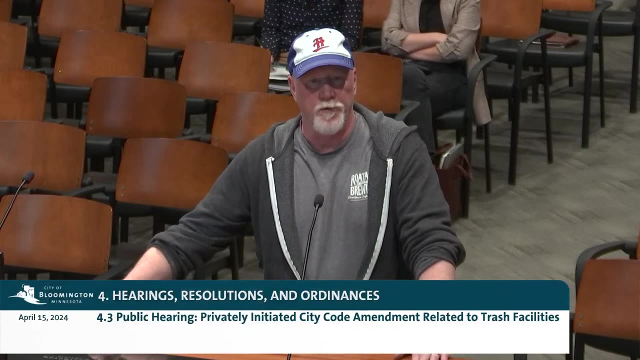 anything you'd like to add to the to the discussion with us tonight. good evening, welcome evening, mayor council. no, not really. I don't really have a whole lot more to add. I just feel like, from what I understood the risks of why they had put that code in. I feel like we are addressing those very 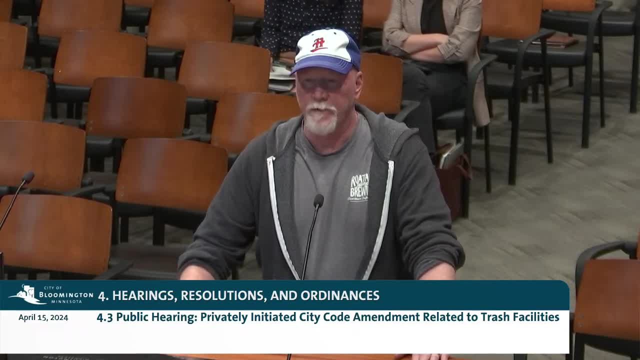 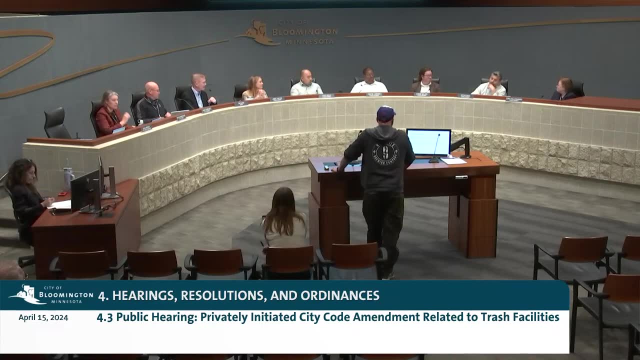 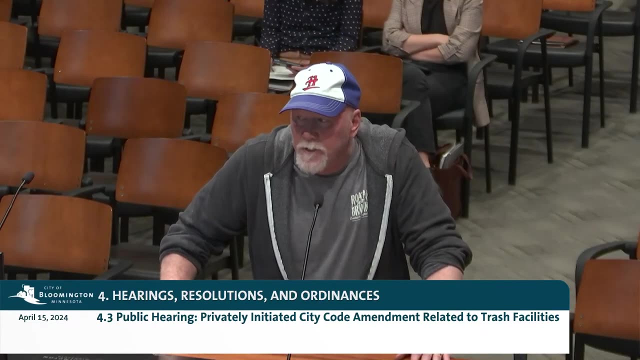 well with the proposal we have. so with that, I would just ask the council mayor for your consideration. very good, thank you. any questions of mr countrymen? councilmember Rivas, I do have a question for you. I've seen. what kind of food are you gonna be producing in the facility? it's gonna be a pizza focused kitchen. 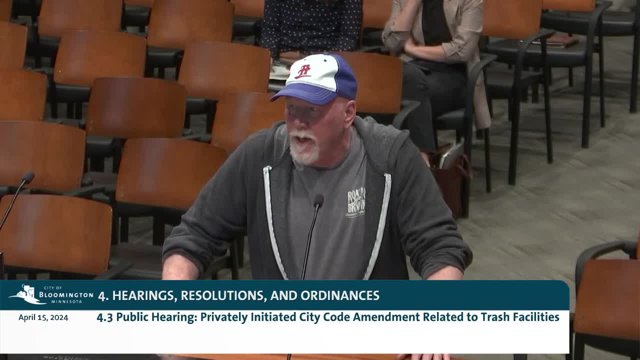 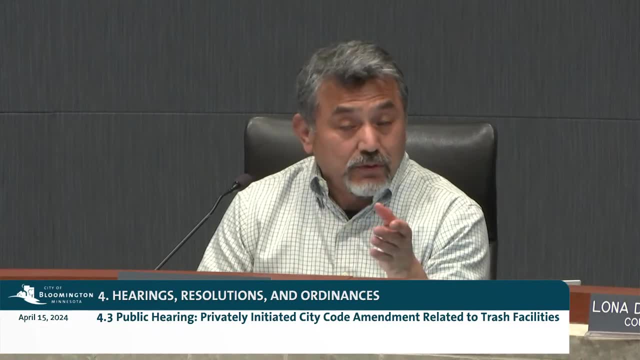 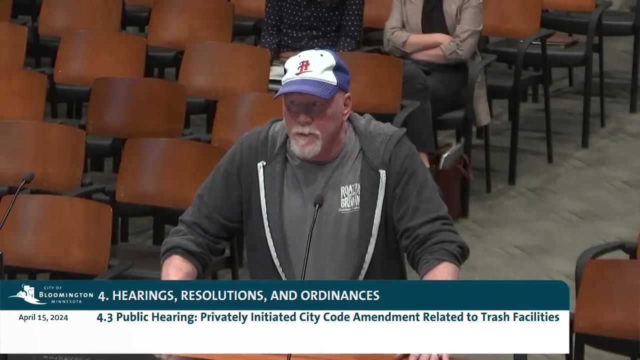 with some sandwiches. there'll be some vegan options, vegetarian options, some salads, but it's not gonna be a super large menu. it's gonna be mostly pizza focused, so it'll be just a piece that will be the main item, provided, mostly cold, or it'll be a combination thereof. there will be. 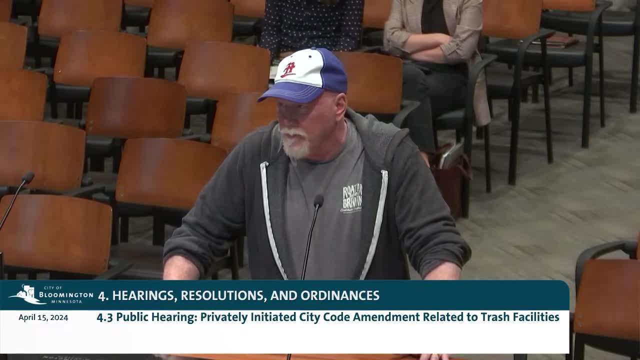 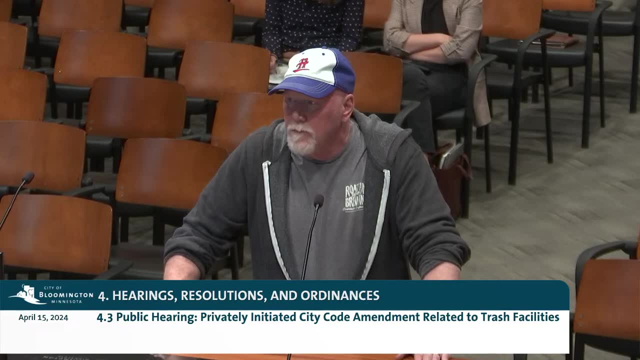 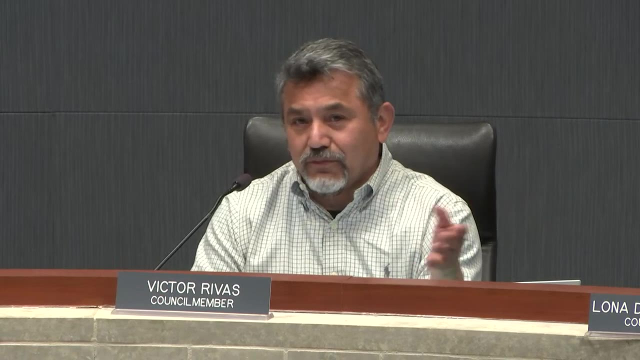 some cold items as well, but there also will be some hot sandwiches, like a chicken caprese caprese, which is a vegetarian option. so they'll be both hot and cold food. you can see the reason I'm asking you speak it because of the garbage. there's gonna be food items in the trash. so animals, insects and all. 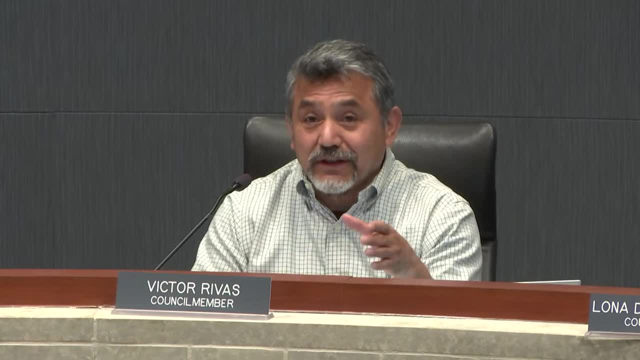 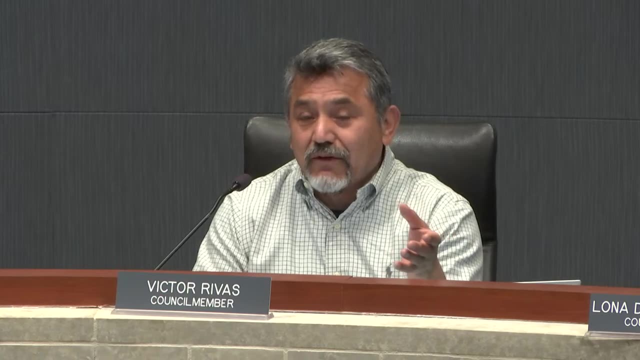 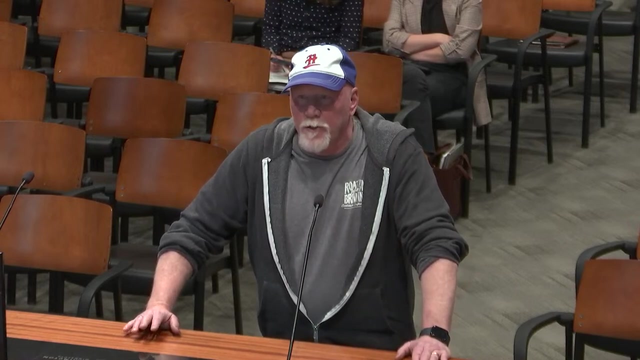 kinds of stuff is. they will come regardless, right the containers, they're gonna be up to standard to the state regulations to have them. you already own those containers at the facility, so we don't own them. we go through Aspen waste. and one thing that I would point out, just 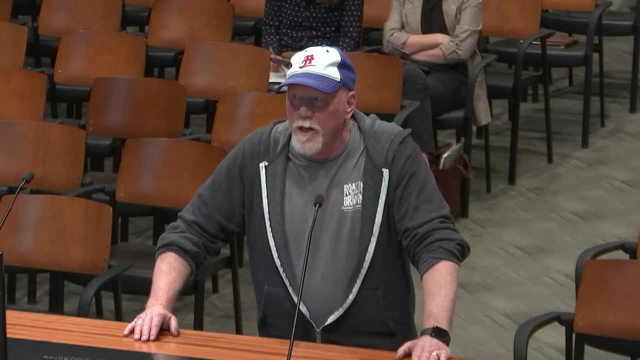 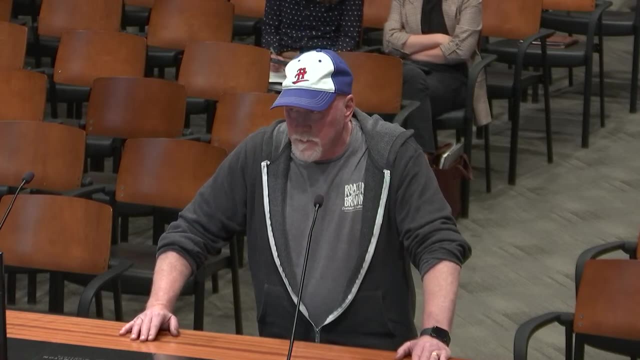 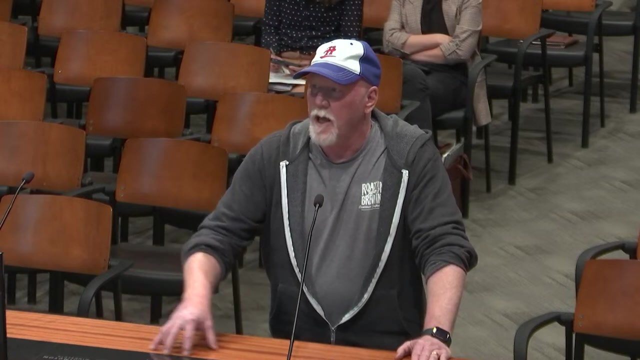 because of the nature of what we are right now is. we are a manufacturer, so we have food trucks five days a week. so we currently bring food garbage out to our garbage containers, but it's not under this because it's a different format. we don't actually produce the food and we have not had any problems with 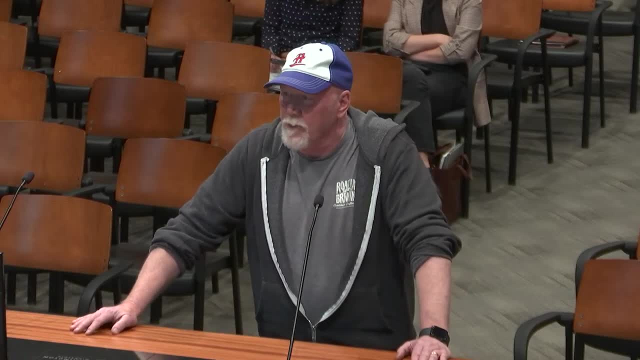 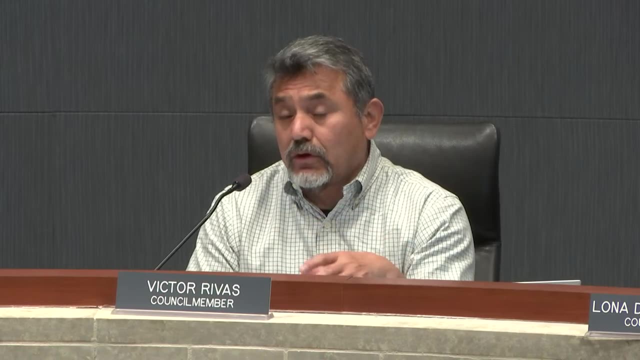 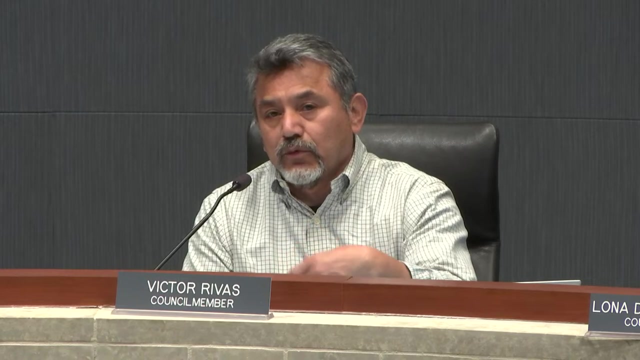 rodents, insects, smells, odors with the existing garbage as it is. that that's exactly what I'm the question I'm asking. you're not producing any of the food that you currently use. therefore, the garbage is not the normal garbage that you will be creating if you're a food manufacturer at this point. if you're. 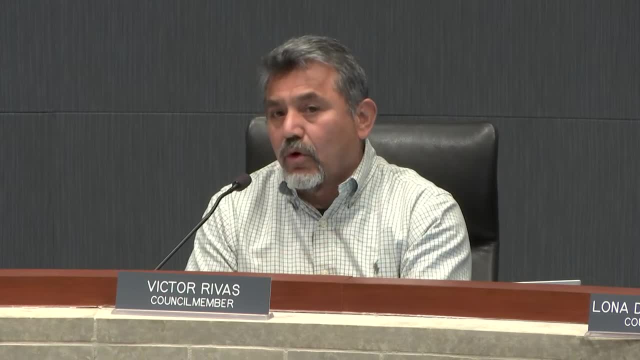 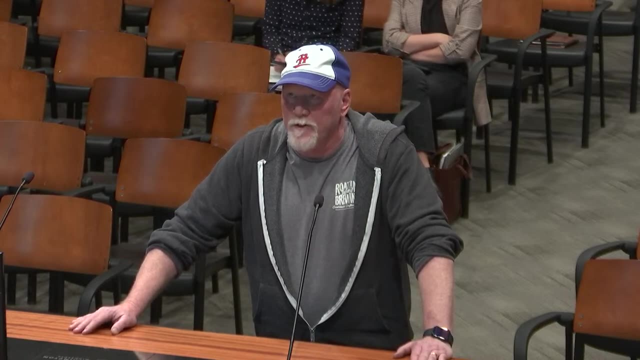 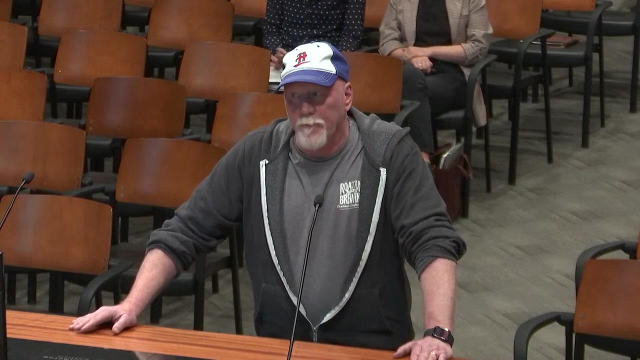 producing food, you're creating a type of garbage that you currently don't have, in a sense, but I would also argue that leftover food it's not going to be the garbage from the preparation, but it's typically the garbage when people are done eating, and that is what we currently are doing. we're 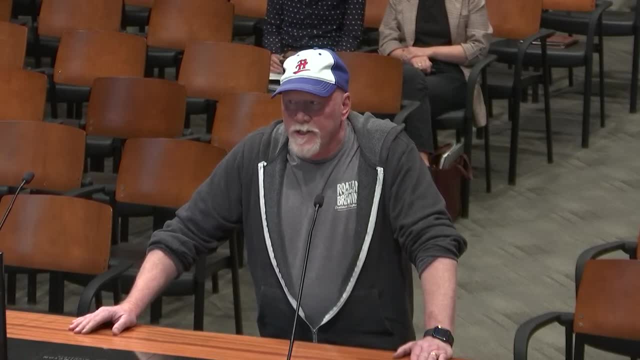 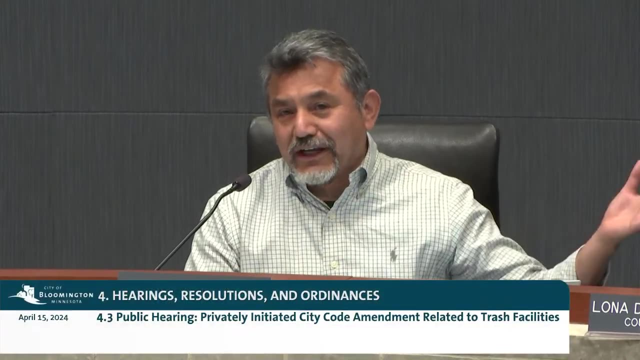 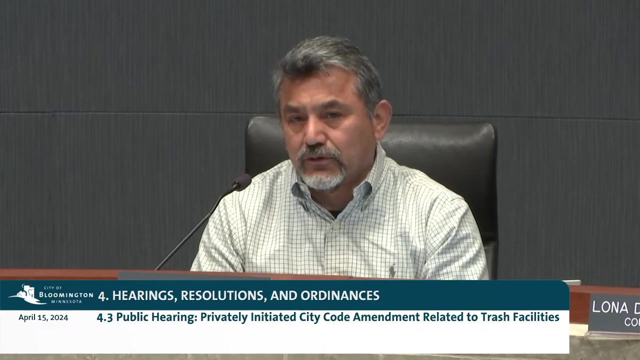 not producing it, but food trucks are. so I don't really think the nature of the garbage is going to change significantly. so what you're asking us to approve- to have those containers on the outside rather than inside the building, right, like normally a food production facility has those containers inside the building. 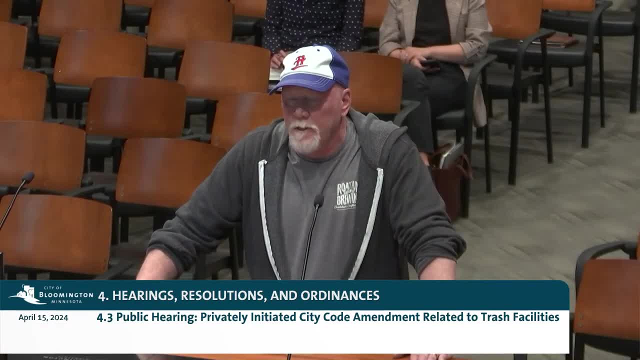 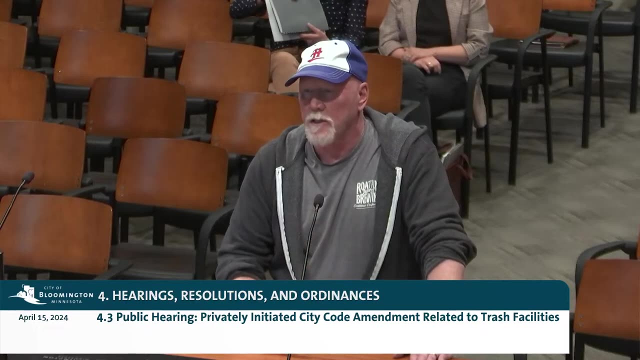 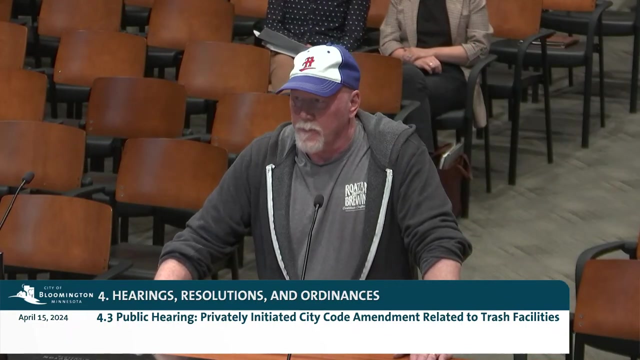 in a garage or so I would say. normally in Bloomington it is required. it is not required in neighboring cities that I have reached out to. so that's part of this is, you know, trying to, in my mind, make Bloomington a more business-friendly. we talked about small business in the beginning. there's a lot of hurdles. that 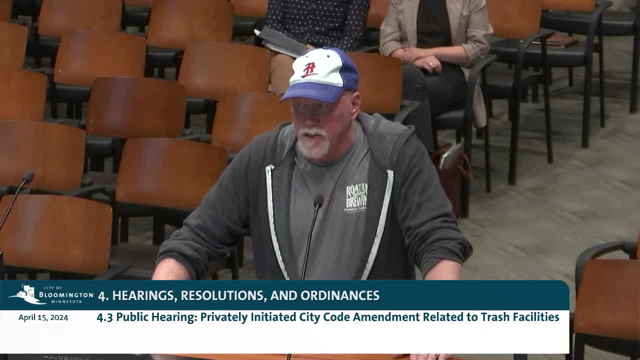 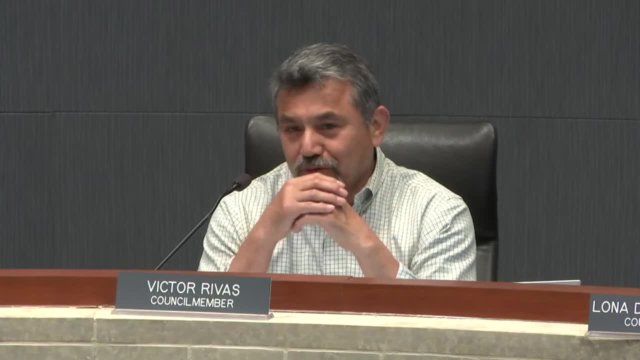 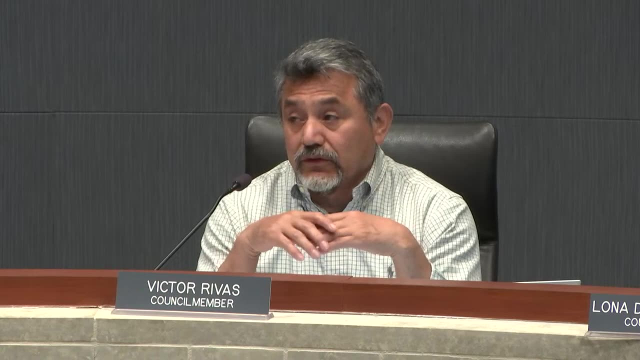 get put up, and putting an indoor garbage facility is expensive. if I may, I actually manage facilities that produce food and it's not only in the city of Bloomington that we are required to provide those indoor facilities for trash. I mean pretty much. a company I work for has facilities all over the state. 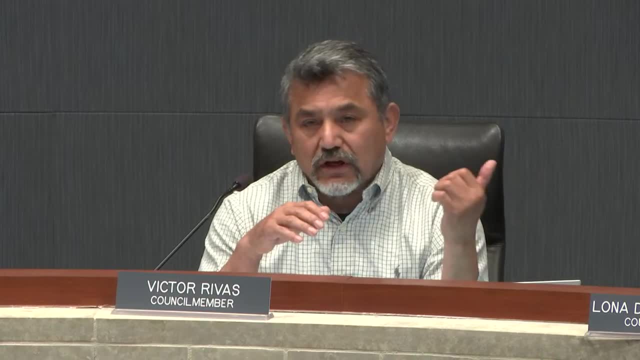 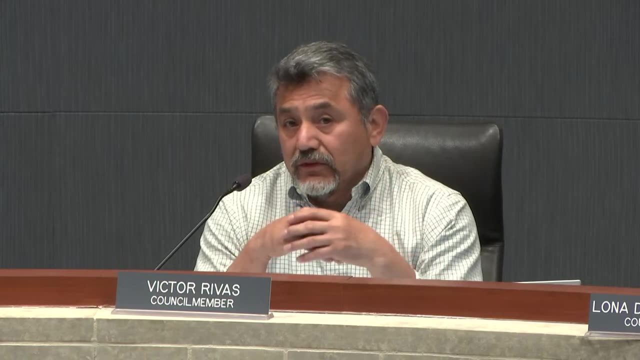 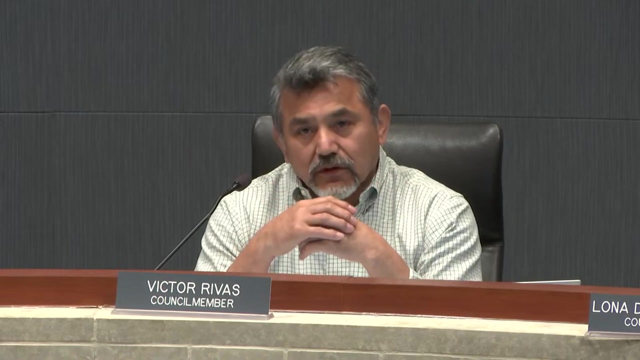 and in every single facility. we don't have any garbage outside the buildings because it's required by the state to have facilities indoors because of the animals, rodents and all kinds of insects that can come regardless, even inside indoors. so you have to maintain those facilities clean at all times. 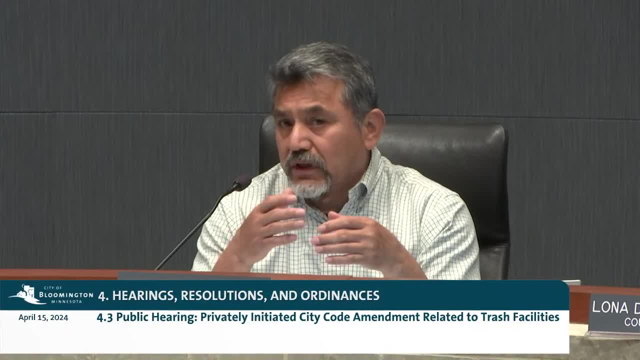 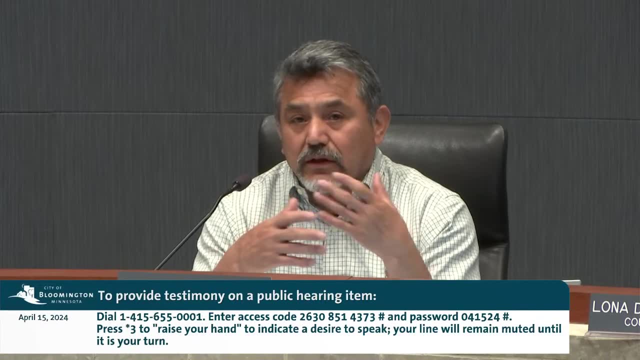 So that's why I'm asking those questions. So, since we're being asked to change the city code specifically just for your business, that's what I kind of worried about it, because I mean it applies only to you, According to the research that has been done. 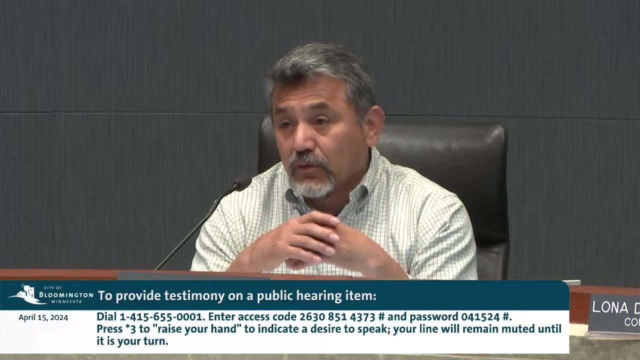 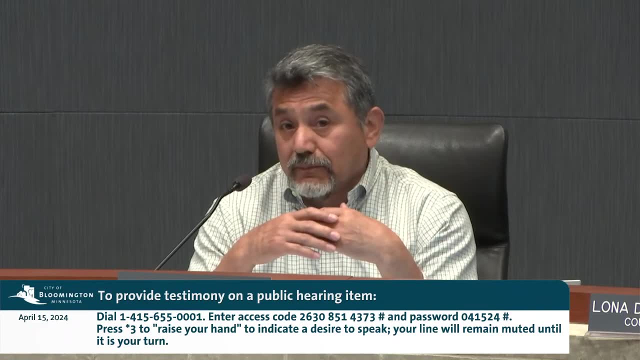 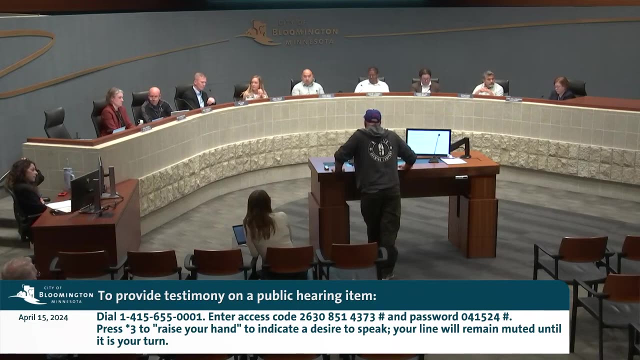 by the city staff. there's no other location that would require those permits, so that's the only thing that I'm concerned about. I mean, it's a state requirement to have indoor facilities for trash. So when I've reached out to other cities- including Edina, Eden, Prairie, I think, maybe Egan- 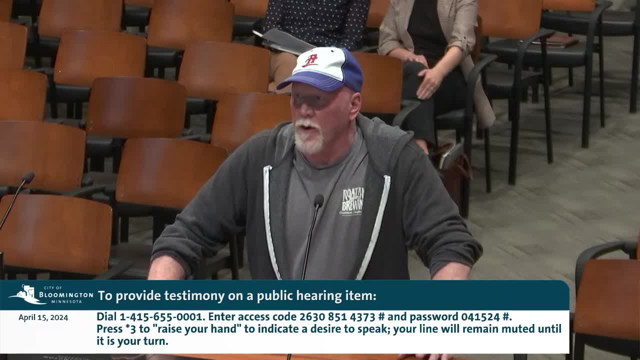 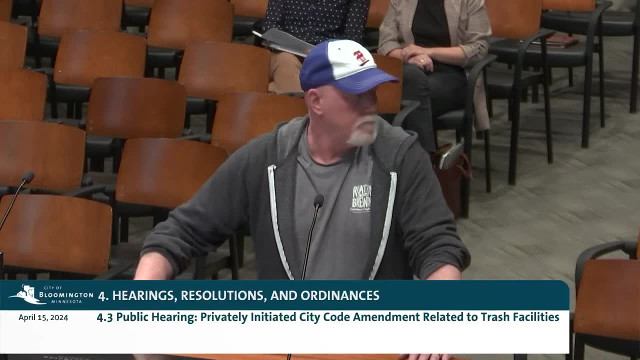 I was told no, and I have it in writing and emails that they are not required. So I do not believe it's a state. I am not. I'm not an expert on that, So you know, did you have that? 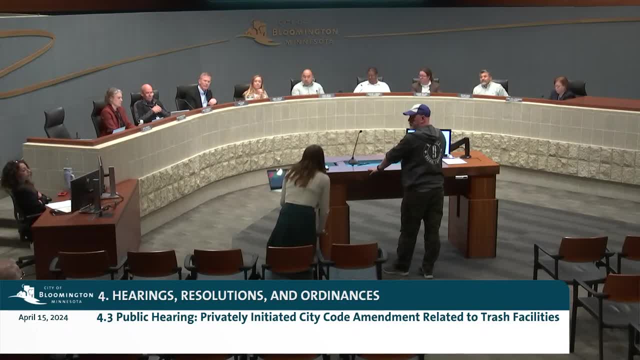 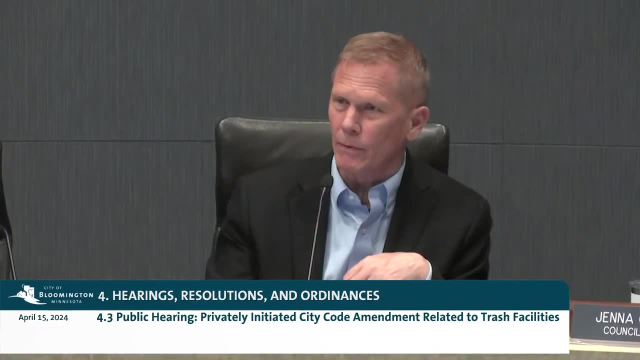 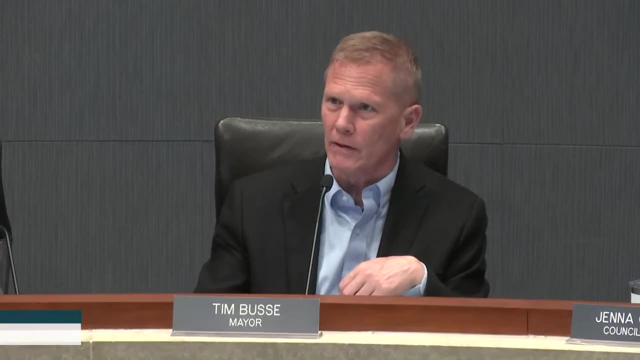 I appreciate that, Mr Countryman. I'd look at Ms O'Day if she's got a more concrete answer. Is Bloomington right now? by requiring indoor trash containers, are we inconsistent with our neighbors or are in fact in our neighboring communities? are those facilities allowed outside? 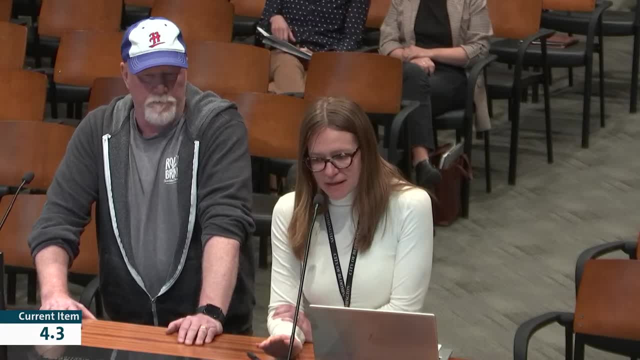 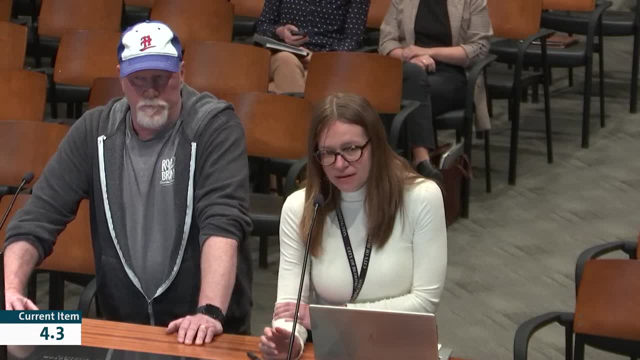 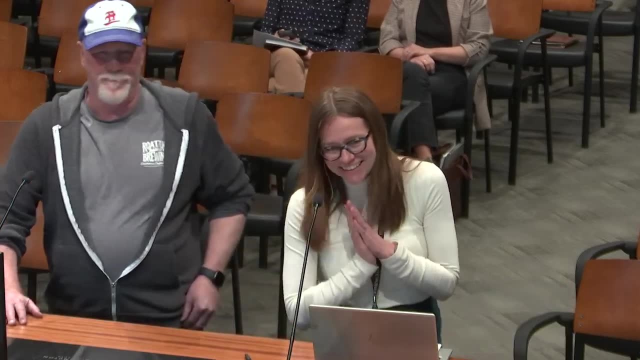 I'm not sure. I'm not sure, I haven't done the research, but I think that we are kind of a special community in that we allow trash indoors. Well, I agree, we're a special community. I won't argue with you on that. 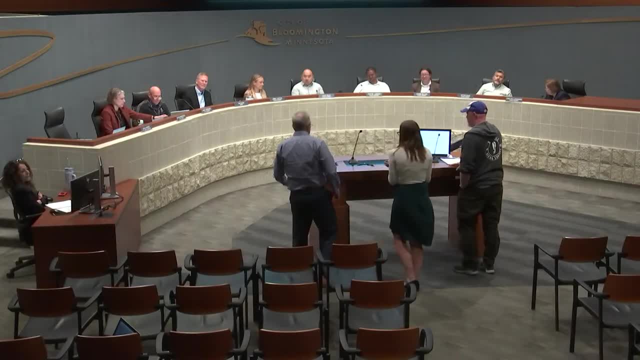 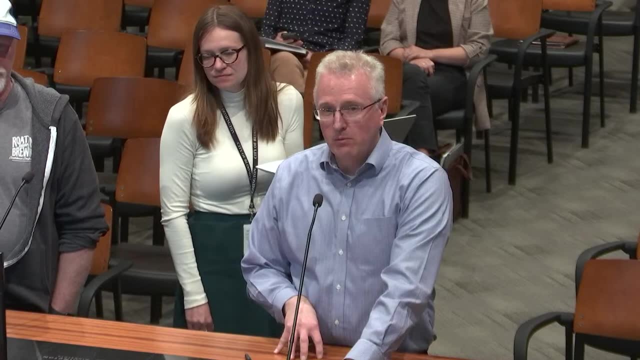 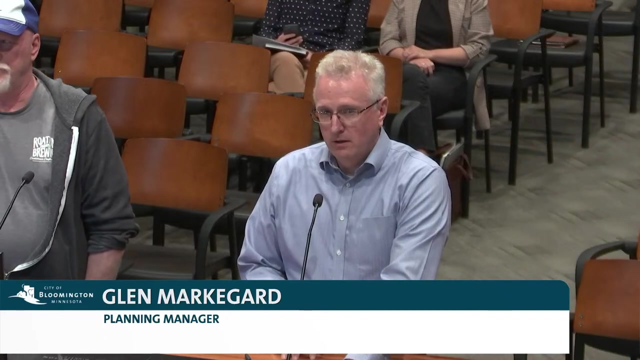 Mr Marker, do you have any insight you're able to provide? Yes, Mayor Boise, council members, we have done a lot of research recently on other city requirements and Bloomington is quite a bit stricter in terms of trash standards than most of our. 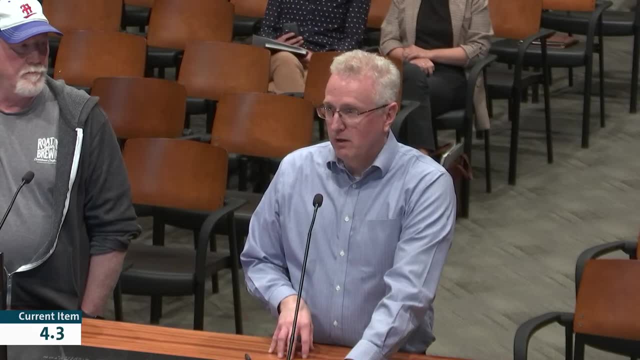 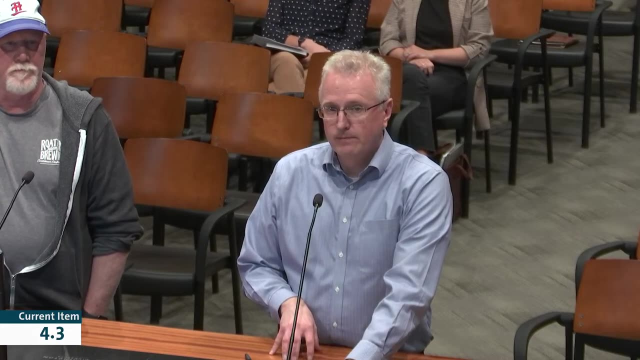 peer communities, The state provision. we'd want to look into that more. I'm not aware of that, but if that exists, we'd want to find out a lot more about that, Absolutely, Thank you. All right, Council Member Rivas. any follow-up questions? 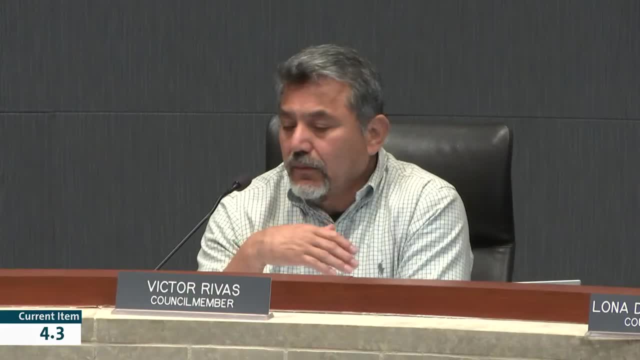 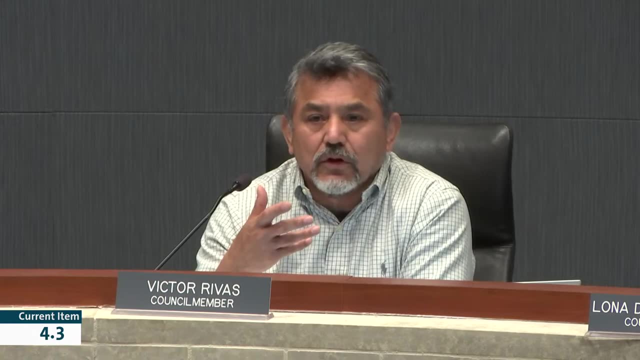 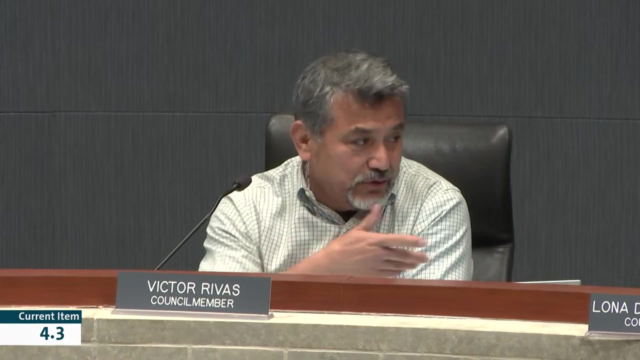 Anything else? No, Again, I'm not all against any of the small business. On the contrary, I support small businesses 100%. I just ask these questions because I happen to work. It's considered a small business we were just discussing here. They do own about 100 facilities- I'm sorry, but still considered small businesses- and we're required to have all these to the state. As a matter of fact, we just had an inspection last week and they're very rigorous inspections. 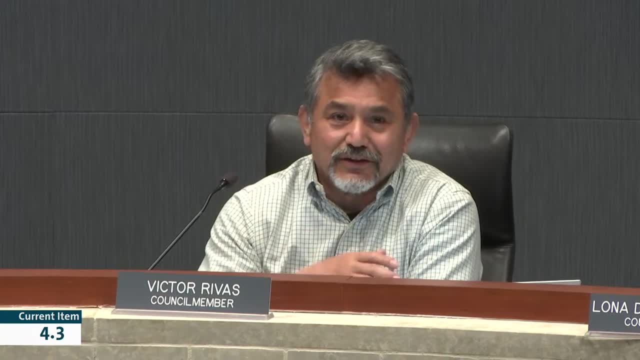 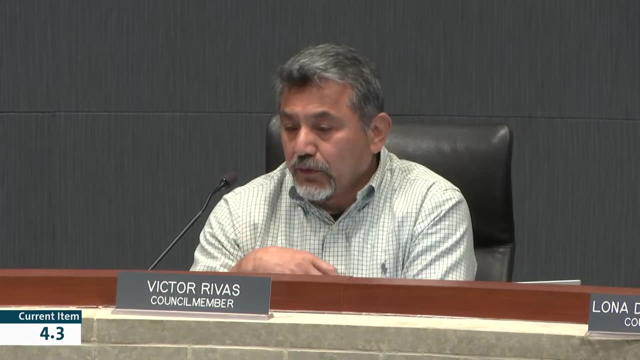 three days for eight hours a day, inspecting every single aspect of the operation. So that's the reason I bring it up, I mean because If we're going to start doing that, it's a thin line to walk through, you know, because 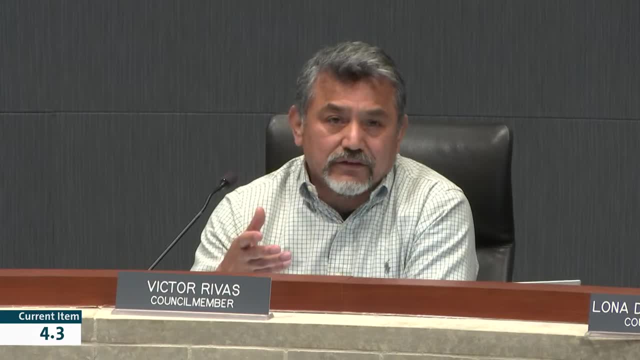 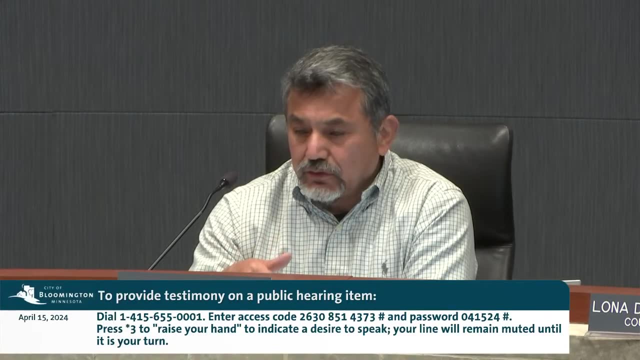 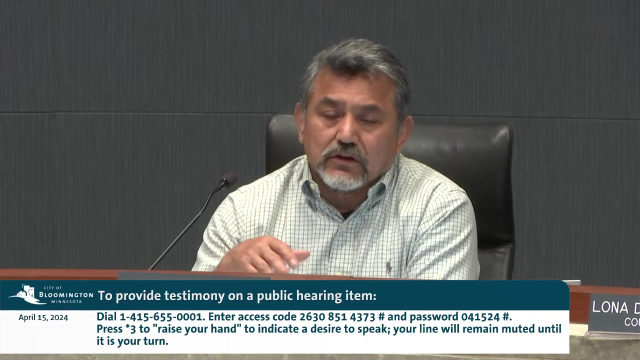 there are a lot of other businesses that require or are asking for permits or variances in the ordinances that the city currently has, and if we're going to start doing this, it has to be done across the board. I just wouldn't like to see any specific business to be taking advantage of what the city is. 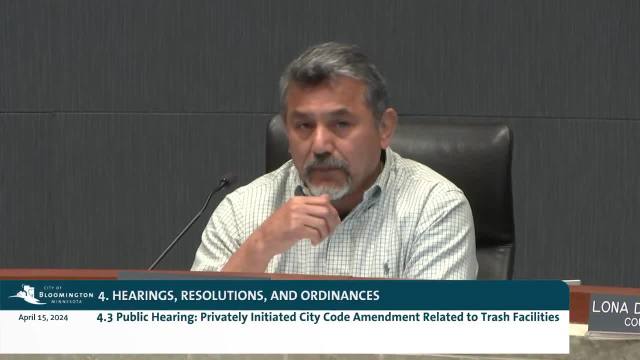 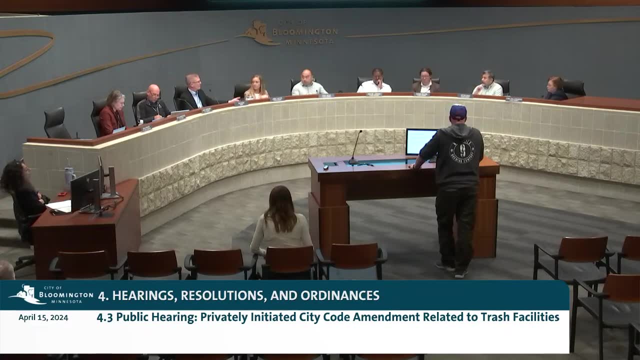 facilitating when other businesses are struggling to try, So I think it's important to get things done on their behalf as well, And I'm talking about small businesses also. So, with that said, I don't have any more to say Thank you. 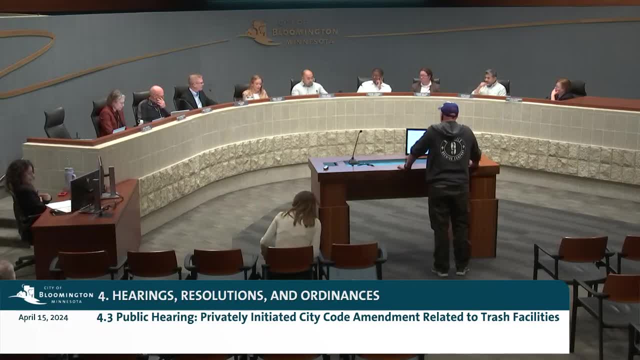 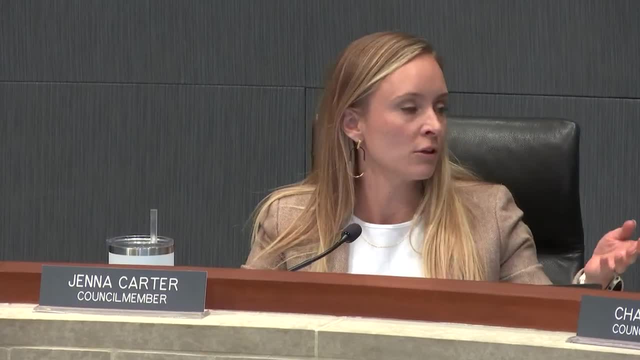 Council Member Carter and Council Member D'Alessandro. Council Member Carter. Thank you, Mayor, I guess I'm just wondering if maybe the difference here is that like the type of business right, I'm assuming that you don't work for a restaurant or a brewery, or I think the state regulations apply to different types of business, and I don't think that they apply to breweries, Breweries or restaurants. I think that's more at the local level, And so I'm just wondering if maybe that's the biggest difference. 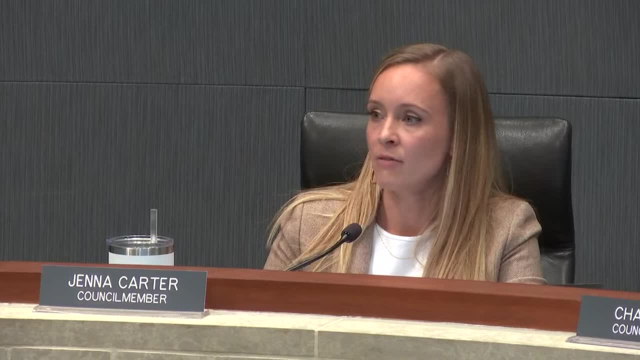 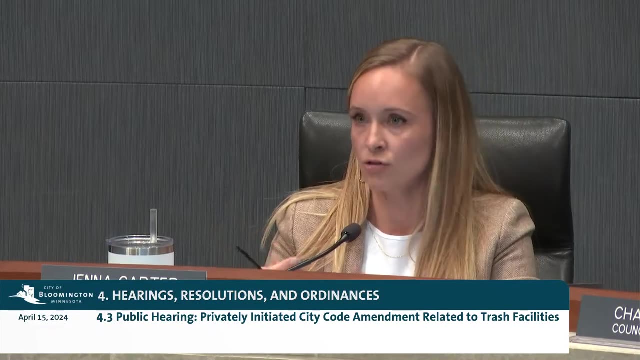 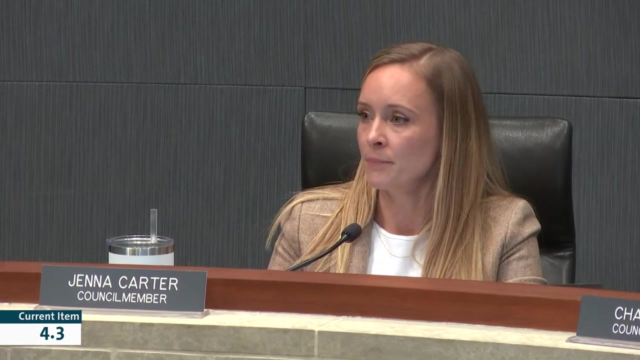 And what I'm hearing is that there may have been similar concerns on the staff side but, because of your situation being in industrial 500 feet not doing fried foods, that it addresses the concerns that were brought up and that if other businesses were to say a distillery- 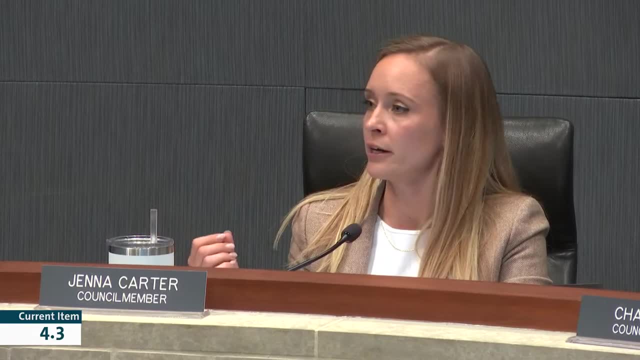 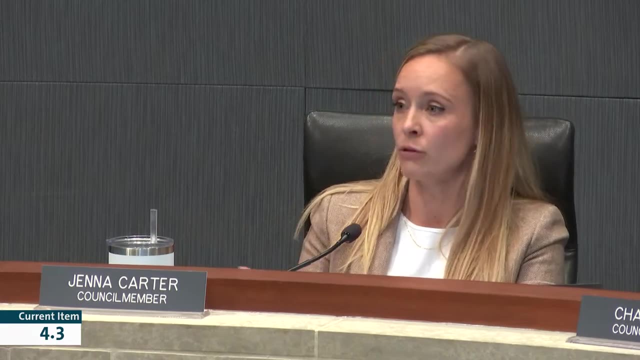 open In another part of Bloomington, an industrial area, this would also apply to that business, So it wouldn't be just Nine Mile. It would be other businesses that meet the requirements and we're not opening it up to all restaurants across the city. 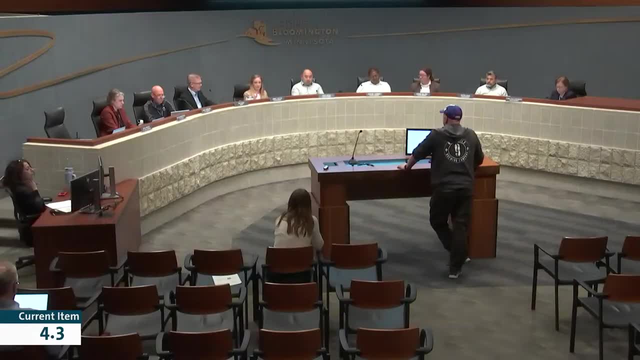 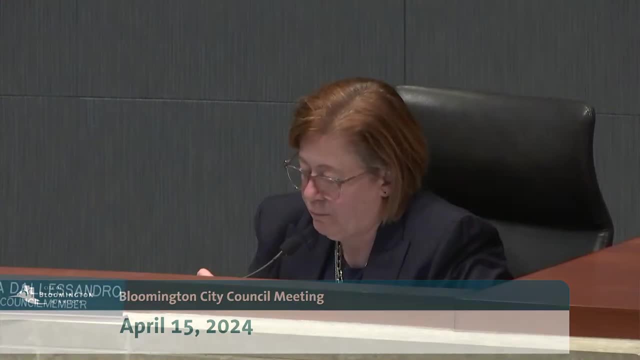 It's really. There are specific standards. Yes, Correct, That is correct. Okay, Council Member D'Alessandro. And thank you for that, Council Member. That's good clarification. I think you're correct, Council Member D'Alessandro. 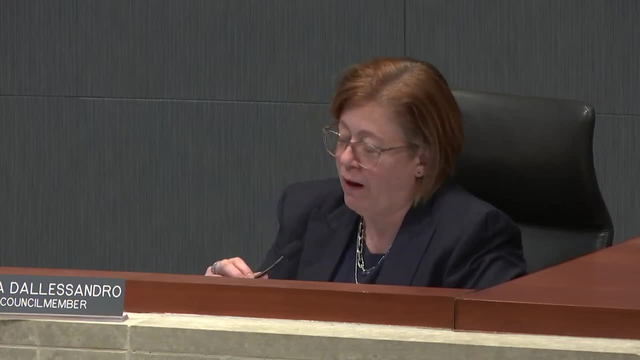 I was just going to ask the question. Mr Mayor, I have comments to make, but I'm assuming we're going to do the public hearing first. right, We're going to do the public hearing first. I just wondered if you had any additional questions. 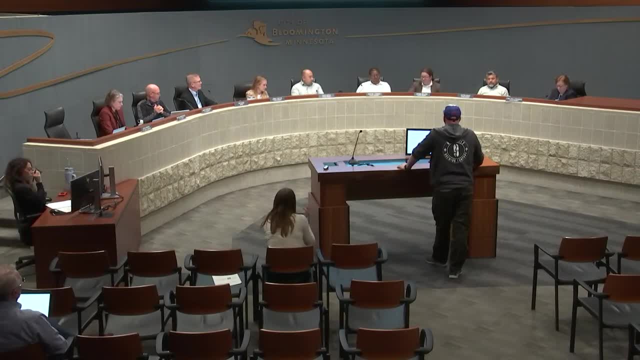 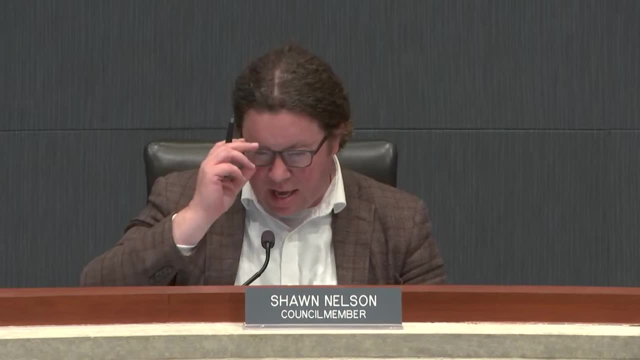 I don't have any questions for Mr Countryman. Thank you, Council Member Nelson. questions to ask You have a question? Why are we looking at changing the ordinance versus a variance? And the reason I ask that is when we looked at that hot dog stand over by Sonic, weren't? 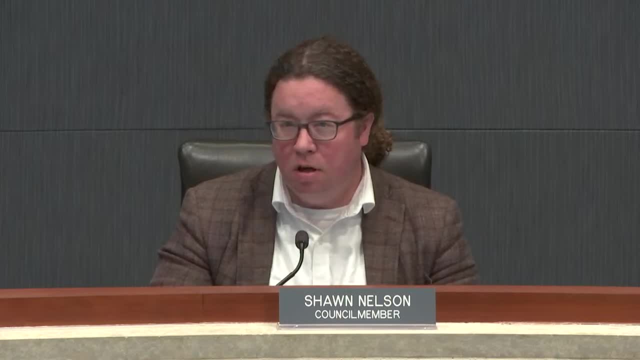 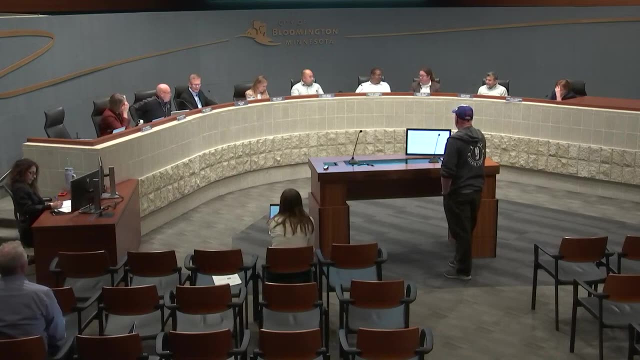 we doing a variance there. for their outdoor trash They ended up going to Woodbury or something I was going to say I don't recall. the hot dog stand over by Sonic. Yeah, Mr Mayor and Council Members, I believe Council Member Nelson is referring to the 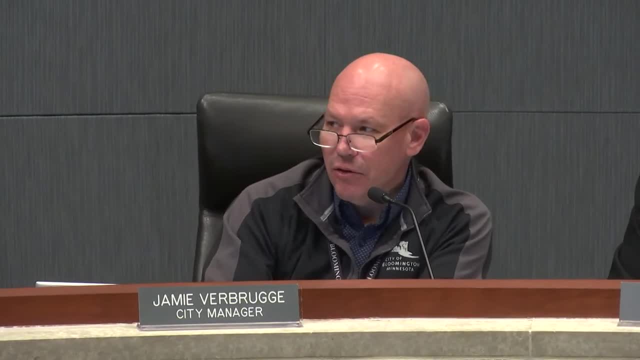 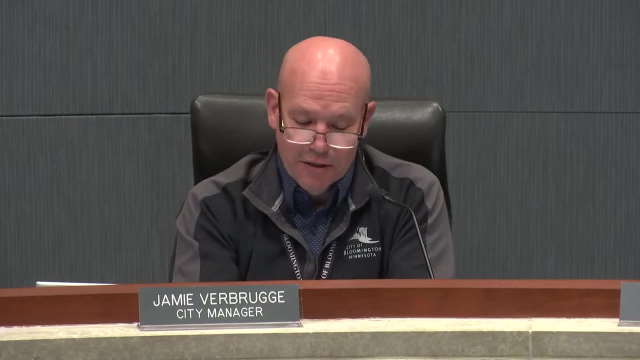 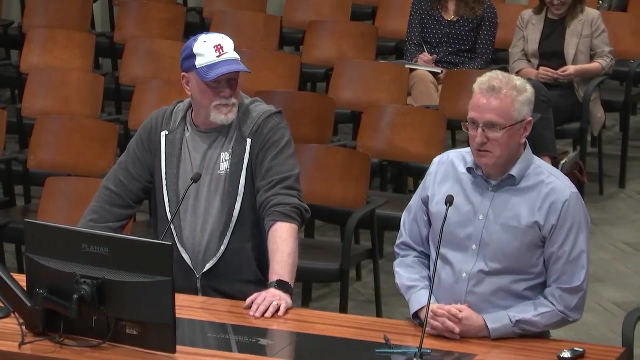 Portillo's application back in around 2018 or so. Yeah, it is. I'm still longing for the Portillo's, since it didn't come here. Mr Market Guard insight on this. Yes, Mayor Busse. Council Member Nelson. 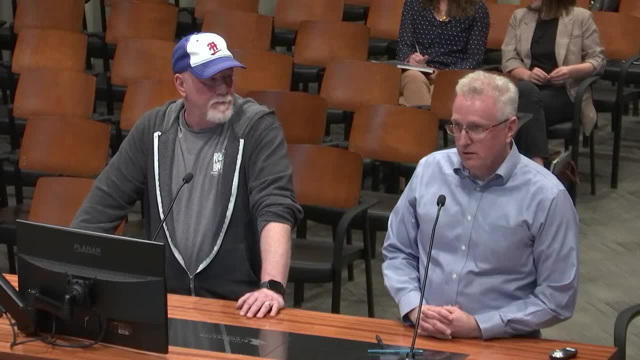 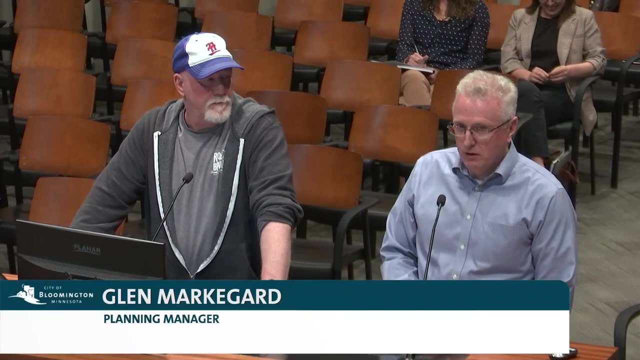 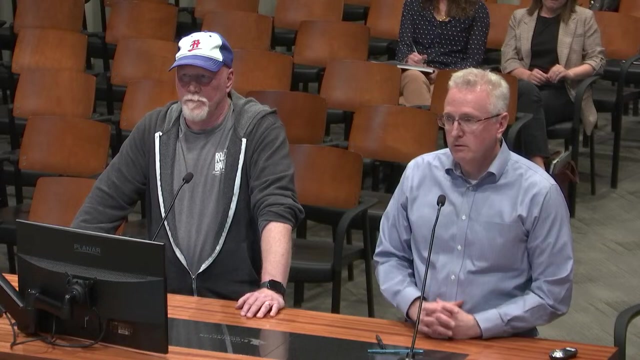 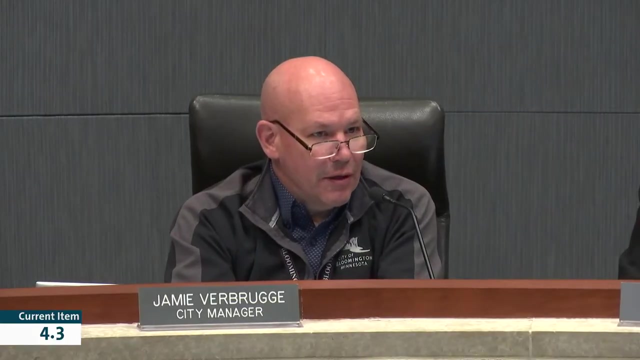 We did have an application several years ago from Portillo's, Knox and American And ultimately they withdrew the application. But before they withdrew it they had been requesting flexibility on the Bloomington trash standards to do outdoor trash. Mr Mayor and Council Members, so I think the question you're asking about a variance. 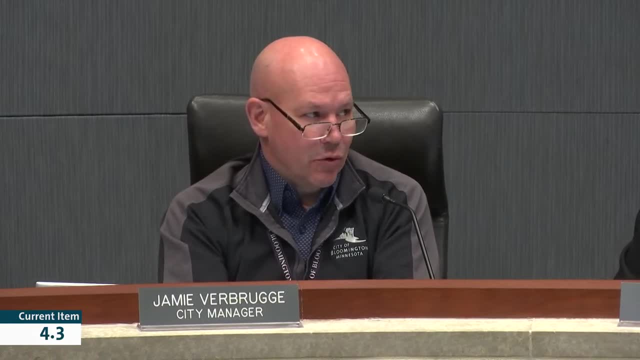 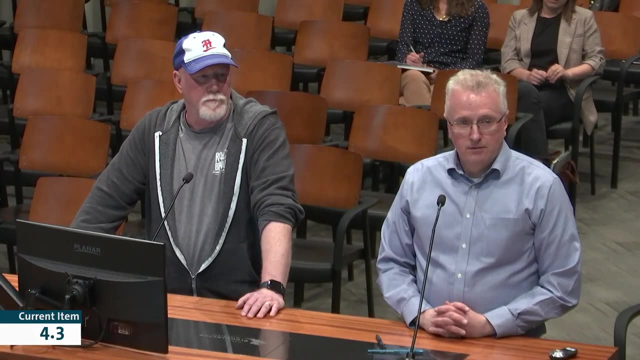 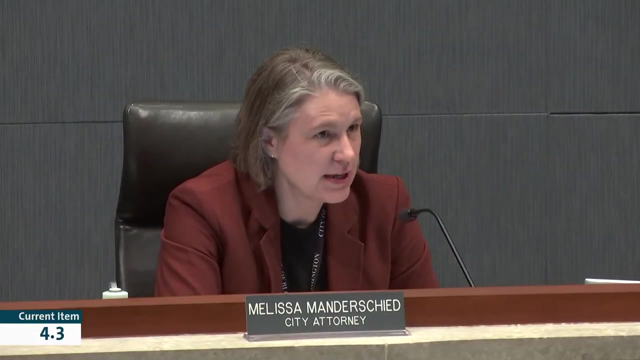 is a variance is specific to a land use and not an ordinance. Is that correct, Or do we have variances for this particular provision? Mayor Members, variance is typically more suited for things like setbacks. This is coming across to me more as a use of the property. 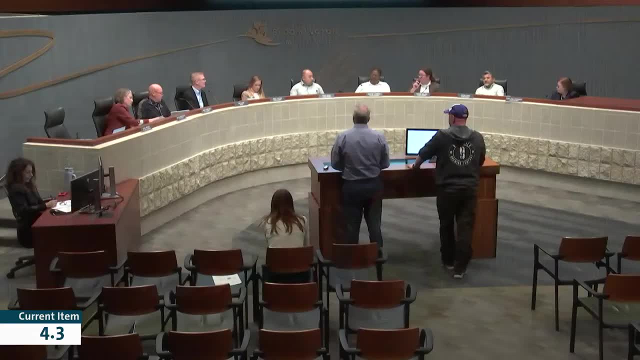 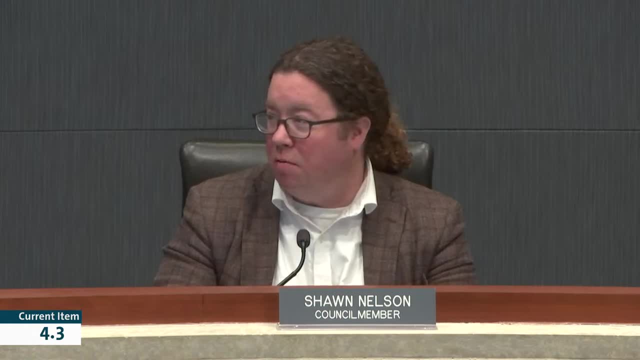 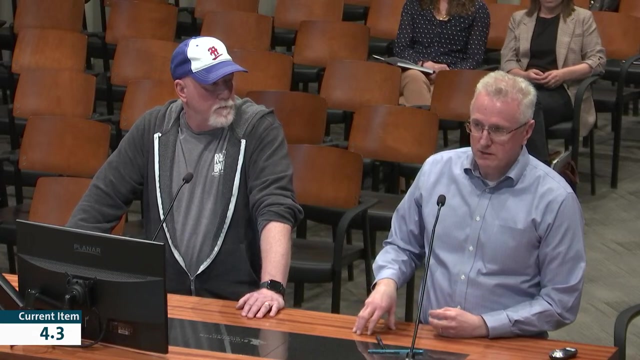 Because we weren't changing an ordinance for their when we were considering their outdoor trash. So what process were we going to do there? Mayor Busse, Council Member Nelson, In that application they were requesting flexibility through the plan development. So it's the PD. 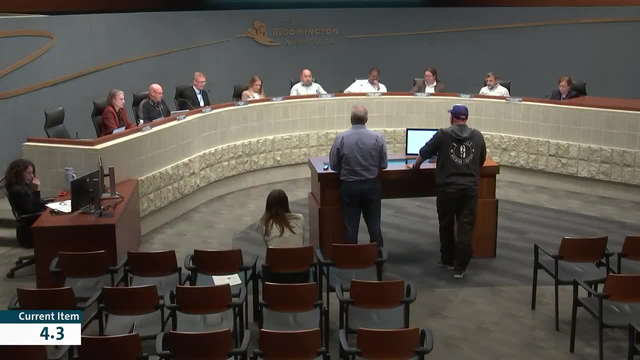 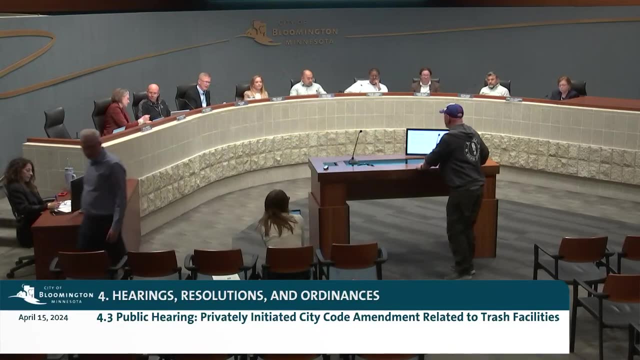 Process: PD process. Okay, Thank you, all right if there's no further questions. council, why don't we get to the public hearing? if we could, thank you, council mayor. thank you, mr countryman. uh, this is a public hearing. this is item 4.3. 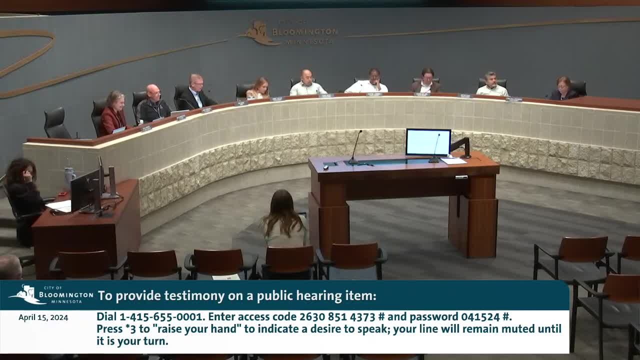 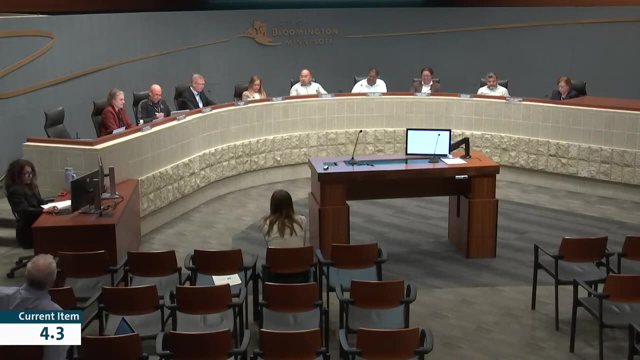 public hearing regarding a privately initiated city code amendment related to trash facilities. anyone in the council chambers wishing to speak on this? ms mercer, do we have anyone on the phone wishing to speak? no one on the phone wishing to speak. last call to anybody in the council chambers. 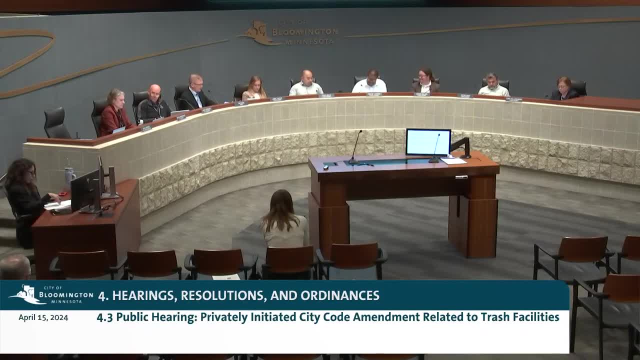 council. no one on the phone, no one coming forward in the chambers. i would look to look for a motion to close the public hearing in item 4.3. this so: motion by council member loman, second by council member dallas honder, to close the public hearing. 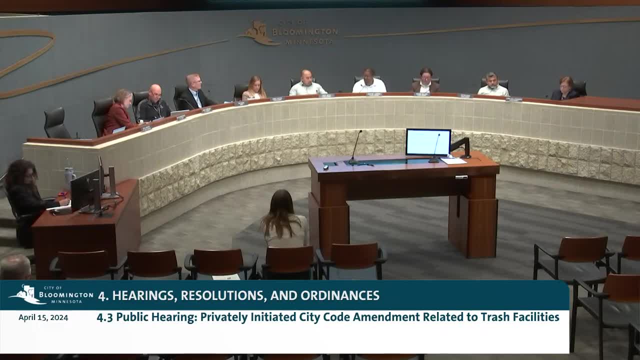 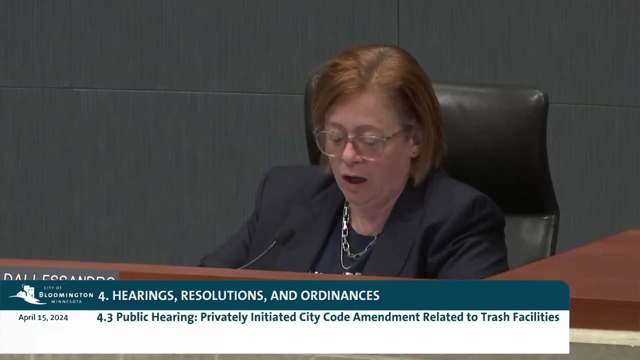 in item 4.3: no further council discussion on this. all those in favor please signify by saying aye, aye. opposed motion carries 7-0. closing the public hearing. comments on that. comments on that, uh, comments on that, uh, councilmember d'alessandro. thank you, mr mayor. um, okay, a couple of things. uh, one, um, if it was up to. 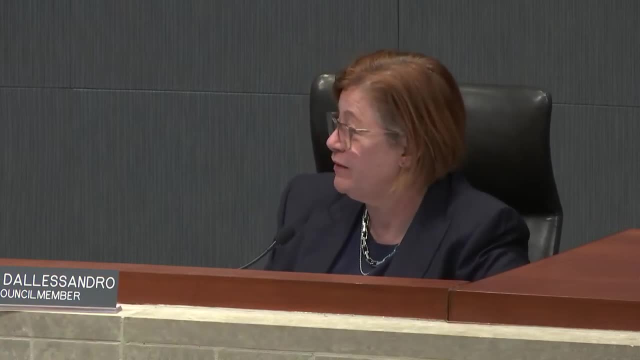 me we would just get rid of this whole thing. i can't stand the fact that we make this burden so difficult. if i go to valley view- uh, play a lot today- and i look at the organics recycling bin right there, i see no rodents, i see no insects, i see nothing. it is not the problem we think it is. 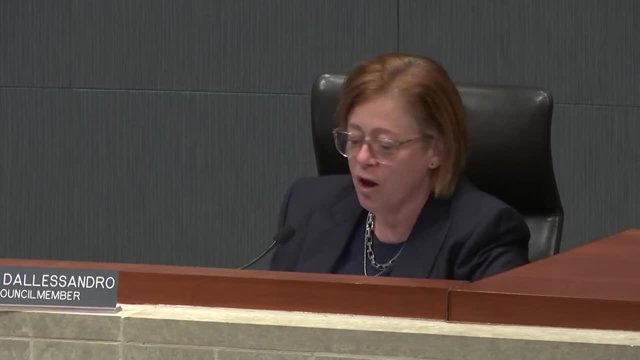 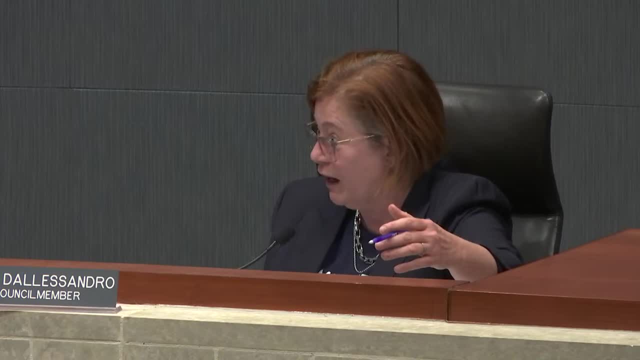 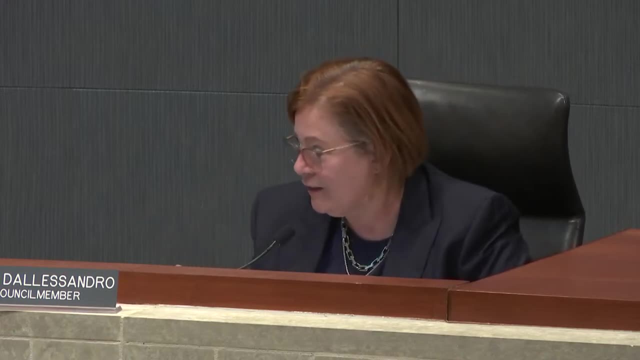 to a you know, a garbage bin, right a dumpster, if I will, and throw that stuff in there and walk back. She's not escorted, She's not under lighting. that specific, She's not anything. I'm not sure we. 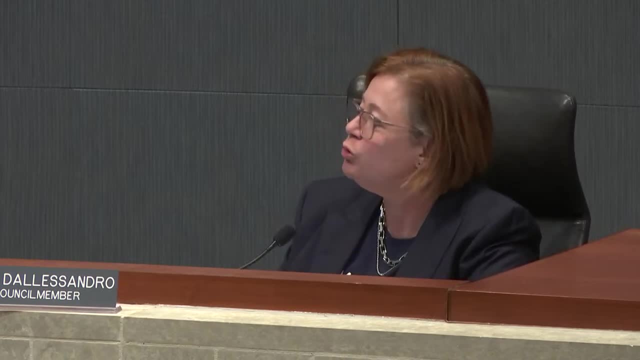 have the safety problem that we think we have. At the end of the day, this unduly burdens people who want to open restaurants. Bars- they don't have to do this. Hotels- they don't have to do this. People who get food served to them, like by delivery vans or food trucks, for example. 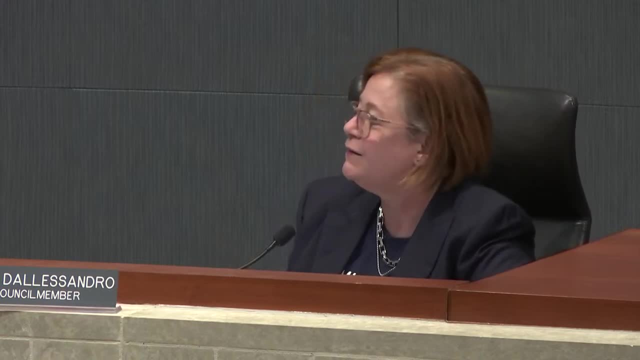 don't have to do this. We just specifically put the burden on a restaurant, and it doesn't make any sense to me, not to mention the fact that I can prove to you on three separate occasions, including the problems that Europolis is having by asking them to build out for this thing, when 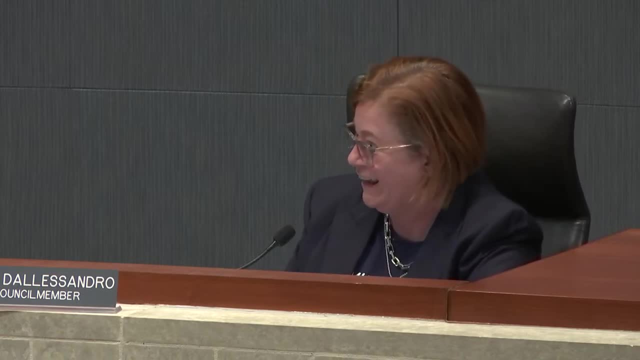 he probably could be done by now if we just let him do his thing. The good folks that own our Indian Street Kitchen had to go to a diner to find a place to make their restaurant. They're Bloomington residents. They went to a diner to find their opening because we made it so burdensome to them, because they were going to take a facility that wasn't already a restaurant, with all of our bells and whistles and our 10,000-gallon grease interceptors and all the other crap, and they were going to turn it into one, and so we just made it really really, really hard, and so they said: screw it, I'm going to a. 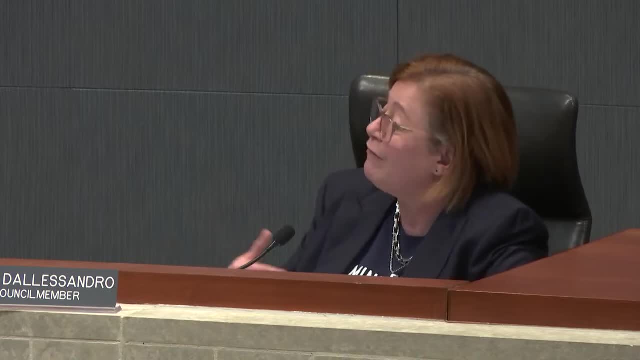 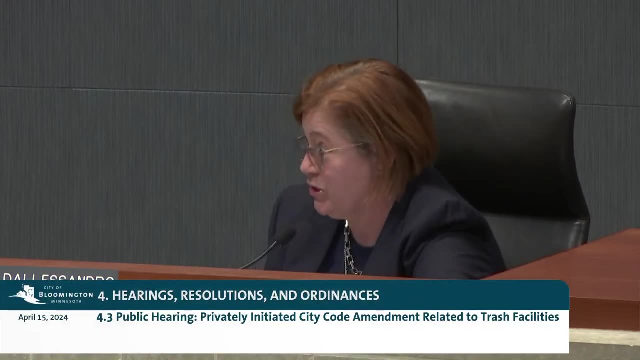 diner. We just need to stop doing this. That's what I'm trying to say. Having said that, thanks for my soapbox moment. having said that, if this is a step in the right direction, I'm 100% in favor of this. I would actually like to see us amend this code fully to give restaurant. 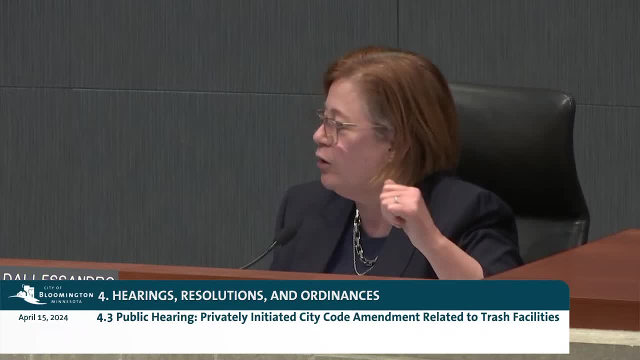 entrepreneurs. how many of them did we hear today? I think I heard at least one of our CEOs has a restaurant right. Good luck getting it done in here, unless you find a restaurant. I mean the folks at Momo's, for example. they were lucky. A place opened up next to. 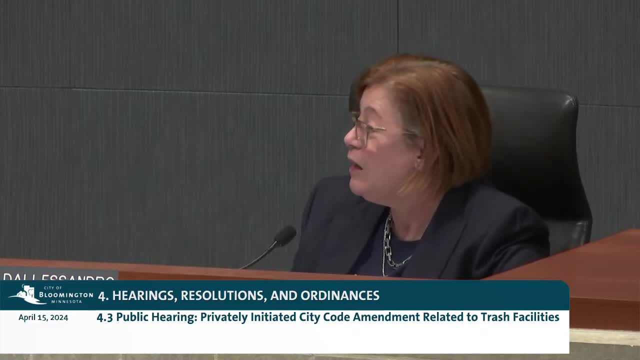 North Star. that was already a restaurant, so they didn't have to go through all this. but the folks that you know didn't find that place. they're somewhere else because we make it so impossible. so I love the attention to detail that we have, but I think it's oftentimes 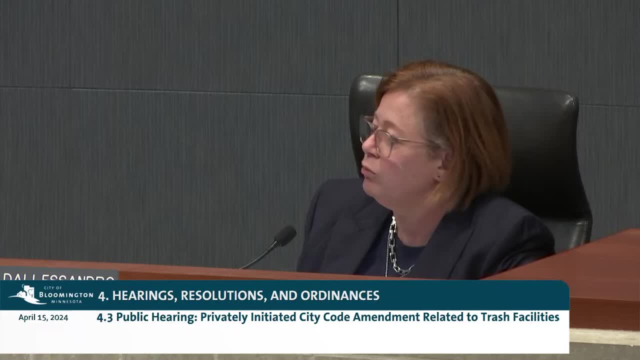 overly burdensome and if we're trying to spur, you know like good activity- I think of 90th and Penn and how we have some great restaurants in there like Kenny's Roast Beef and KOTU and everything like that- If any other space in that place wanted to become. 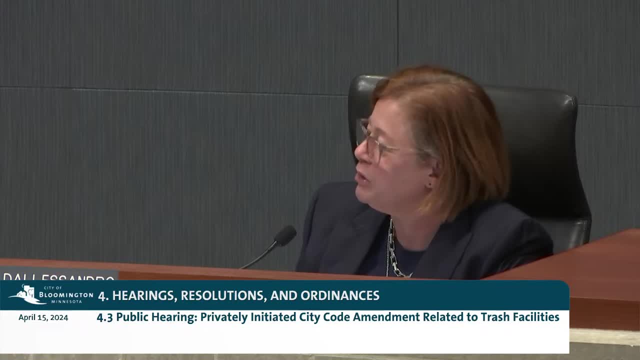 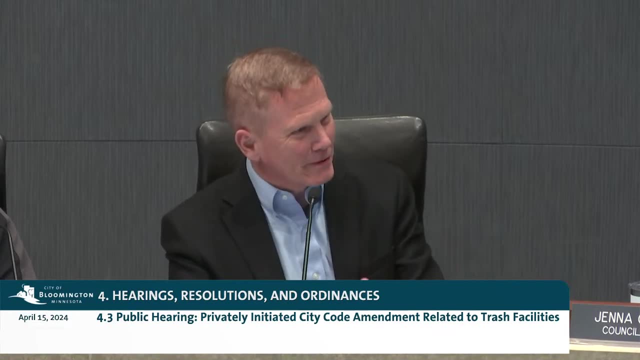 a restaurant, we would make it impossible, and that's just something we should probably do something about. Thanks, I appreciate your comments, Councilmember. I'll remind you that, as we do these public hearings, we like to stick to what we're talking. 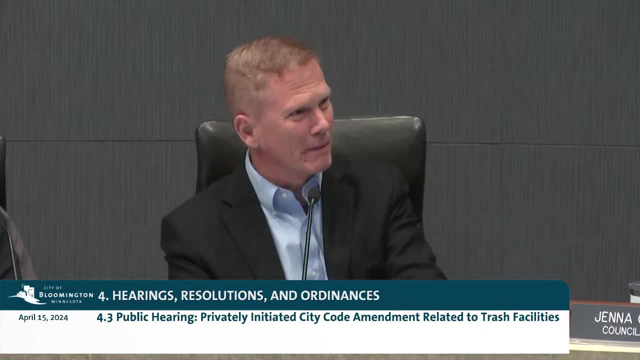 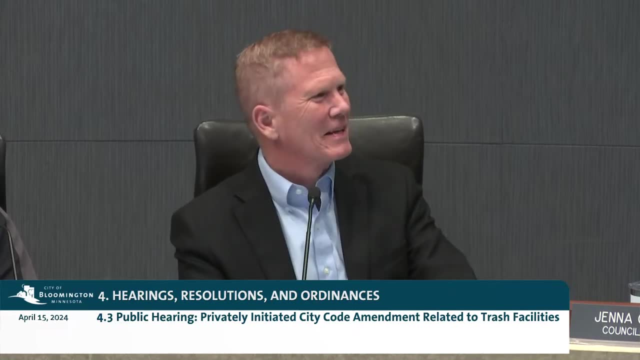 about to the topic on hand. What I heard you say was you were in support of this amendment for the reasons that you Exactly. Very good, Okay, Good to know. Thank you, Council. additional questions or comments on this? Councilmember Mua. 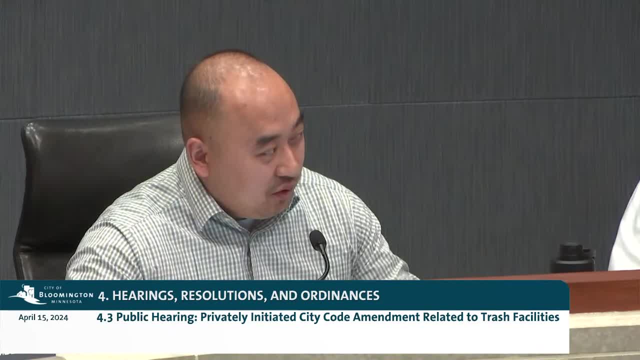 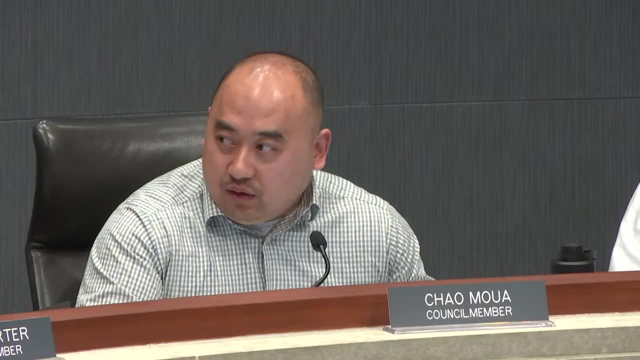 I would like to say thank you, Mayor. I agree wholeheartedly with what Councilmember D'Alessandro has spoken about. I think Nine Mile Brewery has proven that they're great neighbors within Bloomington. They've proven that the concept works in Bloomington. 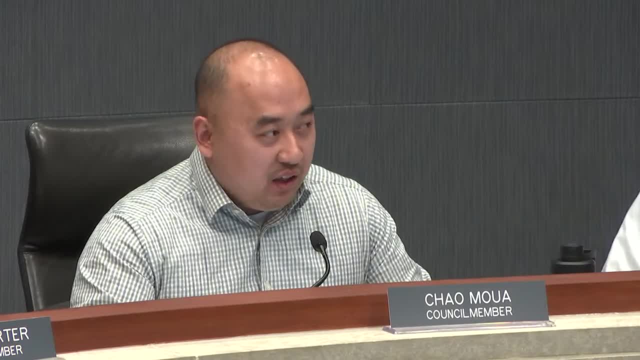 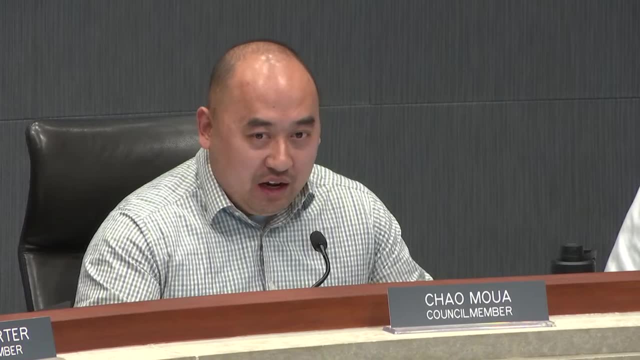 and expanding on this gives us the ability to prove again that Bloomington can have a robust not only brewery industry in Bloomington but a restaurant industry in Bloomington if we're able to get out of the way of small business owners, And so I am very much supportive. 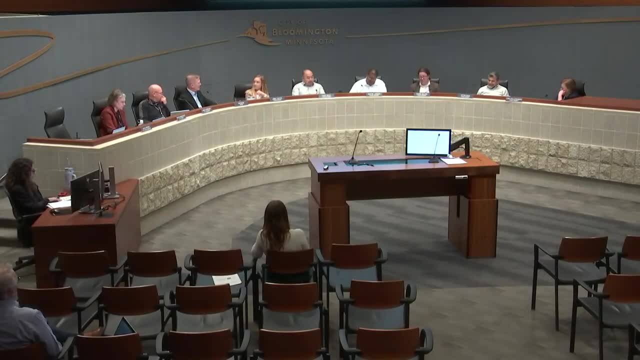 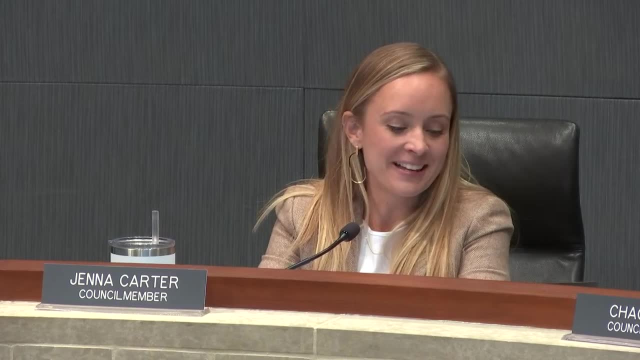 of this: Councilmember Kerner and Councilmember Lohman. Councilmember Kerner. Thank you, Mayor. I would just say I agree, I echo Lohna's sentiments and I will say I think, when I was reviewing the planning, commission meeting minutes. 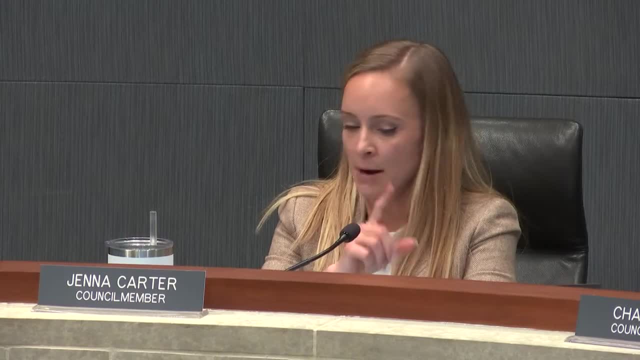 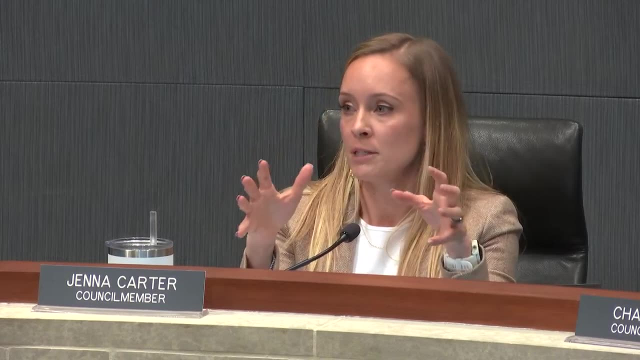 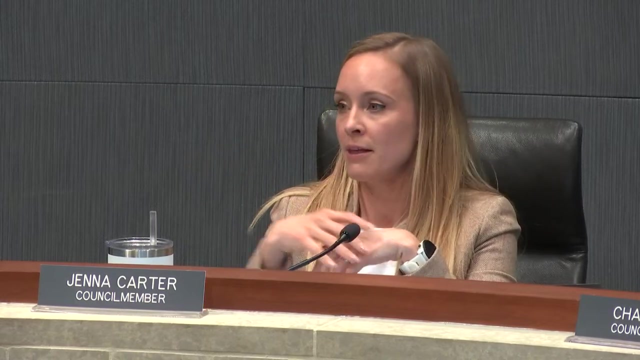 I do think I recall maybe staff making comments about considering this and other things, as we talk more broadly about making it easier to be a small business owner in Bloomington and specifically even a restaurant owner in Bloomington. So I would assume then that this will probably be considered again as part of that process. 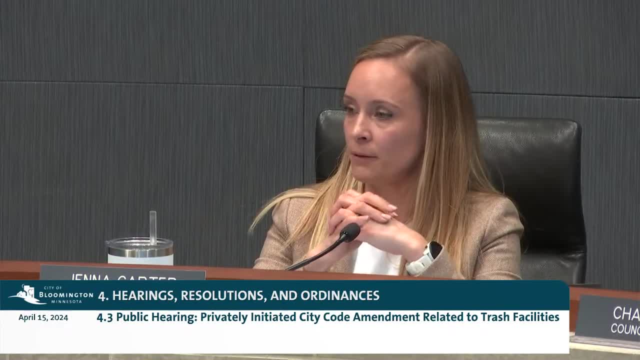 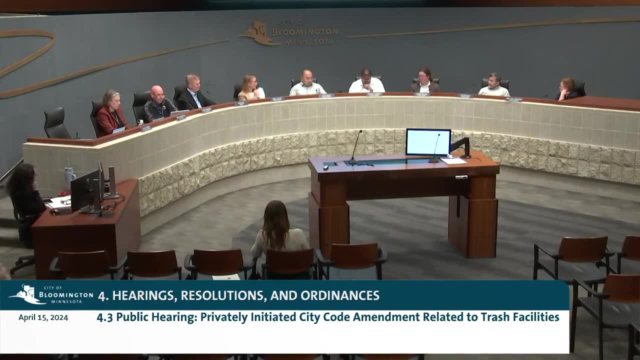 of looking at our codes and making things easier. Yeah, I'm seeing lots of head nods, So thank you. Yeah, I'm supportive, though, Council Member Lowman. Thank you, Mayor. I'm a part of an organization that is in the process. 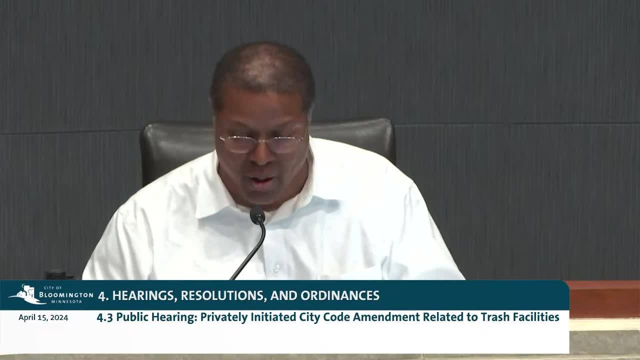 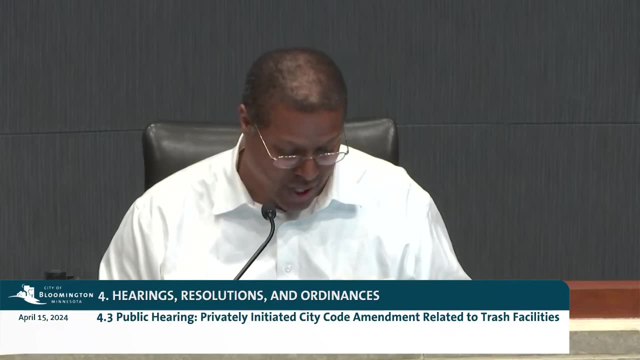 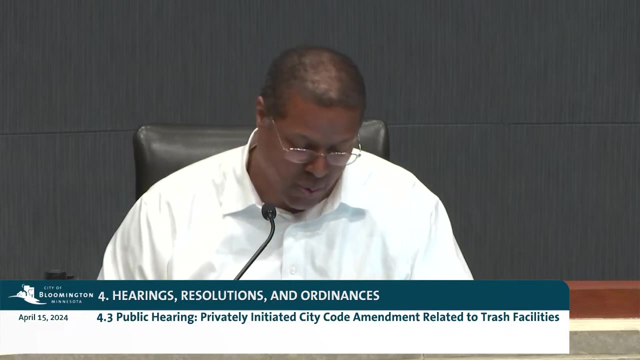 of attempting to do something at a Nine Mile Brewery And out of just a caution, I am going to abstain from this vote because I do not want to have any sense And I understand the strict standard of what a conflict of interest is, but I want to just be sure. 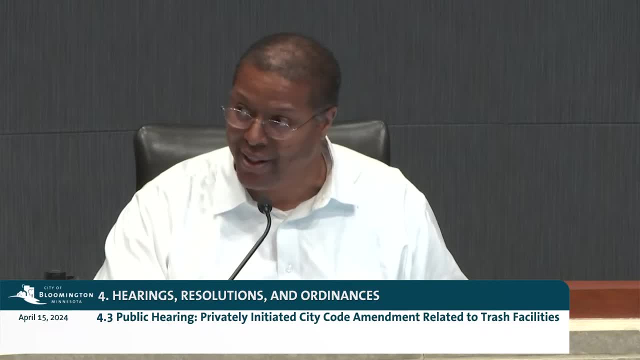 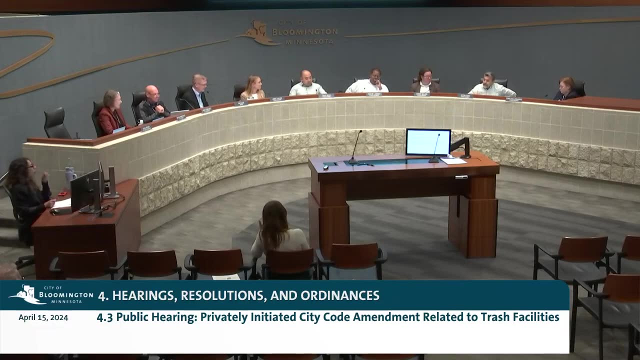 that I am being careful to not do anything in that manner, So I'll be abstained from this vote. I appreciate that. Council Member. Council Member Rivas. I just want to make it clear I have nothing against the facilitation for small businesses. 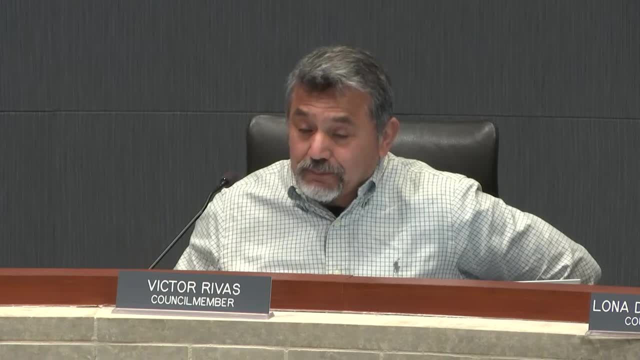 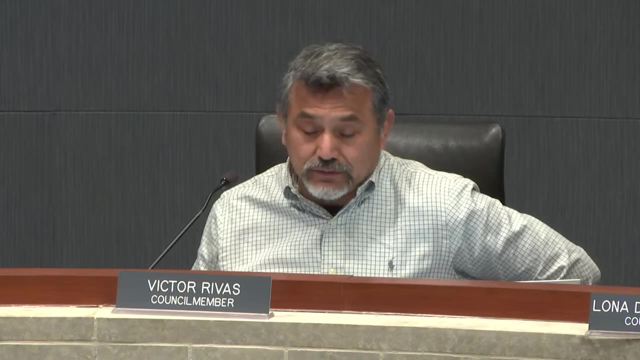 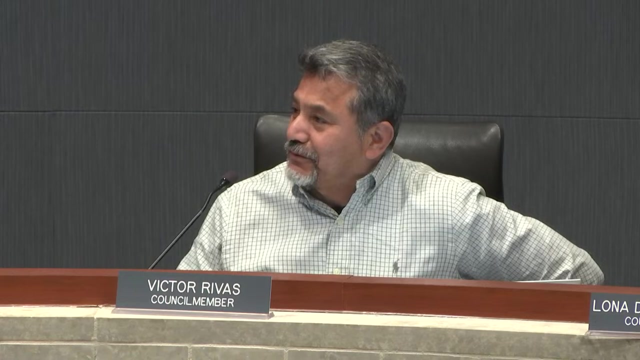 or restaurants in particular to open in Bloomington. However, If anybody here has any experience when it comes to restaurants or hotel kitchens, I can tell you with certainty that if Bloomington didn't have the standards that it has for grease traps and exhaust systems and all of that, 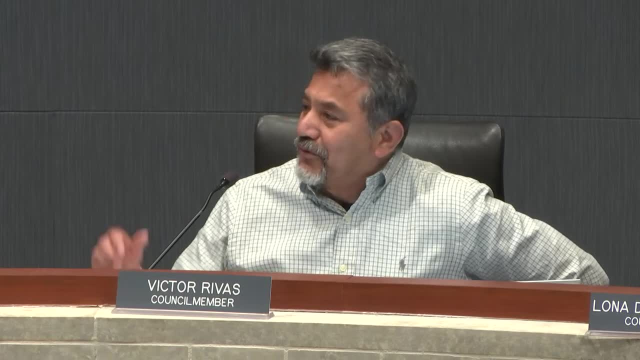 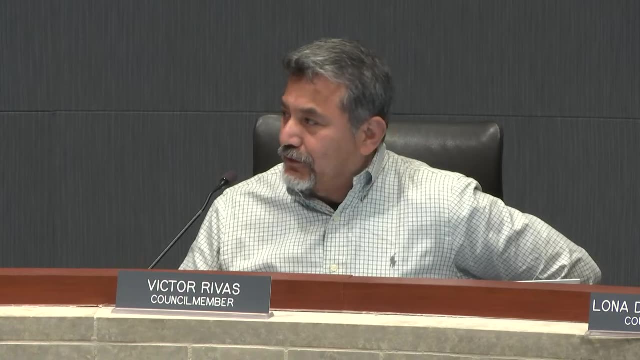 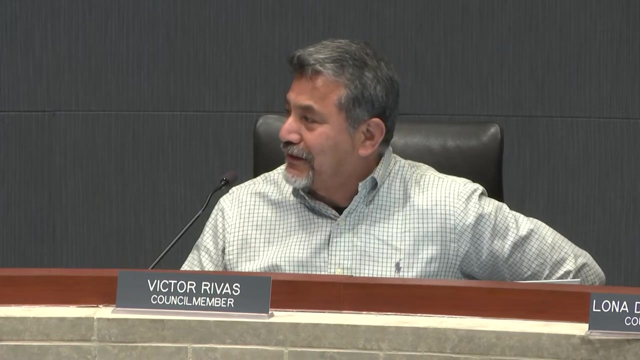 the potential hazard for fires and for the sewer systems to back up into large areas is there And I can tell you, if any of you has ever experienced a grease trap from a restaurant backing up, it's not pleasant at all And it's not only to the location. 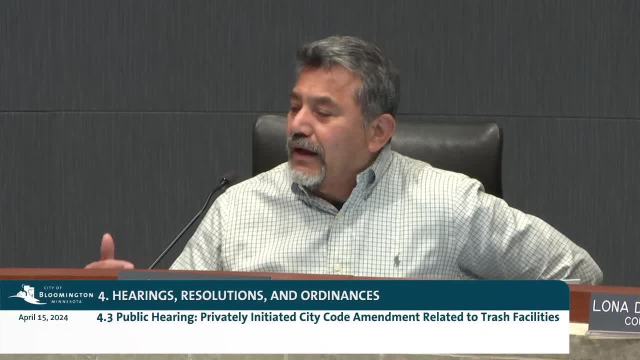 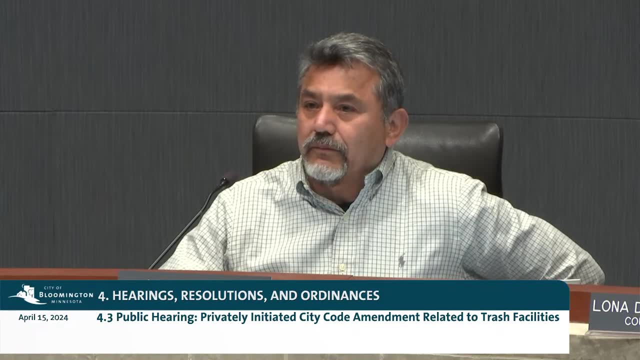 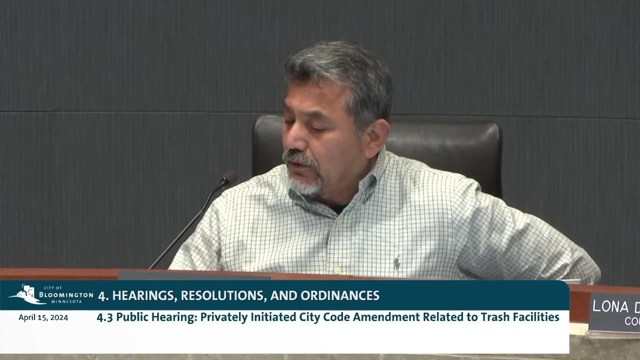 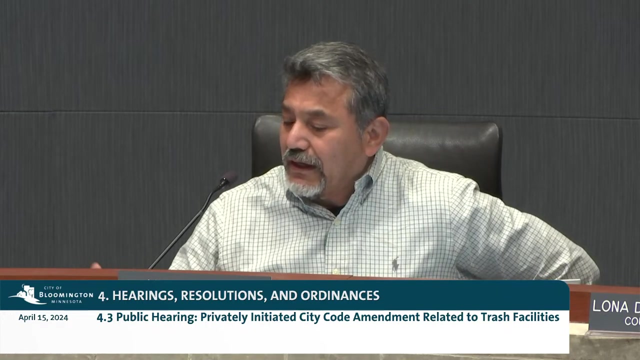 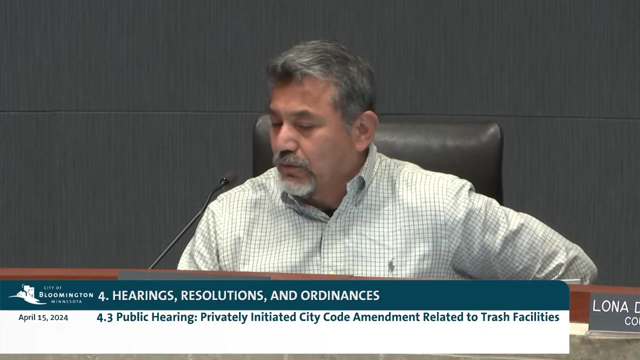 It can. it has large ramifications. That's why those standards are put in place. And to compromise those standards- just to, you know, alleviate the request from a particular entity, I don't think it's a feasible thing to do. Any thought that can be brought into this conversation is always welcome. 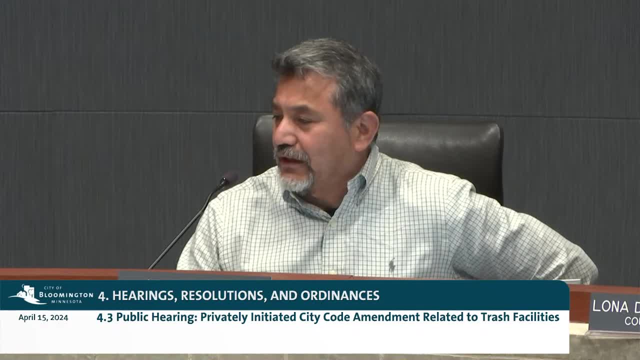 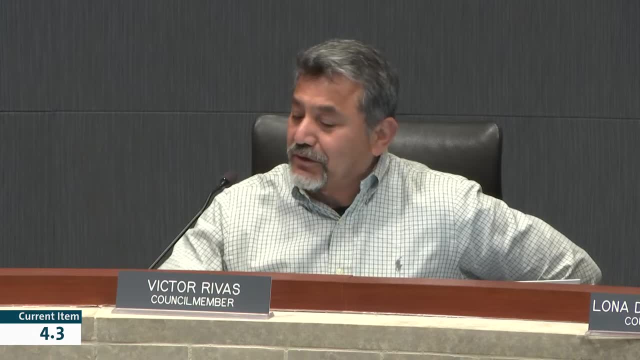 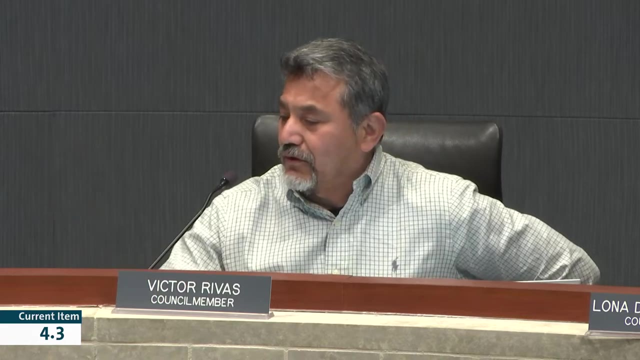 But I just say that because the standards that the city has put in place as old as they can be. they work Times have changed, but the repercussions of a grease trap or a potential contamination of any food production facility is always there. Thank you, 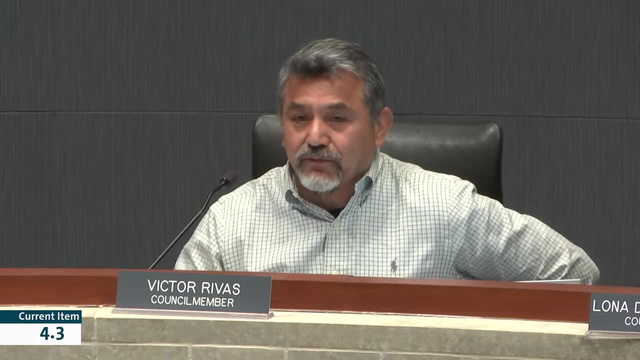 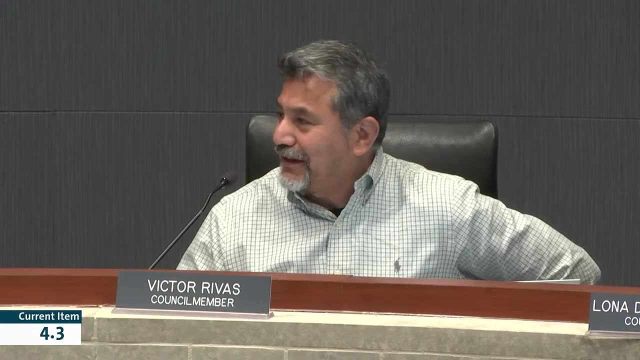 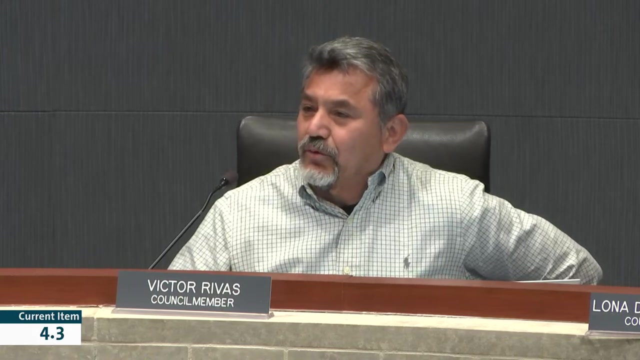 With that said, and I can tell you, for the last four years, working in hotels and the hospitality industry has put me in, has given me the ability to see accidents and things that took place, And that's why all those regulations are put in place. 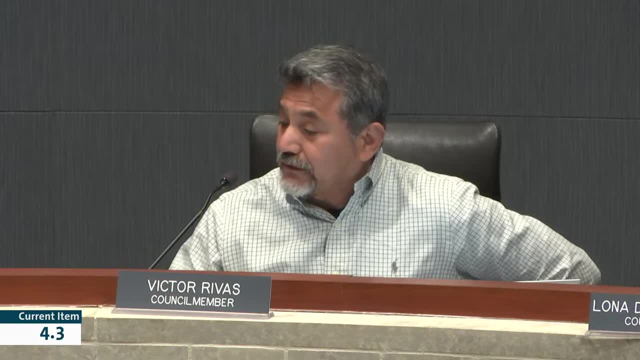 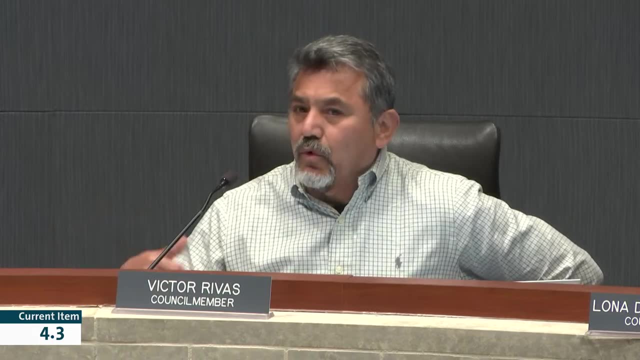 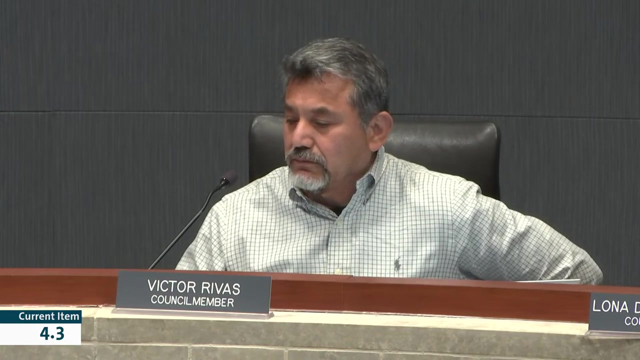 to avoid the problems that can be created. With that said, if the council is happy with passing these things, so please do it. I again: the more small businesses we have, the better off the city is, But at the same time, with caution, I will not support these myself. 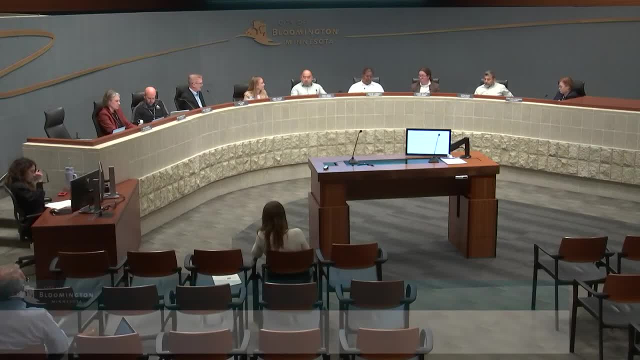 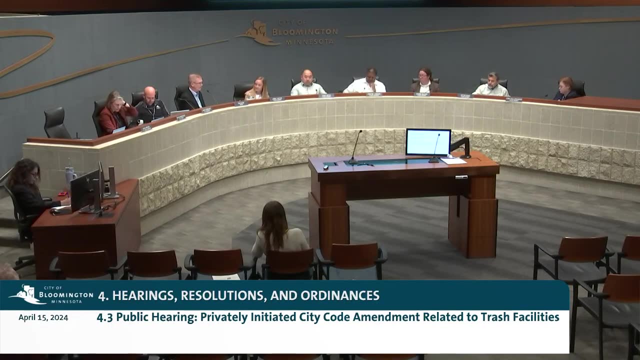 Thank you. council member. Council additional comments: Anything to bring forward? If not, I would look for action on this council. Council member D'Alessandro. Sure, I ought to put my mind to it. I'm going to put my mind to it. 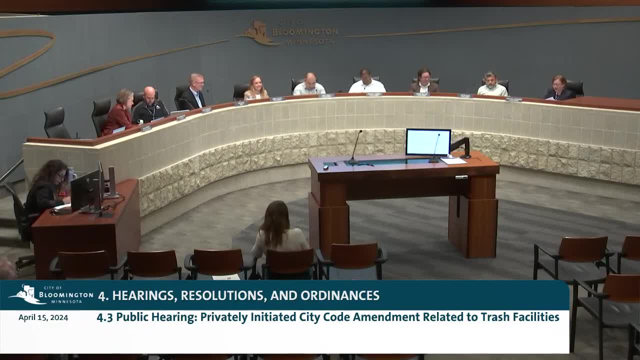 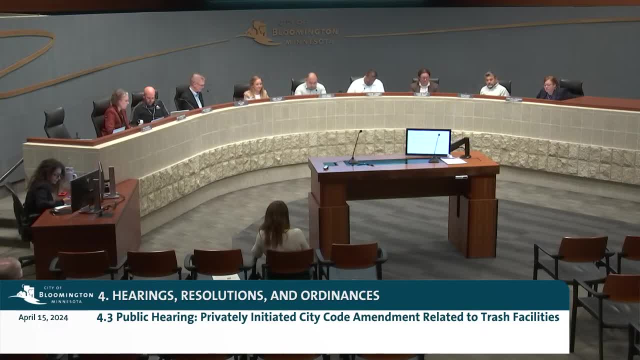 Oh, it's in my screen. Okay, I move to adopt ordinance that changes the standards relating to trash and recycling facilities for food service facilities located in industrial zoning districts, thereby amending chapter 21 of the city code. Second Motion by council member D'Alessandro. second by council member Mua, to adopt the ordinance changing standards related to trash and recycling facilities for food service facilities located in industrial zoning districts, amending chapter 21 of the city code. 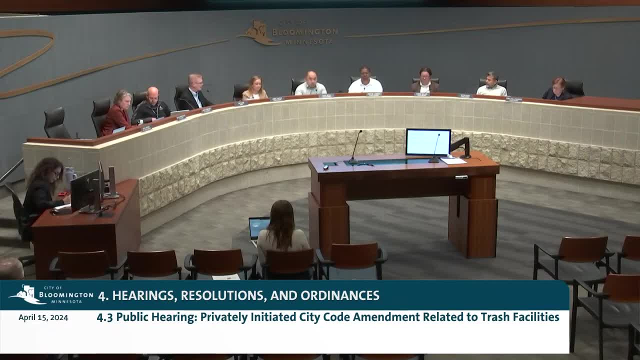 OF THE CITY CODE. ANY FURTHER COUNCIL DISCUSSION ON THIS HEARING NONE. ALL THOSE IN FAVOR, PLEASE SIGNIFY BY SAYING AYE, AYE, OPPOSED AND AN ABSTENTION BY. 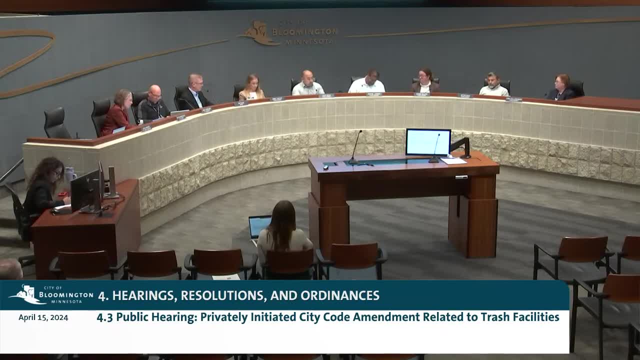 COUNCILMEMBER LOMAN, SO FIVE IN FAVOR. COUNCILMEMBER RIVAS, OPPOSED AND COUNCILMEMBER LOMAN: ABSTAINING FROM THAT, SO MOTION PASSES. 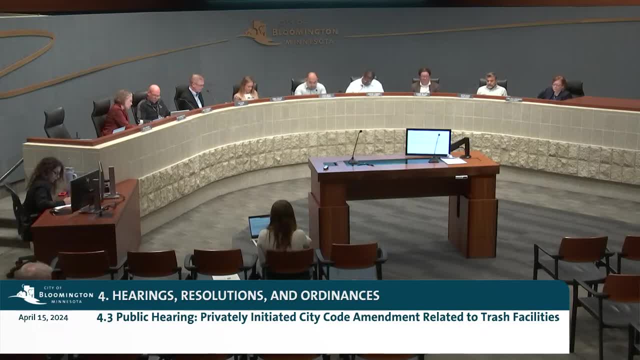 TIME FOR SUMMER PUBLIC AND COUNCILMEMBER DELISANDRO'S SUMMARY PUBLICATION. PLEASE, I MOVE RESOLUTION AUTHORIZING SUMMARY PUBLICATION OF THE ORDINANCE TO MODIFY STANDARDS RELATED TO TRASH AND. 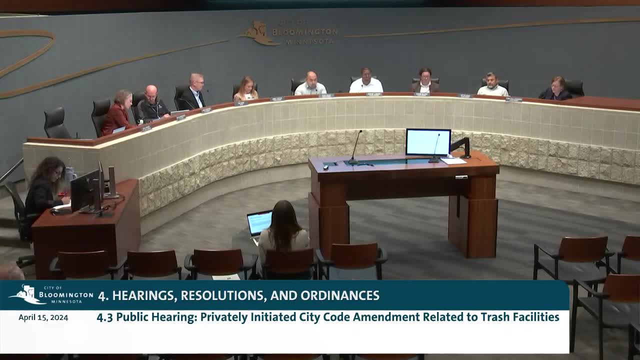 RECYCLING FACILITIES FOR CERTAIN FOOD SERVICE FACILITIES AND INDUSTRIAL ZONING DISTRICTS, THEREBY AMENDING CHAPTER 21 OF THE CITY CODE, MOTION BY COUNCILMEMBER DELISANDRO SECOND, BY. 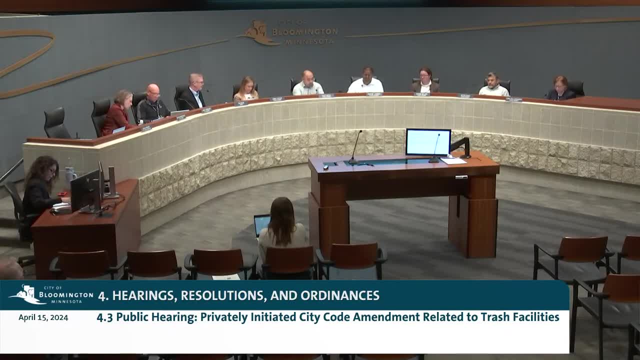 COUNCILMEMBER MUHA FOR SUMMARY PUBLICATION ON ITEM 4.3.. NO FURTHER COUNCIL DISCUSSION. ALL THOSE IN FAVOR. PLEASE SIGNIFY BY SAYING AYE, AYE. 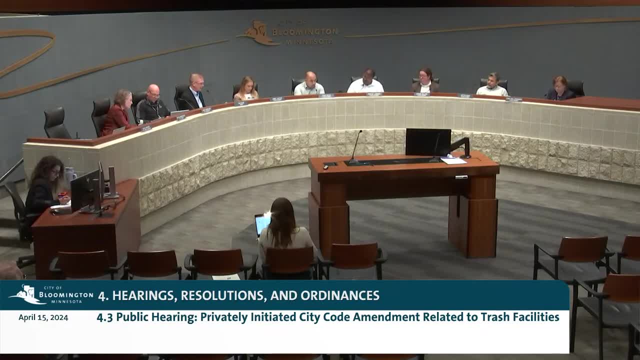 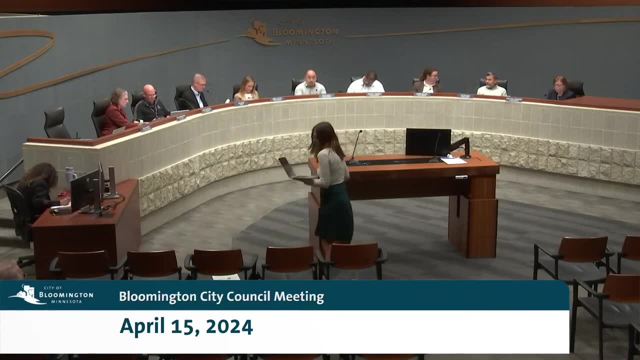 OPPOSED MOTION: CARRIES 6-1 WITH COUNCILMEMBER RIVAS OPPOSING SUMMARY PUBLICATION. THANK YOU VERY MUCH. AND, MR COUNTRYMAN, WHEN CAN WE EXPECT TO SEE PIZZA? 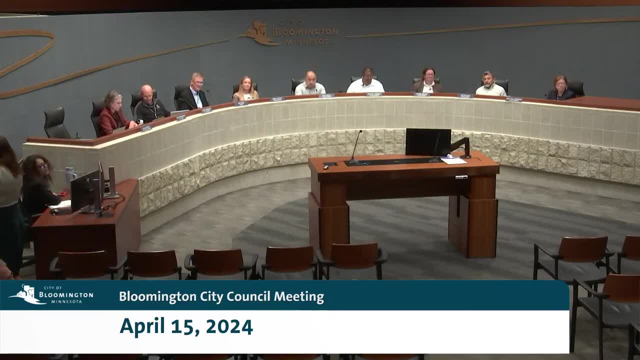 WE ARE HOPING THE FIRST WEEK OF JUNE WONDERFUL, BUT WITH CONSTRUCTION YOU NEVER KNOW. RIGHT, RIGHT, THANK YOU ALL, WELL, THANK YOU. THANKS FOR BEING HERE TONIGHT. ITEM 4.4 ON OUR AGENDA OUR. 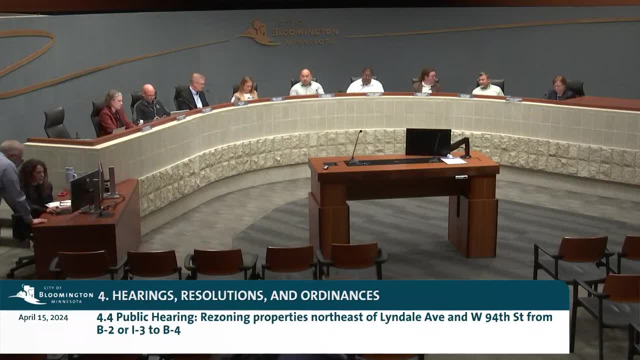 THIRD AND FINAL PUBLIC HEARING OF THE EVENING. THIS IS A PUBLIC HEARING REGARDING THE REZONING OF PROPERTIES NORTHWEST OF LYNDALE AVENUE AND WEST 94TH STREET, FROM B2 OR I3 TO B4.. 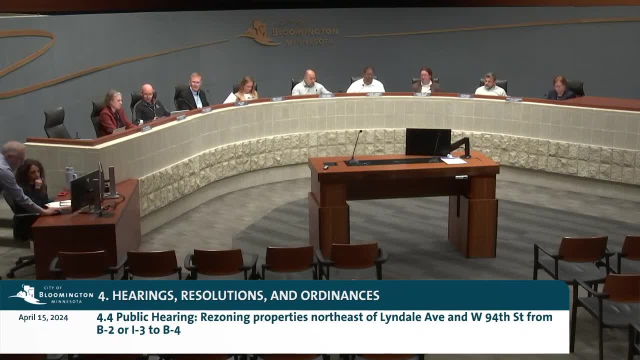 AND MR RAMLER-OLSON IS WITH US THIS EVENING, I THINK, YES, YES, I'M WITH YOU. CAN YOU HEAR ME? THERE YOU ARE. I DIDN'T SEE YOU IN THE BUILDING, BUT THERE YOU ARE. 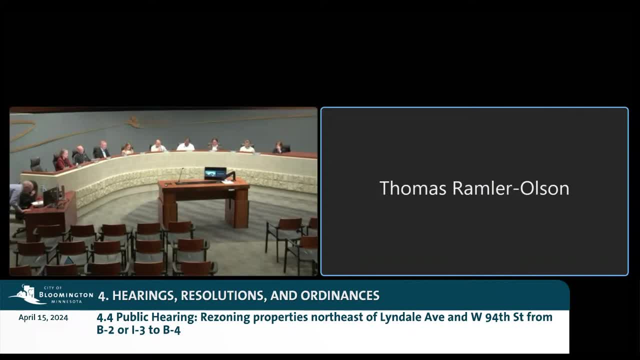 YES, WE CAN INDEED HEAR YOU. OKAY, I APOLOGIZE. I'M UNDER THE WEATHER AND I BELIEVE I'M ABLE TO PRESENT. HOPEFULLY, I'LL AVOID ANY POPPING FITS TO DELAY THIS. 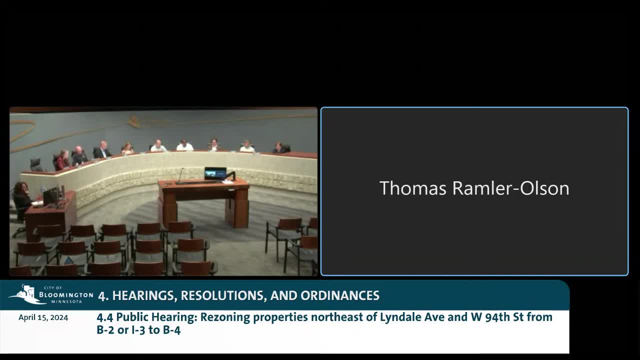 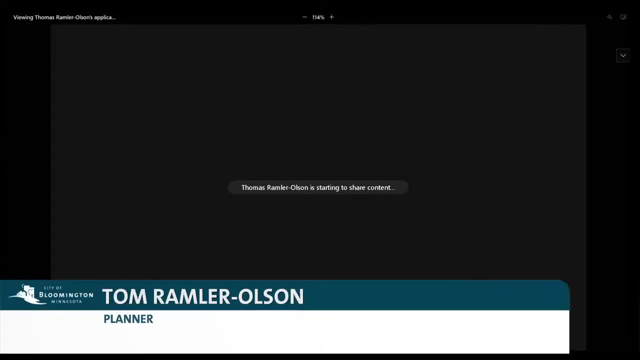 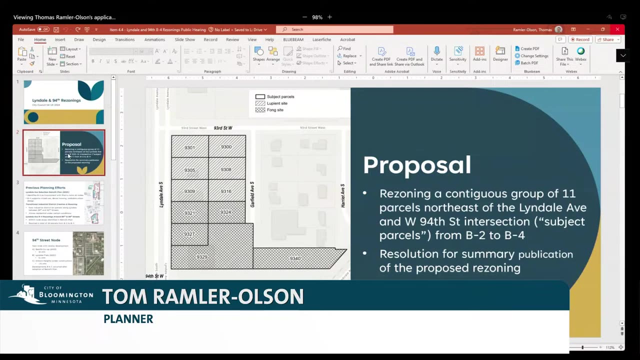 BECAUSE I KNOW IT'S A LATE NIGHT SO WE CAN JUST MOVE ON WITH IT. SO HERE I'LL SHARE MY SCREEN. CAN EVERYONE SEE IT? YES, WE CAN. OKAY, TERRIFIC. SORRY ABOUT THAT. 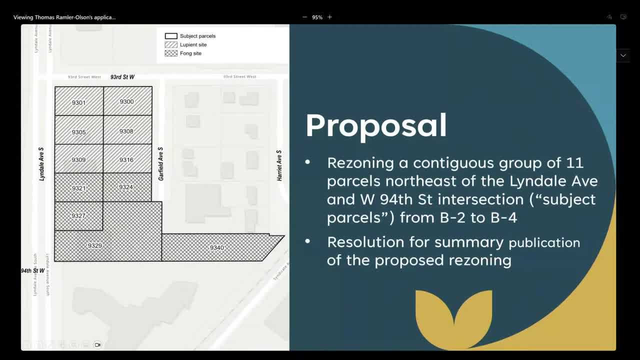 MR MERRICK, CAN I INTERRUPT REAL QUICKLY, TOM, CAN YOU? CAN YOU THERE? YOU GO NEVERMIND. JUST PUT IT INTO SLIDE MODE, PERFECT, OH, YES, YES, CERTAINLY. THANK YOU, JAMIE. 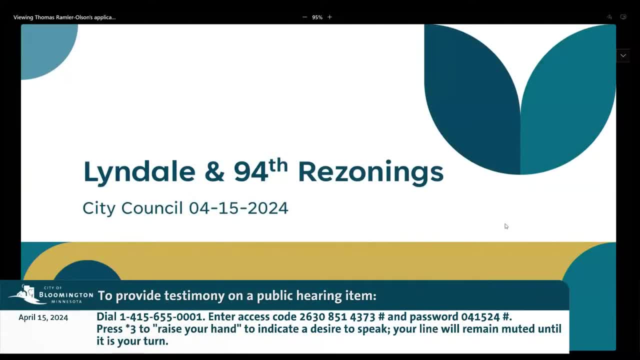 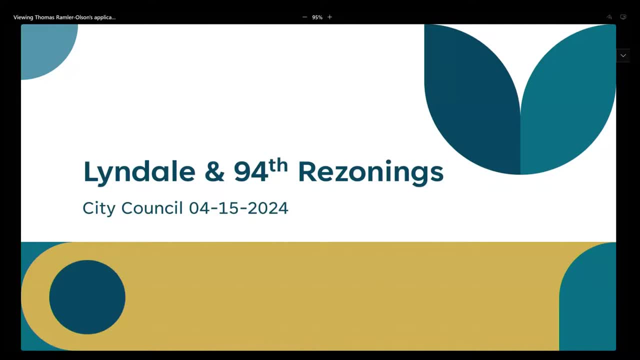 YES, OH, OH, OH, BOY, I'M SKIPPING AHEAD. I DON'T WANT TO GIVE AWAY THE GAME ALL RIGHT, SO YEAH. THE ITEM BEFORE YOU IS A PROZERY ZONING OF PROPERTIES. 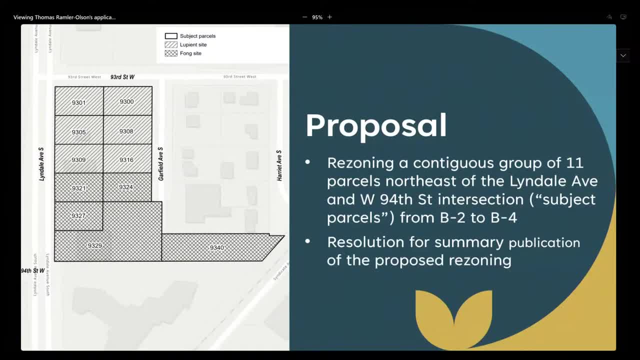 APPROXIMATELY 11.. A SLIGHT CORRECTION TO HOW IT WAS INTRODUCED: THESE PROPERTIES ARE NORTHEAST OF THE INTERSECTION OF 94TH AND LYNDALE, SO IT'S A GROUP OF 11 PARCELS. 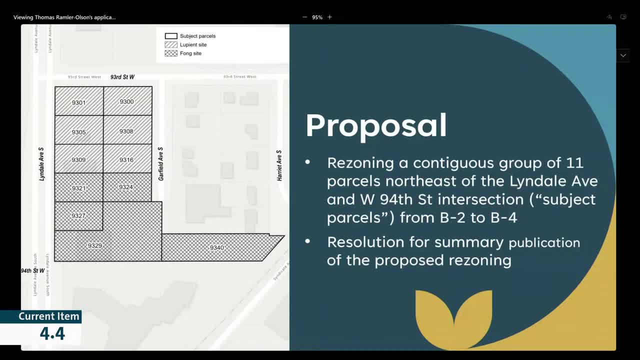 NORTHEAST OF THAT INTERSECTION AND IT'LL BE A REZONING FROM B2, I SHOULD SAY B2 OR I3, BECAUSE ONE OF THE PARCELS IS CURRENTLY ZONED I3. SO IT'S FROM B2 OR I3 TO B4.. 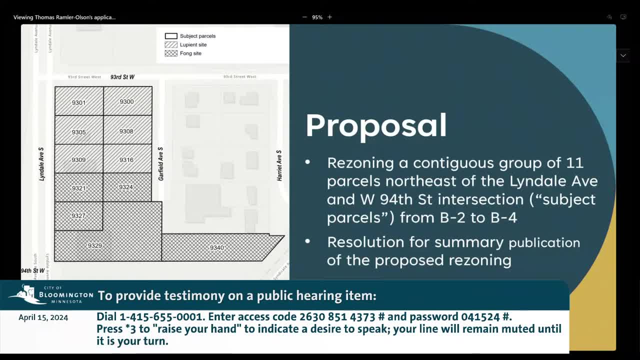 AND A SECOND PART OF THIS PROPOSAL IS A RESOLUTION DRAFTED FIRST. THAT WOULD BE SUMMARY PUBLICATION OF THE PROPOSED REZONING, SHOULD YOU CHOOSE TO ADOPT IT. OKAY, A LITTLE BIT OF CONTEXT. 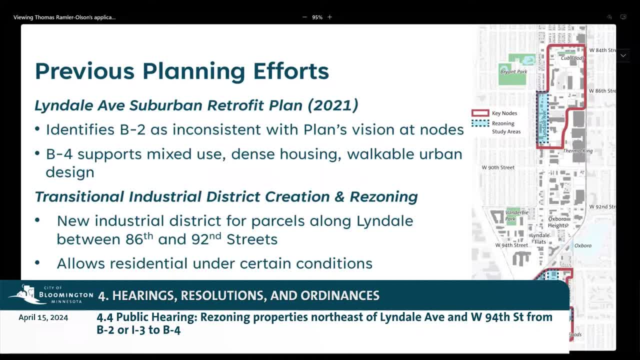 I'LL ZIP THROUGH THIS. THERE'S BEEN SOME PREVIOUS PLANNING EFFORTS THAT HAVE LED UP TO THIS POINT. THERE WAS THE LYNDALE AVENUE SUBURBAN RETROFIT PLAN, ADOPTED IN 2021.. 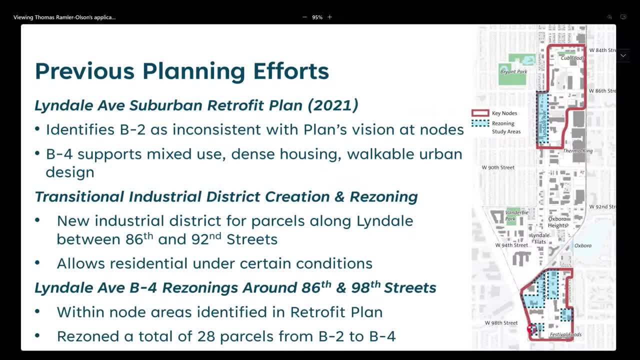 THIS IS KIND OF AN OUTGROWTH OF THAT. THE AREA IDENTIFIED NORTHEAST OF THIS INTERSECTION WAS NOT SPECIFICALLY IDENTIFIED IN THE PLAN ITSELF, BUT I'LL GET INTO WHY WE FEEL IT IS APPROPRIATE FOR THIS. 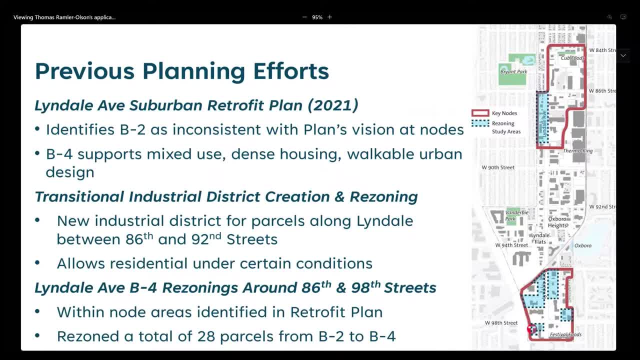 REZONING ACTION. FOLLOWING THAT IN 2021, WE HAD THE CREATION OF THE TRANSITIONAL INDUSTRIAL DISTRICT AND THE REZONING OF A GROUP OF 28 PARCELS ON THE EAST SIDE OF. 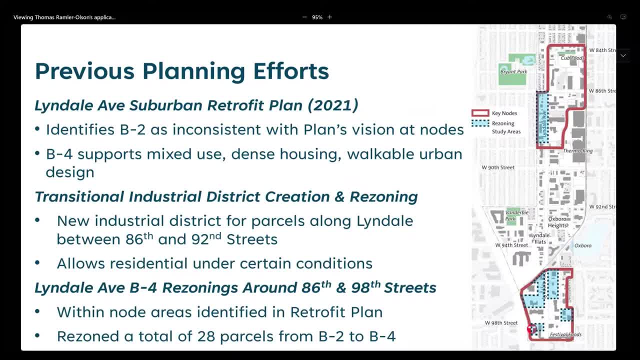 LYNDALE. THAT WAS A DIRECT ACTION DESCRIBED IN THE RETROFIT PLAN, AND THEN, AFTER THAT SEPTEMBER OF LAST YEAR, SO SEPTEMBER OF 2023,, THERE WERE A LOT OF PARTICIPATION. 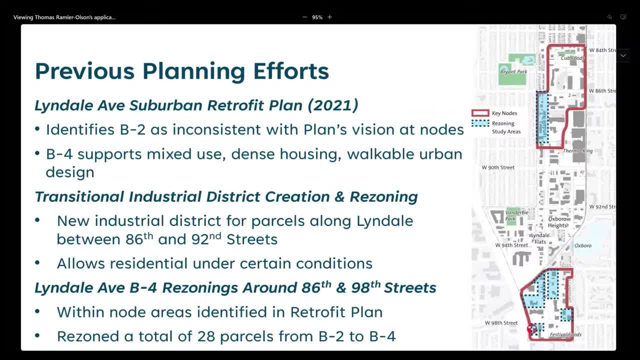 THERE WERE ANOTHER SET OF REZONINGS, THIS TIME PARCELS AROUND LYNDALE AVENUE, INTERSECTIONS WITH 86th AND 98th STREET. ALL THOSE PARCELS IDENTIFIED WERE B2 AND THEY WERE APPROVED. 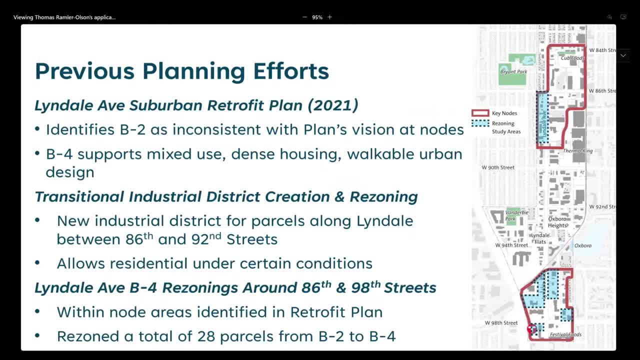 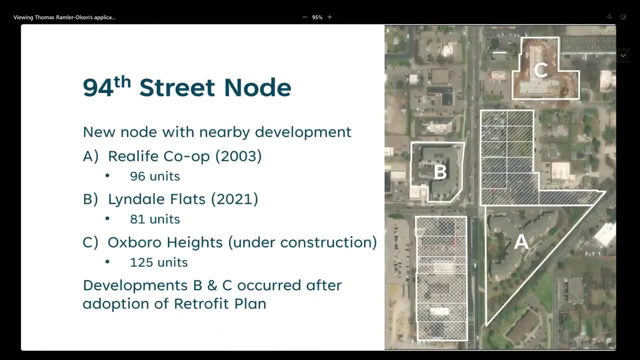 FOR REZONING FROM B2 TO B4.. AND THAT WAS AGAIN IN SEPTEMBER 18TH OF 2023.. SO I JUST MENTIONED THAT THIS NODE OR THIS INTERSECTION WASN'T SPECIFICALLY CALLED OUT. 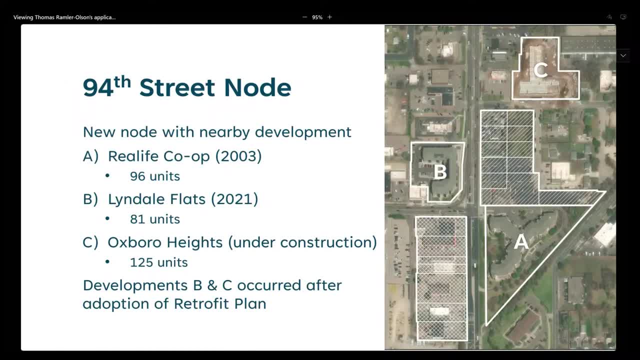 IN THE RETROFIT PLAN, BUT IT'S ORGANICALLY SHAPING TO BE A NODE, AS WAS IDENTIFIED AT 86th AND 98th STREETS. THERE'S ALREADY BEEN A LOT OF DEVELOPMENTS AT THIS INTERSECTION. 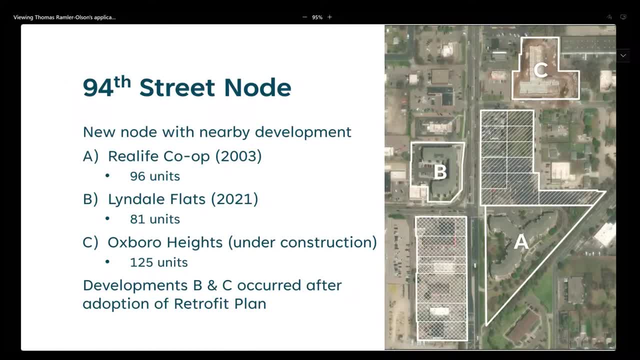 IN 2003,. THERE WAS THE REAL LIFE CO-OP- THAT ADDED 96 UNITS. SENIOR LIVING AND, JUST IN 2021, IS LYNDALE FLATS. THAT'S THE POLYGON IDENTIFIED AS B: THAT WAS 81 UNITS. 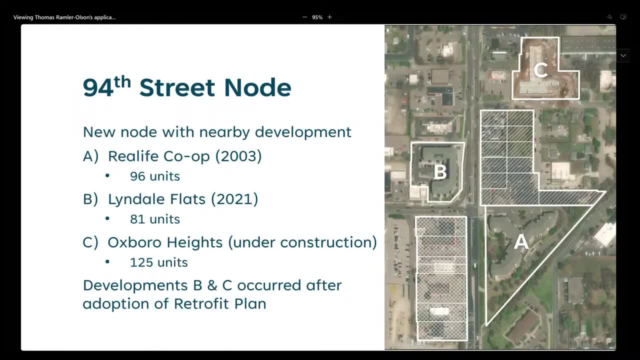 AND UNDER CONSTRUCTION STILL IS OXBOROUGH HEIGHTS, WHICH WILL ADD 125 UNITS. SO THE DEVELOPMENTS OF LYNDALE FLATS AND OXBOROUGH HEIGHTS WERE ALL AFTER THE RETROFIT PLAN. SO THIS IS REALLY A JUST KIND OF. 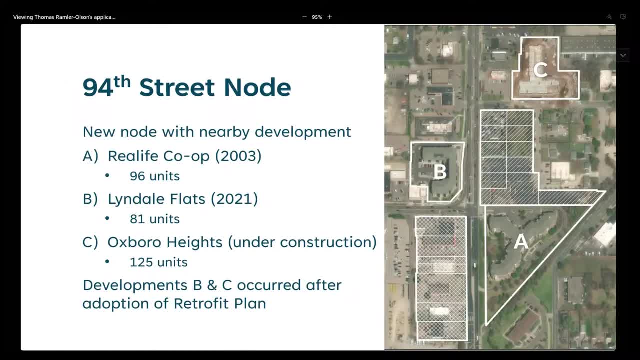 AN ORGANIC EVOLUTION OF THIS NODE FROM WHAT IT WAS TO SOMETHING THAT HAS MORE ACTIVITY BECAUSE OF THE ADDED HOUSING UNITS, AND WE FEEL THAT IT THEREFORE QUALIFIES AS THE CREATION OF. 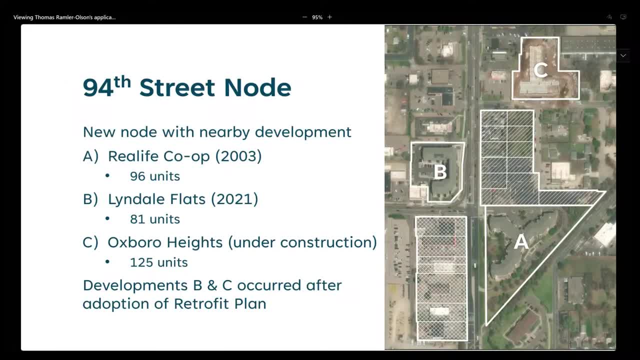 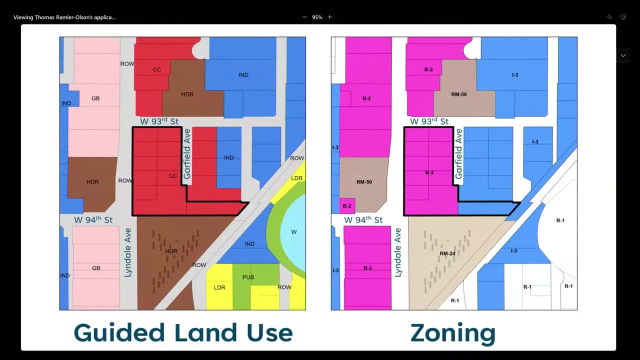 ANOTHER, OR WE'RE SUPPORTING THE CREATION OF THIS NODE BY PROPOSING THESE ADDITIONAL REZONINGS AT THE NORTHEAST OF NORTHEAST OF THIS INTERSECTION. HERE IS A LOOK AT THE GUIDED LAND. USE AROUND THE PROPOSED OR. 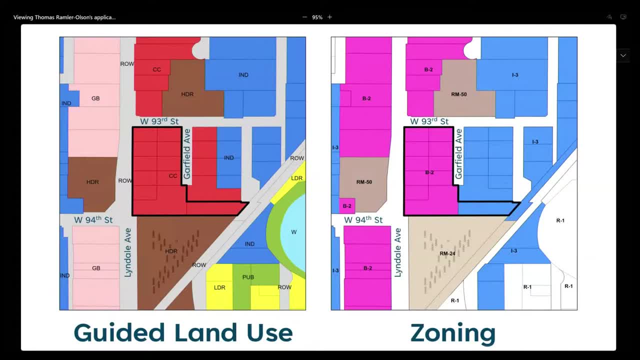 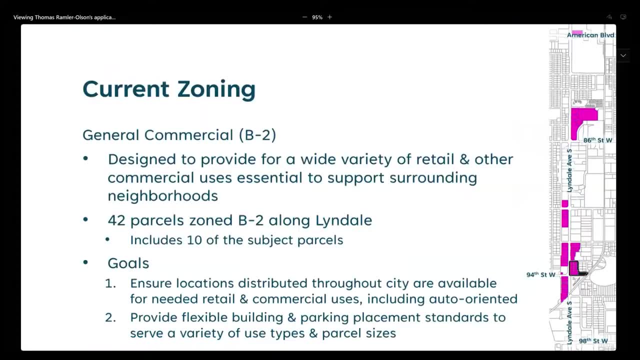 THE IDENTIFIED PARCELS PROPOSED FOR REZONING AND THE ZONING ITSELF. SO THE CURRENT ZONING IS B2.. THERE ARE 42 PARTICULAR PARCELS, INCLUDING TEN OF THE SUBJECT PARCELS THAT ARE STILL. 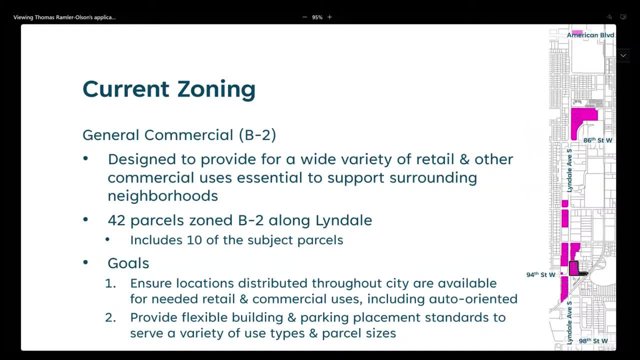 ZONED B2.. SO, EVEN WITH THIS REZONING, THERE WOULD STILL BE A PRETTY GOOD AMOUNT OF PARCELS THAT WOULD RETAIN THE ZONING OF B2.. SO THAT WOULDN'T REMOVE ANYTHING. 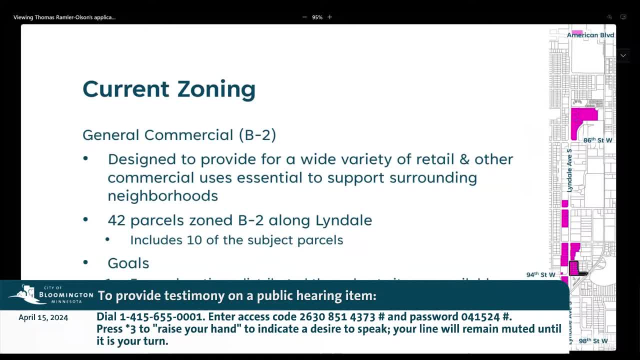 FROM THOSE PARCELS. IT WAS EVEN DISCUSSED DURING THE CREATION OF THE RETROFIT PLAN THAT SOME AMOUNT OF B2 PARCELS WAS APPROPRIATE, GIVEN THE SERVICES THEY PROVIDE: CARWASH, GAS STATION, THOSE TYPES OF. 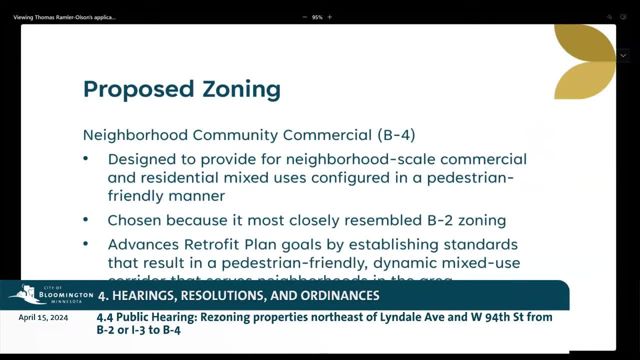 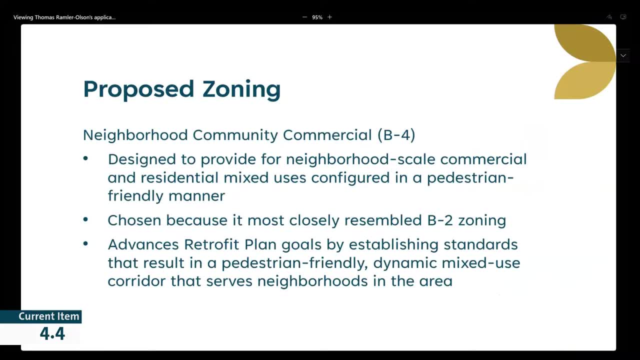 USES AND THE PROPOSED ZONING IS B4, FOR TEN OF THOSE PARCELS. AGAIN, ONE IS CURRENTLY ZONED I3. AND B4, WAS YOU KNOW. IT'S DESIGNED TO PROVIDE FOR A. 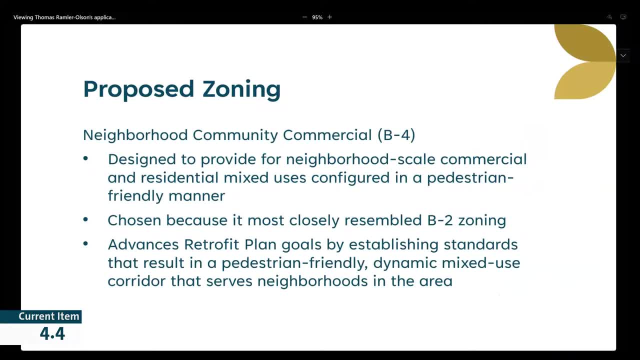 NEIGHBORHOOD SCALE, COMMERCIAL, RESIDENTIAL MIXED USE. IT'S MORE PEDESTRIAN FRIENDLY. THAT'S WHY IT WAS HIGHLIGHTED IN THE RETROFIT PLAN ITSELF AND IT WAS ALSO CHOSEN AS A 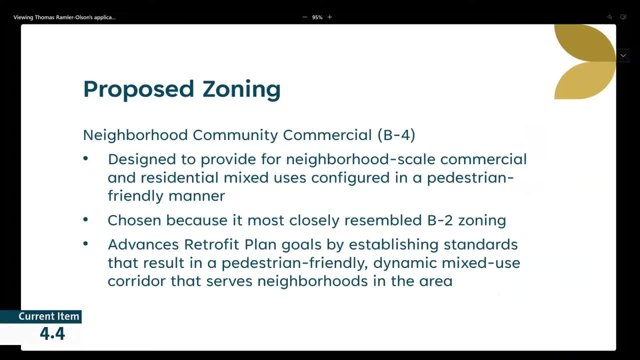 SUITABLE REPLACEMENT FOR B2, BECAUSE IT CLOSELY RESEMBLED THE B2 DISTRICT AND SO IT ADVANCES. THE RETROFIT PLAN GOALS WHILE, ALSO NOT UPSETTING TOO MANY OF THE ESTABLISHED BUSINESSES IN THE 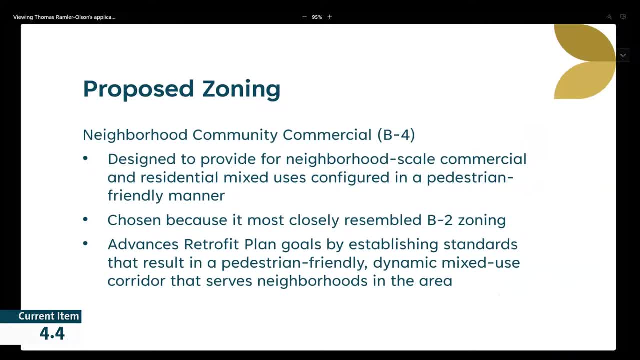 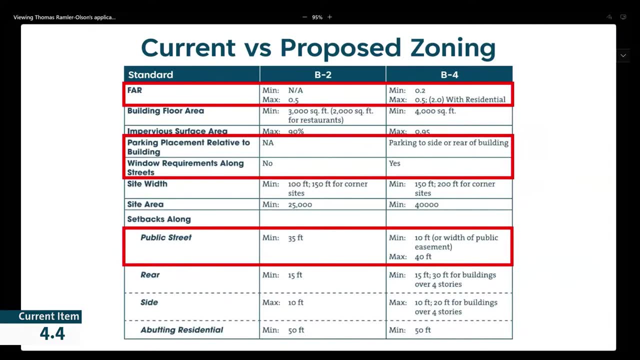 CORRIDOR BECAUSE OF THE SIMILARITIES BETWEEN B2 AND B4.. BUT THERE ARE NOTICEABLE DIFFERENCES. THOSE INCLUDE A HIGHER FLOOR AREA. RATIO: IF RESIDENTIAL IS INCLUDED IN DEVELOPMENT, THE PLACEMENT OF PARKING ON THE 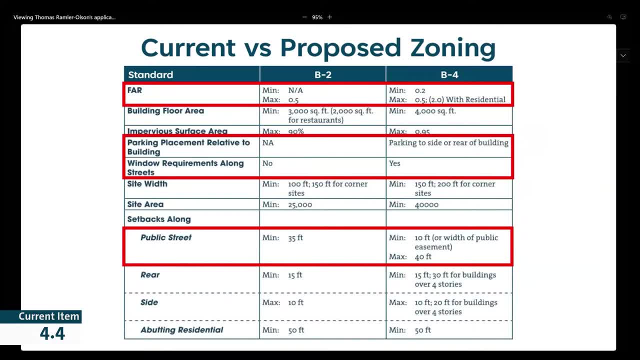 SIDE OR REAR, A GOOD AMOUNT OF GLAZING ALONG THE SIDEWALK OR STREET FRONT AND THE SHALLOWER SETBACKS ALONG PUBLIC STREETS. SO AGAIN A MORE PEDESTRIAN, FRIENDLY TYPE OF URBAN FORM. 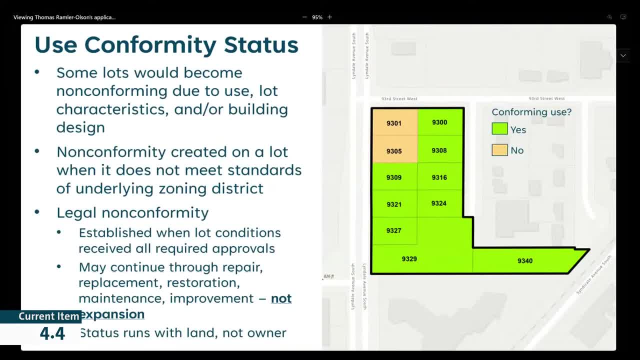 ALONG LYNNDALE USE. CONFORMITY IS ALWAYS A CHALLENGE WITH SOME OF THESE PROPOSED REZONINGS. FORTUNATELY, THERE ARE ONLY A COUPLE OF LOTS THAT WOULD HAVE A LEGAL, NONCONFORMING USE ON IT. 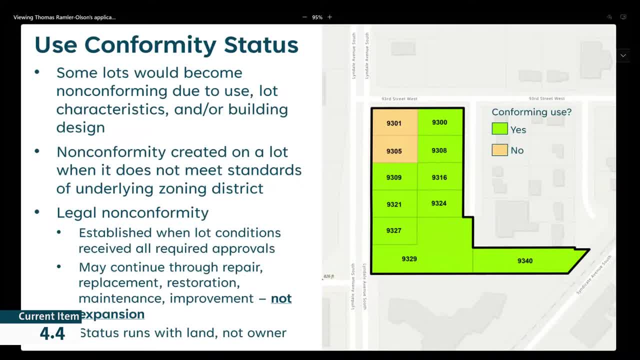 SHOULD THE REZONING BE APPROVED AND THEY COULD CONTINUE THAT WAY IN PERPETUITY, UNLESS THERE WERE SOME THINGS, THERE ARE CERTAIN TRIGGERS WHERE IT HAS TO BE BROUGHT INTO CONFORMANCE. 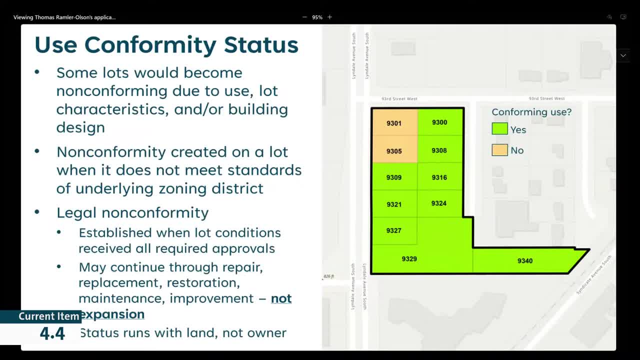 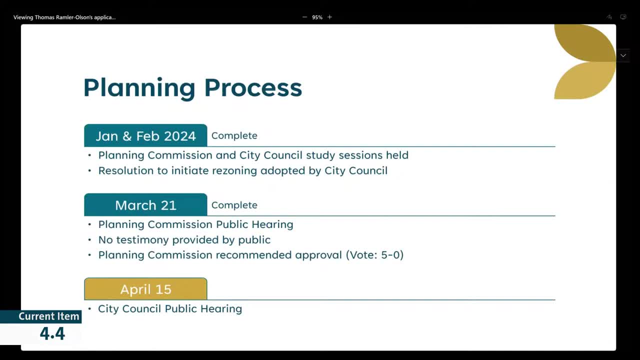 BUT NONETHELESS. THIS IS A PRETTY GOOD INDICATION OF THIS ACTION AND HOW IT AFFECTS EXISTING PROPERTIES. THE PLANNING PROCESS IS ITSELF. IT KICKED OFF LAST YEAR, BUT IN JANUARY, FEBRUARY, THIS 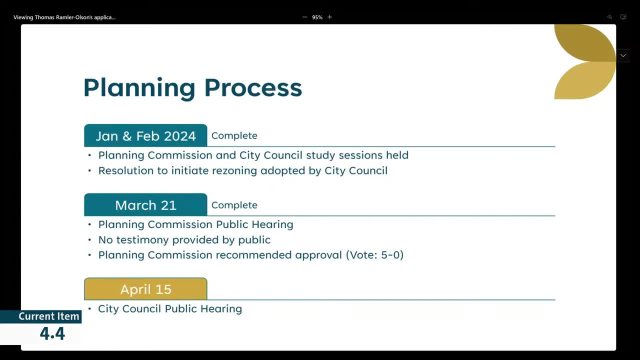 YEAR WE HAD SOME STUDY SESSIONS, IF YOU'LL RECALL, IN FEBRUARY, IN FRONT OF COUNCIL, AND IT WAS AT THAT FEBRUARY MEETING THAT THERE WAS A RESOLUTION TO INITIATE THE 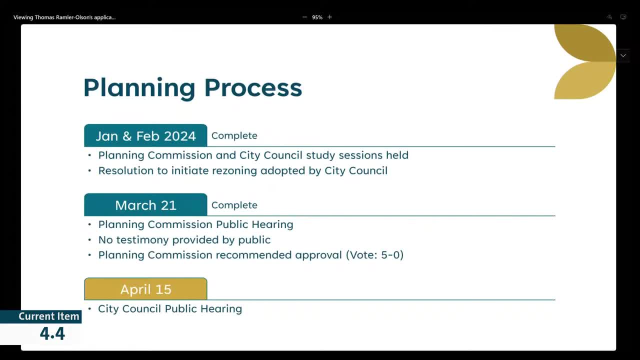 REZONING. THAT WAS ADOPTED BY COUNCIL. ON THE 21ST, WE HAD A PLANNING COMMISSION MEETING. I'LL TALK ABOUT THAT A LITTLE BIT LATER. THERE WAS NO TESTIMONY PROVIDED. 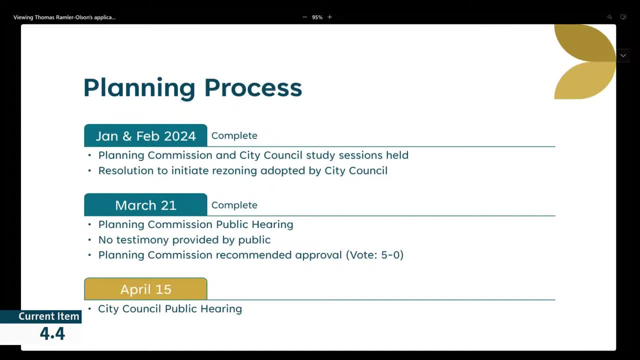 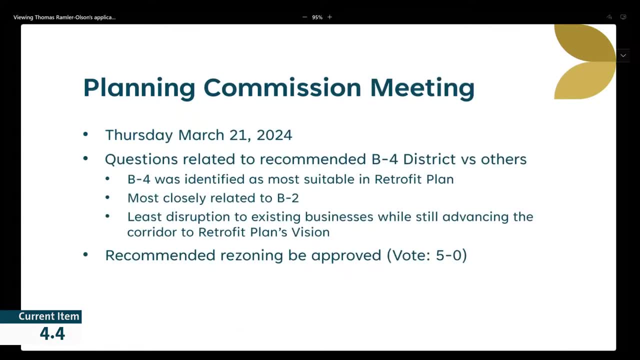 AT THAT MEETING AND, AS YOU CAN SEE, THE PLANNING COMMISSION DID RECOMMEND APPROVAL UNANIMOUSLY FIVE TO ZERO. AND AT THAT PLANNING COMMISSION MEETING THERE WERE SOME QUESTIONS RELATED TO WHY. B4 WAS. 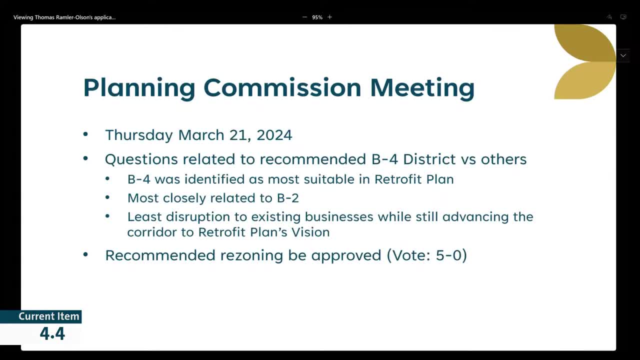 PREFERRED OVER OTHER. EXCUSE ME, SORRY MY APOLOGIES, WHY B4 WAS PREFERRED OVER OTHER ZONING DISTRICTS, OTHER COMMERCIAL RELATED ZONING DISTRICTS AND, AS I MENTIONED BEFORE. 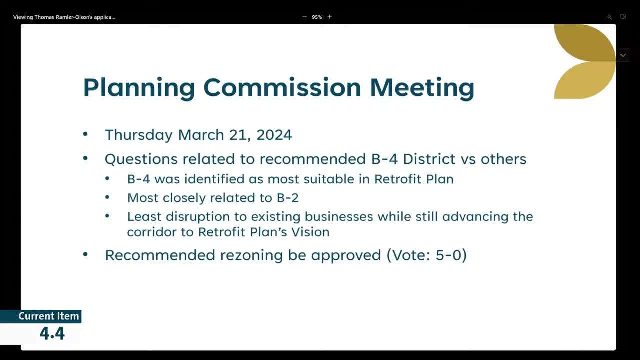 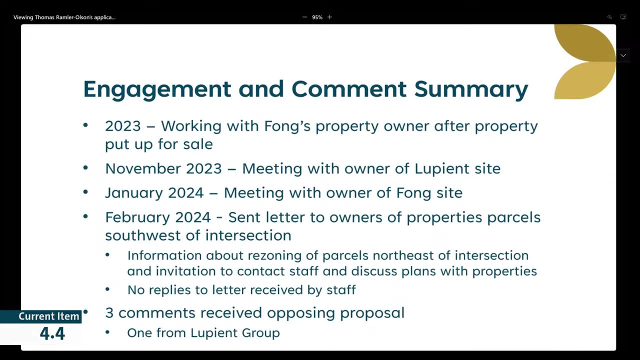 BECAUSE OF ITS RELATIONSHIP TO THE B2 DISTRICT AND HOW IT WOULDN'T BE AS DISRUPTIVE WHILE STILL ADVANCING THE GOALS OF THE RETROFIT PLAN. SO THERE WAS SOME ENGAGEMENT AS PART OF THIS PROJECT. 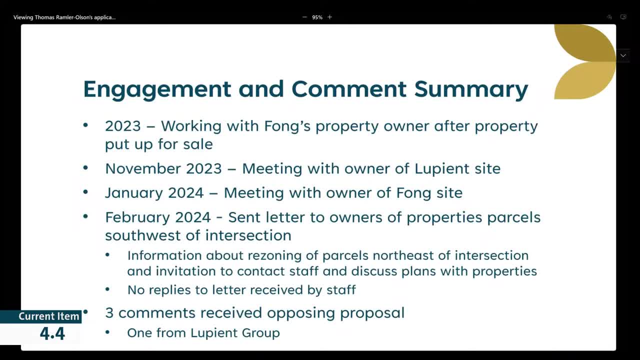 THERE WERE TWO OWNERSHIP GROUPS: THE LUPEAN GROUP, THAT OWNED THE SIX PARCELS, AND PHONGS, WHICH OWNED THE SOUTH FIVE PARCELS. WE REACHED OUT TO BOTH OWNERS AND WE HAD MEETINGS WITH THEM. 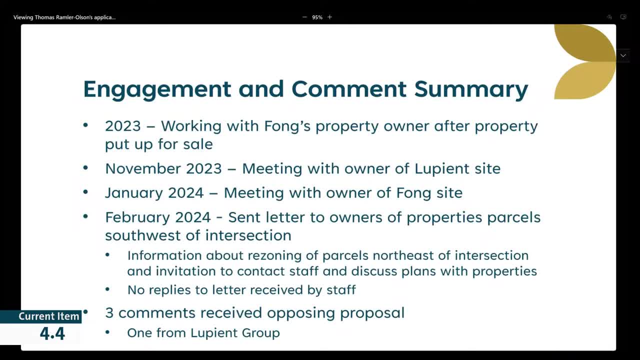 BOTH. IN FEBRUARY WE SENT A LETTER TO THE OWNERS OF THE PROPERTIES, AND YOU KNOW, LETTING THEM KNOW ABOUT THE STUDY SESSIONS, AND THAT THE PUBLIC HEARINGS WERE COMING UP AND WE DID RECEIVE SOME. 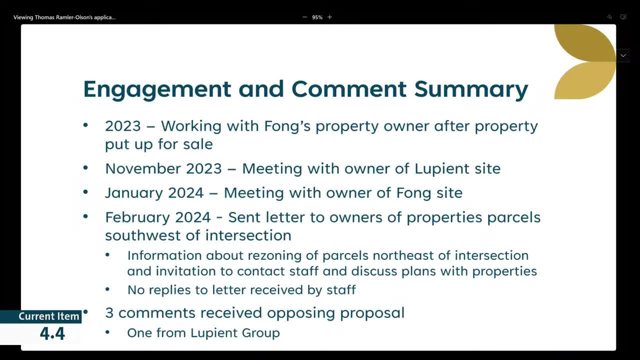 REPLIES. I'M SORRY, I SHOULD CHANGE THAT BULLET POINT. WE DID RECEIVE SOME REPLIES TO THAT LETTER FROM THE LUPEAN GROUP. WE GOT ONE REPLY FROM THEM. THEY WERE OPPOSED BECAUSE THEY 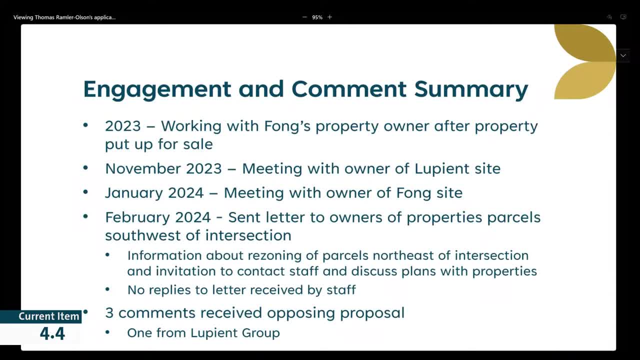 FELT. IT WAS IN THEIR VIEW THAT THIS REZONING WOULD MAKE IT MORE DIFFICULT TO REDEVELOP THEIR PROPERTY. TWO OTHER COMMENTS CAME FROM RESIDENTS OF THAT REAL-LIFE CO-OP JUST SOUTH OF THE IDENTIFIED. 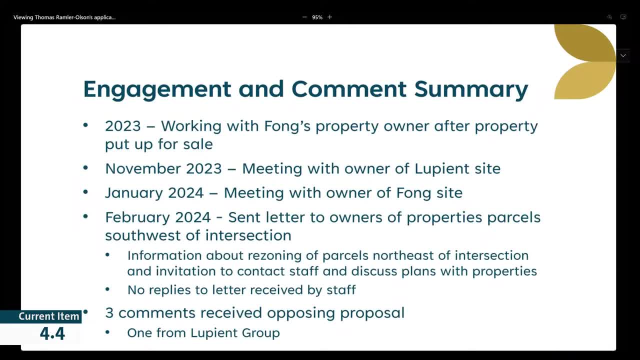 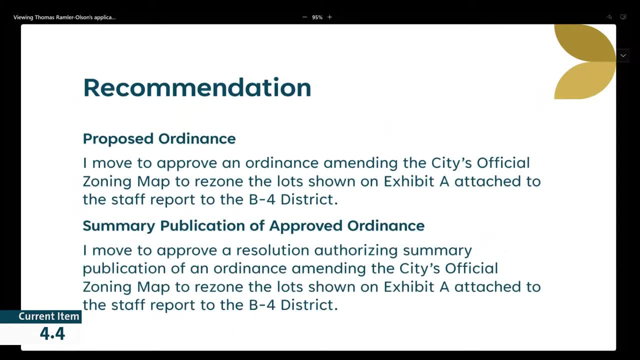 PARCELS UNDER CONSIDERATION. BOTH CORRESPONDENCES ALSO WERE IN OPPOSITION TO THE PROPOSED REZONING, BUT NONETHELESS WITH THAT STAFF STILL RECOMMENDS ADOPTION OF THE PROPOSED REZONING. 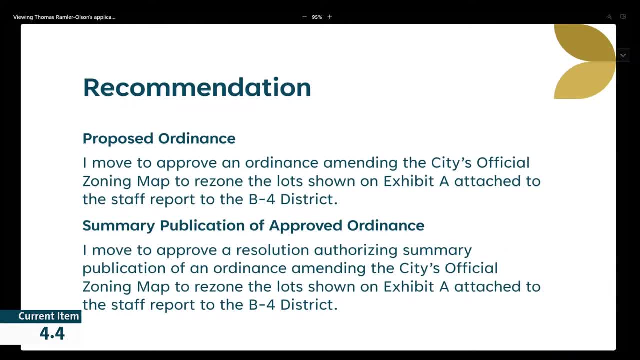 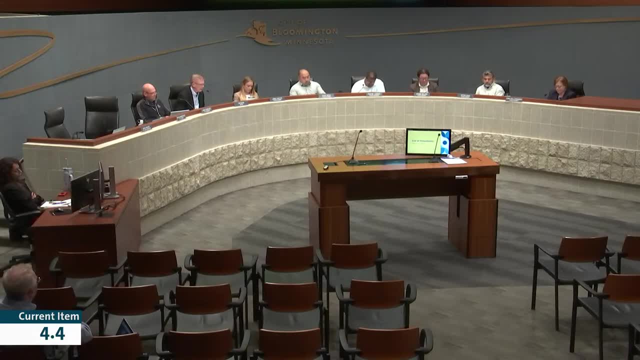 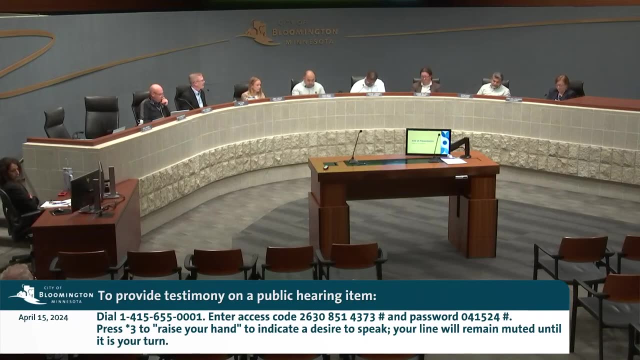 AND THERE'S LANGUAGE ON THIS SLIDE FOR YOU. IF YOU CHOOSE OTHERWISE, I'M AVAILABLE TO TAKE ANY QUESTIONS THAT YOU MAY HAVE. THANK YOU, MR RANDLER-OLSON. I HOPE THAT DIDN'T TEXT YOUR COLD TOO BAD OR YOUR COUGH. 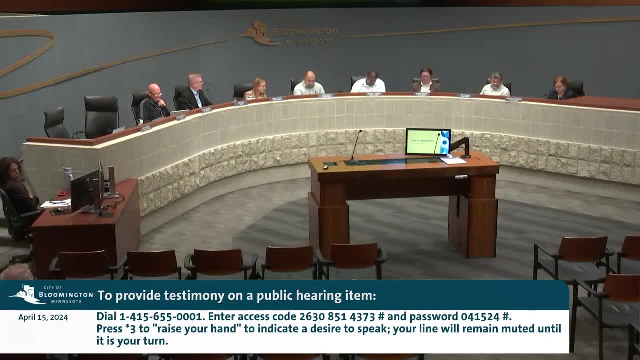 NO, NO, NO, I'M GOOD. OKAY, THANK YOU, MAYOR. WELL, DONE COUNCIL. ANY QUESTIONS? COUNCIL MEMBER LOMENT. THANK YOU, MAYOR. I HOPE YOU'RE FEELING BETTER. 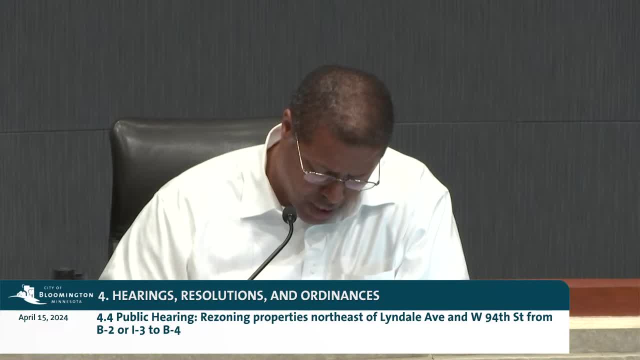 WITH YOUR COLD THERE, SO THEN WITH THE. THERE WAS SOME OPPOSITION THERE WITH REAL-LIFE, IS IT JUST? DO YOU THINK YOU UNDERSTAND? IT WAS JUST CONFUSION IN TERMS OF WHAT WAS BEING PROPOSED THERE. I MEAN I SEE IN THE STAFF. 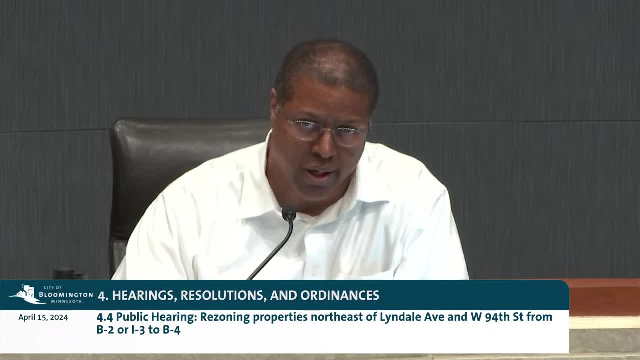 REPORT THAT THERE'S REALLY JUST THE TWO. YOU KNOW, IT'S JUST THE AUTO DEALERSHIP PIECE THAT DOESN'T SEEM TO CARRY THROUGH MAYOR COUNCIL MEMBER LOMENT THE HOW STAFF UNDERSTOOD THOSE. 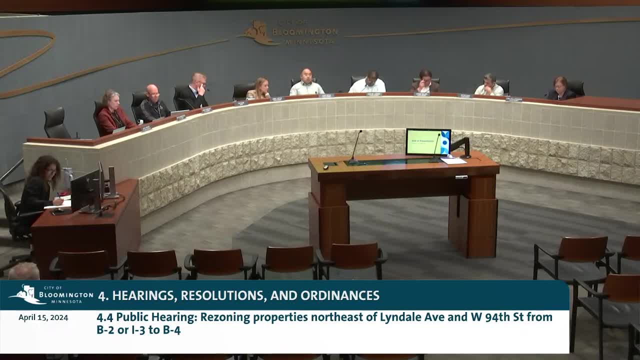 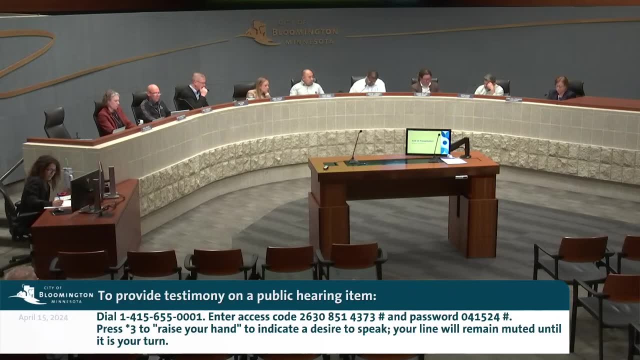 LETTERS OF OPPOSITION FROM RESIDENTS AT THE REAL-LIFE CO-OP. THEY WERE CONCERNED ABOUT JUST THE NORMAL BYPRODUCTS OF ADDED UNITS, ADDED DEVELOPMENT, SO TRAFFIC, CONGESTION, THOSE. 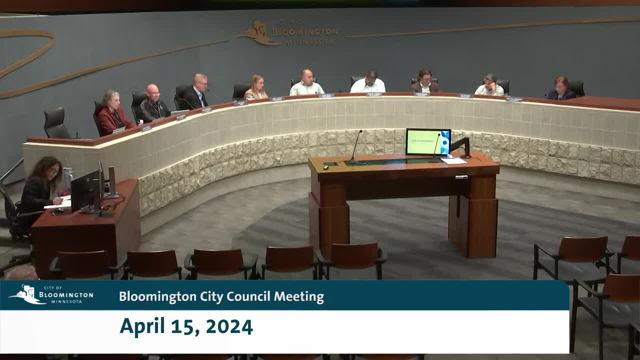 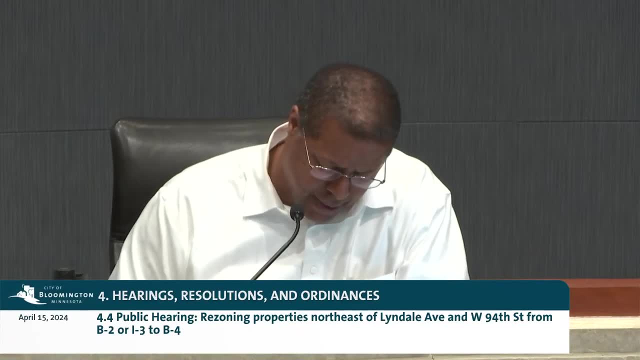 APPEARED TO BE THE MAIN REASONS FOR OPPOSITION. OKAY, NOT IN MY BACKYARD DEAL, OKAY, SO THEN. SECONDARILY, MY QUESTION WOULD BE WITH RESPECT TO THE BUILDING FLOOR AREA. 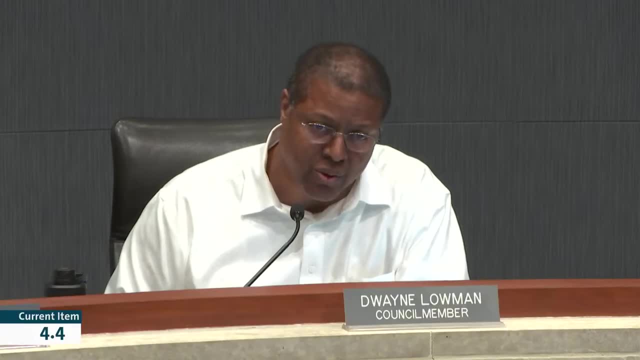 IT LOOKS LIKE AS IT RELATES TO RESTAURANTS, THAT IN THE B-2 YOU COULD HAVE IT AS 2,000 SQUARE FEET FOR RESTAURANT PIECES OF FUNDS. IS THAT STILL AN ASPECT OF THE? 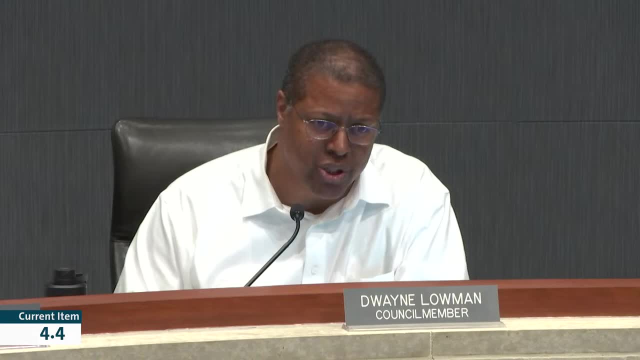 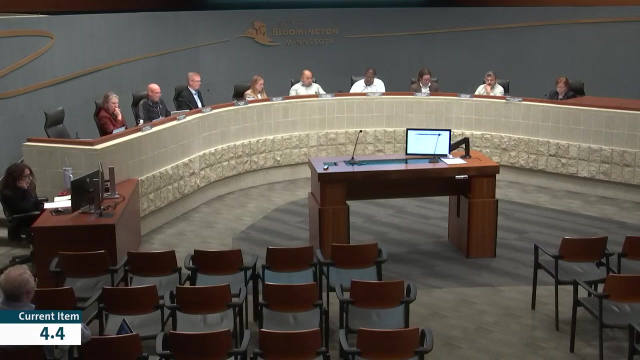 B-4 ZONE AT ALL, AND THEN, JUST FOR MY KNOWLEDGE, IF YOU LOOK AT DAVID FONG'S HOW MANY SQUARE FEET, WAS THAT MAYOR COUNCILMEMBER? I'M UNAWARE OF WHAT. THE FLOOR AREA. 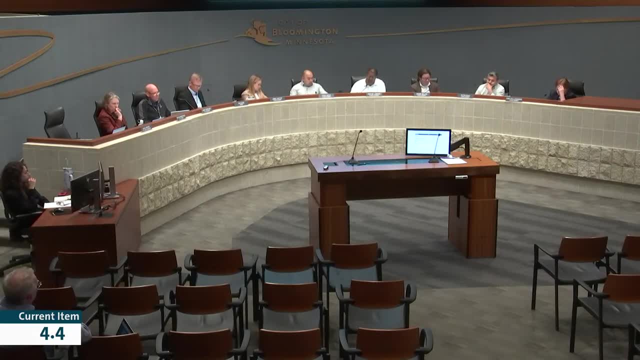 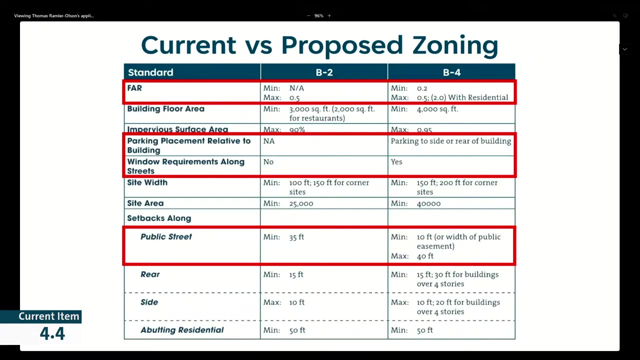 WAS OF FONG'S, SO I'M UNABLE TO COMMENT ON THAT. YEAH, YOU ARE READING THIS TABLE CORRECTLY, WHERE THERE IS A 2,000 MINIMUM SQUARE FOOT FOR RESTAURANTS, AND THEN UNDER B-4. 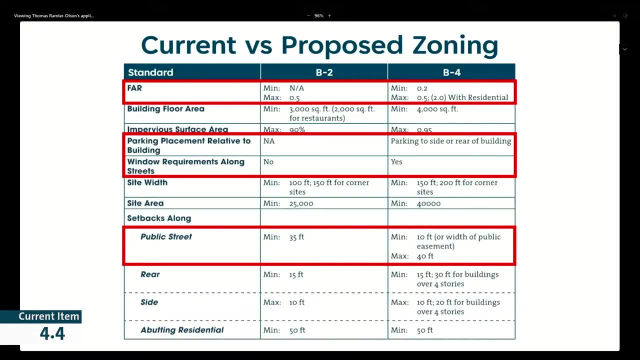 THAT WOULD ANY DEVELOPMENT WOULD HAVE A MINIMUM FLOOR AREA OF 4,000 SQUARE FEET AND WE ASSUME, OR WE'RE FAIRLY CONFIDENT, THAT, IN ORDER TO DO THE TYPE OF DEVELOPMENT WE'RE EXPECTING AT THESE PROPERTIES. 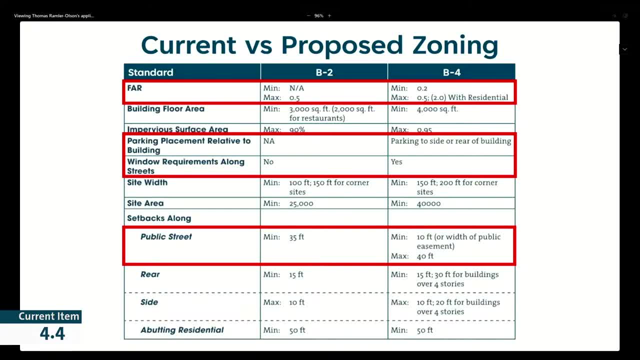 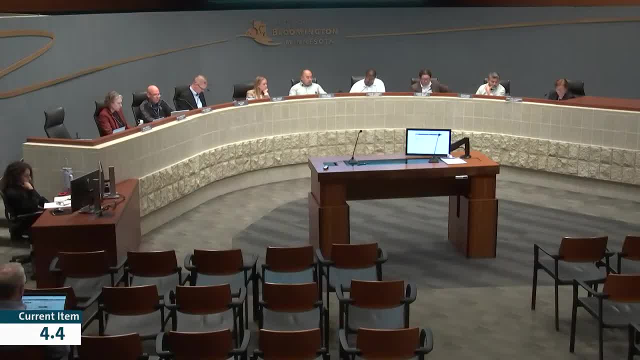 THESE LOTS WOULD HAVE TO BE COMBINED AND ASSEMBLED INTO A FASHION IN ORDER TO ACCOMMODATE THE TYPE OF DEVELOPMENT. THAT WOULD ADVANCE THE. YOU KNOW THAT STAFF WOULD SUPPORT AND THAT WOULD ADVANCE THE. 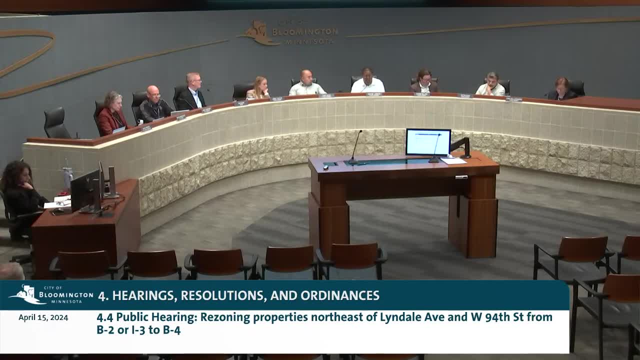 RETROFIT PLAN. SO YOU'RE THINKING: NO MATTER WHAT, IF YOU HAD A SMALLER RESTAURANT, YOU COULD PROBABLY SQUEEZE IT IN THERE WITH THE PLAN DEVELOPMENT OR SOME OTHER TYPE OF OKAY. 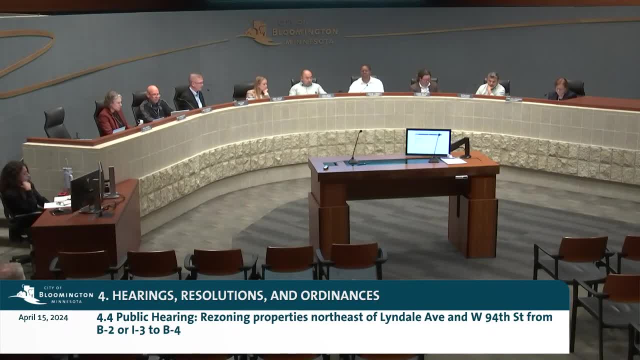 I GOT IT. THAT'S GOOD. GOOD ENOUGH FOR ME. THANKS, COUNCIL. ADDITIONAL QUESTIONS. COUNCILMEMBER MUA. THANK YOU, MAYOR. IS THERE ANY CONCERN WITH THE FONGS ABOUT THIS REZONING AND? 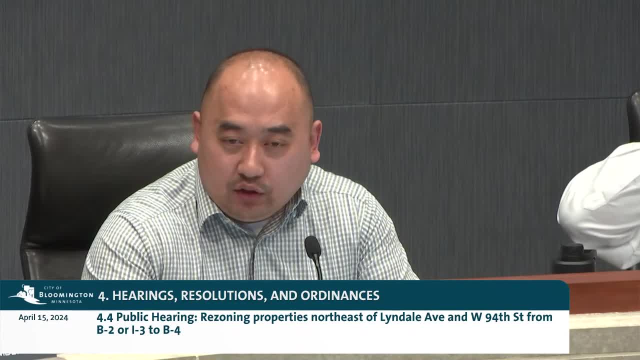 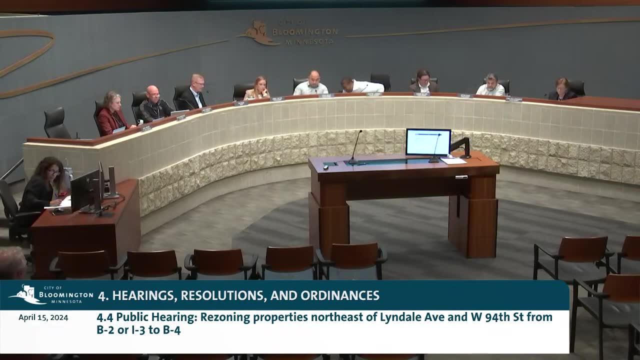 IMPACTING THEIR ABILITY TO SELL THE PARCELS, BECAUSE I JUST DROVE BY THERE TODAY AND I SAW A BIG SIGN UP FOR SALE. SO JUST WONDERING HOW THAT IMPACTS, OR COULD IMPACT THAT. 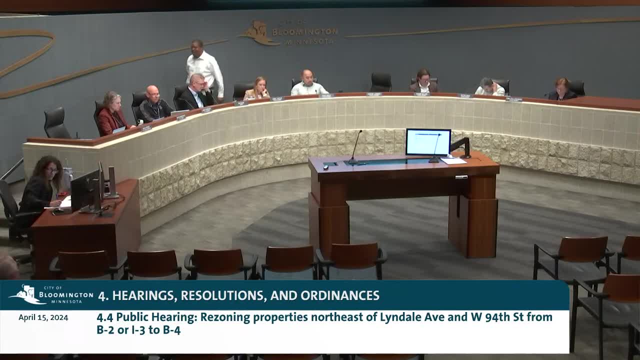 MAYOR COUNCILMEMBER, WE- THIS IS ACTUALLY KIND OF FEEDS INTO THE ENGAGEMENT WE'VE BEEN DOING, NOT DIRECTLY RELATED TO THIS PROJECT, BUT WE KNEW THAT FONGS WAS PUT ON THE MARKET AND 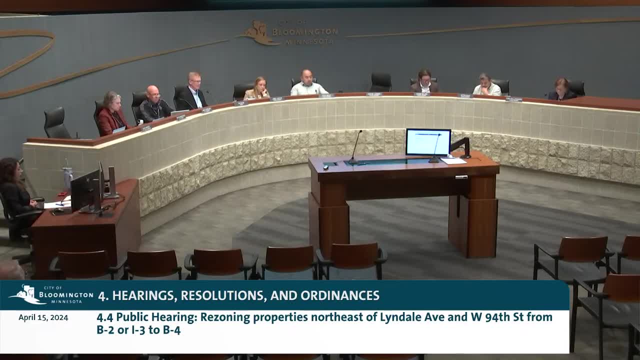 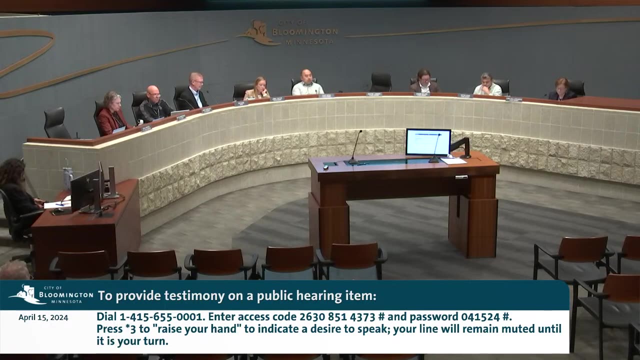 THAT DEVELOPERS WOULD BE INTERESTED IN WHAT SORT OF GUIDANCE OR DEVELOPMENT FORM THE CITY WOULD SUPPORT, AND SO WE'VE BEEN IN CLOSE CONTACT WITH THEM. THERE HAVE BEEN SOME PERSPECTIVE DEVELOPMENTS KIND OF. 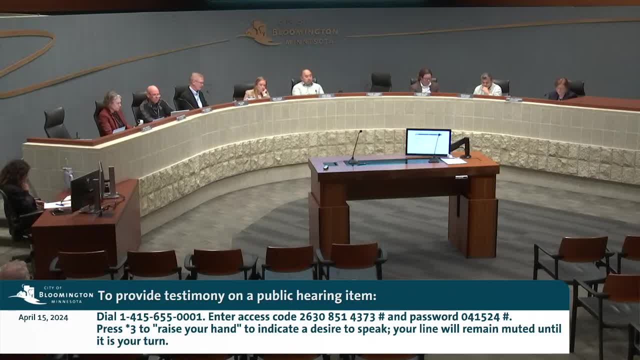 BANDIED ABOUT, BUT NOTHING FIRM AND NOTHING'S BEEN, NOTHING'S TAKEN HOLD AT THE MOMENT. I BELIEVE THIS REZONING WILL HELP ADVANCE. THEY'LL BE GIVEN MORE CLEAR GUIDANCE WITH THIS REZONING. 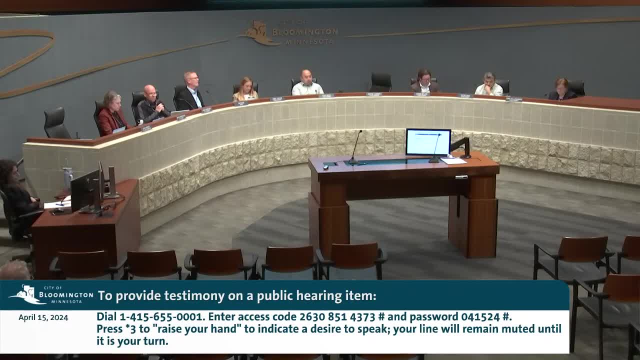 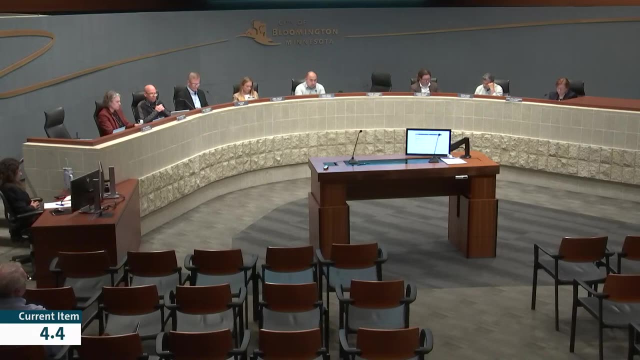 AND AS FOR ANY SORT OF CONCERN, I DON'T BELIEVE FONGS IS IN ATTENDANCE RIGHT NOW, BUT WE HAD A GOOD DISCUSSION WITH THEM AND WE REACHED OUT SEVERAL TIMES TO INFORM THEM OF THIS PROJECT, AND 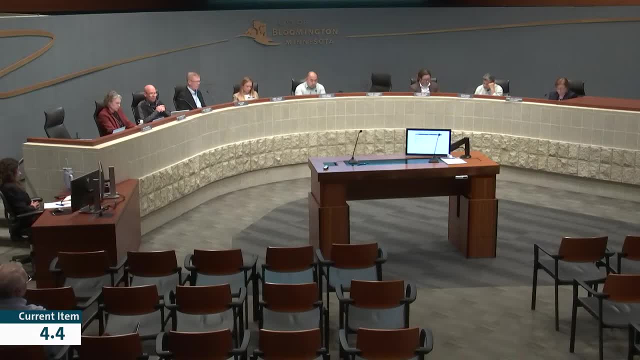 TO OFFER OUR TIME TO HAVE ANY DISCUSSIONS WITH ANY. YOU KNOW IF THEY HAD ANY CONCERNS TO HAVE THOSE CONVERSATIONS NOW. SO WE'VE MADE OURSELVES AVAILABLE, BUT OTHERWISE WE HAVEN'T. WE HAVEN'T HEARD FROM 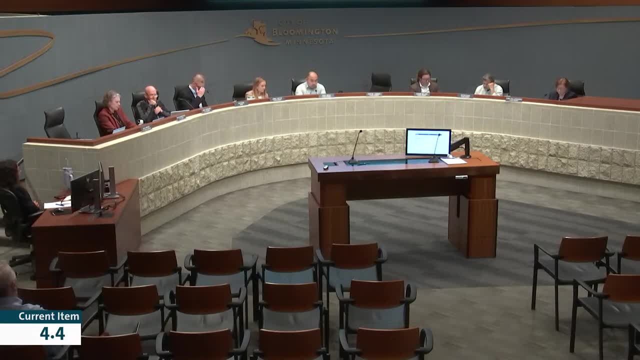 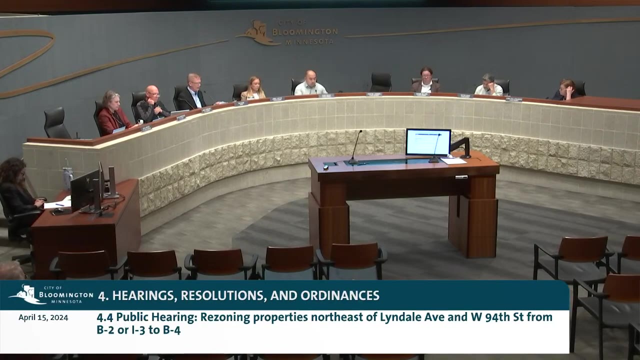 THEM SINCE THIS? SINCE THEY RECEIVED A NOTICE FOR THIS PUBLIC HEARING COUNCIL? ADDITIONAL QUESTIONS. IF NOT, THANK YOU, MR RAMLER OLSEN. WE'RE GOING TO OPEN THE PUBLIC HEARING IN CASE QUESTIONS. 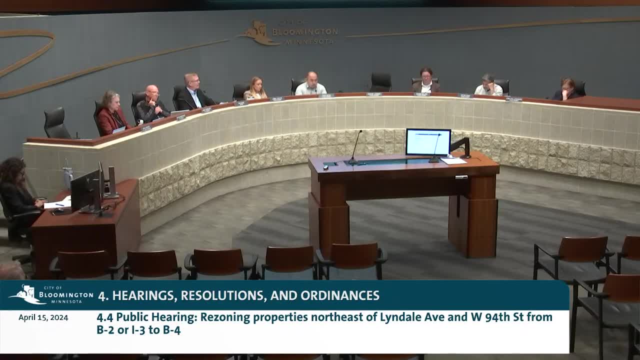 ARISE HERE, I WILL OPEN THIS PUBLIC HEARING ON ITEM 4.4.. THIS IS A PUBLIC HEARING REGARDING THE REZONING OF PROPERTIES NORTHEAST OF LINDALE AVENUE AND WEST 94th STREET. 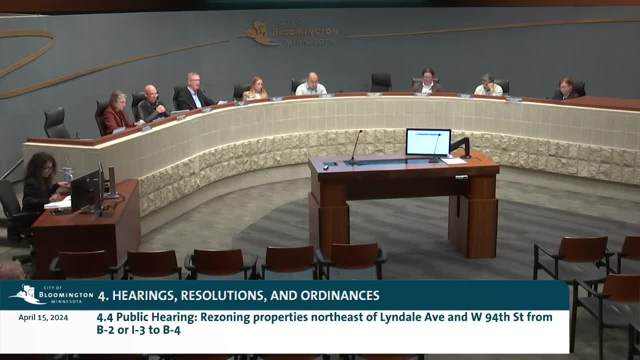 FROM B2 OR I3 TO B4.. IS THERE ANYONE IN THE COUNCIL CHAMBERS WISHING TO SPEAK ON THIS THIS EVENING? MS MERCER, IS THERE ANYONE ON THE LINE WISHING TO SPEAK? 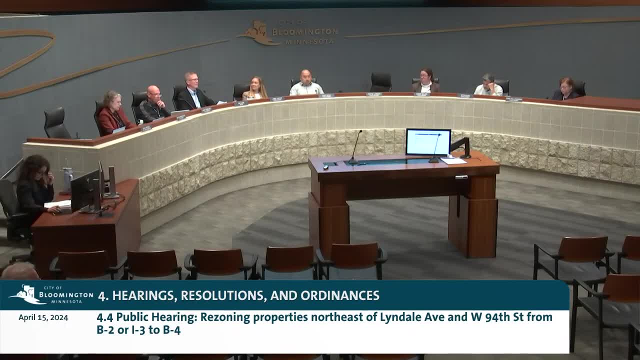 OH, I'M SORRY, I DID NOT SEE YOU. COME ON FORWARD. IS THIS ONE ON? YES, YES, IT IS. WE'LL NEED YOU TO IDENTIFY YOURSELF OFFICIALLY FOR THE RECORD, IF YOU COULD, THOMAS. 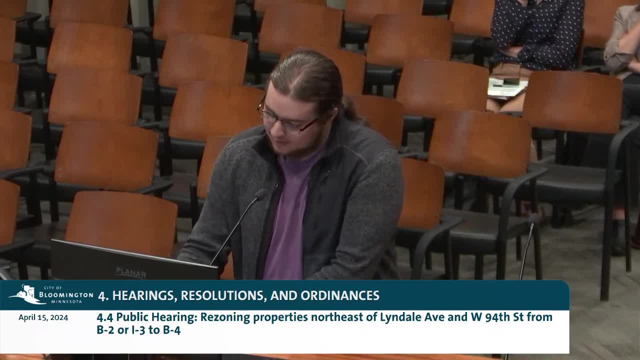 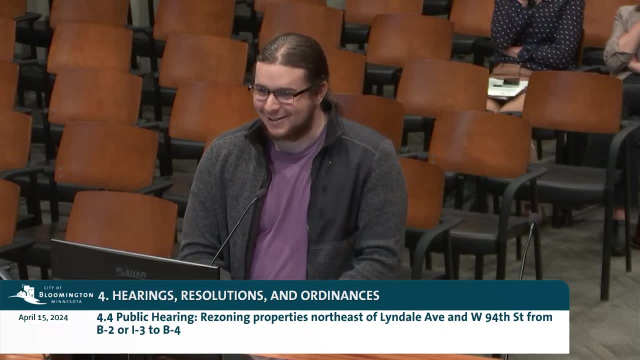 MY NAME IS ROBERT COLEMAN APOLOGIZE. I'M COMING HERE TO SPEAK ABOUT THIS REZONING. I'M KIND OF SUCKS. A LOWMAN STEPPED OUT FOR A MOMENT BUT I REMEMBER THAT WHEN I WAS 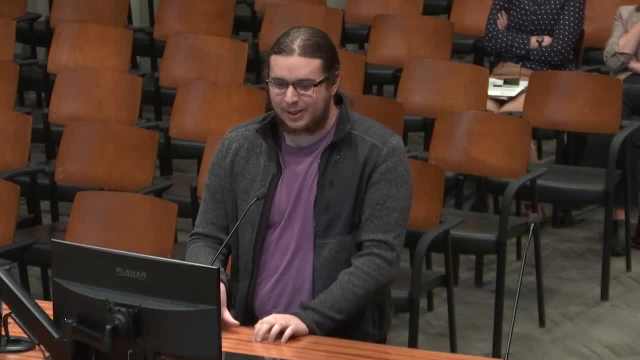 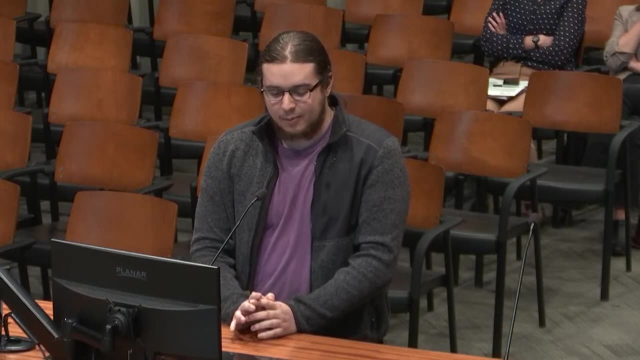 WATCHING THE ORIGINAL APPROVEMENT FOR THE REFIT PLAN. I REMEMBER COMMENTS BY HIM THAT HE WANTED SOMETHING THAT WAS MORE UNMISTAKABLY. URBAN WAS THE WORDING THAT HE USED, AND I AGREE WITH THAT. 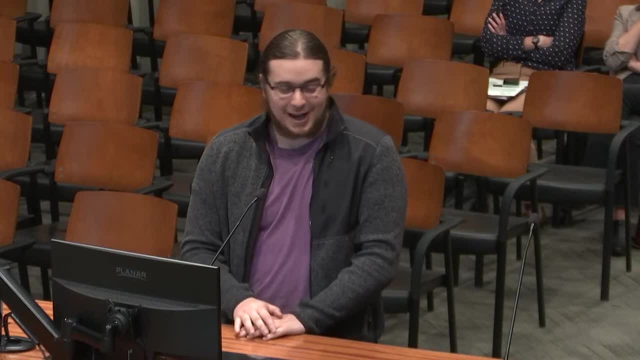 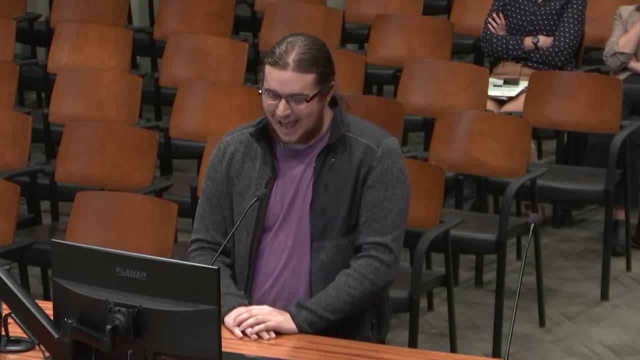 I DON'T SEE. I WISH I HAD THE TIME TO COMMENT WHEN THE PLAN WAS ORIGINALLY BEING DISCUSSED- WHICH I WISH I HAD IT. JUST I DON'T SEE HOW THE B4 ZONING ACTUALLY ACHIEVES THE 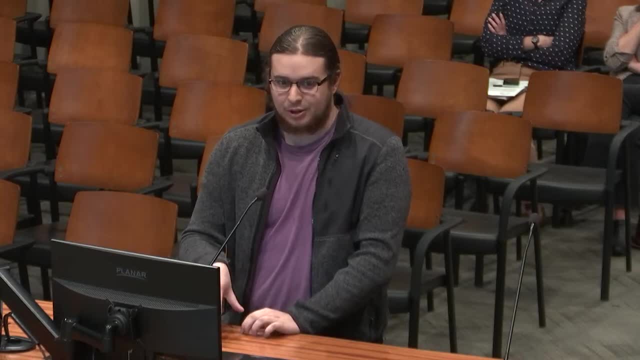 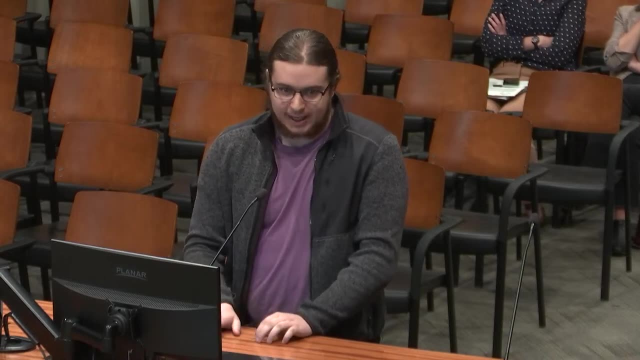 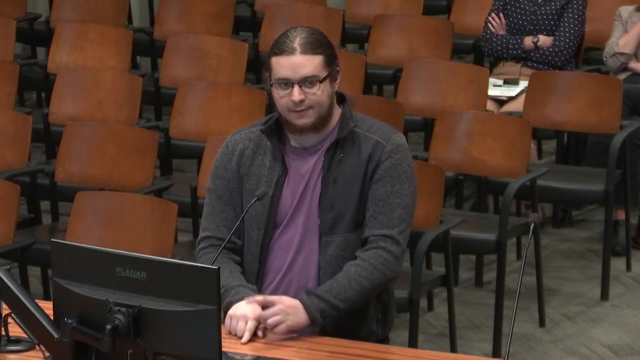 GOALS OF CREATING A DENSER, MORE WALKABLE AREA. I, ON MY DAILY COMMUTE, I WHICH IS WALKING. I WALK THROUGH THE SOUTHWEST CORNER OF VALLEY WEST AT FRANCE AND OLD CHOCOPY ROAD. 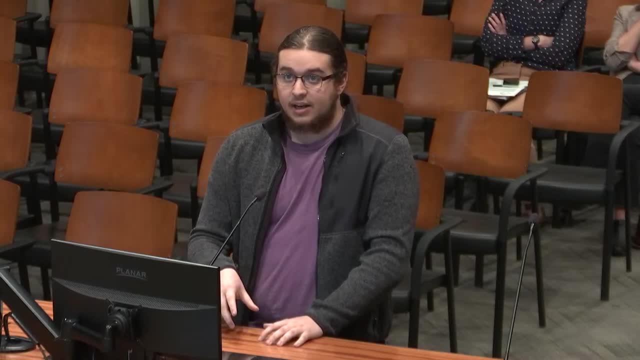 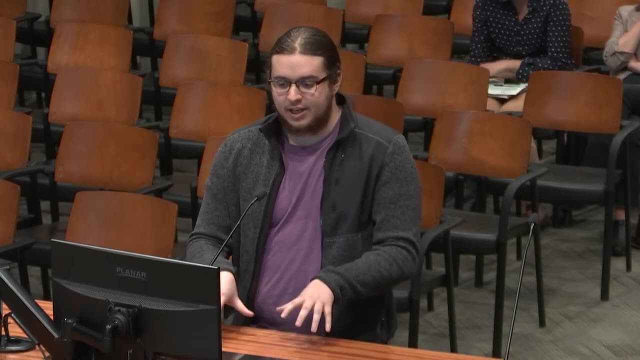 AND THAT AREA IS ZONED B4. AND IT DEFINITELY YOU CAN TELL THE DIFFERENCE BETWEEN WHAT IS ZONED B2 AND B4 IN TERMS OF THAT LIKE IT'S A MORE PLEASANT WALK. 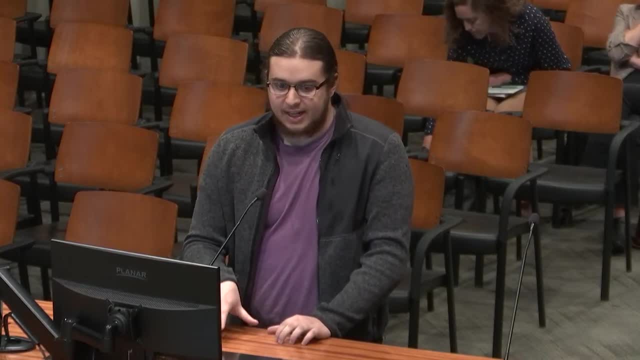 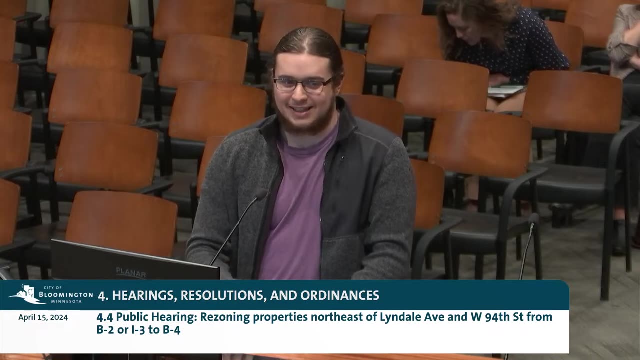 EXPERIENCE FOR SURE. BUT IT IS NOT MORE WALKABLE. THAT'S SOMETHING. THAT IS A COMMON MISCONCEPTION IN TERMS OF THE DEFINITION OF IT. LIKE I CAN WALK THROUGH A LOT OF PLACES. LIKE THERE ARE SIDE I MEAN. 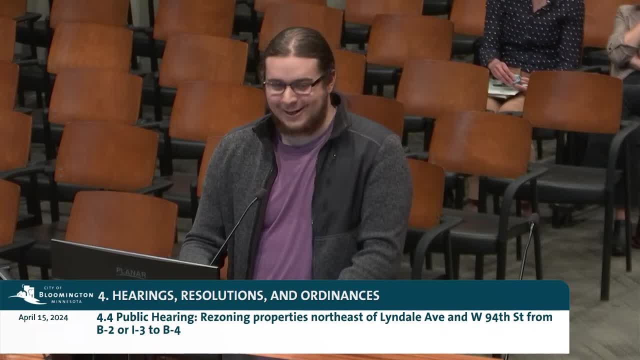 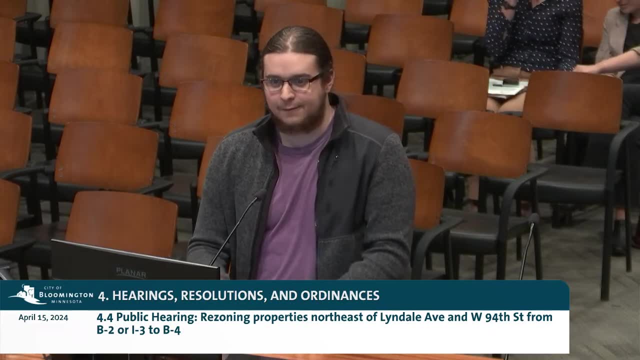 THERE'S NOT A LOT OF SIDEWALKS, BUT I'M WALKING ON THE STREET SOMETIMES, BUT WHEN WE THINK OF WALKABLE, IT'S MORE ABOUT LIKE: CAN YOU LIVE YOUR LIFE WHILE WALKING TO? 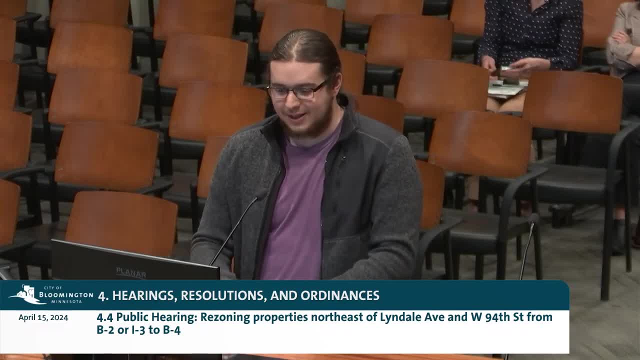 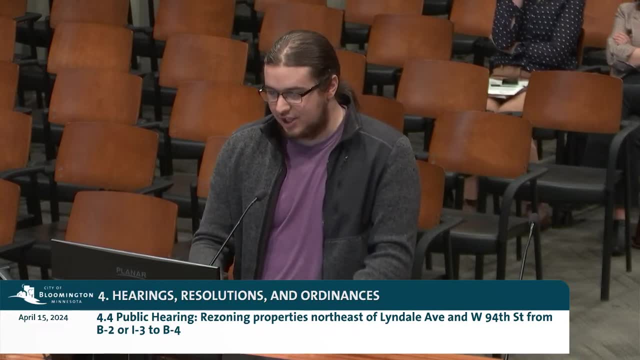 DO YOUR ERRANDS AND TO GO TO YOUR- YOU KNOW YOUR RECREATION- AND TO PARKS AND ALSO YOUR HOUSING, AND I DON'T SEE HOW THIS ACHIEVES IT. THE FLOOR AREA RATIO DOES NOT. 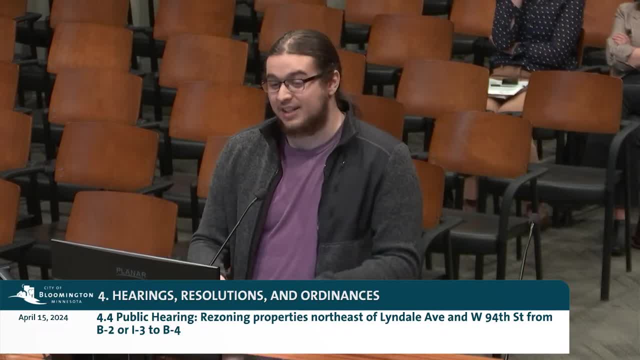 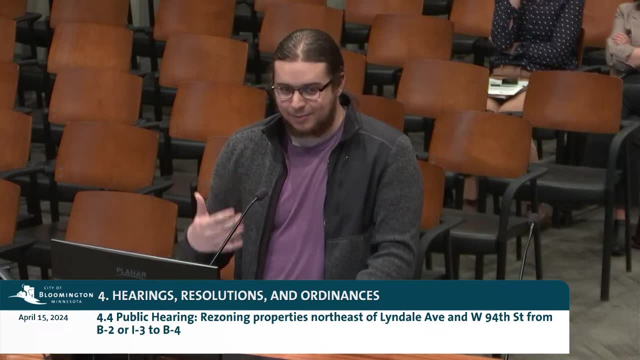 CHANGE IF YOU DON'T HAVE COMMERCIAL AND THERE'S NO GUARANTEE THAT THE DEVELOPMENTS THERE ARE GOING TO HAVE COMMERCIAL. THE MAIN WHAT I IMAGINE MOSTLY WOULD BE THE ISSUE WITH THE NUMBER OF PARKING SPOTS. YOU 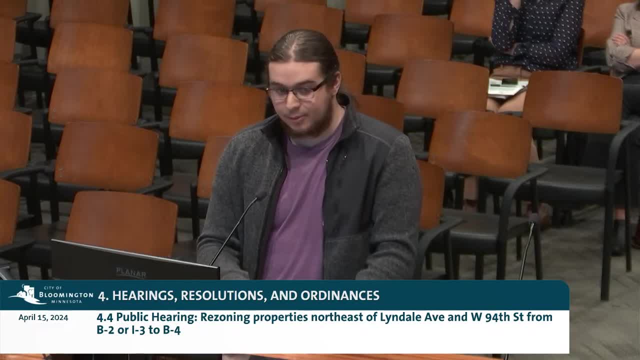 WOULD BE REQUIRED. THERE'S NO CHANGE TO THE NUMBER OF PARKING SPOTS, AND MAYBE YOU COULD SEE SOME OF THAT FLEXIBILITY COMING THROUGH THE OPPORTUNITY HOUSING ORDINANCE, BUT THOSE ARE LIKE. 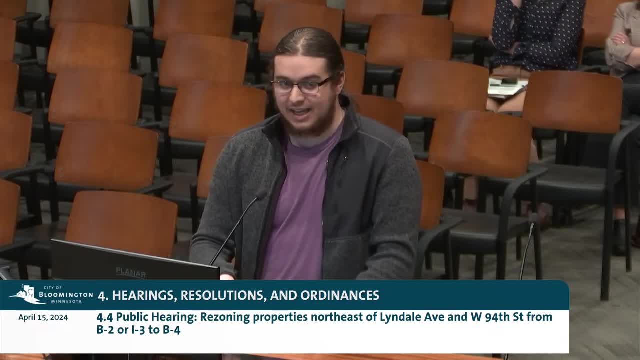 THE CHALLENGES THAT WOULD ACTUALLY BE PUTTING IN COMMERCIAL TO THOSE SPOTS, BECAUSE IF IT'S NOT SURFACE AND IT'S UNDERGROUND, AND THAT'S A BIG COST AND IN TERMS OF LIKE THE OTHER THAN THAT THE. 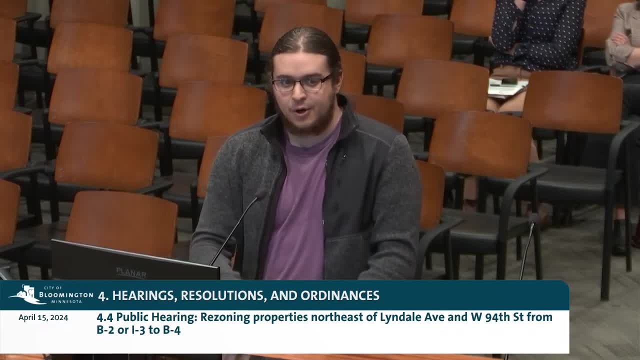 ONLY MAJOR CHANGE IS THAT THE PARKING HAS TO BE TO THE SIDE OR TO BEHIND, AND WHEN I THINK OF THE POP EYES, THERE'S NOT ANY PARKING BETWEEN THE BUILDING AND THE SIDEWALK, AND OTHER THAN THAT. THAT'S EVERYTHING ELSE. 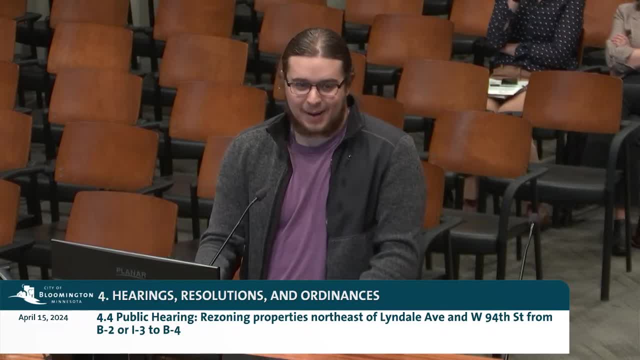 I MEAN OTHER THAN THE. I THINK I MEASURED LIKE. THE SETBACK WOULD HAVE TO BE TEN FEET CLOSER IF YOU WERE BUILDING A SIMILAR SITE. THERE'S LIKE, THERE'S NOTHING. 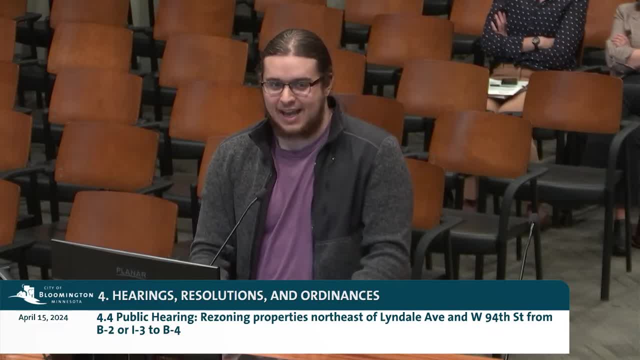 ELSE STOPPING THAT AUTO-ORIENTED LAND USE AND ACTUALLY CHANGING IT INTO WHAT COULD BE A MORE WALKABLE AREA? THAT'S MY MAJOR CHANGE. THAT'S MY MAIN CONCERN. I FEEL LIKE. IF OBVIOUSLY NOT. 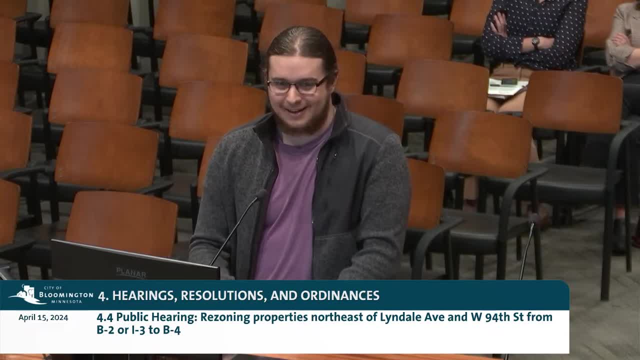 GOING TO CHANGE MIDWAY. WHAT THE ZONING? WHAT ZONE YOU'RE GOING TO CHOOSE FOR THE RETROFIT? BUT I FEEL LIKE IF THE DEFAULT FOR THE B4 ZONING WAS MIXED: USE AND HAVING RESIDENTIAL AND THEN. 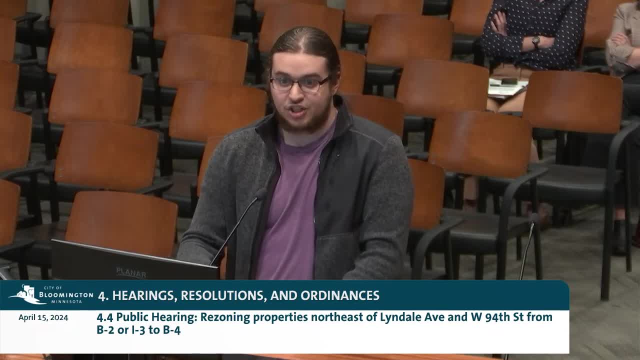 HAVING THE IT, NOT HAVING RESIDENTIAL, BE LIKE A CONDITIONAL. I THINK THAT WOULD BE A GOOD IDEA, AND ALSO IN THE B4 ZONING. IF YOU IN THE B4 ZONING SAY MAYBE. YOU REDUCE THE PARKING MINIMUMS BY 20%- 25% BEFORE YOU ADD THE POTENTIALLY THE OHO FOR THE PARKING MINIMUMS. OTHER THAN THAT, I DON'T SEE HOW THE B4 ZONING REALLY ACHIEVES. 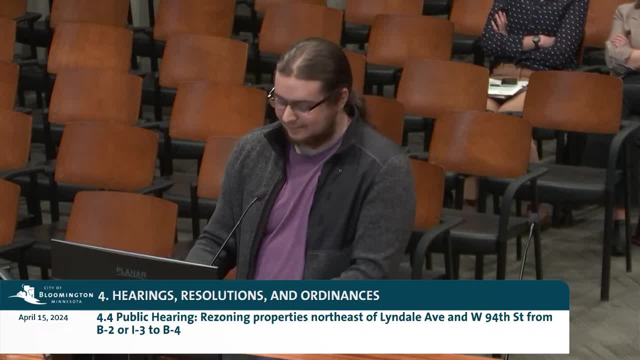 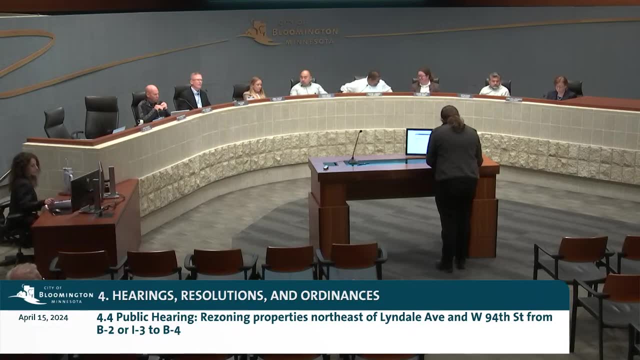 THE GOALS. THAT IS SET OUT IN THE RETROFIT FROM MY PERSPECTIVE. THANK YOU VERY MUCH FOR YOUR COMMENTS AND I'M SORRY I DIDN'T RECOGNIZE YOU AS YOU STOOD UP. I APOLOGIZE FOR THAT. 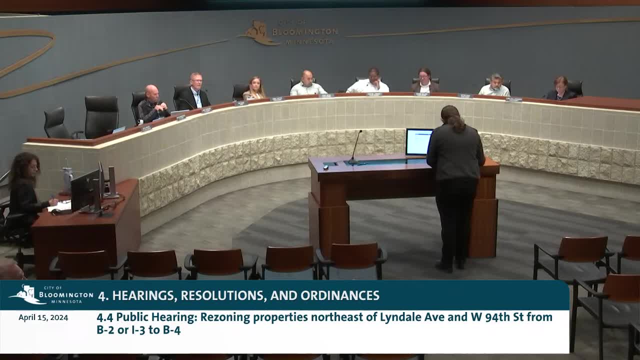 ANYONE ELSE IN THE COUNCIL CHAMBERS WISHING TO SPEAK ON THIS? MS MERCER, DO WE HAVE ANYONE ON THE PHONE WISHING TO SPEAK? LAST CALL FOR ANYBODY IN THE CHAMBERS. 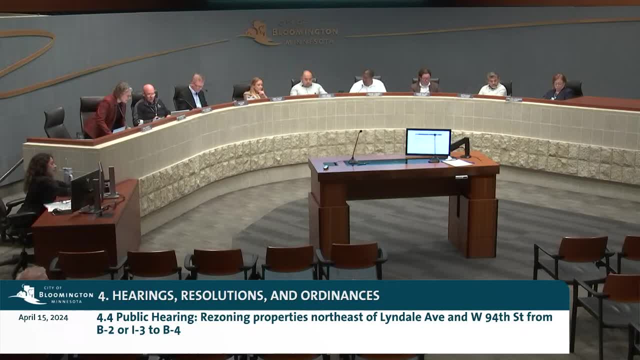 COUNCIL. NO ONE COMING FORWARD IN THE CHAMBERS. NO ONE ON THE PHONE. I'D LOOK FOR A MOTION TO CLOSE THE PUBLIC HEARING ON ITEM 4.4 THIS EVENING, SO MOVED TO CLOSE THE. 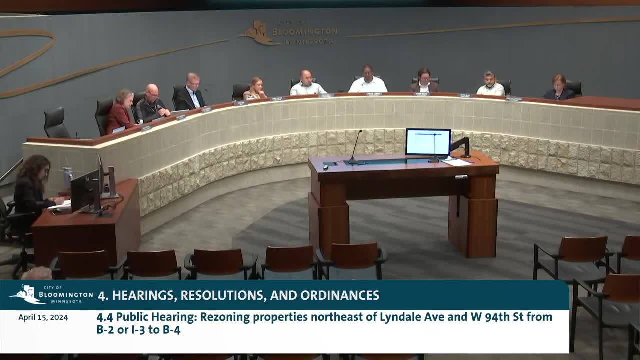 PUBLIC HEARING. MOTION BY COUNCIL MEMBER DALLASANDRO TO CLOSE THE PUBLIC HEARING ON ITEM 4.4.. NO FURTHER COUNCIL DISCUSSION ON THAT. ALL THOSE IN FAVOR, PLEASE. 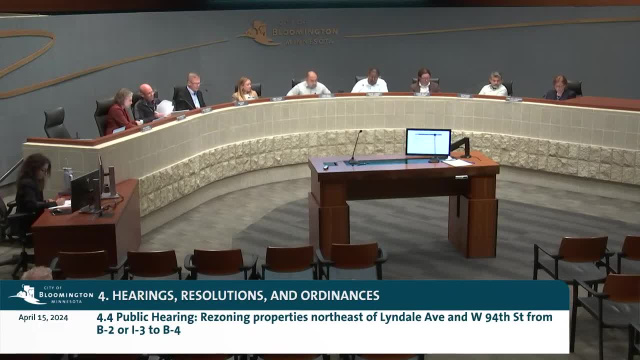 SIGNIFY BY SAYING AYE. OPPOSED MOTION CARRIES 7-0.. COUNCIL QUESTIONS ON THIS OR DISCUSSION REGARDING THIS: PROPOSED ZONING CHANGE COUNCIL MEMBER LOMAN. 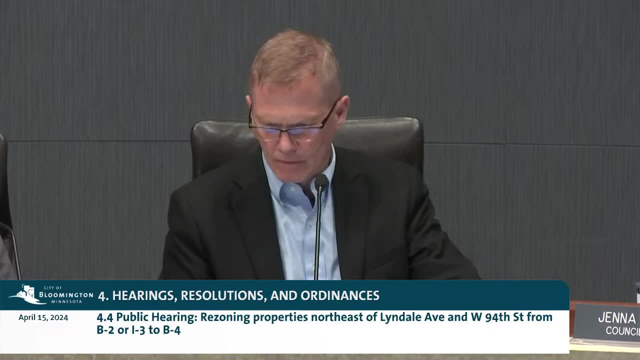 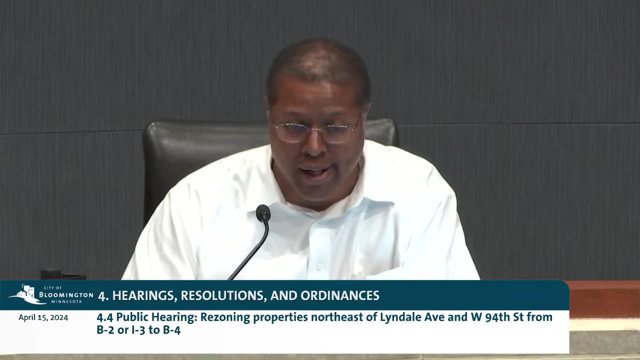 SO I WOULD PUT THAT THE QUESTION THAT OUR PUBLIC COMMENTER PUT FORTH TO US WITH THIS BEFORE, IN TERMS OF THE WALKING STANDARDS THAT WE PUT FORWARD: WHAT DOES THIS GUARANTEE US THAT THAT IS SOMETHING TO BE DEVELOPED IN? 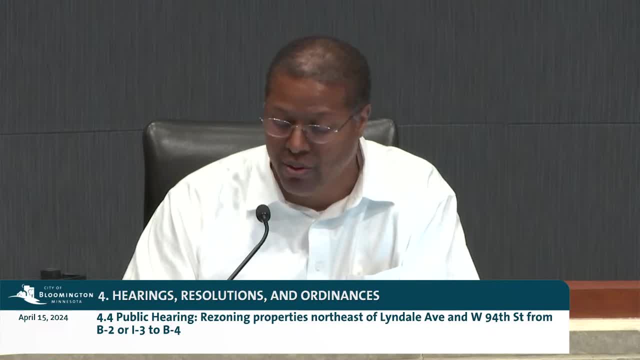 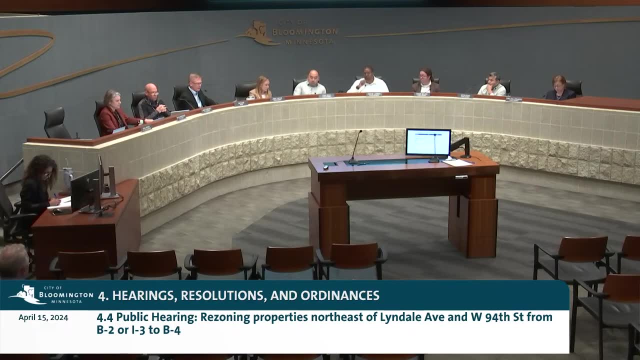 THAT AREA. IS THERE A BETTER ZONING CODE? THAT WOULD ALLOW US TO DO THAT. MR RAMLER-OLSON, ARE YOU STILL WITH US? OH, YES, YES, I AM. I'M SORRY, WAS THAT A QUESTION TO ME? 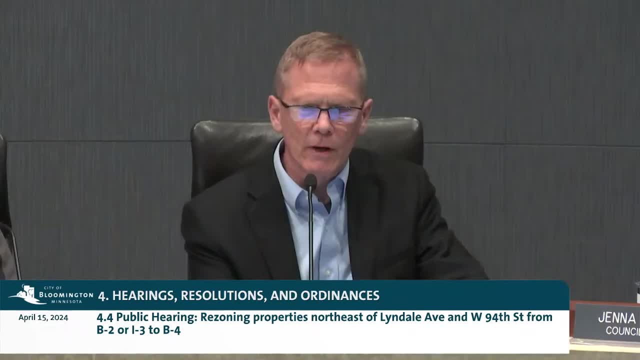 WELL, I THINK THE QUESTION JUST IN GENERAL: THE BENEFITS OF THE B-4 AS OPPOSED TO ANOTHER POSSIBLE ZONING STANDARD THAT WE COULD CONSIDER TO MAKE THIS A BIT MORE WALKABLE OR A BIT MORE OF. 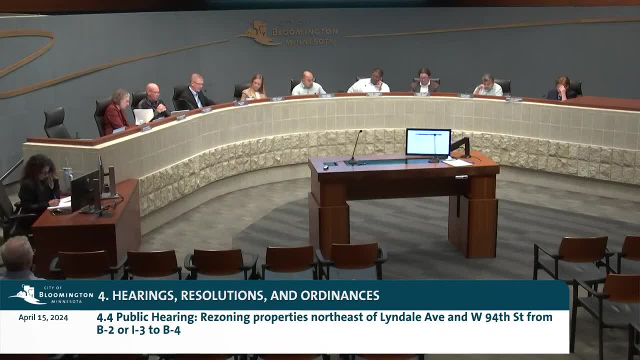 AN URBAN FEEL TO IT. YES, THANK YOU, MAYOR. THANK YOU, COUNCILMEMBER, LOMAN, THE. I WILL JUST SPEAK SAYING THAT I WAS NOT THERE FOR ALL THE DISCUSSIONS AROUND THE. 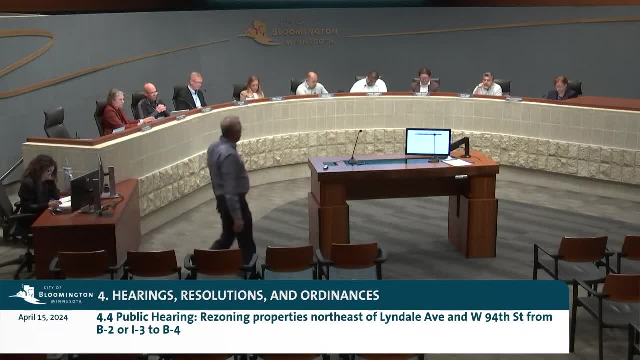 RETROFIT PLAN. THE REASONING THAT WAS GIVEN TO ME SECOND HAND BY PLANNERS, THAT WERE THERE IS, AND SOMETHING THAT I COVERED IN A PREVIOUS SLIDE IS THAT THE OPTION FOR B-4 WAS NOT THERE. 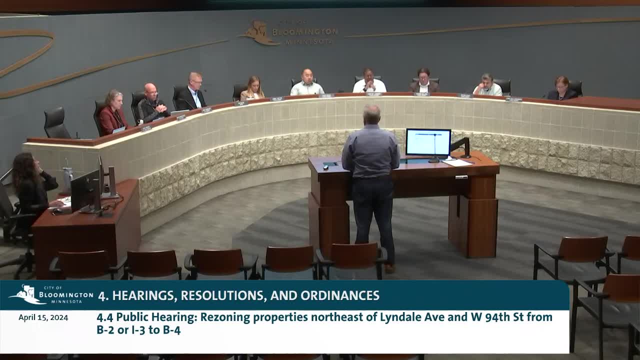 THE REASONING THAT WAS GIVEN TO ME IS THAT THE OPTION FOR B-4 WAS A MORE, WAS AN EASIER ZONING DISTRICT TO IMPLEMENT, AT LEAST FOR TRANSITIONING FROM WHAT IS B-2 TO B-4 OR FROM THE AUTO. 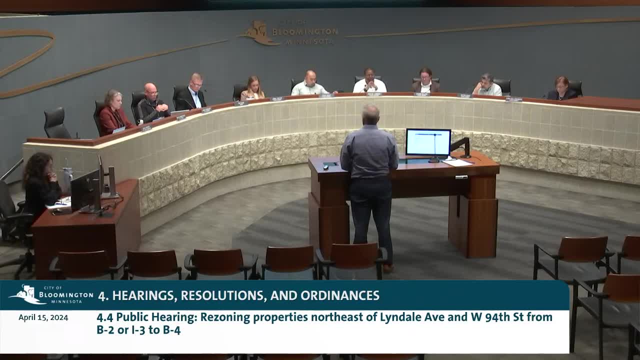 ORIENTED NATURE OF B-2 TO THE MORE PEDESTRIAN FRIENDLINESS OF B-4, WITHOUT DISRUPTING TOO MUCH AGAIN. THERE'S A LOT OF SIMILARITIES BETWEEN B-2 AND B-4, BUT THE B-4 STANDARDS DO REFLECT. 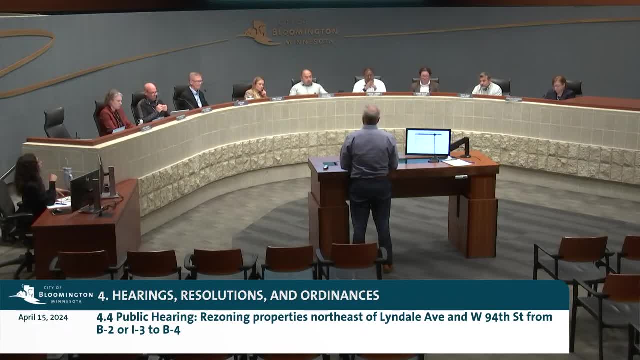 MORE PEDESTRIAN FRIENDLY URBAN FORM, AT LEAST FOR THE ZONING DISTRICTS THAT WE HAVE AVAILABLE. ON THE BOOKS, I CAN'T SPEAK TO THE PARKING REQUIREMENTS, BUT THERE IS THAT ABILITY TO GO BIGGER WITH ADDING. 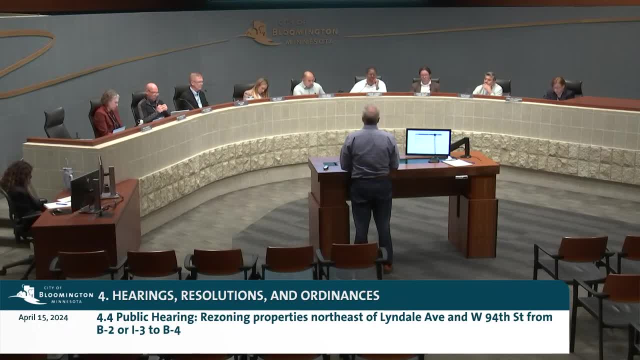 RESIDENTIALS. SO HAVING A MORE MIXED USE FIELD FOR DEVELOPMENT WILL ALLOW MORE, BIGGER DEVELOPMENT AND RELOCATING THAT, PARKING TO THE SIDE OF THE REAR DOES HELP WITH INCREASING THE PEDESTRIAN SAFETY OF THE AREA. 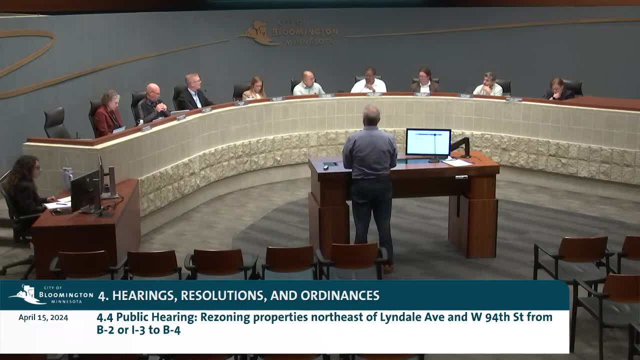 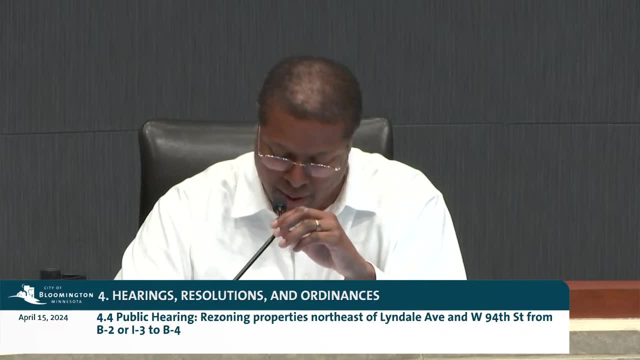 AGAIN WINDOW REQUIREMENTS. I CAN UNDERSTAND IF YOU WEREN'T THERE. I APPRECIATE THAT. GIVEN THE LATENESS OF THE HOUR HERE, TRYING TO MOVE THIS ALONG A LITTLE QUICKER, I HATE TO INTERRUPT YOU THERE. 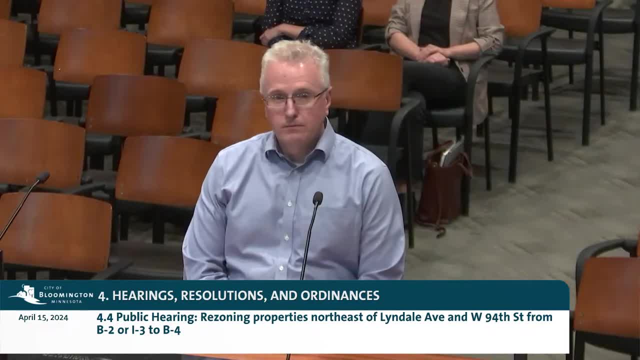 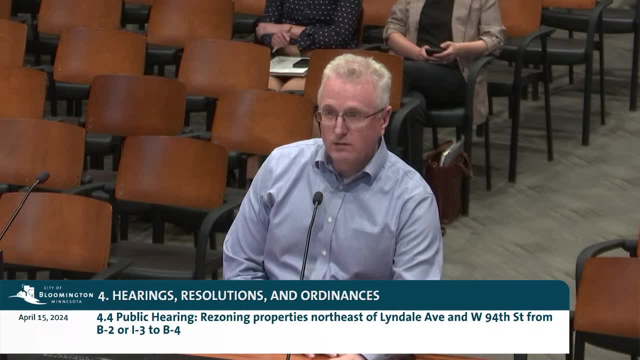 WHY DON'T WE ASK? MR MARKERGART IS AT THE PODIUM AND OBVIOUSLY WAS VERY INVOLVED IN THE LINDALE AVENUE. RETROFIT, MR MARKERGARTEN. SURE I'M THERE, BUSSY COUNCILMEMBER. 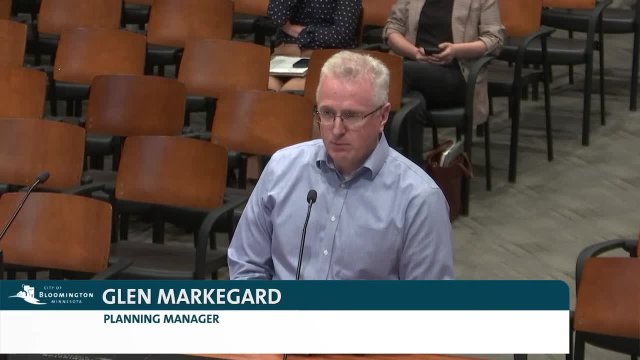 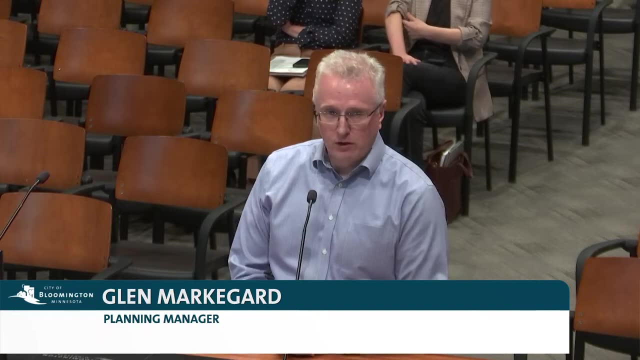 LOMAN. I THINK THERE ARE SEVERAL KEY ASPECTS OF BEFORE. THAT WOULD MAKE IT QUITE A BIT MORE OF AN URBAN CHARACTER, KIND OF WHAT'S CALLED FOR IN THE LINDALE AVENUE RETROFIT PLAN. 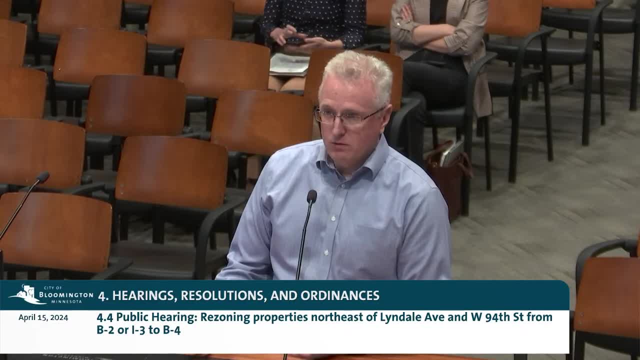 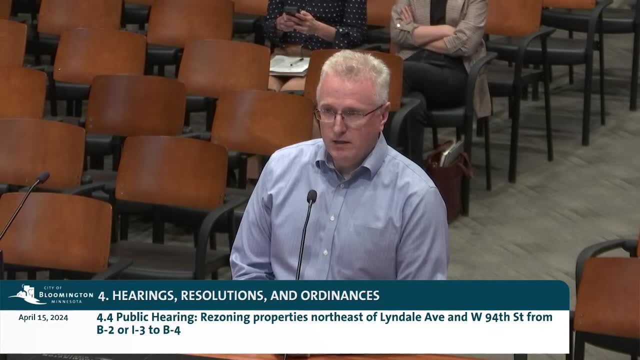 A FEW THINGS THAT STAND OUT ARE THE FACT THAT IT ALLOWS RESIDENTIAL USES WHEREAS BE TO DOES NOT ALLOW RESIDENTIAL USES. A LOT OF THE MARKET INTEREST TO DATE IN THAT AREA HAS BEEN FOR. 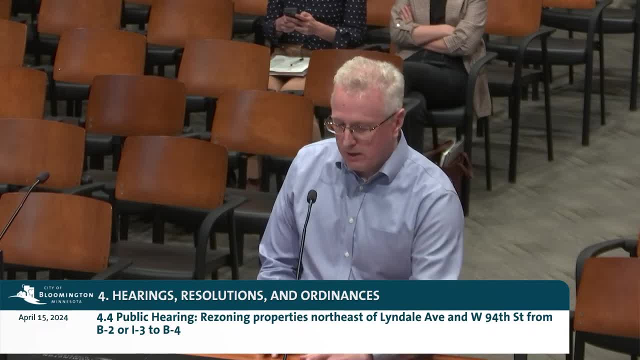 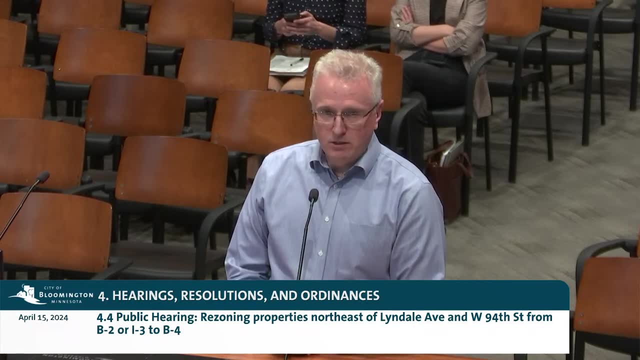 RESIDENTIAL. ANOTHER REALLY IMPORTANT ASPECT IS THAT THE BEFORE DISTRICT DOES NOT ALLOW A LOT OF THE MORE AUTO-ORIENTED USES THAT ARE ALLOWED IN THE B-2 DISTRICT. THINGS LIKE CAR WASHES, AUTO. 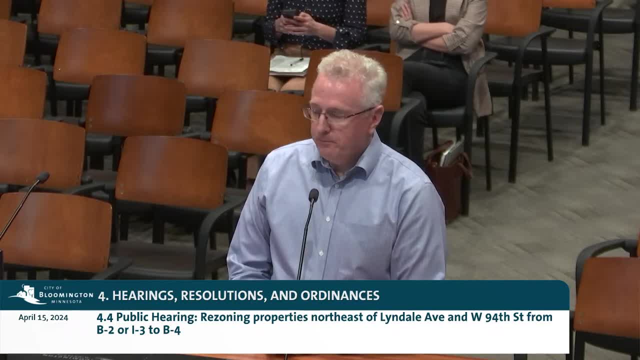 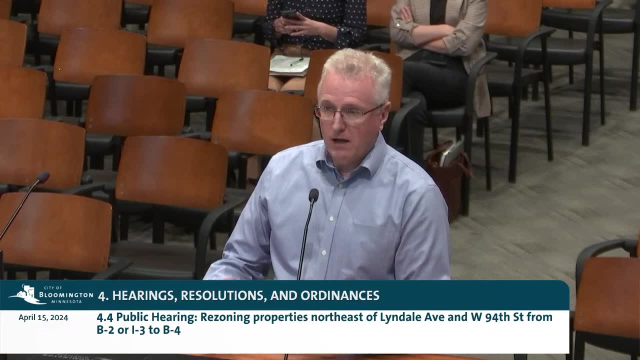 SERVICE FACILITIES, AUTO DEALERSHIPS, AND THEN, BEYOND THAT, THE BEFORE DISTRICT HAS SOME DRIVE THROUGH DISTRICTS. WHILE IT ALLOWS DRIVE THROUGHS IT HAS SOME TAMING STANDARDS IN THE WAY THAT YOU DESIGN THE. 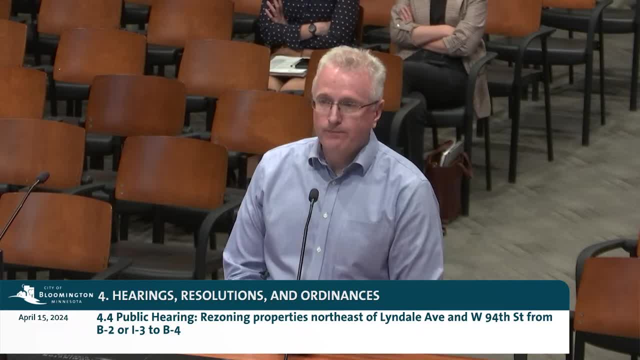 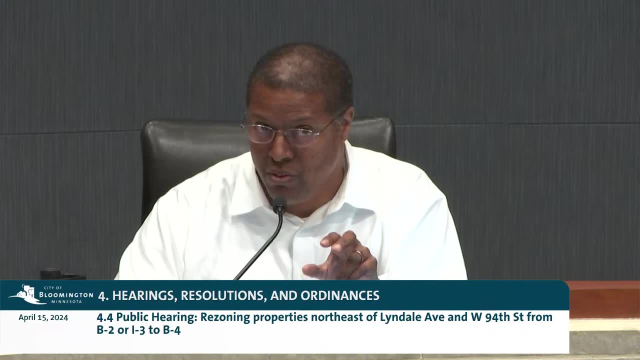 DRIVE THROUGHS THAT MAKE IT A LOT MORE PEDESTRIAN COMPATIBLE. SO I GET THAT, BUT MY QUESTION IS: IS THERE ONE THAT WOULD BE MORE URBAN, AS OPPOSED TO THE B-2, B-4?? 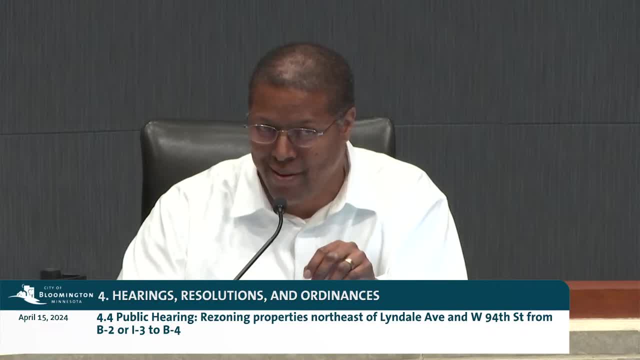 IS THERE SOMETHING ELSE THAT GETS ME EVEN MORE URBAN THAN THIS? MAYOR, BUSSY, COUNCILMEMBER, LONELAND, THERE ARE A FEW DISTRICTS, HOWEVER THE STANDARDS IN THOSE. 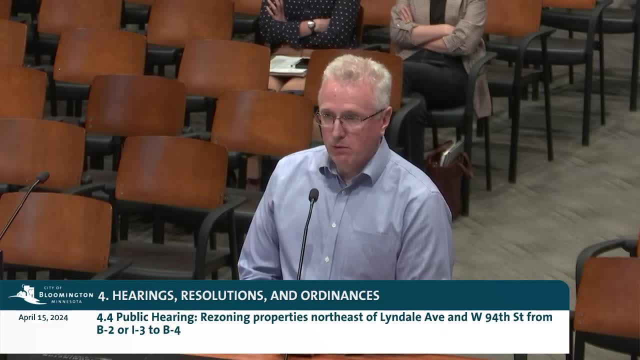 ARE SO HIGH IN TERMS OF MINIMUM FLOOR AREA RATIO THAT WE THINK IT MAY BE CHALLENGING TO DEVELOP OR REDEVELOP THE FONGS OR LOOPIAN SITE UNDER THOSE STANDARDS, BUT THEY DO APPLY IN PARTS OF. 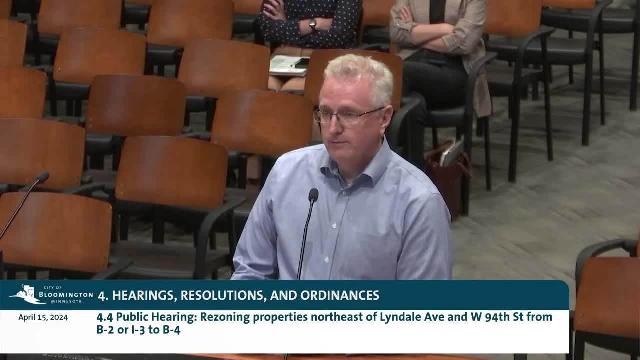 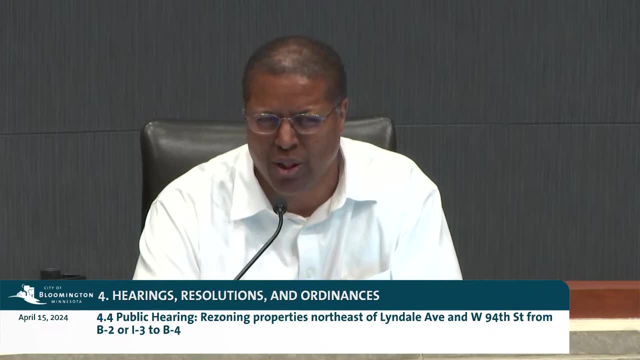 SOUTH LOOP AND THE PENN AMERICAN DISTRICT. YEAH, BECAUSE, THAT WAS WHAT I WAS THINKING OF. THE SOUTH. WHAT ARE WE DOING OVER AT SOUTHTOWN SPECIFICALLY WITH THAT? WHAT ARE WE ZONING THAT? 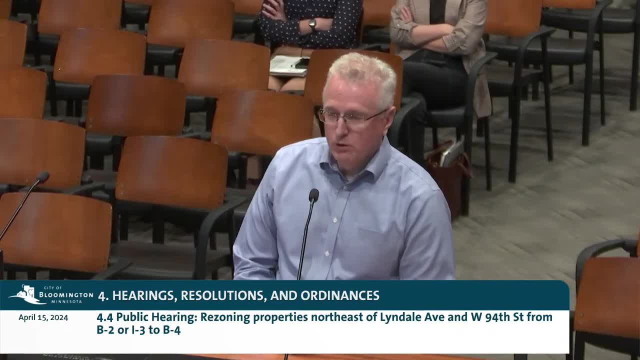 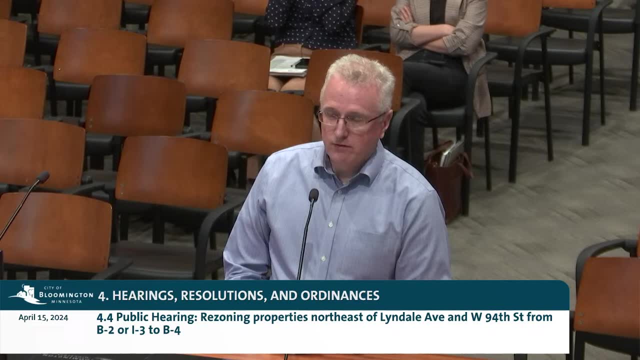 IS THAT B-4? IN THAT AREA, MAYOR, BUSSY, COUNCILMEMBER, LOWMAN, SOUTHTOWN FALLS WITHIN THREE ZONING DISTRICTS: C-3,, C-5, AND C-4.. 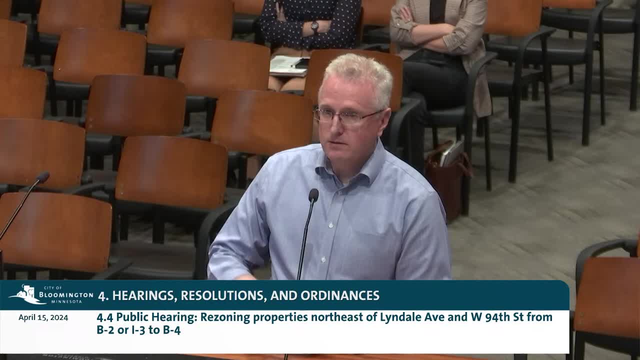 THE C-5 DISTRICT ALSO APPLIES TO A LOT OF THE PENN AMERICAN REDEVELOPMENT. THAT'S THE DISTRICT THAT HAS A PRETTY INTENSE MINIMUM FLOOR AREA RATIO THAT WE THINK WOULD JUST BE CHALLENGING TO ACHIEVE. 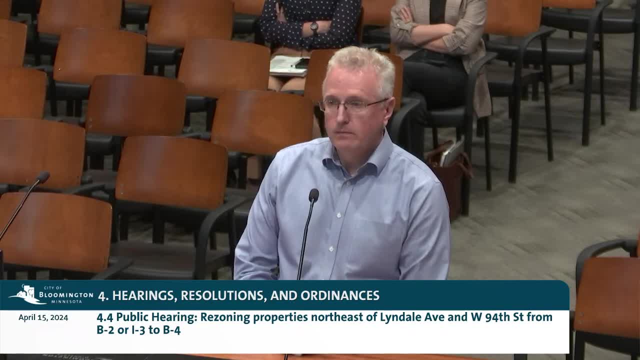 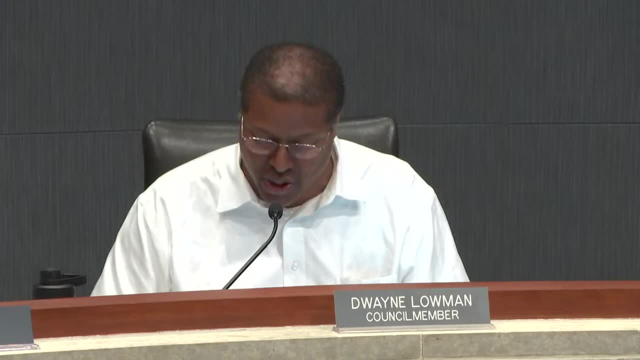 AT THE FONG SITE. THANKS, THANKS FOR THAT CLARIFICATION. IT ALMOST SEEMS TO ME- AND I KNOW THIS IS BEYOND THE SCOPE OF THIS PARTICULAR DISCUSSION- THAT MAYBE WE MAY WANT TO LOOK. 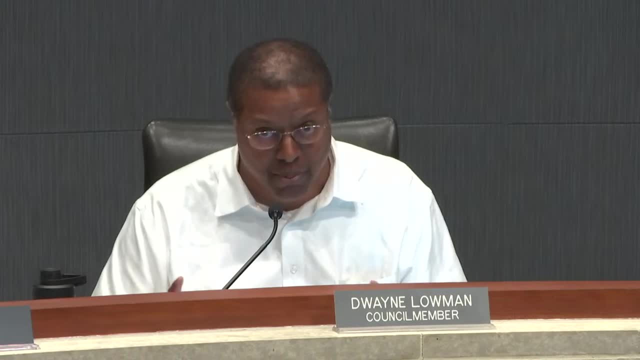 AT A DIFFERENT ZONE, BUT GIVEN WHAT I'VE HEARD TONIGHT, B-4 SOUNDS LIKE THE MOST REASONABLE DECISION, AND THAT'S WHAT STAFF CAME FORWARD WITH TODAY COUNCIL ADDITIONAL. 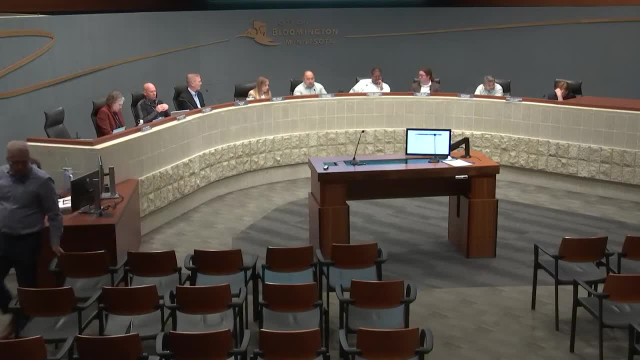 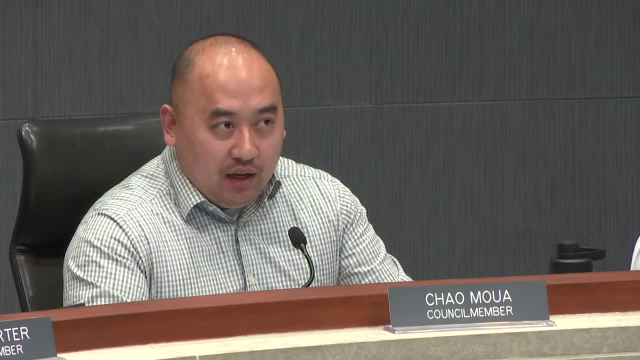 COUNCILMEMBER MUA. THANK YOU, MAYOR. MY CONCERN WITH THIS IS WHAT WE'VE SEEN WITH: THE RESIDENTIAL PIECE OF IT AND HOW RESIDENTIAL BECOMES THE MAJORITY OF IT. AND 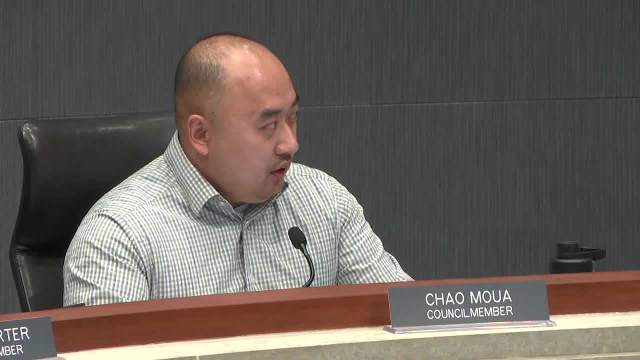 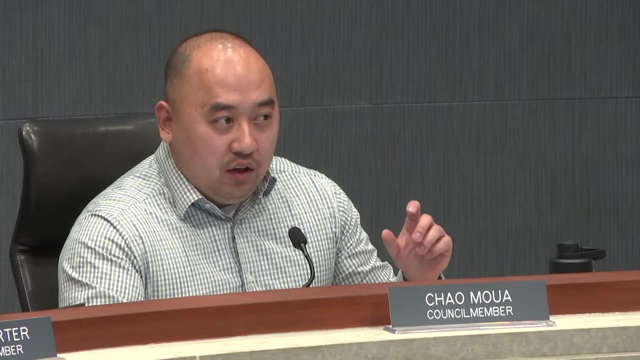 THEN THE COMMERCIAL ASPECT GETS SHRUNK. SO WHAT I WOULD NOT LIKE TO SEE IS THIS GETS REZONED TO B-4, PLANS COME IN, INCLUDES RESIDENTIAL, AND THEN THE MARKET ALL OF A SUDDEN CAN'T. 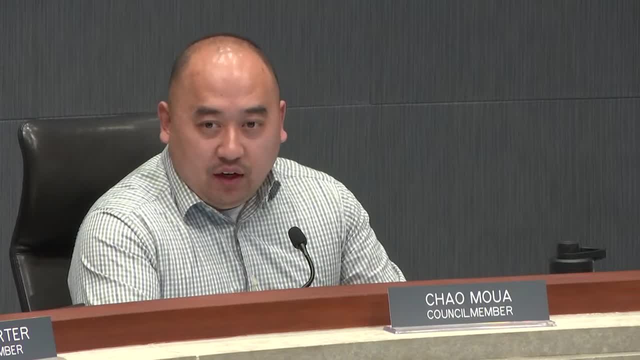 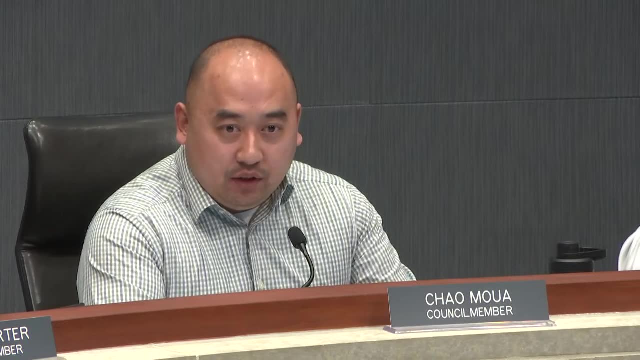 SUPPORT MORE COMMERCIAL AND WE HAVE TO SHRINK IT, WHICH TAKES AWAY FROM THE WHOLE PURPOSE OF HAVING A COMMERCIAL CORRIDOR, COMMERCIAL DISTRICT AND THE WALKABILITY ASPECT OF IT OF I. 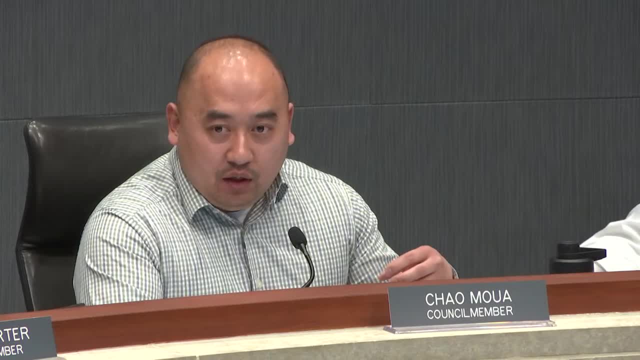 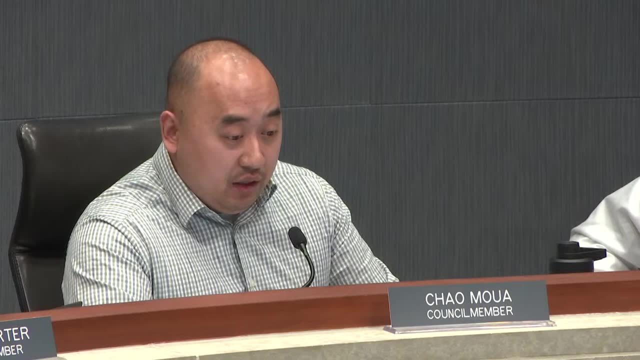 CAN LIVE IN MY HOME AND WALK AND SHOP AND VISIT BUSINESSES, AND SO I DO THINK THERE IS A DIFFERENT OPPORTUNITY ESPECIALLY FOR THIS PIECE, CONSIDERING THE DEVELOPMENT RESIDENTIALLY, THAT'S ALREADY. 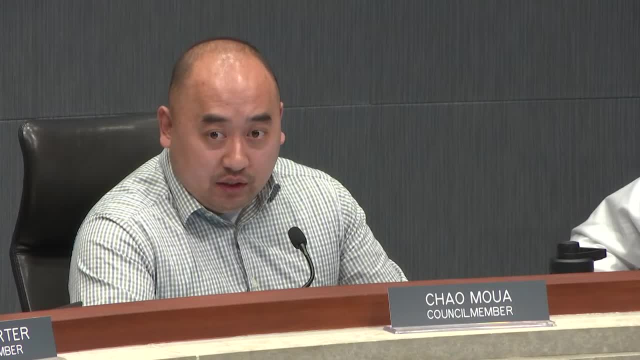 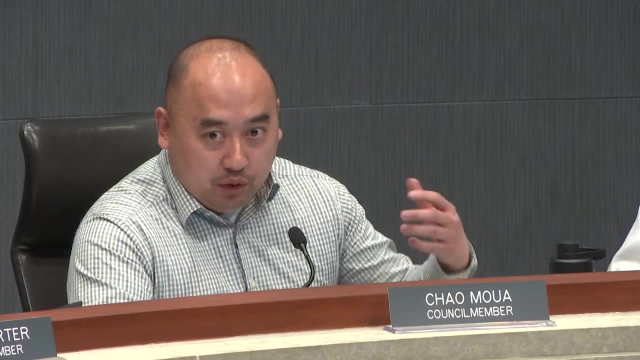 HAPPENED AROUND IT BUT TO REALLY DRIVE THE FACT THAT THIS IS A COMMERCIAL DISTRICT, AND I WOULDN'T LIKE TO SEE US TRANSITION AND HAVE THIS BE USED ALTERNATIVELY TO JUST BUILD MORE HOUSING EVEN THOUGH WE. 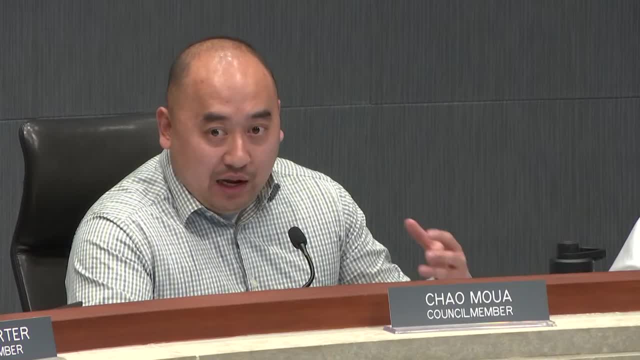 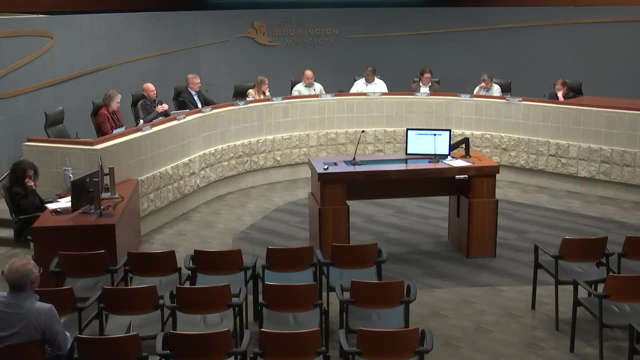 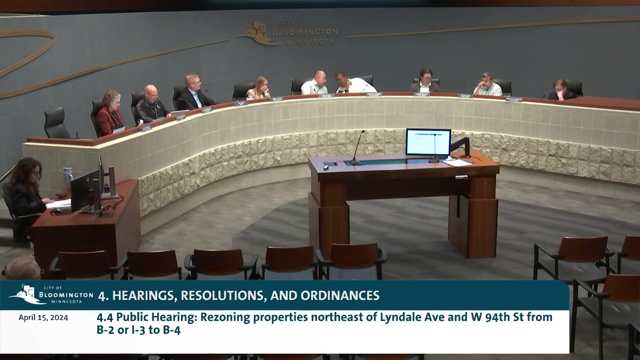 NEED MORE HOUSING, BUT IT TAKES AWAY FROM THAT. ONCE THE HOUSING PIECE BECOMES THE PRIMARY OBJECTIVE. ANYTHING ELSE COUNCIL ALL RIGHT. WE'VE HEARD A COUPLE. 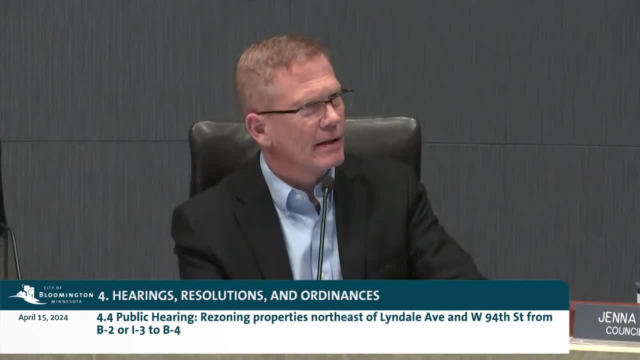 OF THINGS. IF THE COUNCIL IS COMFORTABLE WITH THE B-4 RECOMMENDATION BY STAFF, I'D LOOK FOR ACTION ON THIS IF THERE WOULD BE SOMETHING ELSE THAT WE WOULD WANT TO. 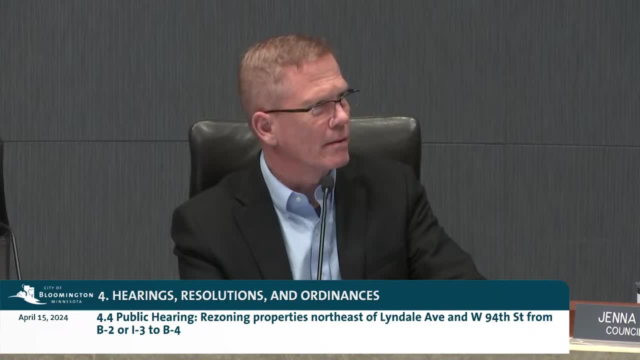 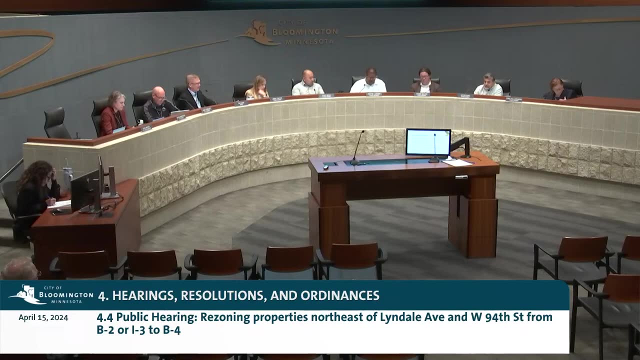 CONSIDER ON THIS. I'D ENTERTAIN THAT AS WELL, BUT HESITANTLY COUNCIL MEMBER LOMAN, YEAH. SO I THINK WHAT THE IDEA HERE IS. GIVEN C-4 WOULD BE AN EXAMPLE OF SOMETHING THAT. 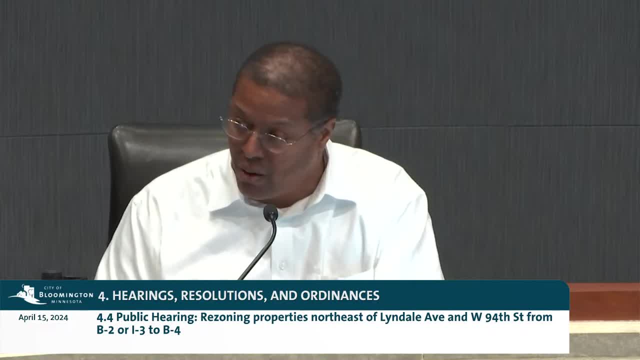 WOULD FIT WHAT COUNCIL MEMBER MUA IS TALKING ABOUT, AND SO LET'S CONSIDER C-4.. I KNOW YOU'RE RELUCTANT TO DO IT, BUT LET'S JUST GET IT OUT THERE. LET'S ASK THE QUESTION SO WE. 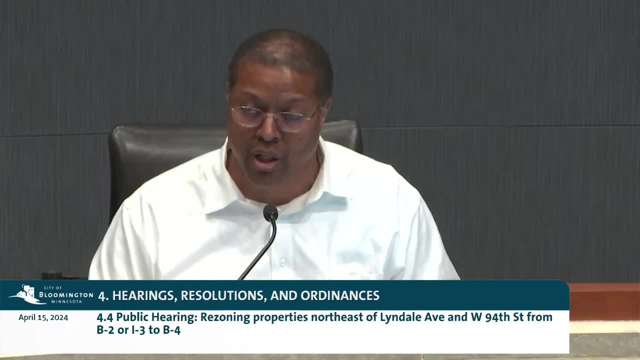 CAN QUICKLY RESOLVE THIS AND SEE WHAT ISSUES WE WOULD HAVE WITH THE C-4.. I AGREE WITH COUNCIL MEMBER MUA IN TERMS OF WHAT WE'RE TRYING TO DO THERE AND MY CONCERNS THERE, AND I THINK THIS. 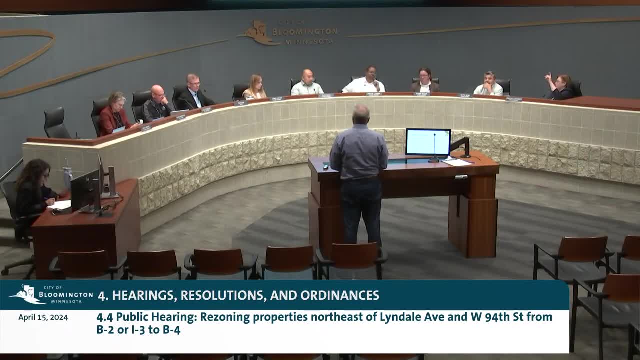 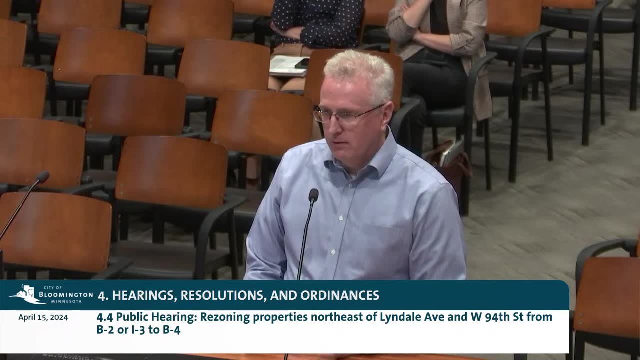 ALSO ADDRESSES SOME OF THE WALKABILITY PIECES: MR MARKERGUARD, YEAH, MAYOR BUSY, COUNCIL MEMBER, MUA. ONE THING TO POINT OUT ABOUT THE B-4 DISTRICT AND THE OTHER MIXED. 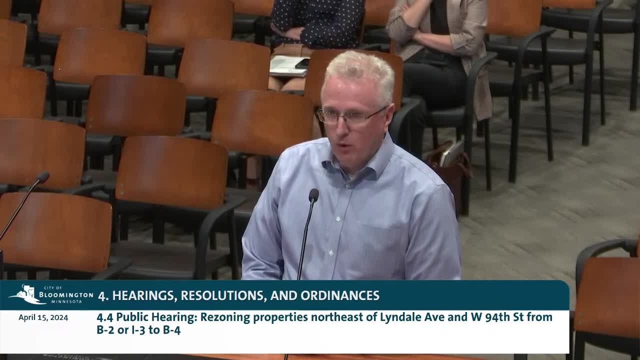 USE DISTRICTS IN BLOOMINGTON IS THAT THEY DO REQUIRE A MINIMUM LEVEL OF NON-RESIDENTIAL USE WHILE THEY ALLOW RESIDENTIAL, THEY ALSO REQUIRE, YOU KNOW, X AMOUNT OF NON-RESIDENTIAL IT VARIES BY DISTRICT. 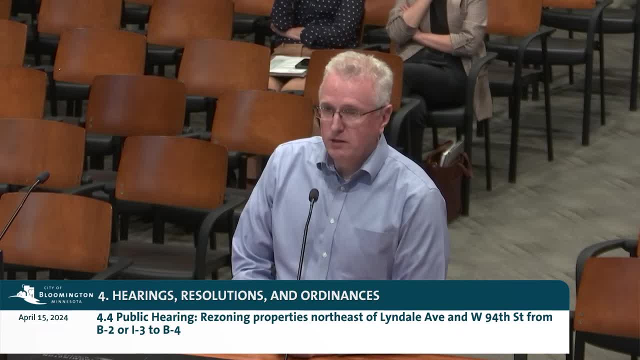 PEOPLE CAN REQUEST FLEXIBILITY TO THAT, BUT IT WOULD BE A DISCRETION UP TO THE DISCRETION OF THE COUNCIL, WHETHER OR NOT TO GRANT THAT FLEXIBILITY TO REMOVE THE COMMERCIAL OR LOWER IT SUBSTANTIALLY. 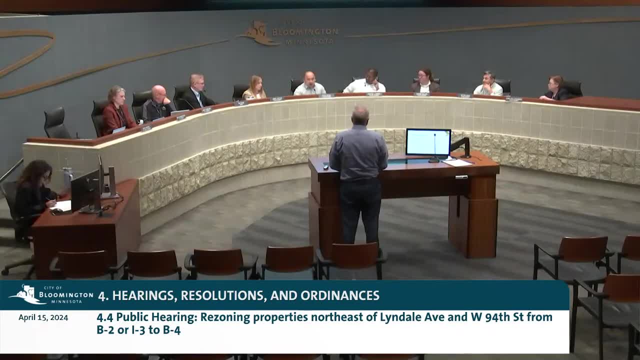 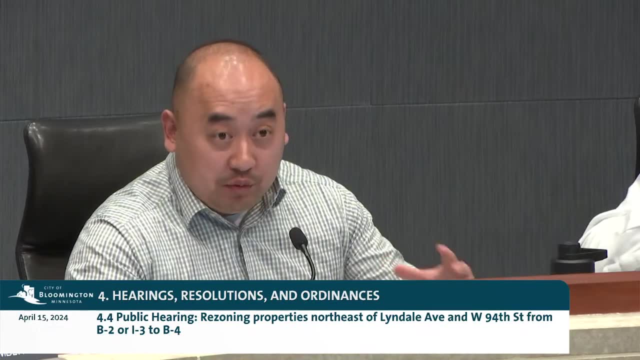 AND THAT HAS BEEN MY CONCERN IS: WE HAVE BEEN ALLOWING THE REDUCTION AND CONTINUING TO ALLOW THE REDUCTION, WHICH, TO ME, TAKES AWAY FROM THE PURPOSE OF WHAT B-4 IS MEANT TO DO. 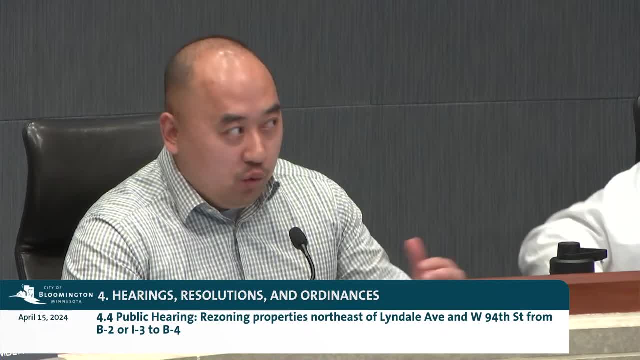 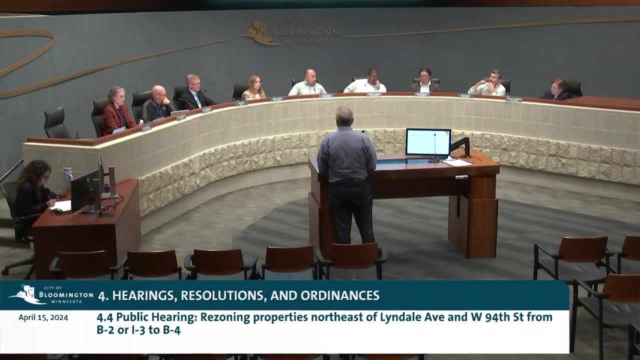 SO THAT'S WHERE MY CONCERN IS. I DON'T WANT TO SEE US CONTINUE ON THAT PATH OF REDUCING AND REDUCING, AND REDUCING ALONG THAT. THANK YOU, COUNCILMEMBER DEL ALESSANDRO. 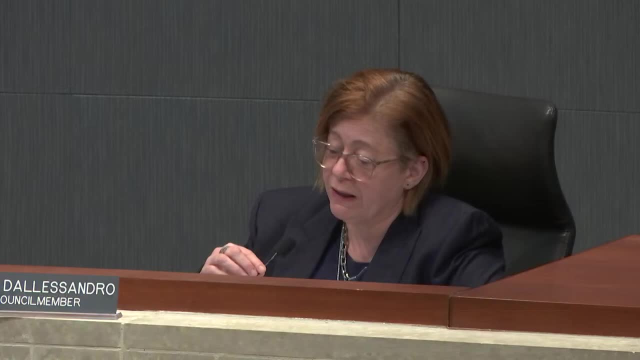 THANK YOU, MR MAYOR. I UNDERSTAND THE POINT THAT COUNCILMEMBER MUA IS MAKING. IF I REMEMBER CORRECTLY, THE ONLY TIMES THAT WE HAVE DONE THAT HAS BEEN UNDER THE OPPORTUNITY HOUSING ORDINANCE. 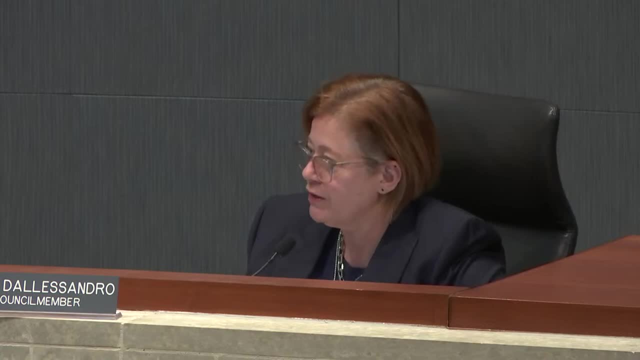 WHERE WE USED IT TO BROKER THE AFFORDABLE HOUSING UNITS, AND SO I THINK THAT'S A FAIR POINT. BUT I THINK WE HAVE TO THINK ABOUT THE GOOD ASSOCIATED WITH THAT, AND IF OUR CHOICES ARE NINE. 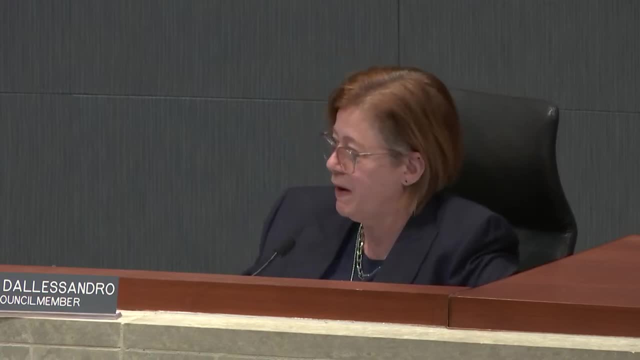 AFFORDABLE UNITS VERSUS 1500 SQUARE FEET OF COMMERCIAL SPACE. I THINK WE SHOULD WEIGH THAT ON A CASE-BY-CASE BASIS AND SOMETIMES THAT MAKES SENSE AND SOMETIMES THAT DOESN'T. 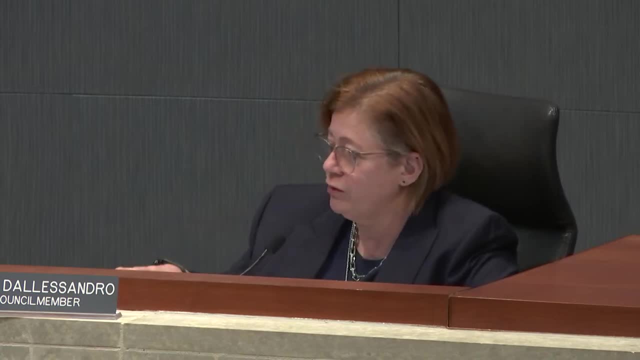 I REMEMBER, FOR EXAMPLE, WHEN WE TALKED ABOUT THE 8200 HUMBOLT NOBLE APARTMENTS. WE DIDN'T GET ANY COMMERCIAL SPACE THERE, AND I WAS SAD ABOUT THAT, BECAUSE I REALLY WANTED A COFFEE. 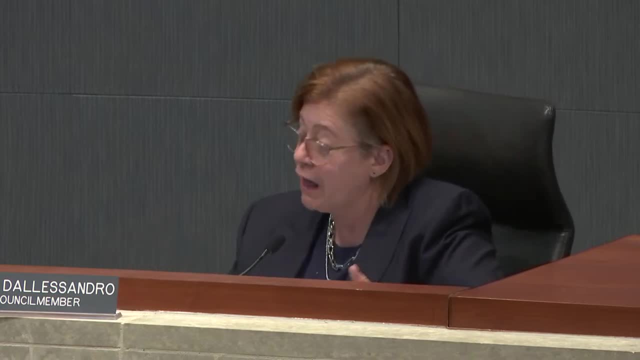 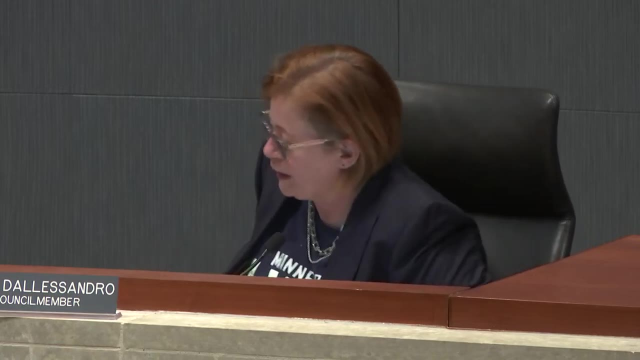 SHOP THAT I COULD WALK TO, BUT WHAT WE DID GET WAS 10% OF THOSE UNITS AT A RATE OF 50%, I THINK, OR SOMETHING LIKE THAT. SO IT WAS EVEN BETTER THAN OUR NORMAL, YOU KNOW, 80, 60%. 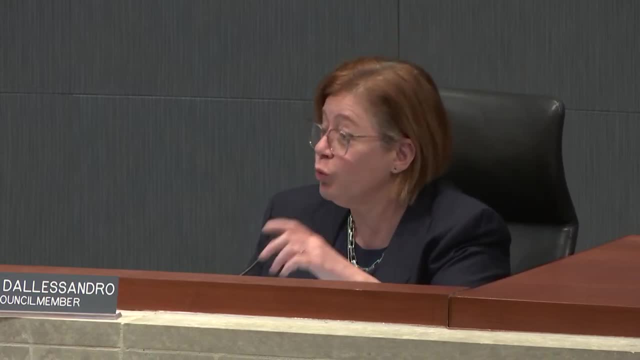 I MIGHT HAVE THAT WRONG, BUT YOU KNOW, I AGREE COMPLETELY THAT WE CAN MAKE SOME TRADE-OFFS, BUT I DON'T THINK THAT WE'VE EVER- AND FORGIVE ME IF THIS IS INCORRECT, MR MERKERGARD, I 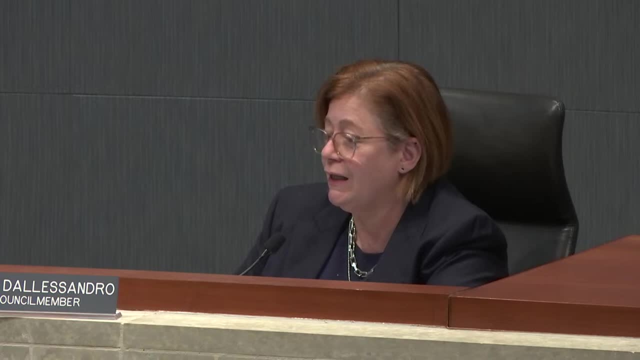 DON'T THINK WE'VE EVER SAID YOU DON'T HAVE TO HAVE ANY AT ALL, UNLESS WE WERE MAKING A TRADE AGAINST THE OPPORTUNITY HOUSING ORDINANCE, AND THAT'S JUST A COMPETING PRIORITY QUESTION. 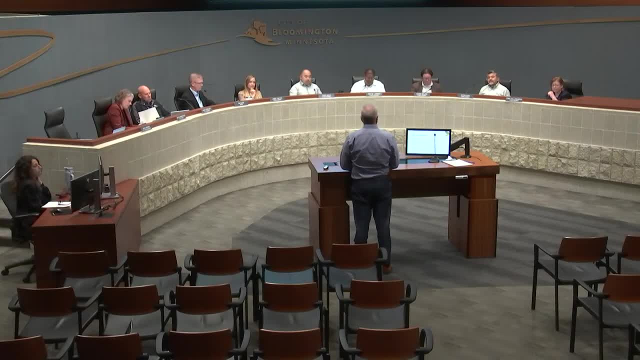 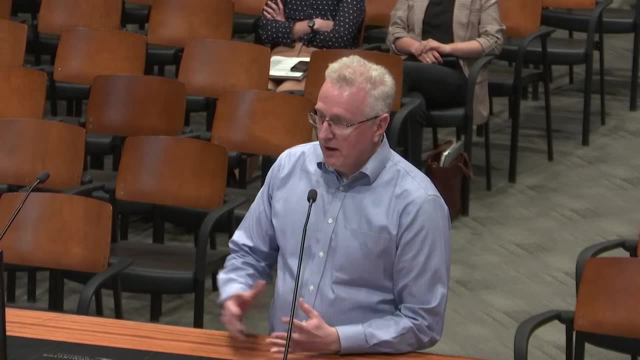 AND I AGREE WITH YOU COMPLETELY ON THAT FRONT. DO I HAVE THAT RIGHT? MAYOR BOYCE, COUNCILMEMBER D'ALESSANDRO, THAT'S CORRECT. THE SAME THING, THE SAME THING. I THINK THE CITY HAS NEVER GONE TO ZERO ON THE NONRESIDENTIAL REQUIREMENT, HOWEVER MANY SITES HAVE BEEN REZONED TO MULTI-FAMILY RESIDENTIAL AS OPPOSED TO A MIXED USE DISTRICT. SO FOR EXAMPLE, THE OTHER TWO. 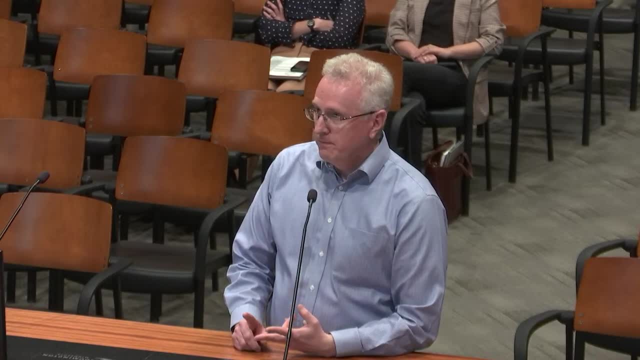 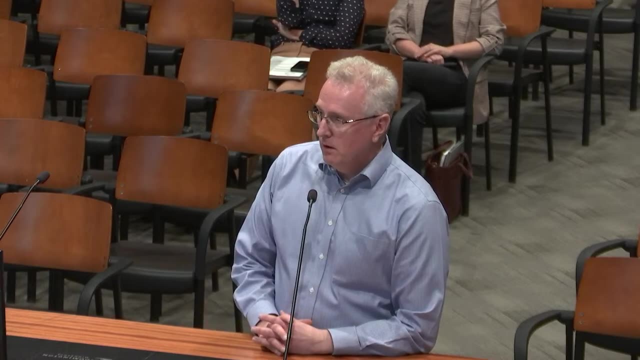 PROJECTS UNDER DEVELOPMENT IN THIS NODE. OXBURGH HEIGHTS AND LINDALE FLATS- BOTH WERE REZONED TO A MULTI-FAMILY DISTRICT, SO THEY HAVE NO COMMERCIAL AT ALL. WOULD WE CONSIDER DOING THIS. 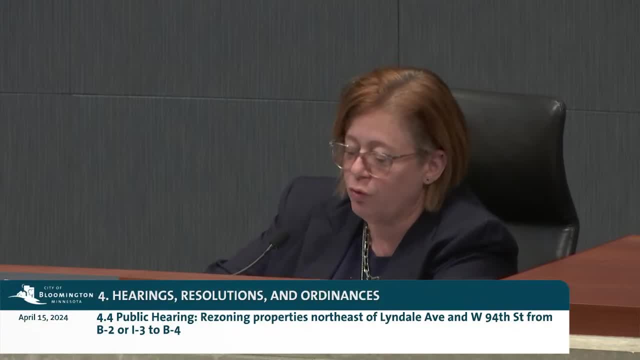 CHANGE FROM B2 TO B4 OR I3 TO B4 AND THEN TURN AROUND AND CHANGE IT AGAIN. I MEAN, I GUESS TECHNICALLY WE COULD BUT WOULD WE IF THE POINT OF THIS PARTICULAR MOVE TONIGHT IS TO CREATE A 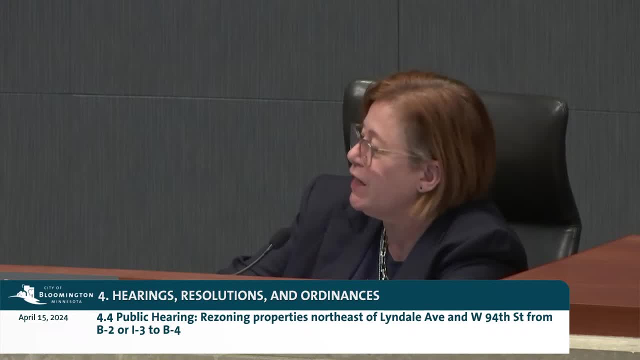 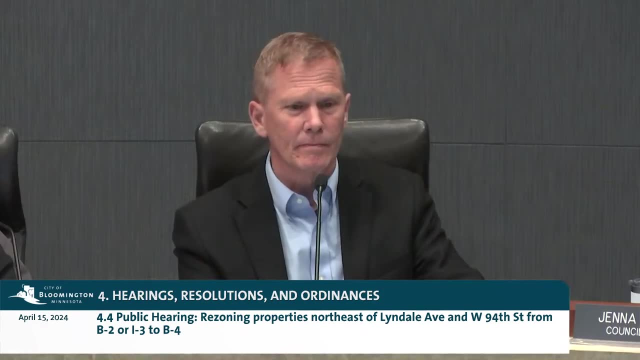 ZONE OF OPPORTUNITY, THAT'S OF A CERTAIN SIZE THAT WILL ENABLE DEVELOPMENT. I THINK COUNCIL MEMBER. I THINK TECHNICALLY, YES, WE COULD. I THINK, PRACTICALLY, ZONING IS. 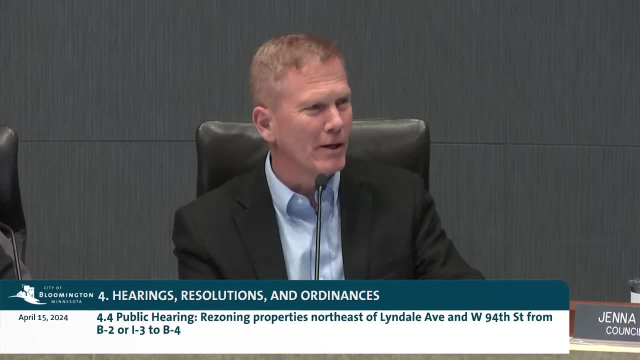 A LONG GAME. YOU PLAY THE LONG GAME. YOU DON'T PLAY IT FOR TOMORROW, YOU PLAY IT FOR TEN YEARS FROM NOW, OR FIVE YEARS FROM NOW, AND I THINK TO UNDERSTANDING THE CONCERNS THAT COUNCIL. 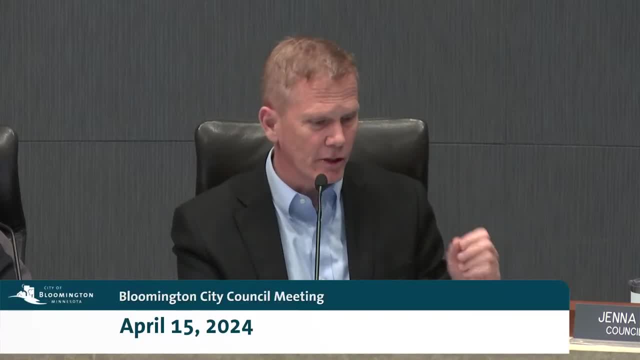 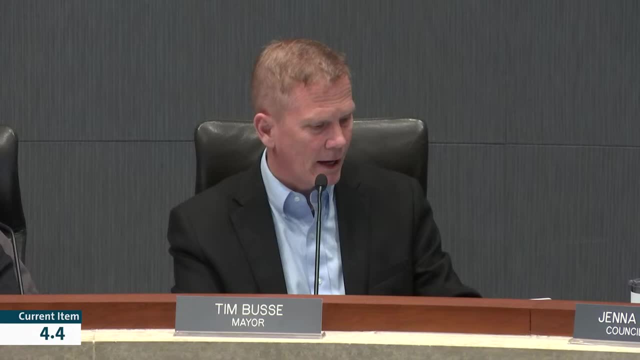 MEMBERS MUA AND LOMAN HAVE BROUGHT UP AND HAVE BEEN AND ARE CERTAINLY LEGITIMATE. I DO THINK, THE WAY THE B4 IS WRITTEN, TO HAVE THE MIXED USE AND MIXED USE OPPORTUNITIES. I DON'T THINK. 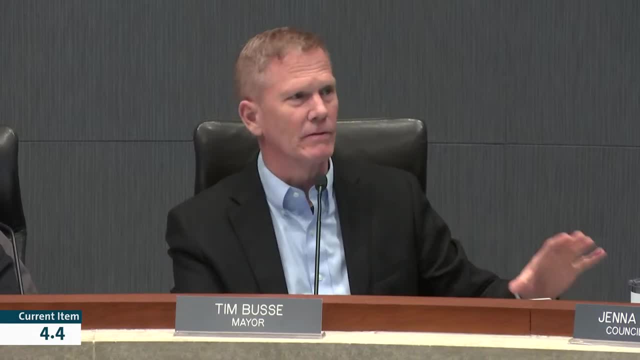 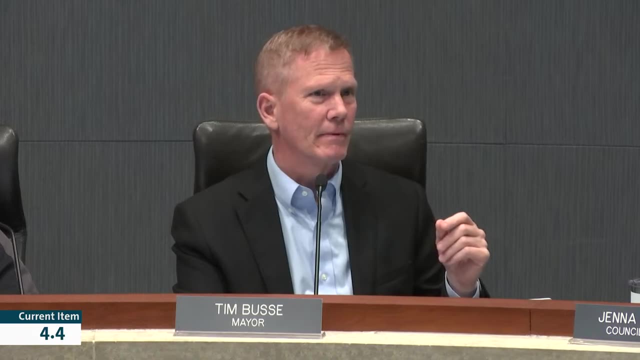 IT WOULD COMPLETELY PUSH OUT ANY BUSINESS, ANY RETAIL POSSIBILITIES, COMPLETELY IN FACT. I THINK WE HAVE SEEN THE MORE THAT WE'VE BEEN TALKING ABOUT THE MORE HOUSE, THE MORE ROOFTOPS THERE ARE. 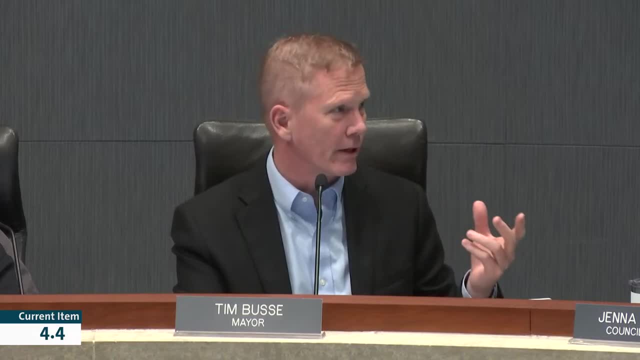 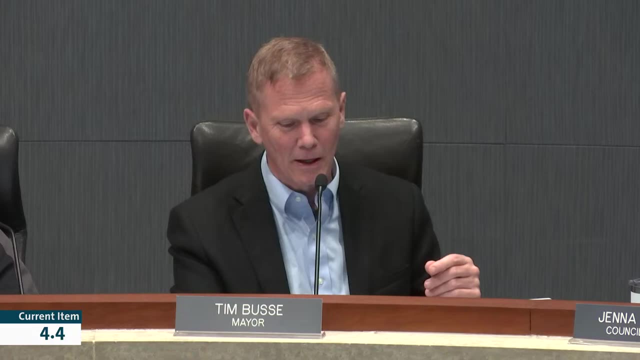 THE BETTER IN TERMS OF RETAIL, IN TERMS OF BUSINESSES MOVING INTO AN AREA- NOW WE'VE ALSO SEEN WHERE IT DOESN'T QUITE WORK OUT THAT WAY IN TERMS OF A GROCERY STORE OVER IN THE SOUTH LOOP. BUT I THINK 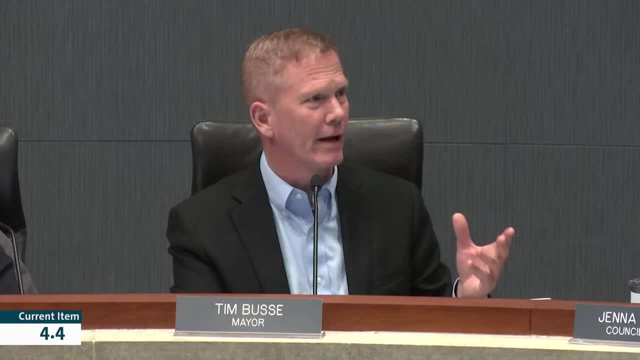 IN GENERAL, THE MORE ROOFTOPS, THE MORE PEOPLE LIVING THERE, THE BETTER THE OPPORTUNITIES FOR RETAIL TO BE LOCATED ALONG LANDALE AVENUE AND SURVIVE AND DO WELL, IT'S A MATTER, IT'S JUST A. NUMBERS GAME AND SO, IN ANSWER TO YOUR QUESTION, YES, WE COULD CHANGE IT AGAIN. BUT I THINK THE GOAL OF DOING THIS TYPE OF ZONING IS TO LOOK OUT A NUMBER OF YEARS AND LET THE MARKET KIND OF PLAY. 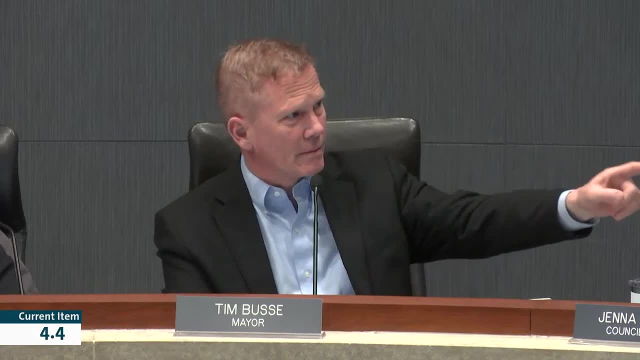 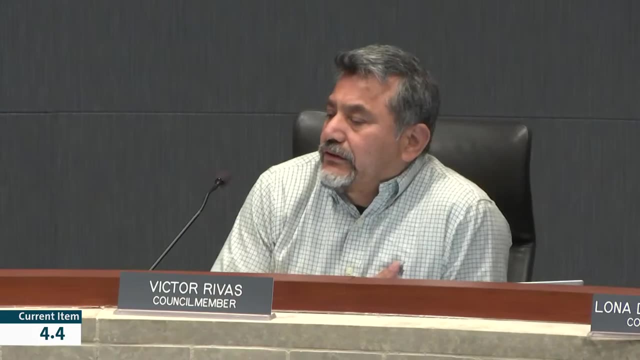 ITSELF OUT. I SAW COUNCILMEMBER RIVAS WITH HIS HANDS UP, AND THEN COUNCILMEMBER LOMA, COUNCILMEMBER RIVAS. ARE THERE ANY GUARANTEES THAT THE DEVELOPMENT WOULD ALSO? 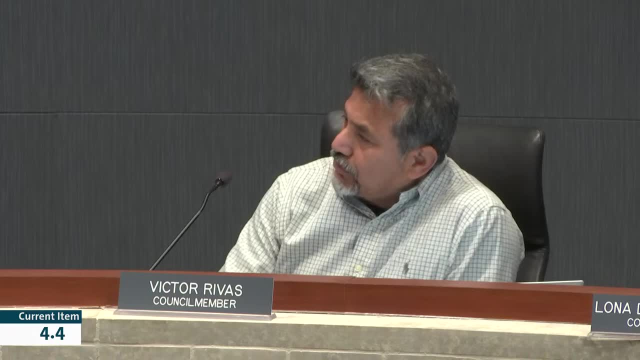 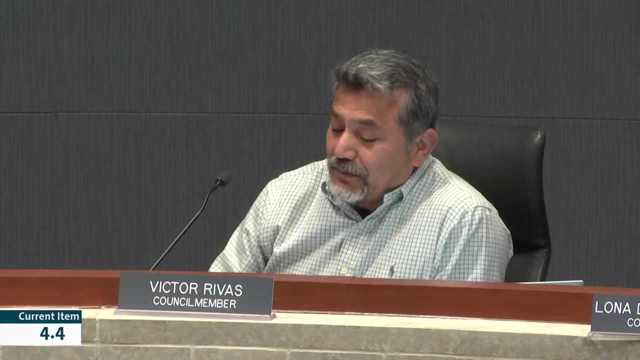 OR ANYTHING THAT IS BUILT IN THERE, WILL HAVE THE COMMERCIAL AND THE RESIDENTIAL AS QUALITY. I MEAN IT'S TO ME. I THINK B4 JUST MAKES PERFECT SENSE IN THAT AREA. EVEN THOUGH I, YOU KNOW A LOT. 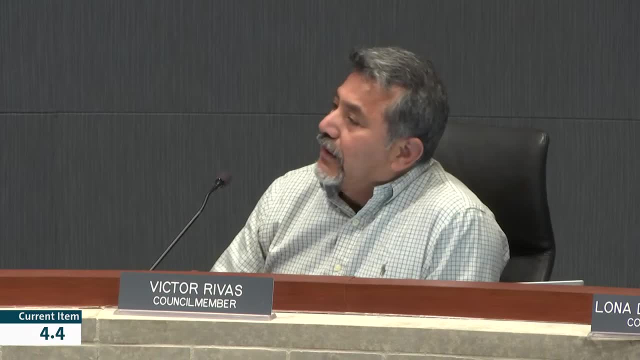 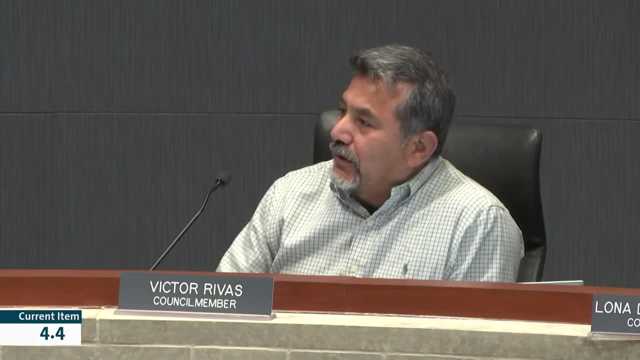 OF THE PEOPLE THAT I SPEAK TO ARE AGAINST IT. I BELIEVE THAT THE CITY DOES NEED THAT, AND IT'S ONE OF THE BEST THINGS THAT I HAVE HEARD SO FAR SINCE I BECAME A COUNCILMEMBER. THAT 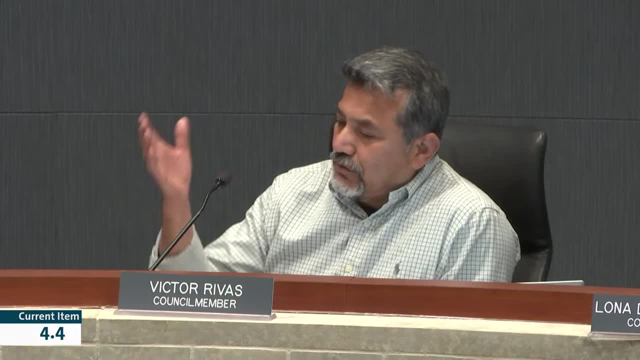 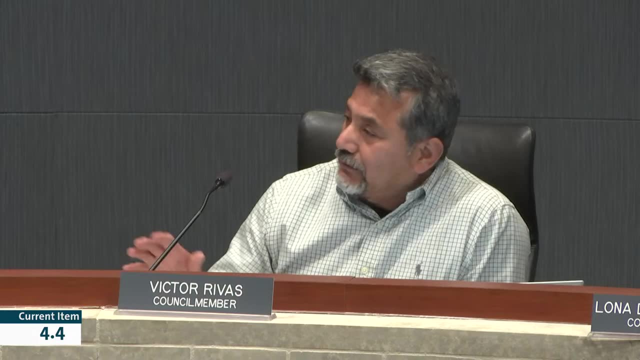 YOU KNOW B4 ACTUALLY. LIKE YOU MENTIONED, THE MORE ROOFS WE HAVE, THE MORE OPPORTUNITY FOR BUSINESS THERE IS, AND I THINK THIS IS PROBABLY SOMETHING. THAT IS MUCH MADE IN HEAVEN. 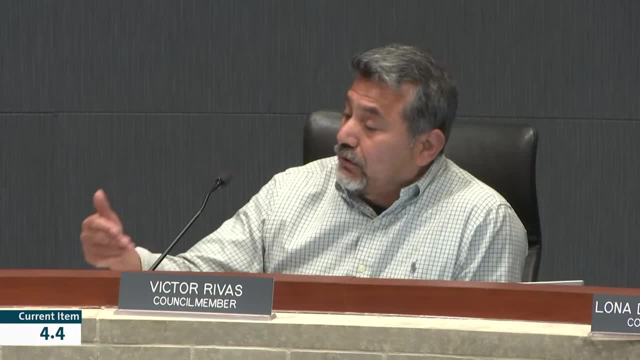 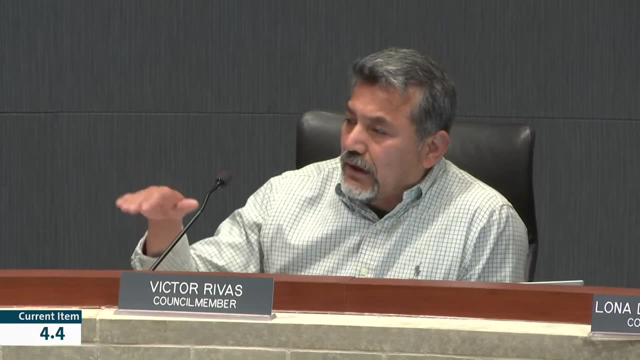 YOU KNOW, THERE IS SOME RESERVATIONS, YES, BUT IF WE ENCOURAGE THE BUILDERS- WHOEVER THE DEVELOPER IS- TO PROVIDE ANY RESIDENTIAL UNITS WITH LOWER FLOORS AVAILABLE FOR COMMERCIAL, I THINK THAT WOULD BE PERFECT. 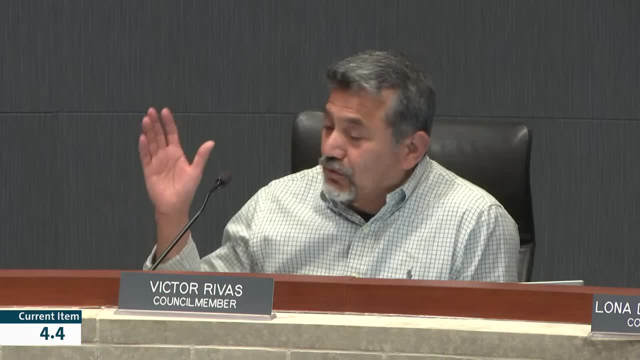 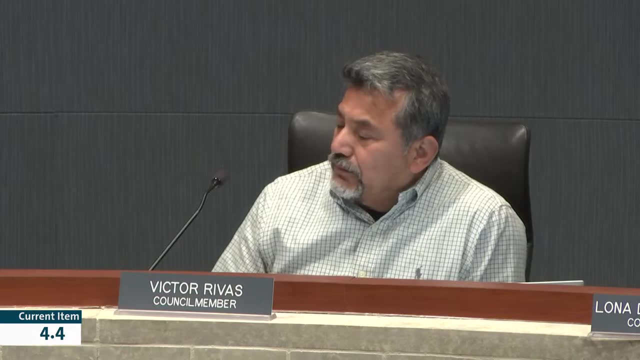 IN THAT AREA AND WE NEED IT. I MEAN THE AREA LOOKS DECREPIT ANY TIME YOU DRIVE IN THERE, SO SOMETHING LIKE THIS WOULD BE SOMETHING THAT WE NEED TO PROVIDE. SO I'M SORRY THAT I YOU KNOW. 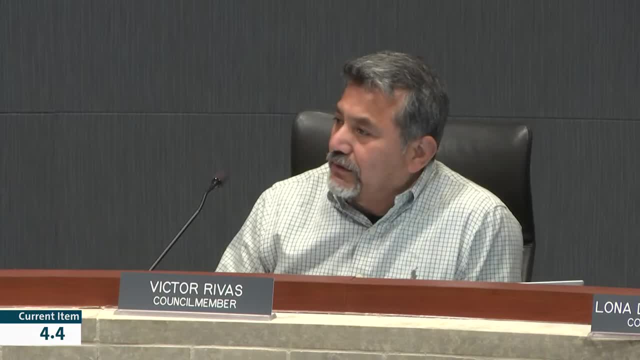 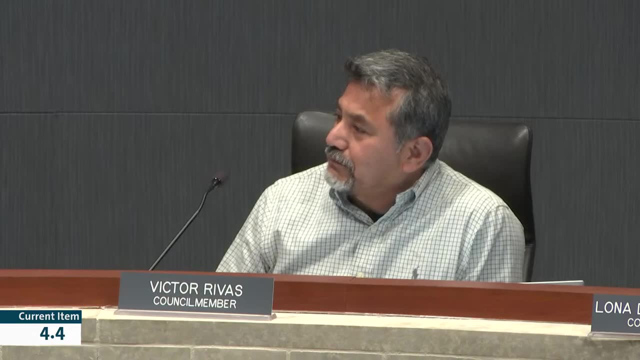 DON'T SEE EYE TO EYE WITH YOU, GENTLEMEN, BUT I THINK IT'S ONE OF THE BEST THINGS THAT I HAVE SEEN SO FAR COME UP TODAY, SO I WILL BE 100% BEHIND THIS VERY GOOD. 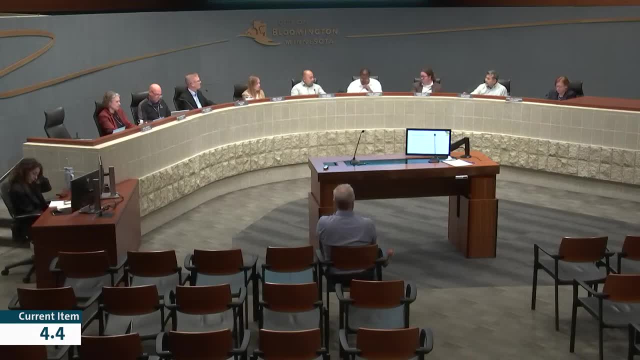 MR LOMAN: YEAH, I GOT NO PROBLEM WITH THE B-4, BUT YOU KNOW WHAT? HEY, I WANT TO SEE IF WE CAN AMEND THIS AND TRY C-4 ON THIS AND SEE IF WE'VE GOT SUPPORT. 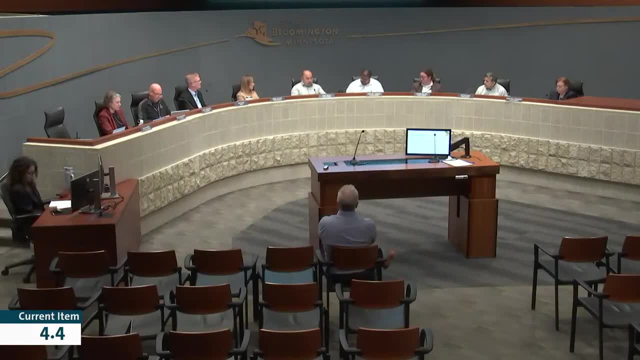 THERE. IF NOT, WE CAN VOTE IT DOWN AND MOVE ON. SO LET'S FIGURE, WE CAN JUST MOVE THIS A LITTLE QUICKER. I'LL MOVE TO AMEND THIS FROM A B-4 TO A C-4.. SECOND: 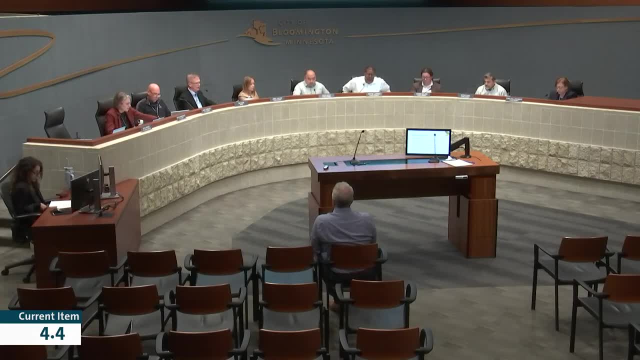 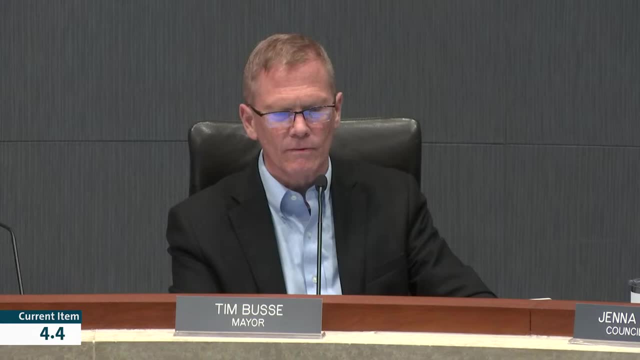 MOTION BY COUNCILMEMBER LOMAN, SECOND BY COUNCILMEMBER MUA AND, IF I'M READING THIS CORRECTLY, HE'S MOVING THAT WE APPROVE AN ORDINANCE AMENDING THE CITY'S OFFICIAL ZONING MAP. 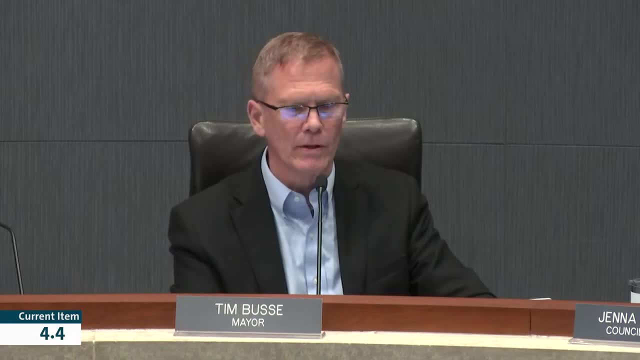 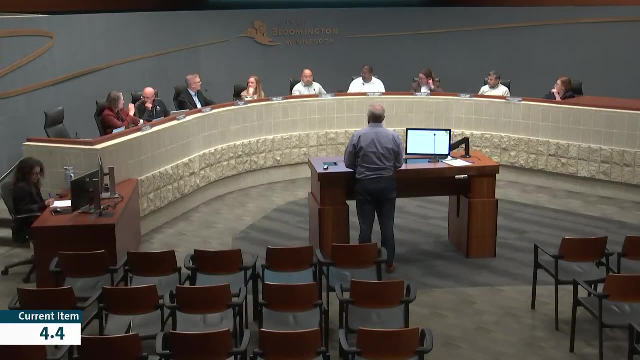 TO REZONE THE LOTS SHOWN ON EXHIBIT A, ATTACHED TO THE STAFF REPORT, TO THE C-4 DISTRICT AS OPPOSED TO THE B-4 DISTRICT. AM I STATING THAT CORRECTLY? YEP. 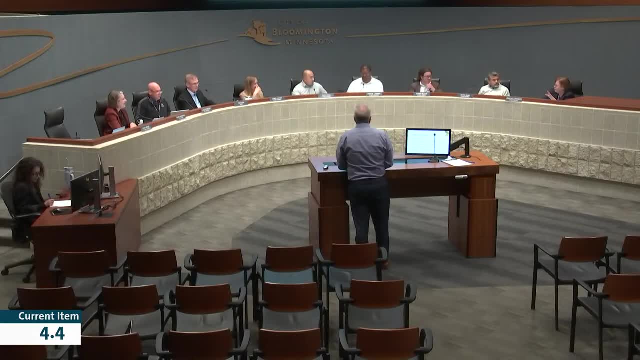 MR MAYOR, I THOUGHT I HEARD FROM MR MERKERGARD THAT THE PROPOSED PROPERTIES CAN'T QUALIFY FOR C-4 BECAUSE THEY'RE NOT BIG ENOUGH, SO LIKE THERE'S NOTHING WE CAN. 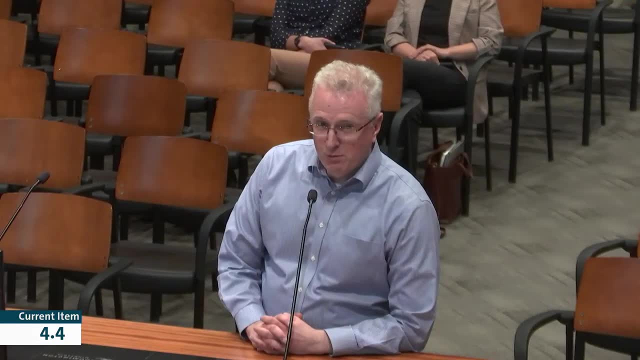 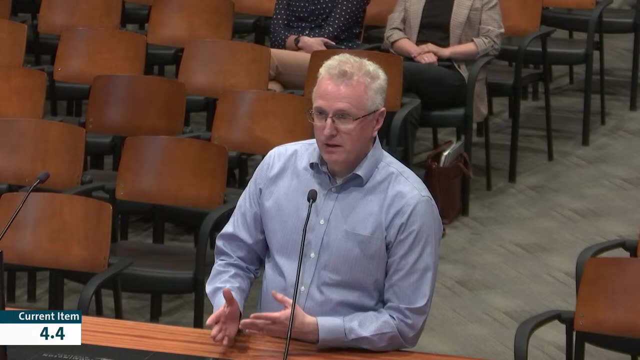 DO WITH THAT? DID? I UNDERSTAND THAT CORRECTLY, MAYOR BUSSE, COUNCILMEMBERS, I BELIEVE TO CHANGE THE ZONING DISTRICT, WE WOULD HAVE TO INITIATE REZONING TO A. 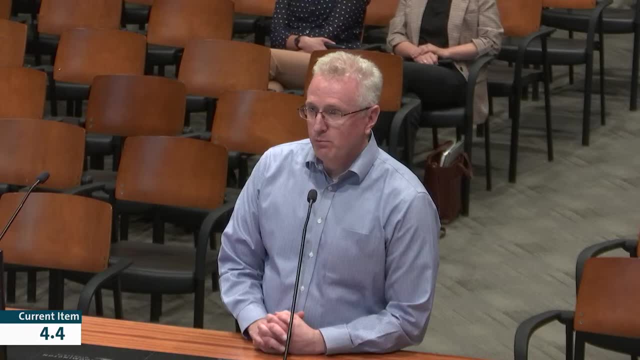 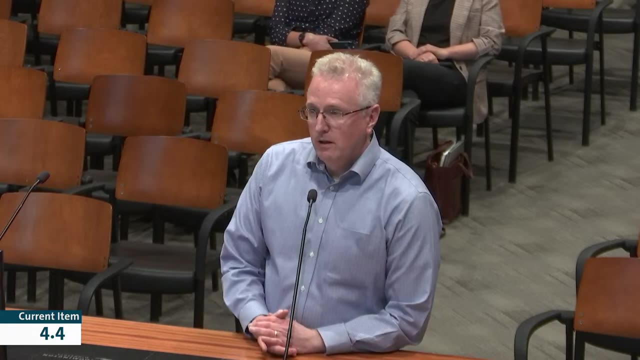 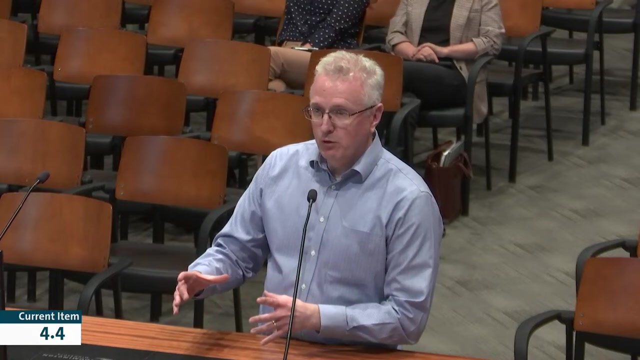 DIFFERENT DISTRICT, HAVE PUBLIC HEARINGS FOR THAT AND PROVIDE NOTICE. THE C-4 DISTRICT IS A OFFICE DISTRICT SO IT WOULD NOT ALLOW RETAIL. THE C-5 DISTRICT IS THE FREEWAY VERSION OF THE B-4 DISTRICT. 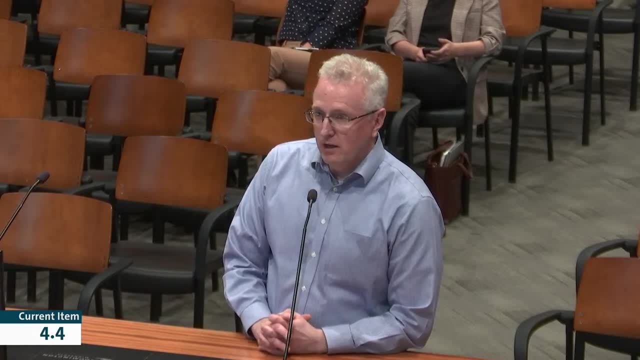 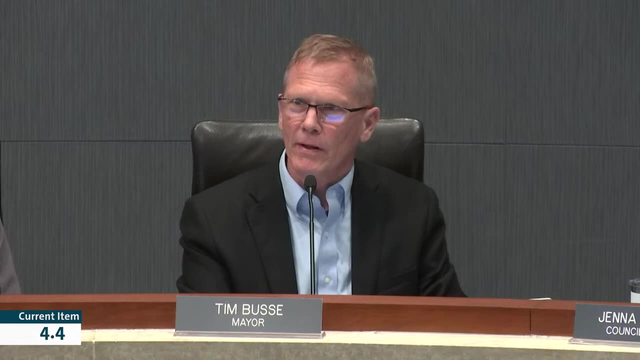 THAT HAS A LOT MORE INTENSITY. WE DO THINK IT WOULD BE CHALLENGING TO REDEVELOP UNDER THAT AT THIS LOCATION. SO THANK YOU, MR MERKERGARD, FOR CORRECTING ME THERE. IN FACT, WE WOULD HAVE TO GO. 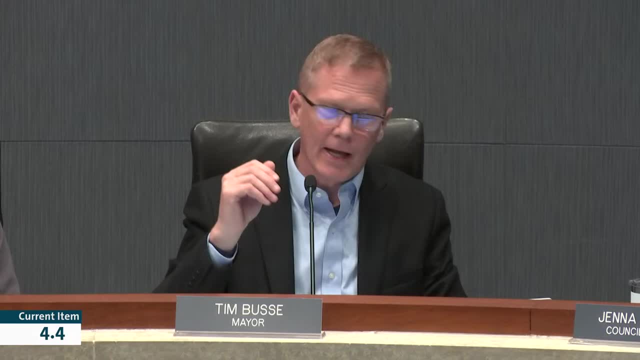 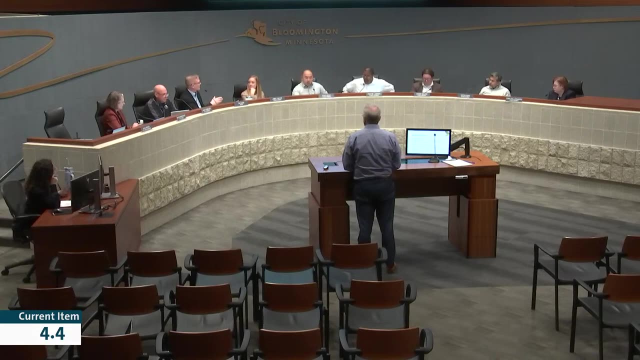 THROUGH THE WHOLE PROCESS AGAIN. I APPRECIATE THAT, AND SO I THINK WHAT YOUR MOTION WOULD BE, COUNCILMEMBER LOMAN WOULD BE TO SIMPLY REJECT THIS AND START THE PROCESS OVER AGAIN. 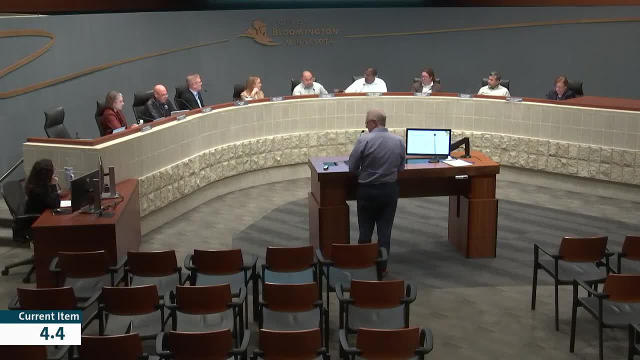 OR TO VOTE NO, OR TO VOTE NO, AND I THINK THAT'S WHAT WE'LL DO. WE'RE GOING TO WITHDRAW THAT, SO WE DON'T GET IN A BIG MESS HERE AND I'M HAPPY, UNLESS THERE'S. 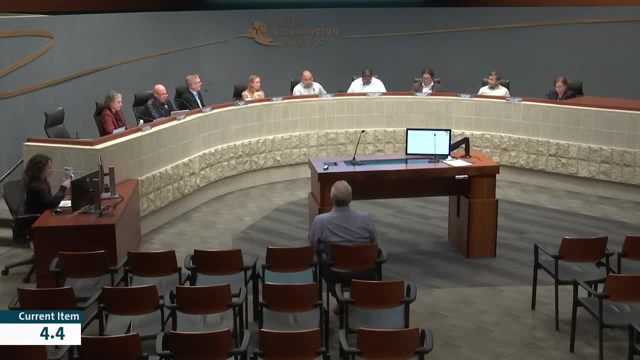 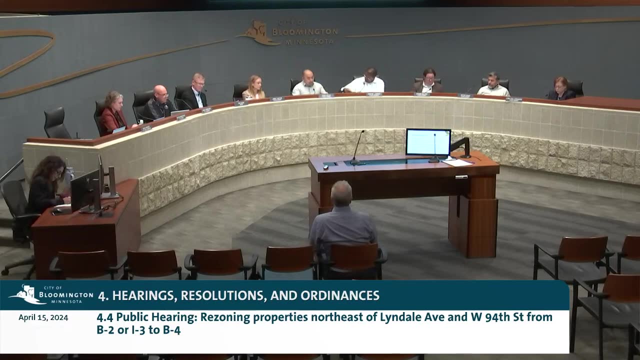 ANY MORE COMMENTS. I'M HAPPY TO MOVE THIS THING. ANY MORE COMMENTS. COUNCILMEMBER LOMAN, WHY DON'T YOU MOVE US ALONG? HERE WE GO, LET'S SEE HERE. GET TO THE MOTION HERE. 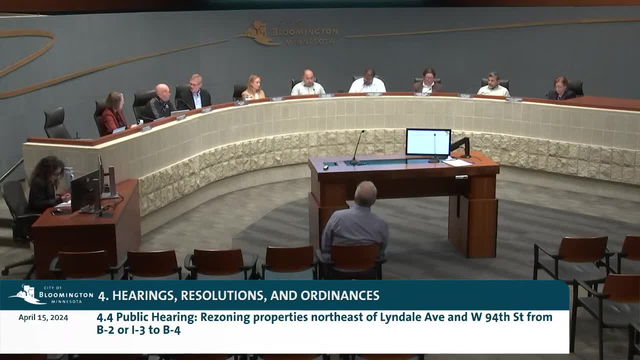 WE ALREADY CLOSED THE PUBLIC HEARING, SO I'LL MOVE TO ADOPT AN ORDINANCE AMENDING THE CITY ZONING MAP BY REZONING PROPERTIES SHOWN IN EXHIBIT A FROM B2 GENERAL COMMERCIAL OR. 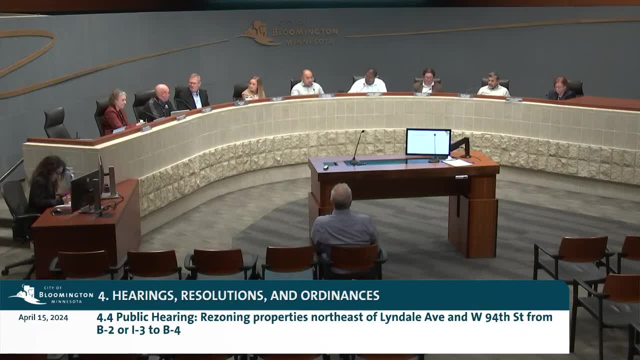 I3 GENERAL INDUSTRIAL, TO B4 NEIGHBORHOOD, COMMERCIAL. WE HAVE A MOTION. DO WE HAVE A SECOND COUNCILMEMBER DEL ASSANDO WITH A SECOND TO APPROVE THE ORDINANCE? 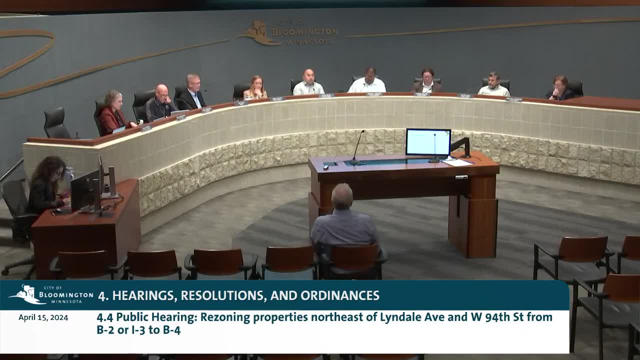 AMENDING THE CITY'S OFFICIAL ZONING MAP- REZONE EXHIBIT A TO THE B4 DISTRICT. ANY FURTHER COUNCIL DISCUSSION ON THIS? IF NOT ALL THOSE IN FAVOR, PLEASE STAND BY. 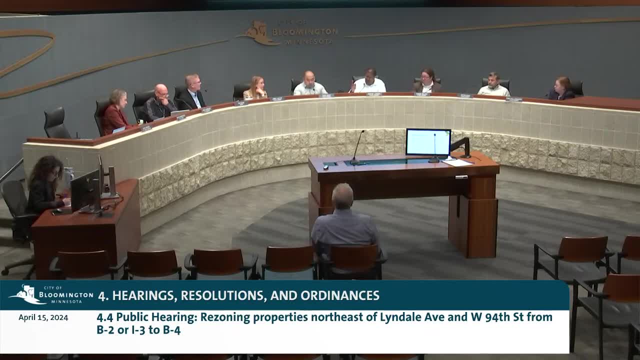 SIGNIFY BY SAYING AYE, AYE, AYE, OPPOSED, NO. SO THE MOTION CARRIES 5-2 WITH COUNCILMEMBERS LOWMAN AND COUNCILMEMBER MUA VOTING. 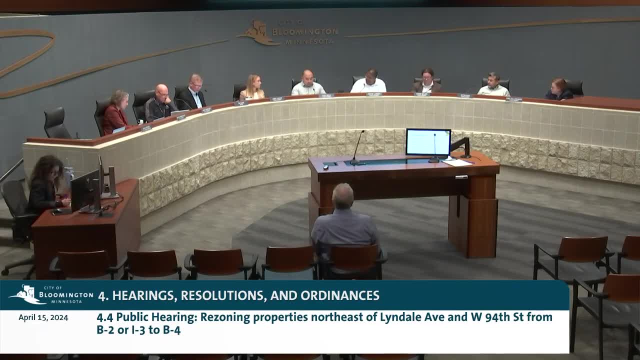 AGAINST. ARE YOU READY FOR THE SUMMARY PUBLICATION? IF YOU WOULD LIKE TO DO SUMMARY PUBLICATION, I'D BE HAPPY TO MOVE IT. GO AHEAD. I'LL MOVE TO ADOPT A RESOLUTION AUTHORIZING SUMMARY. 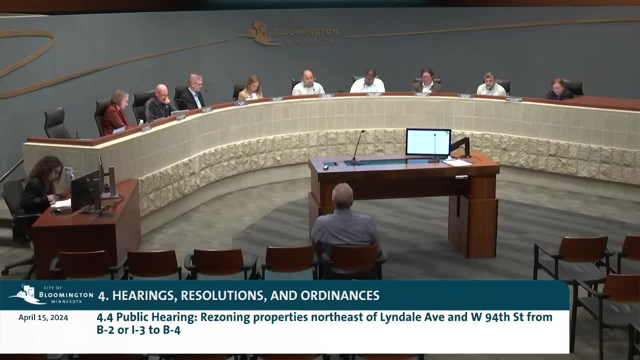 PUBLICATION OF THE ORDINANCE AMENDING THE CITY ZONING MAP BY REZONING PROPERTIES SHOWN IN EXHIBIT A, FROM B2- GENERAL- COMMERCIAL- TO I3- GENERAL INDUSTRIAL TO B4- NEIGHBORHOOD. 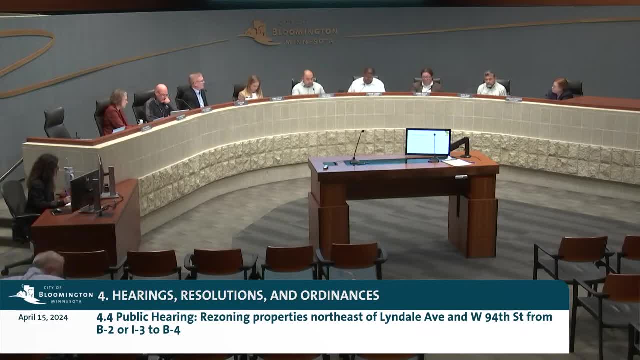 COMMERCIAL MOTION BY COUNCILMEMBER LOWMAN, SECOND BY COUNCILMEMBER DALLASANDO, FOR SUMMARY PUBLICATION ON ITEM 4.4.. NO FURTHER COUNCIL DISCUSSION. 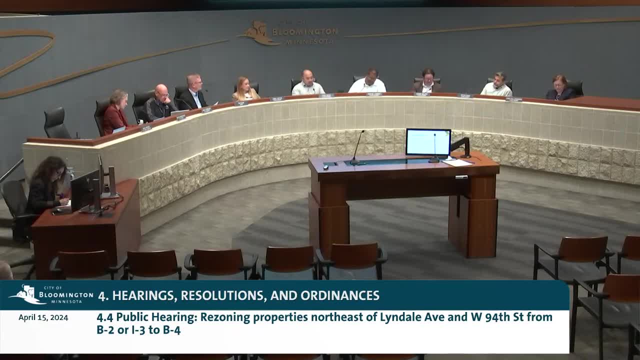 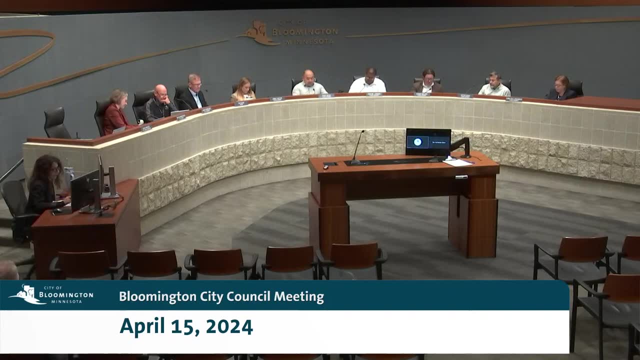 ALL THOSE IN FAVOR. PLEASE SIGNIFY BY SAYING AYE, AYE. OPPOSED MOTION CARRIES: 7-0 ON SUMMARY PUBLICATION: MR RAMLER-OLSON, THANK YOU, THANKS FOR STICKING WITH US. 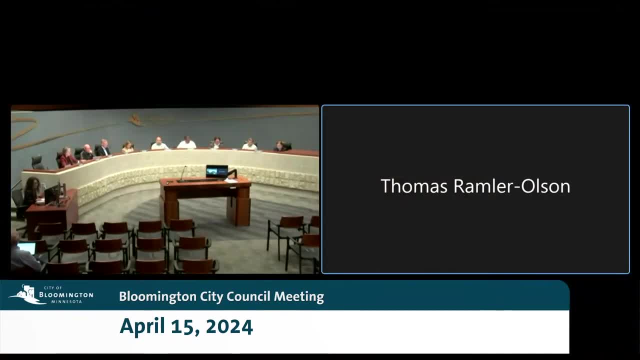 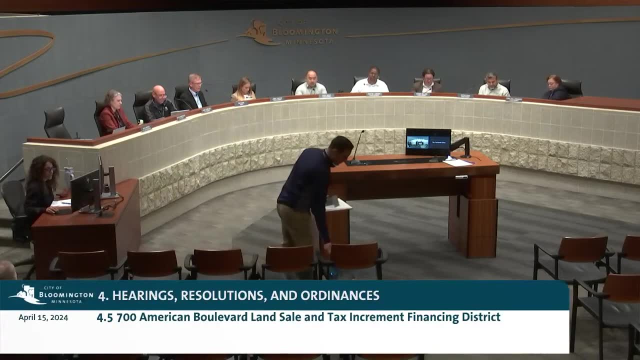 HOPE YOU'RE FEELING BETTER SOON. THANK YOU. THANK YOU, MAYOR. THANK YOU, COUNCILMEMBERS, HAVE A GOOD NIGHT. THANK YOU, YOU TOO OUR FINAL ITEM UNDER ITEM 4: THIS EVENING IS ITEM 4.5.. 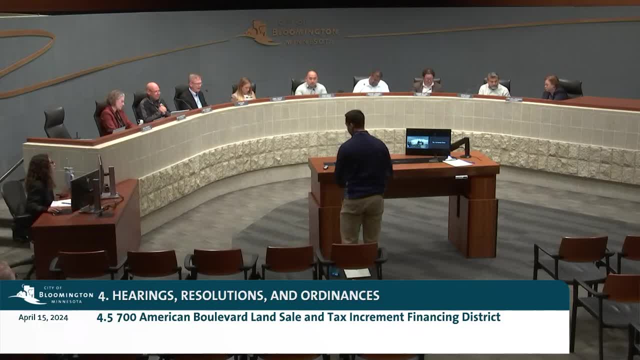 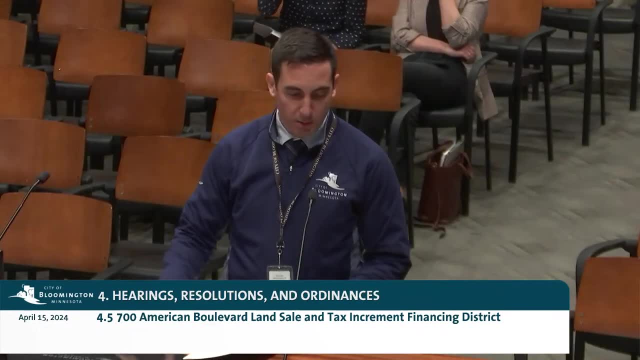 THIS IS THE 700 AMERICAN BOULEVARD LAND SALE AND TAX INCREMENT FINANCING INFORMATION. MR PALERMO, FROM OUR PORT AUTHORITY, IS HERE. GOOD EVENING AND WELCOME. THANK YOU, MR MAYOR COUNCILMEMBERS. 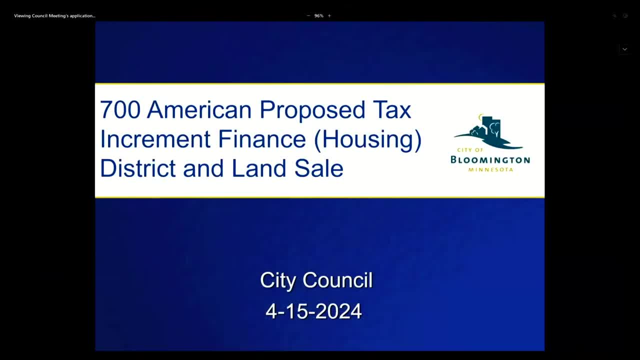 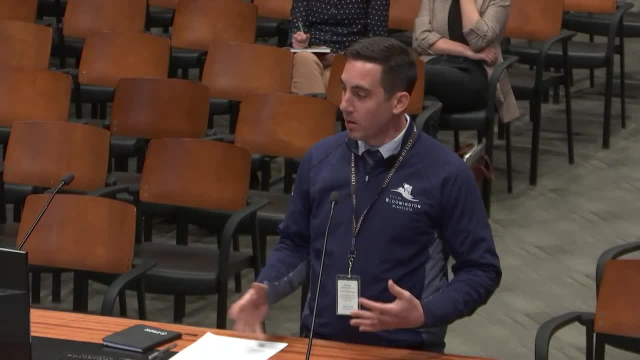 I'M HERE TODAY TO TALK ABOUT 700 AMERICAN. AS YOU MAY REMEMBER, FROM THE PAST YEAR AND A HALF ABOUT A MONTH AGO, WE TALKED ABOUT A TERM SHEET AND NOW WE'RE GETTING TO THE FINANCIAL. 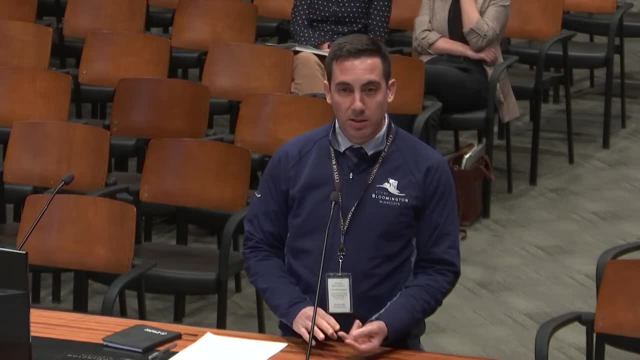 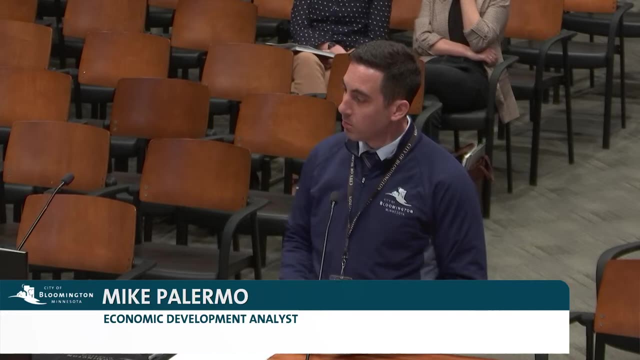 PACKAGE. SO THERE ARE TWO PUBLIC HEARINGS THAT WILL OPEN AND HOLD TONIGHT TWO SEPARATE VOTES BUT TO SIMPLIFY THINGS, WE BROUGHT IT AS ONE AGENDA ITEM. SO THE FIRST THING YOU'LL OPEN. 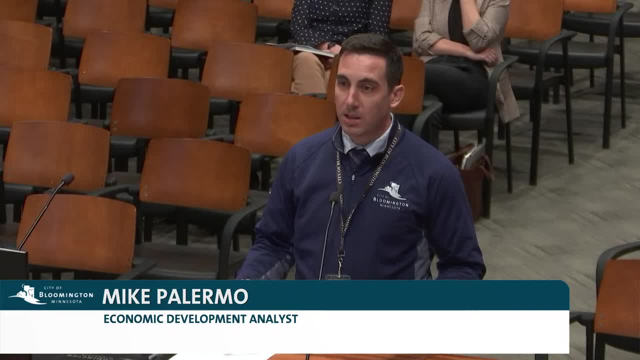 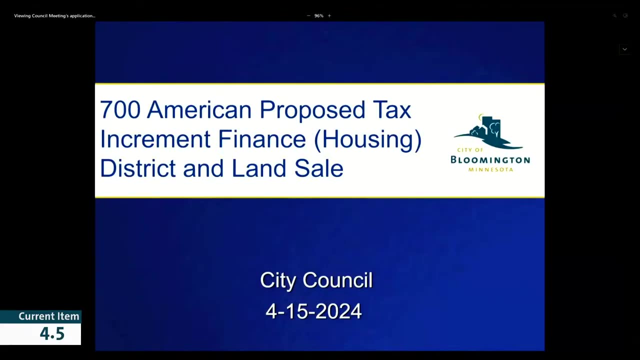 A PUBLIC HEARING FOR WOULD BE THE LAND SALE, THE CITY OWNS THE PROPERTY AND THE OTHER ITEM WOULD BE FOR THE TAX INCREMENT FINANCING DISTRICT. SO YOU'RE WELL FAMILIAR WITH THE SITE, BUT FOR THE SAKE OF THE 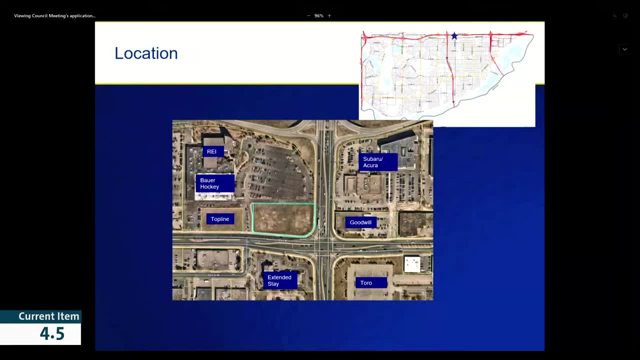 PUBLIC HEARING. THE PROPERTY IS LOCATED AT 700 AMERICAN BOULEVARD WEST, THE VACANT LAND THERE HIGHLIGHTED, NEAR THE REI, AT THE CORNER OF LINDALE AND AMERICAN BOULEVARD. IT'S 128 SENIOR HOUSING. 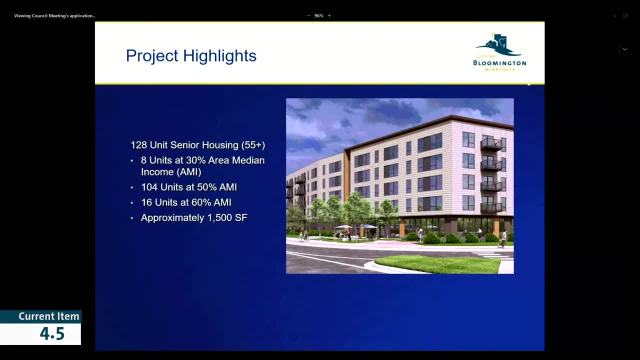 BUILDING. THIS IS ACTIVE SENIOR. EIGHT UNITS ARE PROPOSED TO BE AT 30% AREA MEDIAN INCOME, 104 UNITS WOULD BE AT 50% AREA MEDIAN INCOME AND 16 UNITS WOULD BE AT 60%. 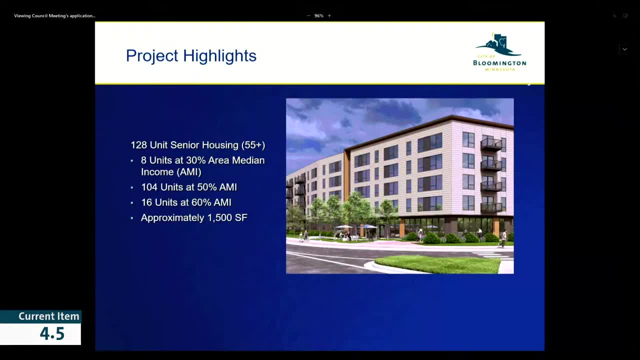 SO THIS AVERAGES AT ABOUT 50% AREA MEDIAN INCOME. THERE'S A SMALL COMMERCIAL SPACE, ABOUT 1500 SQUARE FEET, WHICH WOULD HAVE SOME SORT OF LOCALLY ORIENTED BUSINESS. SO I'LL WALK YOU QUICKLY. 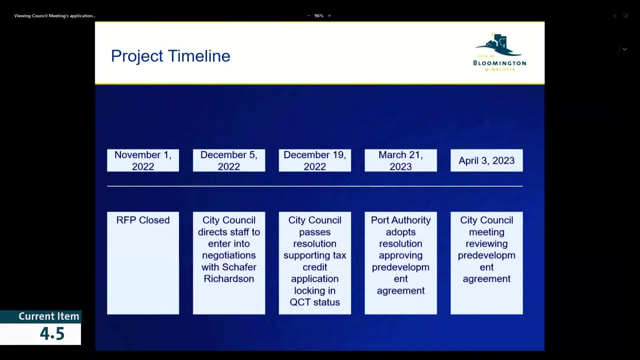 THROUGH THE TIMELINE. WE OWN THE PROPERTY. THE CITY OWNS THE PROPERTY, SO WE PUT OUT AN RFP REQUEST FOR PROPOSAL IN 2022.. WE AFTER REVIEWING THE PROPOSALS WITH COUNCIL DIRECTION. WE SET UP A 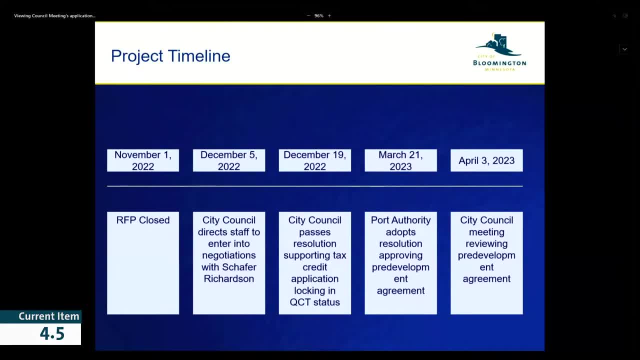 NEGOTIATION WITH THE COUNCIL AND STARTED NEGOTIATIONS WITH SHAEFER RICHARDSON TO DEVELOP THE SITE. THEY THEN WORKED ON THEIR ENTITLEMENT PROCESS, WORKED THROUGHOUT 2023, AND AT THE END, 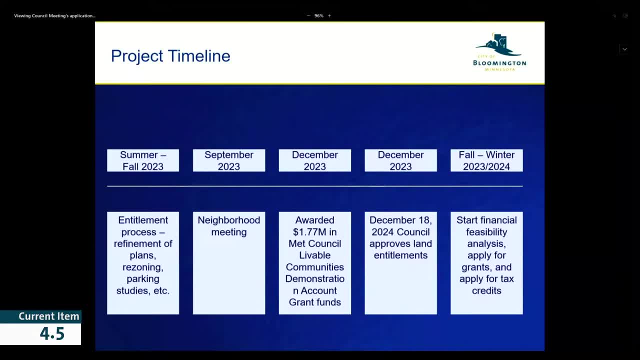 OF DECEMBER, WE PASSED REZONING TO RM100 AND THE APPROVAL FOR THE BUILDING AND DEVELOPMENT. DURING THAT TIME, WE ALSO WERE AWARDED A GRANT FROM THE MET COUNCIL FOR 1.77 MILLION THAT. 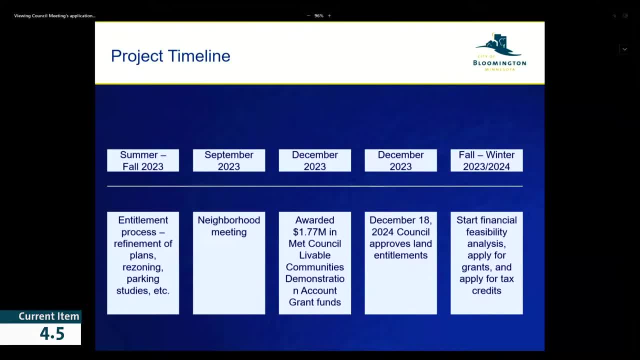 WILL HELP SUPPORT THE AFFORDABLE UNITS IN THIS PROJECT. THEN WE STARTED TO DO THE FINANCIAL ANALYSIS. THE PROJECT WAS AWARDED LOW INCOME HOUSING TAX CREDITS IN JANUARY, SO WE REVIEWED THE TERM SHEET. 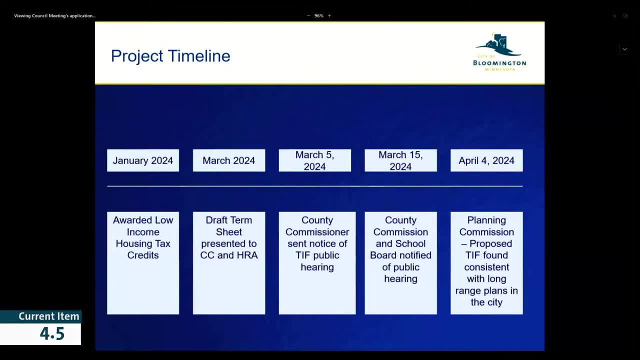 AND ON MARCH 5TH, FOR THE SAKE OF KNOWING THAT WE WERE GOING TO DO TAX INCREMENT FINANCING, WE NOTICED THE COUNTY COMMISSIONER. MARCH 15TH, WE PUT NOTICE TO THE. 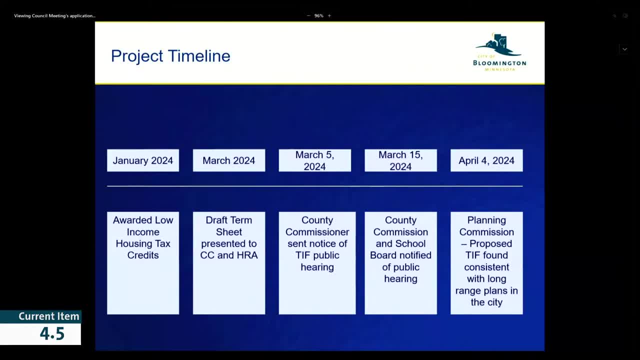 COUNTY COMMISSION AND THE SCHOOL BOARD NOTIFYING OF THE PUBLIC HEARING. AND THEN, ON APRIL 4TH, WE HELD OUR PLANNING COMMISSION MEETING WITH THE STATE AND THE STATE OF MASSACHUSETTS TO REFORM THE PROPOSED TAX INCREMENT. 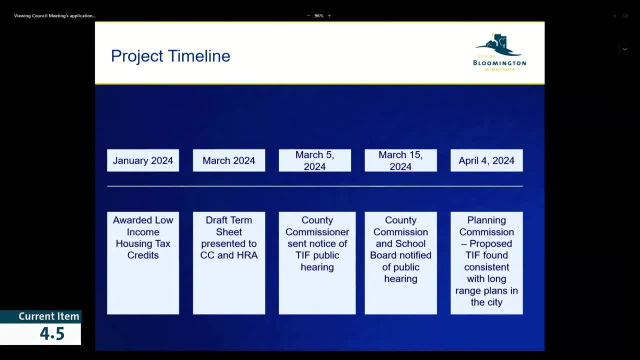 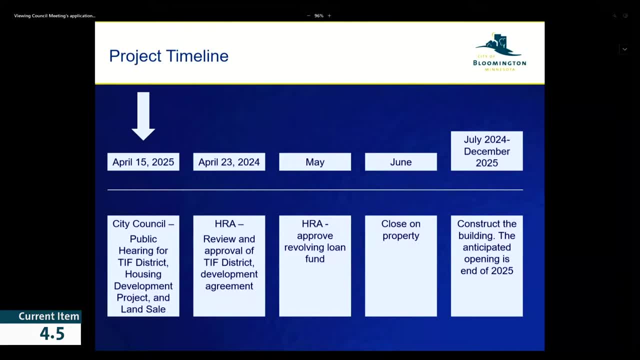 FINANCING DISTRICT AND UNDER STATE STATUTE. WE NEED TO FIND THAT THE PROPOSED TAX INCREMENT FINANCING DISTRICT IS CONSISTENT WITH LONG RANGE PLANS, WHICH THEY PASSED A RESOLUTION IN SUPPORT. SO HERE WE ARE, AT APRIL 15TH. 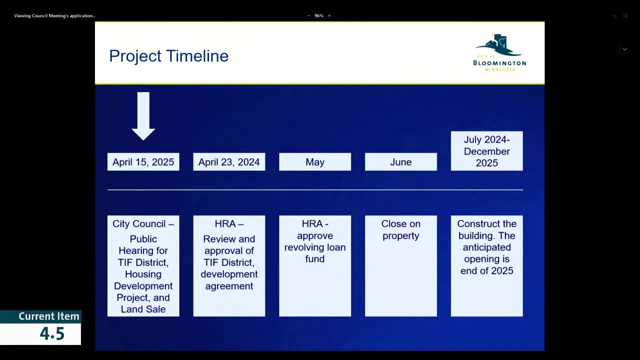 LIKE I SAID, WE'LL HAVE TWO PUBLIC HEARINGS: ONE FOR THE TAX INCREMENT FINANCING DISTRICT- THE TIFT DISTRICT- AND ONE FOR THE SALE OF THE PROPERTY. NEXT WEEK IT WILL GO TO THE HRA. 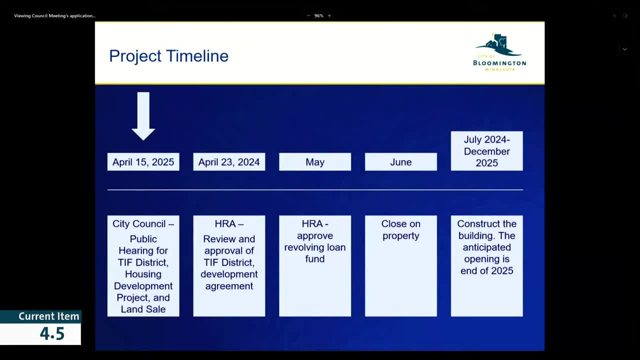 INCREMENT FINANCING DISTRICT. THEY ARE DOING THE TIFT DISTRICT. IT MADE SENSE FOR THEM TO DO THE DEVELOPMENT AGREEMENT, AND THEN THEY WILL ALSO BE APPROVING THE REVOLVING LOAN FUND, THE AFFORDABLE HOUSING. 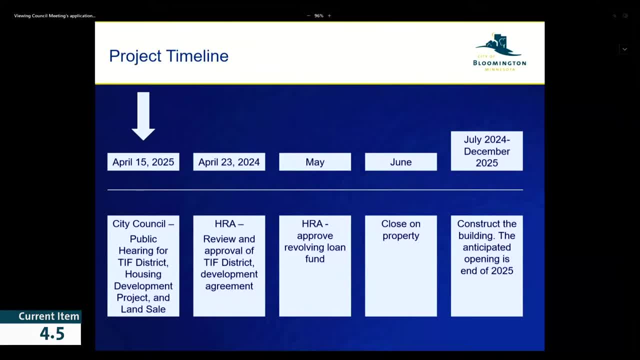 TRUST FUND COUNCIL HAS DIRECTED THEM TO KIND OF MANAGE THAT ALREADY, AND SO WE'RE HOPING TO CLOSE ON THIS PROPERTY MID-JUNE AND THEN FROM THERE, THEY'LL START CONSTRUCTION IN JULY, AND 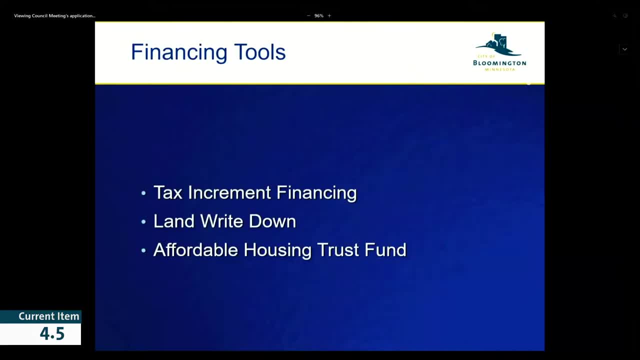 HOPEFULLY, IT IS ANTICIPATED THEY'LL BE COMPLETE DECEMBER OF 2025.. AND THEN WE'RE GOING TO GO THROUGH THESE QUICKLY AND HOW THEY RELATE TO WHAT WE'RE PROPOSING TODAY. SO TAX INCREMENT, FINANCING: I. 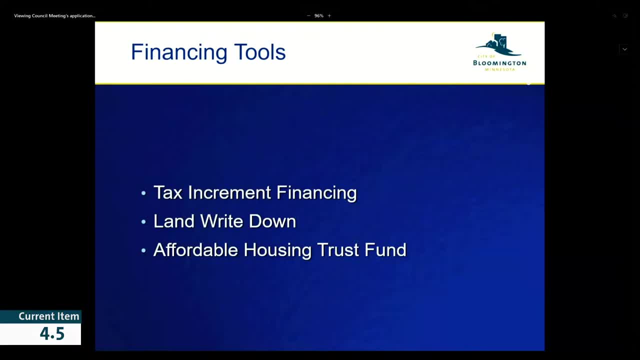 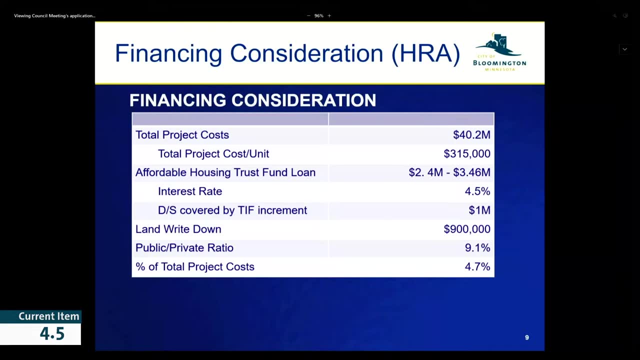 MENTIONED. WE'RE ALSO PROPOSING A LAND WRITE DOWN FROM THE ORIGINAL SALE PRICE AND THE AFFORDABLE HOUSING TRUST FUND. SO THE PROJECT IS ABOUT A $40 MILLION PROJECT YOU CAN SEE PER UNIT IT'S. 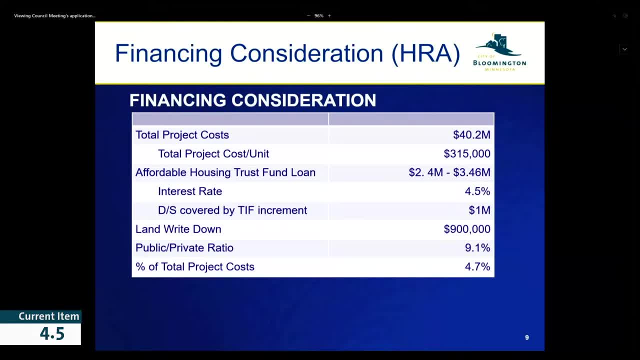 315,000 PER UNIT. WE ARE PROPOSING TRUST FUND LOAN OF 2.4 TO 3.46.. WE'RE NOT ENTIRELY SURE WHAT THAT NUMBER WILL BE. WE'RE WAITING TO HEAR BACK FROM. 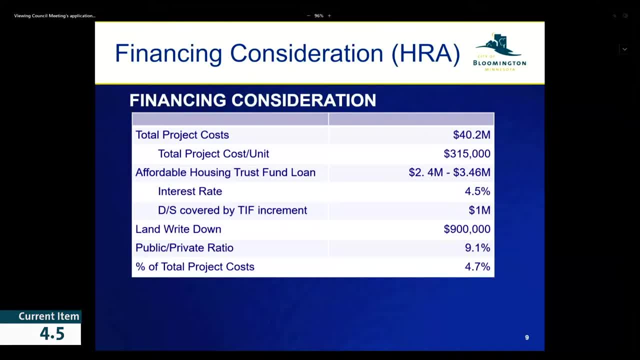 HENDIMAN COUNTY IN EARLY MAY AND IF WE'RE AWARDED AFFORDABLE HOUSING, INCENTIVE FUND GRANT. SO, DEPENDING ON WHAT THAT GRANT AMOUNT IS, IF WE DO RECEIVE THAT, WE'LL KIND OF ADJUST THAT. 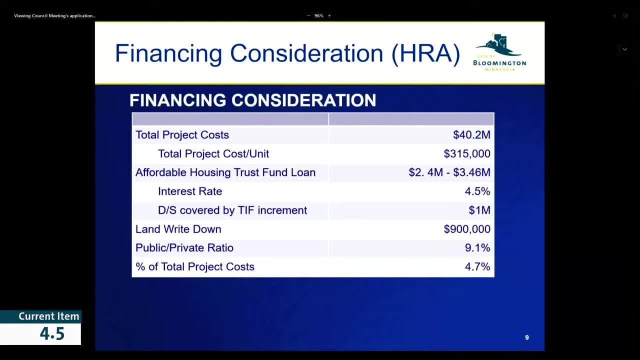 NUMBER, SO WE HAVE SOME FLEXIBILITY, BUT 3.46 IS THE MAXIMUM WE CAN GIVE AS THE REMAINING BALANCE OF OUR AFFORDABLE HOUSING TRUST FUND. IT IS A REVOLVING LOAN FUND. 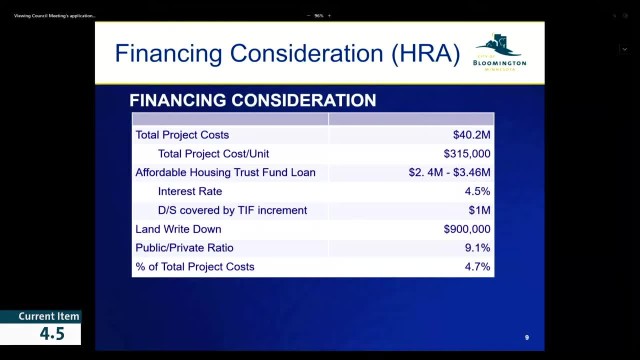 SO YOU CAN SEE HERE IT'S 4.5% INTEREST. THIS IS A LITTLE BIT DIFFERENT THAN THE INTEREST RATE THAT WE USED TO FULFILL THE TRUST FUND, WHICH WAS A LOAN. SO WE TAKE THAT DIFFERENCE IN. 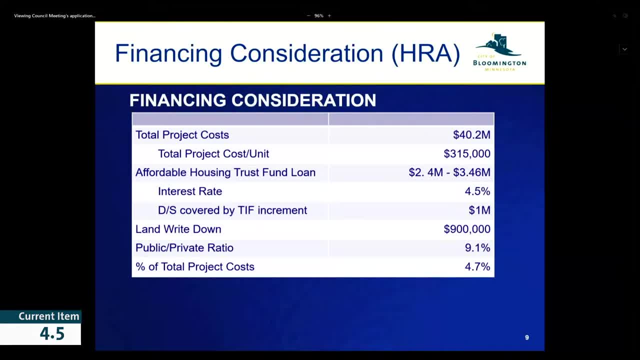 INTEREST, AND THAT'S HOW WE ARE GROWING THIS OVER TIME BUT AT THIS TIME, YOU KNOW, THIS IS OUR FIFTH PROJECT IN- I BELIEVE- FIVE YEARS NOW. IT WILL TAKE SOME TIME TO GROW. 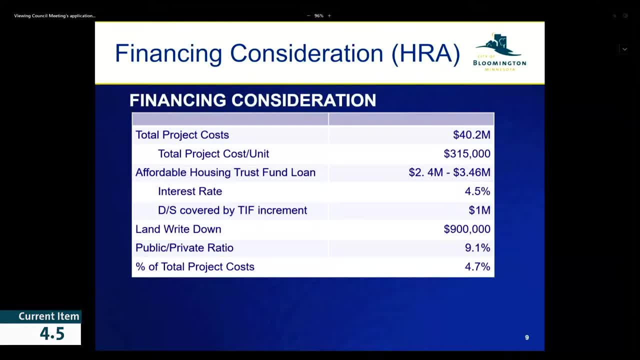 THAT ABOUT. YOU KNOW THESE PROJECTS 25, SOME TAKE, 5,, 10,, 15 YEARS. YOU KNOW TO GROW THAT BALANCE BACK, BUT WE'RE ALSO COLLECTING TAX INCREMENT FINANCING. SO THAT IS. 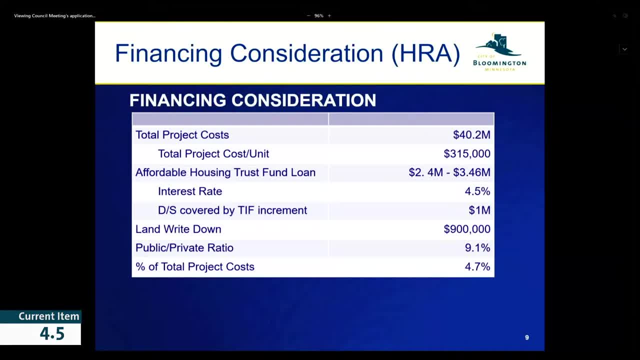 A LITTLE BIT DIFFERENT. WE'RE ALSO PROPOSING A LAND WRITE-DOWN OF $900,000.. WE'LL BE PAYING PART OF THIS LOAN BACK. WE'LL BE CAPTURING THAT AS WELL AS POOLED TIF INTO OUR FUNDS. 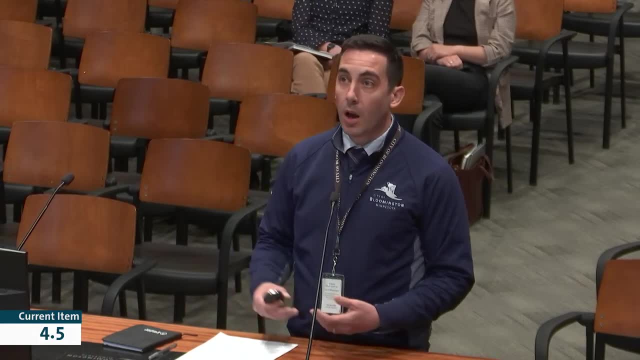 AND SO AT THE END OF THE PROJECT, THEY'LL BE PAYING. YOU KNOW, PAYING A LOAN BACK. THIS IS A LOAN, SO WE ARE GROWING OUR TRUST FUND. IN THE END, WE'RE ALSO PROPOSING A LAND. 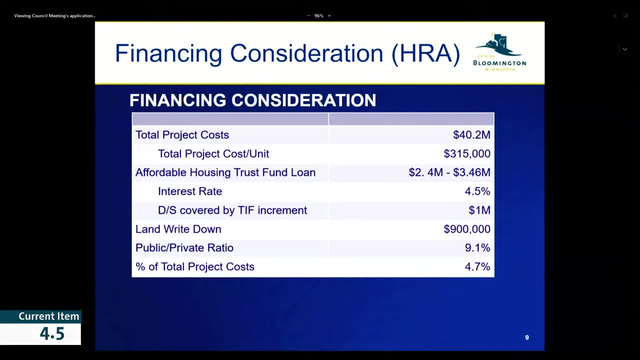 WRITE-DOWN OF $900,000, AND I'LL GO INTO THAT A LITTLE BIT MORE IN A SECOND. SO THIS IS A LAND WRITE-DOWN OF $900,000 WHEN IT COMES TO PUBLIC SUBSIDY COMPARED TO OTHER. 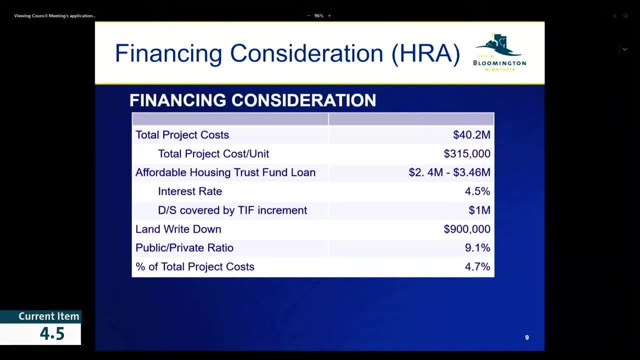 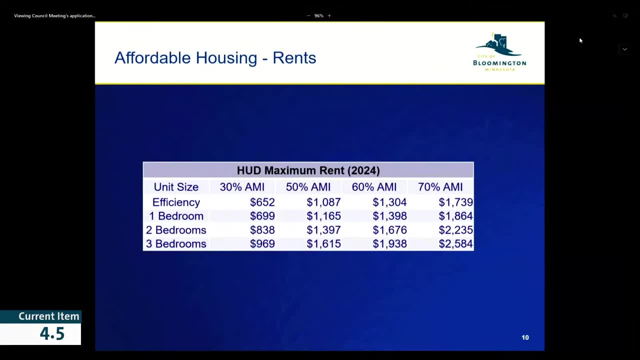 PROJECTS: UH-OH, I THINK WE UNCLICKED THAT, SORRY. SO JUST A QUICK OVERVIEW OF THESE: ARE THE MAXIMUM RENTS FOR WHEN WE'RE TALKING ABOUT AREA MEDIAN INCOME. SO AT 60% WHICH THIS ENTIRE? 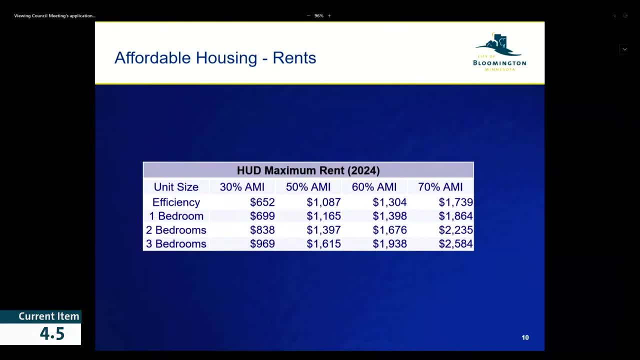 BUILDING WILL BE A FAMILY OF 4,000 ANNUALLY. 50% IS 62,000.. AND 30%, YOU MAKE 37,000.. SO YOU CAN SEE THERE'S A GREAT NEED WHEN YOU HAVE THAT INCOME. 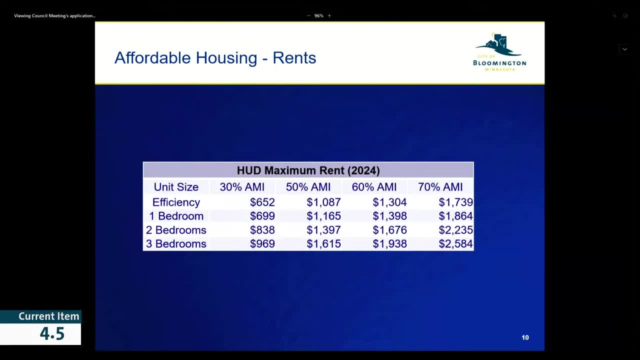 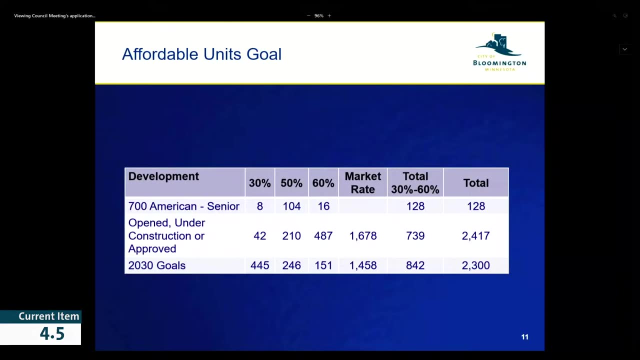 FOR AFFORDABLE HOUSING. AND THESE ARE WHAT THE RENTS TRANSLATE INTO THE CLICKER WORKS. WHEN YOU HAVE TO CLICK ON THE SLIDE, YEAH. WHEN YOU CLICK OFF THE SLIDE BECAUSE YOU'RE YEAH. 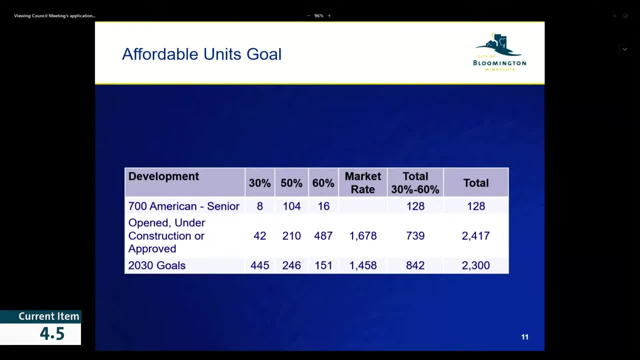 NO FORWARD. OH, HERE WE GO, WE'RE GOOD. SO THIS RELATES TO OUR MET COUNCIL GOALS AND OUR COMPREHENSIVE PLAN, OUR ALLOCATION FROM THE METROPOLITAN COUNCIL FOR 2030.. 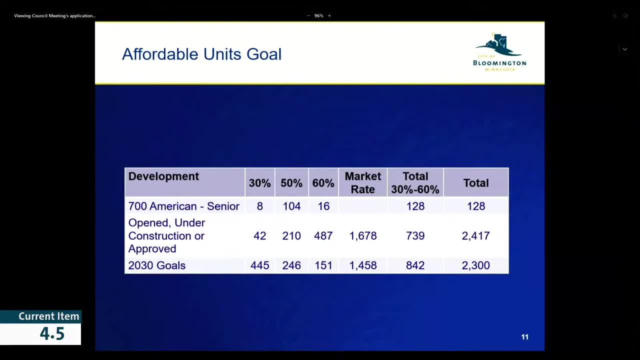 WE HAVE KIND OF SET GOALS ON DIFFERENT INCOME BANS TO PROVIDE AFFORDABLE HOUSING UNITS. OBVIOUSLY, 30% IS THE GREATEST NEED. IT'S ALSO OUR LARGEST AMOUNT OF UNITS THAT WE NEED TO PROVIDE. 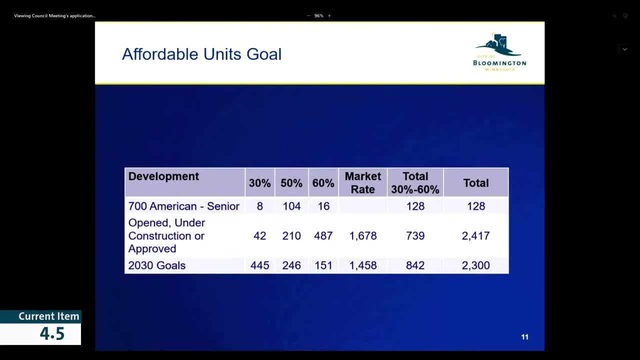 WE'VE ONLY PROVIDED 42 SINCE WE STARTED THIS IN 2020.. THIS WILL ADD EIGHT, SO ABOUT A 20% INCREASE, BUT STILL A LARGE WAY TO GO ON THAT NUMBER. BUT THIS PROJECT KIND OF INCREMENTALLY GETS US THERE. 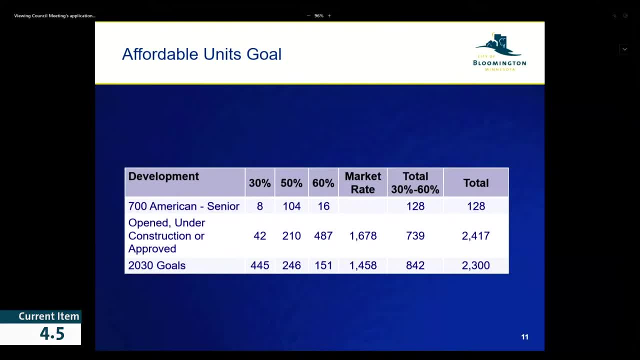 AND YOU CAN SEE IN OUR 50%, WE'RE JUST ABOUT TO MEET THE GOAL, AND THIS PROJECT WILL HELP. TIP US OVER THE TOP OF THAT. BUT 60% UNITS, WE'VE BEEN ABLE TO DO THAT. 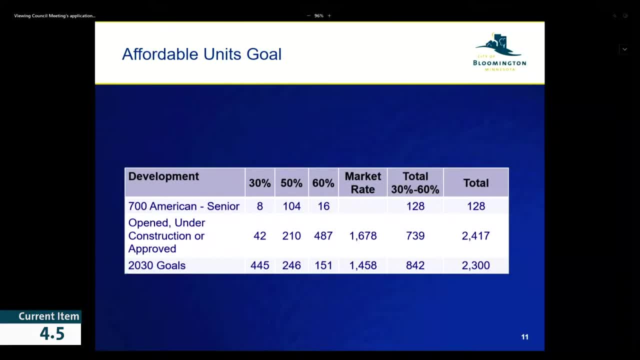 THE AFFORDABLE OPPORTUNITY HOUSING ORDINANCE HAS REALLY KIND OF INCENTIVIZED THAT AND KIND OF PRODUCED THOSE UNITS IN A MEANINGFUL WAY BUT GETTING THAT DEEPER SUBSIDY WHICH THIS PROJECT 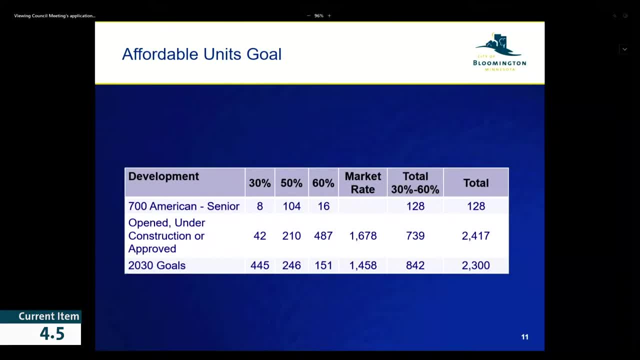 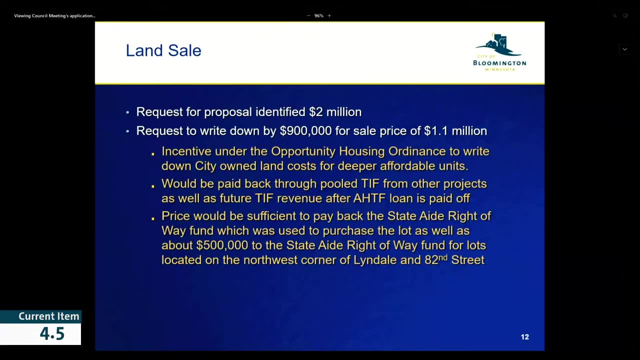 PROVIDES IS REALLY WHAT OUR TARGETS ARE. SO, GOING INTO A LITTLE BIT MORE DETAIL ON THE LAND WRITE DOWN, THIS IS AN INCENTIVE ON THE OPPORTUNITY ORDINANCE THAT YOU CAN REQUEST, SO THEY'VE REQUESTED THAT. WE HAD SET THE PRICE AT $2 MILLION IN THAT ORIGINAL PROPOSAL. THAT'S CONSISTENT WITH OTHER PROPERTIES IN THE AREA OF SIMILAR SIZE. BUT AS WE GOT INTO SOME OF THOSE DEEPER UNITS WITH THE 30%, 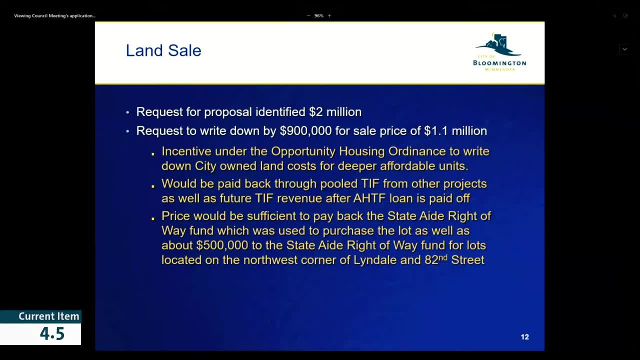 UNITS. THIS IS JUST A WAY TO KIND OF FILL THAT GAP. WE DO HAVE A SOURCE TO KIND OF PAY OURSELVES BACK ONE WHEN WE DO TAX INCREMENT FINANCING DISTRICTS. WE OFTEN POOL MONEY AND YOU CAN USE THAT. 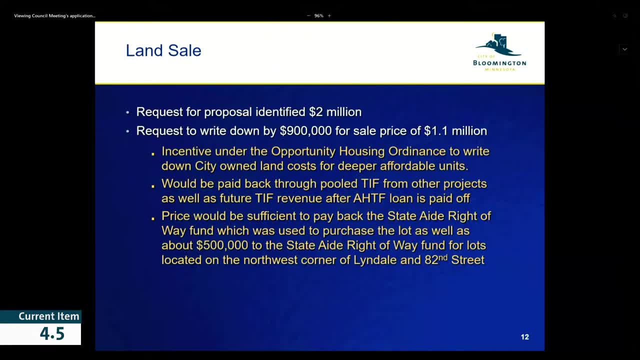 POOLED MONEY FOR AFFORDABLE PROJECTS. SO WE HAVE THAT IN THE SHORT TERM AND IN THE LONG TERM, AS THIS LOAN IS PAID BACK, WE'LL CONTINUE. WE'LL UTILIZE THE TAX INCREMENT IN THAT, BUT WE'LL 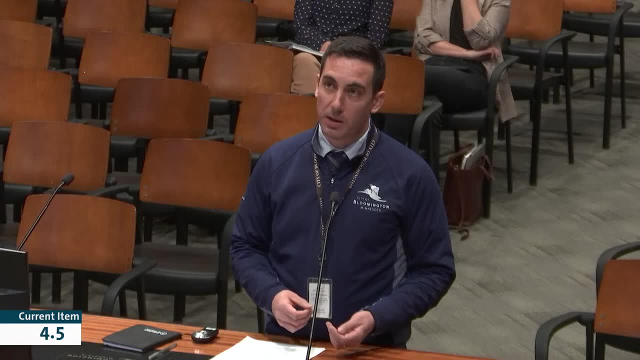 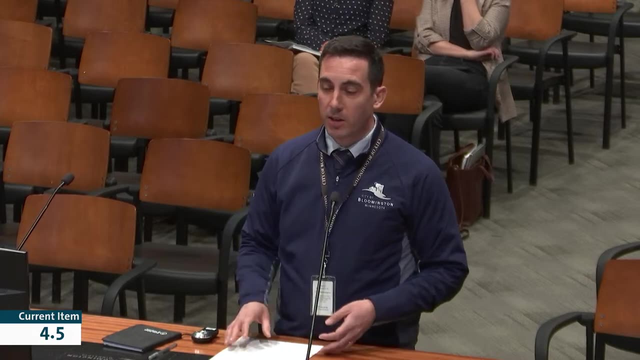 ONCE THAT'S PAID BACK, WE WILL CONTINUE TO CAPTURE THE INCREMENT AND HELP PAY THAT BACK AS WELL. WE WERE COMFORTABLE WITH THE PRICE. PART OF OUR CONSIDERATION FOR THE SALE PRICE IS THAT WE OWE. 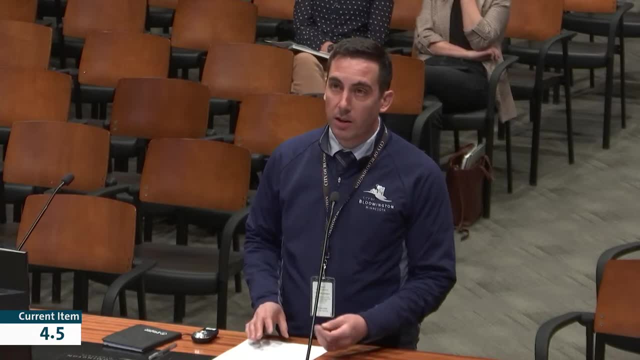 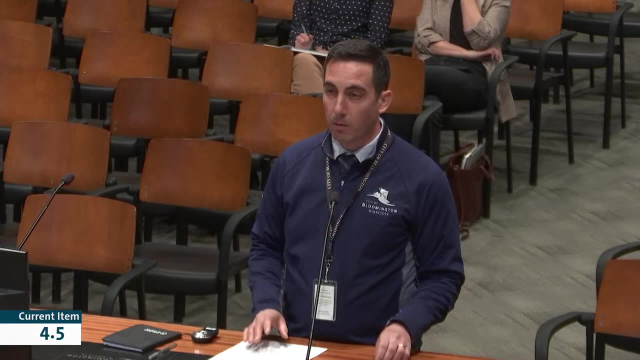 MONEY IN OUR STATE RIGHT-OF-WAY ACQUISITION FUND. THIS IS ABOUT $600,000 THAT WE STILL OWE ON THIS PROPERTY, SO THIS WILL HELP FULFILL THAT AND WE'LL BE FINE IN THAT CASE. 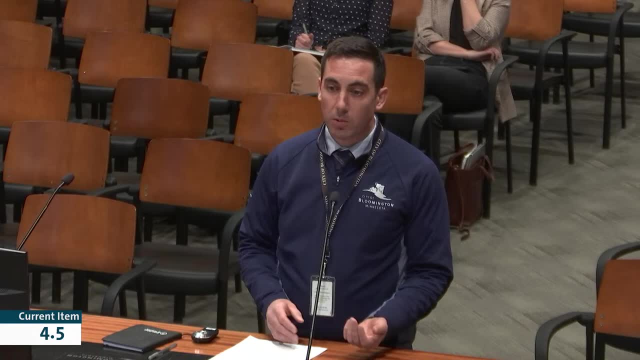 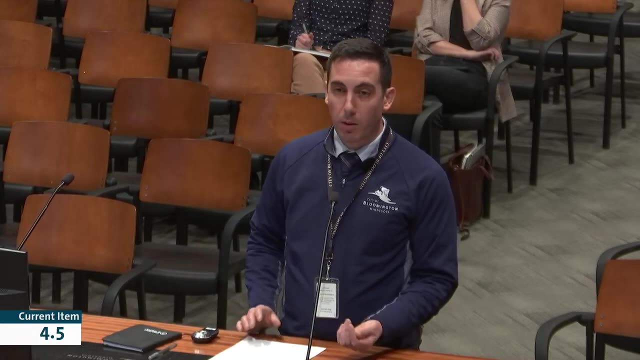 WE'LL HAVE A REMAINING $500,000 THAT WE WILL THEN WE'RE PROPOSING AT THAT TIME WE CAN CHOOSE TO APPLY THIS TO THE STATE RIGHT-OF-WAY TO ACCOUNT FOR PROPERTIES AT LYNDALE AND 82nd STREET. THAT 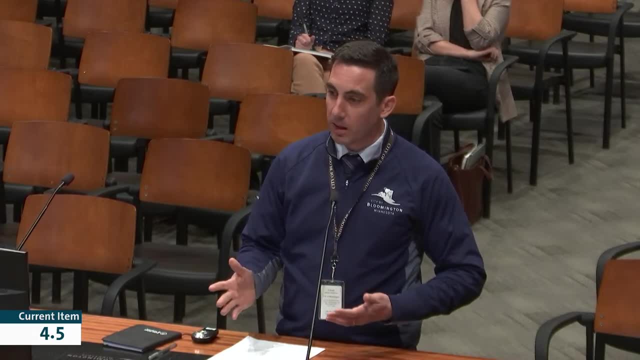 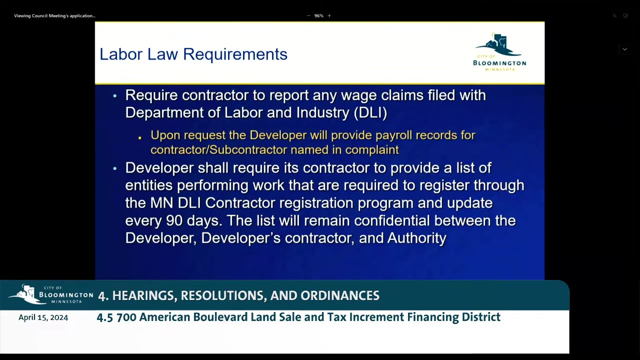 WERE ALSO PURCHASED WITH RIGHT-OF-WAY ACQUISITION FUNDS TO HELP KIND OF FACILITATE, THAT BUT THAT'S A DISCUSSION FOR ANOTHER TIME AT THE DECEMBER 18th MEETING. 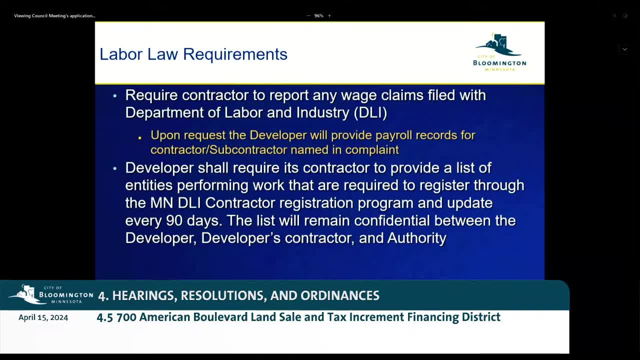 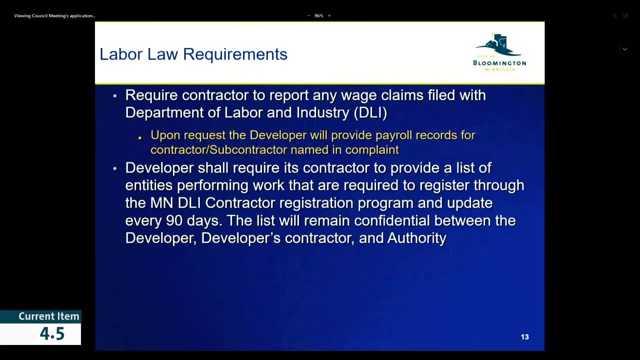 YOU MENTIONED ADDING INTO THE DEVELOPMENT INCREMENT LANGUAGE ABOUT LABOR PRACTICES. THIS IS KIND OF WHERE WE'VE LANDED WITH THE DEVELOPER. WE WERE WORKING IN PARTNERSHIP WITH OUR LEGAL DEPARTMENT. 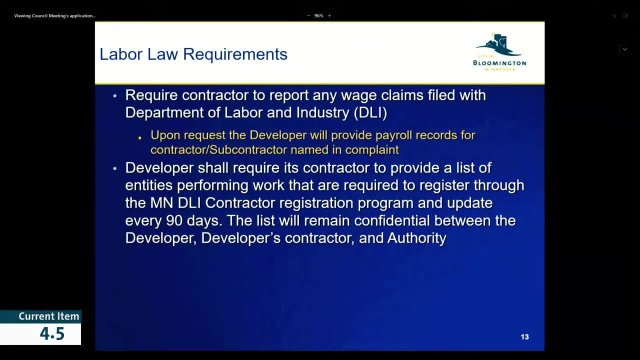 WE ARE PROPOSING THAT WE GET NOTIFIED IF THERE IS ANY WAGE CLAIMS THAT ARE FILED WITH THE DEPARTMENT OF LABOR AND INDUSTRY. WE ARE ALSO THEN ARE ABLE TO REQUEST PAYROLL RECORDS FOR CONTRACTORS AND SUBCONTRACTORS. 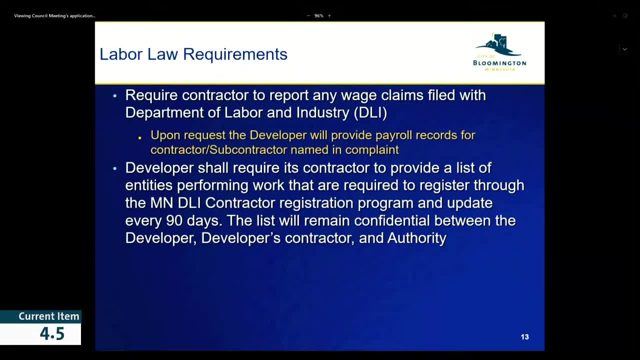 TO SEE WHAT'S GOING ON, AND WE ALSO WANT TO MAINTAIN KIND OF A REGULAR CHECK-IN THAT WE SEE WHAT THE CONTRACTORS AND SUBCONTRACTORS ARE, SO WE KIND OF HAVE AN IDEA OF WHO'S WORKING ON THE PROJECT AS WELL. 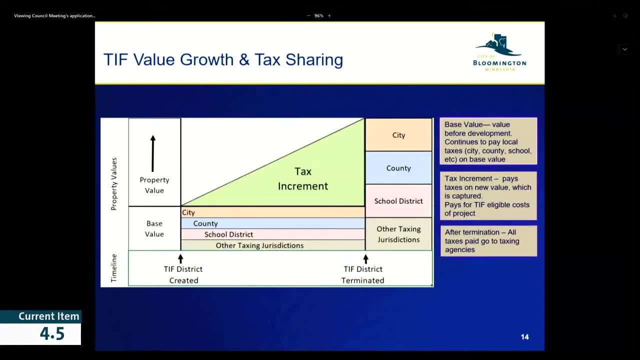 SO MOVING INTO THE TAX INCREMENT FINANCING DISTRICT, JUST TO KIND OF A QUICK OVERVIEW OF HOW TAX INCREMENT WORKS. RIGHT NOW THERE'S KIND OF A BASE VALUE OF TAXES THAT ARE BEING GENERATED FOR THIS PROPERTY. WE HAVE THIS $40 MILLION PROJECT. 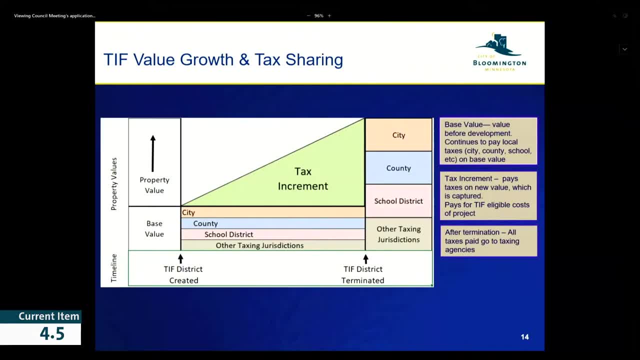 THAT'S HAPPENING, SO THE VALUE IS GOING UP. YOU'RE GENERATING MORE TAXES AND THAT VALUE GOING UP- KIND OF GREEN TRIANGLE- IS THE INCREMENT, SO THAT INCREMENT WE CAN THEN RECAPTURE TO PUT INTO PUBLIC. 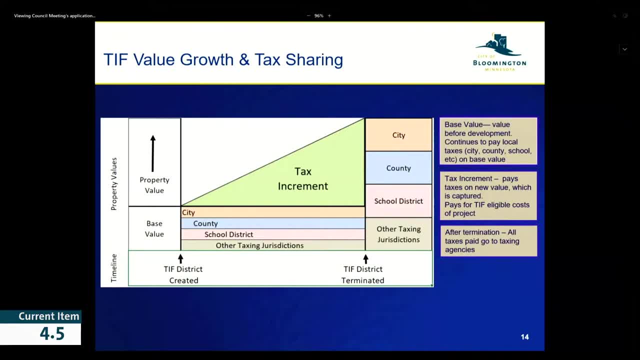 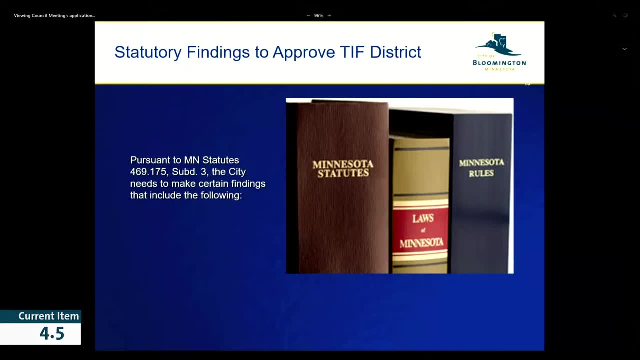 DISTRICT AND THEN THE TAX INCREMENT. INCREMENT IS GOING TO BE IMPROVEMENTS IN THE PROJECT AND IN THIS CASE, THE HOUSING UNITS ARE THE PUBLIC GOOD BUT TO ORDER, TO QUALIFY THAT THERE ARE, FOR THAT WE HAVE TO. 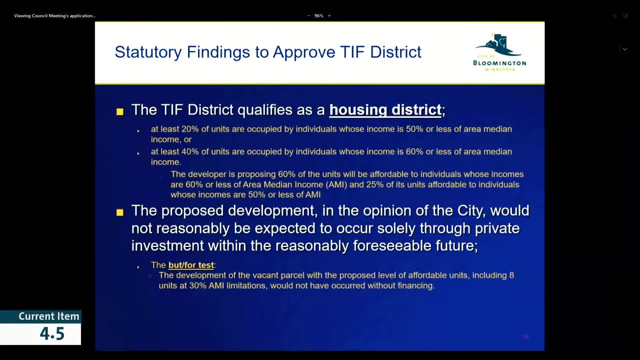 MEET CERTAIN REQUIREMENTS UNDER STATE STATUTE, INCLUDING: DOES IT QUALIFY AS A HOUSING TAX DISTRICT? THERE'S DIFFERENT TYPES OF DISTRICTS. THIS ONE WOULD BE A HOUSING DISTRICT. YOU EITHER HAVE TO HAVE 20% OF 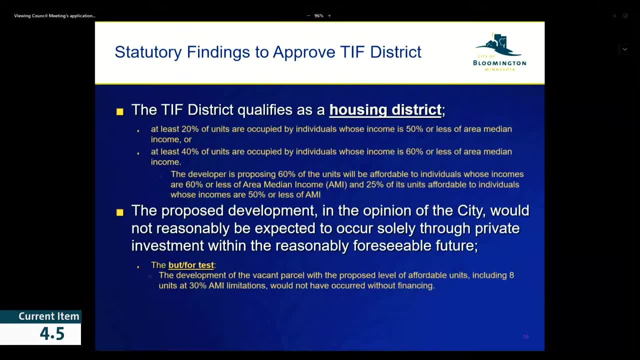 THE UNITS AT 50% OR 40%, AT 60% AREA MEDIA INCOME, AND THIS IS 100%, SO EASILY MEETS THAT BUT YOU ALSO NEED TO HAVE THE BUT FOR TEST. WOULD WE BUT FOR THIS TAX. 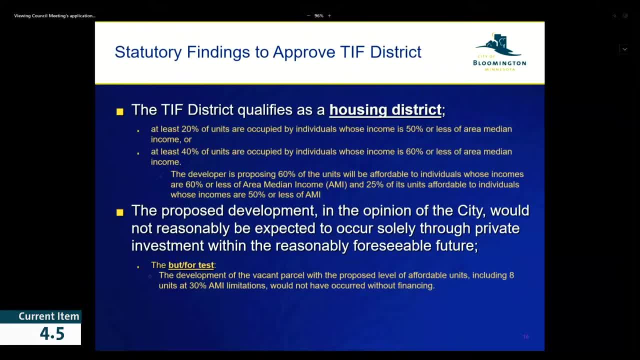 INCREMENT FINANCING WOULD THIS PROJECT WORK AND ANALYZING THE PRO FORMA YOU KNOW, AS YOU SAID, YOU SAW, WE ONLY HAVE 42 UNITS AT 30% AMI, SO WE REALLY WOULDN'T BE ABLE. 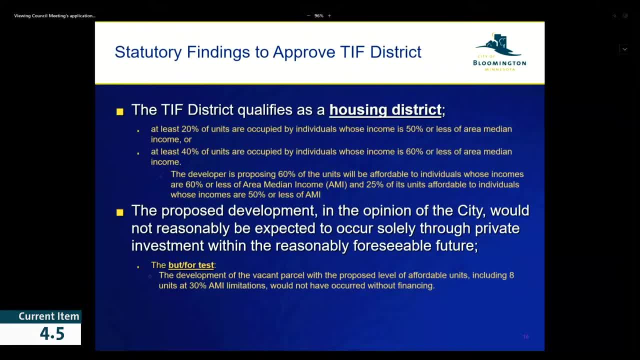 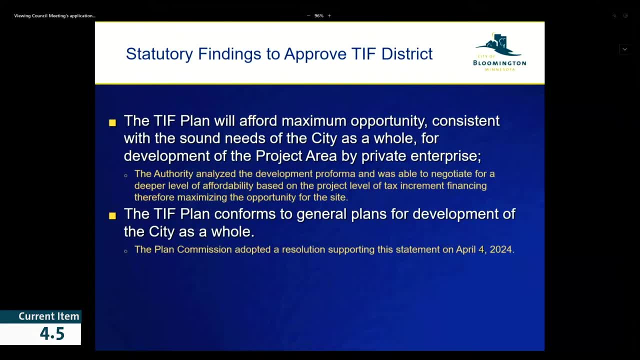 TO GET THOSE UNITS AT THIS AFFORDABLE LEVEL WITHOUT THIS INCREMENT FINANCING ADDITIONALLY THIS LEVEL OF DEVELOPMENT, IT WOULDN'T HAPPEN WITHOUT THIS FINANCING AND LIKE I HAD MENTIONED IT. 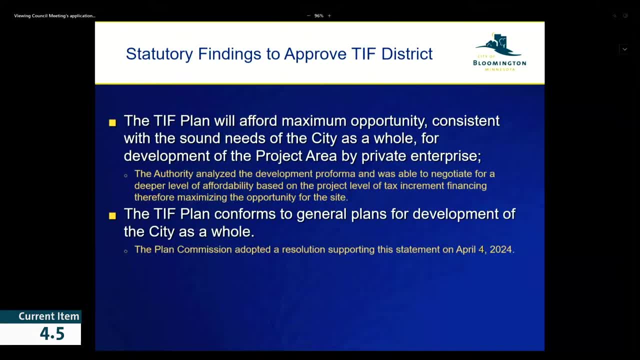 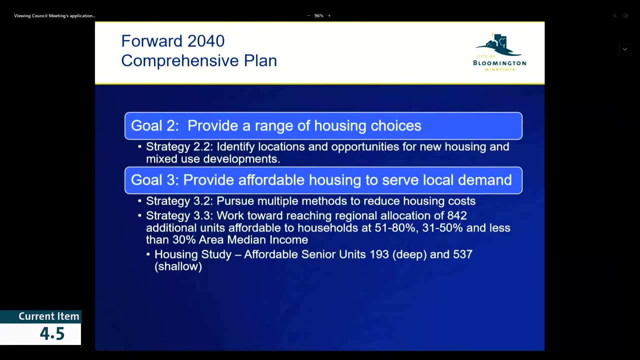 CONSISTED WITH LONG RANGE PLANS. PLANNING COMMISSION HAS REVIEWED THAT BUT TO GIVE YOU AN IDEA, IT MEETS TWO OF OUR MAIN HOUSING. GOALS IN THE COMPREHENSIVE PLAN PROVIDE A RANGE OF HOUSING. 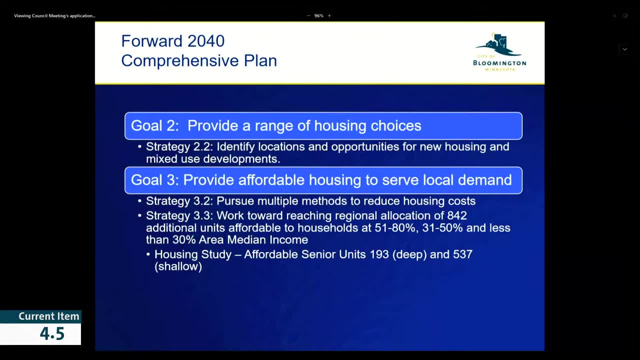 THIS IS SENIOR HOUSING. IT'S AFFORDABLE. HOUSING. IT'S A MIXED USE, DEVELOPMENT AND SERVE OUR LOCAL DEMAND. YOU SAW WHAT OUR ALLOCATION WAS FROM THE MILE COUNCIL AND HOW. 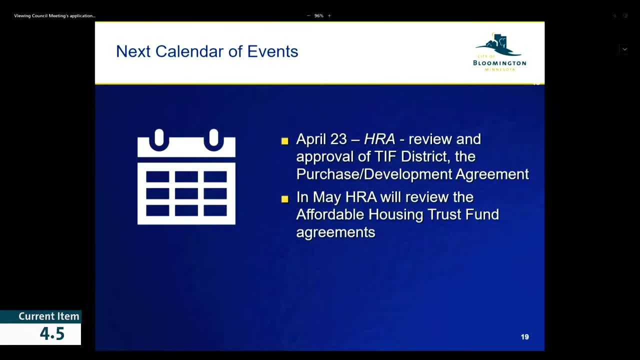 WE'RE ADDRESSING THOSE SO LIKE I HAD MENTIONED NEXT STEPS. NEXT WEEK, HRA WILL REVIEW THIS FOR THE TIF DISTRICT AND THE PURCHASE AND DEVELOPMENT AGREEMENT, AND THEN THEY'LL ALSO BE SHORTLY. 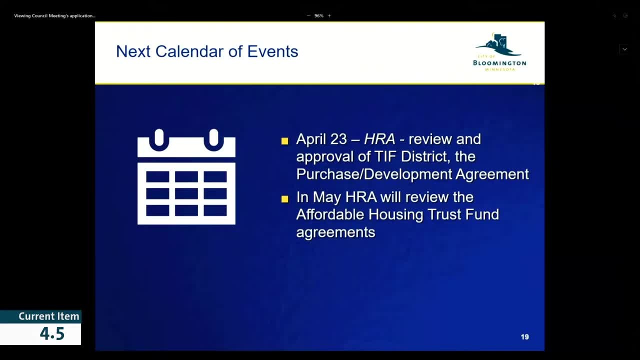 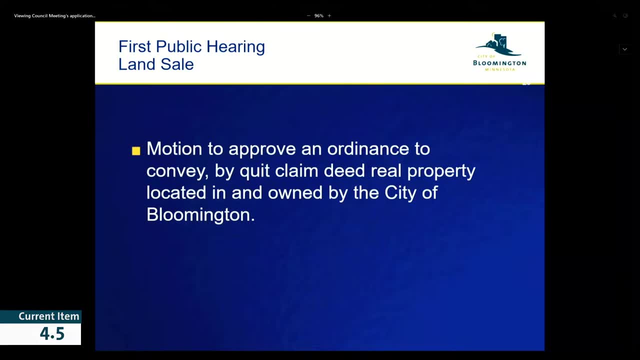 AFTER VIEWING THE AFFORDABLE HOUSING TRUST FUND AGREEMENT, AND SO WITH THAT, I'M HAPPY TO ANSWER QUESTIONS, AND THERE'S THE FIRST QUESTION THAT I WANTED TO ASK: IS THERE ANY OPPORTUNITIES FOR? 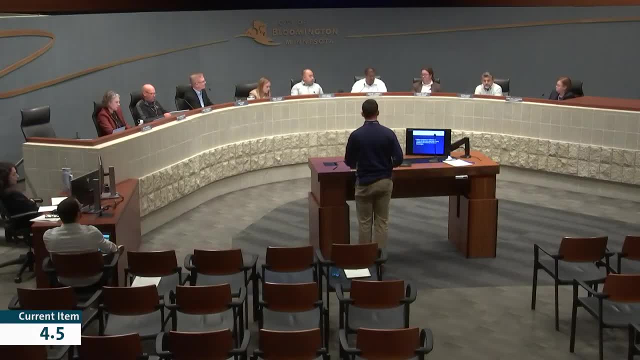 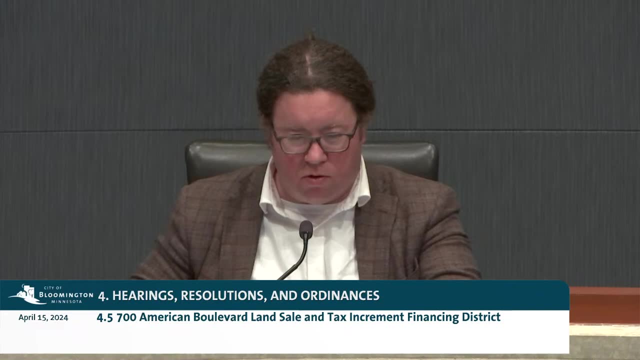 THE COUNCIL TO ADDRESS THE PROBLEM OF TWO PUBLIC HEARINGS, THAT WE'LL HAVE TO OPEN AND CLOSE AND VOTE ON COUNCIL. ANY QUESTIONS HERE? COUNCIL MEMBER NELSON. THANK YOU. 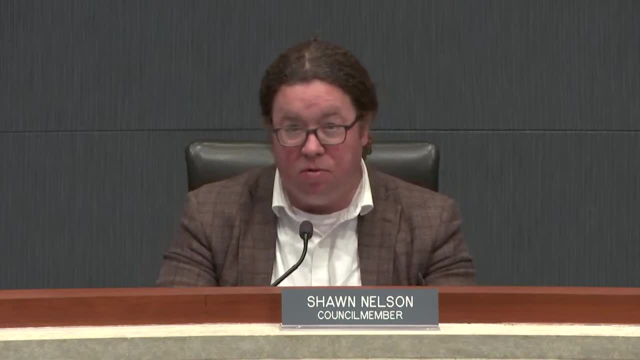 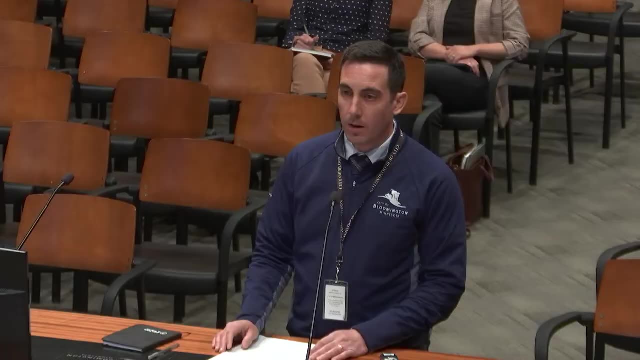 FOR THE BUT-FOR TEST- THAT INCLUDES ALL OF THE AFFORDABLE UNITS- CORRECT BECAUSE, PRESUMABLY THEY COULD BUILD THIS WITH LESS SUBSIDY IF THEY DID ALL THE MARKET RATE HERE, BUT THEY DID ALL THE MARKET. 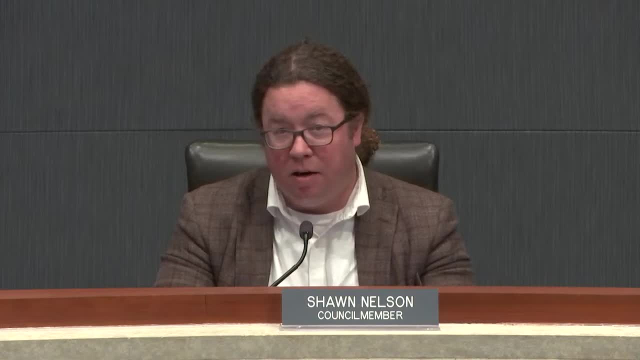 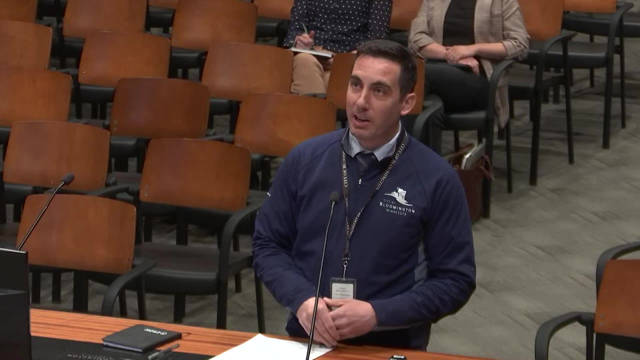 RATE HERE. THEY DID 8 AT 30%, 9% FOR OUR ORDINANCE, AND THEN DID THE REST OF THE MARKET. RATE IS THAT ACCURATE, MR MAYOR, COUNCIL, MEMBER NELSON, I DON'T KNOW EXACTLY IF THAT WOULD STILL BE ACCURATE IF THEY DID ALL MARKET RATE HERE. IF IT WOULD WORK, I THINK THE DEVELOPER WOULD BE BETTER ABLE TO ANSWER THAT ON WHAT THOSE FINANCES LOOK LIKE. MY GUESS IS THAT THEY PROBABLY 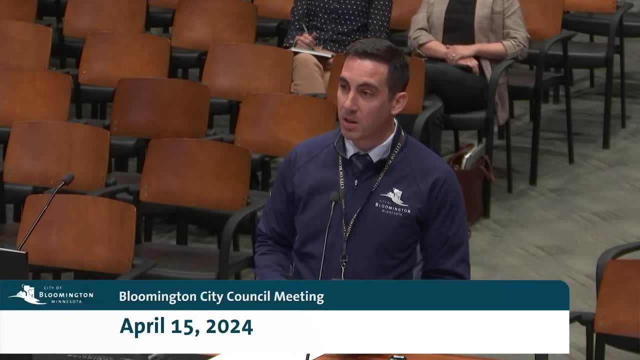 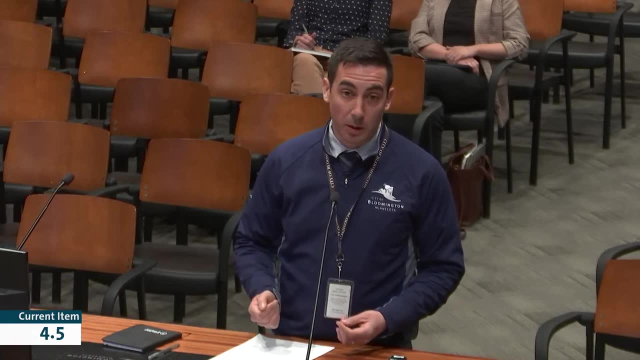 COULDN'T DEVELOP IT AT THE SAME INTENSITY. IT'S A PRETTY 128 UNITS. IT'S PRETTY LARGE. FOR EXAMPLE, DOWN THE STREET AT 1801 AMERICAN THAT DID GO THAT ROUTE. THEY WERE ONLY ABLE TO PRODUCE. 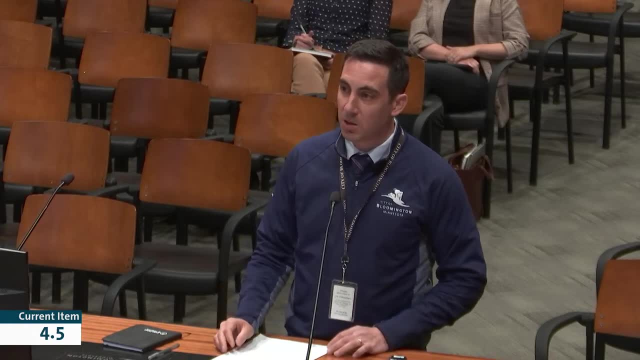 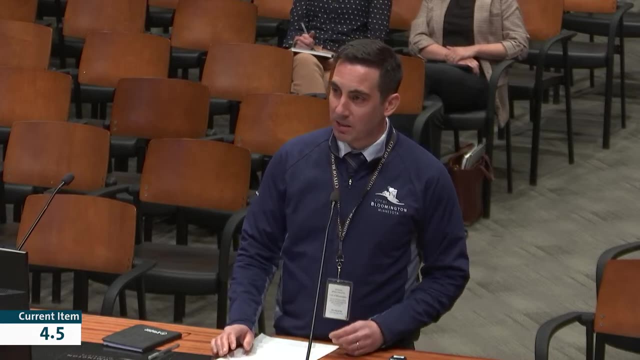 99 UNITS ON THAT SITE. SO THIS IS ALMOST 30% MORE UNITS ON THE SITE. SO, SPECULATIVELY, I WOULD SAY, IT MIGHT STILL BE TOUGH FOR THEM TO DEVELOP AT THE SAME INTENSITY, BUT FOR THIS. 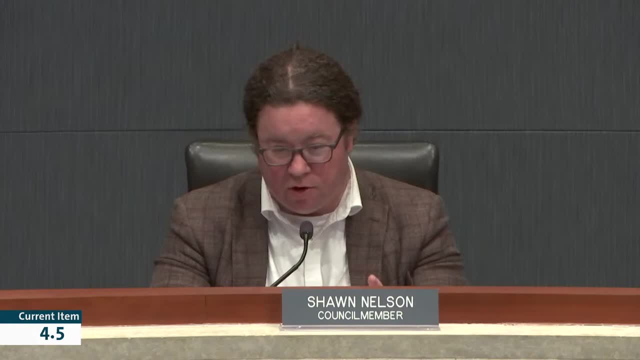 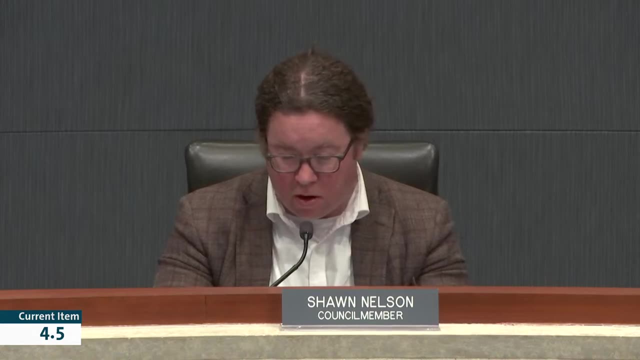 FINANCING. OKAY, AND I GUESS, PART OF MY QUESTION IS: YOU KNOW, AND I THINK I'VE ASKED THIS BEFORE- BUT THE AREA THAT WE HAVEN'T BEEN ABLE TO PERFORM WITH THE OHO IS AT 30%. 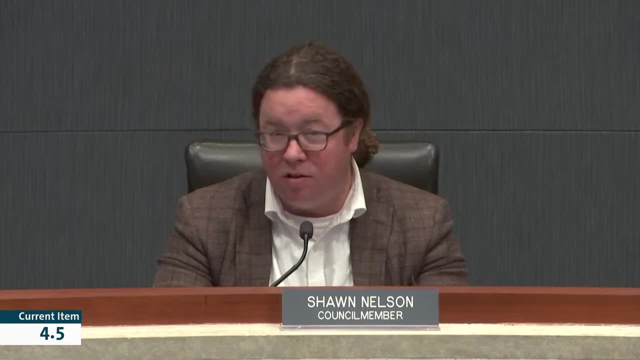 WE'VE ALREADY MET OUR GOALS AT 50 AND 60.. I MEAN WE'VE ALMOST QUADRUPLED IT AT 60 OR SOMETHING LIKE THAT, AND WOULD WE BE BETTER OFF JUST GETTING 20 UNITS OF 30%? 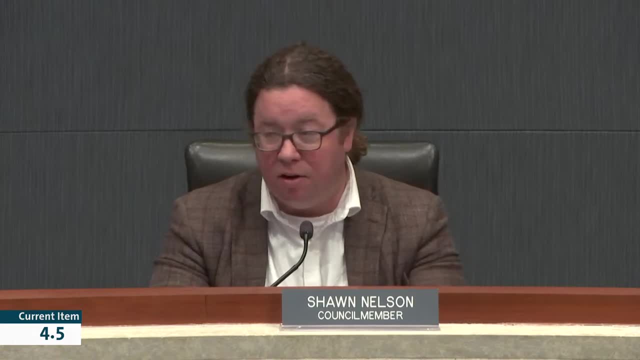 AT 30% AND LET THE REST OF THEM BE MARKETPLACE. EVEN IF WE HAD TO USE OUR TOOLS HERE, WE'D STILL BE BETTER OFF WITH OUR GOALS. WE'LL BE ABLE TO DO THAT, BUT YOU KNOW, IF WE'RE 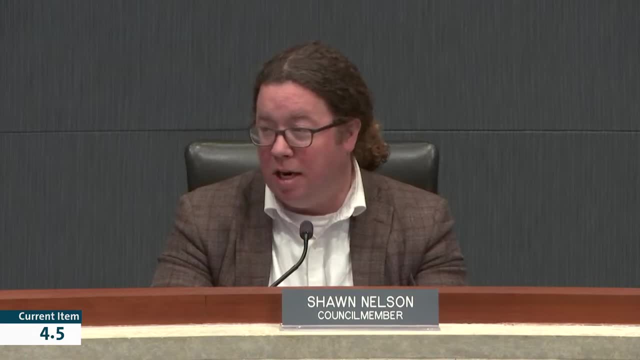 LOOKING AT GOALS. I'M JUST CONFUSED AS TO WHY WE'RE LOOKING. WE'RE NOT LOOKING AT THE GOAL ACTUALLY. WE'RE JUST DOING MORE OF SOMETHING THAT WE'VE DEMONSTRATED. MAYBE WE DON'T. 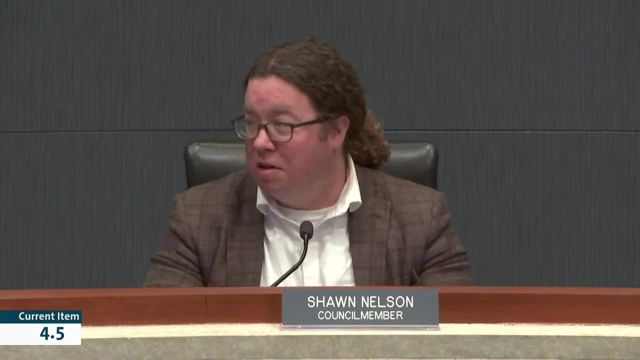 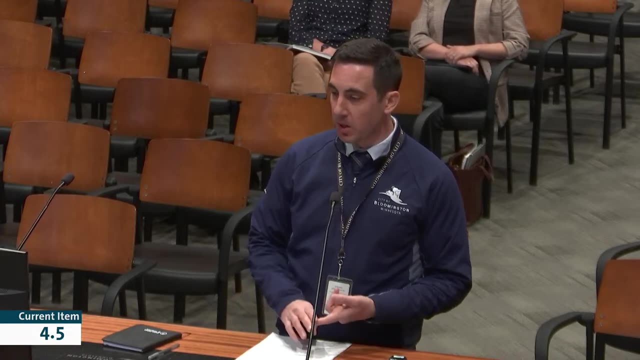 NEED TO DO AS MUCH OF. IS THAT MAKING SENSE, MR MAYOR, COUNCILMEMBER, NELSON, I UNDERSTAND THAT, I THINK WITH THIS SITE. YOU KNOW, THE CITY OWNS THE PROPERTY. SO THERE IS THAT. 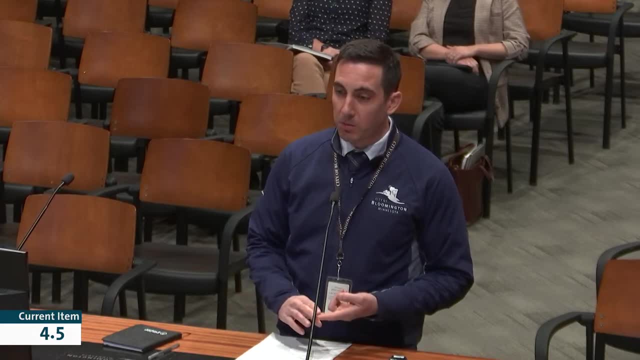 FINANCIAL CONSIDERATION AND BEYOND THAT, IN THE LIND WE WERE TALKING ABOUT THE LINDELL RETROFIT PLAN, EARLIER TOO, THIS IS THE GATEWAY TO THAT. SO ONE OF OUR GOALS FOR THE 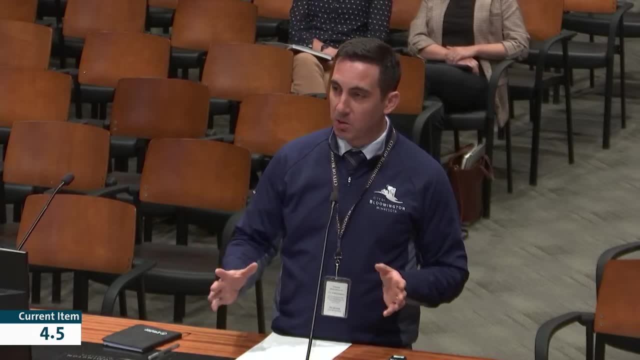 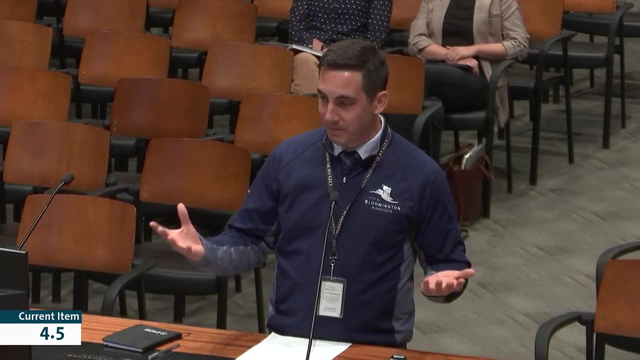 SITE WAS HAVING A KIND OF HIGH-INTENSITY MIXED-USE GATEWAY FEATURE. ON THE CORNER WHEREAS A 30-UNIT APARTMENT BUILDING. YOU KNOW, LESS YOU KNOW DOESN'T PROVIDE THAT. 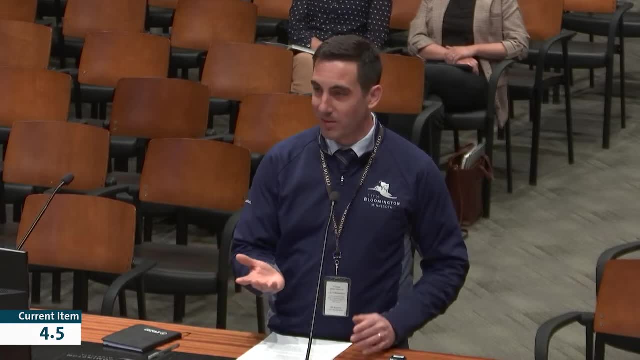 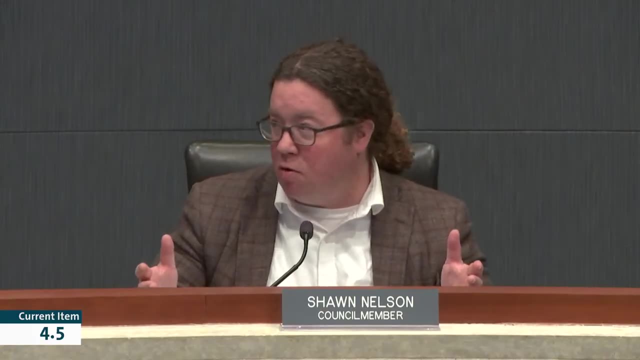 KIND OF GATEWAY FEATURE BUT THAT IS A POLICY DECISION FOR YOU ALL TO MAKE. JUST I MEAN ONE LAST POINT. I MEAN: THE UNITS ARE GOING TO BE THE UNITS, OUR ORDINANCE SAYS YOU HAVE 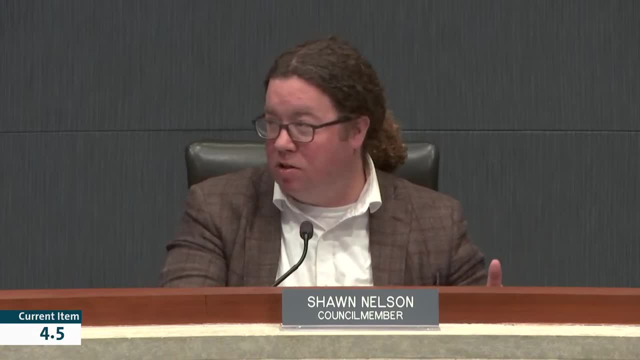 TO BUILD A COMPARABLE UNIT, REGARDLESS OF IF IT'S AFFORDABLE, THE AFFORDABLE UNIT OR NOT, SO THEY'RE ALL GOING TO BE PRETTY MUCH THE SAME. WE'VE ALREADY DETERMINED THAT THROUGH OUR ORDINANCE. SO THE COSTS TO BUILD IT ARE THE SAME. BUT IF THEY COULD GET HIGHER RENT FOR HALF OF THOSE PLACES, DOESN'T THAT JUST EITHER GIVE THEM MORE MONEY TO PUT INTO REDUCING THE RENT FOR THE REST? OF THEM, OR MAKE IT SO THAT WE DON'T HAVE TO PROVIDE AS MUCH INCENTIVE, WE DON'T HAVE TO DO A LAND BUILDING, WE DON'T HAVE TO WRITE DOWN. YOU KNOW MAYBE WE DON'T DO TIF. 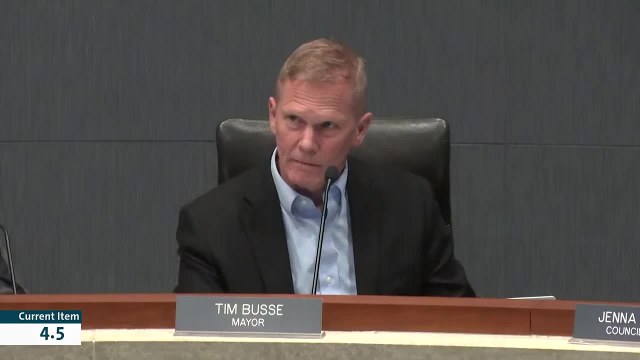 THERE'S OTHER FUNDING SOURCES. I BELIEVE WE HAVE THE DEVELOPERS HERE. SO IF YOU TWO DON'T WANT TO TRY AND TACKLE THIS, MAYBE WE COULD MAYOR, IF I MIGHT. I THINK 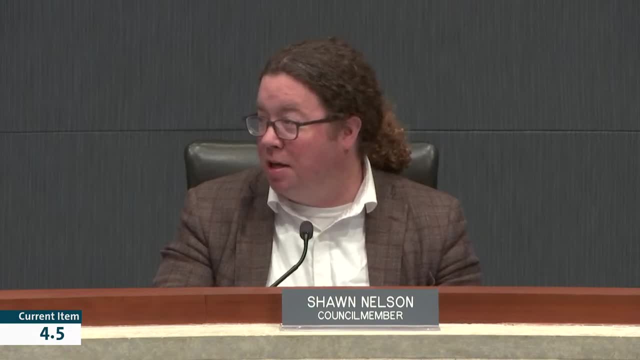 I'VE COVERED THIS BEFORE. I JUST WANTED TO BRING IT UP. I THINK WE TALKED ABOUT IT LAST TIME, AND SO I DON'T MEAN TO BELABOR IT AT 10 O'CLOCK AT NIGHT, I JUST IT. 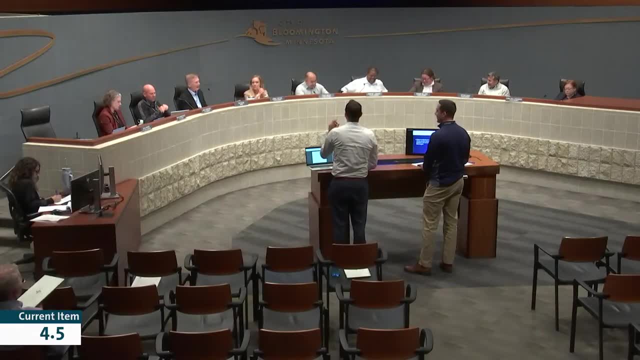 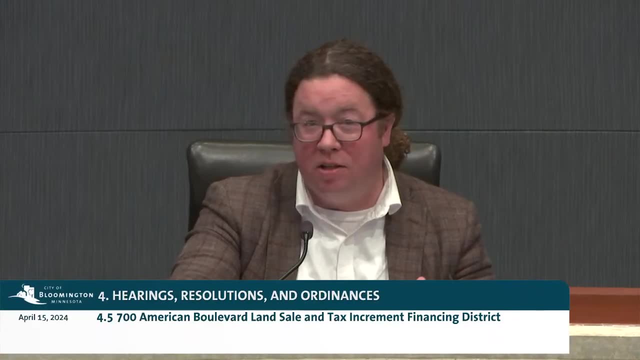 UNDERSTOOD WAYNE, STOP KICKING ME. I JUST WANT TO MAKE THE POINT THAT YOU KNOW THE FUTURE PROJECTS. I MEAN THIS ONE, HONESTLY, IS A STRUGGLE FOR ME TO SUPPORT, BASED ON THAT. 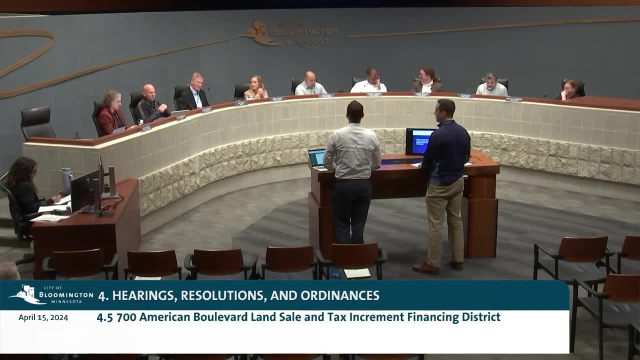 SORRY, WE COULD HAVE DONE BETTER. I CUT MYSELF OFF MR MAYOR AND COUNCIL MEMBERS. I JUST WANTED TO HIGHLIGHT TOMORROW ACTUALLY AT THE PORT AUTHORITY. WE WILL BE. 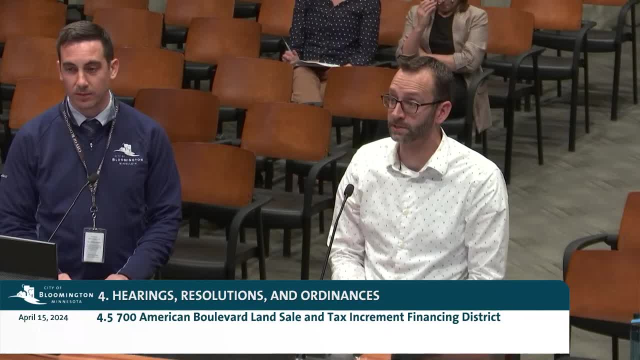 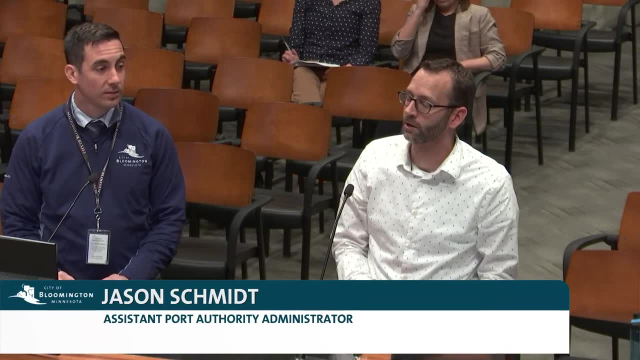 HAVING THE TWIN CITIES HOUSING ALLIANCE PRESENT ON THIS AND GIVE US A LITTLE BIT MORE INFORMATION AND SO THEY'LL BE HITTING ON WITH REGARDS TO 30% AMI UNITS AND KIND OF THE STRUGGLE OF. 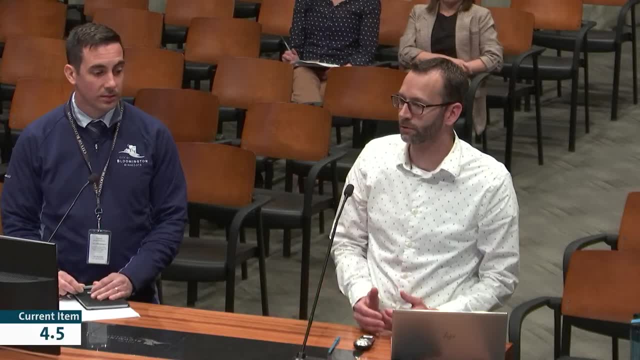 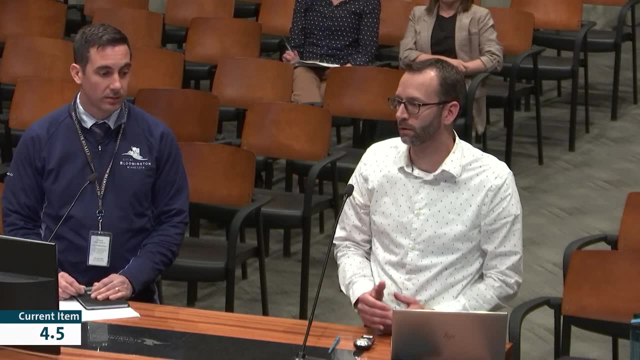 PLACING THOSE IN WITH MORE AFFORDABLE PROJECTS, AND SO I WANTED TO MAKE SURE THAT THOSE DEVELOPERS HAVE THE RESOURCES TO USE, OR THE RESOURCES TO SUPPORT THOSE 30% AMI PROJECTS. CORRECT: 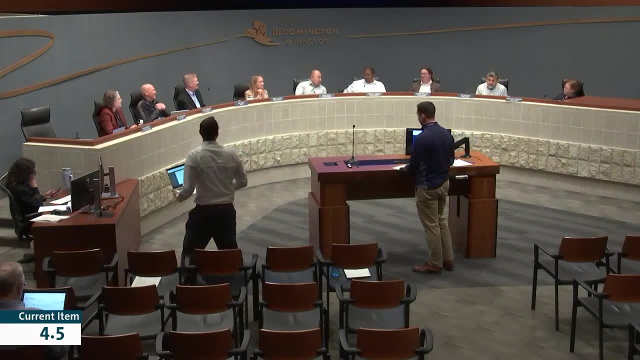 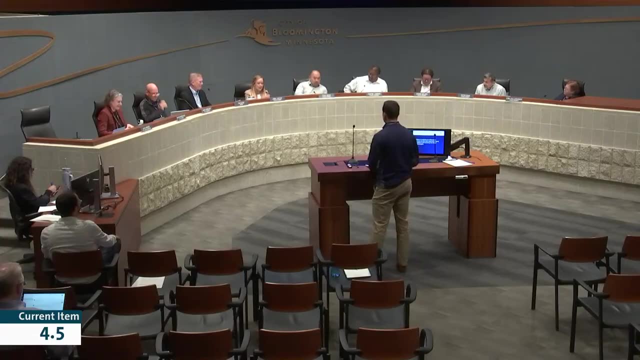 I HOPE SO YOU'RE PART OF IT. COUNCIL MEMBER CARTER. YEAH, THANK YOU, MAYOR. SO I WAS JUST GOING TO SAY I REALLY APPRECIATE COUNCIL MEMBER NICHOLS' COMMENT ON. 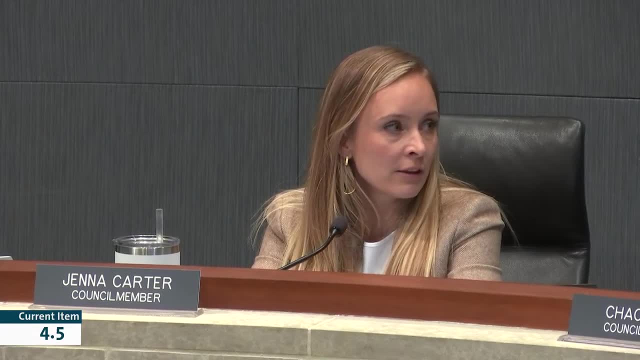 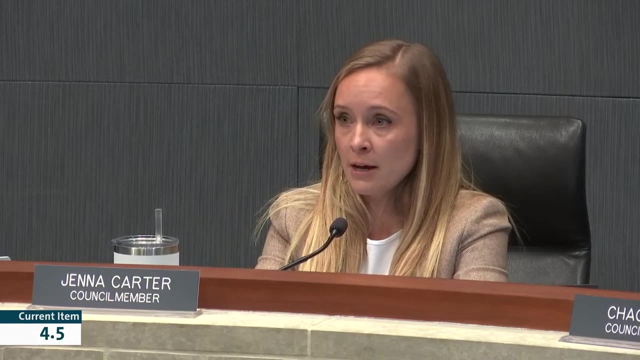 THIS. I THINK IT'S REALLY IMPORTANT TO REFLECT NELSON'S POINT AND I THINK THAT THAT'S DEFINITELY A STRONG CONSIDERATION MOVING FORWARD, AND I THINK WE RECENTLY UPDATED OUR OPPORTUNITY HOUSING ORDINANCE. 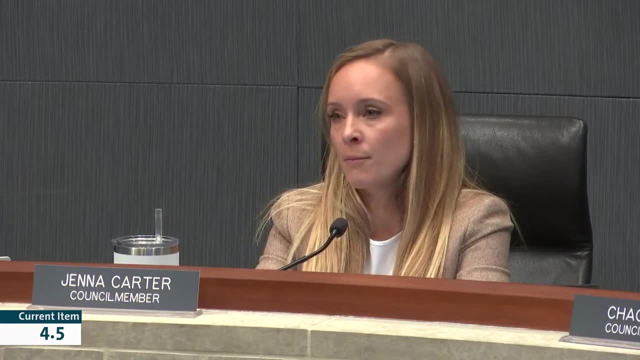 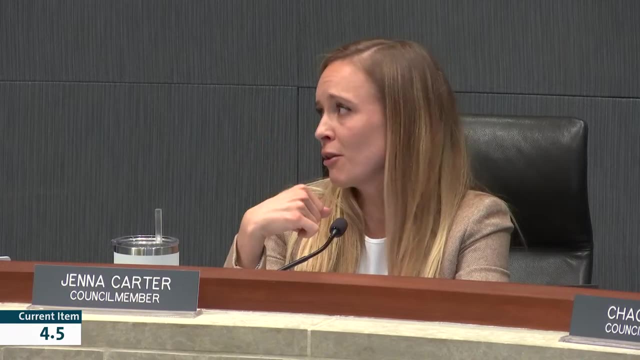 TO REFLECT THE PRIORITIZATION OF THOSE LOWER PERCENTAGES, AND I ALMOST WONDER IF SOME OF THIS IS JUST THE TIMING OF WHEN THIS PROJECT STARTED, BECAUSE IT HAS BEEN A LONG TIME AND AT THAT POINT I DON'T EVEN. 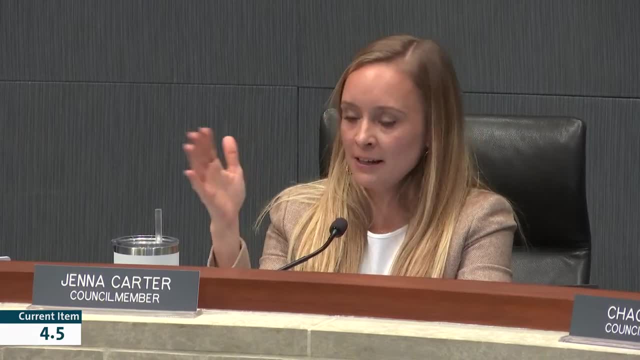 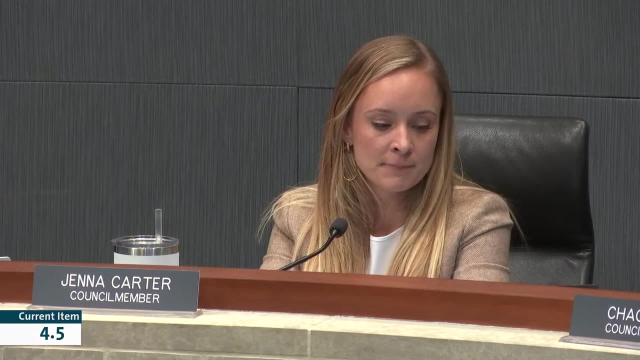 KNOW IF WE HAD THE CONVERSATIONS RELATED TO WHERE THESE PROJECTS ARE GOING TO BE. AND SO, AGAIN, I TOTALLY AGREE AND I THINK FOR THIS PROPOSAL MOVING FORWARD. I THINK THAT'S PART OF THE CHALLENGE THAT THESE 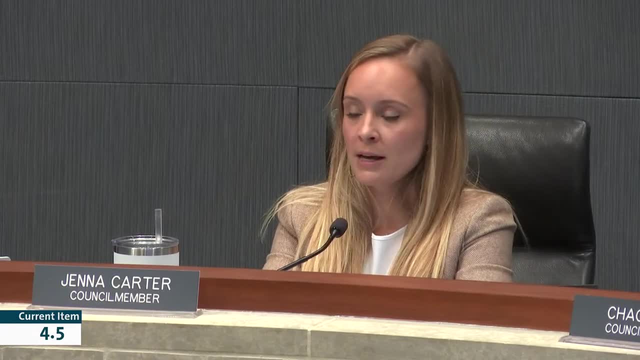 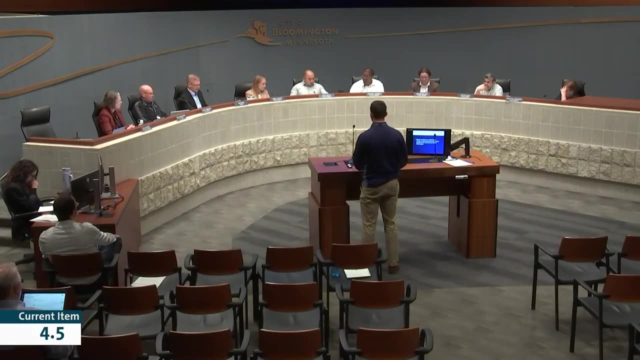 PROJECTS TAKE SO LONG AND, IN PARTICULAR, I THINK, THIS ONE HAD SOME MORE COMPLEXITY TO IT, AND SO, YEAH, THANK YOU. SO COUNCIL ON THE DOCUMENTS IN FRONT OF YOU, THIS DOESN'T. 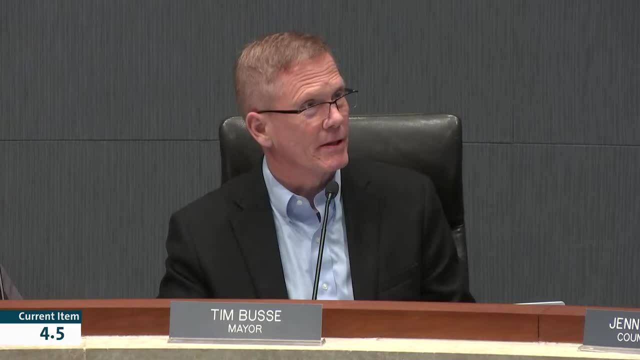 INDICATE THAT THIS IS A PUBLIC HEARING. THIS WAS NOTICED AS A PUBLIC HEARING SOME OF THESE, SO IT IS GOING TO BE A PUBLIC HEARING. WE'RE GOING TO CALL IT AS TWO SEPARATE PUBLIC HEARINGS. 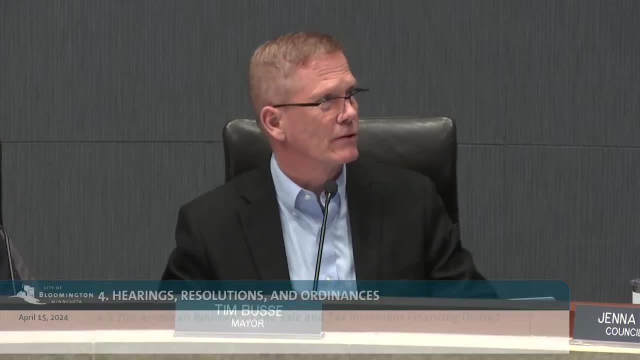 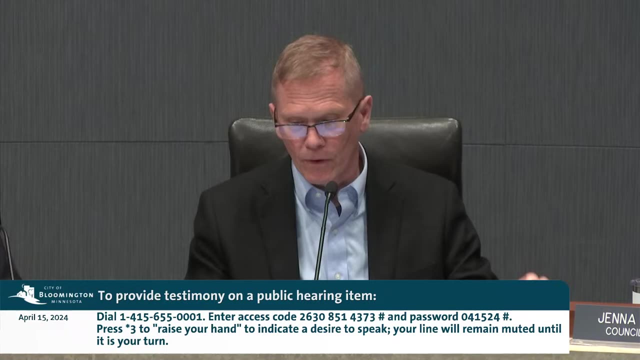 HOWEVER, AS I SAID WITHIN THE DOCUMENTS THAT YOU HAD, IT WASN'T OFFICIALLY NOTED IN THAT WAY. SO WHAT I'M GOING TO DO IF THERE'S NO ADDITIONAL QUESTIONS AND I'D LIKE TO MOVE FORWARD ON. 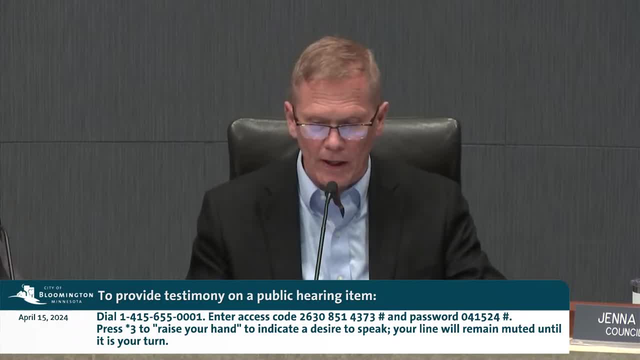 THIS WE HAVE TO CALL AT LEAST A COUPLE OF PUBLIC HEARINGS, SO I'M GOING TO CALL REGARDING ITEM 4.5,. I'M GOING TO CALL THE FIRST PUBLIC HEARING AND THIS WILL BE REGARDING THE. 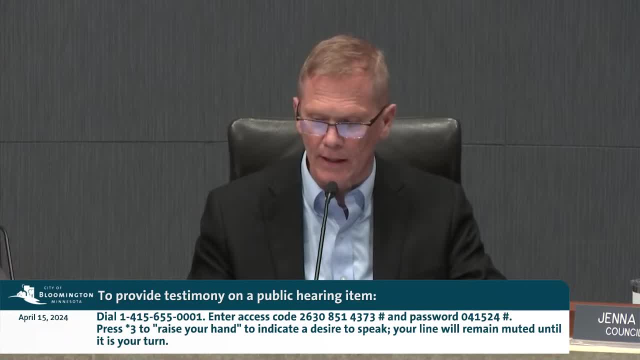 ORDINANCE TO CONVEY BY QUIT CLAIM DEED REAL PROPERTY LOCATED IN AND OWNED BY THE CITY OF BLOOMINGTON. IT'S THE LAND SALE IS WHAT THIS FIRST PUBLIC HEARING IS ABOUT. IS THERE ANYONE HERE IN THE 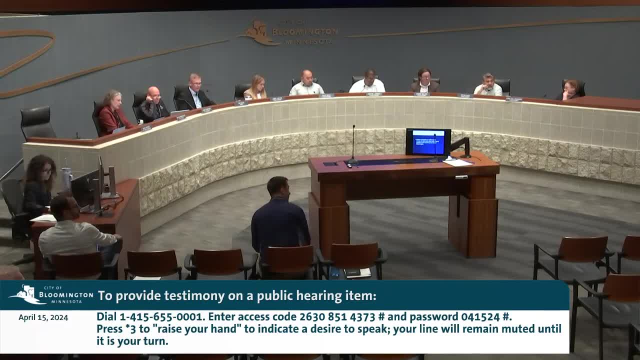 COUNCIL CHAMBERS. WHO WISHES TO SPEAK TO THAT PART OF ITEM 4.5 THIS EVENING? MAYOR AND COUNCIL, MY NAME IS BRIAN SAVIG. THIS IS A LITTLE ABOUT MY PAY. 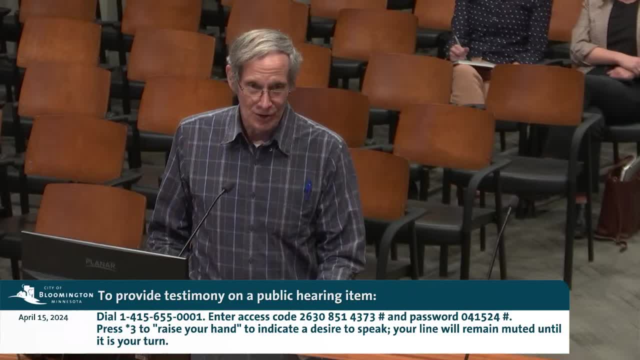 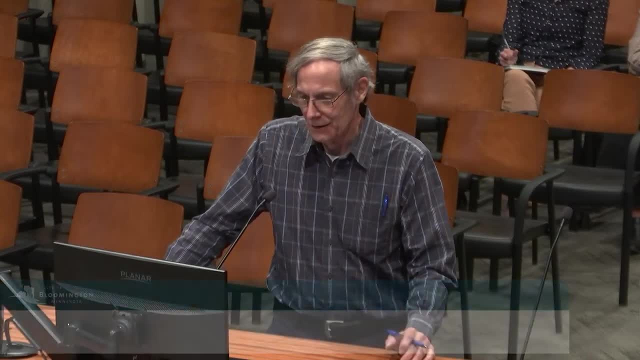 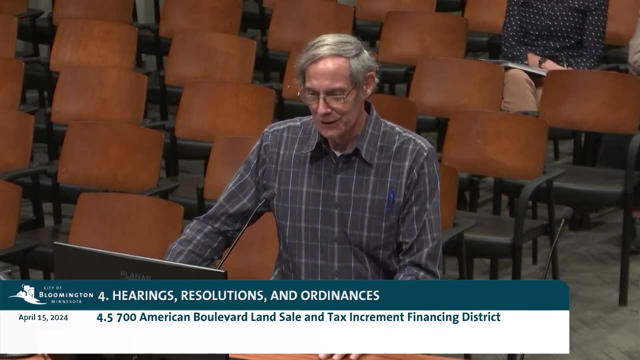 GRADE IN TERMS OF UNDERSTANDING HOW ALL THESE THINGS WORK. BUT A CONCERN I HAVE IS, I GUESS, TWO-FOLD. ONE SEEMS RATHER DIFFICULT TO MOVE INTO AN APARTMENT AND PAY FULL RATE OR SOME PORTION. 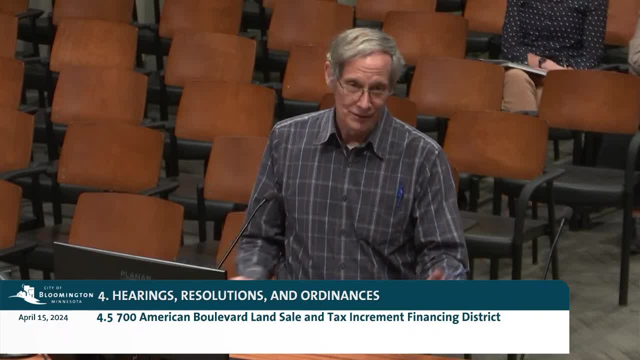 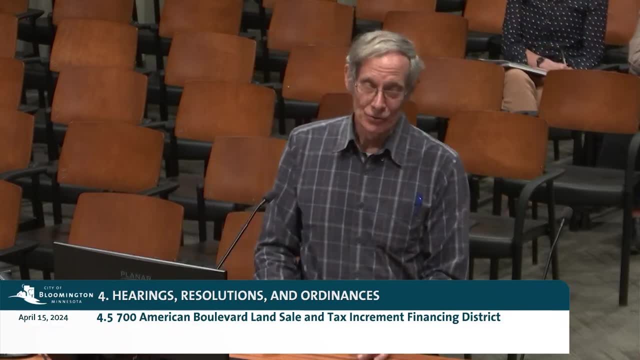 THEREOF, KNOWING. THE PERSON ACROSS THE HALL HAS THE SAME UNIT THAT I HAVE AND THEY'RE PAYING HALF OF WHAT I AM. THERE'S THAT ASPECT AND I DON'T UNDERSTAND HOW THAT WORKS. BUT SECONDLY, IS THERE ANY? 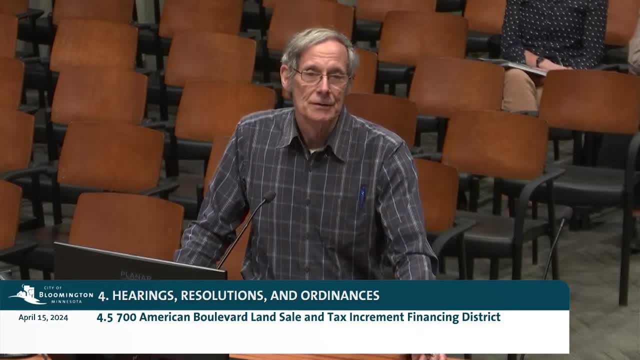 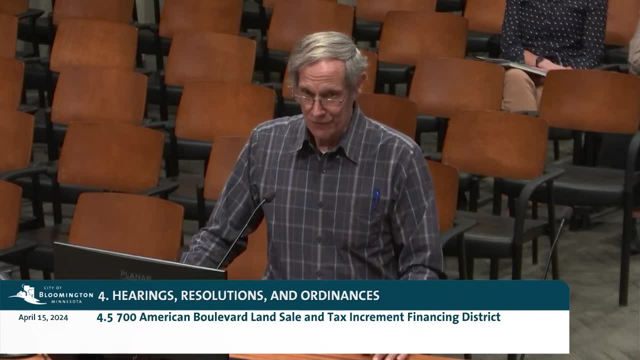 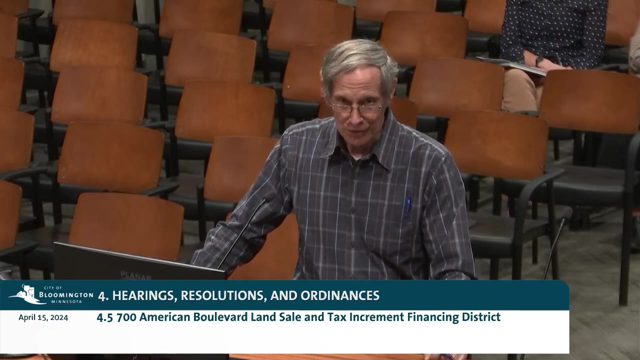 POSSIBILITY THAT BLOOMINGTON RESIDENTS WILL GET PRECEDENT IN PREFERRED TREATMENT IN TERMS OF IF THERE'S ONLY EIGHT UNITS DO BLOOMINGTON RESIDENTS THAT HAVE LIVED HERE 30 YEARS ARE THEY? 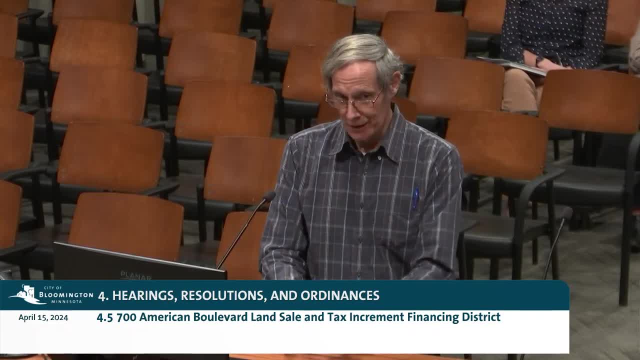 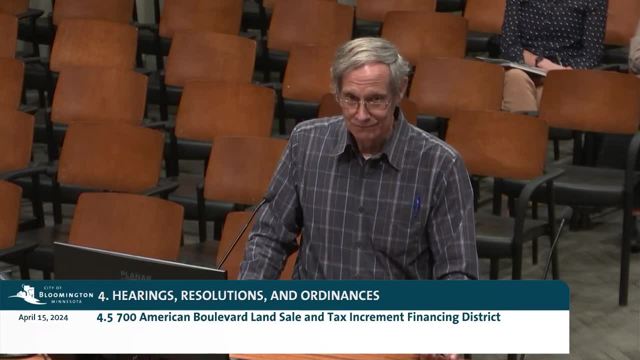 GOING TO HAVE A BETTER CHANCE OF GETTING ONE OF THOSE, THAN SOMEBODY THAT'S NEVER LIVED HERE BEFORE AND WALKS IN AND SAYS: I MAKE 27 GRAND A YEAR NEED ONE OF THOSE BECAUSE WE'RE TAKING A. 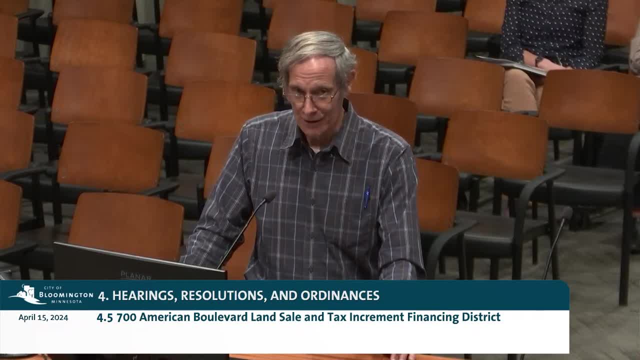 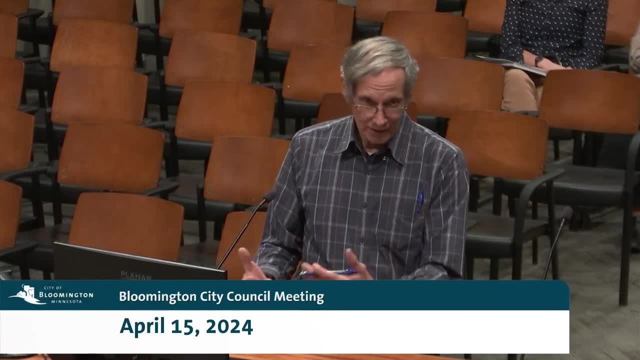 HAIRCUT OF ABOUT 50% ON THE PROPERTY. SO BLOOMINGTON RESIDENTS THAT HAVE LIVED HERE A WHILE HAVE PAID FOR THAT PROPERTY, PROBABLY PAID INTEREST ON IT WHILE IT WAS APPRECIATING AND 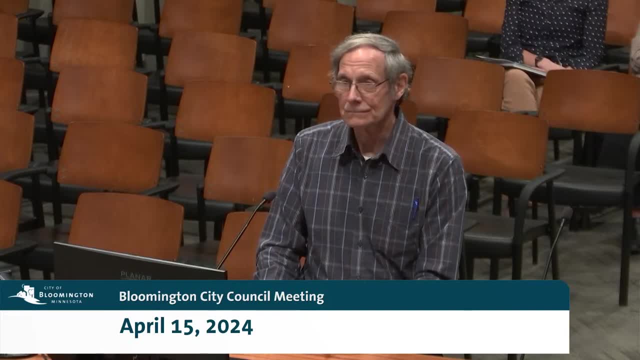 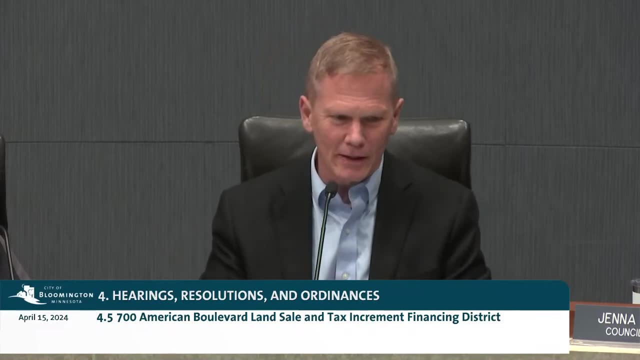 NOW WE'RE GOING TO WRITE OFF HALF OF IT. WE TYPICALLY WOULD HOLD AND ANSWER QUESTIONS AT THE END OF THE PUBLIC HEARING BUT BECAUSE THERE'S NO ONE ELSE HERE, I SUPPOSE WE CAN GET INTO THIS. 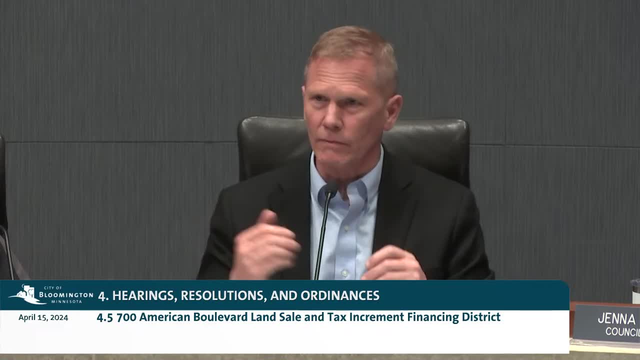 I THINK THE TWO ANSWERS TO YOUR QUESTIONS. FIRST OF ALL, THE NOTION OF SOMEBODY: ACROSS THE HALL NOT PAYING THE SAME, THAT'S BEEN. A POLICY DECISION OF THIS COUNCIL, THAT WE WANT. 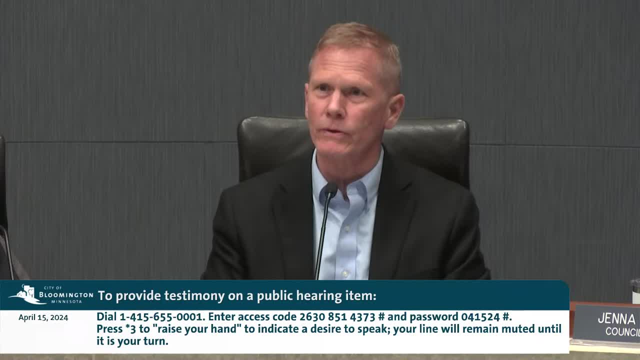 TO BE ABLE TO HAVE. WE WANT TO MAKE HOUSING AVAILABLE TO PEOPLE AT DIFFERENT INCOME LEVELS TO BE ABLE TO LIVE HERE IN BLOOMINGTON. WE WANT TO MAKE SURE THAT THE FOLKS WHO- I THINK YOU- HEARD IT. 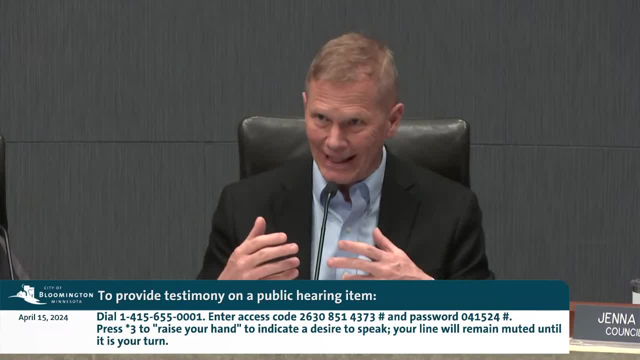 EARLIER, NOT AS A PLACE THAT PEOPLE WANT TO BE, BUT THEY CAN BE AND LIVE IN THE CITY OF BLOOMINGTON. SO THAT'S A COUNCIL DECISION AND A POLICY DECISION. THAT I THINK THE COUNCIL HAS BEEN. 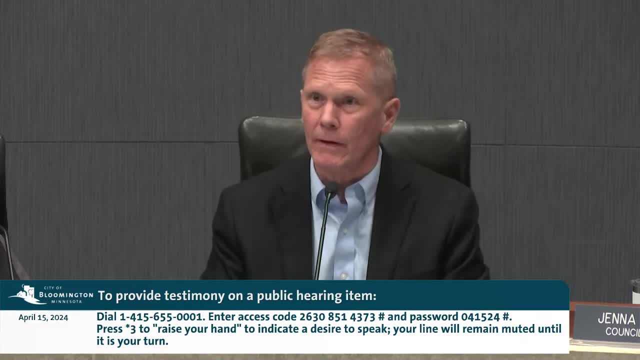 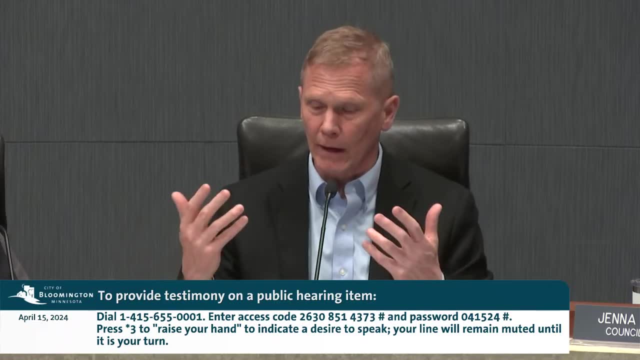 PRETTY ROCK SOLID ON FOR A NUMBER OF YEARS NOW ALONG THOSE LINES, IN TERMS OF WHO IT'S RENTED TO. I DON'T THINK WE CAN SAY THAT THIS EVENING, BECAUSE THAT'S YOU KNOW. I DON'T KNOW THAT WE. 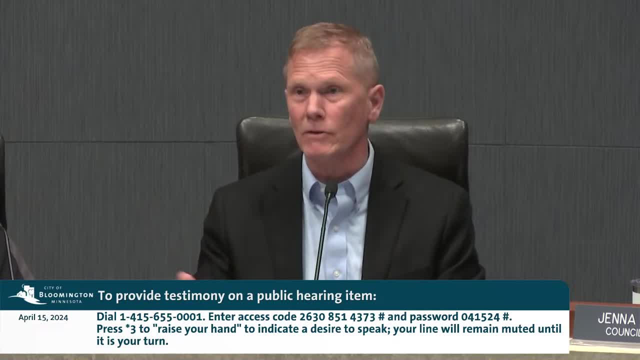 CAN SPECIFICALLY SAY IT'S ONLY AVAILABLE TO BLOOMINGTON BECAUSE, AS WE SELL THIS TO A PRIVATE DEVELOPER, THEN IT BECOMES. AS LONG AS THEY MEET THE INCOME REQUIREMENTS, IT'S NOT WITHIN OUR JURISDICTION. 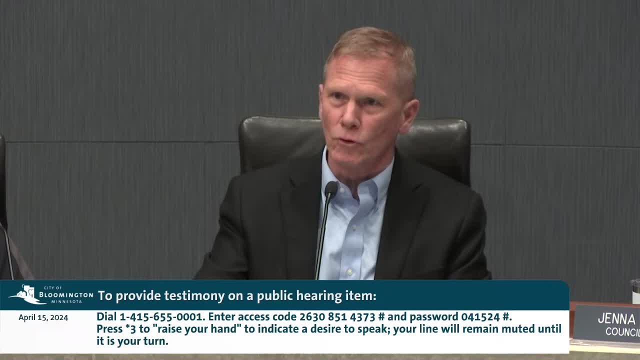 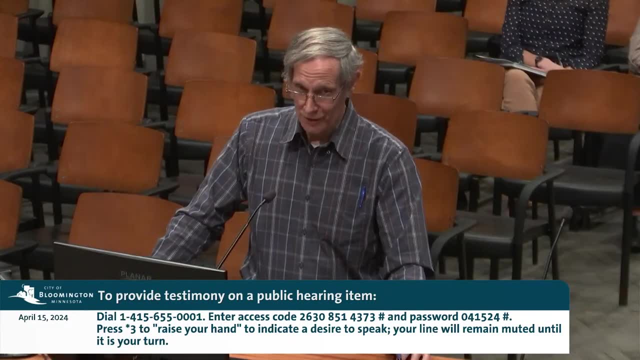 IT'S NOT IN OUR HANDS ANY LONGER TO SAY WELL, YOU MUST RENT AT LEAST X AMOUNT TO BLOOMINGTON RESIDENTS. WE CAN'T DO THAT, OKAY, SO BLOOMINGTON RESIDENTS ARE. 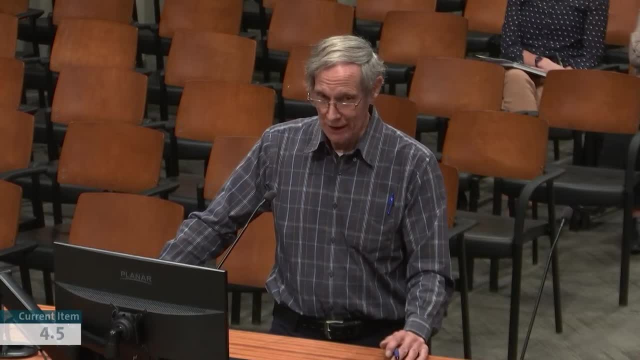 BEING ASKED TO TAKE THE HAIRCUT, BUT THEY DON'T NECESSARILY HAVE ANY ADVANTAGE IN GETTING THE BENEFIT FROM HAVING TAKEN THE HAIRCUT. WELL, I DON'T KNOW THAT I. 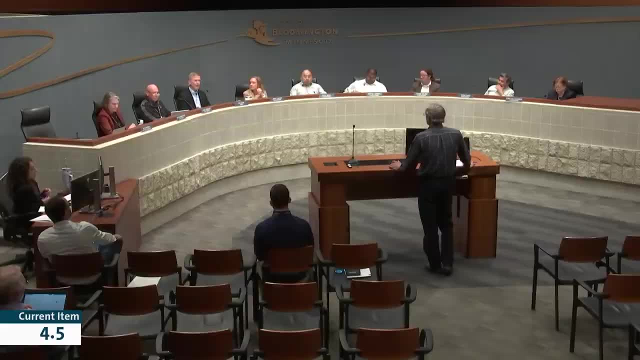 WOULD CHARACTERIZE IT AS TAKING THE HAIRCUT AGAIN. IT'S A POLICY DECISION BY THE COUNCIL. WELL, I MEANT ON THE WRITE-OFF, ON THE WRITE-OFF ON THE SALE OF THE LAND. 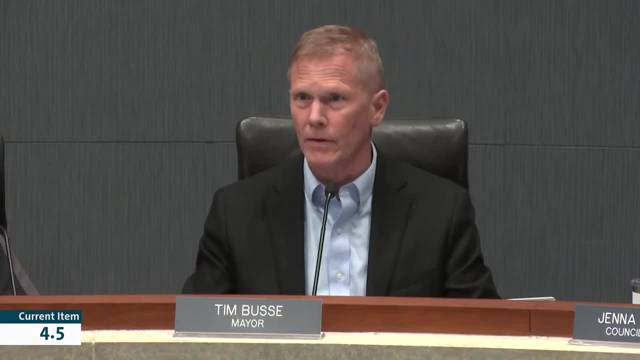 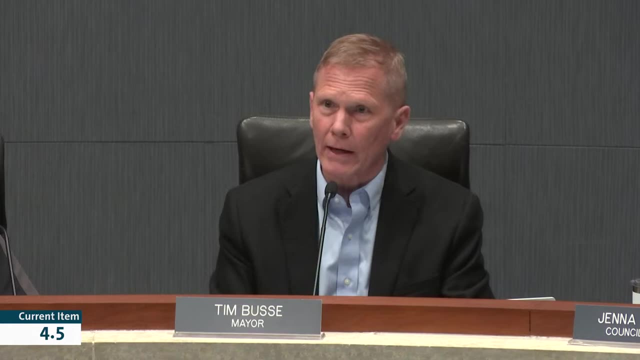 THAT'S PART OF THE POLICY DECISION. IT'S THE WRITE-OFF IS MAKING THOSE APARTMENTS AVAILABLE TO LOW-INCOME FOLKS. BUT YOU ARE CORRECT, WE CANNOT, AS WE JUST CAN'T DO THAT, WE CAN'T GUARANTEE SPOTS TO. 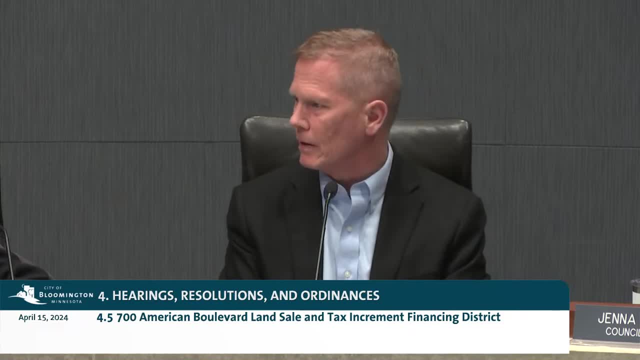 SPECIFIC PEOPLE AND SPECIFIC RESIDENTS OF BLOOMINGTON. MS MANDERSHEID, AM I CORRECT IN SAYING IT IN THAT WAY? MAYOR AND MEMBERS, I THINK IT WOULD BE HELPFUL TO CLOSE. 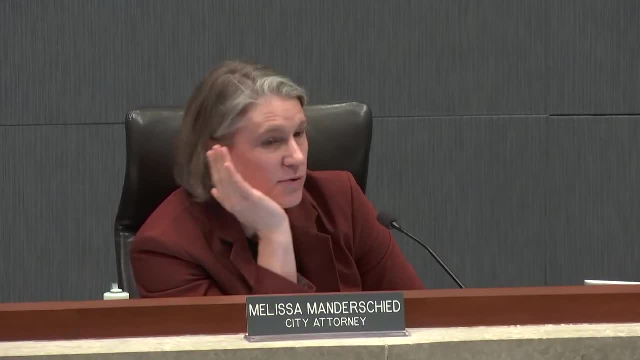 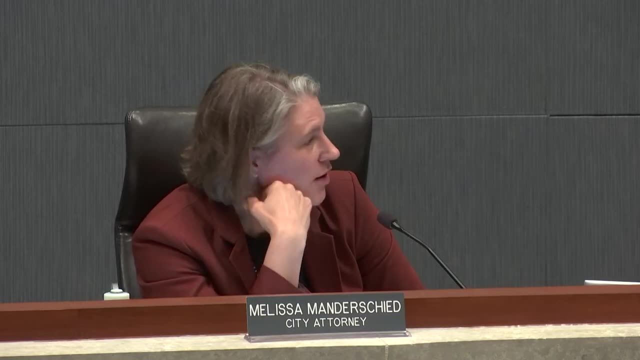 THE PUBLIC HEARING AND SEE IF THERE'S ANY OTHER SPEAKERS, AND THEN WE CAN TALK WITH THE DEVELOPER ABOUT HOW THEY CHOOSE TO RENT. I WOULD SAY GENERALLY THAT IT'S A VERY REGULATED FIELD FOR HOUSING LAWS AND ALL KINDS OF 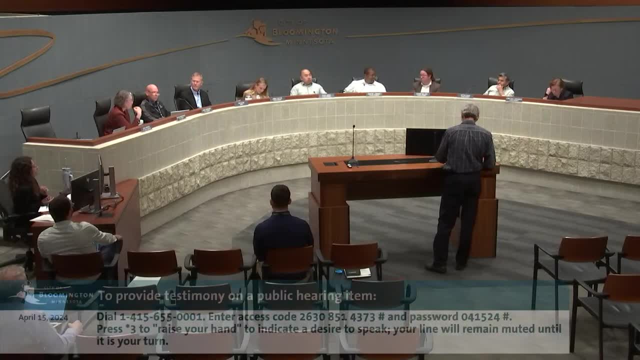 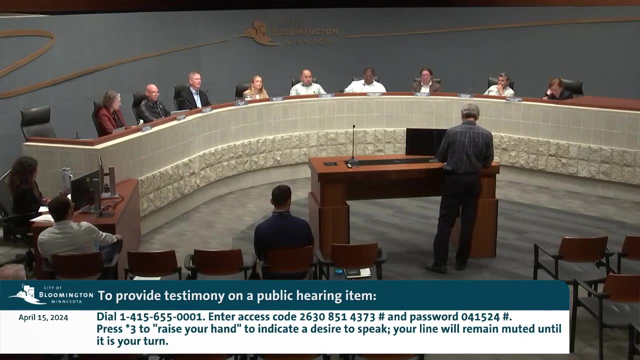 OTHER LAWS AND I'M SURE THAT THEY SEEK TO COMPLY WITH ALL OF THOSE. I'M SURE THEY DO. YEP 4.5 IS THE UNITED YES. IT IS YES. CAN I SAY A? 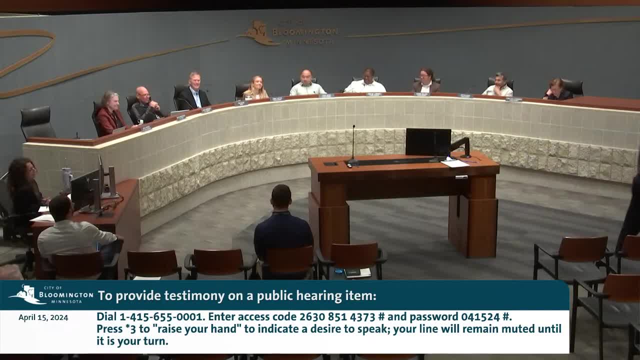 SURE. THAT WOULD BE GREAT. THANK YOU FOR CLARIFYING THAT. I APPRECIATE THAT. OTHERS IN THE COUNCIL CHAMBERS WISHING TO SPEAK ON THIS? MS MERCER, ANYONE WISHING TO? 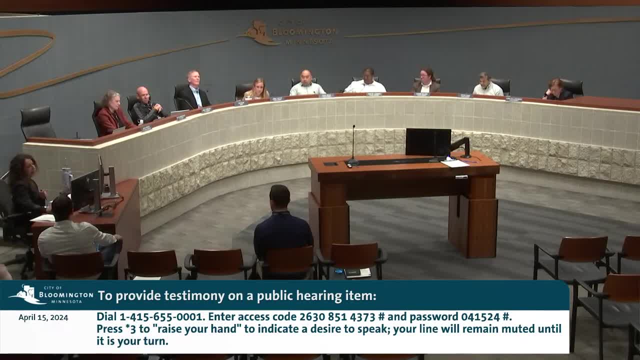 SPEAK ON 4.5 SEE, YOU'VE GOT THE NOTATION FOR US. WE'VE GOT THAT NAILED DOWN. WE'VE GOT THAT NAILED DOWN. THERE IS NO ONE ON THE PHONE. THERE COUNCIL. NO ONE COMING. 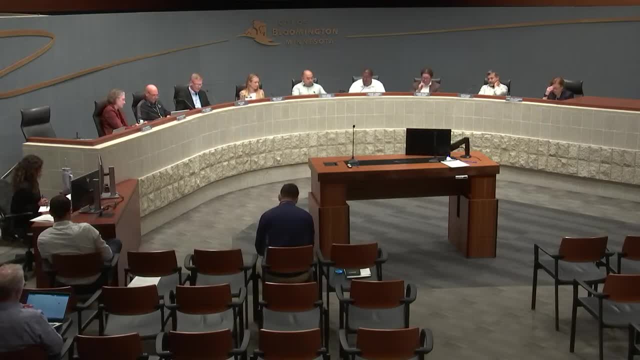 FORWARD NO ONE ON THE PHONE, I WILL LOOK TO CLOSE THE PUBLIC HEARING ON ITEM 4.5 REGARDING THE LAND SALE OF 700 AMERICAN BOULEVARD. SO MOVED MOTION BY COUNCILMEMBER. 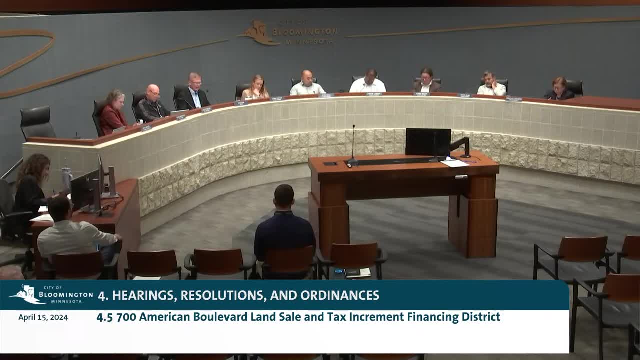 LOMAN, SECOND BY COUNCILMEMBER NELSON TO CLOSE THE PUBLIC HEARING ON THE LAND SALE PORTION OF THIS PUBLIC HEARING. JUST MAKING THIS AS DIFFICULT AS POSSIBLE, AREN'T WE TRYING TO NOTATE WHAT THE 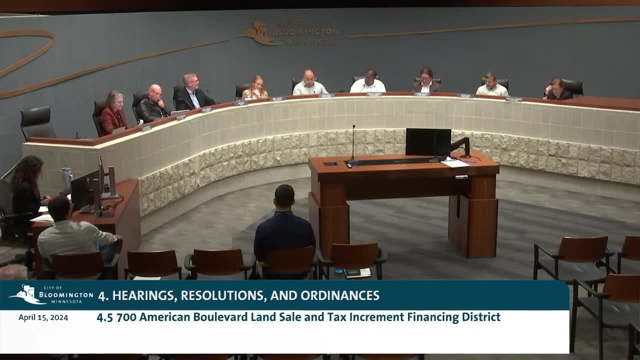 PEOPLE ARE TALKING ABOUT. WE HAVE A MOTION AND A SECOND TO CLOSE THAT PUBLIC HEARING: NO FURTHER COUNCIL DISCUSSION ON THIS. ALL THOSE IN FAVOR, PLEASE SIGNIFY BY SAYING AYE. 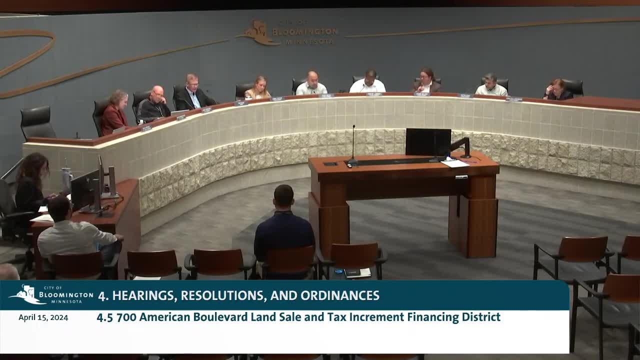 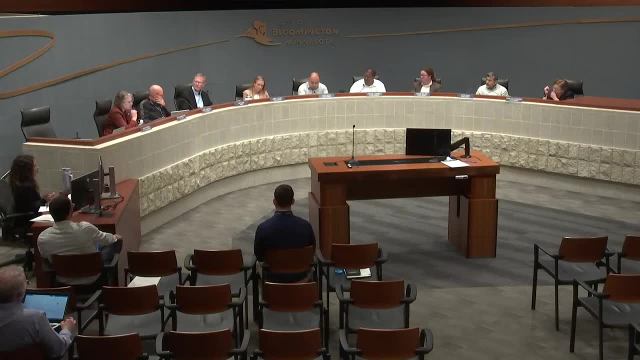 OPPOSED MOTION CARRIES 7-0.. NOW, WOULD IT MAKE SENSE TO GO RIGHT INTO THE NEXT PUBLIC HEARING, OR DO WE WANT TO ANSWER? SOME QUESTIONS MAYBE TALK SPECIFICALLY WITH THE 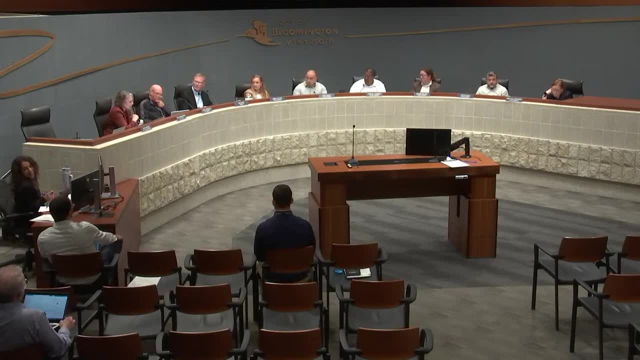 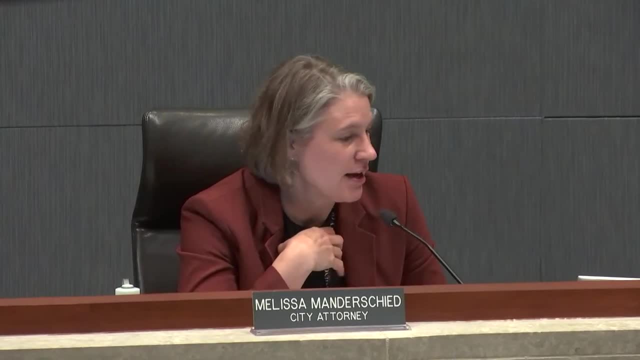 DEVELOPERS OR TAKE THE VOTE. HOW ARE WE DOING THIS ONE AT A TIME HERE, MAYOR MEMBERS? SO WHAT'S HAPPENING HERE? AND IF THIS IS CONFUSING, I WILL TAKE THE CREDIT FOR THAT, BECAUSE I TOLD 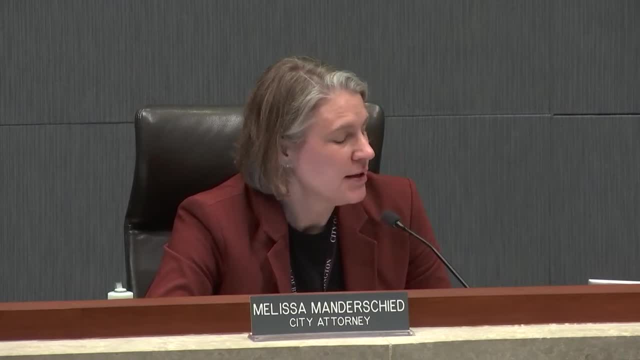 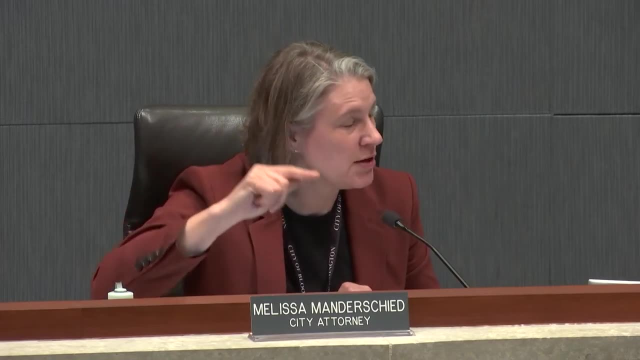 MR PALERMO, TO GROUP THEM ALL AS ONE AGENDA ITEM BECAUSE IN THE PAST, WHEN WE REDID THE AGENDA, THERE WAS A DESIRE, BECAUSE THE SAME PROJECT WAS SHOWING UP IN DIFFERENT PARTS OF THE AGENDA. 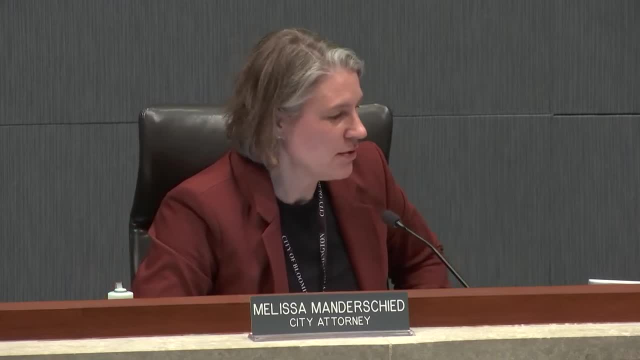 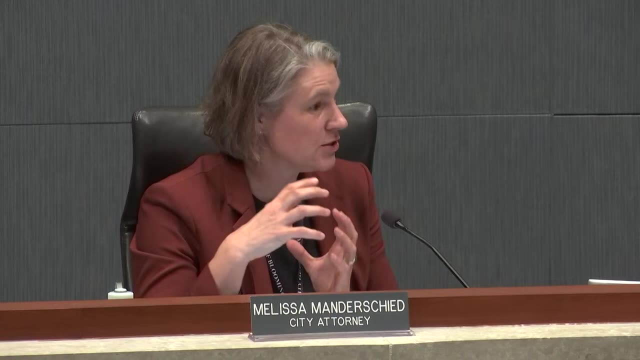 FOR THOSE OF YOU THAT HAVE BEEN HERE FOR A WHILE, AND SO, WHEN WE WORKED ON THAT, WE DECIDED WE WOULD GROUP THEM TOGETHER, SO ALL OF THE ACTIONS THAT RELATE TO 700 AMERICAN ARE COMING TO YOU AT THE SAME TIME. 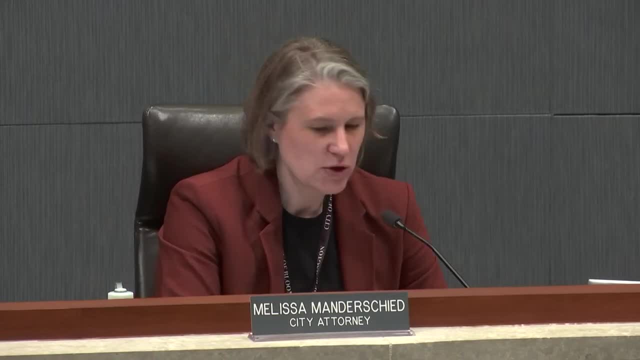 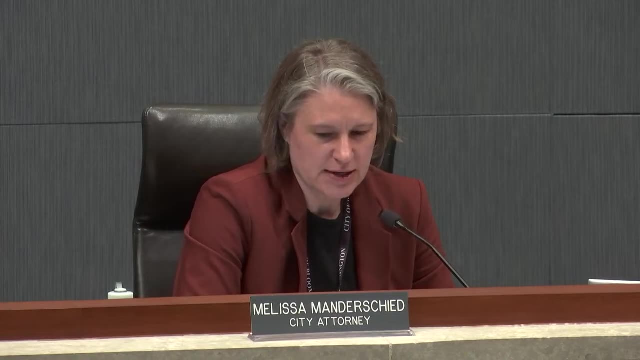 AT THE SAME AGENDA. SO WE COULD HAVE SAID THAT. WE COULD HAVE SAID PUBLIC HEARING IN THE TITLE, BUT WE DIDN'T TONIGHT. WE'LL DO A BETTER JOB NEXT TIME. IT IS CLEAR IN THE TEXT, JUST SO. 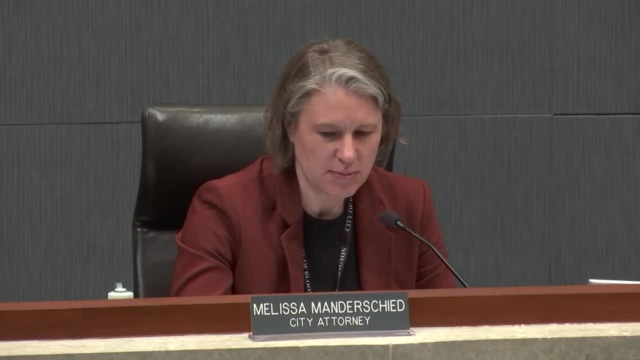 EVERYBODY KNOWS OF THE AGENDA ITEM. IF YOU SCROLL DOWN TO THE BOTTOM OF THE FIRST PAGE OF THE AGENDA ITEM, IT IS THERE. THERE'S ALSO TWO SEPARATE AFFIDAVITS OF PUBLIC HEARINGS, WHICH IS WHY WE'RE DOING TWO? 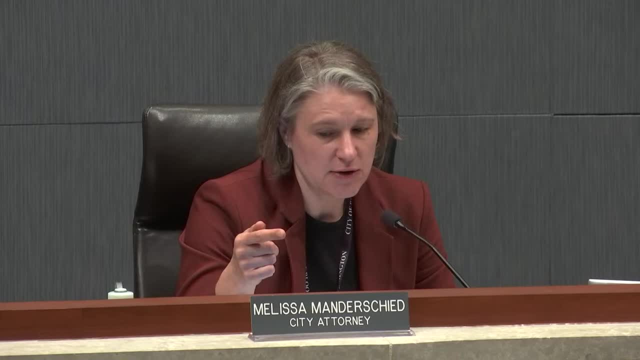 SEPARATE PUBLIC HEARINGS. SO THE FIRST PUBLIC HEARING IS REQUIRED, BECAUSE WE ARE CONVEYING LAND, FIVE VOTES ARE REQUIRED. THAT'S UNDER OUR CITY REGULATIONS. AND THE SECOND PUBLIC HEARING IS TO DISCUSS OR HOLD A PUBLIC. 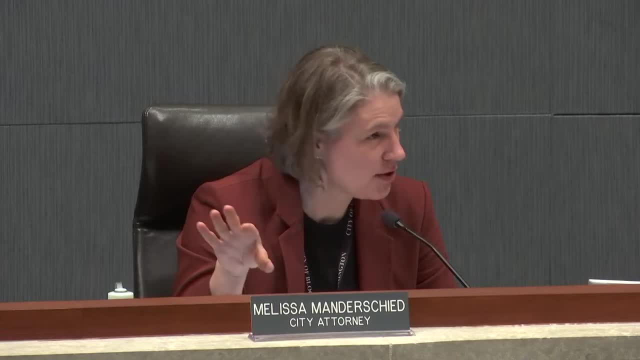 HEARING ON THE CREATION OF A TIF DISTRICT, WHICH IS A SEPARATE ACTION. SO, IF YOU'D LIKE, YOU CAN TAKE ACTION ON THE ORDINANCE TO CONVEY NOW AND THEN MOVE ON TO THE TIF, WHICH IS TWO KIND OF. 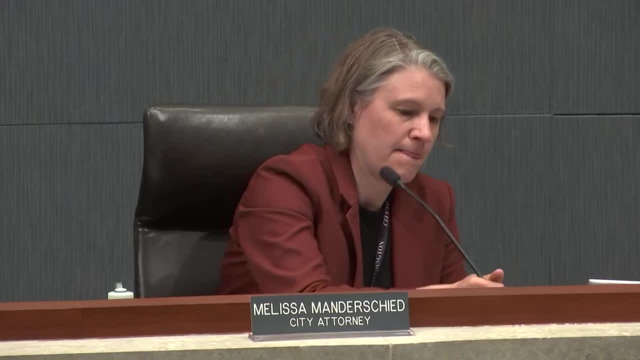 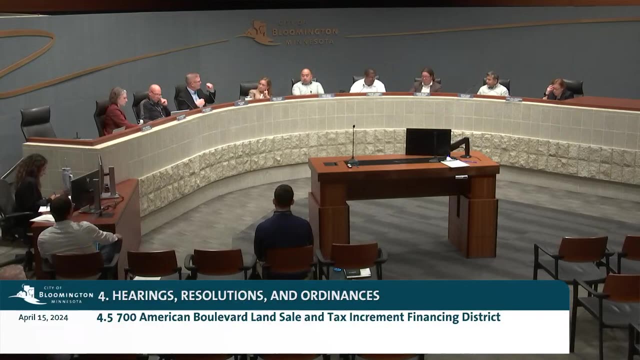 SEPARATE NOTIONS. VERY GOOD, LET'S DO THAT, THEN WE'LL TAKE THEM ONE AT A TIME HERE. SO WE'VE HAD THE PUBLIC HEARING ON THE CONVEYANCE, ON THE SALE QUESTIONS, AND THEN WE MOVE FORWARD ON. 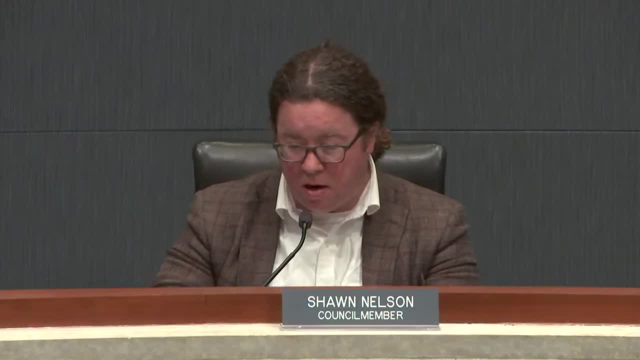 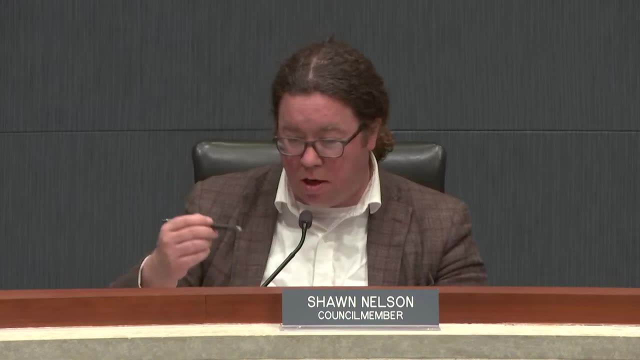 THIS COUNCIL MEMBER, NELSON. THANK YOU, MAYOR. NOT SO MUCH A QUESTION, BUT JUST TWO QUICK COMMENTS TO THE SPEAKER'S QUESTIONS. ONE: YOU WOULDN'T REALLY KNOW THAT THE PERSON ACROSS THE HALL. 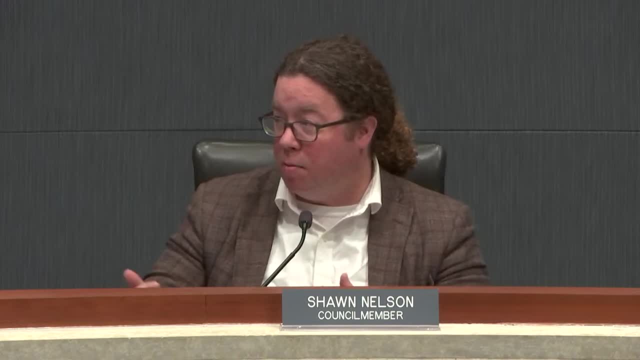 IS PAYING LESS BECAUSE THE UNITS ARE IDENTICAL. THAT'S ONE OF THE POLICY DECISIONS WE MADE AND WHY THOSE UNITS ARE IDENTICAL. IT'S, FRANKLY, ONE OF THE THINGS THAT I QUESTIONED A LOT. 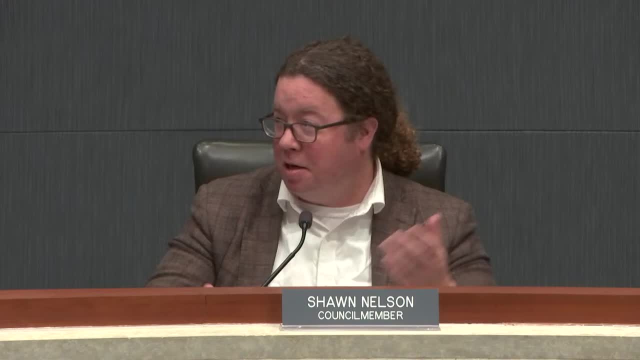 I WAS LIKE WELL, JUST PUT LESS EXPENSIVE STUFF IN IT. JUST LIKE MY NEIGHBOR'S HOUSE AND MY HOUSE MAY BE DIFFERENT. MAYBE THEY GOT NICER STUFF IN THEIR HOUSE. WHAT'S THE PROBLEM? 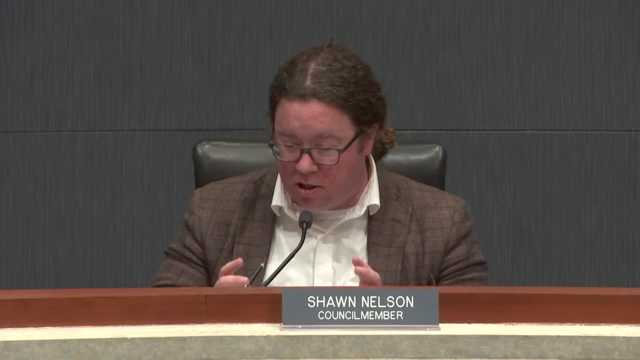 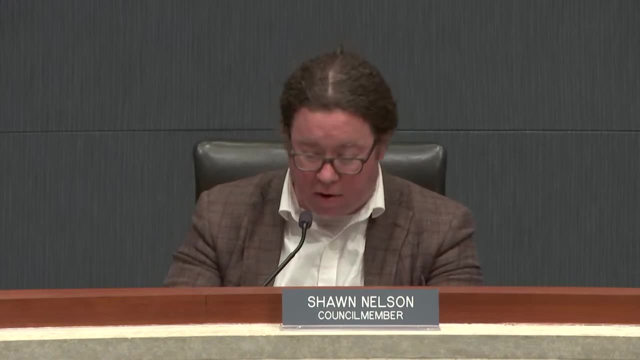 YOU WOULDN'T KNOW AND YOU CAN'T SEGREGATE OUT THE AFFORDABLE UNITS AND SAY, OH, THEY'RE OVER HERE, AND THEN EVERYONE WITH THE BAD VIEW AND ALL OF THAT STUFF. SO JUST TO CLARIFY THAT: 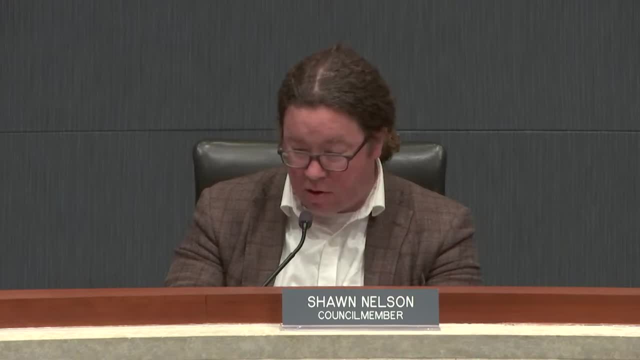 AND TO THE POINT OF FOR BLOOMINGTON RESIDENTS. IT'S ACTUALLY ONE OF THE REASONS THAT I HAVE, IN THE PAST SUPPORTED THIS, EVEN WITH THE MISGIVINGS THAT I RAISED AGAIN ABOUT THE AFFORDABILITY AND THE MIX OF 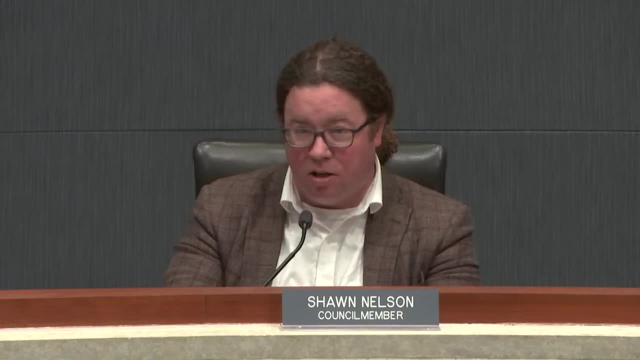 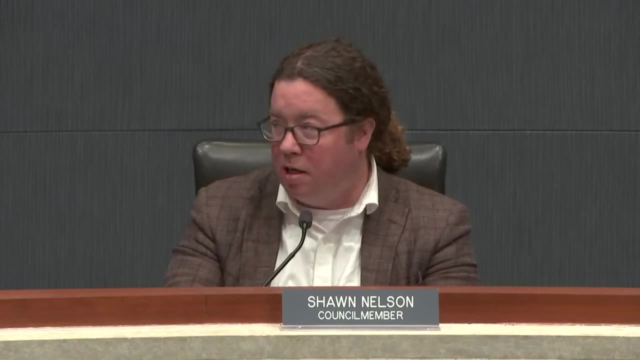 THAT THIS IS A SENIOR PROJECT AND I TALKED TO SO MANY PEOPLE THAT WANT TO STAY IN BLOOMINGTON AND I THINK THAT THE REASON AND THE REALITY IS PEOPLE WANT TO STAY IN BLOOMINGTON BUT 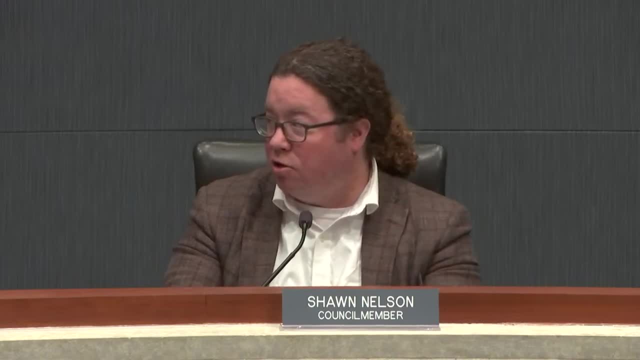 PEOPLE IN EDEN-PRAIRIE WANT TO STAY IN EDEN-PRAIRIE, AND PEOPLE IN COTTAGE-GROVE WANT TO STAY IN COTTAGE-GROVE, AND SO I THINK, PREDOMINATELY THE PEOPLE IN BLOOMINGTON THAT 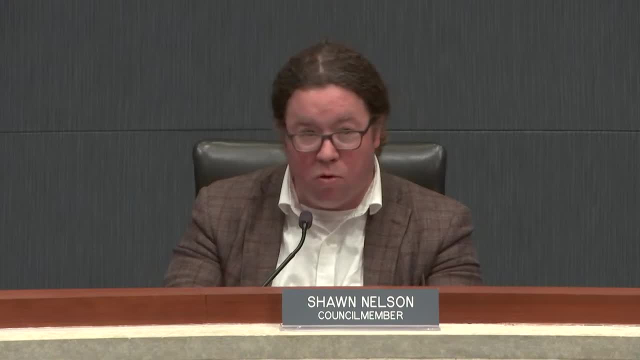 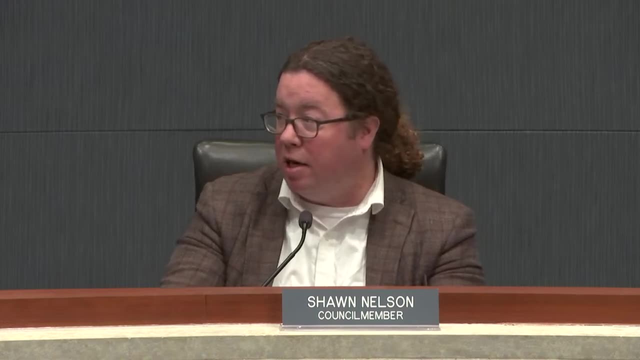 ARE LOOKING FOR THIS MAYBE TO DOWNSIZE OR TO MOVE. THEY'RE LOOKING IN BLOOMINGTON FIRST. I THINK OF MY AUNT AND UNCLE WHO DID THAT AND DIDN'T FIND IT AND ENDED UP IN EGAN INSTEAD. 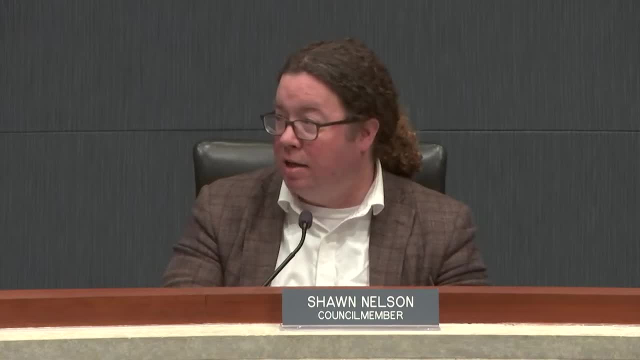 AND FURTHER DRIVE FROM THEIR FAMILY, FROM THEIR GRANDKIDS, ALL OF THAT. SO THAT'S WHY, THAT IS PROBABLY THE PARTICULAR REASON THAT I'VE SUPPORTED THIS PROJECT WITH MISGIVINGS THROUGHOUT. THAT IS BECAUSE I KNOW THAT THIS IS. 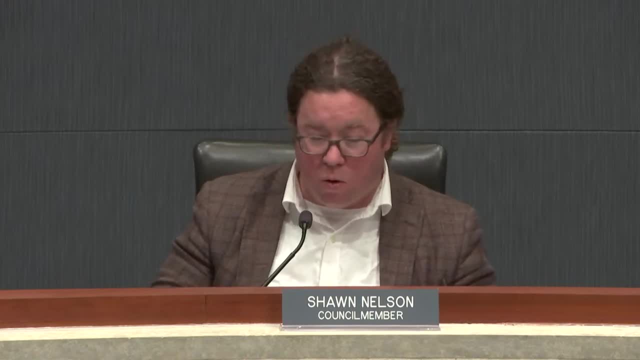 SOMETHING THAT PEOPLE ARE LOOKING FOR, AND IF WE HAVE IT HERE FOR THEM PREDOMINATELY, I TRULY BELIEVE IT WILL BE PEOPLE FROM BLOOMINGTON IN THERE. I WOULD AGREE WITH YOU. 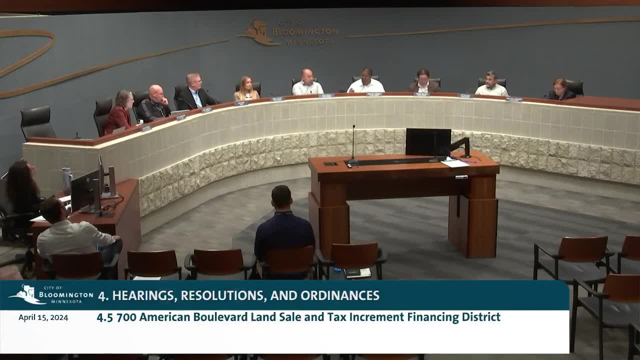 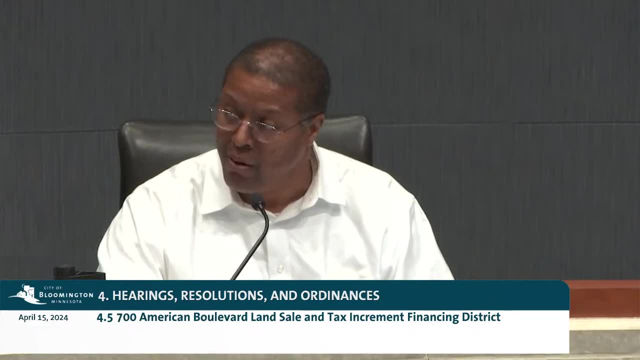 COUNCILMEMBER, COUNCILMEMBER, LOMENT, I'M READY TO MOVE IT. THE ONLY COMMENT I WOULD HAVE IS: ONCE YOU MOVE IN, YOU'RE NOW A BLOOMINGTON RESIDENT, SO THERE YOU GO. 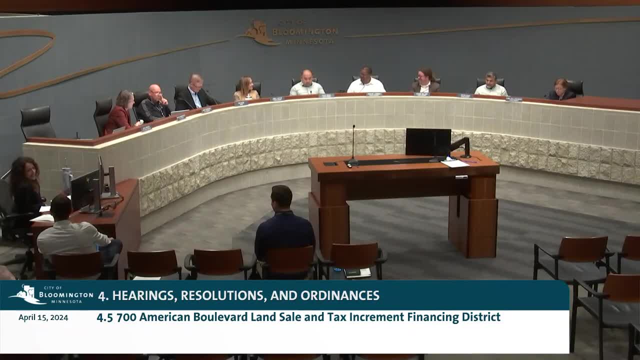 100% BLOOMINGTON. 100% BLOOMINGTON RESIDENT. WELL, THAT'S ONE DAY OR 30 YEARS. ANY OTHER COMMENTS? COUNCIL? OTHERWISE, I'M GOING TO ASK COUNCILMEMBER LOMENT FOR A. 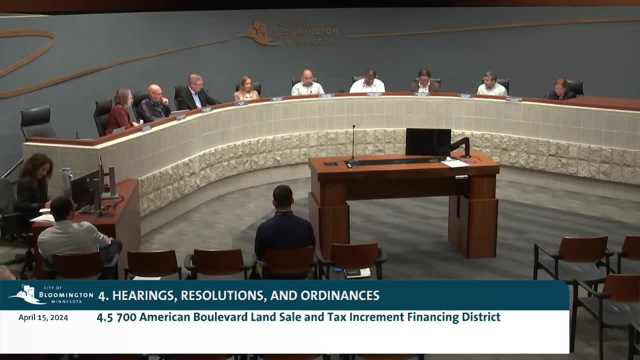 MOTION ON 4.5A HERE. OKAY, THEN I'LL MOVE TO APPROVE AN ORDINANCE TO CONVEY BY QUICK CLAIM. DEED: REAL PROPERTY LOCATED AND OWNED BY THE CITY OF BLOOMINGTON. MOTION BY COUNCILMEMBER. 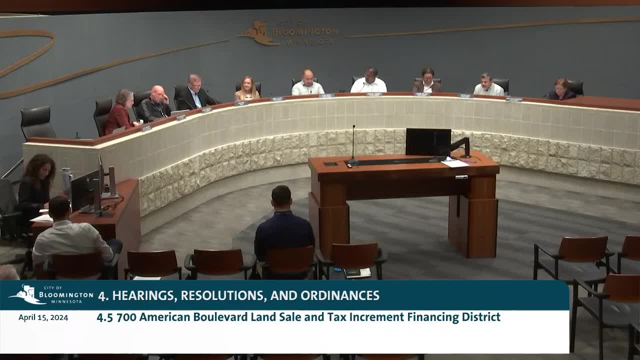 LOMENT SECOND BY COUNCILMEMBER RIVAS TO APPROVE THE ORDINANCE TO CONVEY BY QUICK CLAIM. DEED: REAL PROPERTY LOCATED IN AND OWNED BY THE CITY OF BLOOMINGTON: NO FURTHER COUNCIL DISCUSSION. 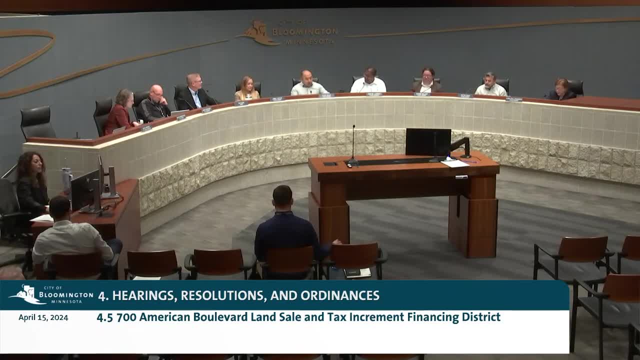 ON THIS. ALL THOSE IN FAVOR, PLEASE SIGNIFY BY SAYING AYE, AYE. OPPOSED MOTION CARRIES 7-0.. SO, WITH THAT, WITH 4.5A DONE, LET'S GO TO 4.5B AND WE'RE. 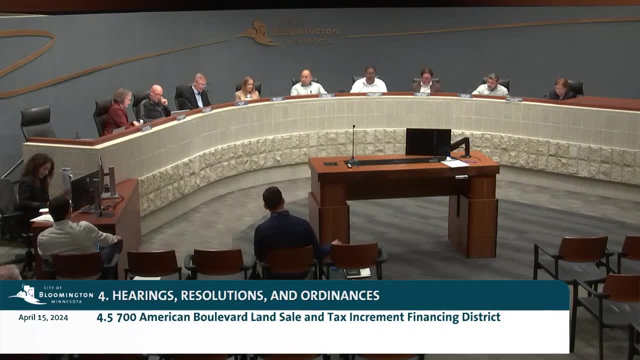 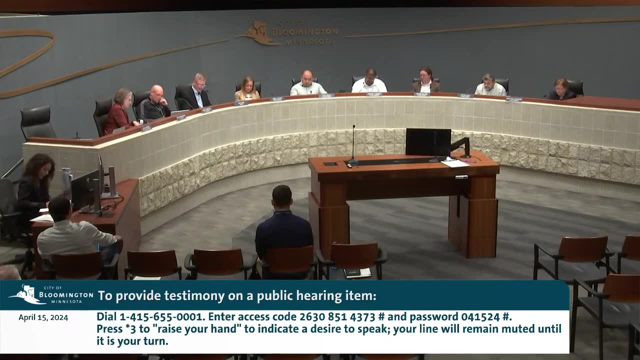 GOING TO OPEN UP A PUBLIC HEARING NOW ON THIS, AND THIS IS THE PUBLIC HEARING TO ESTABLISH THE TAX INCREMENT FINANCING DISTRICT AT 700 AMERICAN BOULEVARD AND TO APPROVE THE TAX INCREMENT FINANCING PLAN THEREFORE. 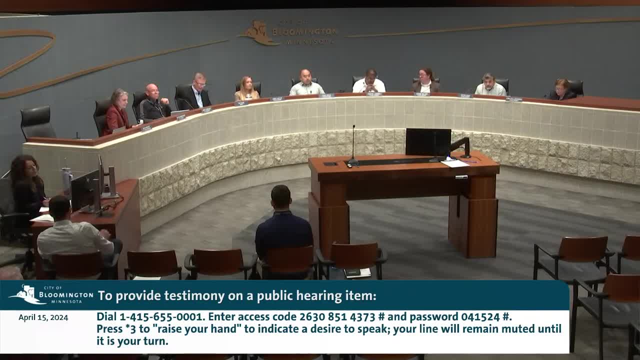 SO IS THERE ANYONE HERE IN THE COUNCIL CHAMBERS WISHING TO SPEAK ABOUT THE ESTABLISHMENT OF THE TAX INCREMENT FINANCING DISTRICT AT 700 AMERICAN BOULEVARD, MS MERCER, ANYONE ON THE? 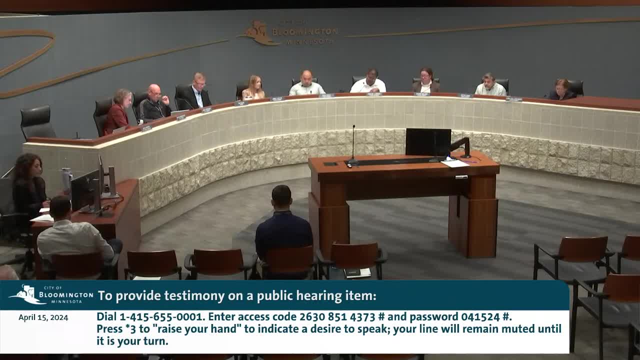 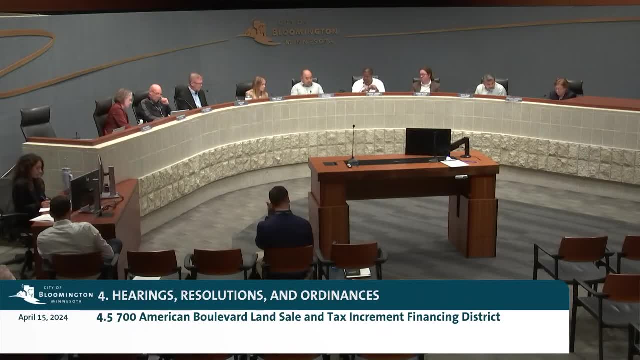 PHONE. NO ONE ON THE PHONE TONIGHT. LAST CALL IN THE CHAMBERS COUNCIL. I LOOK FOR A MOTION TO CLOSE THE PUBLIC HEARING ON 4.5B. ESTABLISHING THE 700 AMERICAN BOULEVARD. 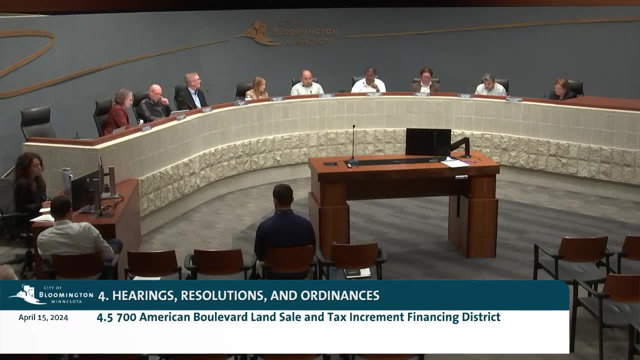 REDEVELOPMENT TAX INCREMENT FINANCING. SO MOVED. THAT'S STATED. SECOND MOTION BY COUNCIL MEMBER LOWMAN. SECOND BY COUNCIL MEMBER NELSON: TO CLOSE THE PUBLIC HEARING ON WHAT WE'RE. 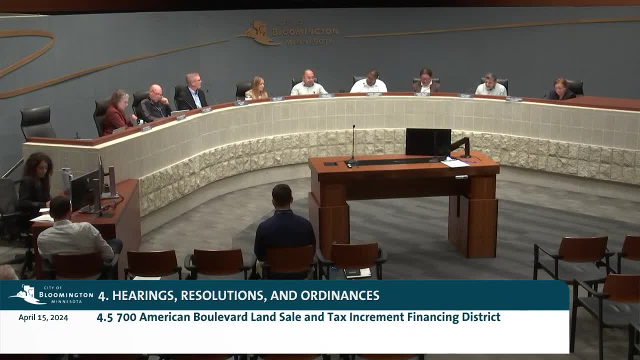 REFERRING TO AS 4.5B: NO FURTHER COMMENTS OR QUESTIONS BY THE COUNCIL ON THIS. ALL THOSE IN FAVOR, PLEASE SIGNIFY BY SAYING AYE, AYE, OPPOSED. 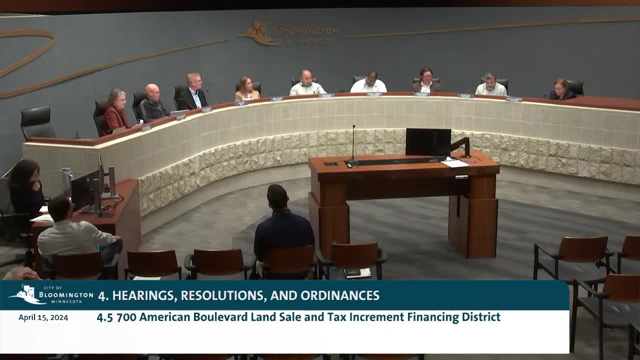 MOTION CARRIES 7-0.. COUNCIL. ANY QUESTIONS ON THIS? ANY ADDITIONAL INFORMATION NEEDED? IF NOT, I WOULD LOOK FOR ACTION ON THIS MAYOR. I'D BE HAPPY TO MAKE THAT MOTION UNLESS. 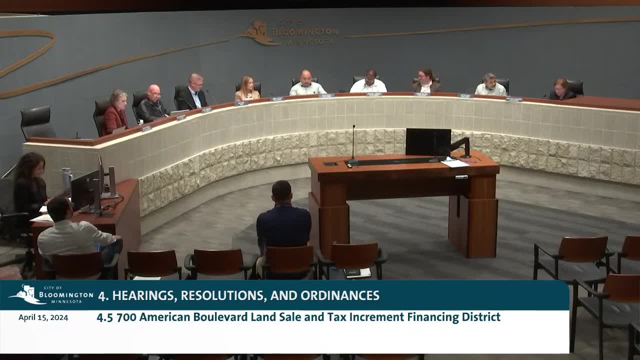 SOMEONE ELSE WANTS TO DO IT? COUNCIL MEMBER LOWMAN. ALL RIGHT, I'LL MOVE TO ADOPT A RESOLUTION ESTABLISHING THE 700 AMERICAN REDEVELOPMENT PROJECT. THEREFORE IN ESTABLISHING THE 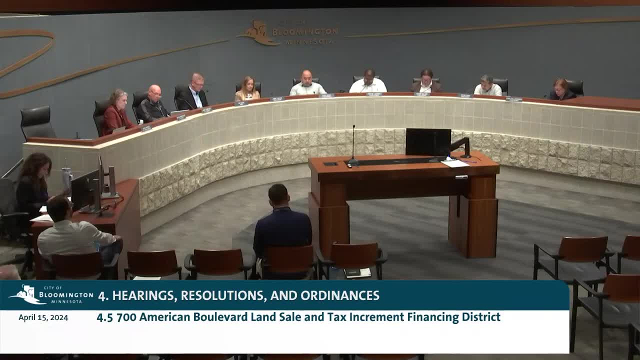 700. AMERICAN TAX INCREMENT FINANCING DISTRICT AND APPROVE A TAX INCREMENT FINANCING PLAN THEREFORE. SECOND MOTION BY COUNCIL MEMBER LOWMAN. SECOND BY COUNCIL MEMBER MUA, TO ESTABLISH THE. 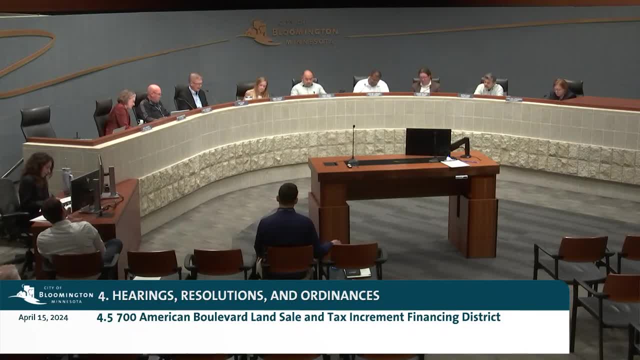 700 AMERICAN BOULEVARD REDEVELOPMENT PROJECT AND THE TAX INCREMENT FINANCING DISTRICT THEREFORE. NO FURTHER COUNCIL, COMMENT OR QUESTIONS ON THIS. ALL THOSE IN FAVOR. PLEASE SIGNIFY BY SAYING AYE. 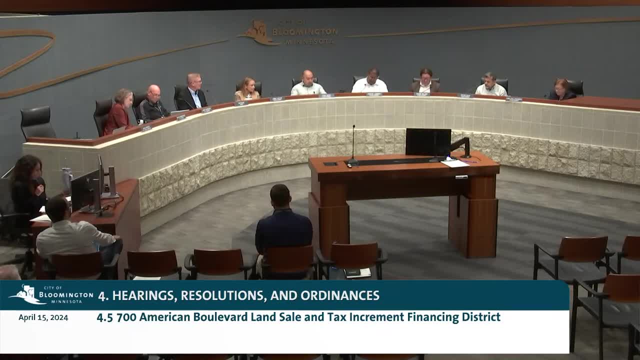 AYE. OPPOSED MOTION CARRIES 7-0.. COUNCIL MEMBER LOWMAN, WHY DON'T YOU BRING US ON HOME? ALL RIGHT, I'LL MOVE A RESOLUTION RELATING TO THE CITY'S TAXABLE. 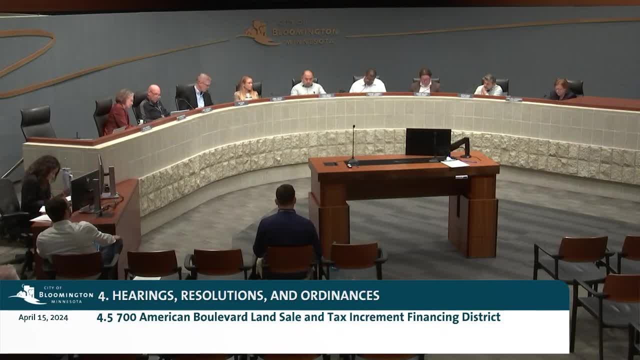 GENERAL OBLIGATION- TAX INCREMENT- REVENUE BONDS- SERIES 2019C. AMENDING RESOLUTIONS 2019-211, AS AMENDED BY RESOLUTION NUMBER 12,, 2020-190, AND APPROVING THE. 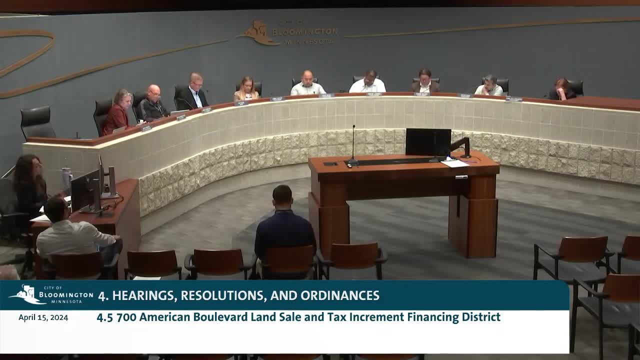 EXECUTION AND DELIVERY OF TAX INCREMENT. PLEDGE. AGREEMENT OF 70 AMERICAN TIF DISTRICT. MOTION BY COUNCIL MEMBER LOWMAN, SECOND BY COUNCIL MEMBER MUA, TO ADOPT THE RESOLUTION RELATING TO THE. 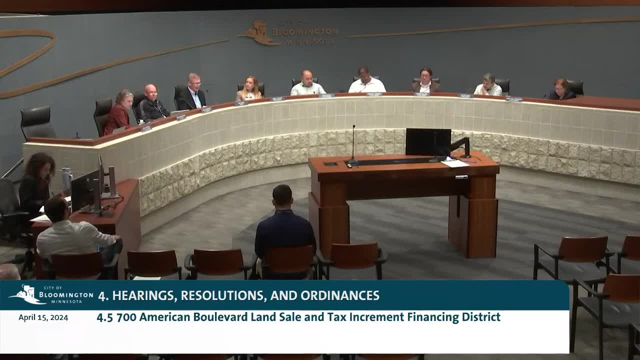 CITY'S TAXABLE GENERAL OBLIGATION: TAX INCREMENT, REVENUE BONDS. NO FURTHER COUNCIL DISCUSSION ON THIS. ALL THOSE IN FAVOR, PLEASE SIGNIFY BY SAYING AYE, AYE. 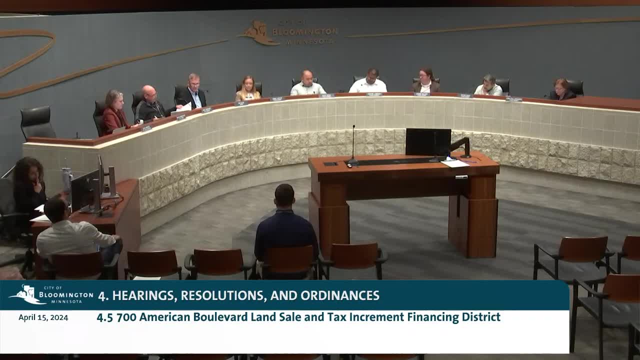 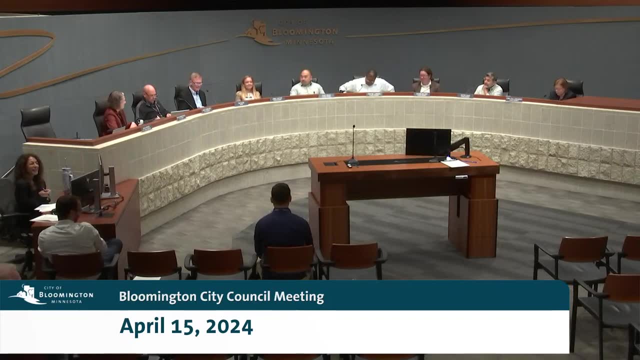 OPPOSED MOTION CARRIES 7-0.. THANK YOU. THANKS FOR THE CLARIFICATION ON THIS. THANK YOU FOR STICKING IT OUT WITH US. APPRECIATE IT. I KNOW IT GETS LATE SOMETIMES. 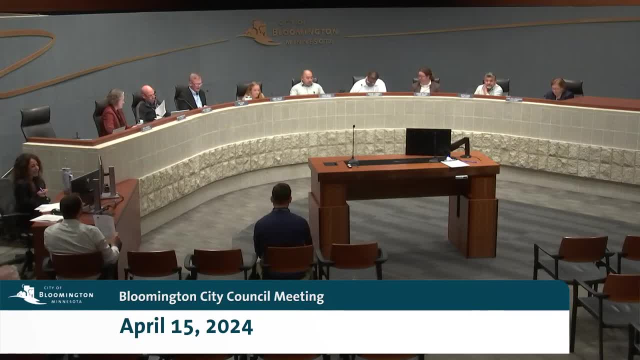 AND I APPRECIATE THAT YOU'RE STILL HERE. SO THANK YOU SO VERY MUCH. WE'LL MOVE ON TO OUR FINAL ITEM OF THE EVENING: OUR ORGANIZATIONAL BUSINESS, AS WE TALKED ABOUT EARLIER WE. 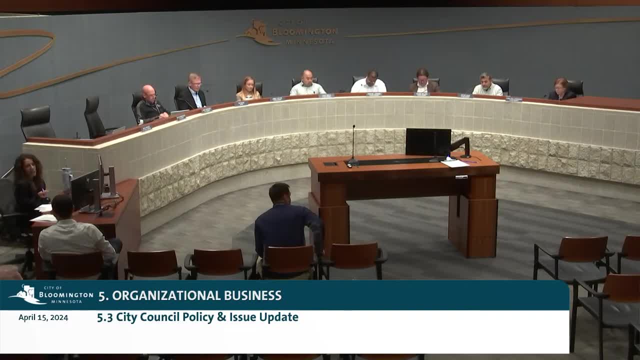 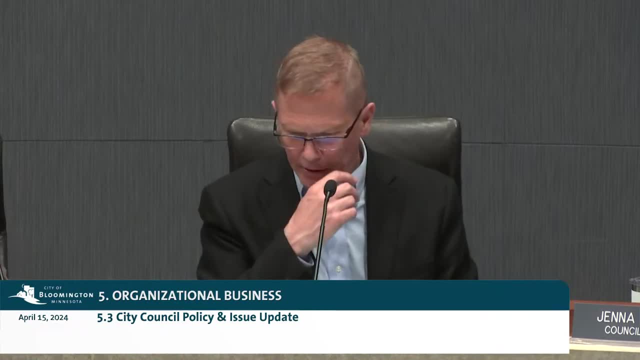 ALREADY COVERED ITEMS 5.1 AND 5.2 EARLIER IN THE AGENDA. THAT BRINGS US TO ITEM 5.3, OUR CITY COUNCIL POLICY AND ISSUE UPDATE FIRST UP, I'M GOING TO. 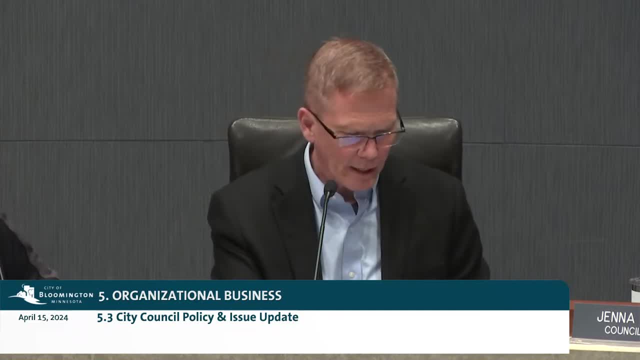 DO A QUICK SUMMARY OF OUR COUNCIL LISTENING SESSION. THAT WAS HELD AT 5.45.. WE ACTUALLY HAD FOUR SPEAKERS. SALLY NESS CONTINUED HER CONCERNS ABOUT DISABILITY PARKING AT 8200 PARK AVENUE. 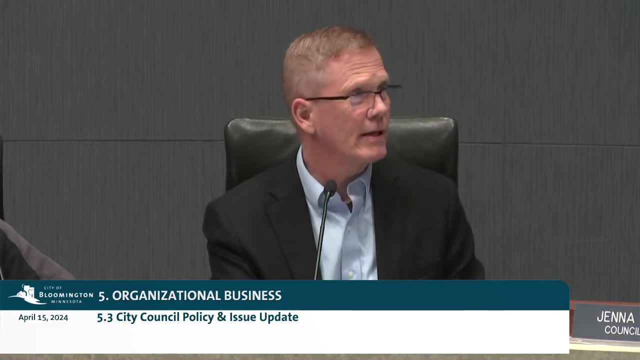 WE HEARD FROM MR BRIAN WOLFE. HE TALKED ABOUT NINE MILE CREEK AND MAINTAINING THE INTEGRITY OF NINE MILE CREEK AND THE ECOLOGICAL BALANCE WITHIN NINE. 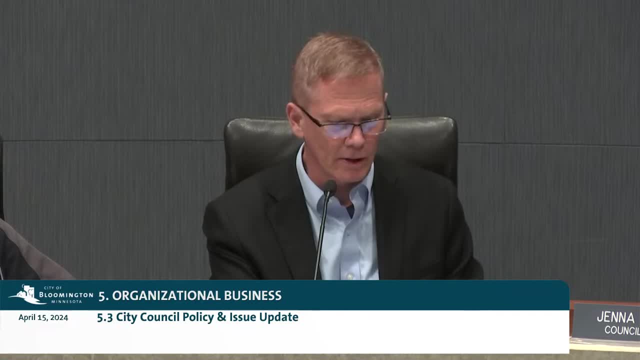 MILE CREEK A GOOD CONVERSATION AND GOOD DISCUSSION WITH HIM. WE HEARD FROM MR ANDY THOOLE WHO ASKED ABOUT THE INTEGRITY OF NINE MILE CREEK AND THE INTEGRITY OF NINE MILE. 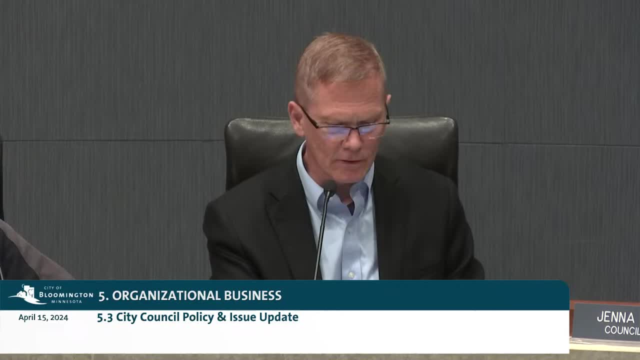 CREEK. HE TALKED ABOUT A VARIETY OF THINGS, INCLUDING THE CITY AND THE SCHOOL DISTRICT WORKING TOGETHER ON A CAREER FAIR. HIS CONCERNS ABOUT SHOPPING CARTS GOING ROGUE ONCE AGAIN ON. 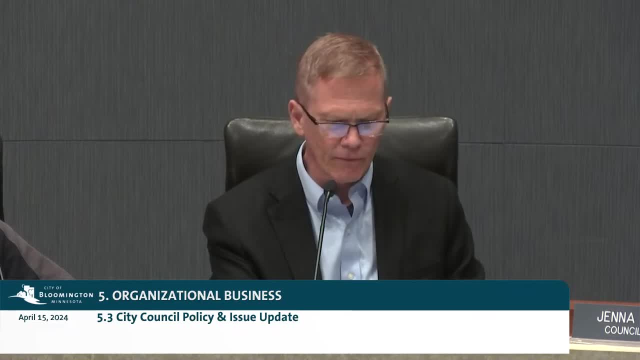 AMERICAN BOULEVARD, WHICH IS AN ISSUE WE'VE HAD IN THE PAST. SO WE'RE GOING TO TAKE A LOOK INTO THAT AND THEN ASKED IF THERE WAS ANY FOLLOW-UP REGARDING THE RECENT GUNFIRE AT DAR AL-FAROUK. 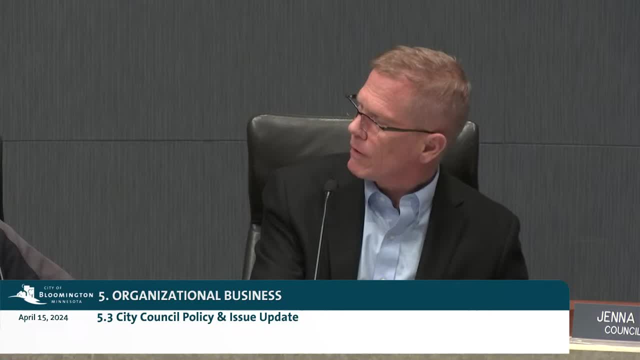 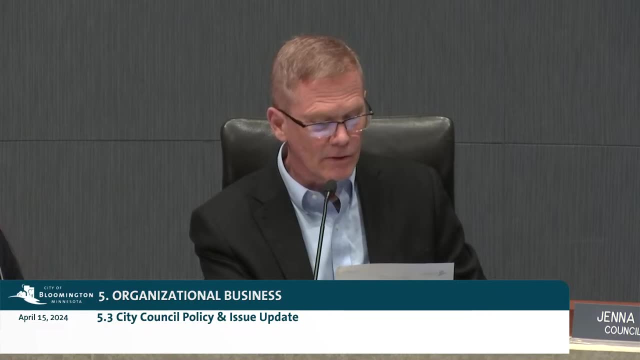 AND THERE WAS NOT ANY FOLLOW-UP FROM ROBERT, AND WHAT WAS ROBERT'S LAST NAME? ROBERT COLEMAN HAD A NUMBER OF QUESTIONS. HE WAS CONCERNED ABOUT THE TIME OF THE LISTENING SESSIONS. 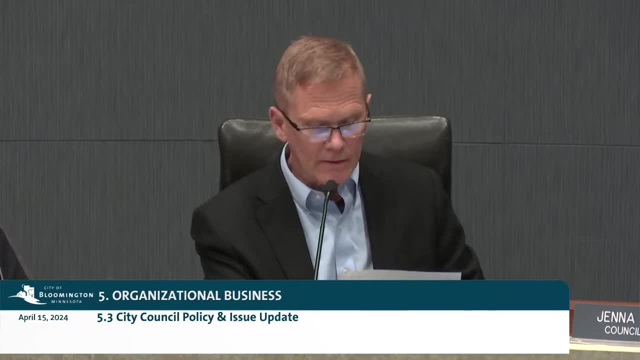 PRIMARILY BECAUSE HE HAD A HARD TIME GETTING TO THEM AND HE HAD SOME SIGNIFICANT CONCERNS ABOUT FINDING AN APARTMENT AND TALKED ABOUT THE COST, THE LOCATION, THE TRANSIT. 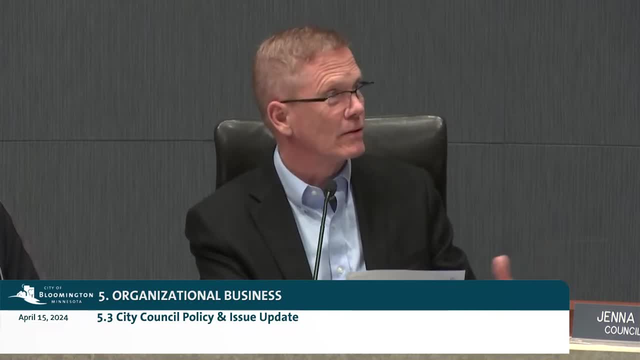 POSSIBILITIES, IT TIES INTO A LOT OF WHAT WE WERE TALKING ABOUT JUST HERE THIS EVENING, AND THE COUNCIL POLICY DECISIONS TO TRY AND MAKE THAT WORK OUT AND MAKE IT WORTHWHILE AND MAKE IT A PLACE WHERE. 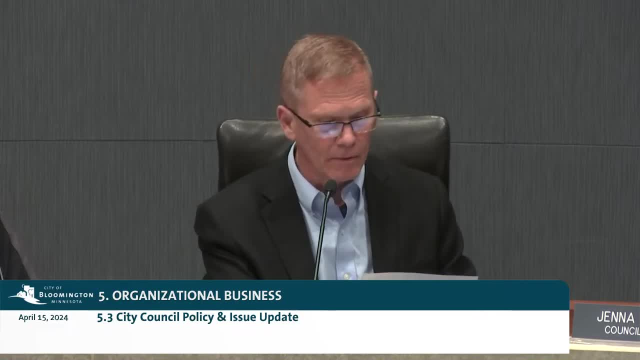 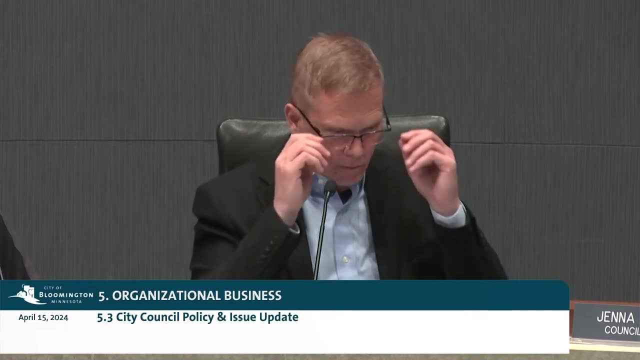 PEOPLE WANT TO BE, AND CAN BE, IN THE CITY OF BLOOMINGTON, SO IT'S GOOD TO CONSIDER THAT CONVERSATION WITH ROBERT THE ONLY OTHER ITEM THAT I HAVE I JUST WANTED TO REPORT. IN YESTERDAY I WAS OVER AT THE 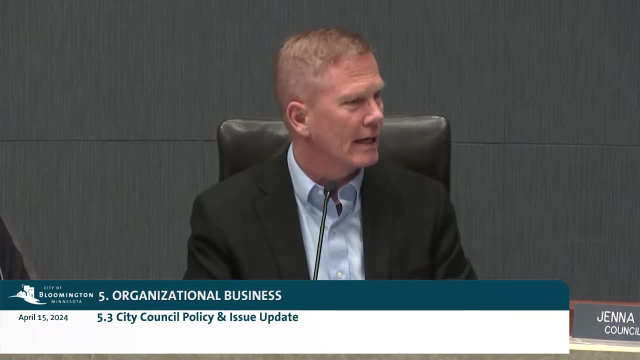 OAK GROVE PRESBYTERIAN CHURCH. THEY HAD AN OPPORTUNITY FAIR FOR THEIR CONGREGATION FOR ALL THE DIFFERENT NONPROFITS IN TOWN. BASICALLY AN OPPORTUNITY FOR THEIR CONGREGATION TO MEET THE 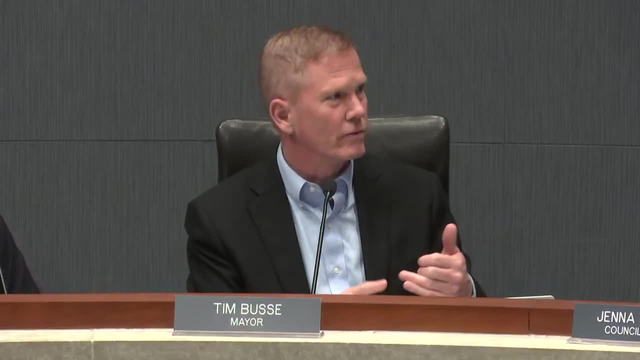 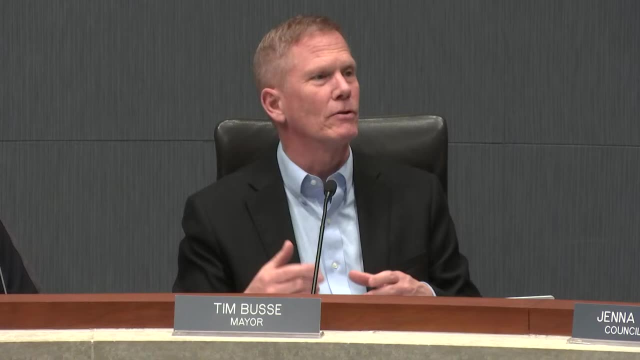 PEOPLE FROM OASIS AND CORNERSTONE AND EVERYBODY ELSE IN TOWN DOING DIFFERENT KINDS OF BRIDGING, EVERYBODY DOING DIFFERENT KINDS OF WORK, AND AN OPPORTUNITY FOR THEIR CONGREGATION TO SIGN UP AND TO. 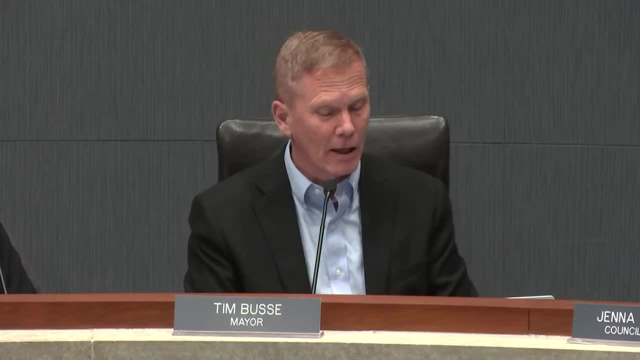 VOLUNTEER AND TO DO THINGS, AND IT WAS A FANTASTIC TIME. IT WAS GREAT TO GET EVERYBODY IN ONE PLACE. I'VE GOT NOTHING BUT COMPLIMENTS FOR THE OAK GROVE COMMUNITY OVER THERE. 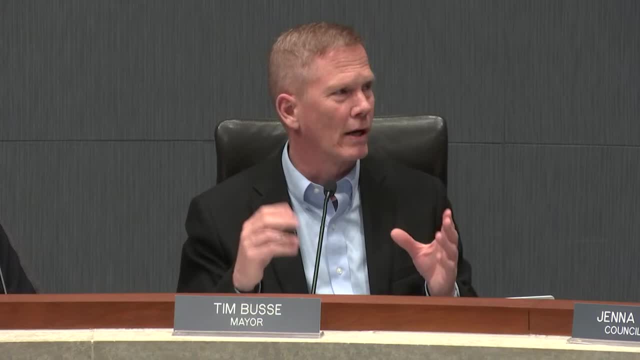 THEY NOT ONLY TALK THE TALK, THEY WALK THE WALK, THEY GET THE WORK DONE. I'M VERY IMPRESSED AND I JUST WANTED TO GIVE THEM THE PUBLIC SHOUT OUT AND THANK THEM FOR THE WORK THAT THEY DID BRINGING. 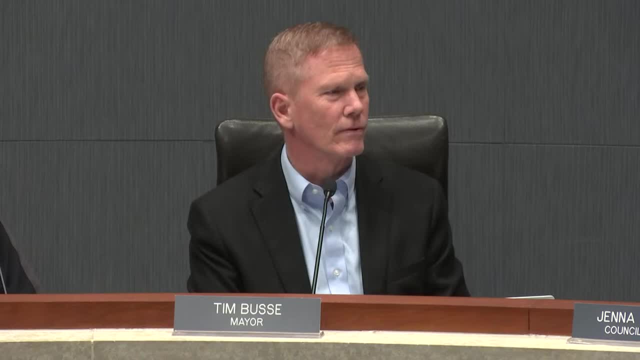 THEIR CONGREGATION TOGETHER AND HELPING OUT WITH OUR DIFFERENT SERVICE INDUSTRY OR SERVICE ORGANIZATIONS WITHIN THE CITY OF BLOOMINGTON. SO WELL DONE TO OUR FRIENDS AT OAK GROVE, PRESBYTERIAN. 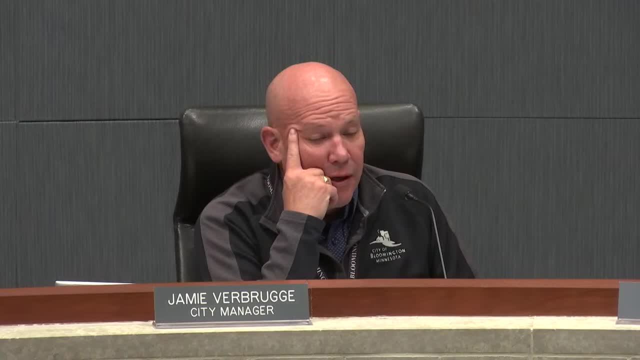 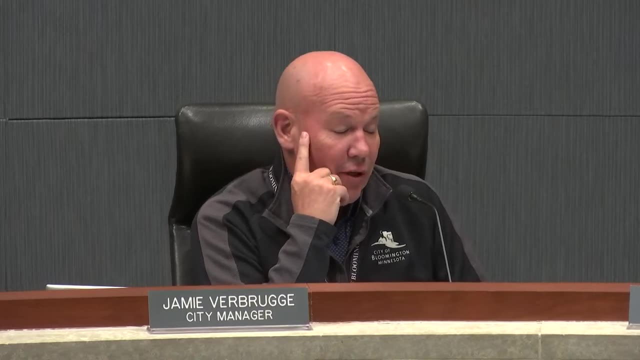 MR VERBRUGHI. THANK YOU, MR MAYOR AND COUNCIL MEMBERS. IT SEEMS A LITTLE EARLY TO BE SHARING THAT WE'VE GOT GOOD NEWS FROM THE LEGISLATURE, BUT WE ACTUALLY HAVE SOME GOOD NEWS. 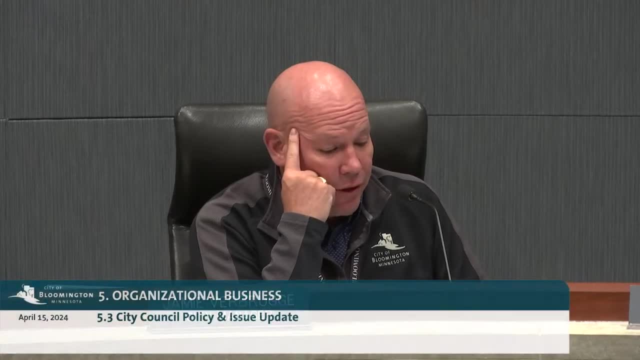 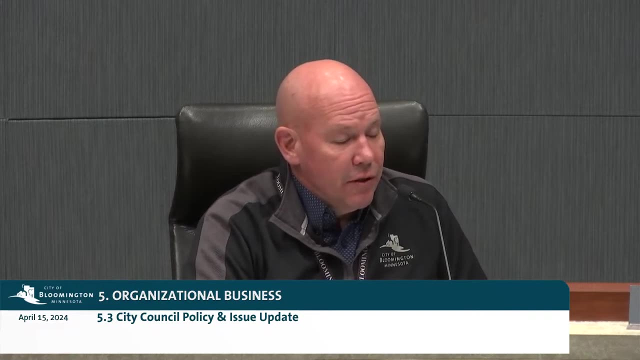 TODAY, COUNCIL WILL RECALL THAT WE WORKED WITH OUR LEGISLATIVE COMMISSIONER, OUR DELEGATION, TO PUT FORWARD LANGUAGE AS A TECHNICAL CORRECTION TO BONDING DOLLARS THAT WERE PROVIDED LAST. 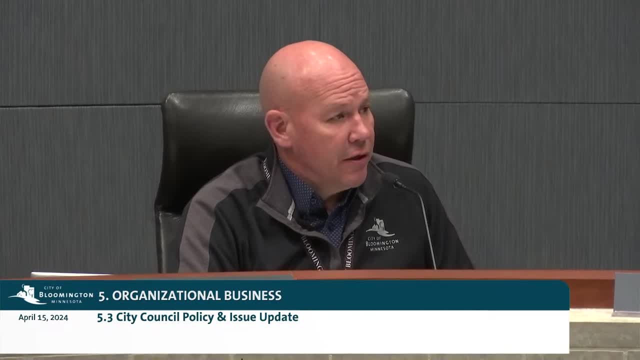 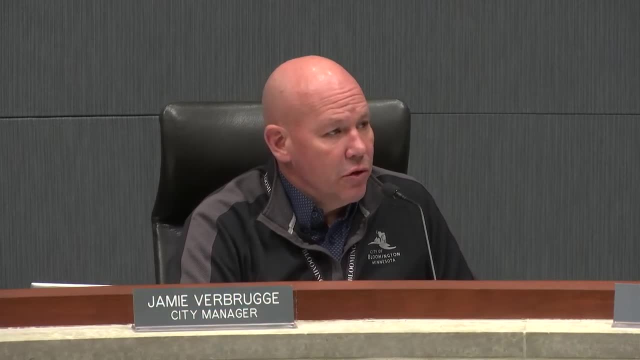 YEAR, WE RECEIVED $1.8 MILLION FOR PRE-PLANNING ACTIVITY OF THE REPLACEMENT OF THE PUBLIC HEALTH BUILDING. THE TECHNICAL CORRECTION THAT WE WERE SEEKING WAS TO INCLUDE THE TWO WORDS TO CONSTRUCT AS. 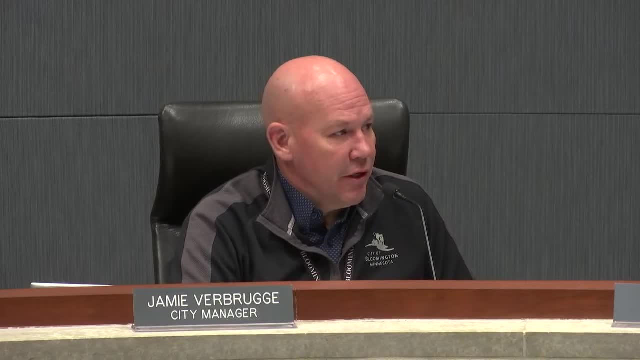 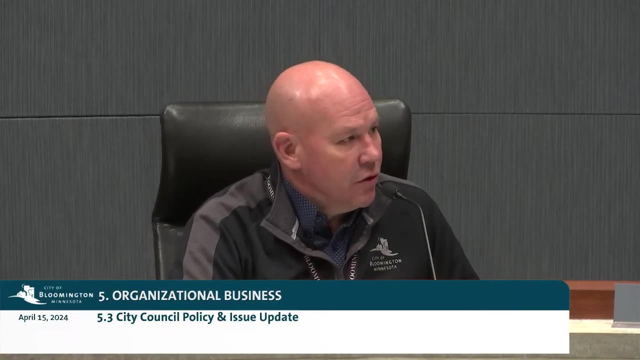 PART OF THE PERMISSION AS PART OF THAT ALLOCATION RATHER THAN JUST THE PRE-PLANNING, SO IT'S PART OF A BUNDLE OF OTHER TECHNICAL AMENDMENTS RELATED TO LAST YEAR'S BONDING BILL THAT WERE PASSED OFF OF THE 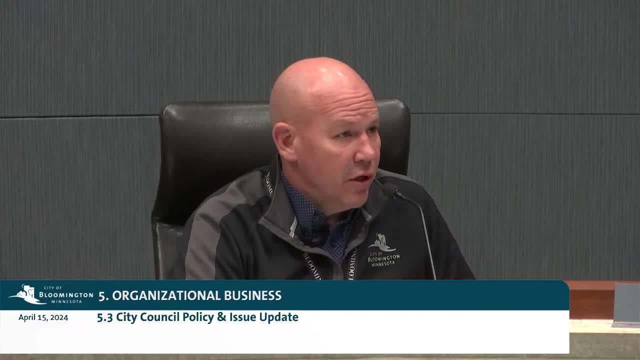 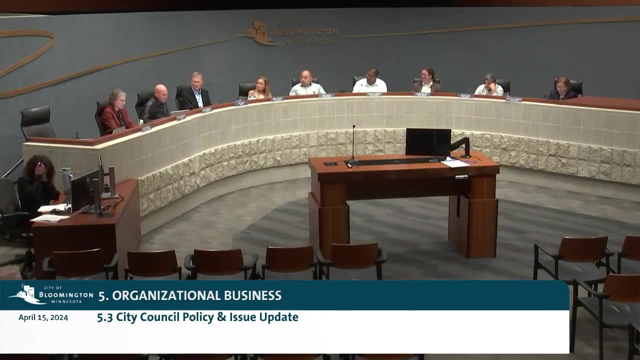 SENATE FLOOR. I BELIEVE THIS WEEKEND AND ON THE WAY TO THE GOVERNOR. SO ONE PIECE OF GOOD NEWS AND WE'LL TAKE IT. THANK YOU, COUNCIL. ANYTHING TO BRING FORWARD. 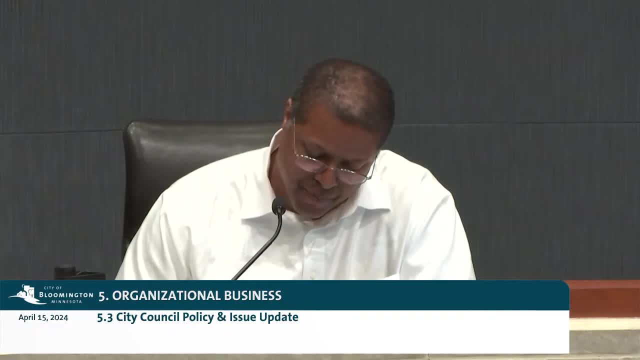 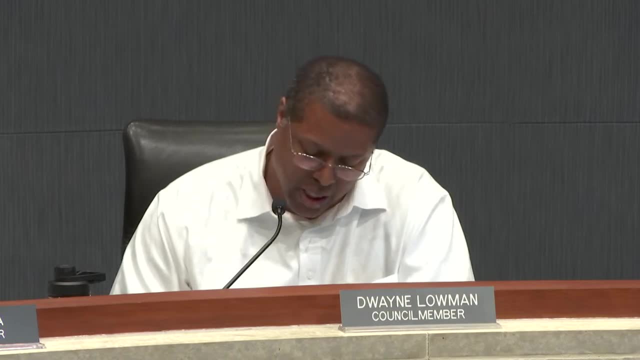 COUNCIL MEMBER LOWMAN. I GOT THREE JUST QUICK THINGS HERE. ONE THING I WANTED TO MENTION JUST MORE AS A COMMENTARY PIECE AS IT RELATES TO THE WATER PARK. I KNOW THAT IN PAST AGREEMENTS. 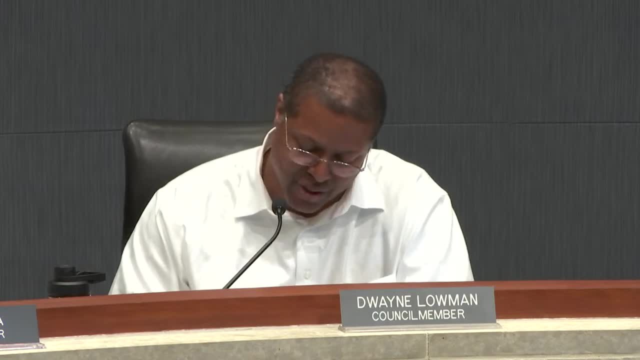 THAT WE'VE TALKED ABOUT WITH THAT WE'VE HAD LABOR PEACE AS IT RELATES TO THE HOTELS, AND I WANTED TO JUST BRING THAT FORWARD JUST AS A REMINDER THAT WE'VE DONE THAT IN THE PAST. 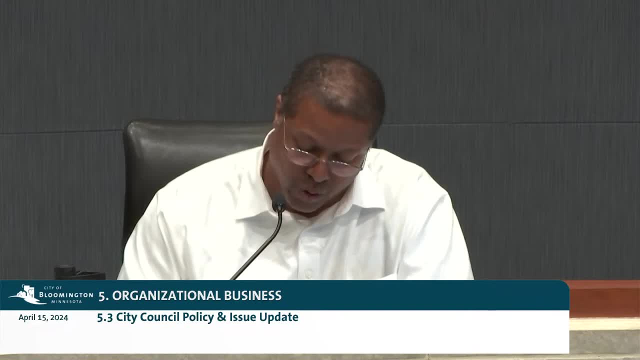 AND I HOPE THAT STAFF IS KEEPING THAT IN MIND AS WE WORK TO CONCLUSION AROUND THE WATER PARK PIECE AND THE ONLY OTHER QUESTION THAT I HAD, AND I KNOW THAT THERE'S BEEN NEGOTIATIONS THAT HAVE HAPPENED WITH KIND OF A. 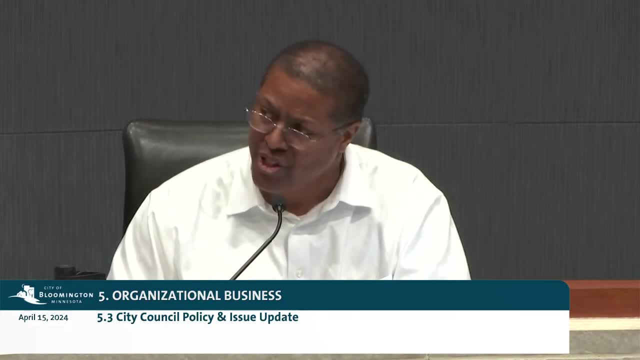 MORE CONCENTRATED GROUP BUT I WANTED TO MAKE SURE THAT WE HAD A LITTLE BIT MORE INFORMATION AROUND THOSE TERM SHEETS AND THAT TYPE OF THING, AND I'M JUST CURIOUS A LITTLE BIT ABOUT A COUPLE OF ELEMENTS. 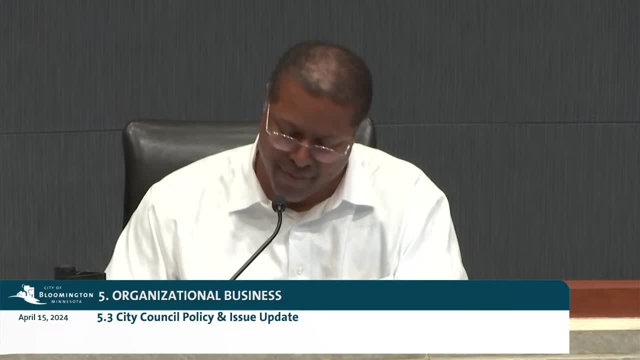 THAT MAY HAVE CHANGED FROM THE LAST TIME WE MADE THE AGREEMENT. I KNOW WE TALKED ABOUT HAVING A. WE JUST HAD A SPECIAL MEETING OF THE SUSTAINABILITY COMMISSION AND ONE OF THE THINGS THAT CAME- 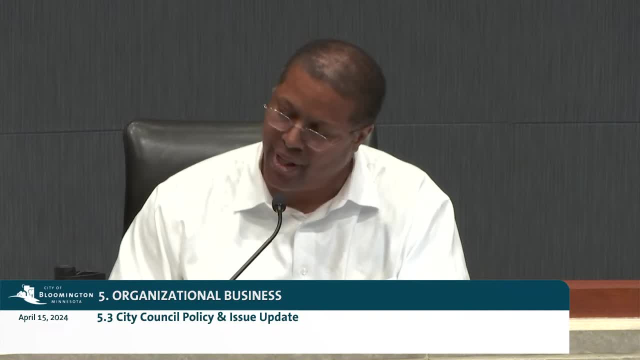 FORWARD WAS A REDUCTION OF. WE USED TO HAVE $5 MILLION KIND OF EARMARKED IN THAT DEAL, AND WHAT I'M UNDERSTANDING IS THAT HAS TO DO WITH THE SIZE OF THE PROJECT BEING REDUCED FROM FROM THE FIVE DOWN TO THREE. 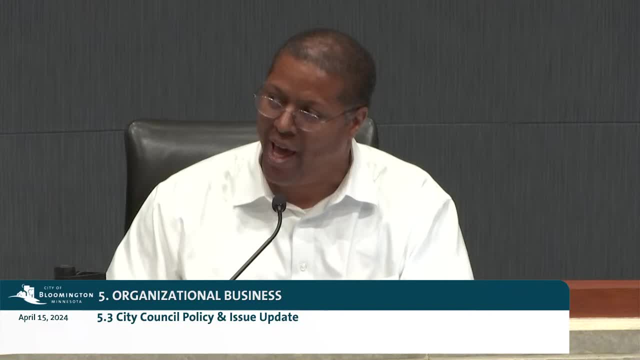 POINT FIVE MILLION, AND I KNOW THAT THERE'S. YOU KNOW, WE DON'T WANT TO HAVE EVERY, EVERY COUNCILMEMBER AND EVERY COMMISSIONER NEGOTIATING, BUT I DID WANT TO, WANT TO ASK ABOUT, ABOUT THAT, JUST SO THAT. 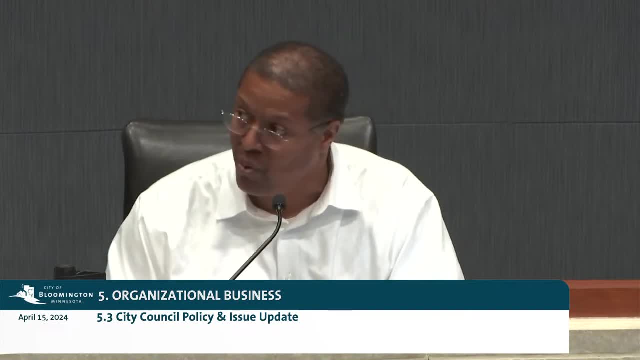 WE'RE ALL KIND OF CLEAR ABOUT THAT AND THE STAFF WANTED TO GIVE ANY MORE CLARIFICATION, OR MAYOR, IF YOU WANTED TO GET SOME CLARIFICATION ON THAT, I THINK THE ONLY CLARIFICATION IT WAS. IT WAS A PROPORTIONAL REDUCTION TO THE. 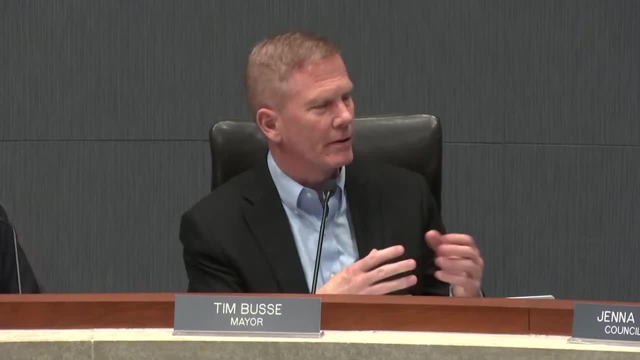 OVERALL COST OF THE OF THE PROJECT AS WELL. SO IT WAS FIVE MILLION, BASED ON THE PREVIOUS COST AS IT CAME DOWN X PERCENT. I CAN'T EVEN RECALL WHAT IT HAS COME DOWN FOR A TOTAL COST. 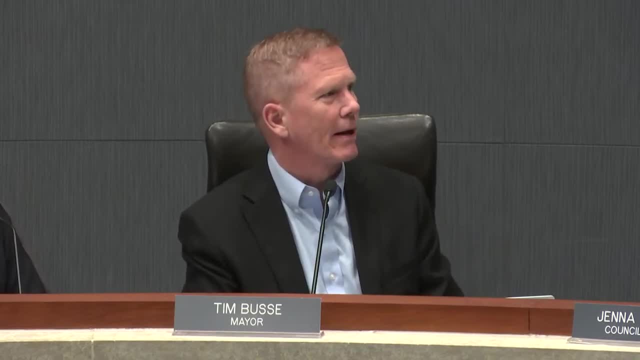 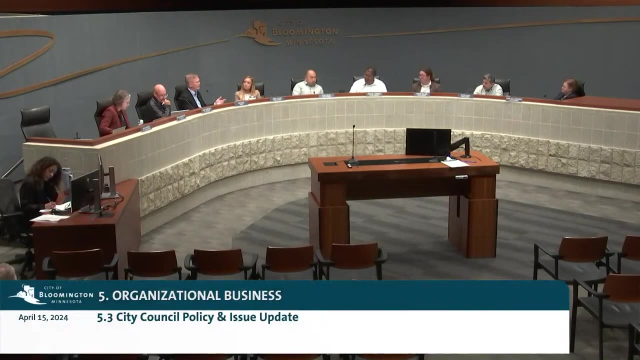 THE REDUCTION IN THE, THE SUSTAINABILITY PIECE CAME DOWN BY THE SAME PERCENTAGE. THAT'S, I THINK, THE, THAT'S, I THINK, THAT, THE, THE, THE EXPLANATION FOR IT: YEAH, THIRTY PERCENT. 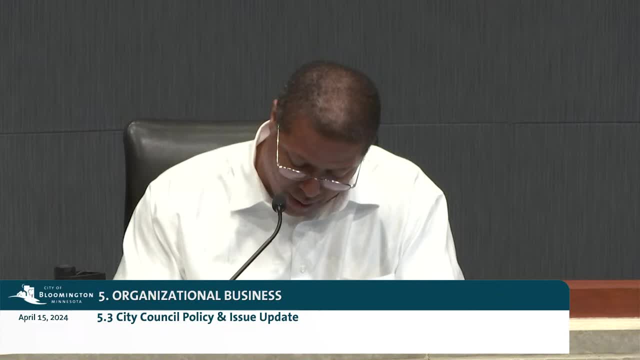 SO IT'S GOOD. SO THEN MOVING ON BEYOND THE WATER PARK PIECE IS. I HAD THE OPPORTUNITY LAST FRIDAY TO DO A COUPLE OF OTHER ITEMS TOO. I GOT A CHANCE TO VISIT WITH THE THE GREEN CLUB FOR. 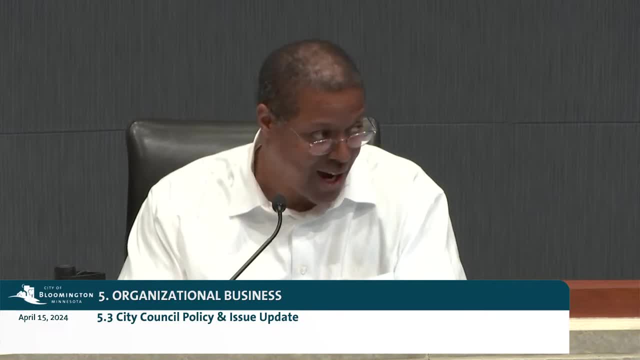 KENNEDY HIGH SCHOOL, THEY NOW HAVE A CLUB THAT'S COMPARABLE TO THE JEFFERSON CLUB, SO I KNOW THEY'RE GOING TO BE LOOKING FOR AT SOME POINT, TRYING TO GET ON, GET ONTO THE SUSTAINABILITY COMMISSION. 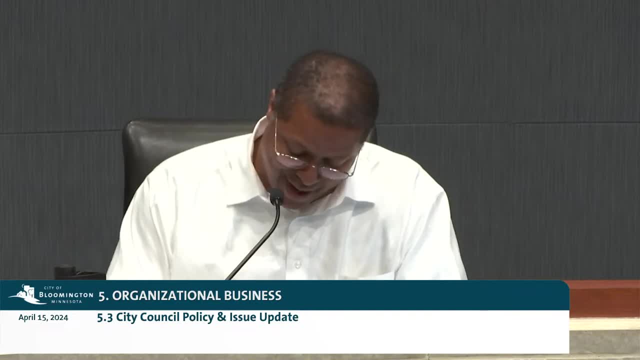 WHICH MAY CREATE A PROBLEM FOR US, BECAUSE WE HAVE A NORMANDALE REPRESENTATIVE AND WE HAVE A JEFFERSON REPRESENTATIVE, SO THAT MAY BE, SOMETHING MAY BE COMING DOWN THE PIKE AT SOME POINT. WE MAY NEED TO KIND OF DECIDE ABOUT. 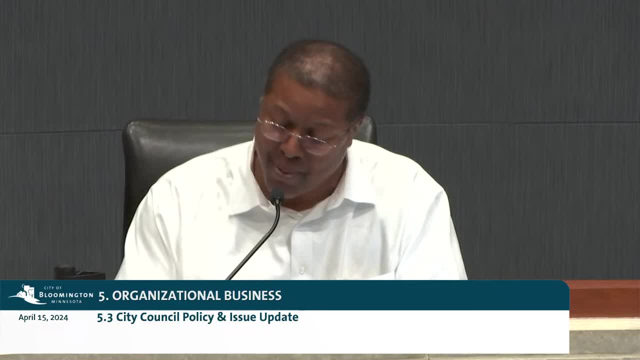 THAT AND THEN I ALSO HAD THE OPPORTUNITY, ALONG WITH THE CITY MANAGER, TO ATTEND THE LEAD PRESENTATION THAT THE MALL OF AMERICA AND A NUMBER OF OTHER STAFF HAD GONE TO, AND THAT, I HAVE TO SAY, WAS PRETTY. 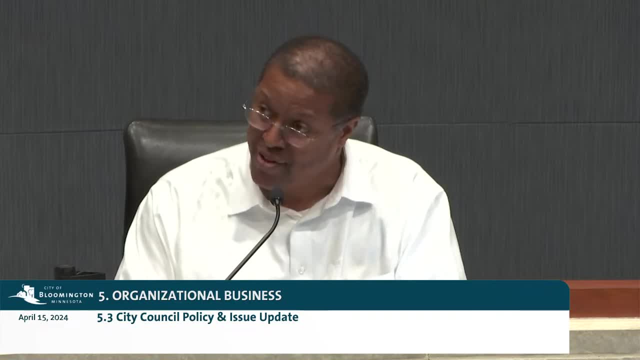 IMPRESSIVE TO SEE WHAT'S POSSIBLE, AND TWO OF THE IDEAS THAT THEY BROUGHT FORWARD WAS THE IDEA OF BECOMING A LEAD CERTIFIED, EITHER A POCKET OF THE CITY OR THE ENTIRE CITY. THAT WE WOULD YOU KNOW MIGHT. 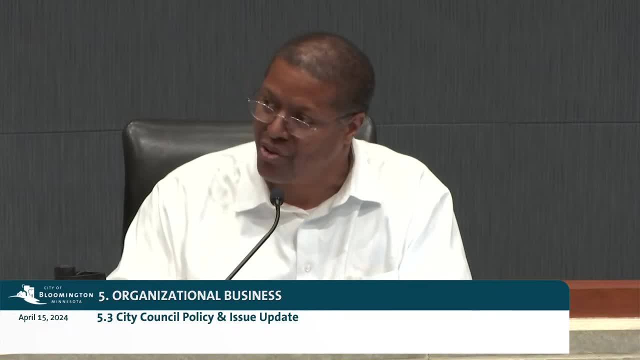 HAVE THE POSSIBILITY OF TAKING THAT ON. I IMAGINE THAT THERE'S GOING TO BE SOME COST ASSOCIATED WITH THAT. NOTHING COMES FOR FREE, AND THEN ALSO THE SECONDARY PIECE WHICH IS WITH WHAT THE MALL WITH THAT WATER PARK. 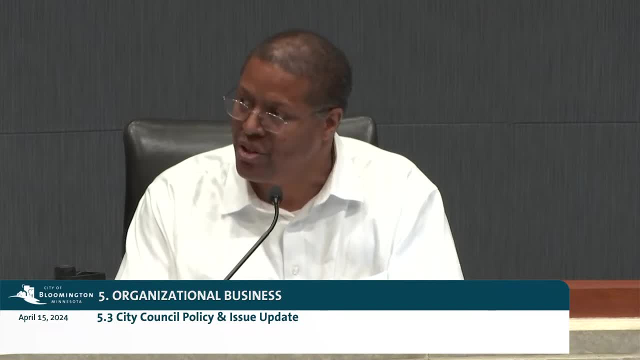 LOOKING TO TRY TO DO THAT AND I KNOW THERE'S PROBABLY SOME PLANS THAT THEY HAD DISCUSSED ABOUT- MAYBE HAVING FURTHER CONVERSATION ABOUT THAT, BUT I DO THINK THAT JUST FROM THIS COUNCIL MEMBER'S 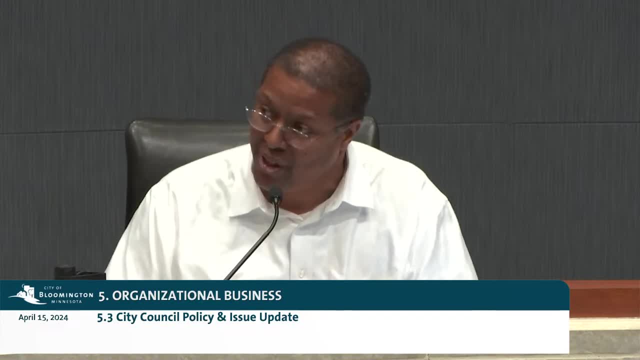 PERSPECTIVE. I DO THINK THAT THAT WOULD BE A GREAT PRESENTATION TO KIND OF IF IT COULD BE HONED DOWN, BECAUSE I THINK THERE'S A HUNDRED AND FIFTY SLIDES. THEY DIDN'T GO THROUGH ALL OF. 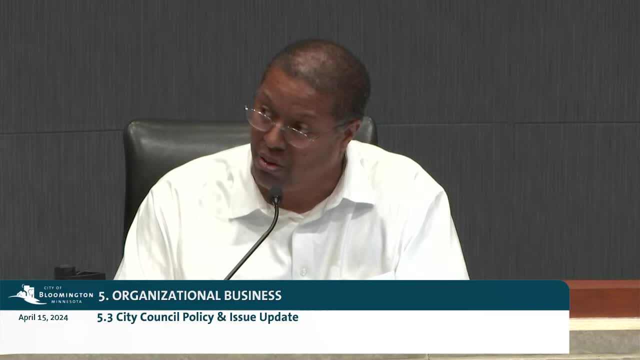 THEM, BUT IT WAS A HALF HOUR PRESENTATION. I THOUGHT IT MIGHT BE SOMETHING. WE MAY WANT TO YOU KNOW IF THE ENTIRE COUNCIL SOME SLIMMED DOWN VERSION OF THAT WHEN IT'S APPROPRIATE TO. 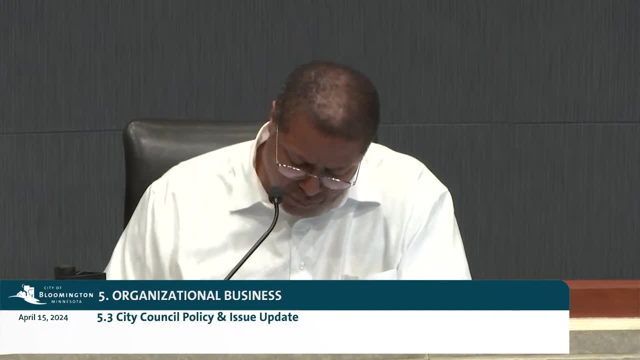 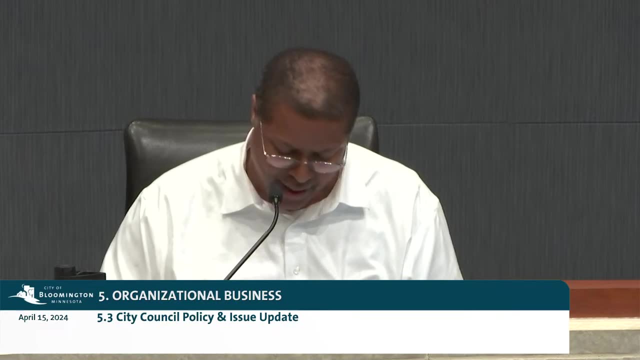 MAYBE LOOK AT THAT IDEA AND THEN FINALLY- AND I WANT TO BE CAREFUL HOW I POSITION THIS AND SAY THIS, BECAUSE I DON'T WANT TO USE A PERSON'S NAME OR THAT KIND OF THING, I'M JUST ASKING A QUESTION OF. 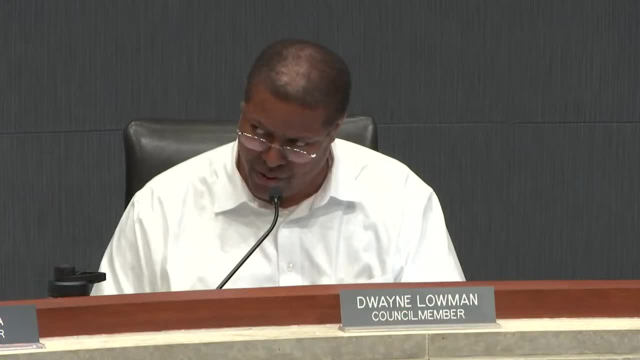 INQUIRY. I KNOW THAT WE GOT A LETTER OF GRIEVANCE, AND WHAT I WANTED TO KNOW IS WHAT IS OUR ROLE AS A COUNCIL IN THAT PROCESS. IF THERE IS ANY ROLE AT ALL, I DON'T WANT TO USE THE PERSON. 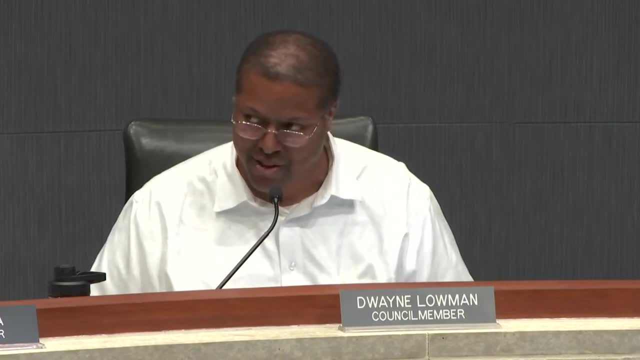 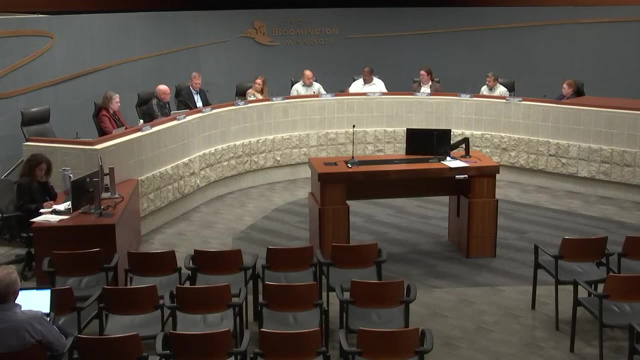 OR WHAT'S GOING ON, BUT IS THERE ANY ROLE THIS COUNCIL HAS IN THAT PROCESS WITH THAT? NORMALLY, I WOULD ASK THIS IN A STUDY SESSION. THAT WOULD BE OFF LINE, BUT WE DON'T HAVE ANY OF THAT. 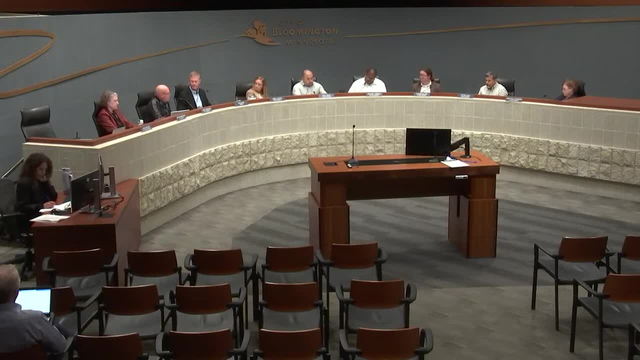 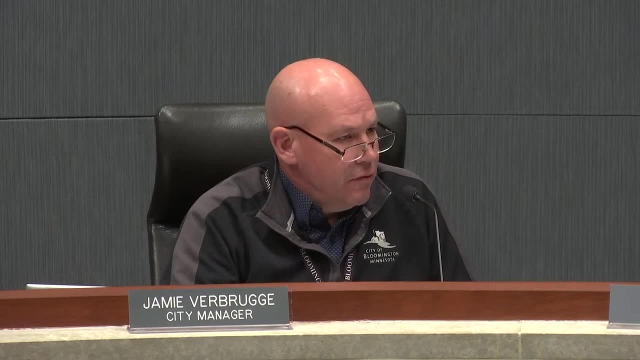 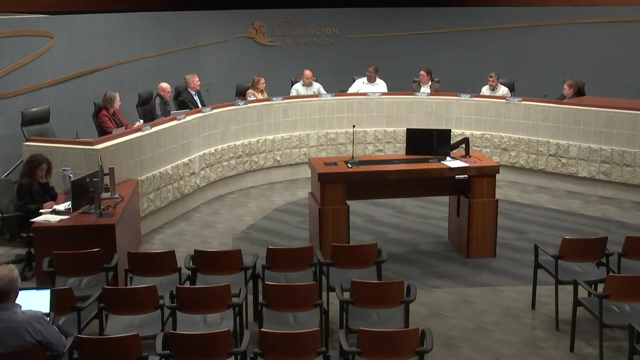 MR MAYOR AND COUNCIL MEMBERS, IF THERE IS A STEP IN THE PROCESS AFTER THE REVIEW THROUGH THE VARIOUS STEPS, IT WOULD BE TO THE MERIT BOARD. THANKS FOR THAT CLARIFICATION. ANYTHING ADDITIONAL? 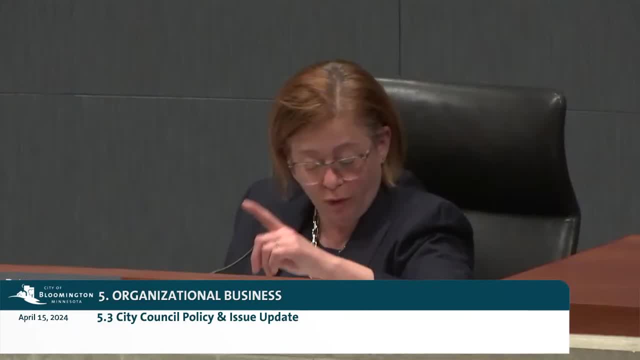 COUNCIL MEMBER D'ALISANDRO, VERY QUICKLY, I PROMISE ONE THING REGARDING THE LEADERSHIP DEVELOPMENT PROGRAM: PRESENTATION: THAT WE SAW TODAY. WE DON'T NECESSARILY, I MEAN. 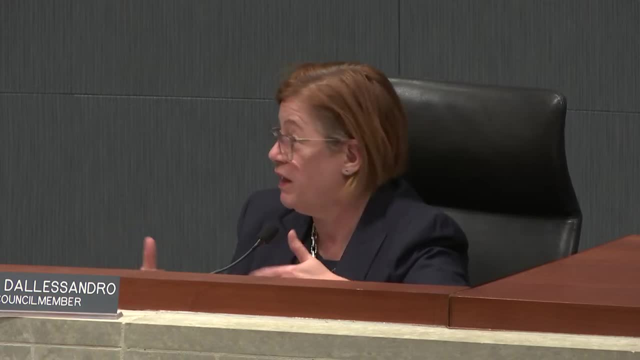 WE'VE GOT THOSE ACTION ITEMS, THE RECOMMENDATIONS, BUT WE DON'T HAVE A PLAN FOR LIKE ACTUALLY MAKING A DECISION ABOUT WHETHER WE'RE GOING TO PURSUE ANY OF THEM. I FEEL LIKE WE OWE IT TO THEM TO. 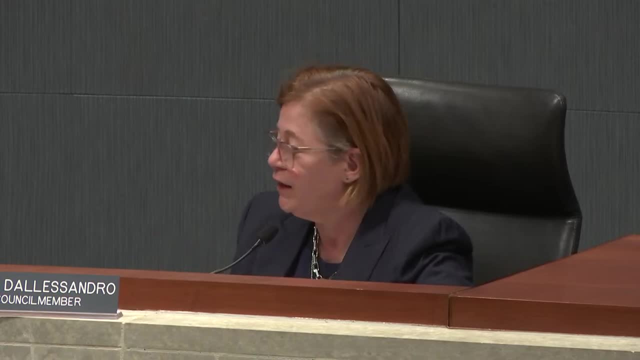 LIKE, SAY, OKAY, YOU PRESENT IT TO US. WE HAVE FEEDBACK FOR YOU ON THAT AND SO, ESPECIALLY SINCE, ALL OUR WORK PLANS BY THE COMMISSIONS AND STUFF HAVE ALREADY BEEN APPROVED AND NOW WE HAVE THIS. SO THE TIMING OF 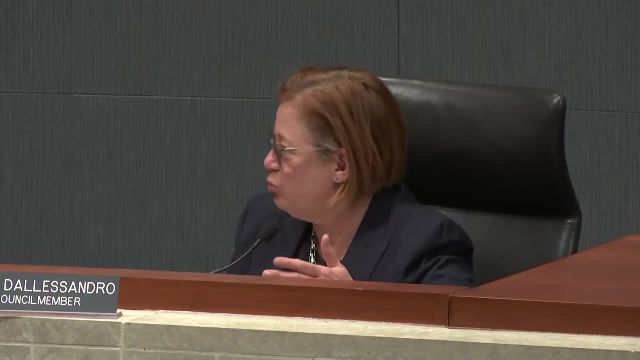 IT IS A LITTLE AWKWARD. I'M JUST CURIOUS, LIKE WHAT IS. WHAT IS THE EXPECTATION THAT THE PROGRAM HAS FOR CITY COUNCIL GETTING BACK TO THEM WITH ACTION ITEMS OR DECISIONS BASED ON THE THINGS THEY? 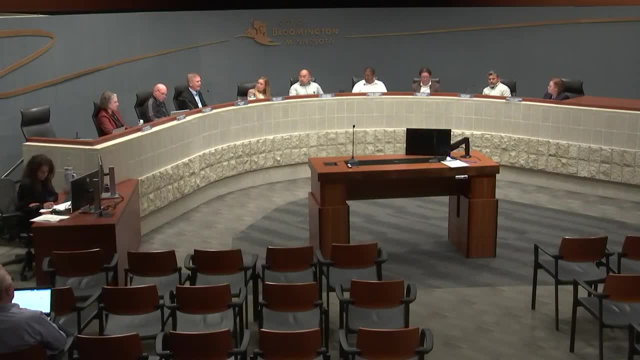 RECOMMENDED. I APPRECIATE THE QUESTION AND I I THINK SOMEBODY MENTIONED EARLIER TONIGHT THE THREE THINGS THEY BROUGHT UP WEREN'T NECESSARILY FAR FLUNG OR FAR FETCHED FROM WHAT A LOT. 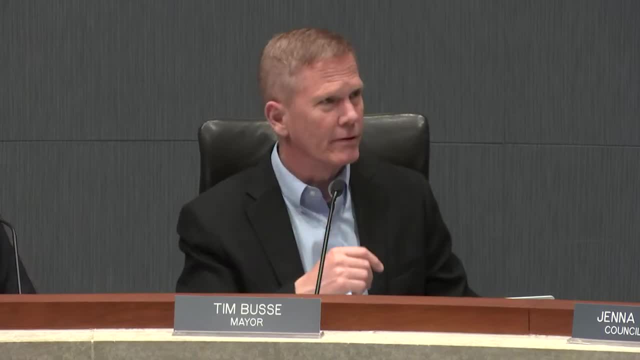 OF THE WORK THAT'S GOING ON RIGHT NOW. PERHAPS, THE TROLLEY PART, PERHAPS MIGHT HAVE BEEN A LITTLE BIT. NOT WHAT WE'RE THINKING, BUT I MEAN TO MAKE THE CITY MORE BIKE ABLE AND MORE WALKABLE AND TO MAKE THE 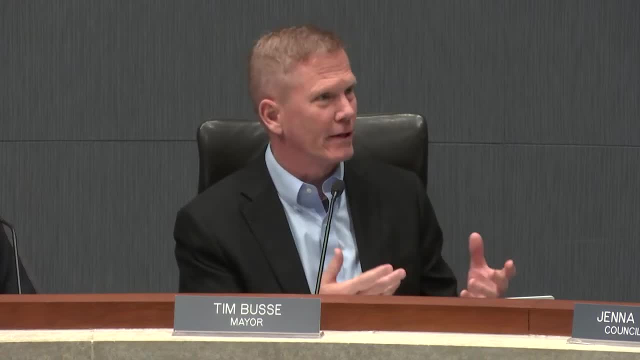 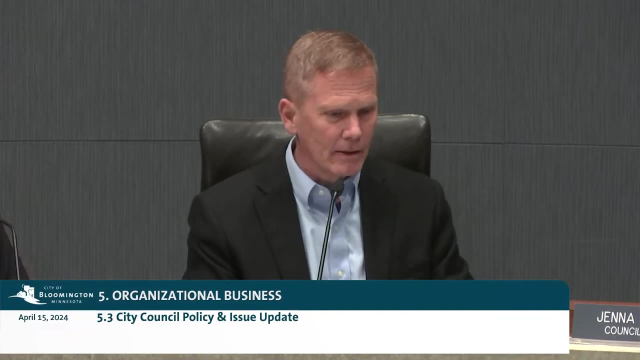 INTERGENERATIONAL THING. I MEAN THAT'S WHAT THE PLAN IS FOR THE COMMUNITY CENTER. I MEAN SO THAT'S THAT WE'RE, AT LEAST, HEADED DOWN THE RIGHT, THE SAME PATH AS WHAT THEY WERE RECOMMENDING. I THINK, THIS BEING THE FIRST. 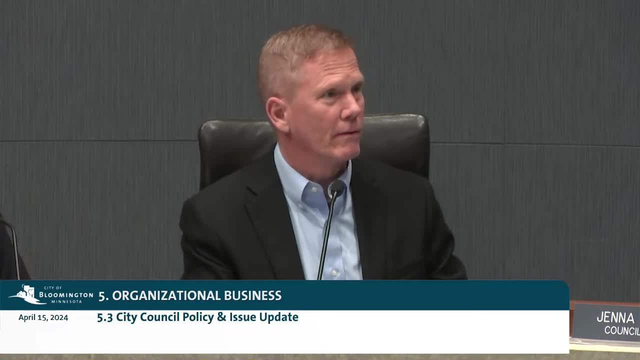 WE'VE HEARD OF IT. I THINK IT'S A MATTER OF HOW WE FIGURE OUT WHAT THE NEXT STEPS MIGHT BE. I MEAN I'LL REMIND YOU THAT THE THE NOTION OF A, A, AN ELECTION, OR PUT IT, PUT IT. 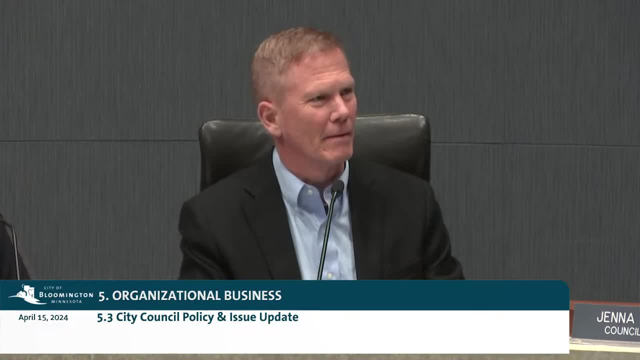 ON THE BALLOT TO CHANGE THE CITY CHARTER TO ALLOW ROOT PUBS IN THE CITY OF BLOOMINGTON WAS SOMETHING THAT CAME FROM A LEADERSHIP PROGRAM AND THERE WAS A RECOMMENDATION THAT CAME FROM THE BLOOMINGTON LEADERS. 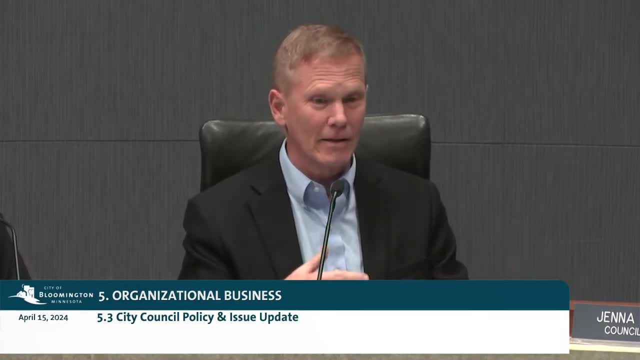 PROGRAM, AND SO IT'S NOT- AND NOW SHE'S ON THE PLANNING COMMISSION. EXACTLY SO I MEAN IT'S, IT'S, IT'S, IT'S, SOMETHING THAT I THINK IT DOESN'T NECESSARILY HAPPEN AT THIS AT. 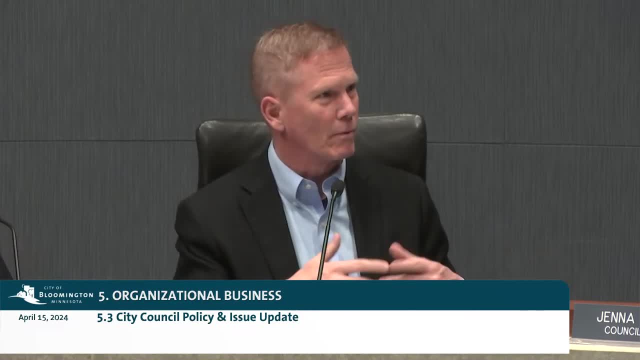 THE SAME MEETING, BUT IT ALSO DOESN'T MEAN IT'S GOING AWAY. I THINK IT WILL PERCOLATE A BIT AND I THINK STAFF WILL TAKE IT, AND I THINK THE INDIVIDUALS MIGHT LOOK AT OPPORTUNITIES FOR HOW THEY CAN. 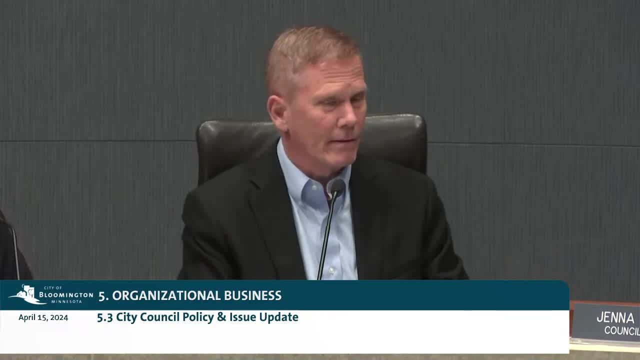 BRING IT FORWARD TO US. BUT I APPRECIATE THE RECOMMENDATIONS AND- AND WE'VE IT'S BEEN PROVEN IN THE PAST- THAT THE RECOMMENDATIONS OF THAT THAT GROUP ARE ACTING ON OKAY. SO TO SUM UP VERY QUICKLY, THERE'S NO. 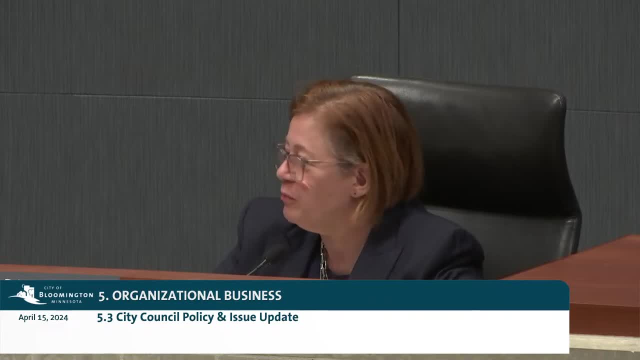 EXPECTATION THAT WE DO ANYTHING WITH IT. MAYBE CITY WILL, MAYBE STAFF WILL, MAYBE THEY WILL, BUT NONE OF US ARE GOING TO BUT THE COUNCIL ITSELF. OKAY, NO, THAT'S JUST, THAT'S FINE. I JUST WANTED TO. 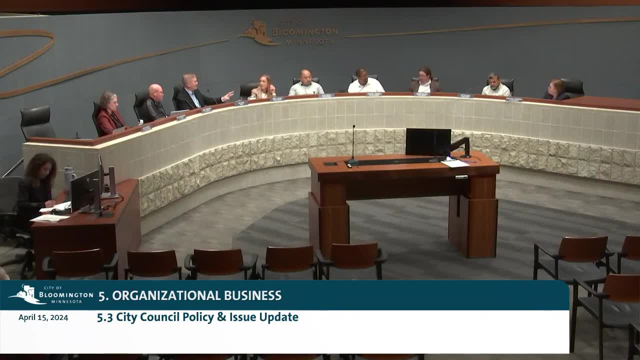 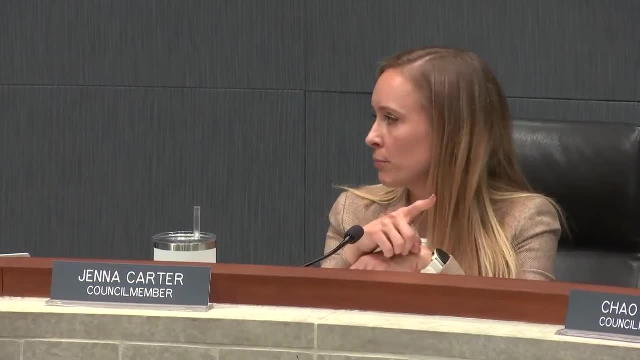 ASK THE QUESTION. GREAT. EXCUSE ME, I DID HAVE ONE MORE THING, BUT DID YOU HAVE A COMMENT ON THAT? YES, GO AHEAD. SO I DON'T RECALL LIKE KIND OF RECOMMENDATIONS COMING FROM PAST COHORTS, LIKE THAT. AND. 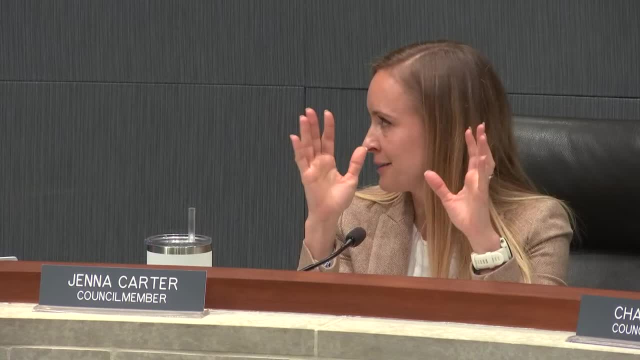 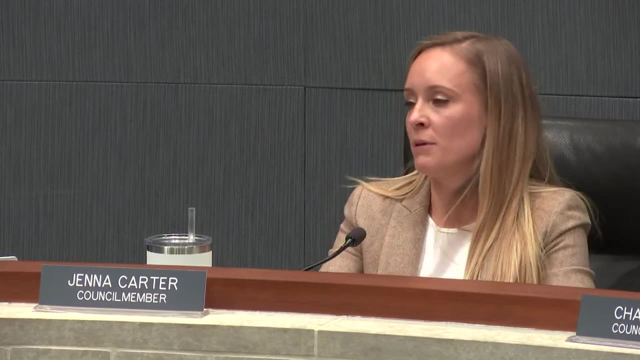 THEY'RE KIND OF SUMMARY OR WRAP-UP, AND MAYBE MY MIND IS JUST. YOU KNOW I MEAN IT'S LATE. THIS WAS A LITTLE NEW THIS YEAR, OKAY, SO I WOULD MY. MY ASSUMPTION WOULD BE THAT YOU. 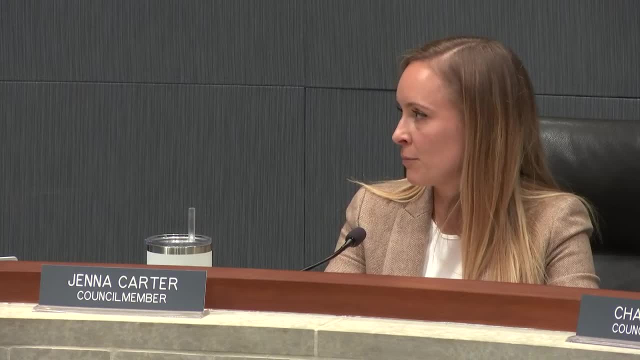 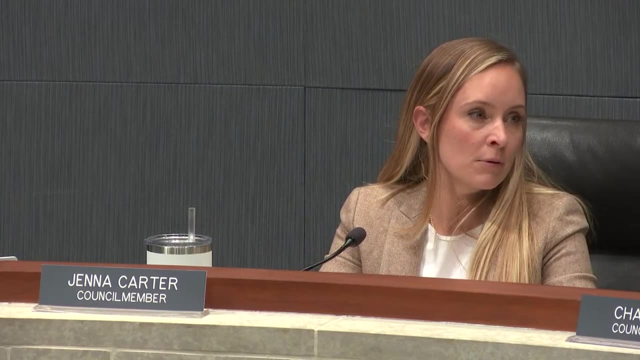 KNOW, IT'S KIND OF AN ACTIVITY AND IT'S A LIKE THERE. IT'S LIKE A CAPSTONE. YEAH, THAT THEY'RE NOT, THAT THERE ISN'T AN EXPECTATION, THAT THEY'RE DELIVERING US PRODUCTS AND PROPOSALS, AND SO THAT'S FINE. I. 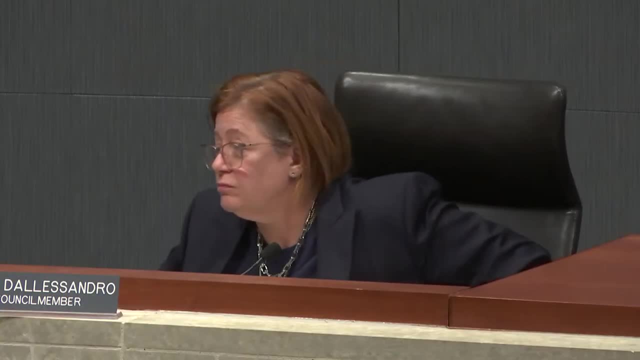 AS LONG AS I MISS, MISS MARIN COUNCIL, I'D SAY THAT DOESN'T PRECLUDE YOU FROM, IF YOU WANT, TO EXPLORE IT AND HAVE STAFF RESEARCH IT. I'M JUST GOING TO SAY WHAT I SAID AT THE 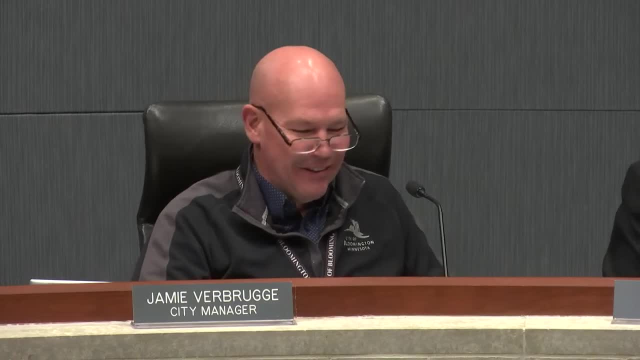 BEGINNING OF THE YEAR, WE HAVE REALLY FULL PLATES, YEAH, RIGHT. AND SO I JUST WANTED TO MAKE SURE, JUST WITH SORT OF THAT COMMON ADMONITION, YEAH, THE EXPECTATION ON THEIR PART ISN'T THAT SOMETHING IS GOING? 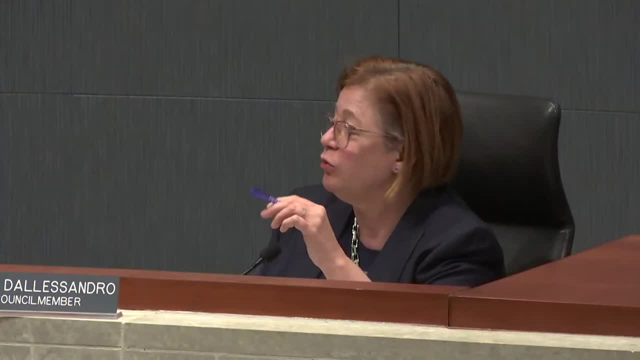 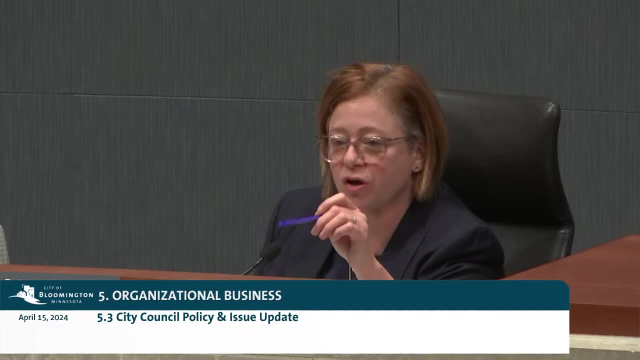 TO BE DONE. SO IF THAT'S, IF THAT'S THE CASE, GREAT, I JUST DIDN'T WANT TO BE MISALIGNED. AND THEY WALKED OUT OF HERE WITH THEIR EXPECTATIONS AND WE DIDN'T DELIVER SECOND THING I'D LOVE TO SINCE. WE SAW THEM. 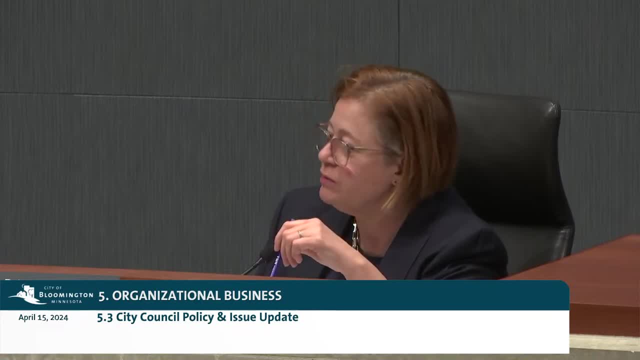 IN THE PLANS CAN WE GET A BALANCE SHEET ON TREES? SO I DON'T KNOW IF THIS- I THIS DOESN'T FEEL LIKE PART OF THE FORESTRY MASTER PLAN THAT WE APPROVED TODAY TO FUND, BECAUSE I FEEL LIKE THIS IS. 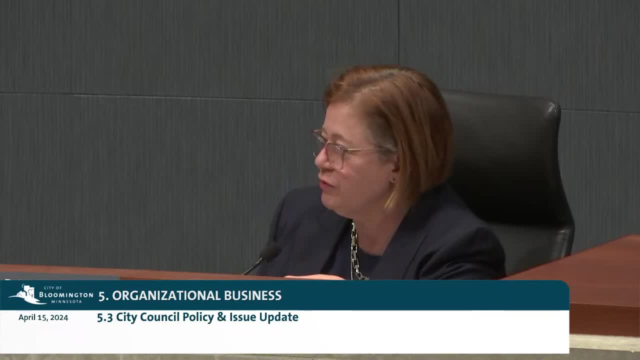 INFORMATION WE SHOULD ALREADY HAVE. WHICH IS WHICH IS. HOW MANY TREES HAVE WE TAKEN DOWN, HOW MANY TREES HAVE WE PLANTED AND HOW MANY MORE ARE WE GOING TO PLANT THIS YEAR? I WOULD LOVE TO JUST GET THAT DATA, BECAUSE I 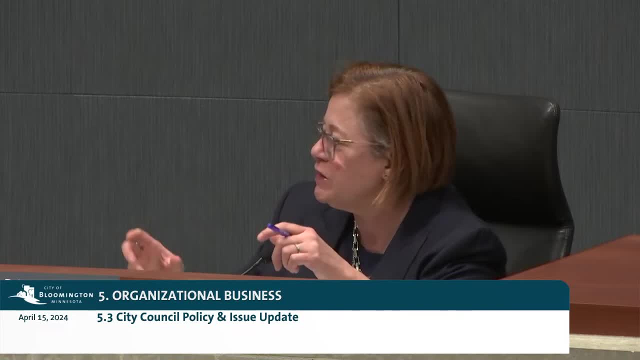 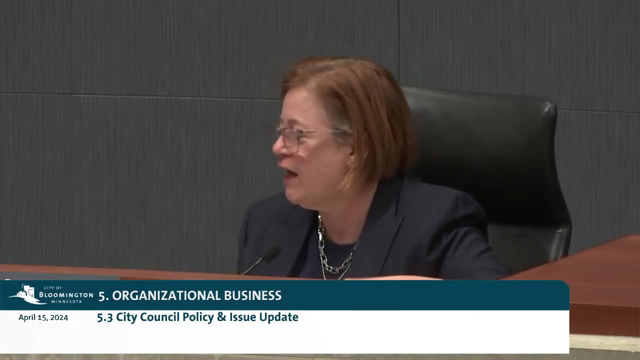 FEEL LIKE WE KEEP GETTING THE DATA ON TREES IN LIKE LITTLE PARCELS. LIKE BRYANT'S GOING TO GET 200 MAYBE- I DON'T KNOW WHAT THE NUMBER WAS- TRETBAW'S GOING TO GET 58 MAYBE.